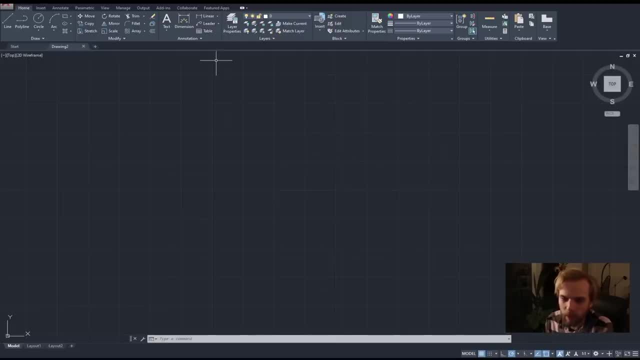 This kind of user interface And you can't really see the top top of the row. but there's basically nothing there that's super important, It's just a bunch of different icons. If you click on the large icon in the top left corner, the large A button- you 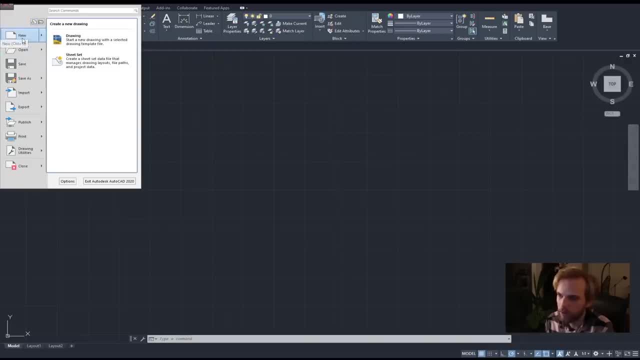 see all of the same tools that are available for you: Create a new file, open an existing one, save files, export files, publish files or print files, I guess Right. So printing is oh, actually, I'll talk about it once we get there right, But the basic menu is here. 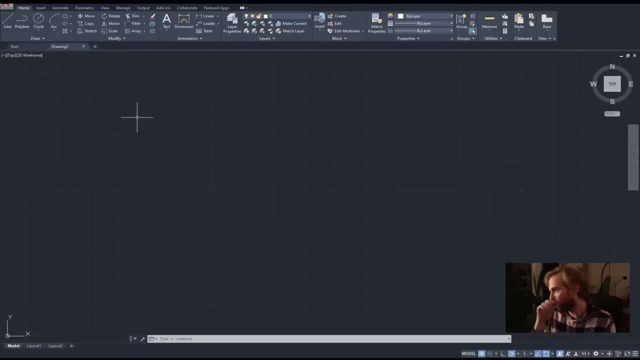 right. It's located underneath that large A button. Underneath it you have what's called the ribbon menu, And this is the ribbon menu has a bunch of tabs, So it's like categories with the tools that you can use. But, honestly, the faster you learn, 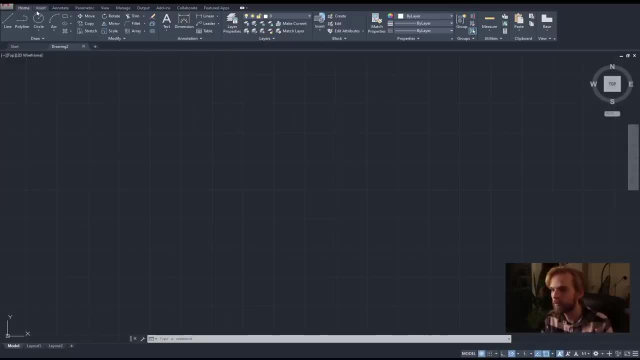 the commands for the tools rather than clicking on the icons of the tools, the better. it is right, Because it just speeds up your drawing process quite a bit once you actually remember the shortcuts or the commands for the tools. So, honestly, I almost never use the icons anymore. I. 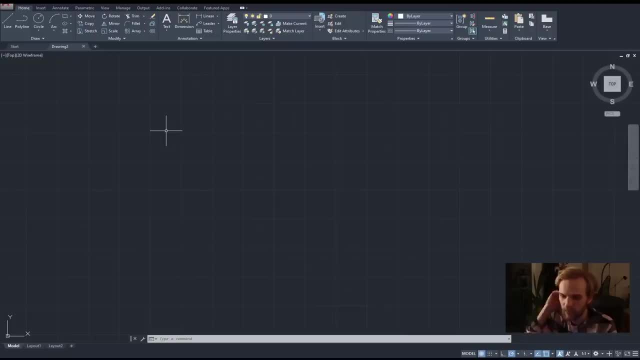 just type in the commands, and anyone that you ask who is using AutoCAD does the same. Nevertheless, we will be kind of clicking on these and looking where they are, but also we will be memorizing the shortcuts for them as well. There is this: 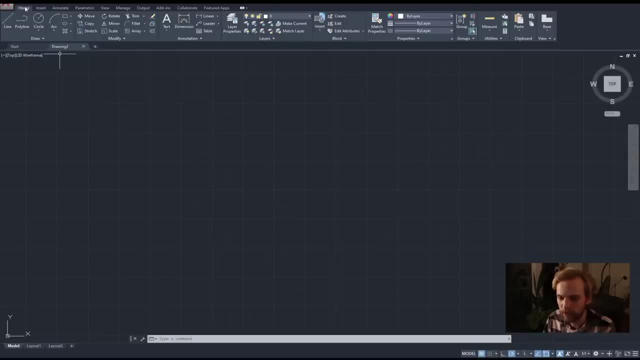 home tab. So the home tab is going to be 99% of the time we are going to be spending in the home tab. Then we have the insert tab. From time to time we will go in here and use one or two tools from. 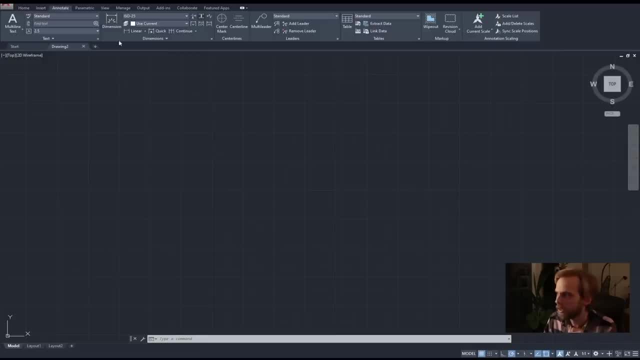 here. There's not much here. Then we have the annotate tab, where, yeah, we will be spending good time here as well. Every other tab is: we ignore it, It doesn't exist to us, We don't care, right. So it's only these three tabs. By now. you might be wondering. well, that you probably have. 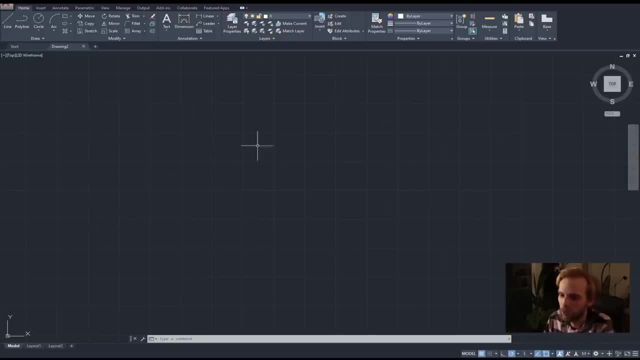 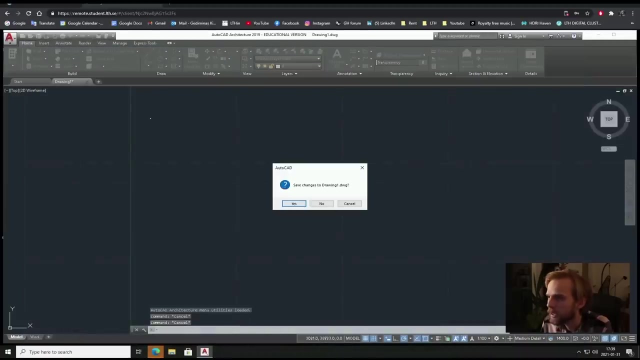 you know more stuff here, right? More floating windows here. That might happen because you either have AutoCAD architecture rather than just regular AutoCAD, or maybe these days AutoCAD just ships with multiple open panels. Actually, can I show you, Let's see, if I close that, No, Start drawing. 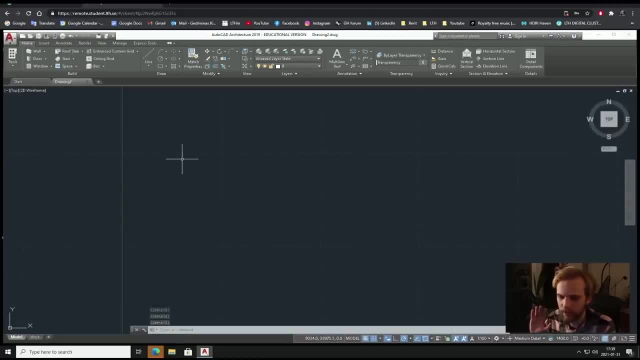 Hmm, It doesn't open up any panels here. but if you have any panels opened up that are just floating on the screen, close them, Click the X buttons and then just close them. You don't need to see them right, Just clean up the screen. One more thing is right now what you see here on the screen. 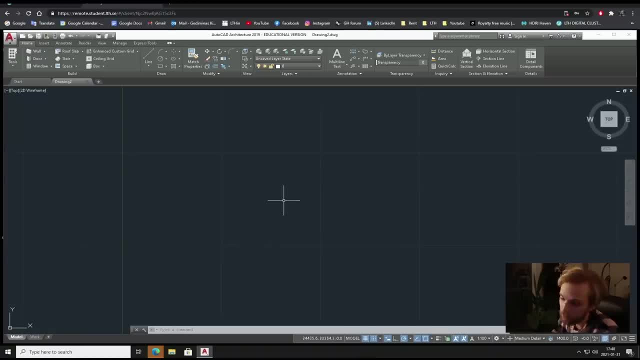 is me logged into a school's computer right? So on the school's computers, for instance, we are running AutoCAD architecture 2019. And it has the home tab, has these three-dimensional tools of wall door and so on, And also it does have the two-dimensional tools. We will not be. 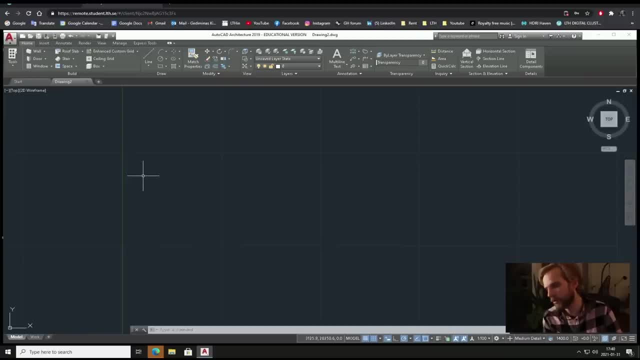 using three-dimensional tools in this course at all, because, first of all, AutoCAD is not that great for three-dimensional modeling compared to competitors. Second of all, it's better to first learn how to draw and then learn how to model, rather than kind of trying to learn everything. 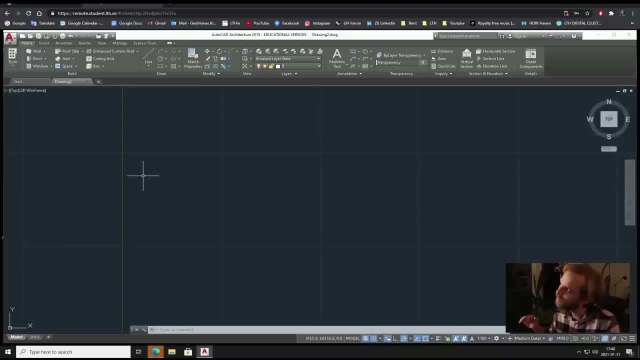 all at once. It's much easier learning curve that way. So we will be only using 2D drawings. There's one more thing that I want to check And I will be checking. I will check if there's a possibility on how to hide this. 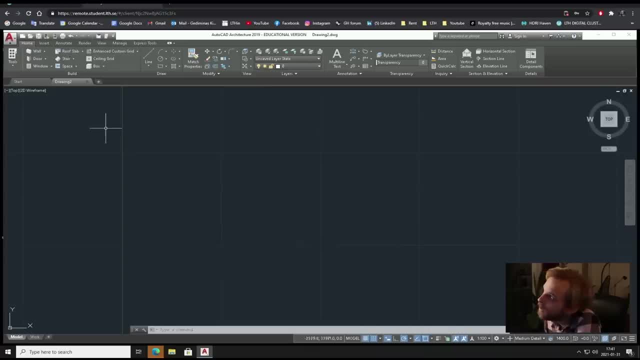 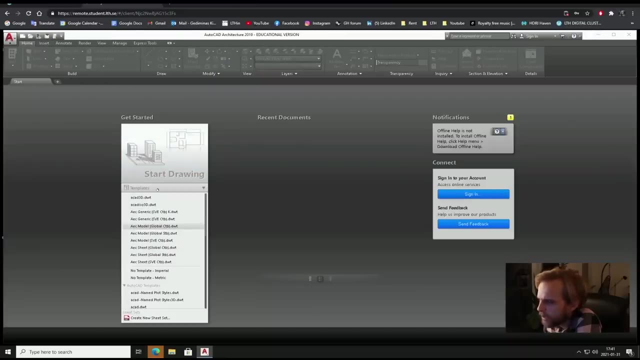 And that the way you hide this is if you use a different profile, a different viewing template, And I'll. I'll just try. Let me close this, Let me try to open it again, But this time around, what if we use no template? metric? 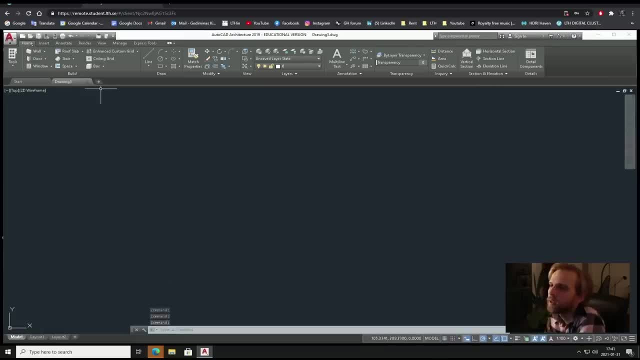 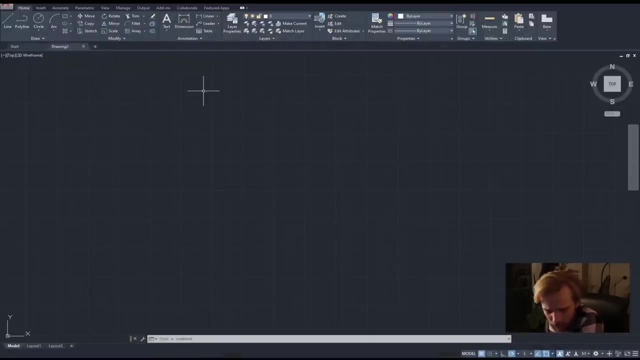 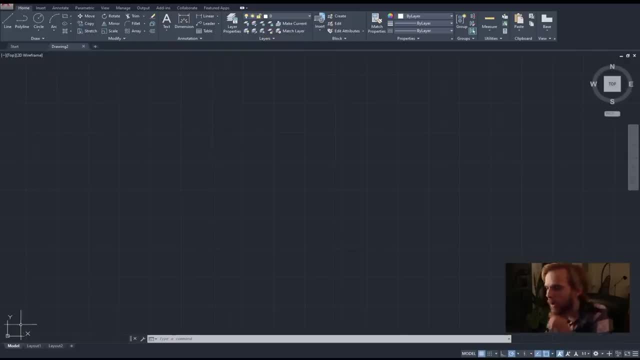 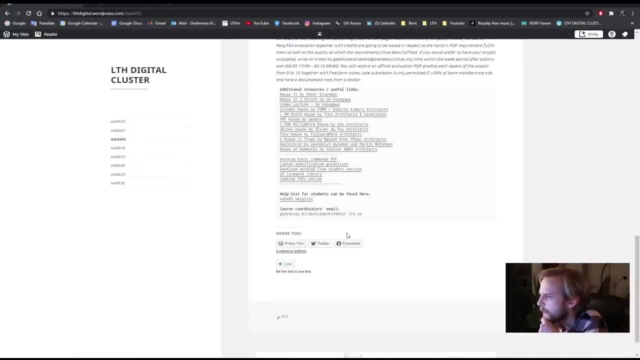 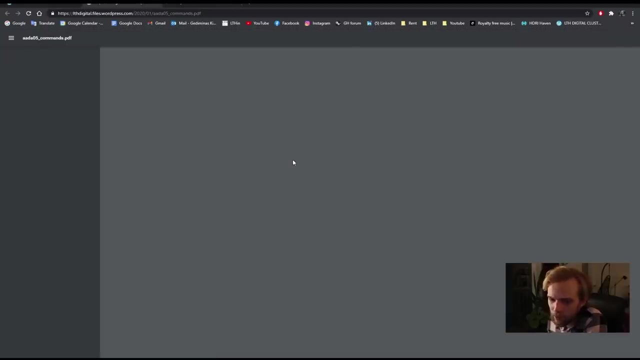 everyone sees, you know where different tools are located. One more thing is the course website. If we go to the course website, it does have AutoCAD basic commands PDF right here which I will open and actually I'll be using it too. And this is not a lot of. 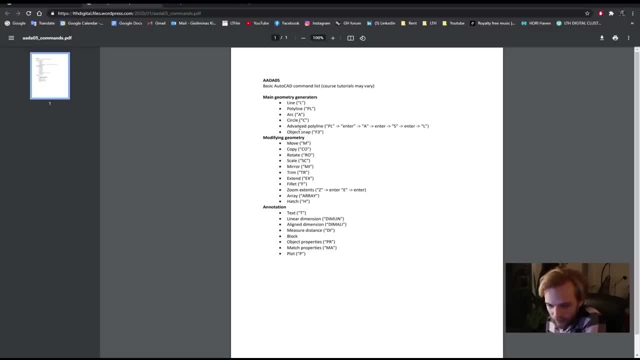 tools. but I will be using it to go through these tools and kind of explain to you what they do before we actually begin- well, most of them before we begin actually going deep into drawing a building. i will be showing how to do that as well, but first let's just kind of look. 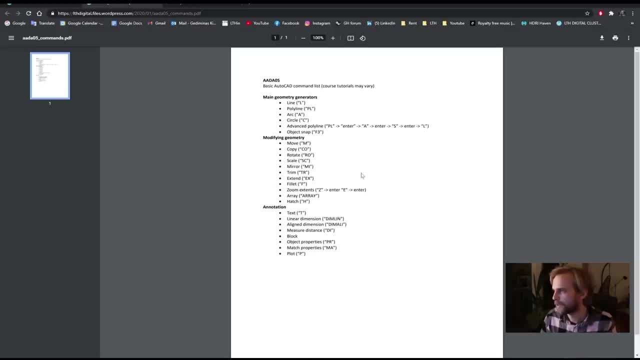 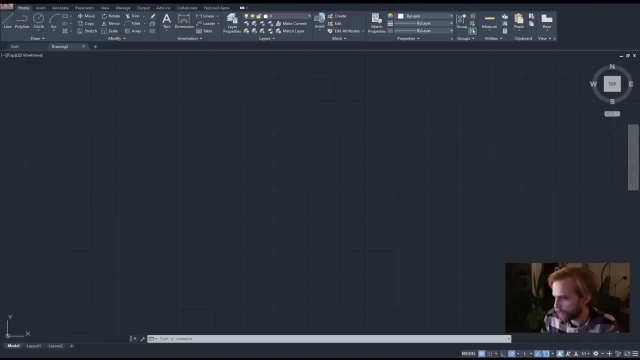 at the tools. um, so have that opened as well. just ready for you, right? so let's jump into autocad, back into autocad, and here there's this grid that you see. here is your main viewport, right, and it's basically a two-dimensional view. you can make it three-dimensional with this box here. 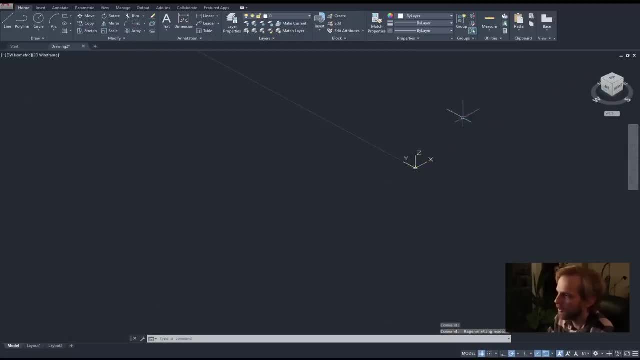 by clicking on the on the side of the box, and now it's. it's a three-dimensional space, three-dimensional grid. but you don't want to do that. so what you do is you just click on the top of the box, like so, and it's going to. 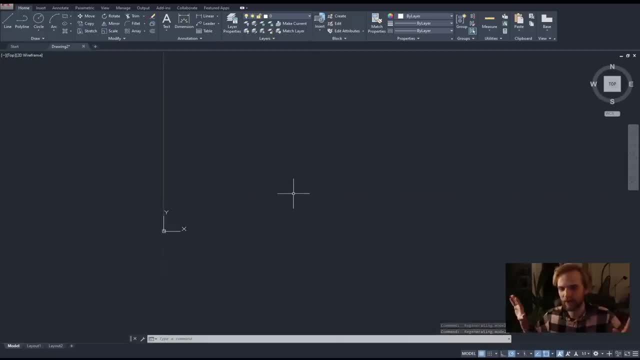 rotate back to two dimensions. we are going to draw it in everything in two dimensions, flat right. if your top, the name top, is not oriented properly, let's see. if it's like so, if it's rotated like so, just use these arrows to kind of rotate it back to to normal. so this is what. 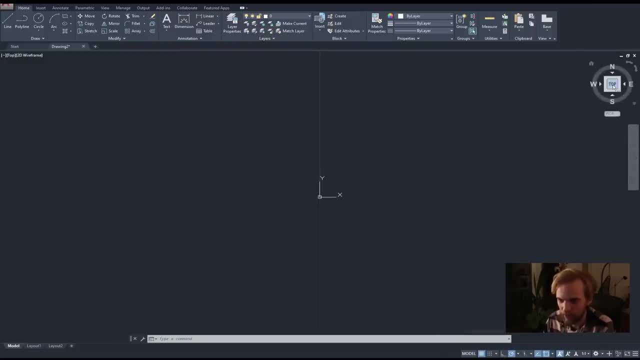 you want to see north, south, east, west, top right. okay, the way you move inside of this view is: there's no, uh, there's no right click and holding right. instead, if you click and hold the scroll scroll wheel of the mouse, you can pan the view right, like that. if you scroll the wheel, of course you zoom out, zoom in, zoom out, zoom in. 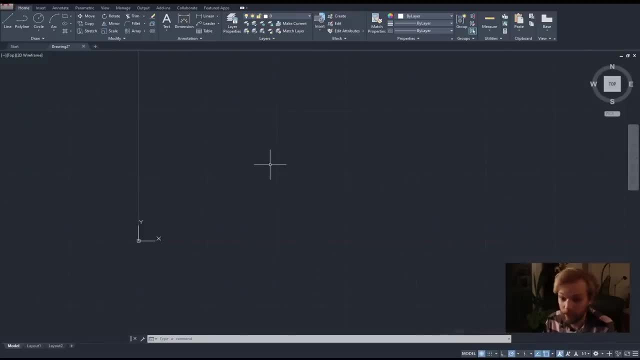 right into the view and and that's it. that's all you need. honestly, you know, you just need to be able to pan the view and zoom into to the cursor. by the way, it always zooms into where you have your your cursor. that's important um selecting objects. it's the is done through. 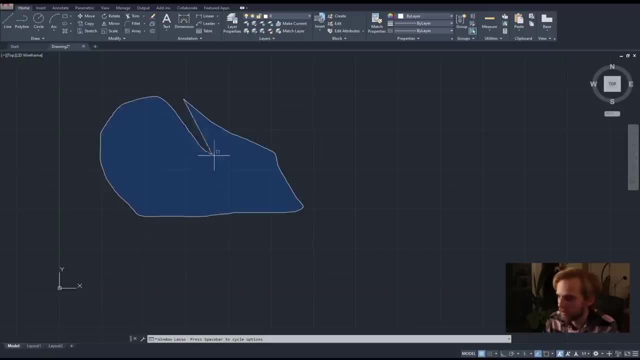 by clicking and dragging the mouse. and by now you will notice that if you click and drag the mouse, um, with the left mouse button, it kind of does this. so this is what's called like a smart selection. i absolutely hate it. i or lasso tool, lasso selection tool method. i absolutely hate it. 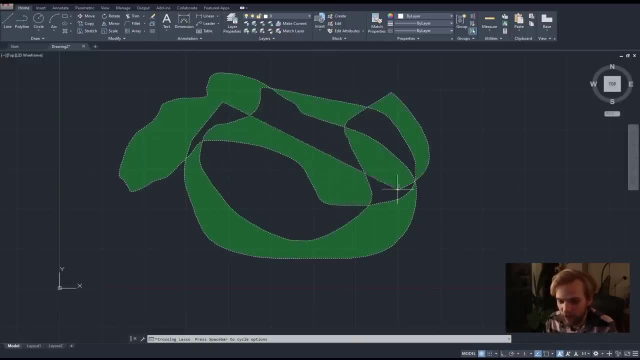 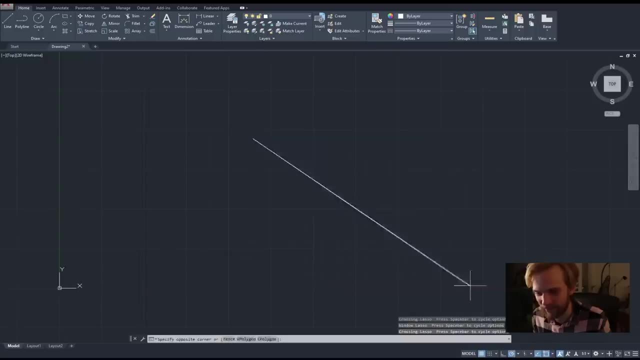 i think it's obnoxious. uh, so the first thing that we will actually do is we will get rid of it. right? so let's get rid of that. i just want it to be like a rectangular marking, but it doesn't let me um to get rid of it. 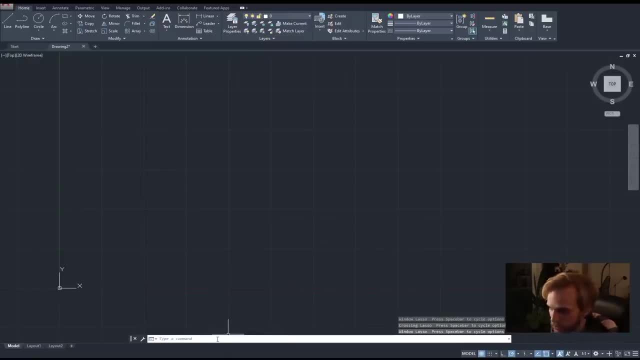 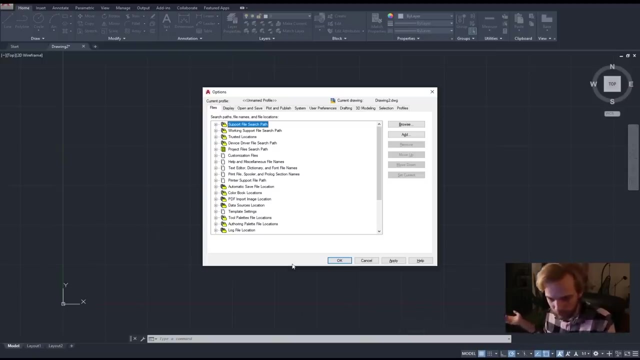 here in the bottom you have the command line. this is where you write all of the commands, right, um? and i can just write options and hit enter. right, so i wrote options, i hit enter and it opens up options for me, options, um, and then in the options, options tab or options menu, i can go to actually 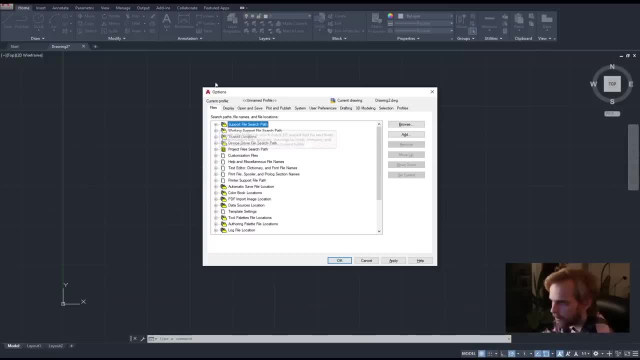 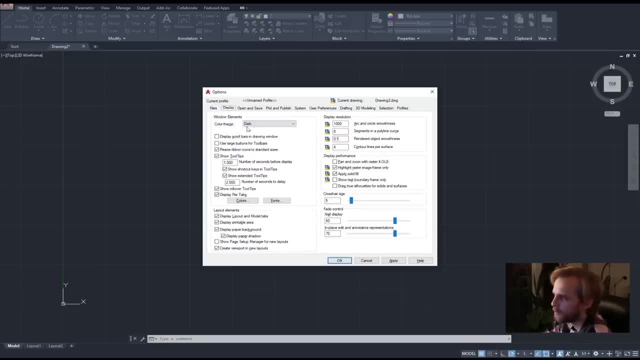 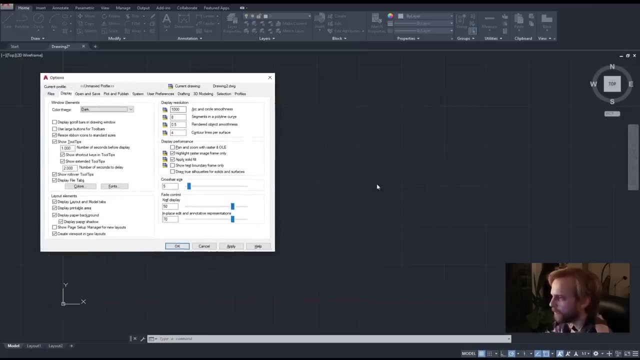 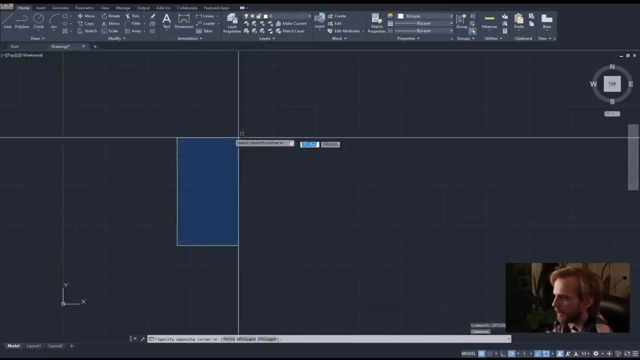 supporting files are located. you don't care about this display is. you can change the color theme between dark and light, whatever crosshair size. um, let me show you. i'll increase the crosshair size to 100 hit, apply, hit, ok, and now my my crosshair looks like this: this is quite useful. when you want to, or my mouse. as you can see, i can take a look at the different options here, so i will give it a name. i will name it like this: uh, my mouse and i want to name it like that. so it's just a couple of options. 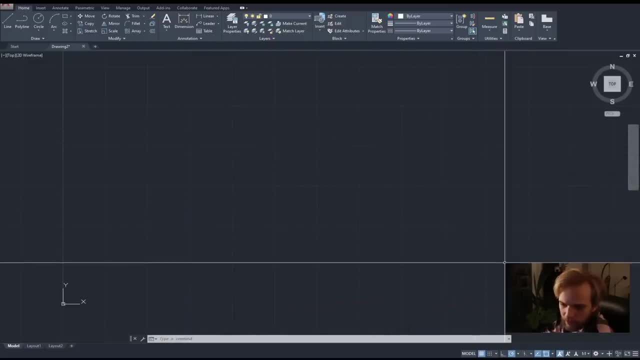 and i will give it a name. i will name it like this and i will give it a name like that. so it's just a couple of options. This is quite useful when you want to align, see if stuff is aligned properly, And I, honestly, I have been using it for quite a while. 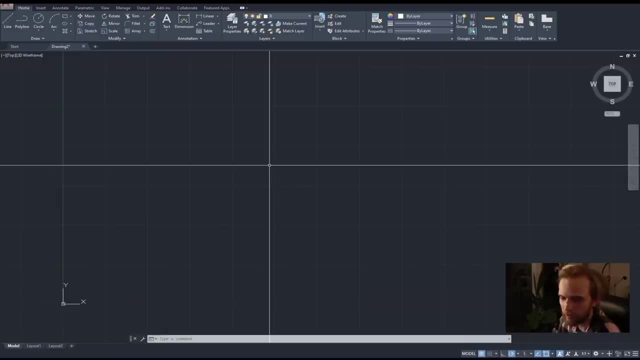 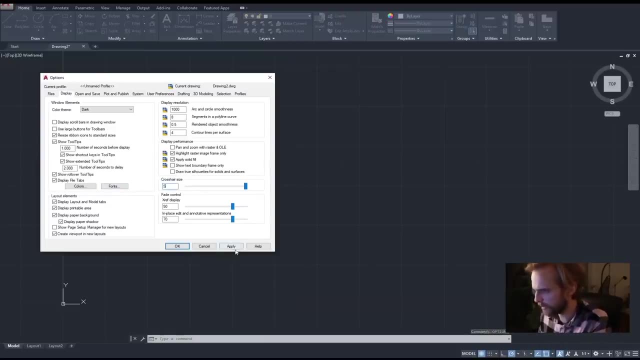 It's quite convenient, But at the same time sometimes it gets in the way. right, I'll type in options again and make it smaller. Was it five? I think it was five, I don't remember, Are you fine? Yeah, it was five. 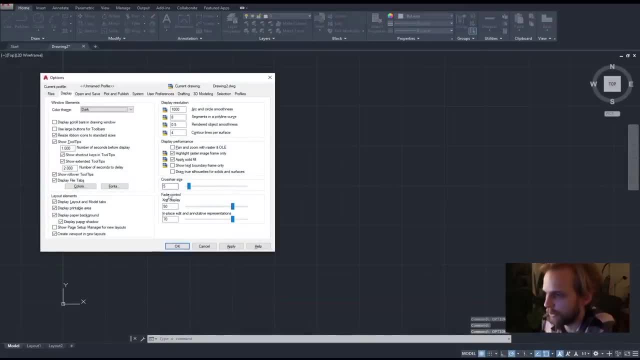 Okay, So I'll change it back to five. Everything else here is just, basically: how are things shown? I wouldn't suggest you going deep into this and changing stuff up. Definitely not now. Later, once you're used to the program Opening and saving, it's basically going to ask you: what kind of format do you want to always save the file in? 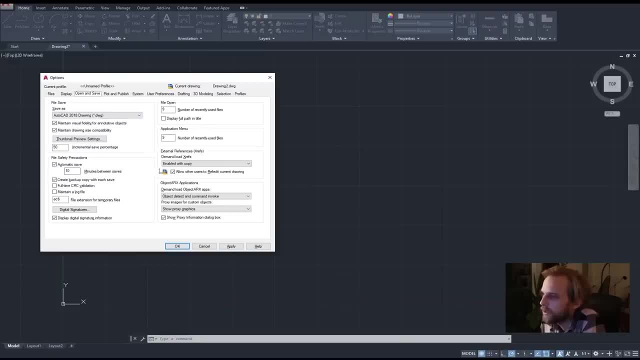 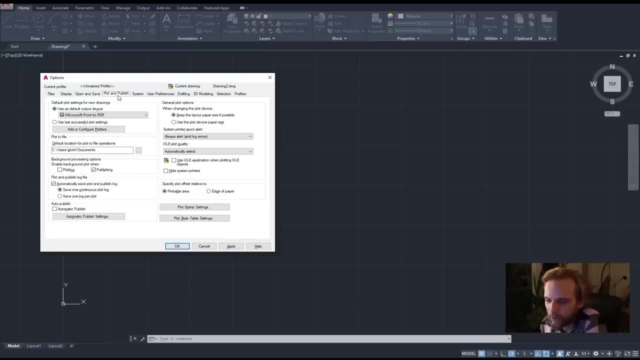 Don't argue with the program. It knows what it's doing, So don't mess around here. Plot and publish as well. It's basically. where will you export out the PDFs? Don't argue with the program System. Let's ignore it. 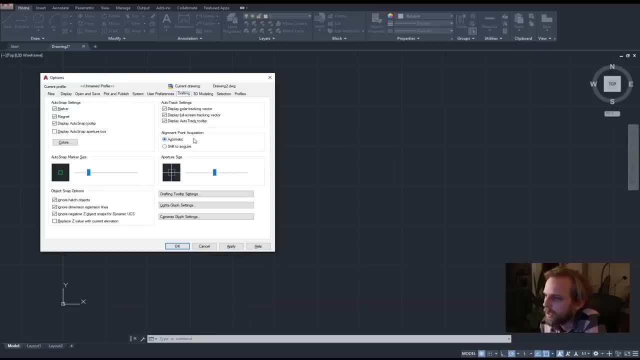 User preferences. Let's definitely ignore it Or wait. Yes, Drafting and 3D modeling. I'm just sorry. I'm just really quickly going through this And seeing if there's anything worth mentioning. Not really Defaults are absolutely fine. 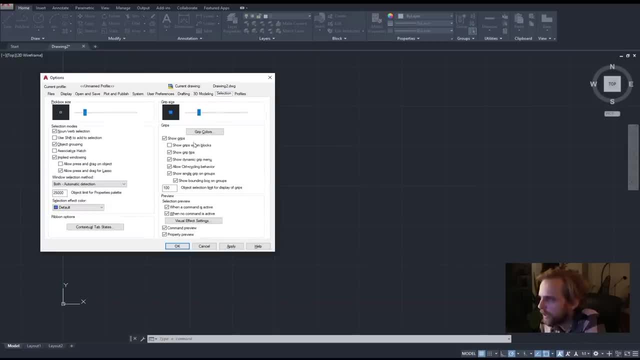 3D modeling. We're not going to do any 3D modeling, So we don't care. And then selection: So this is the big boy Where the culprit behind our lasso tool selection: Right, So it's here. 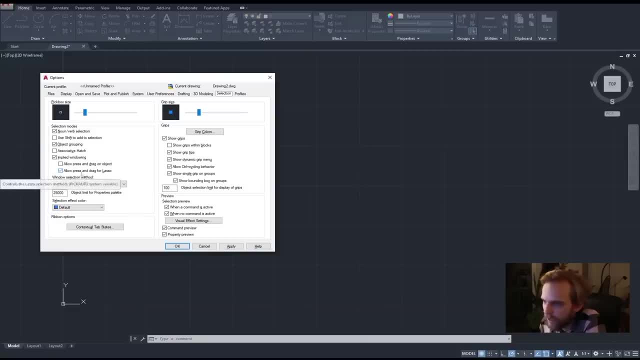 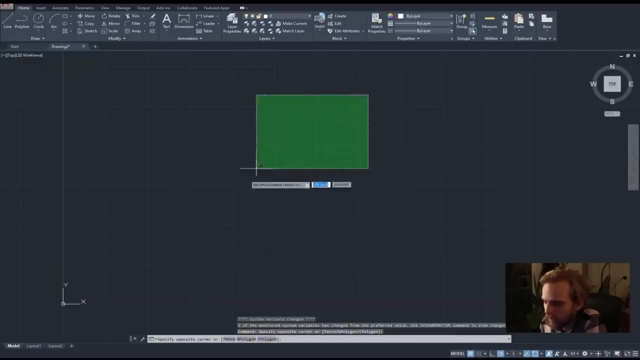 Allow, press and drag for lasso. This line right here And this tick mark right here Is the culprit. So I'll untick it And I'll just hit apply And hit OK, And now it's fine. You'll notice that the color is different. 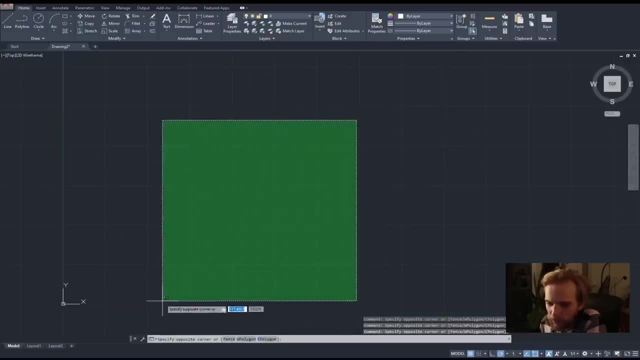 Depending if I'm going from bottom up Or from top to bottom, But it's It's. I will talk about that later. What matters is that it's a rectangle Right And not that ugly lasso, Okay So. 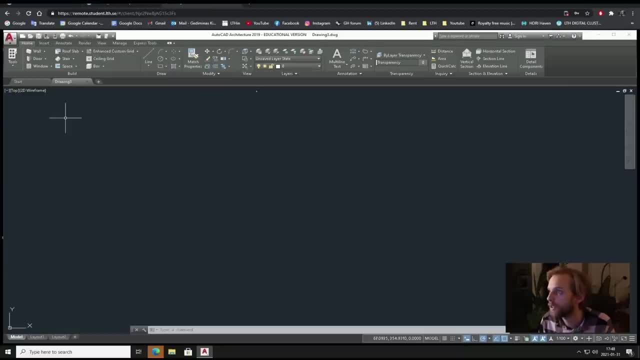 That's the first thing. Let me double check if in the other version, In this AutoCAD architecture version. If it's the same, I'll just go to options Selection. Yeah, It's the same. Allow, press and drag for lasso. 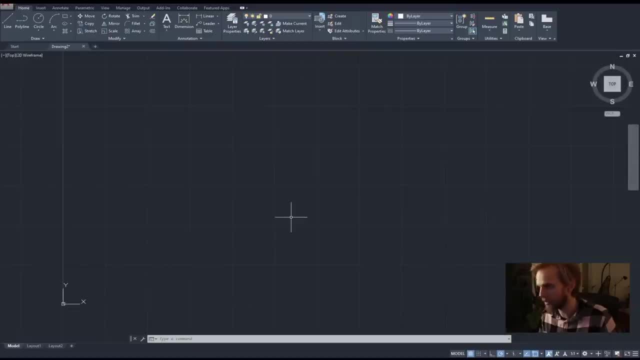 And now it works. Okay, Let's jump back here. So that's that: Below you have model space, Layout space And so on. We will be talking about those During the last tutorial, Not right now. And then you have a bunch of 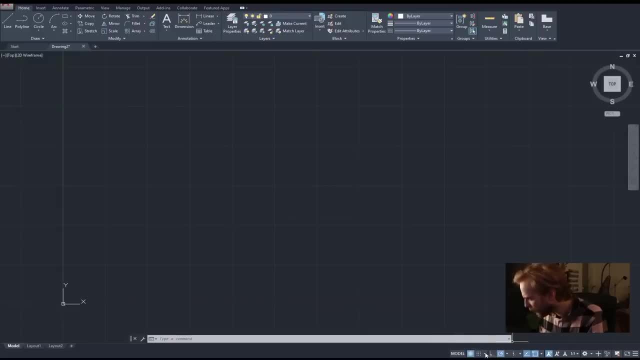 A bunch of stuff here. That is not enough stuff. I want to see more. Oh yeah, Okay, That's enough stuff. That's good. We will talk about those As well Later. For now, Let's actually start. 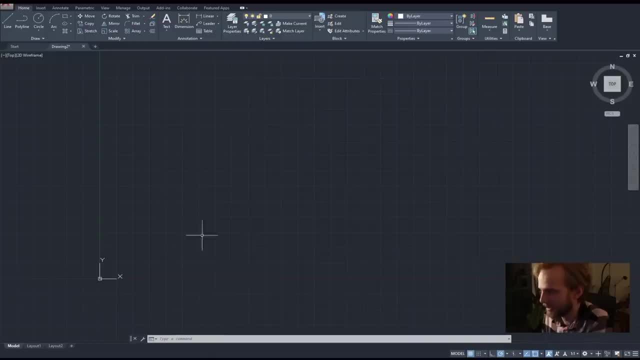 Start looking into the tools And start drawing Right. That's the fun part. Okay. So the question is: What's? what are the units, The measurements in which we draw? Is it centimeters, Is it millimeters, Is it inches? 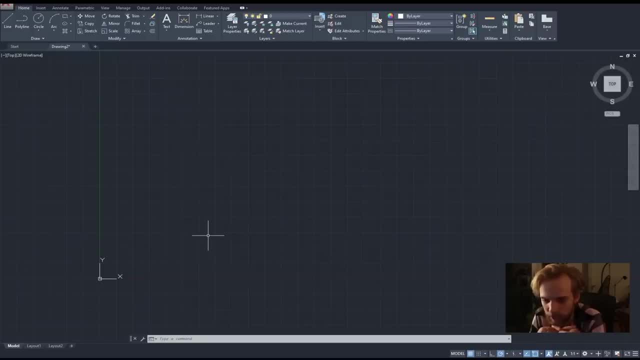 Is it horses per second? You know What kind of dimensions are we talking about. I need to actually make sure that I'm drawing, for instance, in millimeters. I'm used to drawing in millimeters. So what I will do is I will type a command called units. 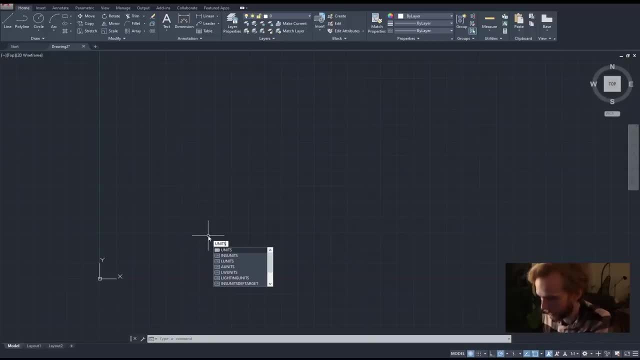 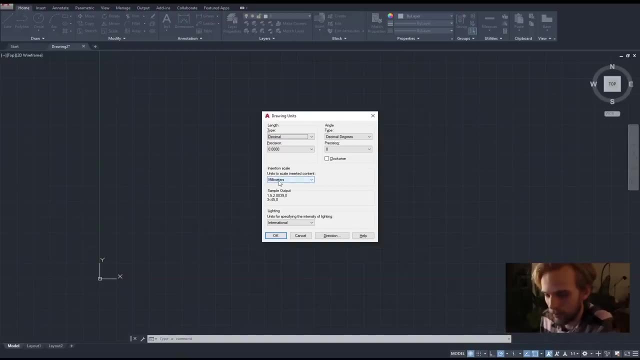 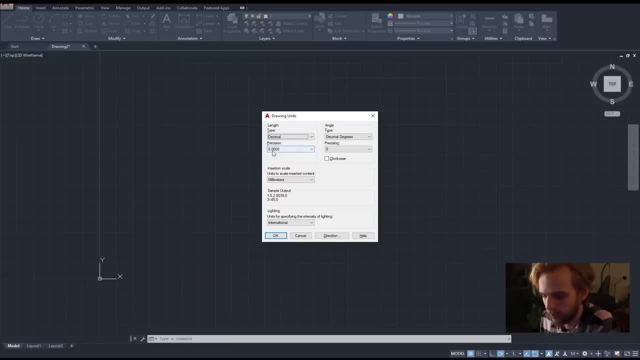 And this is my precision of drawing 0.0000 millimeters Right. So it's pretty damn precise. And degrees are. Oh, sorry, The angle is in degrees, not in radians. That's great. The precision is only full numbers of degrees. 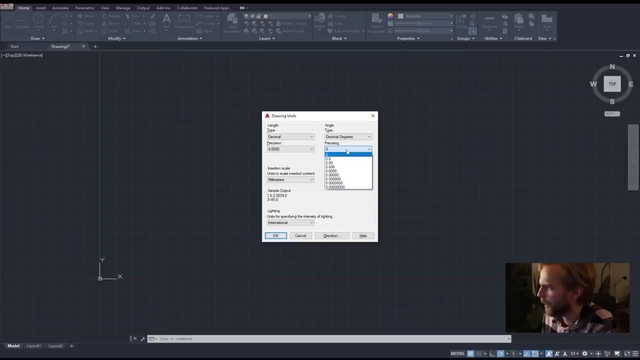 which i have a problem with. i do want the precision to be slightly larger, for four degrees at least. you know one number after the comma, so i'll just choose 0.0. and then lighting, we don't care, we don't care about once i'm i've made sure that it's millimeters and degrees, i'll just hit. 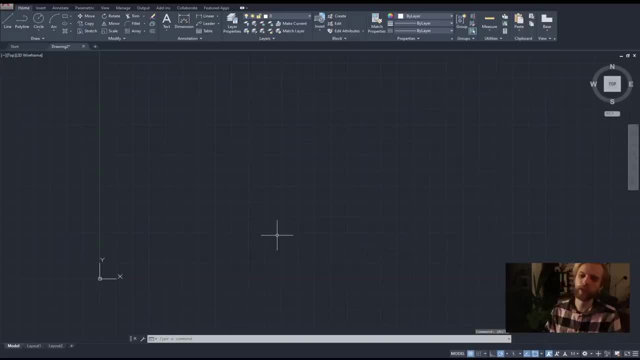 okay, and now we know that we are drawing in millimeters. okay, now it's time to draw. the easiest thing to draw is a line, right? so the line tool is located here, well, the one that says line, and if you don't see it, then you might have this version where, yeah, it's here, right? or? 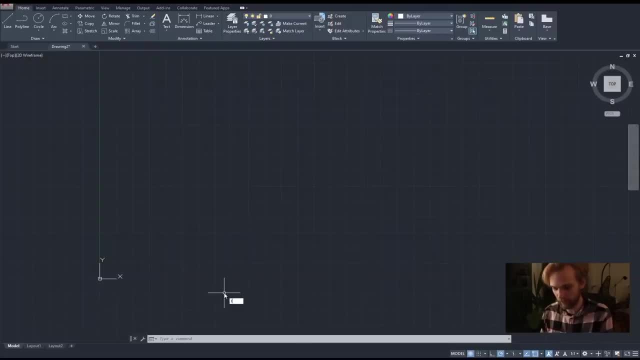 the shortcut for the line tool is l enter. l is short for line tool, short for line. once you hit l enter or you click on this icon here, um, you will start reading. you will need to read what it's asking of you in the command line. so the way autocad communicates with you about what it wants. 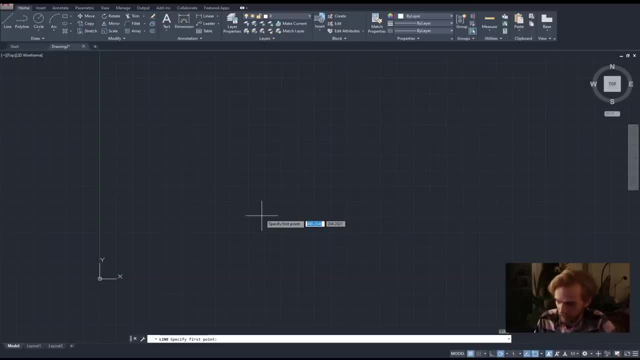 from you to actually be able to draw stuff is through the command line. so here it's asking line specific. specify first point: sure, i need to click somewhere, right, so i'll just click okay. then command line immediately switches to another question. specify next point, right, uh, sure. 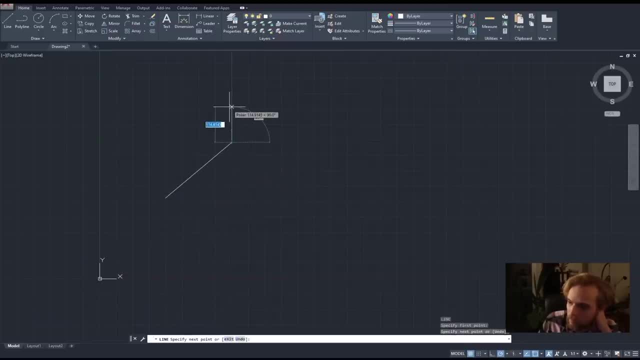 i'll click again and then, uh, autocad keeps asking me to specify next point. uh, okay, next point. okay, so you can see that i, i can keep doing this, this four, four, for a while. right, just keep drawing the, the lines, which is not you know, at some point i want to stop. 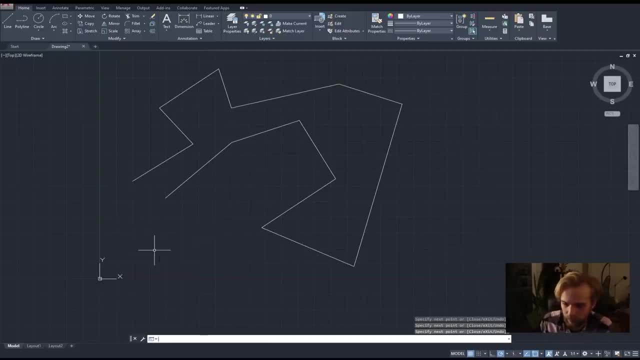 so the way you stop is you just hit enter, right to finish the tool, to finish the command. you hit enter and you have a bunch of lines. so now if i hover my mouse over them i can see that only segments like these straight line segments get highlighted and i can kind of select them right, select this one. 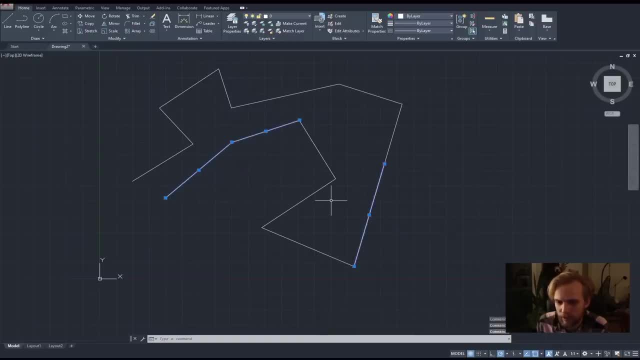 select that one, like that one, for instance, so i can click on them to select. that's cool. how do i unselect? well, I hit escape, escape unselects them. right. what if I want to select many of them without actually, you know, kind of clicking on each individual line segment? well, i can. 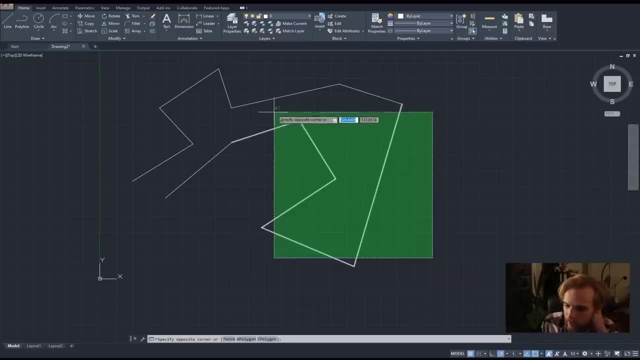 drag this rectangle here around the ones that i seinen selected. essentially i can. I'm going to select, release and these get selected right, Which actually, and then escape to and select, of course, which actually. yeah, let's do a small, small bit, a small. 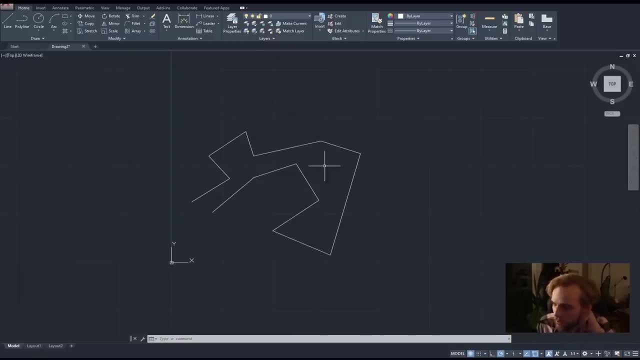 tutorial about selection here, because we already have some geometry that's available for us, So I'm going to. as I mentioned before, there are two ways of how to select: The blue rectangle, which happens when you drag from left to right, and the green rectangle, which 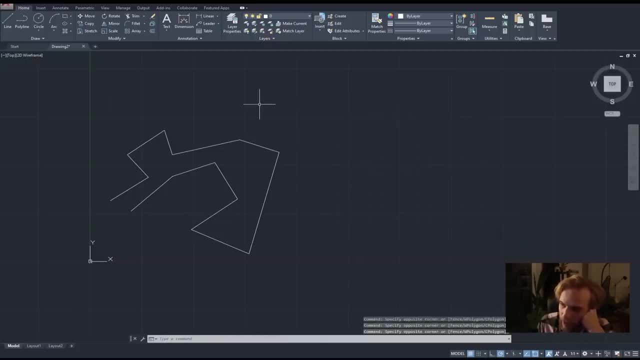 happens when you drag from right to left, right. So the blue rectangle only selects things that are completely inside of that rectangle, right. So, for instance, let's let's look at this line right here, this line right here right. If I drag the blue, 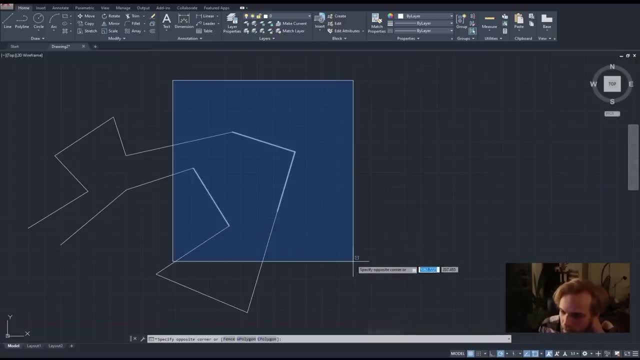 rectangle and it's crossing that line and I release that line, doesn't get selected because it's not fully inside. it wasn't fully inside of that blue rectangle. If I drag a green rectangle and it's crossing the line, in the same way it is going to be selected, right. 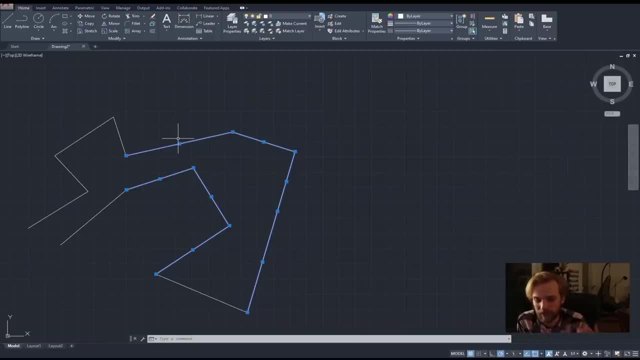 That's because the blue line only selects things that are completely, or blue rectangle. blue selection rectangle only selects things that are completely inside of it, while the green selection rectangle selects things that are inside of it and things that it's hitting, things that 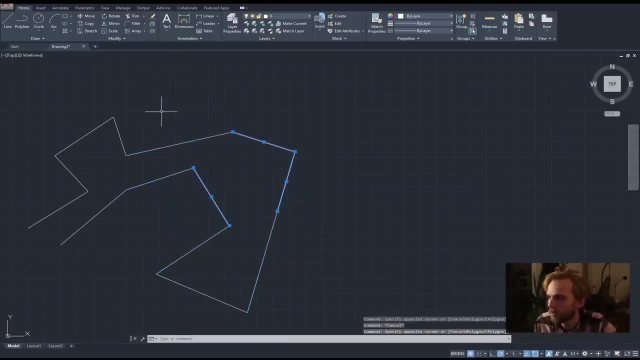 it's crossing right. So, again, the blue rectangle selection looks like that, while the green rectangle selection looks like that because it's hitting this line, hitting this line, hitting this line right. So that's that, Um right. So so now we have something drawn, Cool. Uh, let's select. 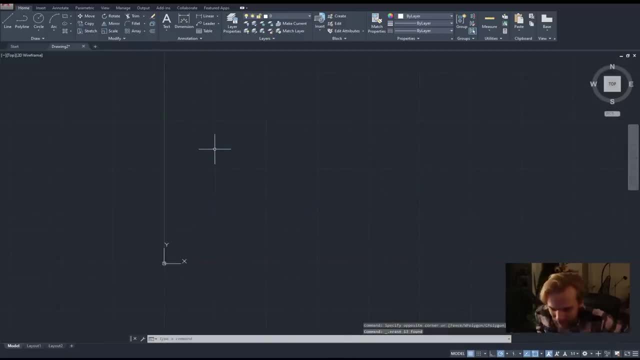 all of it and hit delete. You know, that's how you get rid of stuff. You just hit the delete button. Mac users, Backspace- probably, I don't remember- You can type in delete. I think Yes, erase, sorry, You can type in erase command and it's going to erase it. 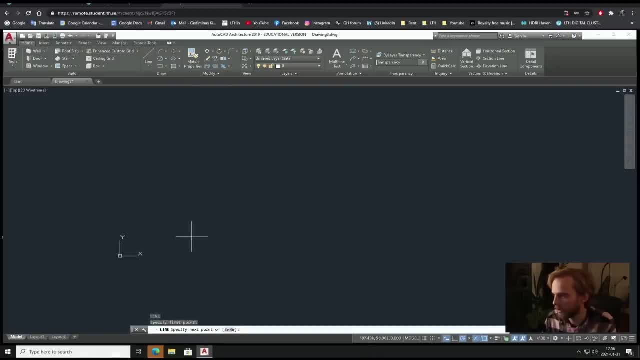 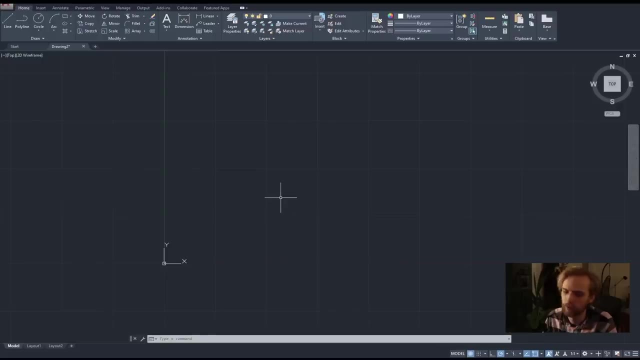 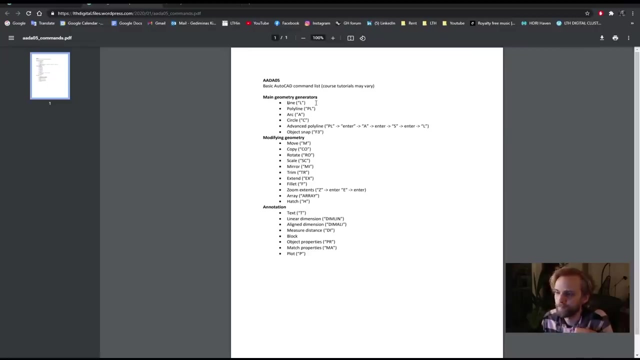 let me just see here l same thing. good, I'm just double checking. if yeah, yeah, okay, double checking. if there are no kind of discrepancies between the two versions, that's good for now. so that's our line tool, which is right here. that's the first tool. 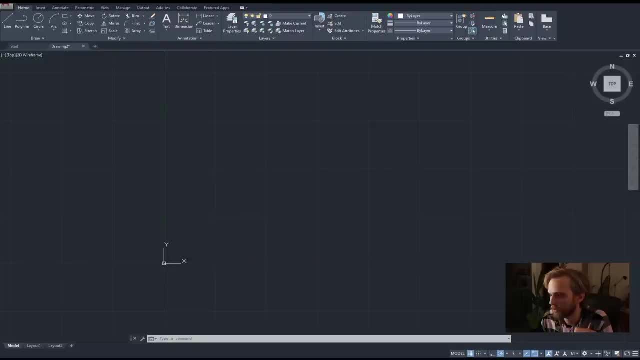 let me talk more about it, just so that you get a better idea of how things are drawn. so that line tool again l enter. for line l enter. I will specify the first point by just clicking, but then the second point, let's say I want it. 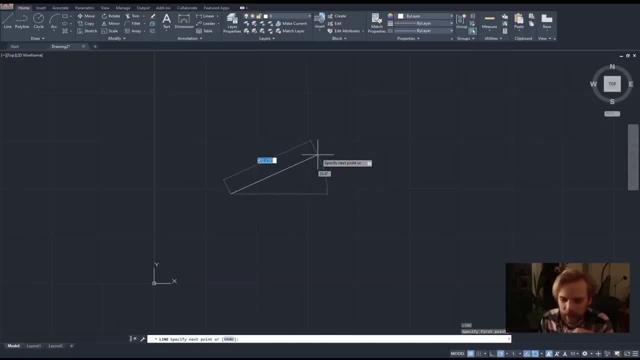 at this angle, whatever angle, right, but I want it to be, let's say, two meters long, right, 2,000 millimeters. so what I do is, before I click again, you know, to finish the tool or to finish the line- before I click again, I can type in the 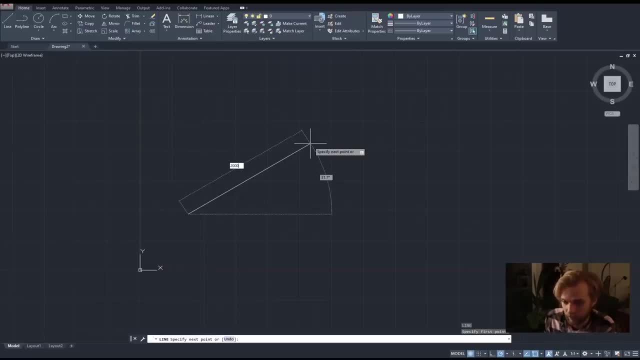 desired length: 2,000,. you know, two meters enter and now it becomes exactly two meters long in that direction Right, which is quite useful. what if I want to draw this line segment completely horizontal, right or completely vertical, doesn't matter- then the tool that does that is called orthographic. 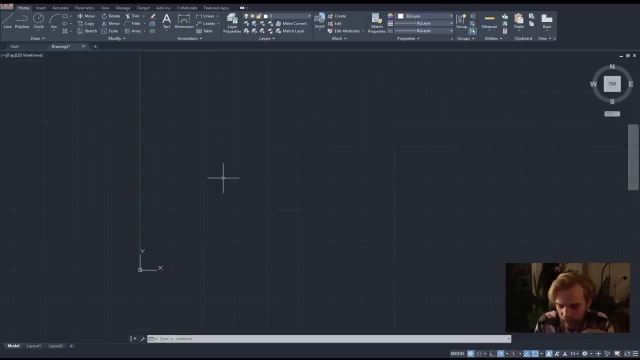 snapping and the shortcut for it is f8,, f8, in the top of your keyboards. f8, or a button that does that, is located right here in the bottom of the screen, ortho mode, and you can see in the brackets it says f8 as well, if ortho mode is turned on. 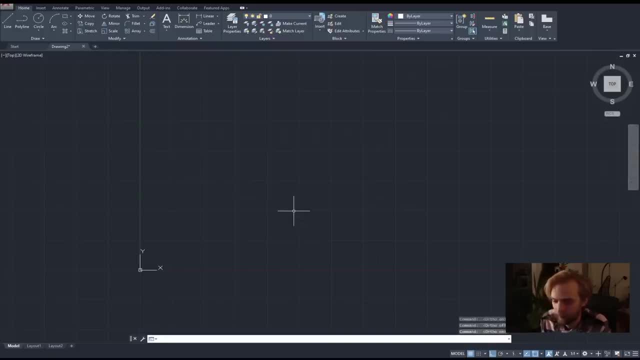 if I click on it or if I hit f8,. right, so with f8, I can turn it on or off. right, if I hit f8, or turn it on and I draw, try to draw the line, and this time let me just use the tool. 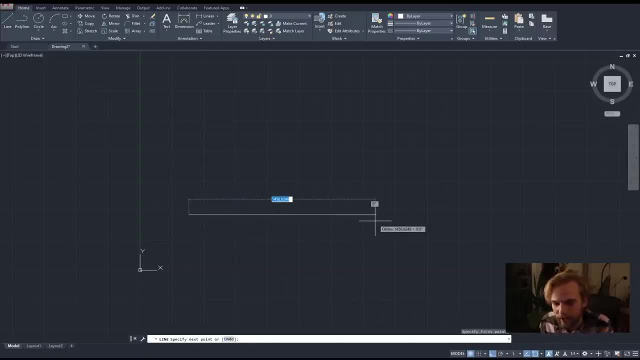 the icon here and I draw the line. you can see that it's locked to either horizontal or vertical position, right, which is quite useful. for instance, I want to say 5,000 millimeters or not. let's do 2,000, 5,000 was way too long. 2,000 millimeters, 500 millimeters, 1,000 millimeters. 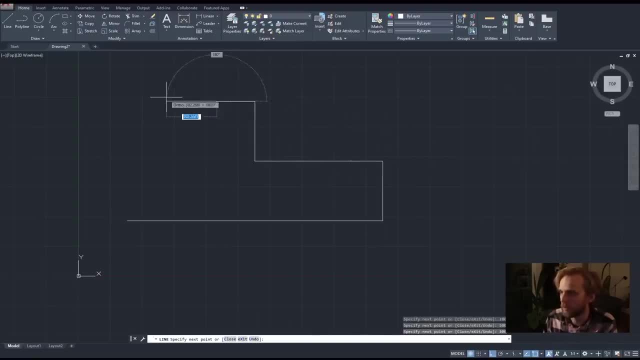 500 more 300 millimeters, 750, I don't know how long. this is probably around 700 millimeters, yes, and then close it off and hit enter right. I can have pretty precise dimensions when I have ortho on, so that's quite useful. I will show you later a few more. 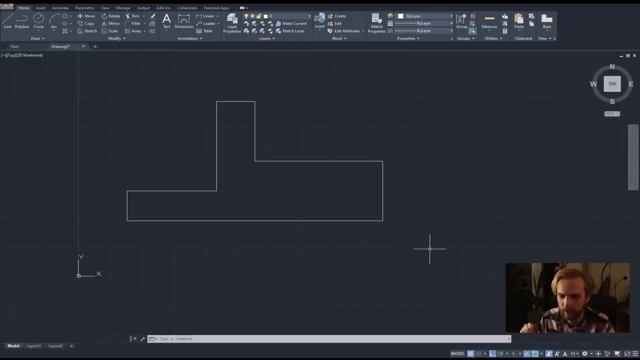 tips and tricks in terms of the angles and snapping to different angles, but ortho, turning ortho on and off is one of the smoothest workflows, let's say, or most useful workflows. let me get rid of this. 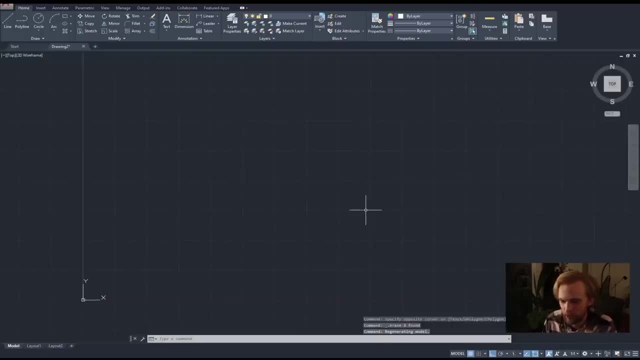 so that's how you, how you work with lines, and then the horizontal and vertical snapping of lines. let me turn off ortho for now. so I either click here on this icon or just hit f8, and I can see that that icon is turned off. now I can also. I need to check here if that's the same thing. 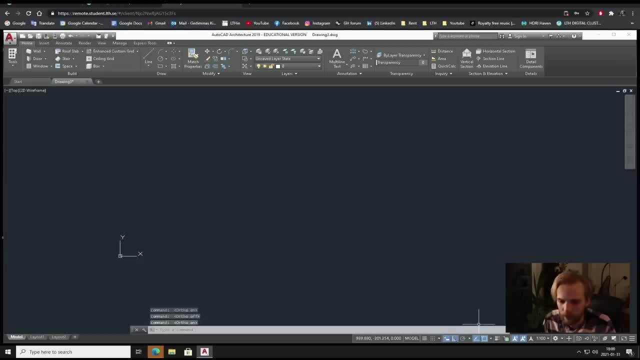 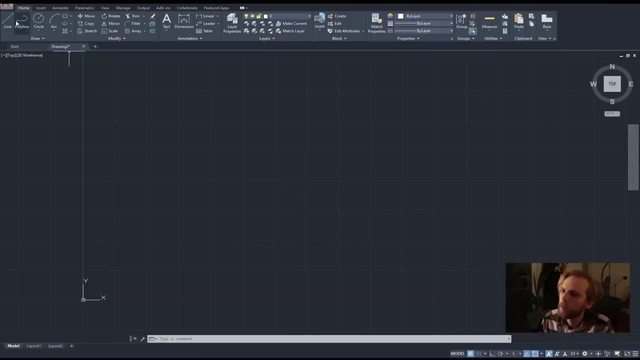 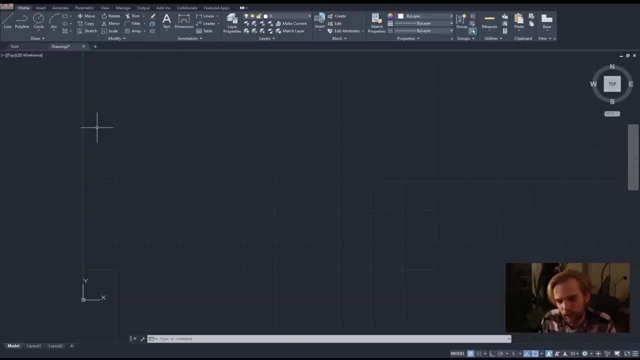 line, uh line tool is the most simplistic tool and it all it can do is just straight line segments that are all, so to say, exploded. they are separated line segments, right. polyline tool, on the other hand, is it. it can contain much more information inside of it. 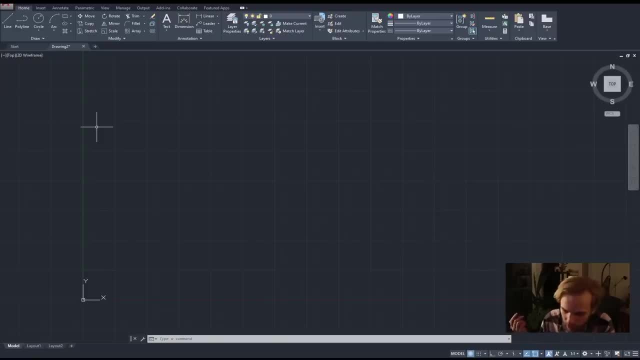 what I mean by that is, first of all, let's learn the shortcut for it. the shortcut is pl, or clicking the icon, of course, but pl- enter gives you the polyline tool and with orthographic snapping turned off, I will just draw quickly. draw a polyline without any dimensions whatsoever. 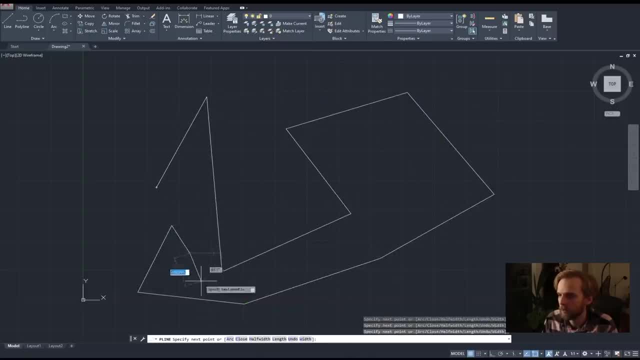 I'll just draw it whatever. I have no idea what I'm drawing, but it is what it is. yeah, let's say something like that and oops, and hit enter to finish the. the um, so now this is a polyline rather than a line tool. if I click on this, you can see that. 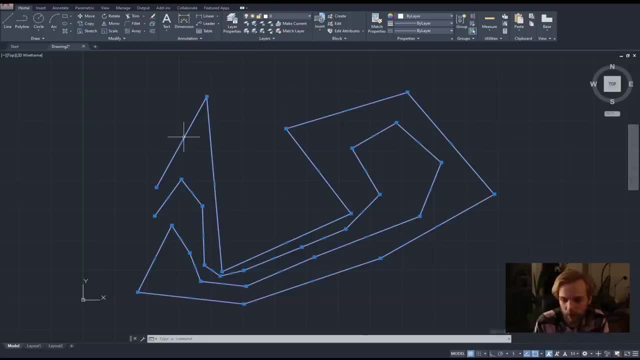 everything gets selected. this is a type of geometry that consists of multiple lines and all of them are joined into a chain of lines. it's super convenient for selection purposes, it's super convenient to work with and it doesn't really have any any drawbacks, um. 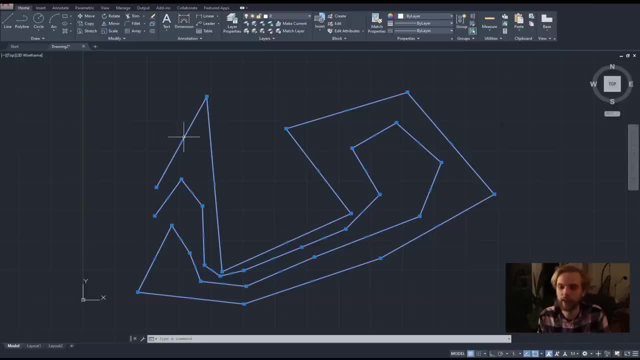 almost all of the lines that I draw during the design process and the technical process later on are polylines, not lines. keep that in mind. um, right, so we have our, our polyline. can you make a polyline into multiple lines? right, can? can you explode a polyline into multiple lines? 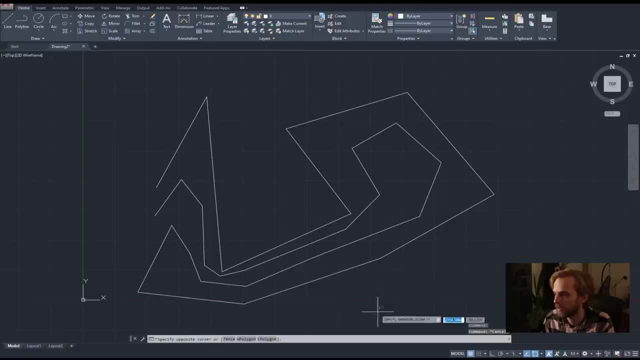 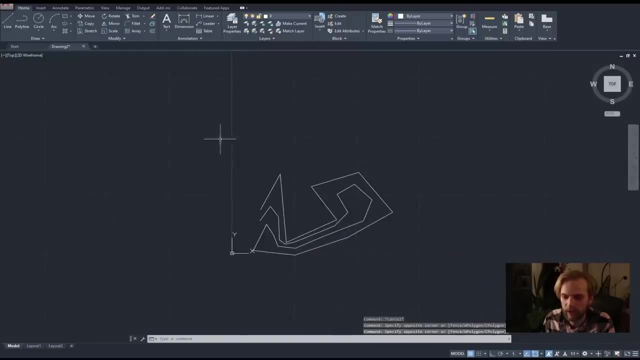 yes, you can. of course you can just select it. oh, by the way, if I use the blue selection rectangle, it will not select unless I have the whole polyline inside of my blue selection rectangle, while with the green one I can just kind of slightly hit it and it will select the whole. 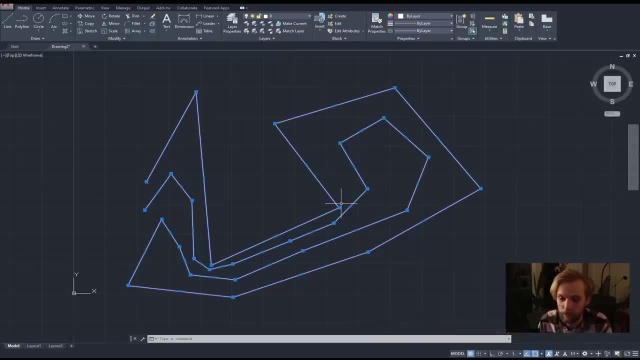 thing quite useful. um so right, we have a polyline. how? how do we make it into multiple lines? how do we explode it? well, we use the explode tool. when we have it selected, we just type in, explode. I think it's e-x-e-l. 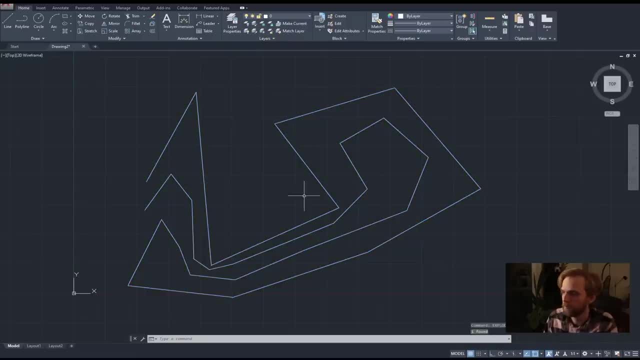 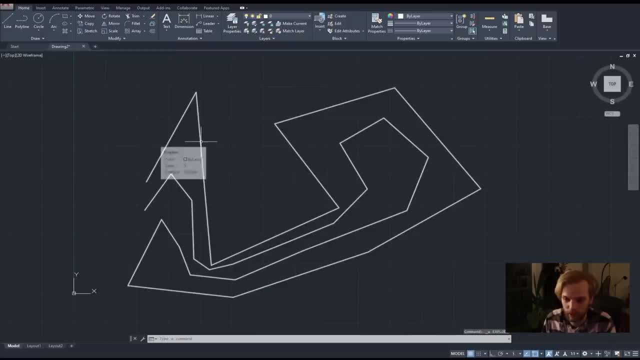 control z. you know undo and it's going to and undo your tool right, control z, control yeah, control z. this is undo. control y, I believe, is redo, um yeah. or if you don't want to do control z, or rather if you already have a bunch of. 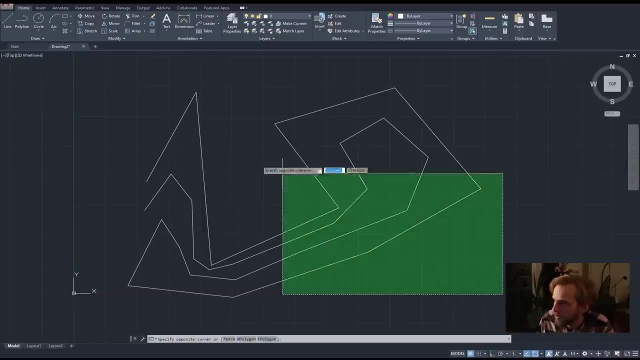 exploded lines and you want to join them up. well, you just select all of them and type in join and hit enter and it just joins all of them up into one polo line, back into one polo line. so there is explode and there is join. right, quite useful, okay. there are more things about. 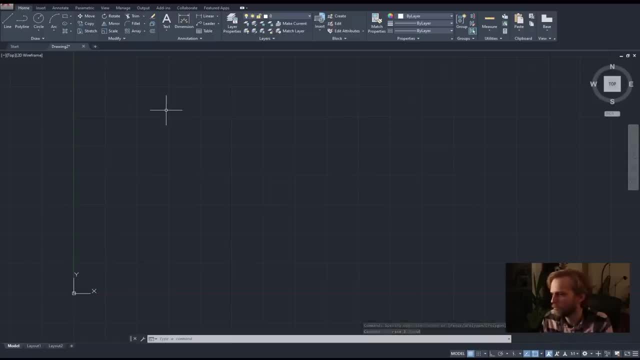 the polo line that i kind of want to show you. let me just think, if it's if it's the time, if it's the time to show you those, uh, those things, well, maybe, uh sure, let's start pretty, pretty hardcore. el enter so polo line. i'll start drawing and i'll just create the first line segment. 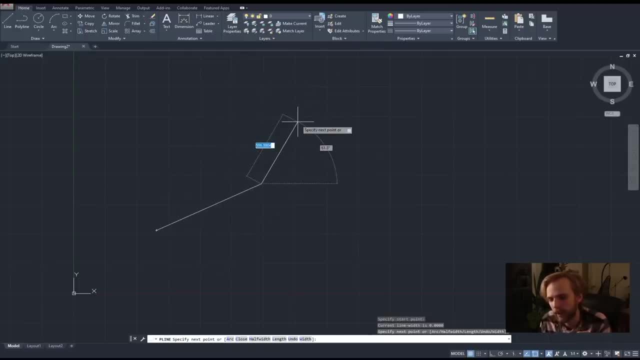 and what if i don't want this to be a straight line? what if i want this to be a curve, an arc? right? i can't do that. do it with a polo line tool here in the bottom. you can see that it's. it does have much more settings to choose from. 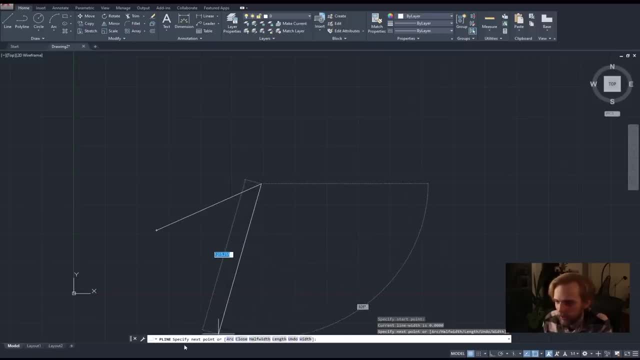 rather than just having give me the next point, because it says: specify next point. or is it an arc? Is it closed? Would you like to close it? Is it halfway? and so on. So there are a lot of hidden settings in these tools that you will learn them once you need them. 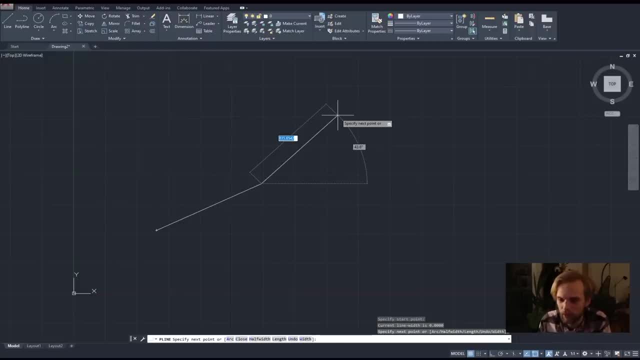 Let's say it like that, right? Once you have a problem to solve, then you will learn that different tools have different like small settings that you can tweak to solve that problem. We definitely don't have time to go through all of the settings of all of the tools in AutoCAD. 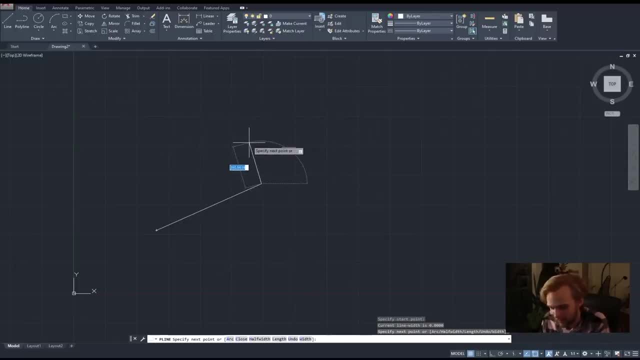 It's a little bit too big for that, But the basic one that I want to show you is the arc right, And you can see that A is highlighted right. So what I'm going to do is I could just click here. 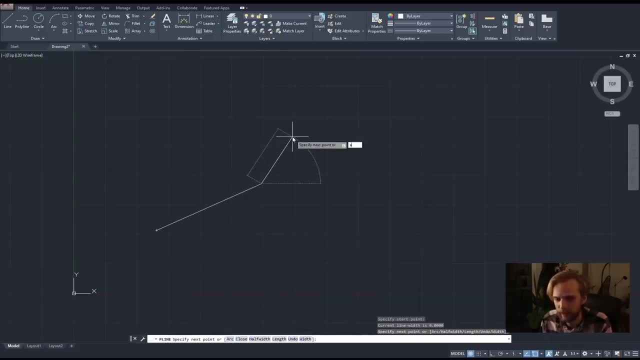 but rather I will press A type in A, as I'm still drawing the polo line, by the way, I'll press A hit enter. And now I'm in what's called an arc mode, right? So you can see that all of the tools have changed. 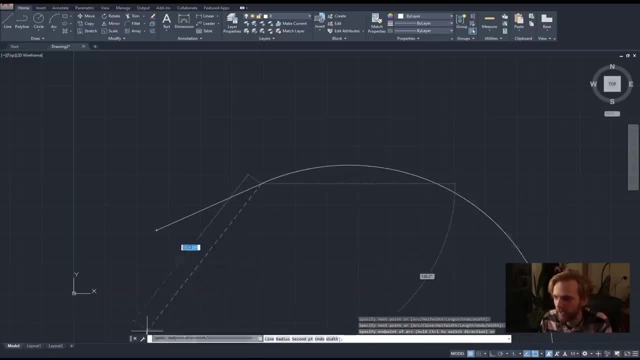 or not. the tools, the settings have changed and I have even more settings to work with, But for now I'll just work with this right. So I have the arc tool and I can mess around with it quite a bit, See. 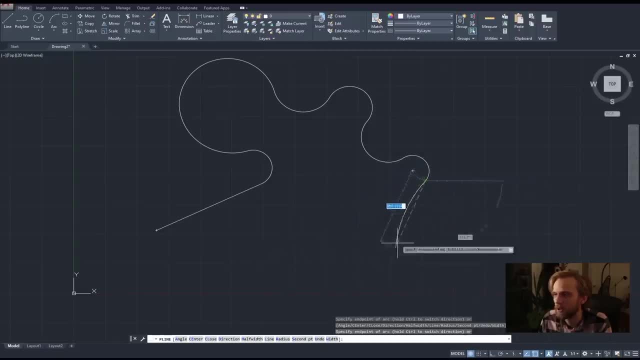 Something like that. And now, if I want to change it back to the line tool, all I need to do is just type in L and hit enter. And now we continue drawing in straight line segments, right. Once we're done, we just hit enter. 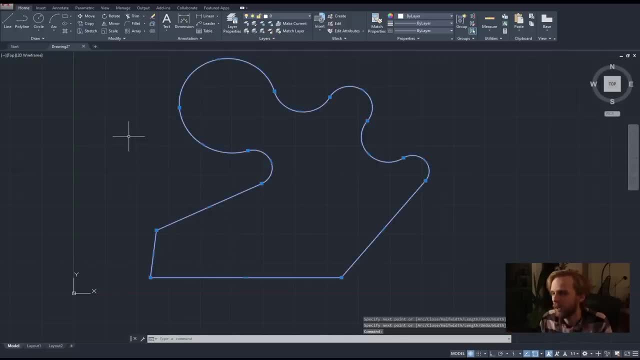 And now we have this kind of polo line, Quite nice, quite useful, which can also, by the way, be exploited. And you know, these settings or these arcs can be deleted off and whatnot. Yo, why is my? okay, my AutoCAD just lagged a bit. 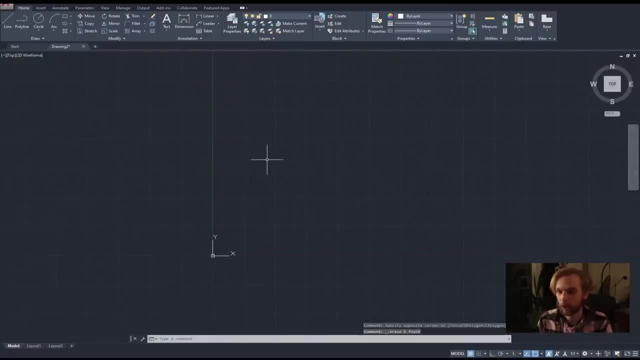 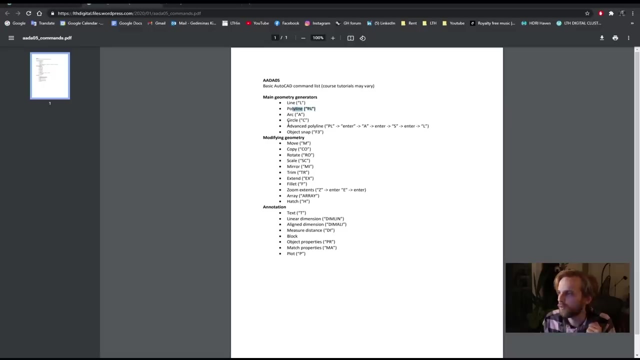 but that's fine. So that's polo line And that's all of the, not all of them, just one hidden setting inside of polo line. I will show you more later, once we actually need them. Right, let's cross off polo line from our list. 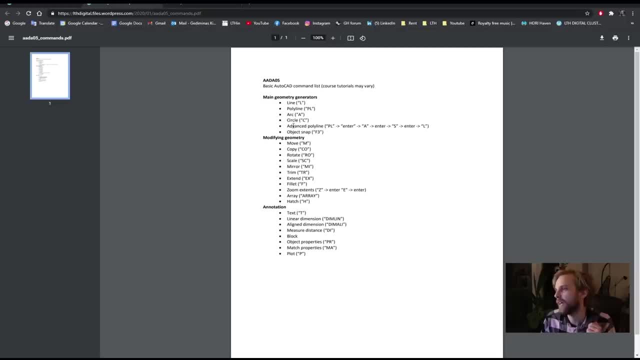 And then we have the arc tool and the circle tool. Oh yeah, I already showed you. I already showed you the advanced polo line. Apologies for that, for not keeping to the script. I just wanted to show it to you. Okay, let's jump to arc and circle tools. 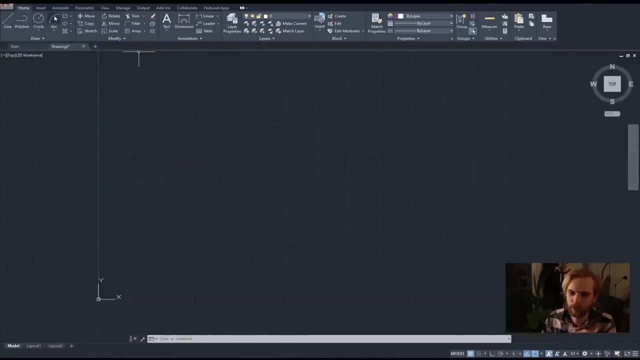 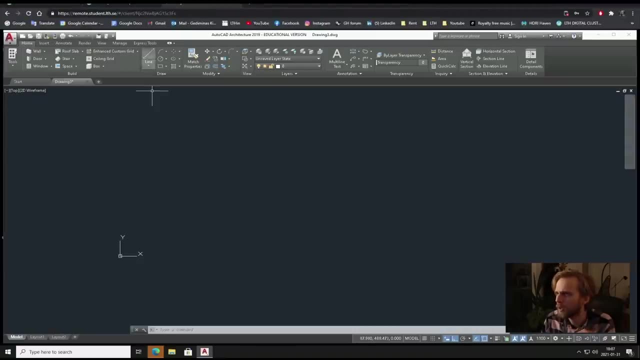 I will. well, they are located here, of course, Circle, arc right And also also here you have the arc and you have the circle, but you don't have the polo line here. But if you expand it by clicking this, 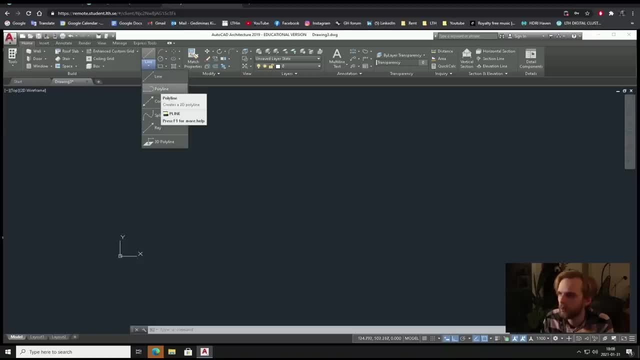 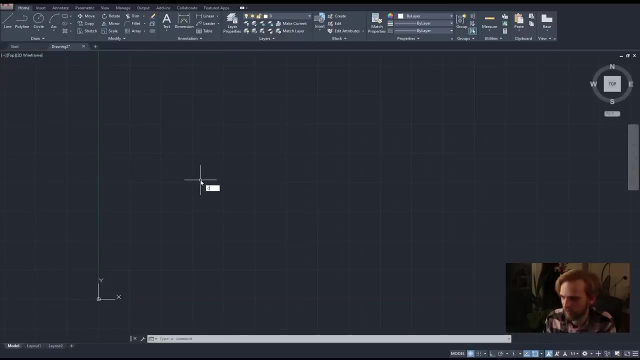 this small triangle. here you will see the polo line pop up here Again, I do suggest you using the command line instead. So we have the arc and the circle. Well, let's start with the circle, It's easier. So circle is C enter. 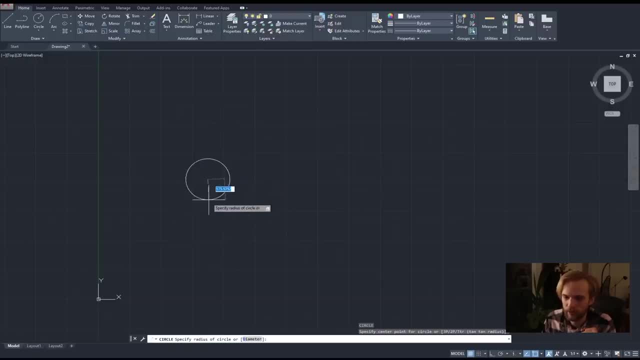 You just click on where you want the circle center to be And you kind of type in the radius that you want, Let's say 250.. Right, so now we know that the diameter of the circle is 500,, radius 250, and it's located right here. 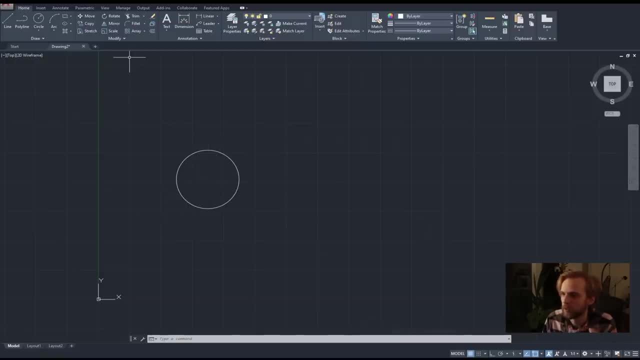 Cool. What else can we do with a circle? Let's see C enter. There is like there are a few options here that we can use And I will, for instance, without clicking anywhere, I will just select this 3.3P option, like that. 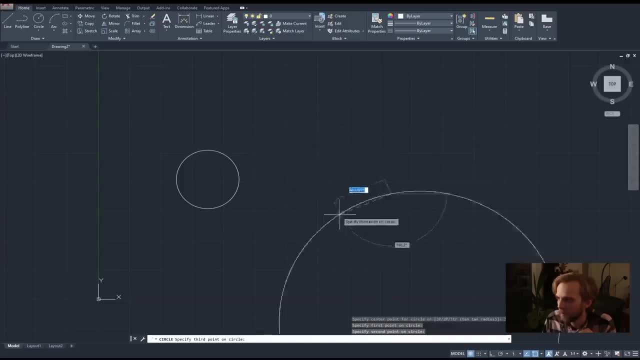 And now I will click three times on the screen Right And you can see that those three clicks that I made describe the circle's position and radius right, So that circle is touching those three points that I clicked. I can do it again. 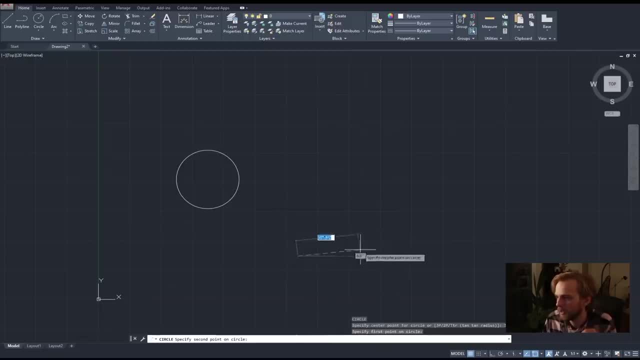 C, enter Three points, Click, Click. And then if I say that well, actually I want the third one to be right here, It's going to be like a very weird circle. Click. So three points, again, circle is touching them. 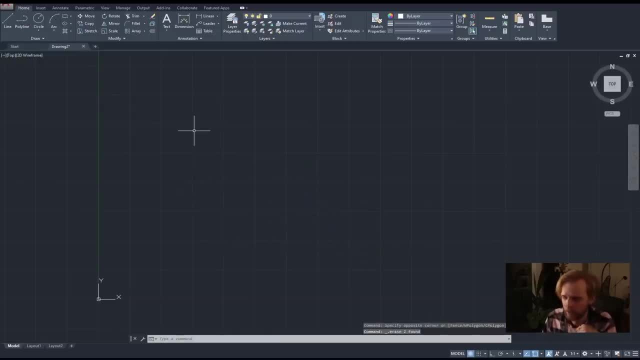 Pretty cool. Then we have the arc tool, which is basically- I believe it's A Yeah, A short for arc- Hit enter And it's basically: specify start point of arc- Okay. Specify second point of arc- Okay. 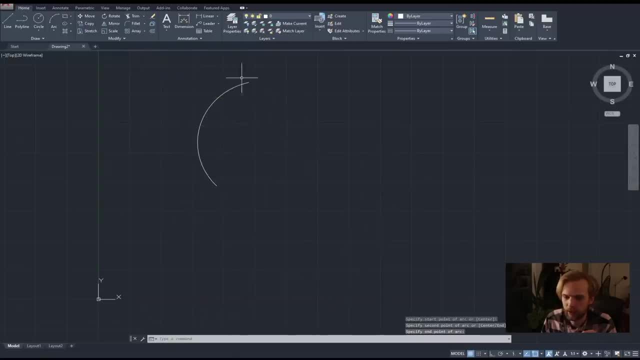 Specify the end of arc. Okay, So we have our arc done here. If I want it to be a little bit, if I want to draw it differently, I can. By the way, when you hit enter, if you don't have any commands running and you hit enter, 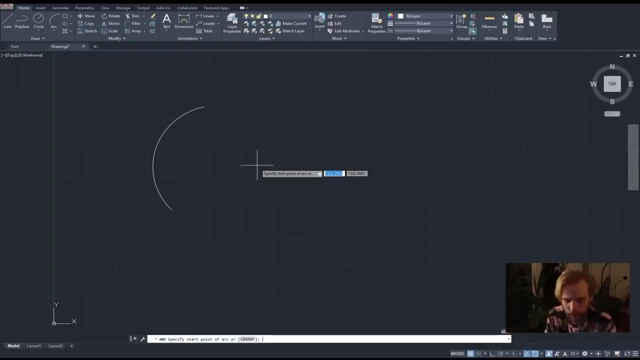 it repeats the last command that you did, So now I don't need to type in A enter, I can just hit enter and it's going to kind of repeat the previous command, which was arc. Instead of specifying the start point, I will choose center here. 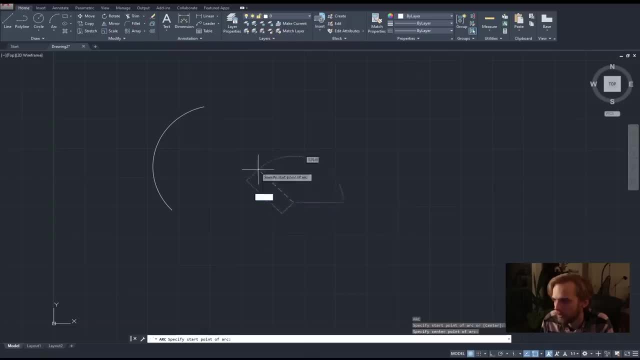 So I'm starting to draw from the center, See from here, And then it's going to ask me to give it the start and to give it the end. Right, I'm basically just drawing part of the circle. Well, arc is an arc is a part of a circle. 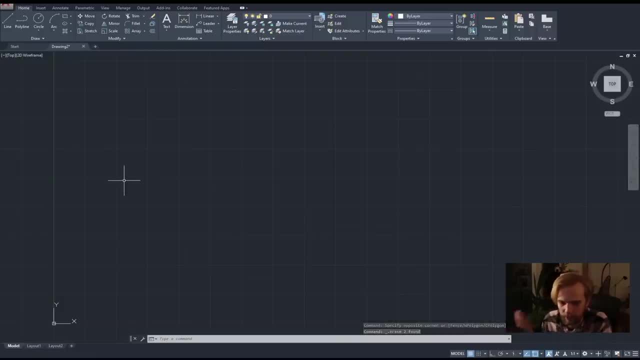 Okay, So that's that, that's the circle And that's the arc, that there's nothing more honestly to them. Um, there's also like rectangle tools and whatnot. Uh, perhaps I should wait, I will be showing your rectangle tools. 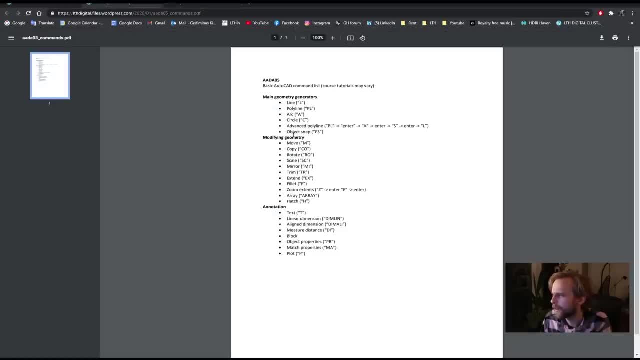 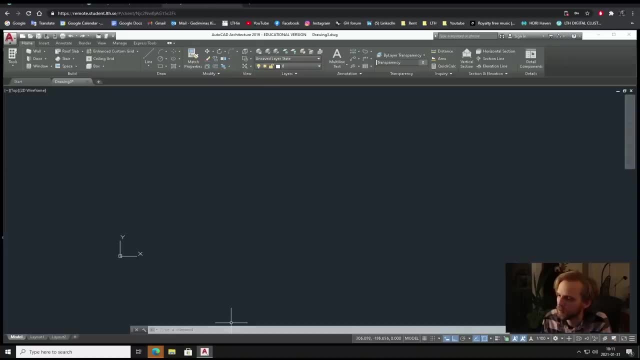 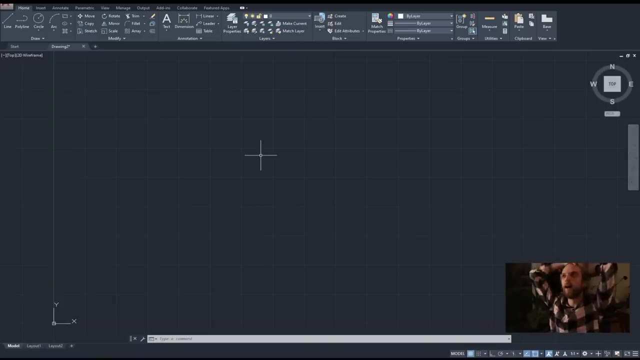 Okay, Rectangle tools later though. There's no, I haven't even written it down here, So sure Let's, let's ignore them. Um, for now, circle arc line, Paul line is enough to describe. Okay, So these four tools- circle arc line, Paul line- are enough. 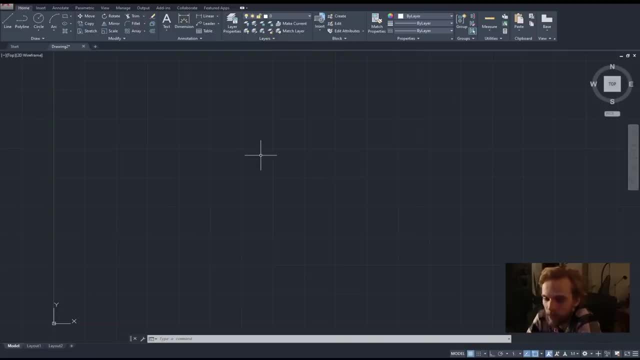 to describe any kind of geometry Absolutely Like: uh, there's no type of geometry that you couldn't draw out with these tools, Right? So the basics are super simple, and what a rectangle is is basically a polo line with, uh like parallel line segments, right? 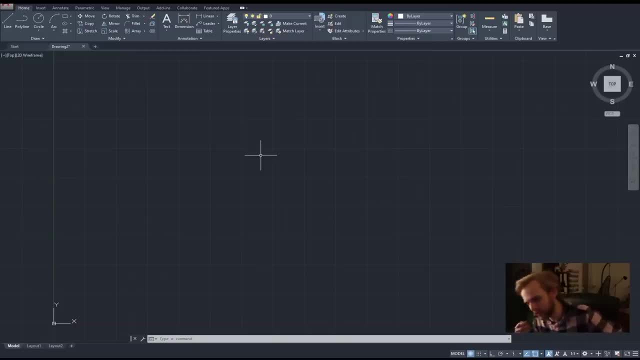 Making it a rectangle. Um, I will just Really quickly show it to you and then we'll jump, jump into snapping possibilities. So, rectangle, rectangle. I just like to write erect, Uh, but wait, R E, C, R, E, C is is enough for for rectangle to start working as a command. 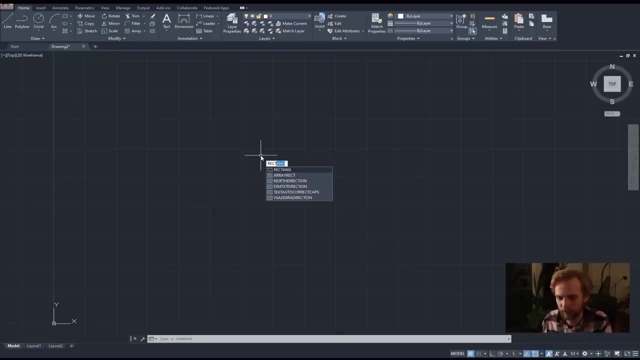 Uh, but I, I don't know why I have a muscle memory of typing in R R E C. Uh, but I, I don't know why I have a muscle memory of typing in R R E C. is enough for for rectangle to start working as a command. 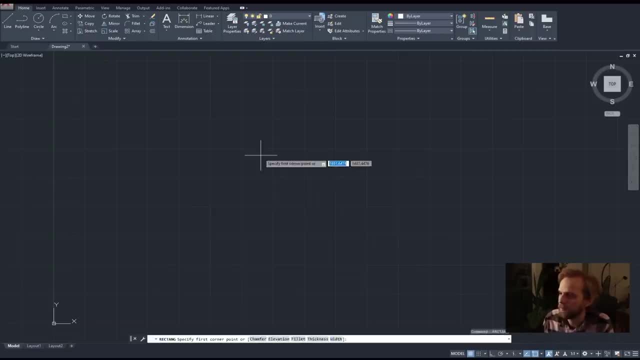 Uh, but I- I don't know why- I have a muscle memory of typing in R, R, E, C, T, Rect. It entered, uh, it's going to start drawing the rectangle and it's going to ask me to give it the first point. 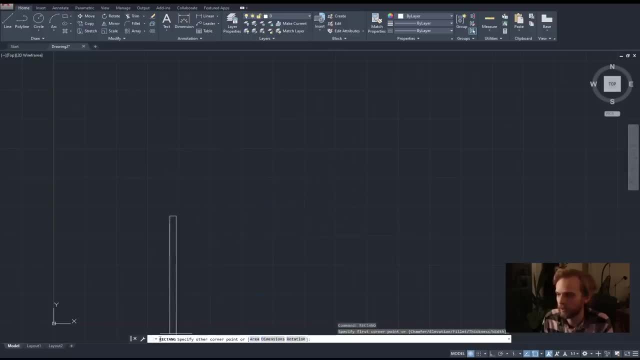 Sure, I will just click, and then it's going to ask me to give it another corner point Right, Or or I can give it the dimensions. So I think dimensions is a much more useful use case than just giving it two points. 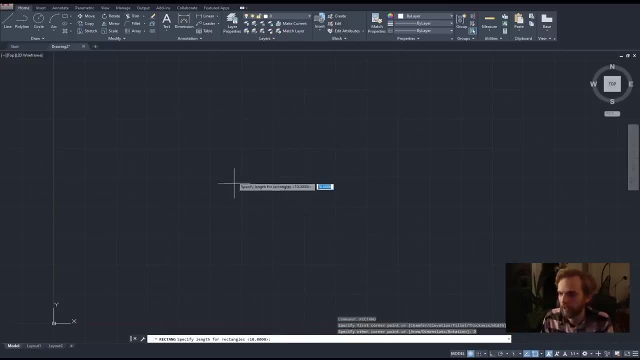 So I will choose dimensions and I'll say: specify length for rectangle. so I will say: well, my length should be again two meters, two thousand millimeters. that's the length. I hit enter. and then I specify width for rectangle. so I'll say: let's do a pretty narrow one. so I'll say: 10 centimeters, 100 millimeters, right, 100 enter. 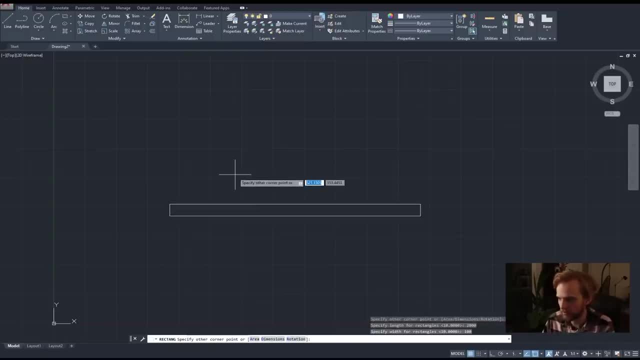 that's it right. it kind of is asking me for: oh right, right, right, sorry, sorry, that's not it once we added the dimensions. now, with a mouse click, I need to specify the alignment of the rectangle. is it going down or is it going up, right down or up, down or up? I'll say up and I'll just. 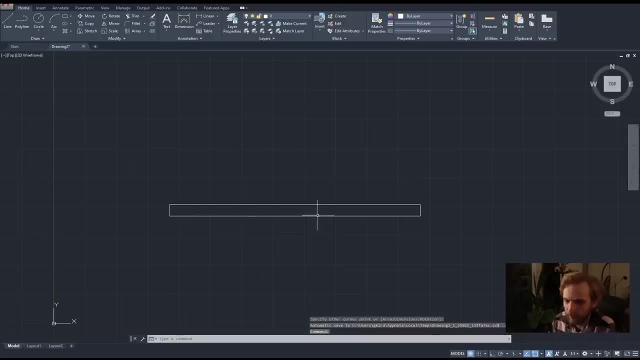 click. that's it. now it's done right and we have a rectangle which is basically just a polo line. if I grab the polo line pl, I start started working with it with ortho on, which is f8, and I typed in 2000 enter, and I typed in 100 enter, 2000 enter. click here enter, that's it. that's this, absolutely like these. 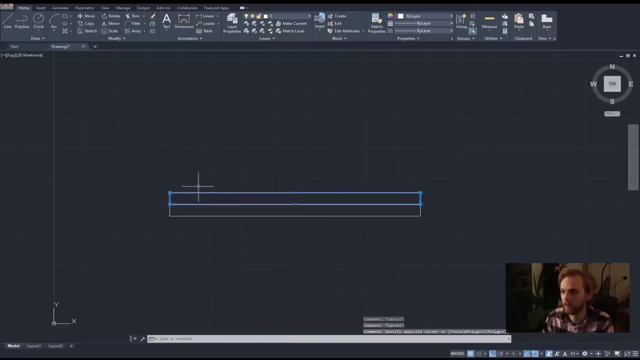 two geometries are absolutely the same. you so that's that, okay, let's. let's look into delete that. let's look into object snapping and ways of how you can snap to different parts of objects and, you know, kind of merge everything together much more, or rather use geometry as reference for creating more geometry. now you'll see what I mean. 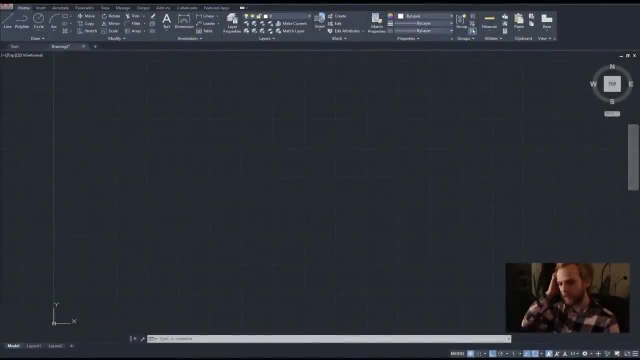 the second. all right, so object snapping here in the bottom right, here you will see, Oh snap, will object snap tool, which basically that small arrow right next to it will expand, will expand. there we go. a menu. oh right, there we go, just fixing it will expand the menu. or what types of sub geometries can you snap to? 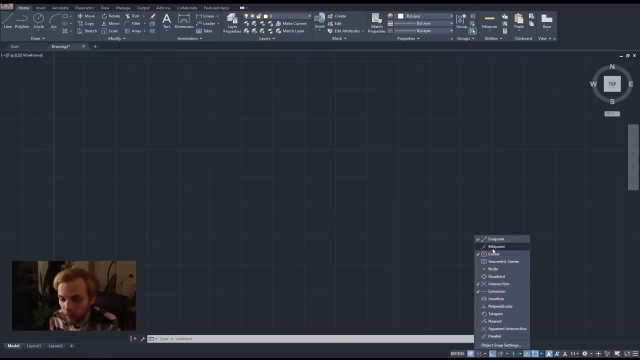 so there are like endpoints of lines, there are midpoints of lines and so on. so I will I'll start showing you different ways- or, or yeah, different ways- of how you can snap to geometry. so for now, let us untick all of the snaps all together, right? so nothing is marked. click anywhere on the screen and let's draw. 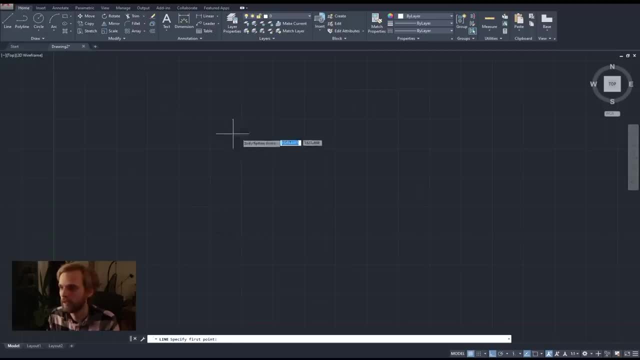 a line, right, just a line line from here, and I will be drawing it straight like vertical. I'll just give it. so if you can't just f8 or ortho snap, turn it on, and then you will be able to, and I'll just give it 2000 millimeters. Hit, enter, Enter again. 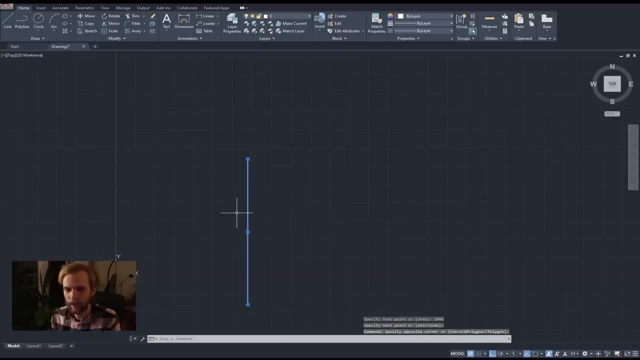 Right Now it's drawn And honestly I just want to move it away from the 0, 0, 0 coordinate. So this guy right here is my 0, 0, 0.. So I will just select it. M enter M to move. I'll just move it. 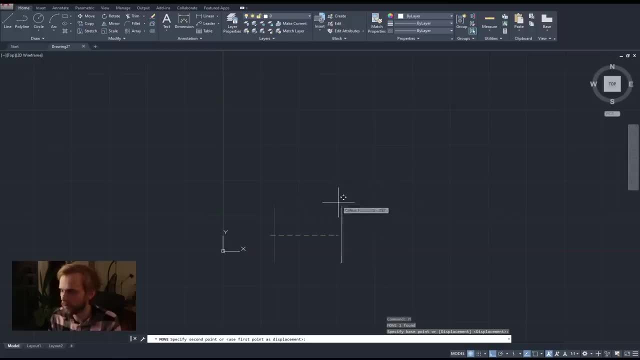 away. So when I try to move it with orthographic snap, maybe I need to do this slower, Sorry. Sorry, I'm speeding. I will select it. M enter, M short for move enter. I will click anywhere on the screen, Doesn't matter where I click, And then, as I kind of move my mouse, you can see that. 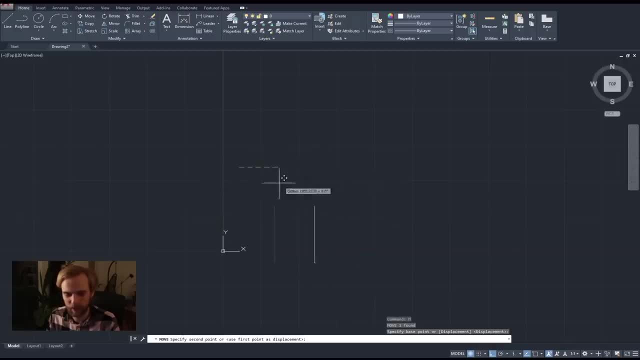 you know, it's being moved in relation to my mouse cursor. Since I have orthographic snapping turned on, it can only move horizontally or vertically right, So I'll hit F8 or turn off ortho snap here And now I can move it anywhere on the screen. So 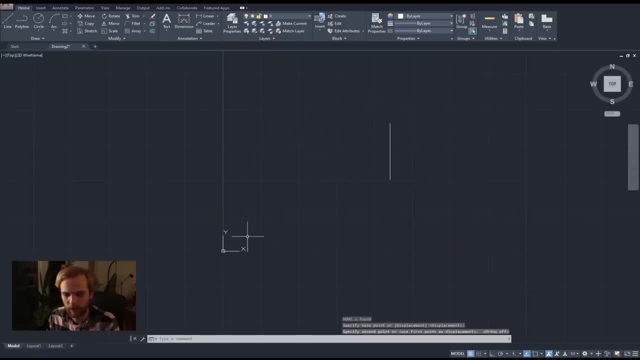 I'll just move it somewhere here, Doesn't matter, Away from the 0, 0, 0.. I'll zoom into it Right. So that's my line tool Now, since we have all of the object snapping turned off. if I want to create a new line, I can do that. So I'm going to do that. So I'm going to do that. I'm going to do that. So I'm going to do that. So I'm going to do that. So I'm going to do that. 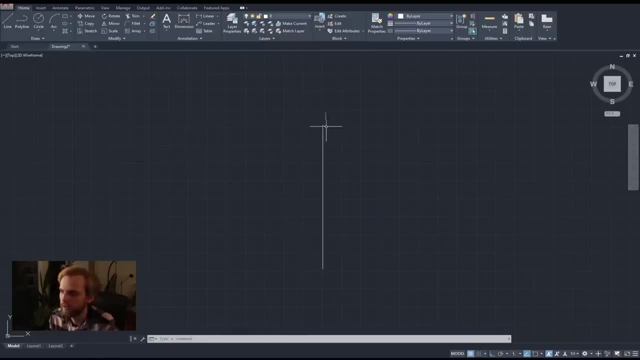 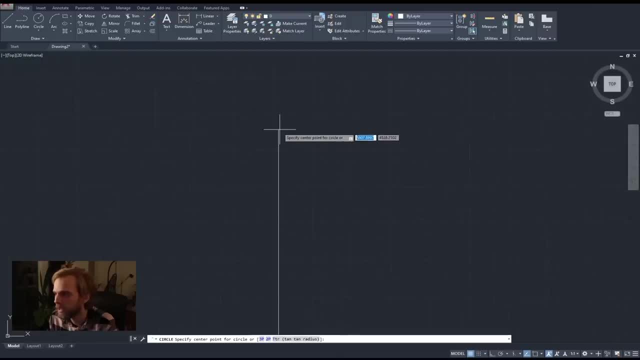 well, I can't snap to it and I can get pretty close, but the closer I zoom in, I keep seeing that there's an error in my. it's going to be an error in my in the center point, where I place it right, So this is not going to work. Instead, let me hit escape. 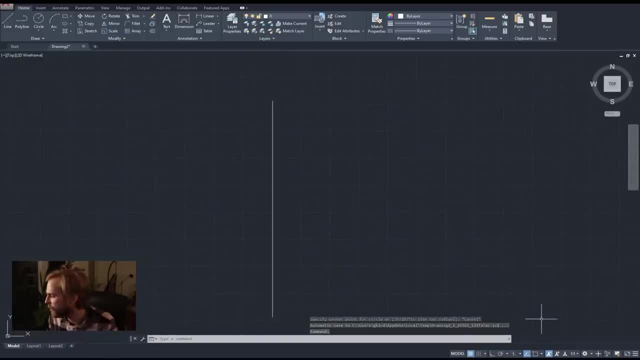 to you know, I'm going to do that, So I'm going to do that, So I'm going to do that, So I'm going to do that. Let's see close that tool. Instead, I am going to check mark the end point, snapping here. 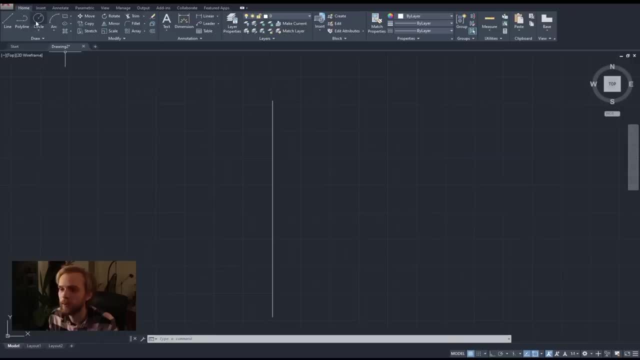 That's enabled now, And now if I choose my circle circle tool, I can click on it. Oh, actually, when I choose my circle tool and I hover my mouse next to the end point, you can see that there's this green. 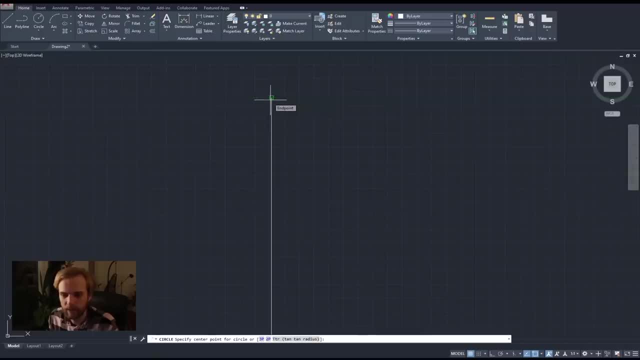 icon appearing. that green icon basically tells me that I am going to snap and I'm going to start drawing from this point, right from this end point, and it even says end point right. that means if I now click, the center point of this circle is right at the end of that line, so I can make it larger. 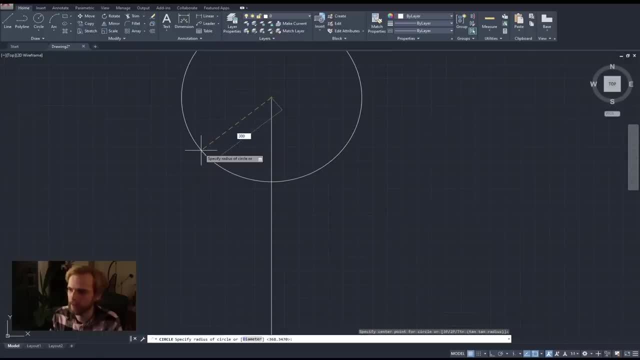 yeah, let's say 300 millimeters and hit enter. so now I have my line tool, or my circle, directly centered around the end point of the line. I can do this again: c, enter from here, 300, enter right. so I have my two circles. that's the first thing that you can snap to. another thing that you can: 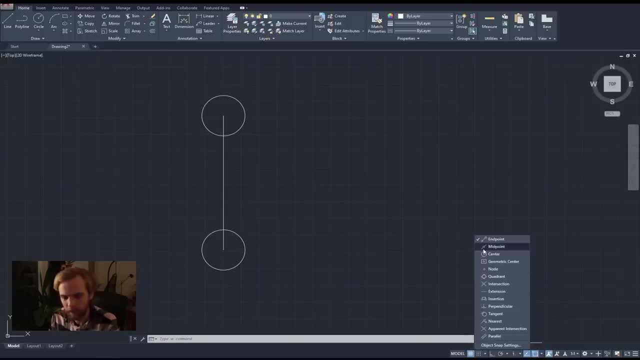 snap to. is this the midpoint, right? so let me enable that. enable midpoint again. I'll get the circle. I'll start drawing the circle, or rather I'll hover my mouse over the where I imagine the midpoint of the line is going to be, which is right here. I'll click and start drawing right. 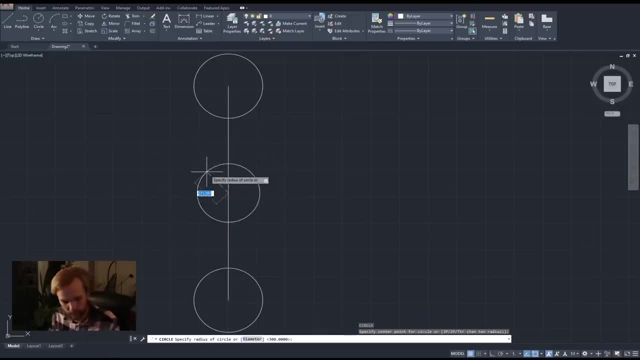 so you can see that it even gives me the mark. let me do that again as I'm hovering. it even gives me the triangular mark here and says midpoint right. I'll draw, drag, draw it out and I'll say 500 for the radius right. so this circle is located directly in the middle. 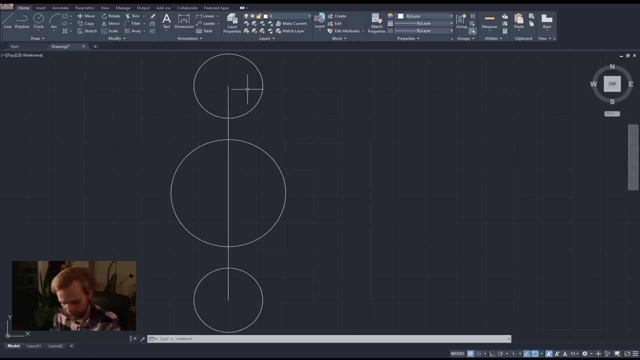 of this line, a circle, at least to my knowledge. yes, the circle doesn't have neither a start or end point, or it doesn't have a midpoint as well, because it's infinite in the middle of the line. so I'm going to draw a circle and I'm going to 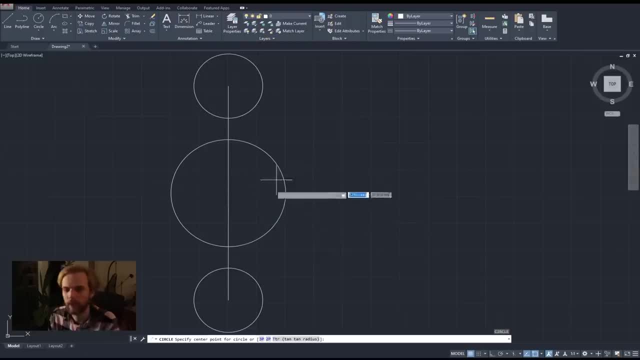 drag the center in this circle under the line. so now let's go over the depth of this or this rectangle, as we went over, as shown, and I'm gonna divide it by this length. right, so I'm gonna, I'm gonna create another circle here from here, okay, and I'm going to change it a little bit. 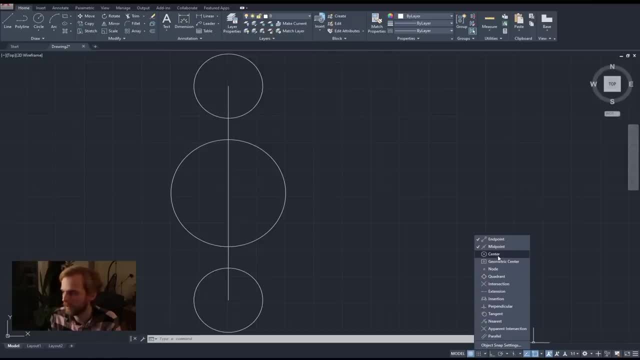 because it only makes sense to split it from the solar head, from this circle, or I won't have the right number. I'm gonna are going to stick this here, so at this point I don't want to save myself after this, so I'm going to change it to look like this: now I'm happy. 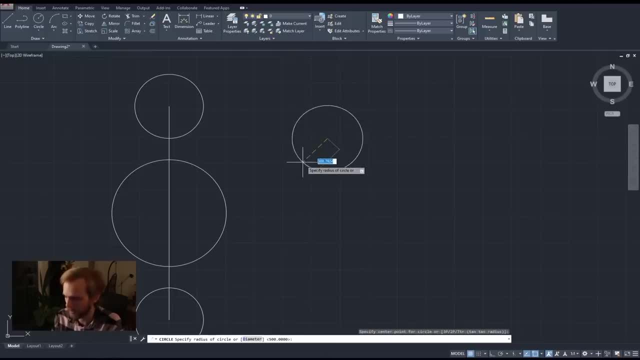 just finished' yeah good, so circle, and i'll just give it 500 millimeters again, right, and i will enable center snapping here. i'll draw- let's just draw- another circle inside of this circle, right? so i'll choose a circle tool again and now, as i, as i hover my mouse on the edge of the circle. 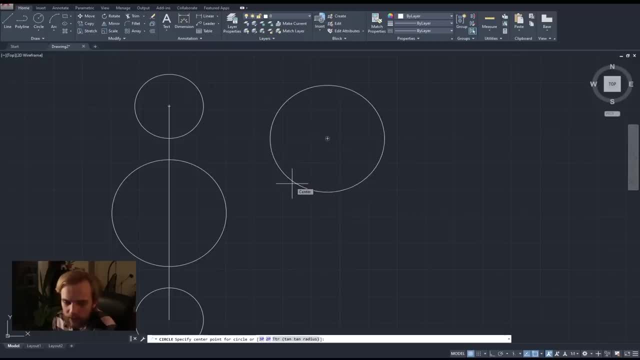 you can see that green uh circle appearing, or green markup appearing, right in the middle right. if i click, my next circle is going to be drawn in the middle of the previous one, right, so i can give it 300 millimeters, for instance, and i can keep doing that, right i? 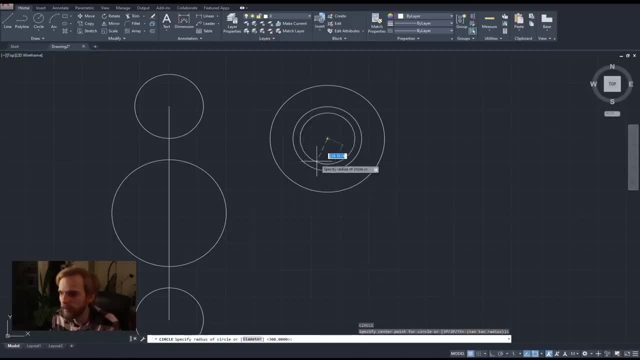 can keep hitting enter to repeat the last command and i can keep drawing drawing it out like so okay, that's one thing, um, next up we have geometric center. so geometric center is different from a center point in the sense that, um, i believe if you have a rectangle, 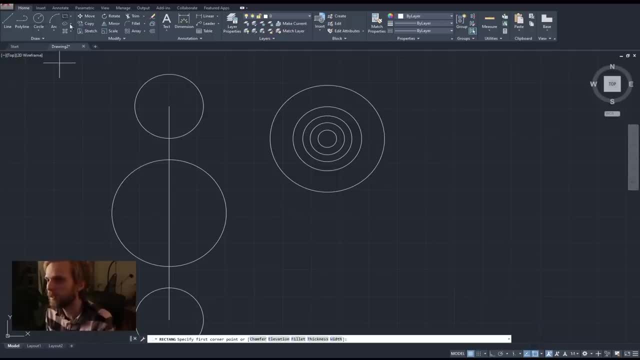 let me just check. i don't want to lie. okay, if you have a, if you just use the center snapping, you can see that the center point is right. it doesn't have um, it only works on arcs and it only works on circles. it doesn't work on closed shapes. so if you have some sort of 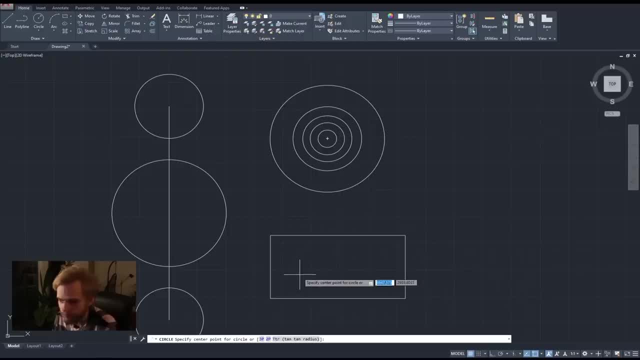 a closed shape, such as a rectangle, then geometric snapping is going to be the way to go, right, so i'll turn on geometric center or geometric center snapping, sorry, is going to be the way to go. i'll turn on geometric center and as i am moving along, this, this, this rectangle you can see 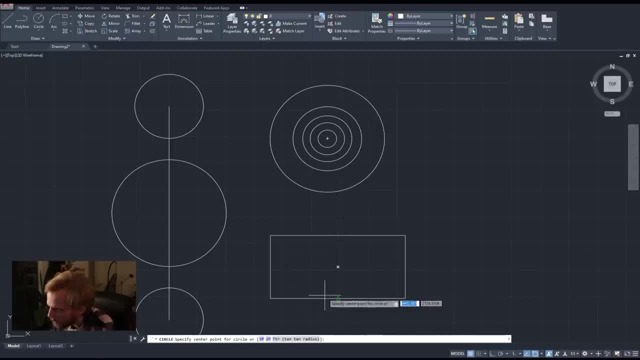 that the middle. while it gives me that snowflake thingy, it doesn't give me a green, green icon, meaning that i can't snap to it. but if now i hover my mouse close to that snowflake, now i'm able, now i'm able to snap, right, i'll repeat it again, hovering my mouse, finding that until i see that. 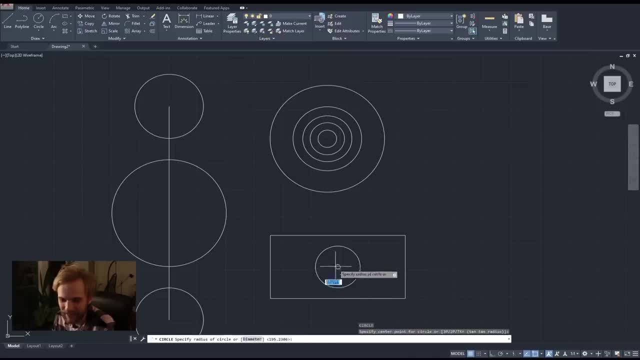 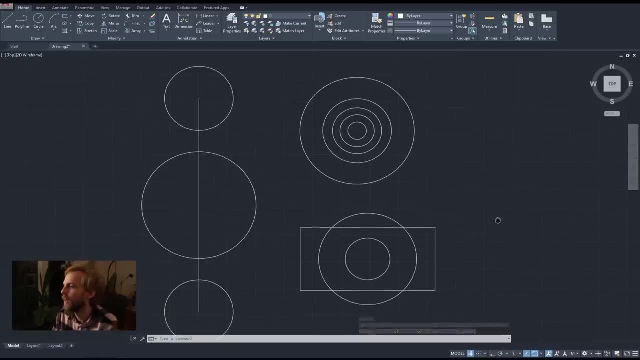 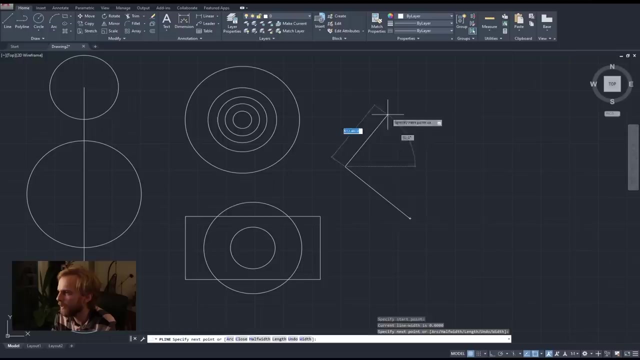 that snowflake appear, clicking on it and dragging out like that: okay, so that's done. um, so that's geometric center. uh, there's more stuff that you can do, for instance, if you have a polo line which makes a weird uh form, something like that, and as long as that polo line is closed, meaning. 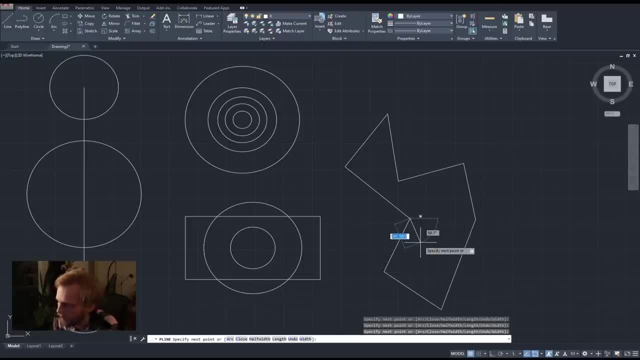 it needs to end where it started, click and then hit enter- right it's. it's a closed polo line right now and i grab a circle. it will show me where the geometric centroid is right and i can't snap to it, but it's of course going to be funky. it is accurate mathematically, it is. 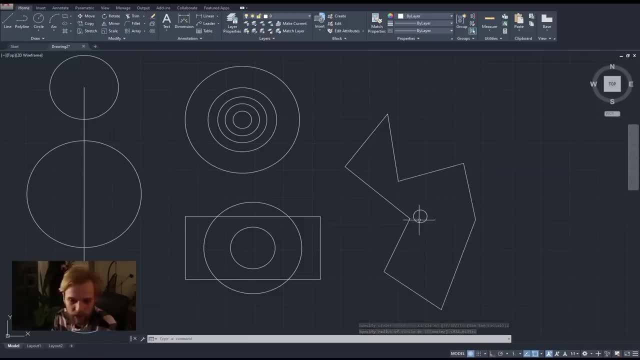 an accurate geometric centroid of this particular shape. but it might be counterintuitive for you visually right seeing it there. the way it's calculated is basically: it's an average of all of the corners, the average coordinate of all of the corners of this polo line, just for for the 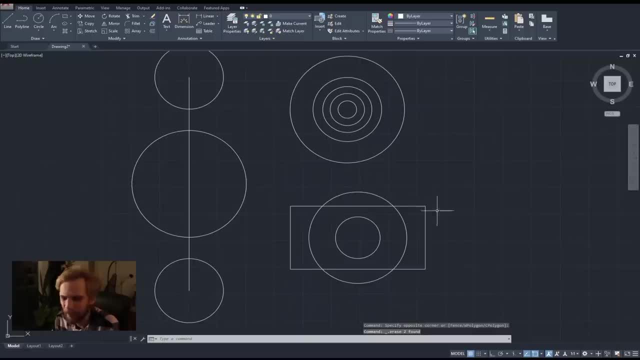 geeks out there who want to know how it works. okay, so that's that. um, then we have node snapping, which i don't care, uh, never use it. it's basically: if you have points in in your, uh, in your drawing, we will not be using points, so we don't care. uh, i will not be even showing you this quadrant snapping. 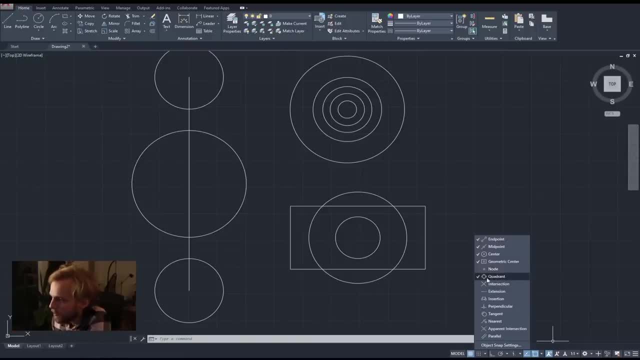 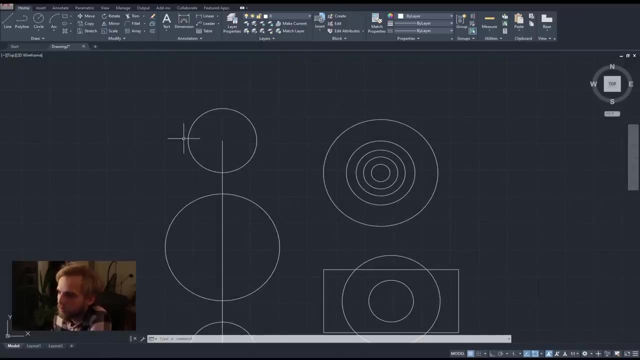 though, is quite useful. uh, if i select it, i tick mark that now, every circle that i drew has a quadrant right, it has a quadrant here, here, here and here. i can actually show them by choosing a circle, or rather on this one, and i can see that now i can. 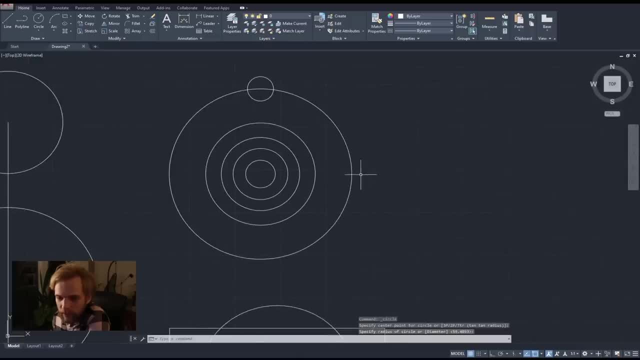 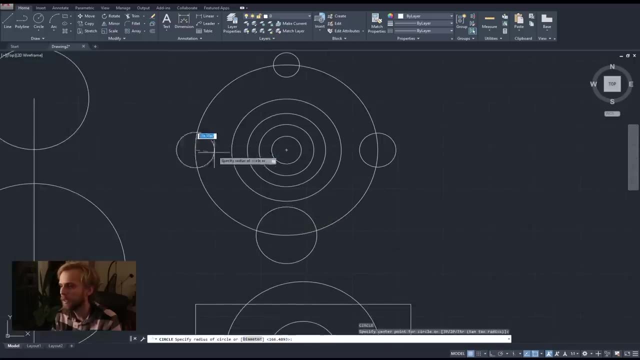 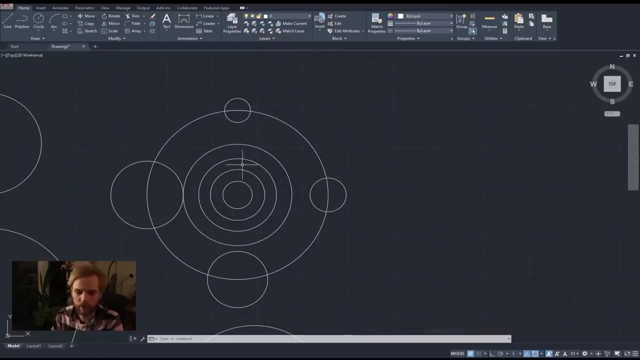 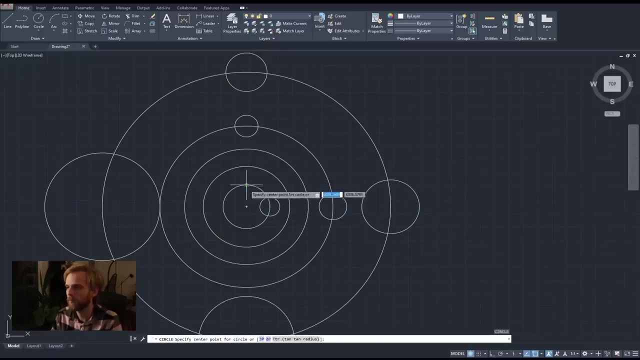 snap to this spot here, i can snap to this spot here, this spot here and this spot here. right, so i can. i can snap to four points on each of the circles. quite useful in in some cases, but it's very useful in some cases, and you can kind of go even deeper and then kind of keep. 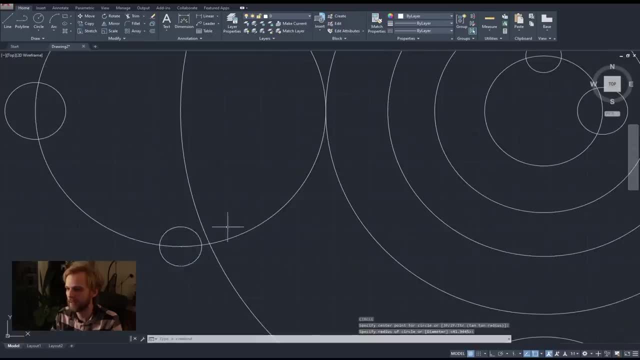 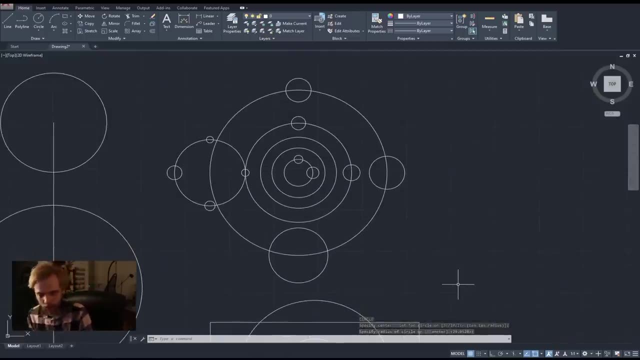 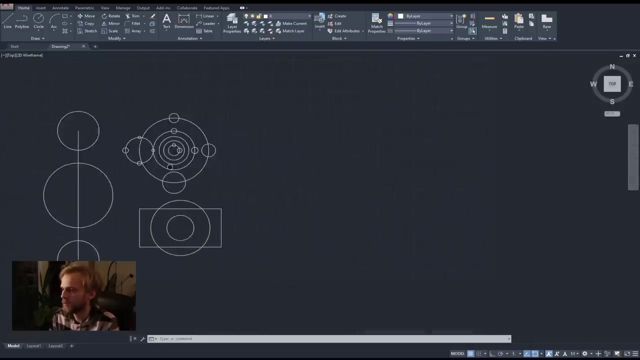 keep snapping to those, to those quadrants, to create pretty, pretty intense graphics. um, right, so that's quadrant snapping next up. we have intersection. so a very simple, simple explanation would be: if i have a line tool, you know, I just draw a line here and I draw another one here, right, Let me actually draw. 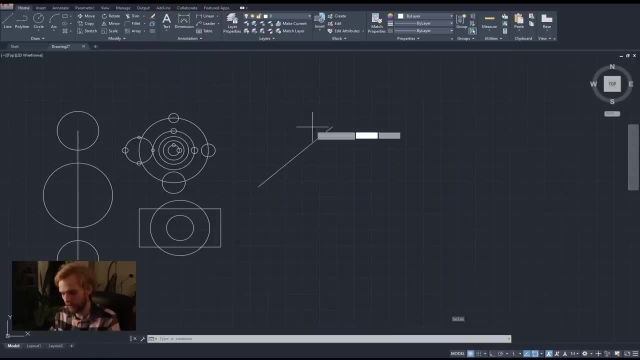 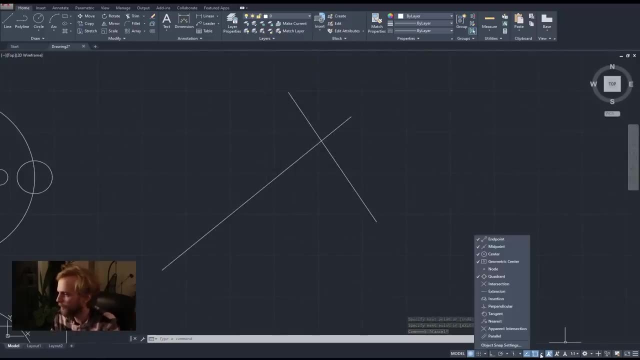 another one. Come on, I'll enter another one right here. If I want to snap to that particular point, I can by using the intersection snap right, So it kind of finds all of the places where two geometries intersect. right, So I can draw a circle around that intersection now. 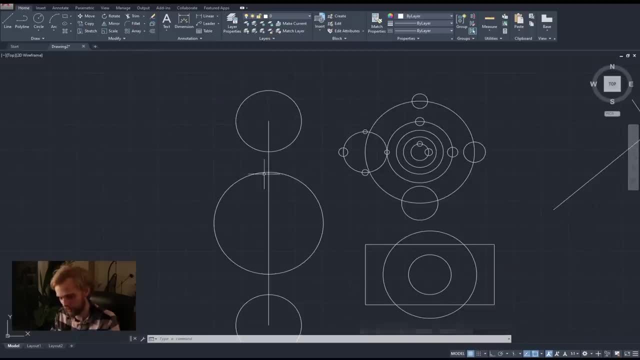 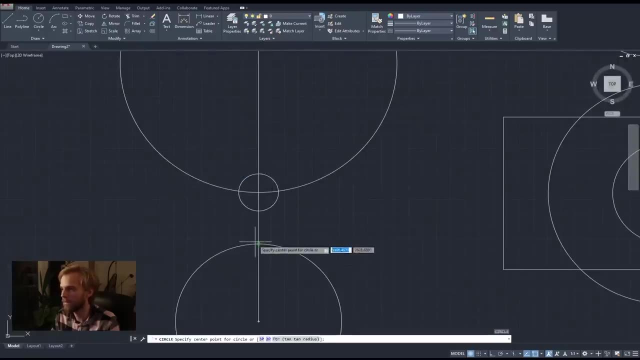 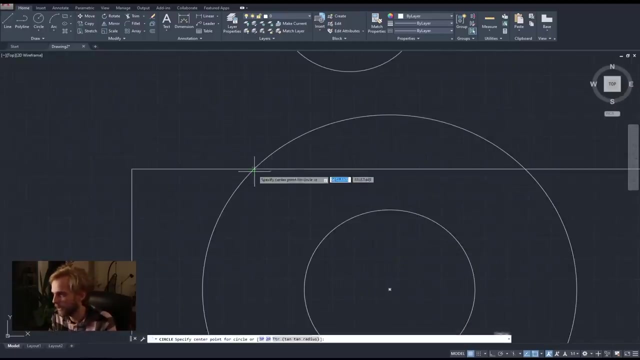 Quite useful In this case. you might kind of be using it for this, for instance, right And then even smaller right. So that's an intersection. So it just finds intersections between any kind of two geometries, any type of two geometries. 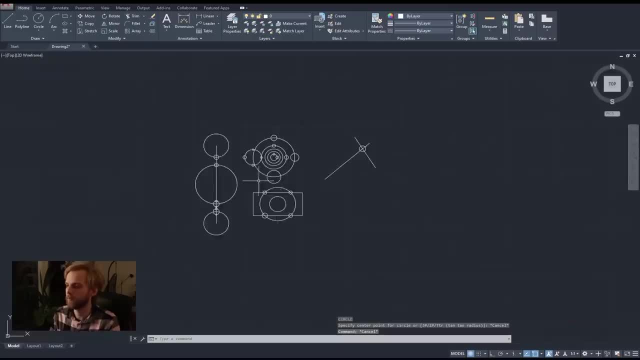 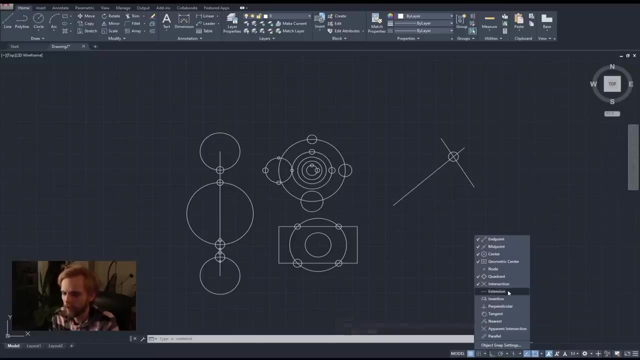 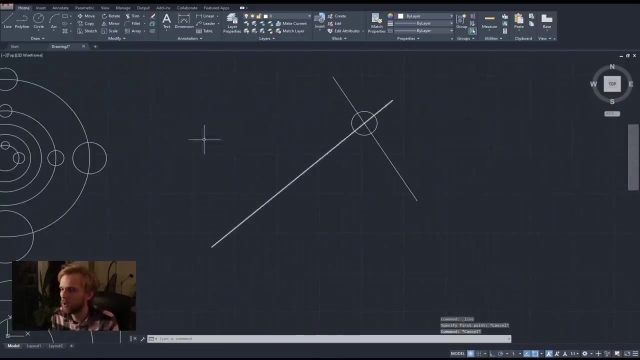 Right. So that's intersection snapping, Next, next, next, There's extension snapping later, not now. Ignore Insertion snapping: no. perpendicular snapping, though, is super useful. Let's say I have a line, or rather, we already have a line I want to draw. 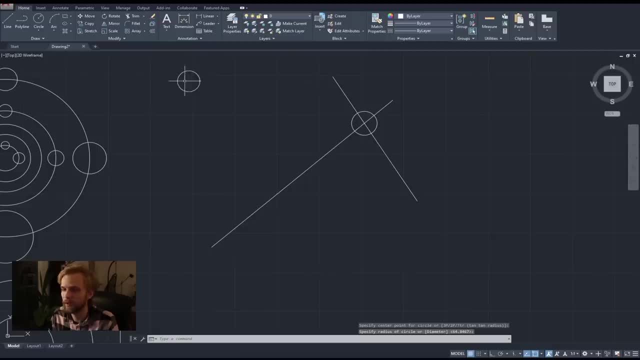 another line from somewhere here, Let's say from the center of this circle. That would go at 90 degrees angle to this line segment, right? So I want to start drawing a line from here, from the middle, and I want it to snap to 90. 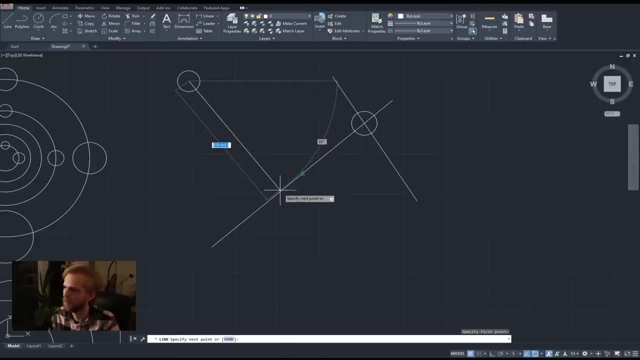 degrees, which is going to be somewhere here, probably somewhere here. I want to snap it at 90 degree angle to this line. So the way I do it is: I enable, I'll escape out of that. Enable perpendicular snapping like this: grab the line tool. 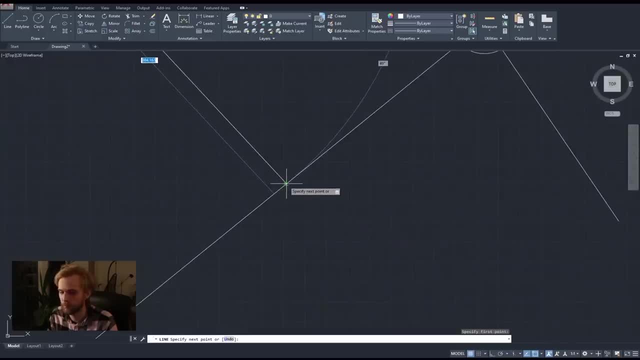 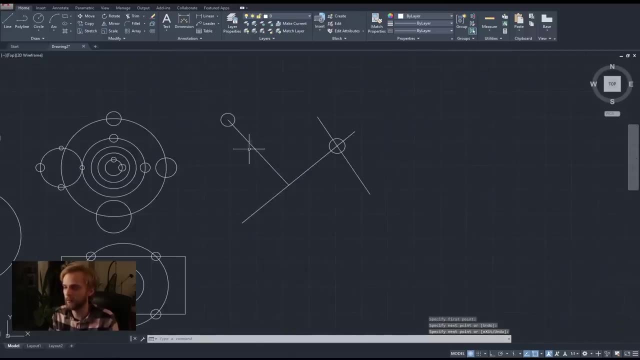 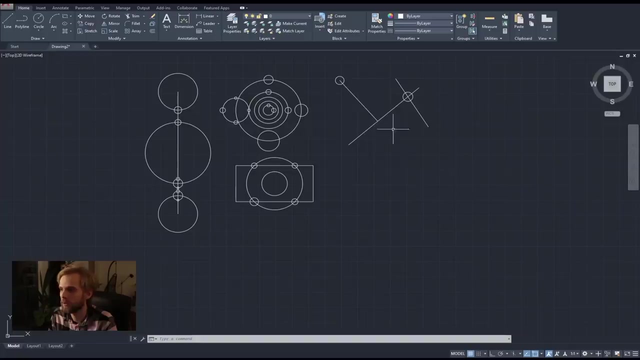 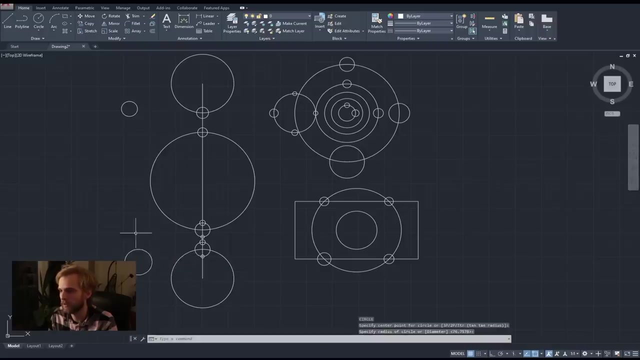 start drawing and then it will give me where the perpendicular snap is. once I click there, hit enter, I can see that between these two lines I have 90 degree angle. really, really useful stuff. if you want to, let me delete that. if you want to, for instance, if you have more circles here and you need to kind of find the 90- 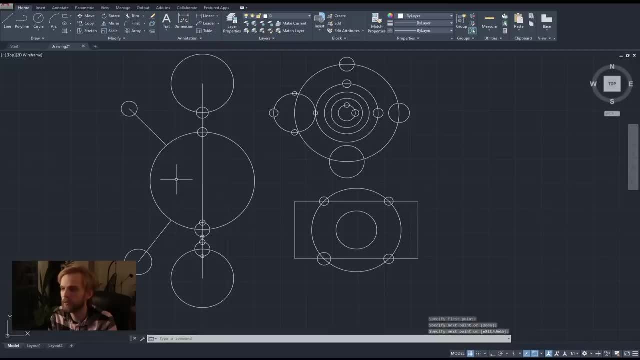 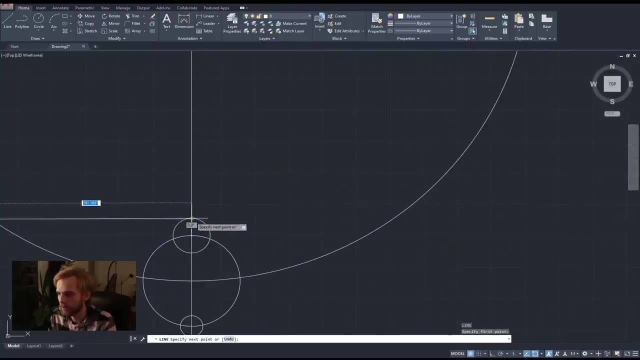 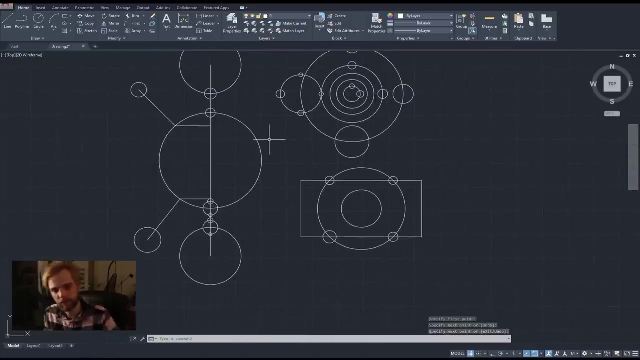 degree snap from these two circles to this circle, for instance. you can always do that and then kind of continue on finding the snaps you. that's a very tight fit. for that I need to zoom in. yeah, right, so that's quite useful. let me get rid of those two lines. 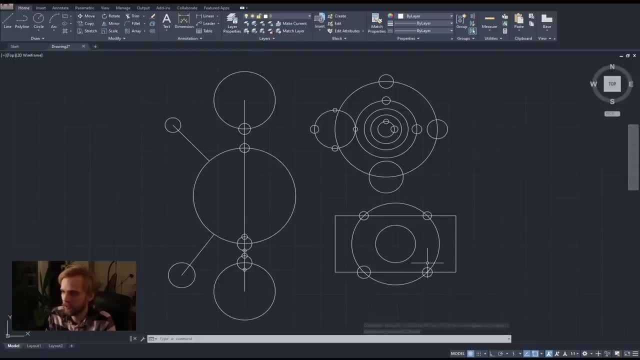 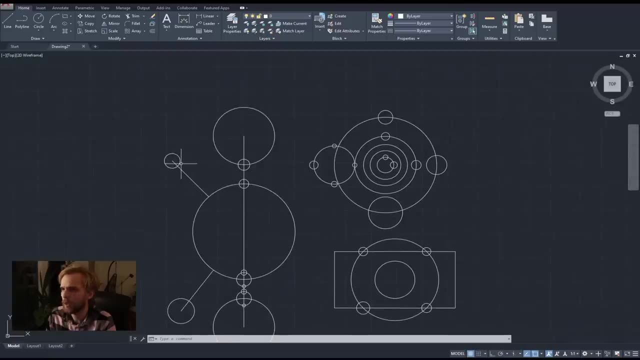 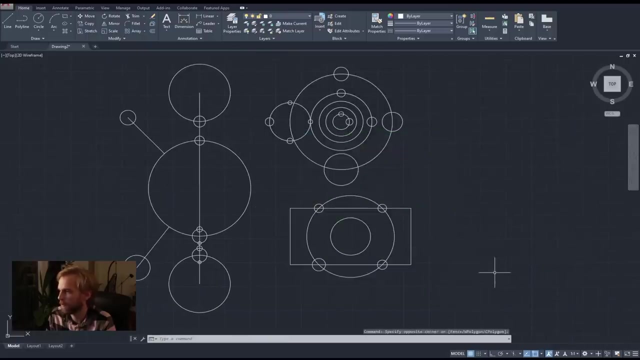 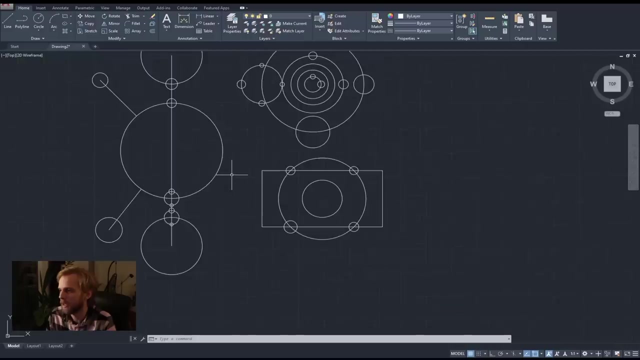 right. so so that's perpendicular, or in other words, 90 degree snapping. then we have tangent snapping. tangent snapping is basically- it's much easier for me to show than it is to actually explain. let's say we have- well, we already have- a circle here, and let's say we want to. 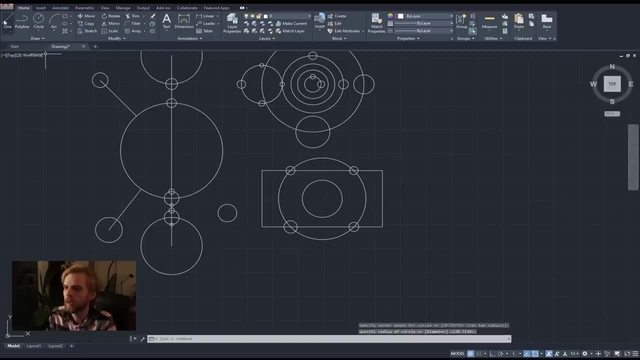 draw. we have one more circle here. we want to draw from the middle of the circle, from here, a line that's going to seamlessly connect to this circle. right here that is called a tangent line, right, and let me make sure that I have it turned on. I. 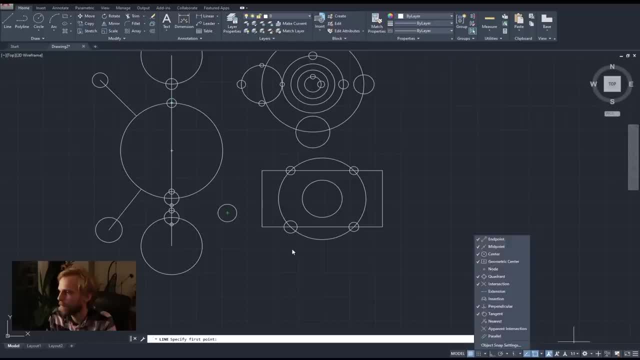 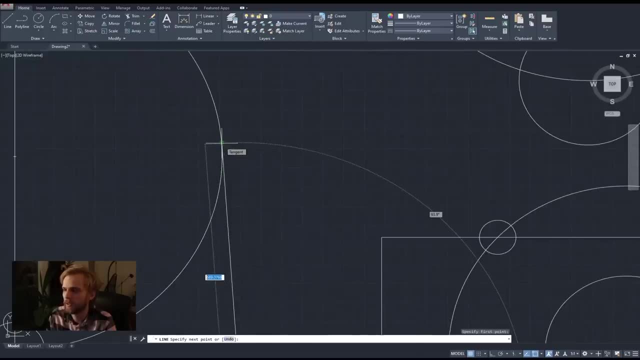 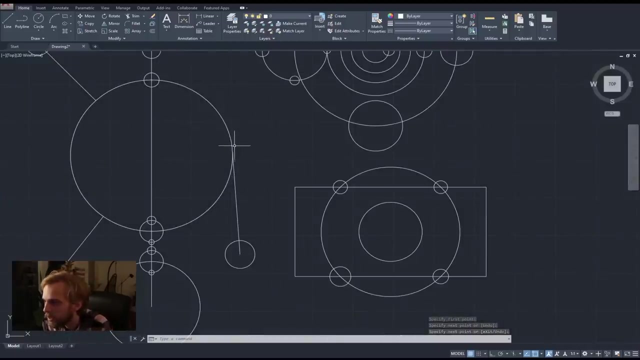 don't tangent. there we go. now we have it turned on and now I can draw from the middle and find this icon here: tangent, click, enter. so now, as the circle is going here, it will seamlessly transition to this line and actually visually explaining it, i think let me do one thing. i will 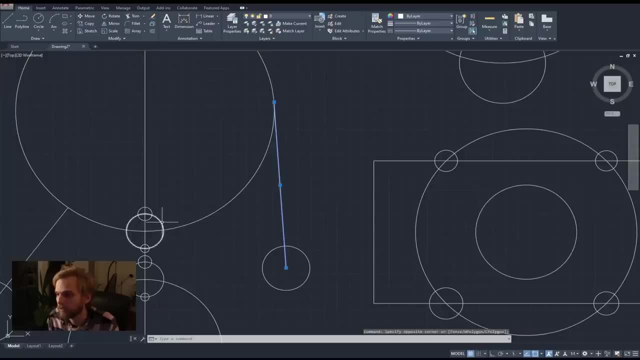 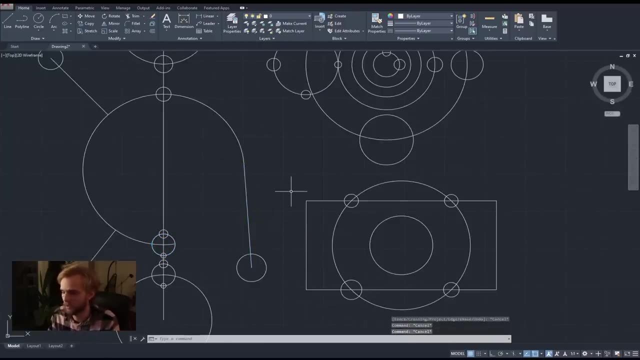 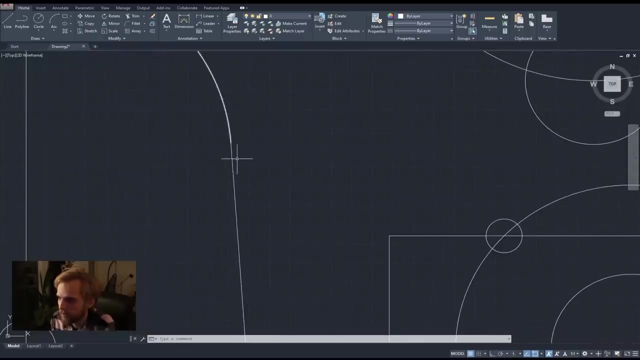 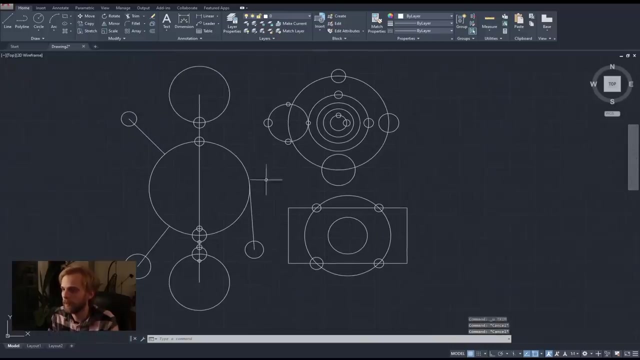 explain that tool in later stages of of this project or of this tutorial. but let me just do do this real, real quick. this line and the way it connects to the arc is now seamless. there there is no sharp corner right, so that's a tangent. let me undo that tensions are quite, uh, quite useful. 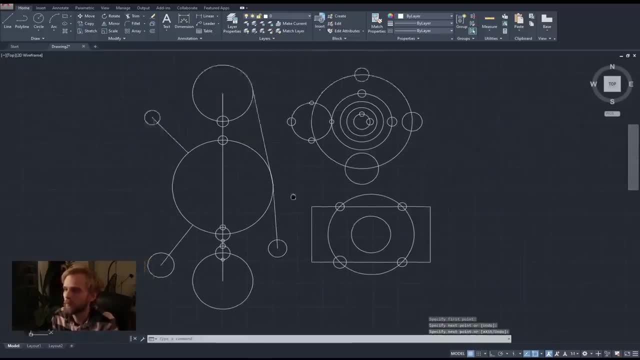 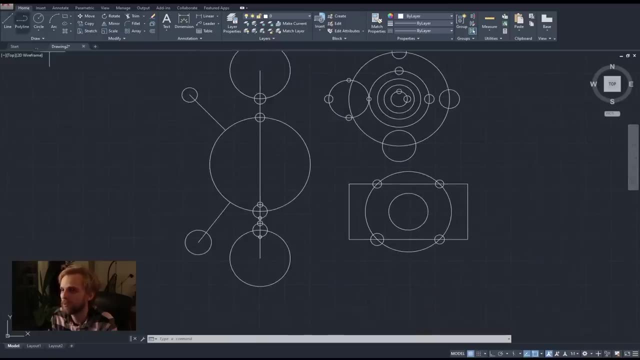 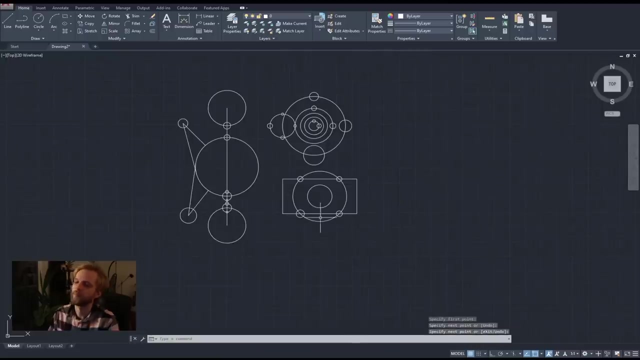 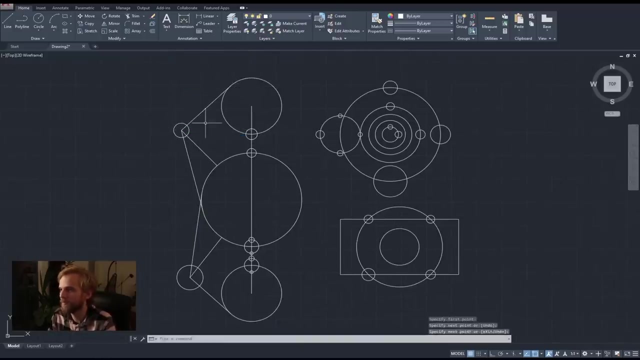 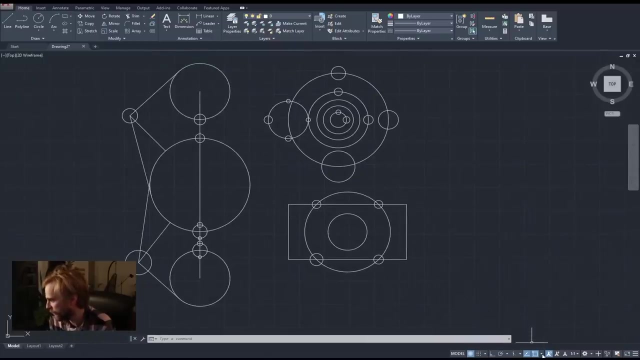 in that regard. um, right, i don't know what i'm, what i'm drawing here, something, something weird, something weird for sure. so we have tangents, right, maybe one goes here. maybe one goes here, sure, why not? um, next, next, next, next, next, next nearest snap, oh, and that's actually going to be. 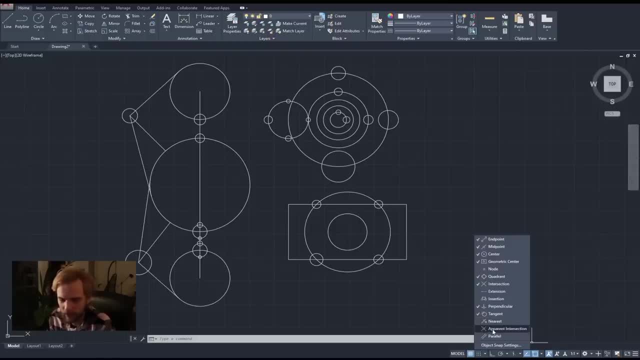 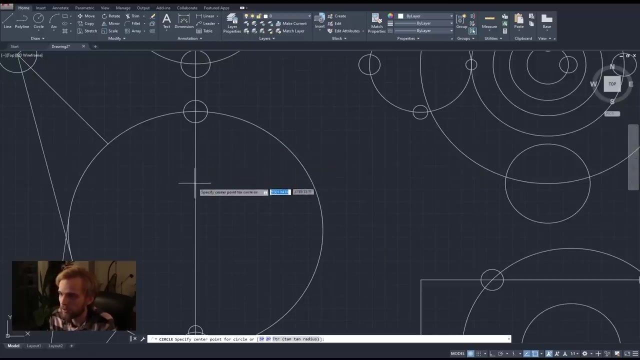 the last one because apparent intersection. i don't like that kind of snapping, i prefer a different work method. uh, so i'll do that next, so i'll not be showing that. nearest snapping is quite, quite useful once you have it turned on and you want to create a circle just somewhere on this line, it will constantly give you. 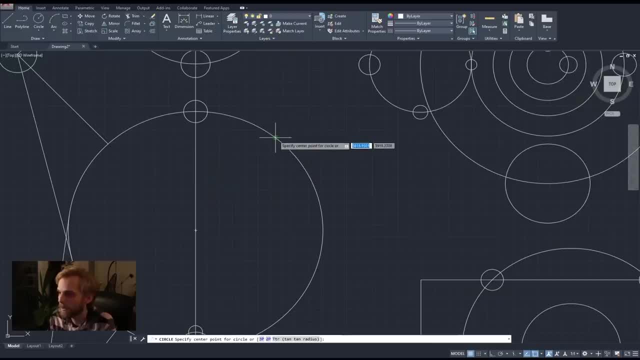 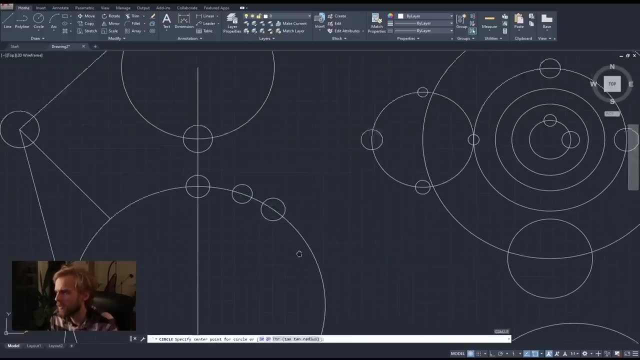 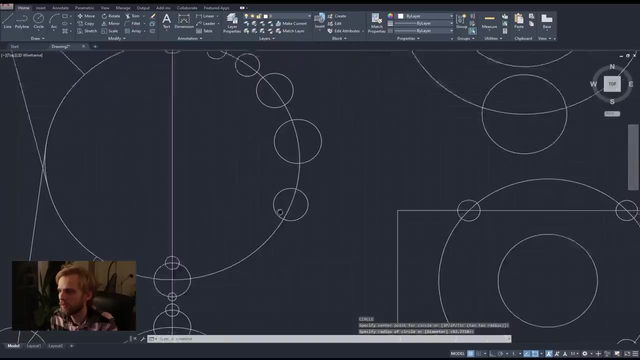 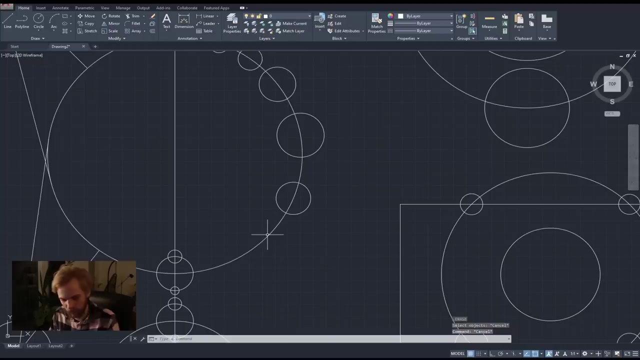 the nearest point to that line, right, or nearest point here, right, or nearest point here, right, so you can kind of just create a bunch, a bunch of of circles on on another. well, if, if you actually don't, don't, if you don't miss it, um c enter a bunch of circles. 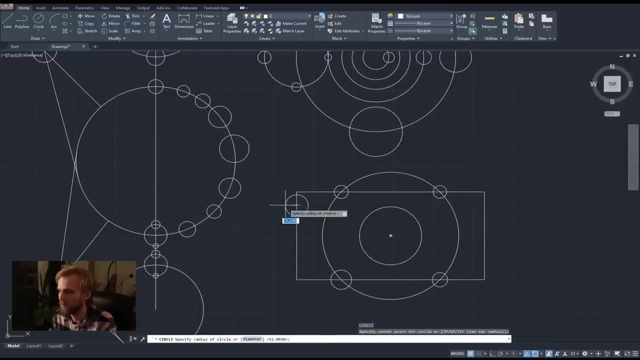 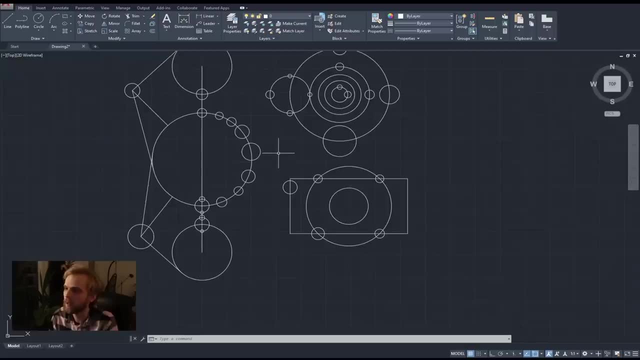 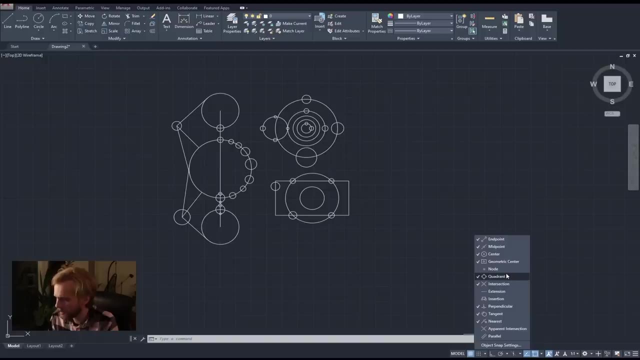 on already existing geometry, right? so that's actually: any point that is closest will be fetched by the nearest snapping. um, that's about it. that's about it in. in terms of snapping tools, um, the key point is to make sure that you have a circle on the right side of the circle, and that's. 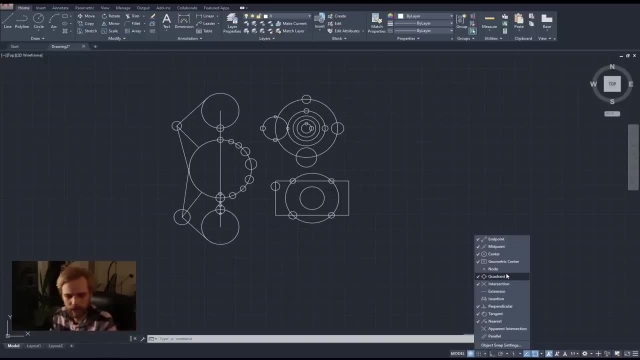 the key point is to make sure that you have a circle on the left side of the circle, on the right side of the circle. thing is, you don't want to have all of the snapping tools enabled because it gets too convoluted. it tries to suggest too many ways of how you can snap to. 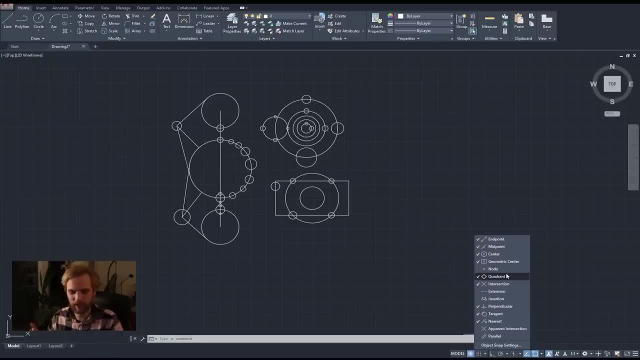 geometry and it it becomes a little bit tricky, a little bit bothersome to work around, work around that. so usually what I like to do is I like to turn off tangent snapping, I like to turn on off, sorry, intersection, quadrant snapping, geometric, center and center, and I just leave end point, midpoint, perpendicular. 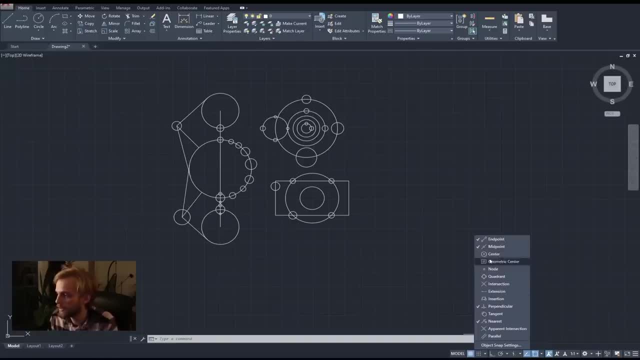 and nearest snapping. those are the mostly used ones. if I need some other snapping method, I will enable it just for that particular tool. a shortcut of how to turn on or off object snapping is f3 button. f3, yeah, usually, I just always have it turned on. 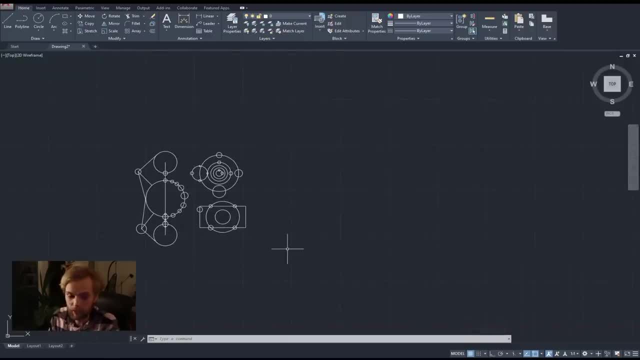 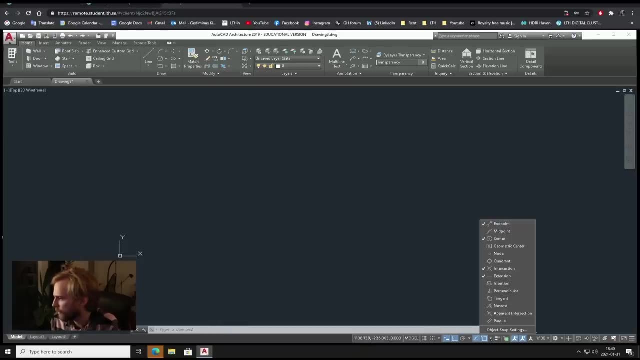 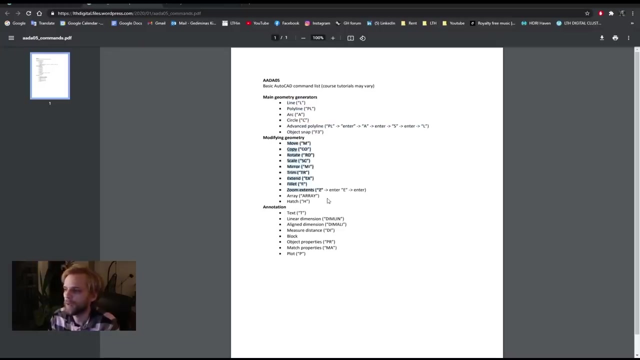 Oh, beautiful graphics that we've made here, right, so that is snapping. right and that is snapping. let's take a look: if everything is all right here, that's the same thing here in this workspace as well. good, very good, right. so next up, we have the different ways of how you can modify geometry. right, so you can move it, you. 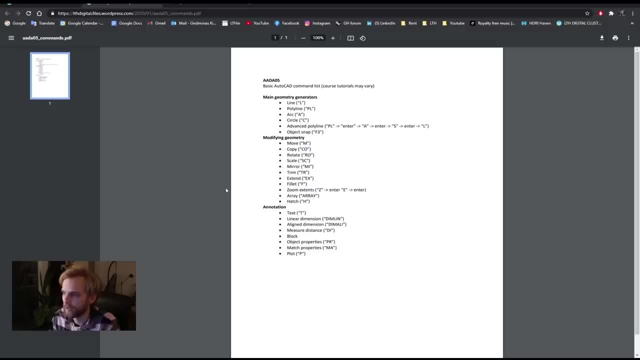 can copy it, you can rotate, scale it: you can move it, you can rotate it, you can rotate, scale it, you can move it, you can rotate, scale it, you can move it. you can scale it, mirror it, trim it, extend it. blah, blah, blah. let's go through them. 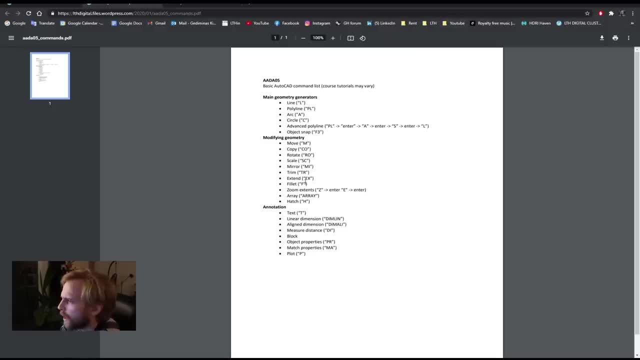 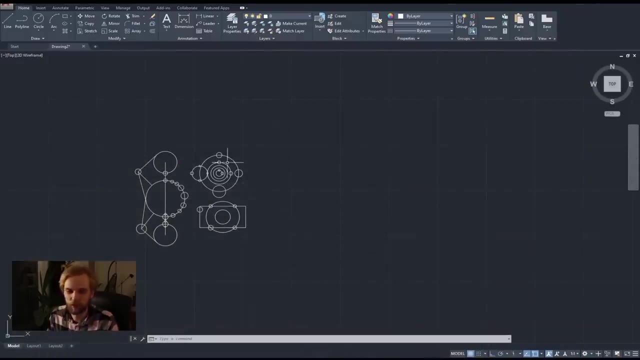 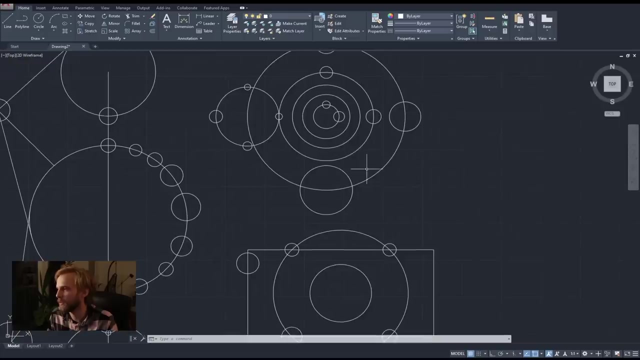 let's go through them and once we are- yeah, once we are- done with this, then we will start drawing our house a little little by little, right? so first thing is: move right. that's a pretty simple one. let's say: I want to. I have this geometry here. I don't know which one to choose. I 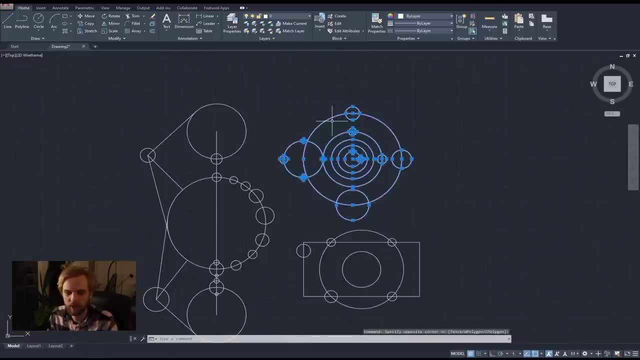 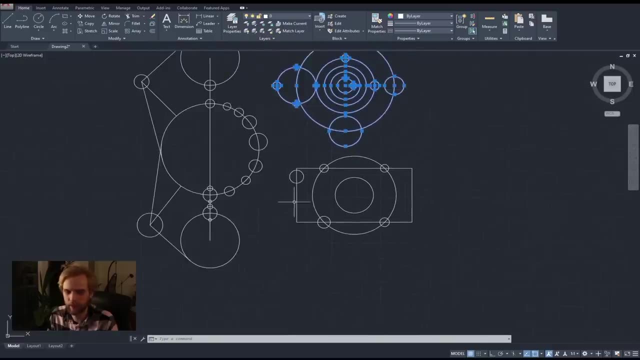 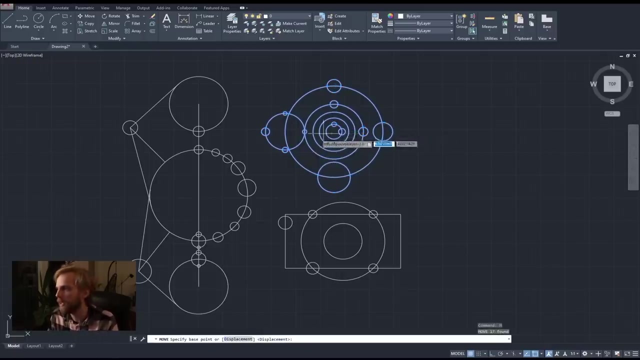 let's say: all of this I have, I want all of this to move away or to move somewhere, maybe to snap to to this point right here. right, I can do that by selecting all of it, typing in M, hitting enter, M short for move, hitting enter, giving it. 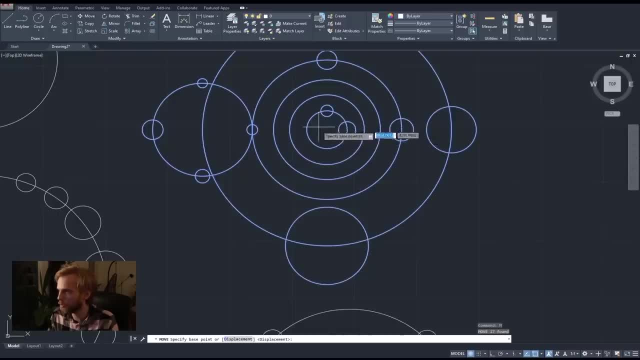 saying the base point, so clicking where I want the base point to be. and I actually want the base point to be in the middle right and I can't select the middle because I turned off the object snapping. so I will actually go in here and turn on center snapping, like here. so now I can select the middle click and I. 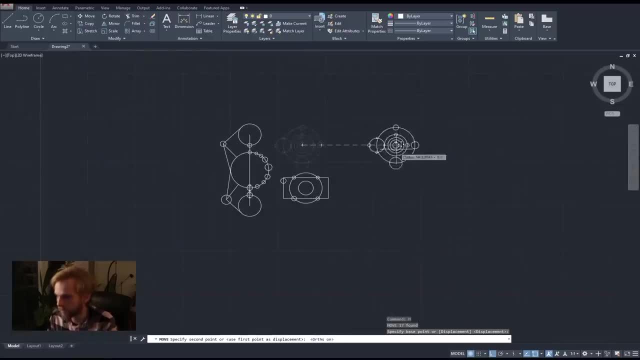 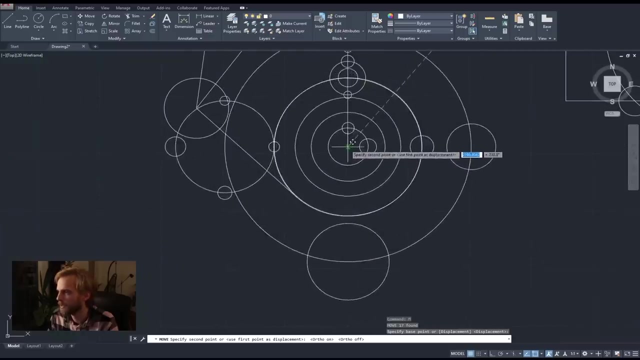 can move it again. if you can only move it horizontally or vertically, then you need to hit f8 or turn off ortho snapping, orthographic snapping. so I can move it now and I will just move it. let's see if to here doesn't matter, or maybe to the midpoint here, yeah sure, to the midpoint. 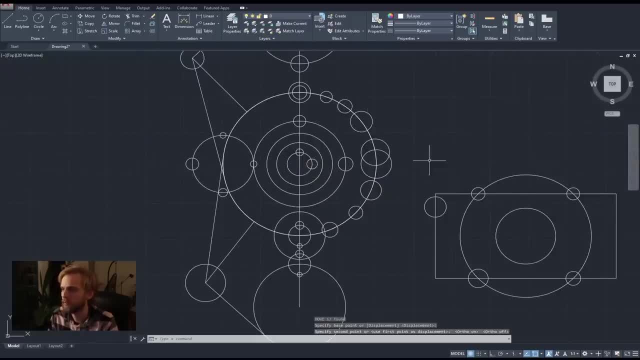 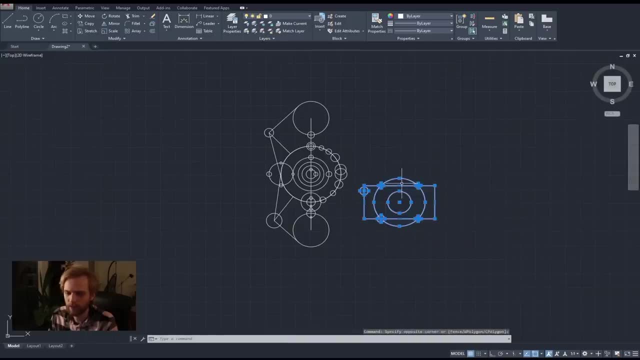 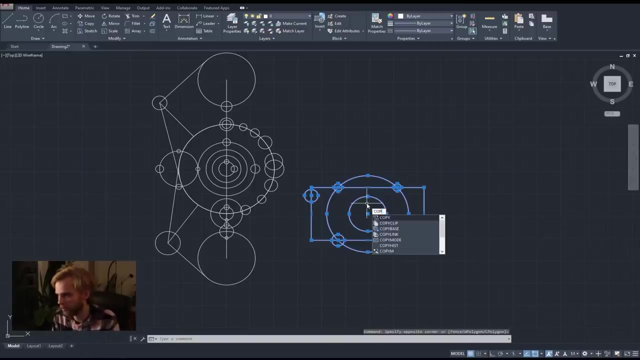 here. I'll just move it to the midpoint here. click again, that's it. it's now located here, right? um, also just like move. there is copy. I can select the geometry. I can type in copy: Co P. I think: yeah, see, oh, okay, see, oh is enough, but I use Co P for some reason. 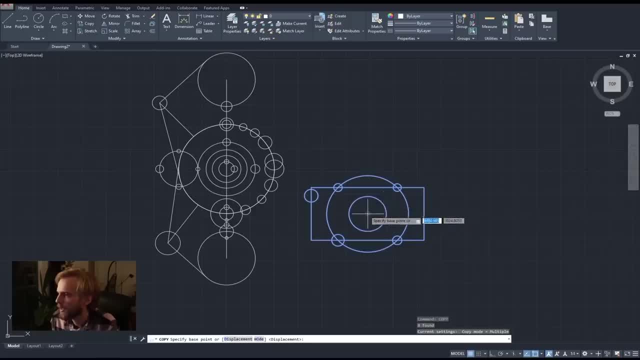 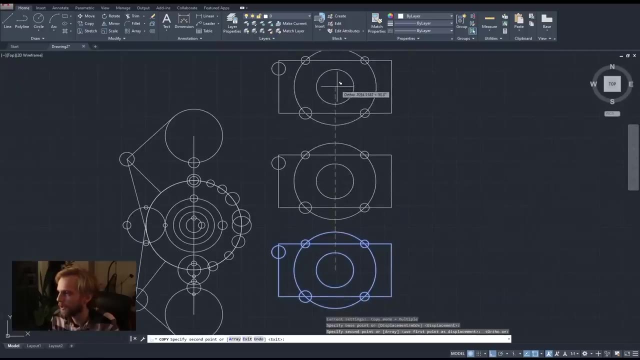 see you enter again from the midpoint. let's say two. for now I'll just kind of make a few copies horizontally, so I'll just hit F, or vertically, I'll just hit f8, click, click. if you want to copy or move something by a fixed amount, then instead. 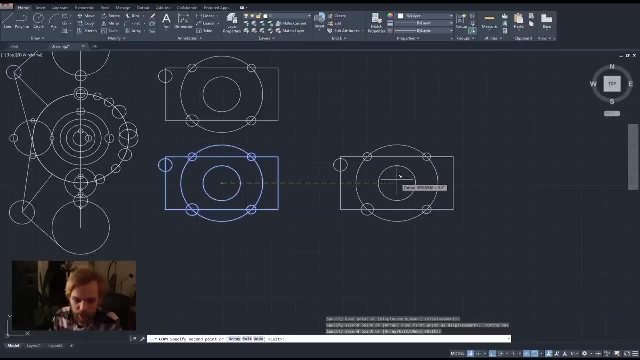 of just clicking. you first describe the direction- let's see, it's my horizontal direction towards here- and then you type in by how much. so I will just say by 500 millimeters enter. well, that's not a lot, but you get the idea right. so the initial geometry was copied to the side. 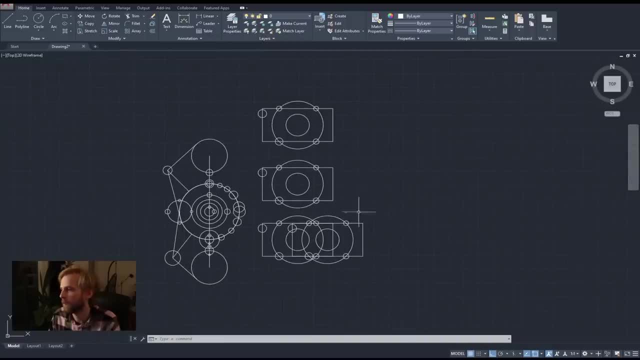 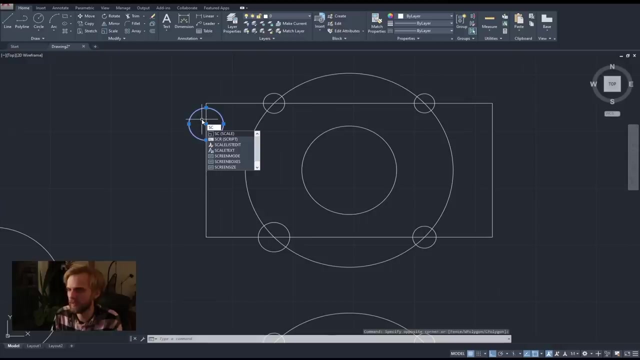 by 500 millimeters. okay, that's move and copy. then we have scale. scale is basically just changing the size of the object. you can either scale a single object, select one scale type in scale or SC, or for scale, enter and then select the point around which you're going to scale. 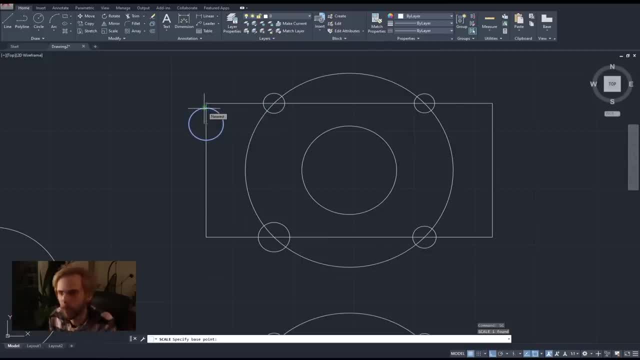 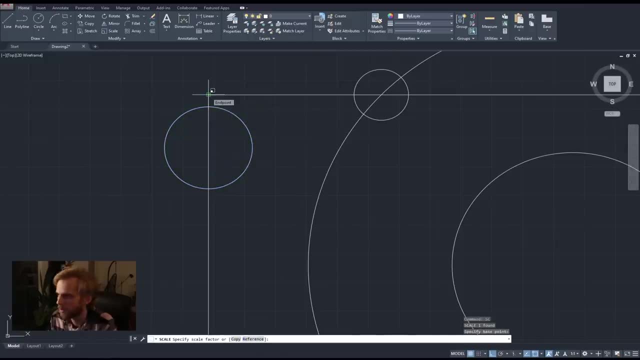 the object from which you're going to enlarge or shrink the object. so let's say it's going to be this corner point right here or the middle of the circle, doesn't matter, this corner point right here. I'll just say that the scale needs to be. 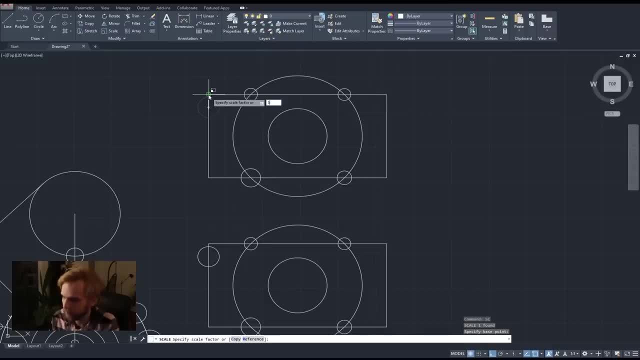 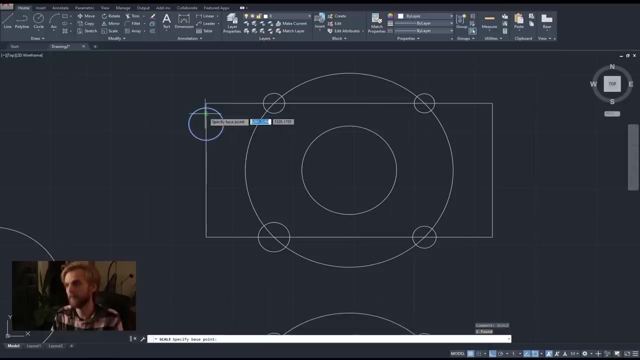 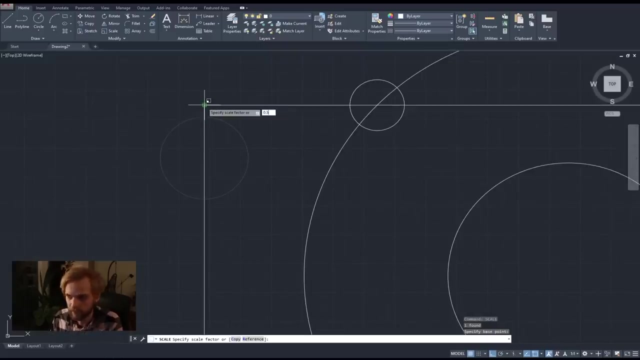 five, right. five is five hundred percent, five times larger, right. so this guy becomes five times larger. I'll ctrl Z to undo, I'll select it again and I'll scale again around the same point, but this time around I'm going to say 0.5, that is. 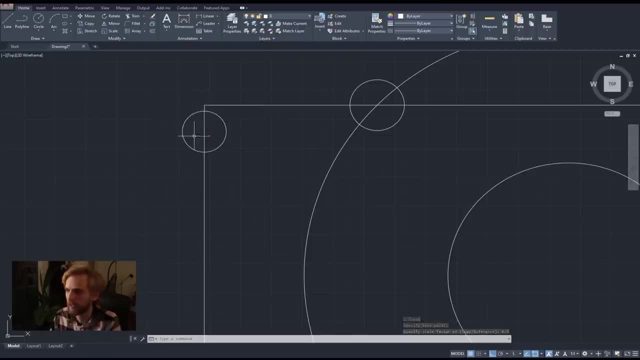 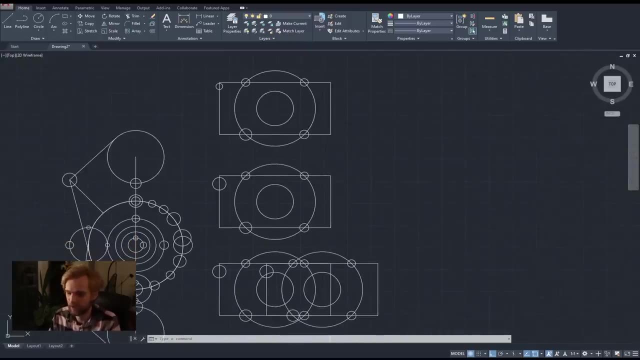 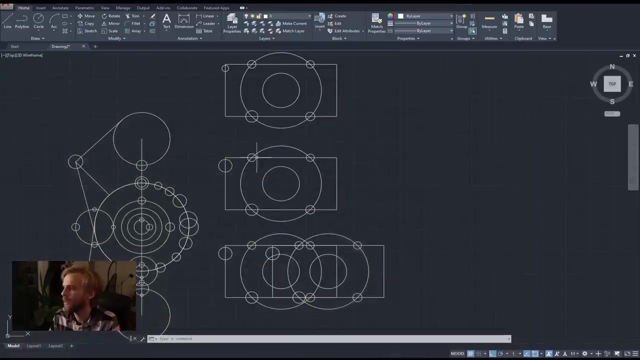 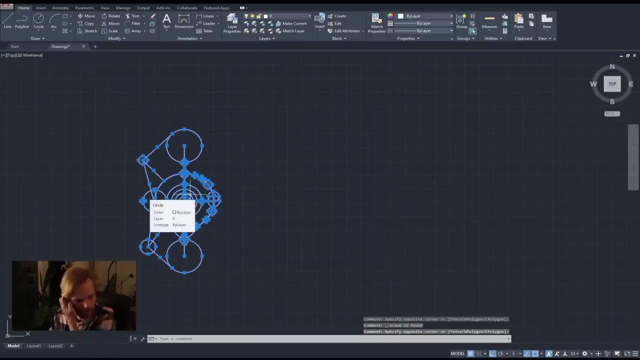 50%, not 500. that is half of the size, right? so it gets shrunken down. that's scaling nothing. nothing fancy about it. then we have a- I believe, mirror, right, yes, we have mirroring, so mirror is quite cool. let me get rid of this. let's say you already have this geometry done, or not done, but 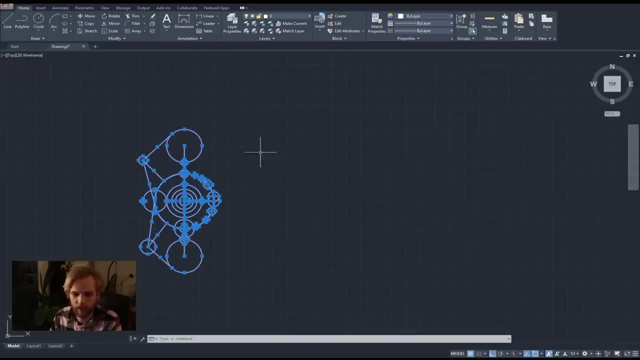 you have some sort of geometry and you want to mirror it to the other side. usually you do that with doors and whatnot. but let's just say you want to mirror it. I can select all of it and type in: mi hit, enter, mi short for mirror. 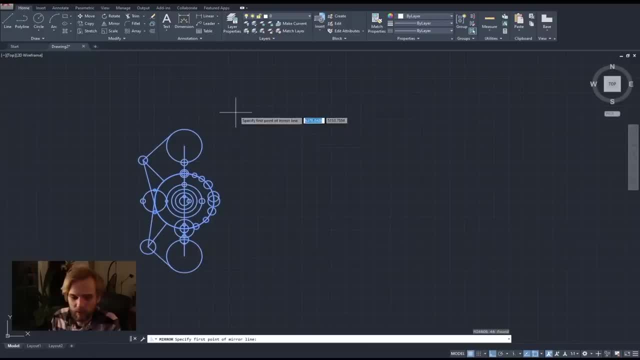 hit enter and then it's going to give me an ask me to draw a mirror line. so it's basically going to be like the line around which it's going to mirror. it's much easier to show than to then to kind of talk about it. so that's my mirror line. let me hit f8 to turn it off and 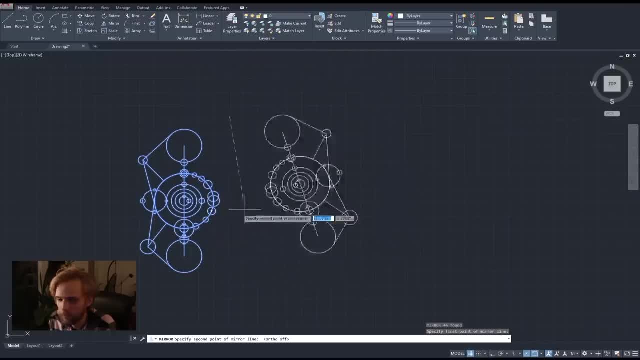 now it's. I think it's even easier to see what's going on, right? so now I can mirror this quite useful right? that's my mirroring and I can do this this way. oh yeah, and once you're finished mirroring, it's going to ask you would. 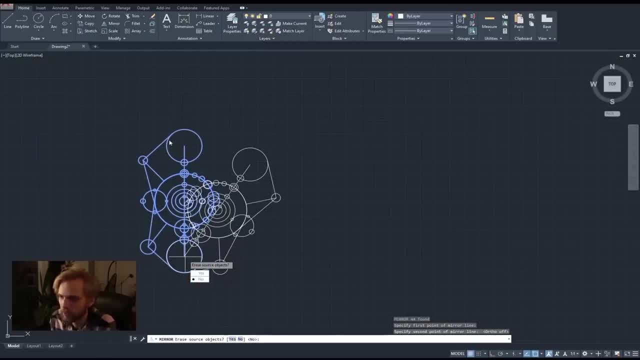 you like to erase source objects or no? so would you like to delete the initial one or would you like to keep it? I will say: don't erase, let's keep it. so, no, so we have mirrored this right and I can kind of do it again: mirror, let's say, between: 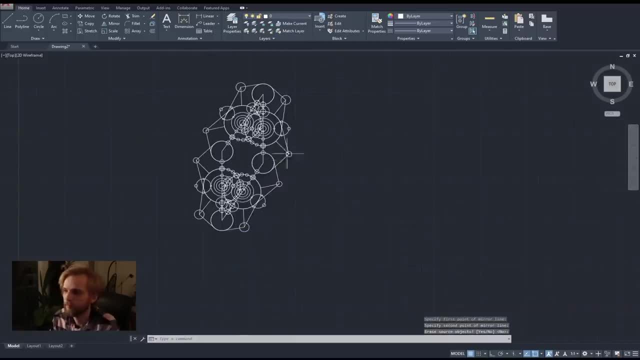 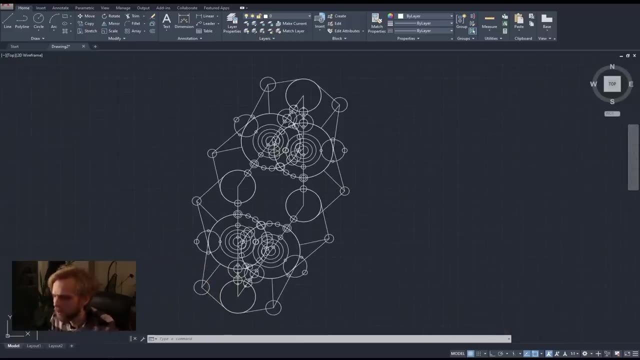 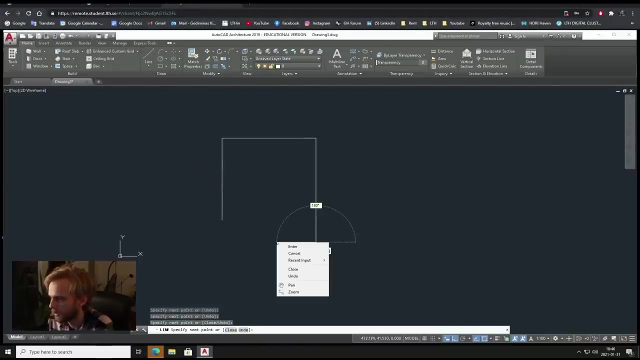 these two points like that enter right now. I have this kind of geometry going on. um, let me just double-check here. whatever any kind of geometry, I select all of it mirror here. well, in case of here, it doesn't ask you right next to the cursor, but it asks you. 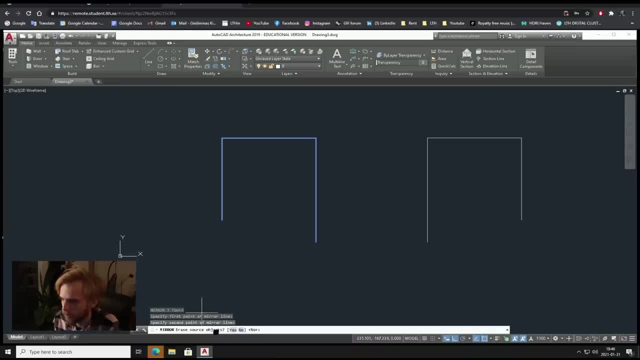 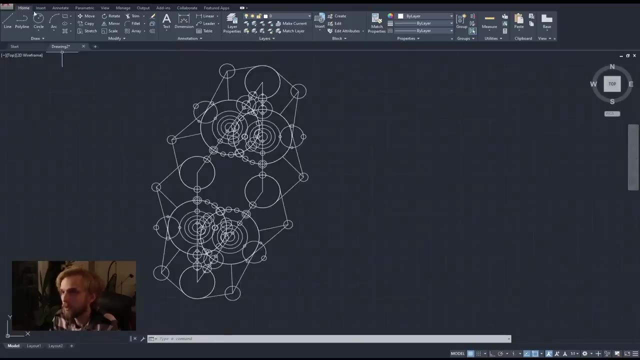 um, here in the in the command line, would you like to erase source objects, yes or no? by default it said to no, so you just hit enter and you know it's done. um, so that works in in in both versions as well. so that's mirroring I really want. 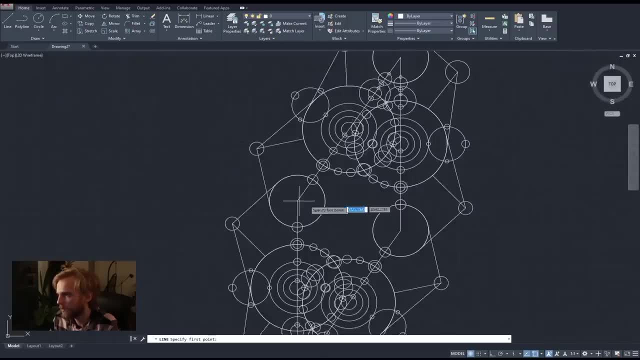 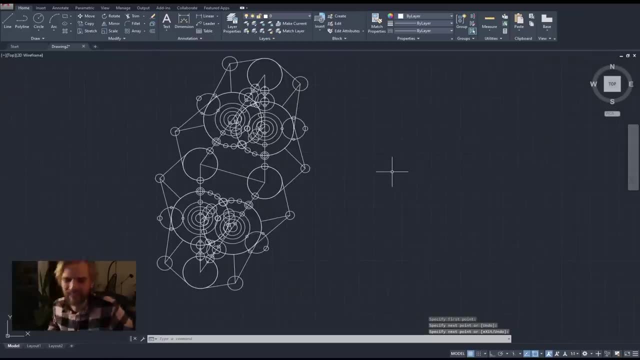 to draw a line here, so I will- um, maybe not from there, maybe from here to here, I don't know. I I just think it's, it's uh, it's gonna look better if we have some some geometry in between, but that's that. that that is basically mirroring next. 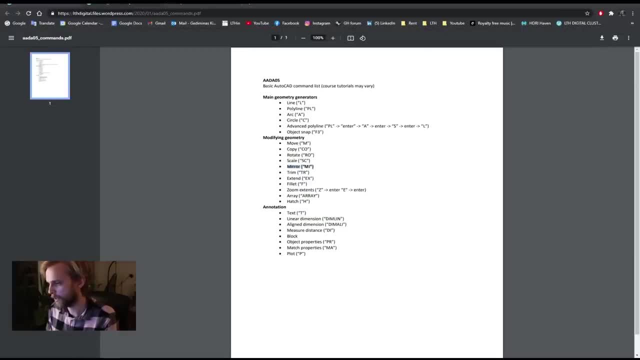 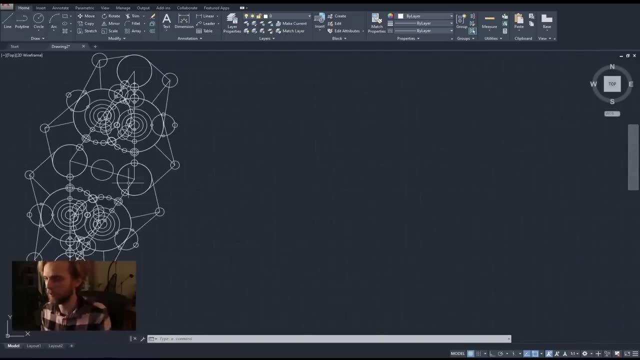 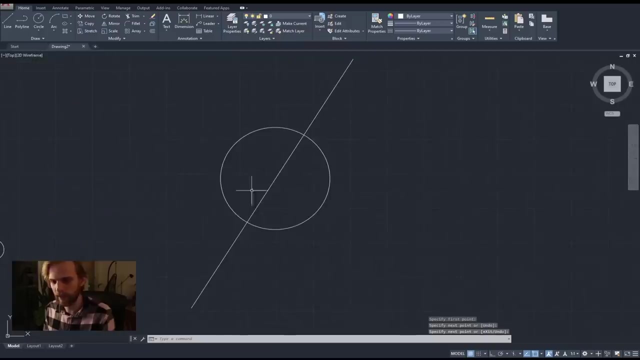 trim, trim and extend. okay, uh, so for trimming, I actually need to show it with a much simpler example, and then we'll go in here and and kind of, I'll show you how to trim stuff in here. uh, so a very simple would be. I have a circle, I have a line right and the line crosses the circle I want. 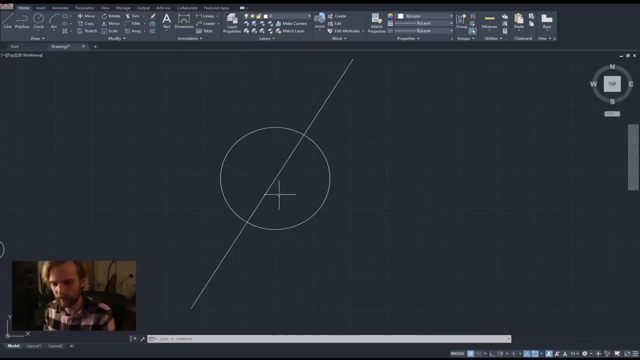 to get rid of this line segment that is inside of the circle, I can type in tr, trim, enter. it's going to tell me to select objects, um, and unfortunately it doesn't say what kind of objects, or select all. so I can just hit enter to say select all, enter right, and it's then just going to say okay, uh what. 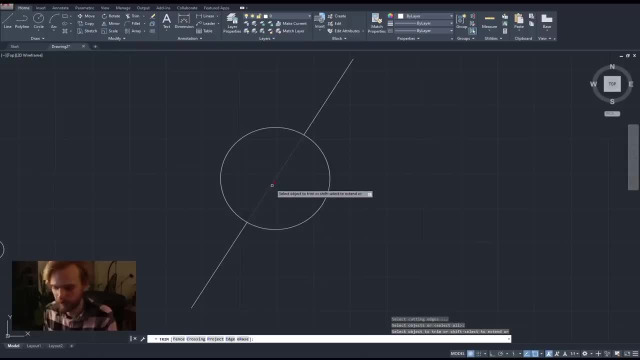 would you like to trim? so I want to trim this right. I just hover my mouse over it and you can see that it's gone. if I click, it's really gone right, so I can trim it away. so what it does, what trimming does? it finds intersections right, intersection moments, and it deletes geometry. 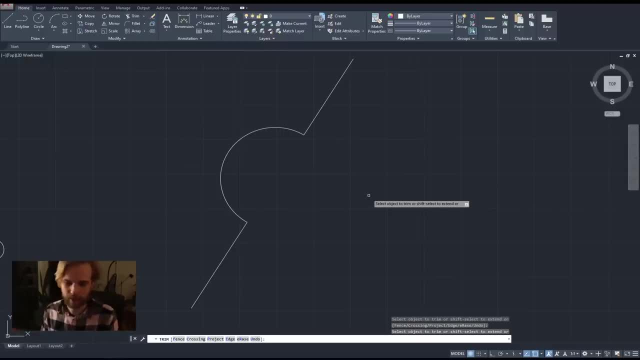 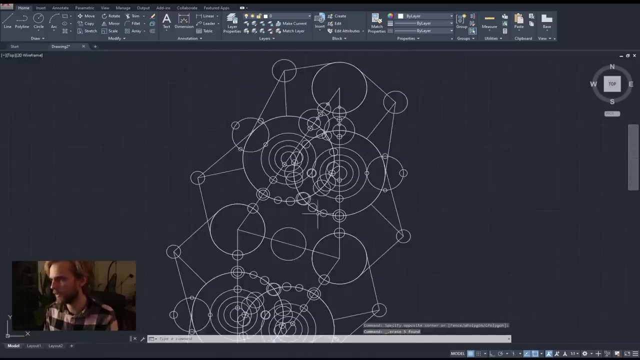 inside of those intersection moments, or not necessarily inside, because you can do, uh, you can do something like this: tr enter, enter, double enter, remember, and then click here, click here, right, it just finds the intersections and kind of deletes stuff, that's, that's sticking out or going in. so you're basically erasing segments, uh, in in that way. so if, if I were to look at the more 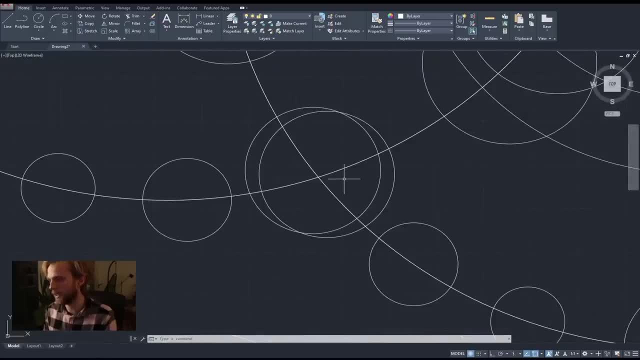 uh, more complex example. let's say I want to clean this up. I can say tr, enter, enter, and then then I can just kind of go to town and keep, keep deleting this and I'll purposely make a mistake, or or not a mistake, but I'll, I'll do a thing that always happens and I'll keep kind of going here and 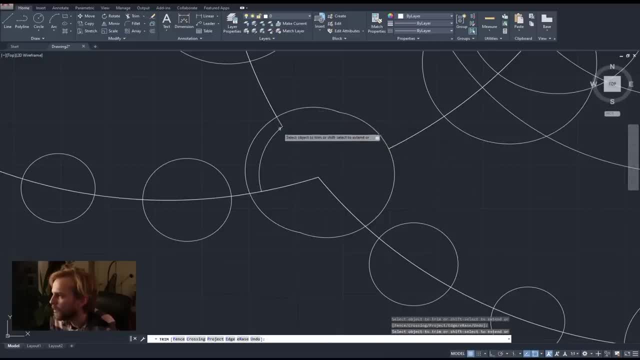 trimming away all of these segments, and at a certain point I can't anymore, so I'll trim away this one. I think, yes, but now I can't trim. well, I can't trim this. there we go. now I can't trim anything else, never mind, now I can't trim anything else, there we go. so 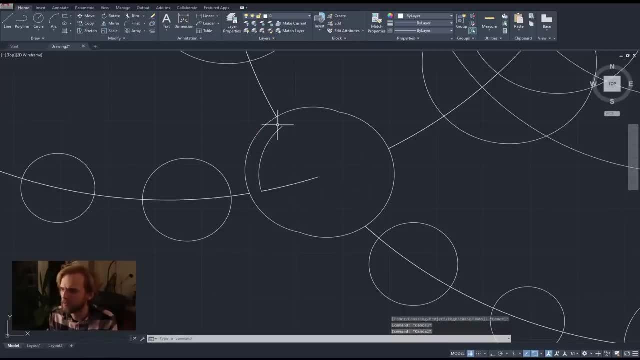 these two segments here right, can't be trimmed, and the reason for that is the they both meet at their end points. so there's no way for me to kind of. you know, these are full segments that are meeting in their end points and they're not being crossed by any geometry, right. so I can't. 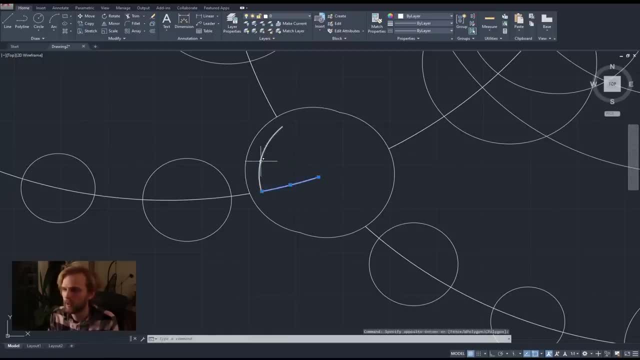 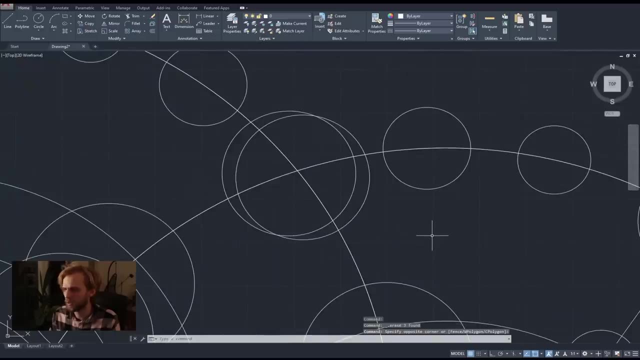 any geometry, right, so the trimming will not work on them. so then i just kind of select them and delete them, right, so that they get trimmed away. as you're using trimming pr, enter it will. you can choose to select objects rather than selecting all, so i can select, for instance, these two objects. 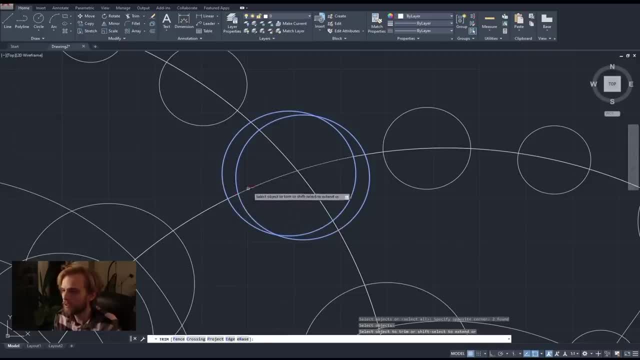 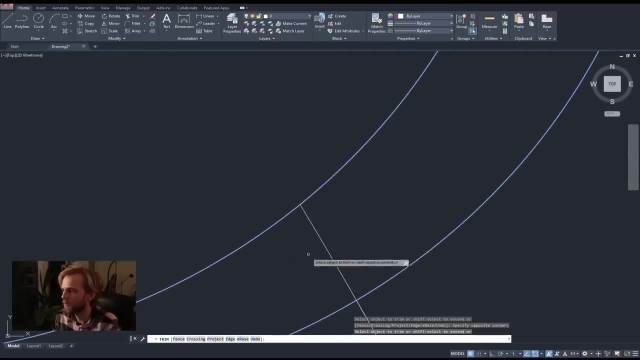 hit enter. and now everything that i trim, right, it's just going to be trimmed by those two objects. and why can't i trim this? i can, it's just i need to zoom in fair enough, right, um? and of course it can also. you can also trim objects. 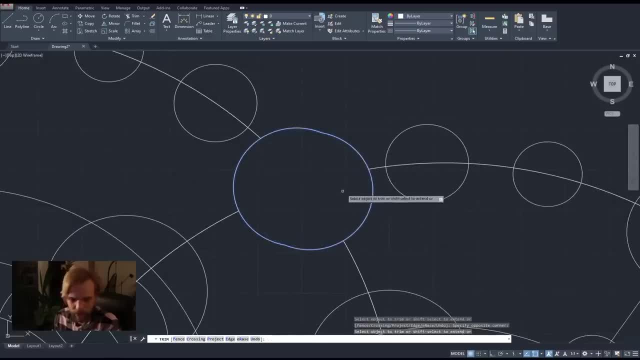 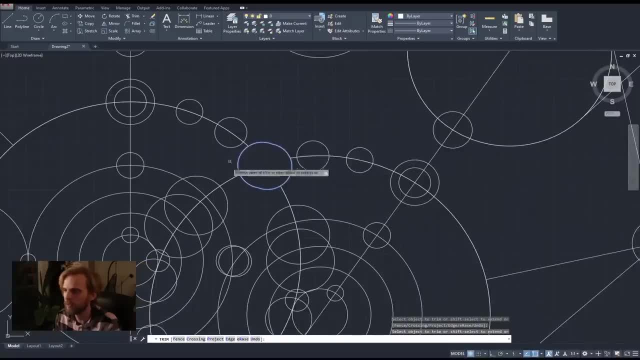 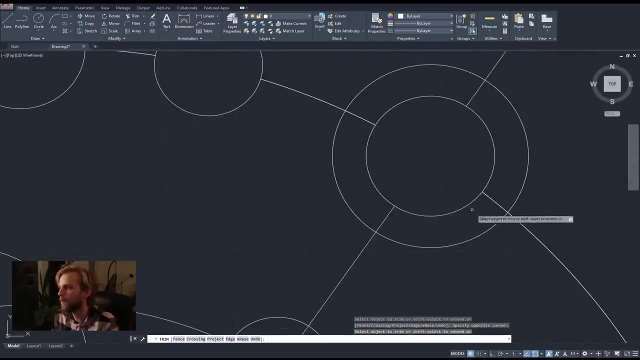 in here and start trimming. it won't let me because it's it. it has nothing to do with with these, this geometry right here. so i do prefer using tr enter and then just hitting enter again and then going, going in here and trimming away. um, anything that i that i want in any part of the drawing, right. 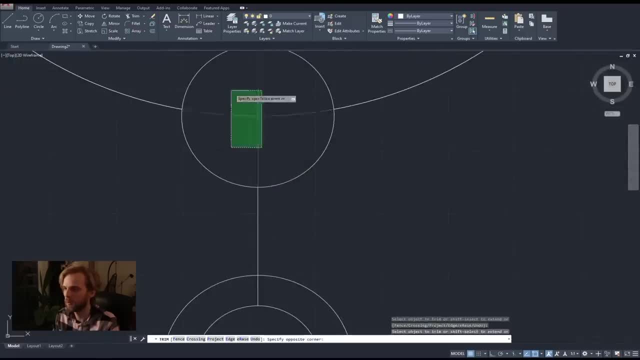 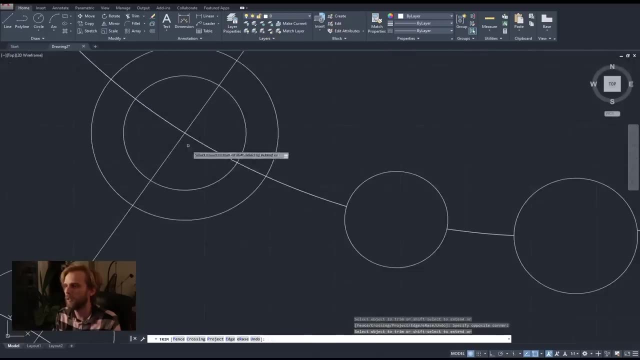 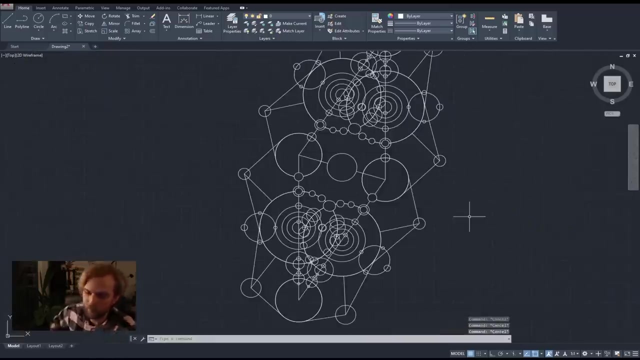 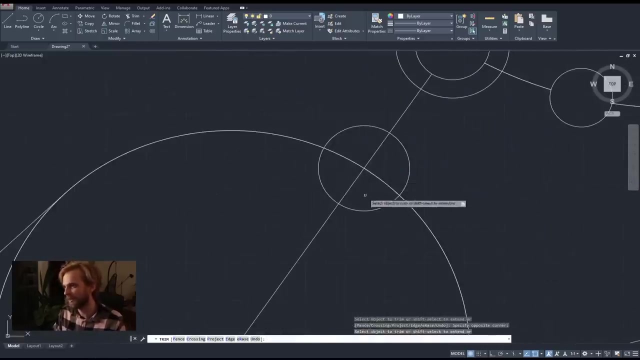 much, much more convenient for me with with that select all method. right, that's. uh, that's that. let me just clean it up, because i like stuff when it's clean. there we go, okay, uh, wait, nope, dr, enter, enter. almost almost forgot about these two. there we go. 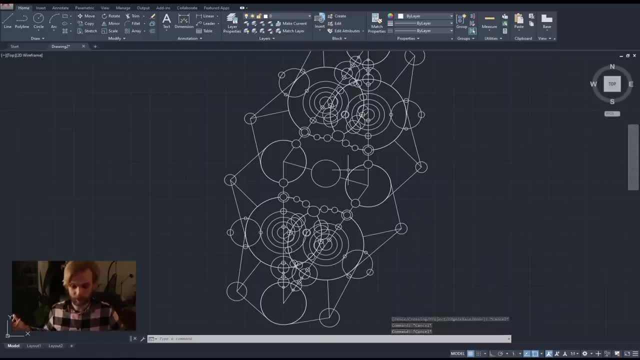 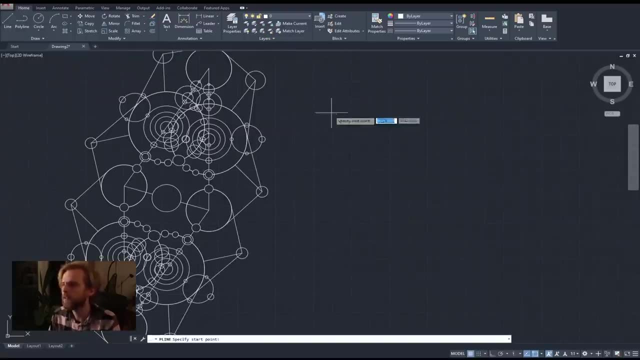 now, now it's fine, um, so that's trimming, that is uh, that is trimming. then we have extend. extend is basically: if you have a polo line and it's doing this, and you have another one and it's doing this and you want this polo line to elongate until it hits this polo line right, or this line. 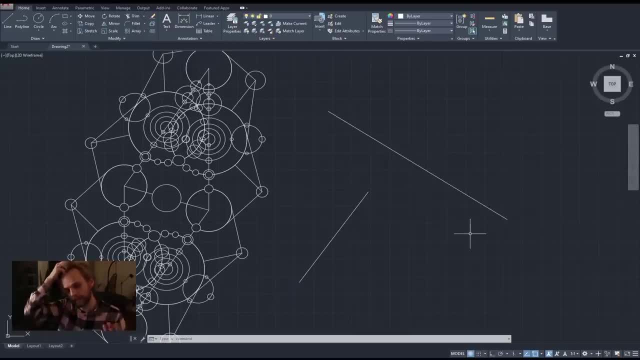 segment elongate until it hits this line segment, that is, extend ex enter. it's going to ask us to either select objects or select. all this time around, i always select the objects, you, and these are the objects towards which i'm going to extend, right? so first, uh, i then select this. 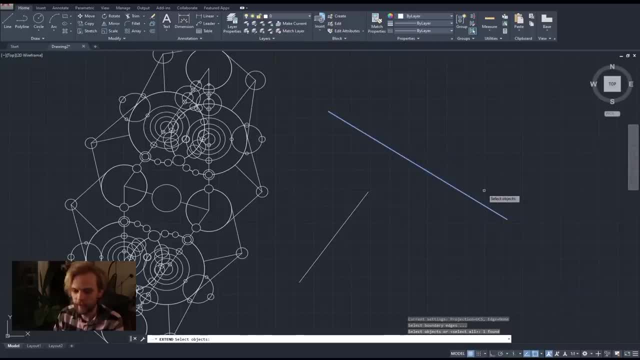 line segment, right, i hit enter and that's important. and then i can click on my other line segment and it's going to be extended towards this object, right? so that's how extend works. um, there are some cases where it's, of course, not going to work, for instance if i just say line. 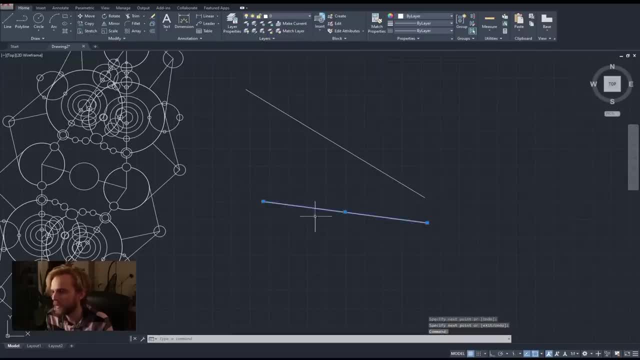 and i want to, and i have this line and i want this line segment to extend towards this one. it won't work, right? if i extend, enter, select this line segment, enter and then try to select this line. it will not work, it will not extend. that's because 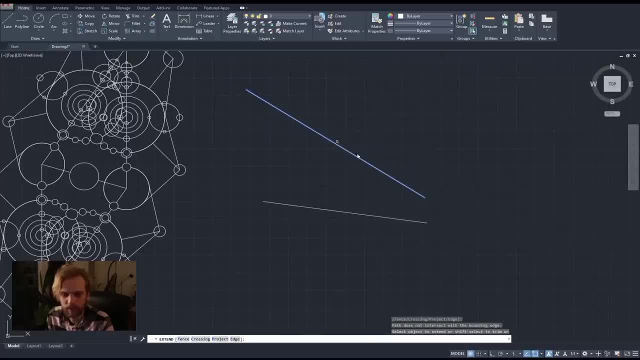 the. there's no way for this line to extend so that it hits this line segment uh, which actually brings us to uh. let's see if it brings us to. yes, it does. it brings us to another tool that's called fillet and the shortcut for it is f? f. enter fillet, right, uh. so fillet basically extends two line segments until 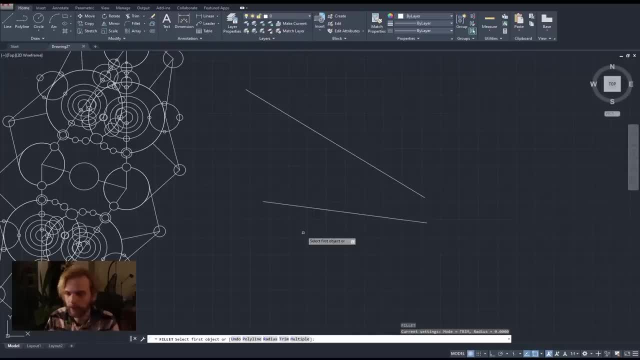 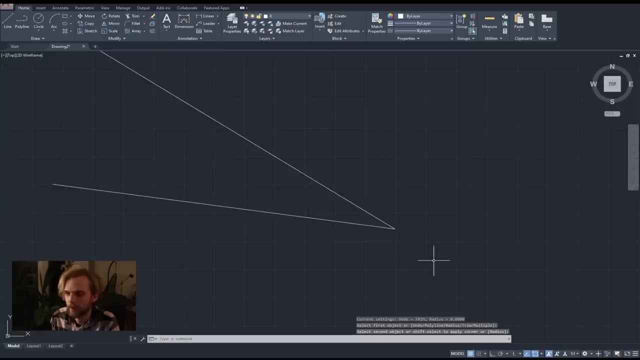 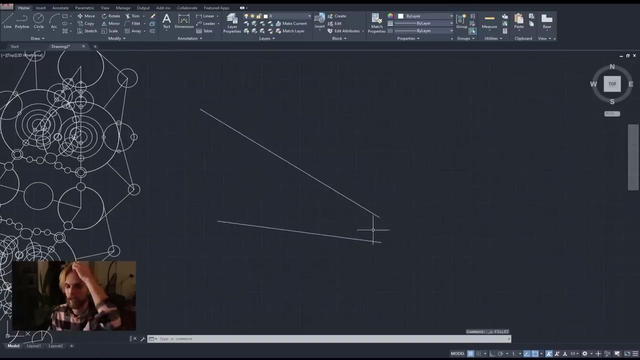 they meet at a corner right. let's see this guy and this guy. if i fillet them, you and you, they get filleted into a corner. the reason why it's called fillet is because you can change the radius of the corner right, so it doesn't need to be a sharp corner. let me control z to undo and let me fill it again. 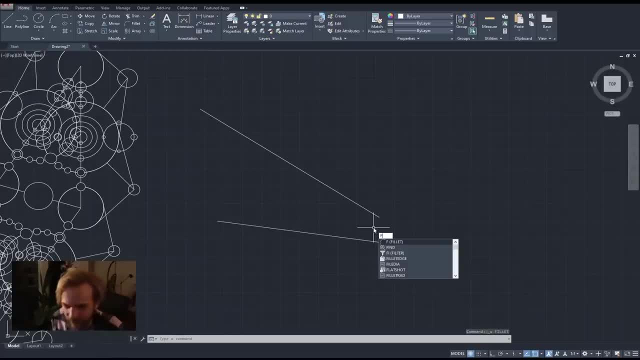 fillet, or i write the full thing f, enter, um, and here i'll just say radius. i'll click on the radius or type in r, enter. it doesn't matter if you click on or type in r and here the radius ended this. この� Smart SCALE 節約 tres回 Крас界 去PC sow, witnessesあります. 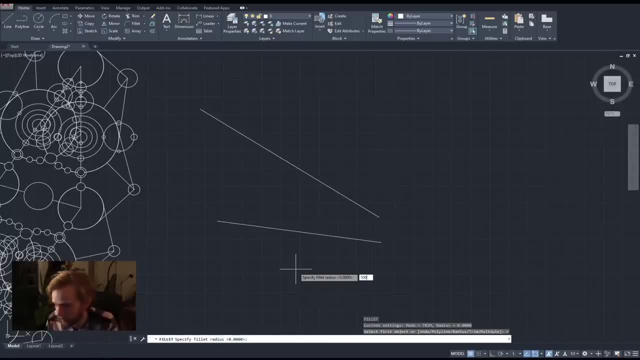 here i can specify a radius, so i'll give it like 500 millimeters. i have no idea how long those lights are, but i- i assume 500 millimeters will work- 100, hit enter and now i will click on the top line, click on the bottom line and you get filleted. quite nice, huh, quite nice, um and it. 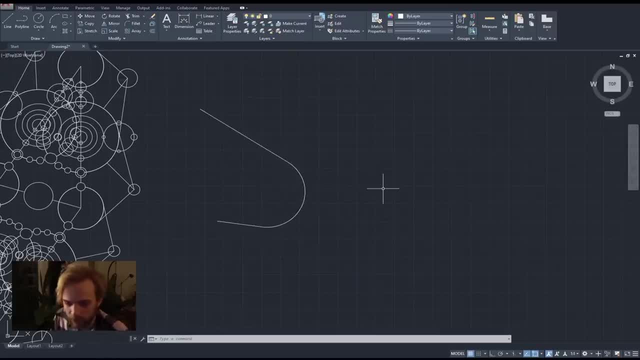 gives us a fillet of radius of 500 millimeters. so that's how fillet works. um, there's also like options for uh fillet where we can see that. no, there's no options for fillet where we can never mind, never mind, ignore, ignore what i said. uh, i thought that it was the same as in rhino, but 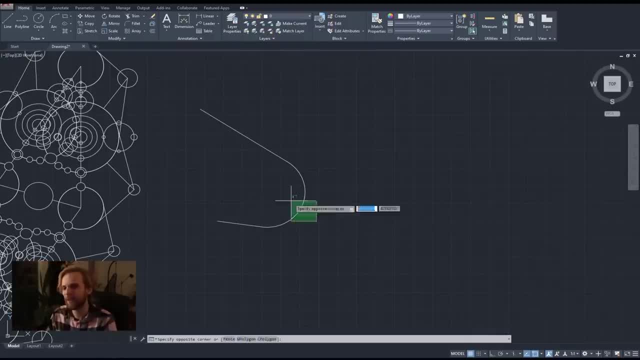 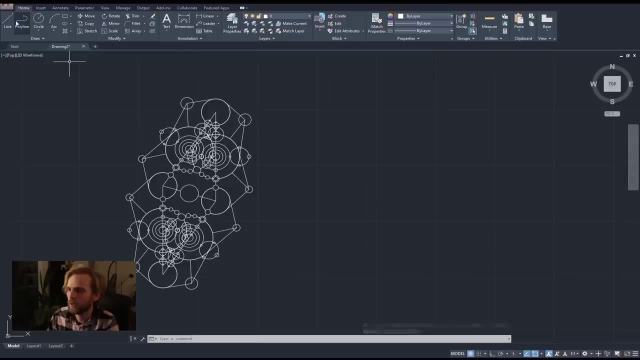 it's not so, just radius. for now, we will just be using radius. delete that. so that's fillet. um. fillet doesn't work with objects that are parallel, of course, because there's no way for you to extend to objects that are parallel to lines that are. 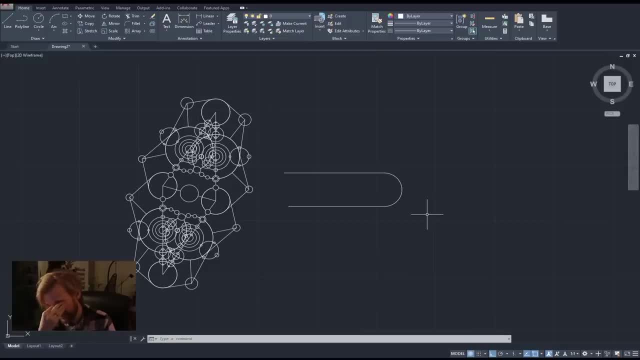 okay, okay, apparently it does work. what the hell? okay, wait, fillet, fillet, radius zero. what if radius is zero? will it not work? then it still works. that's a smart cookie. so then, uh, if you have two objects that are parallel and you try to fillet them, even if the radius you specify the radius to be zero, 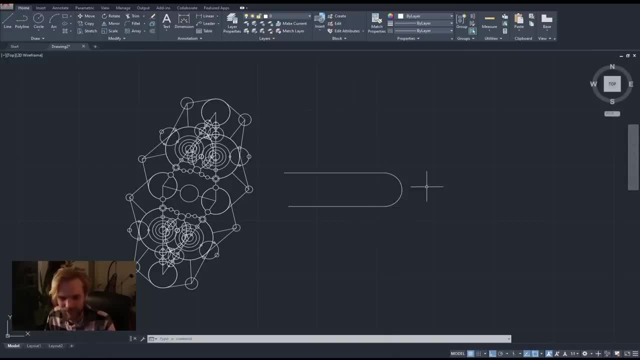 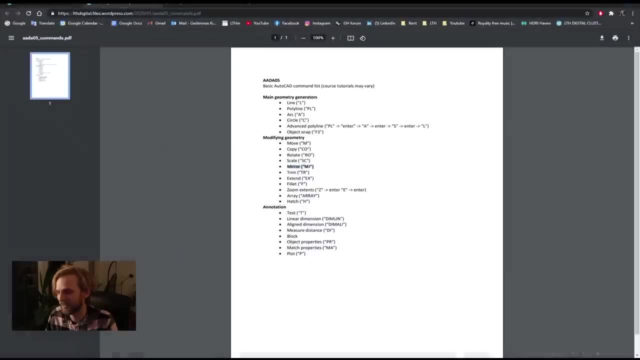 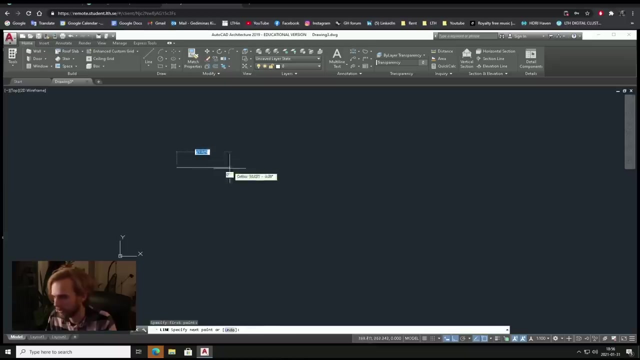 it's going to create an arc that connects the two objects. that's nice. that's a. that's a new functionality of autogad that wasn't there before, definitely wasn't there before. let's see it in the older version of autogad. if that's also the case, well, all older version 2019 is not that old. 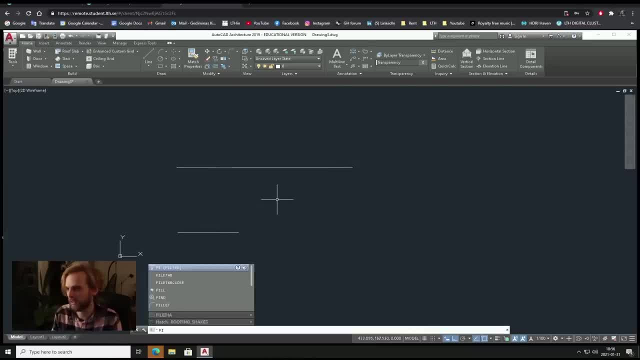 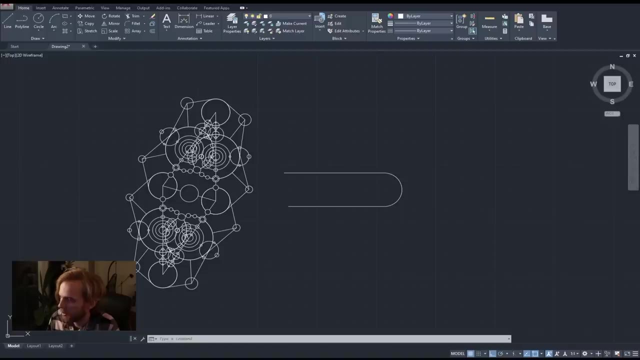 uh, one line segment, another line segment: fillet. come on, fillet, let from here here. yeah, it does work here as well. cool, okay, i'm learning something new as well. so if you have two parallel line segments, apparently it's going to just create an arc between them with the fillet, even if you say you don't want any radius for the fillet to have. 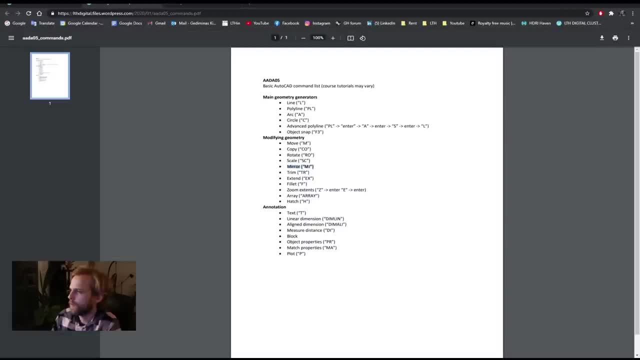 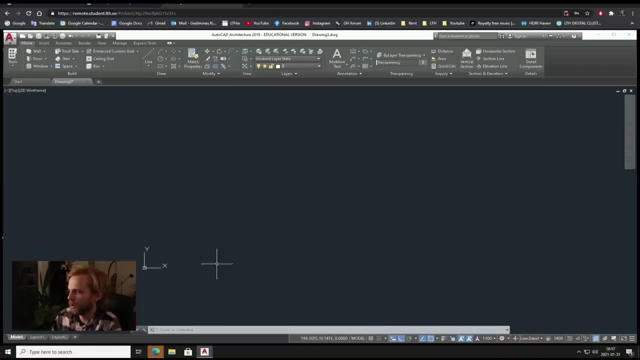 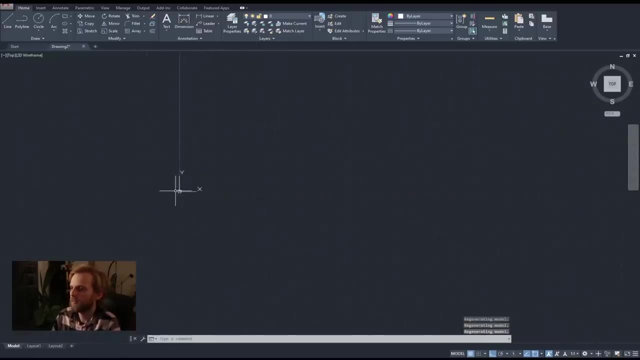 cool. uh, what's next next up? we have zoom extends, okay, so that's an important one. um wait, oh, wrong, wrong, wrong out. let's say here: right, i i've been working on this and i have zoomed out, zoomed out and i messed, messed it up, and i have no idea where i am right. i have absolutely no. 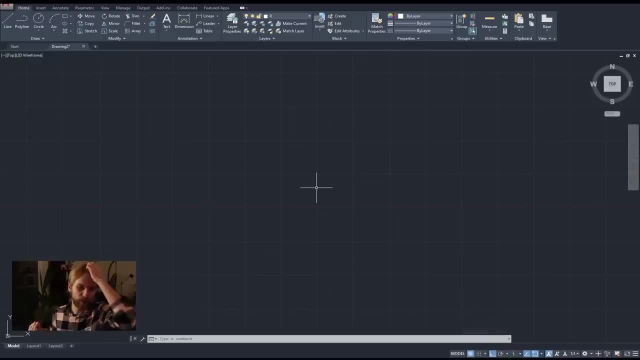 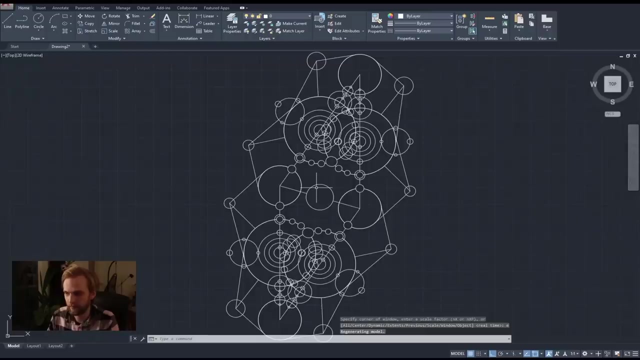 idea what i, where i am, uh. so what you can do is you can say ctrl a to select all. so ctrl a selects everything you have in your drawing. and then what you can do is you can type in z, enter, e, enter and it's going to zoom in to the geometry that you have selected. 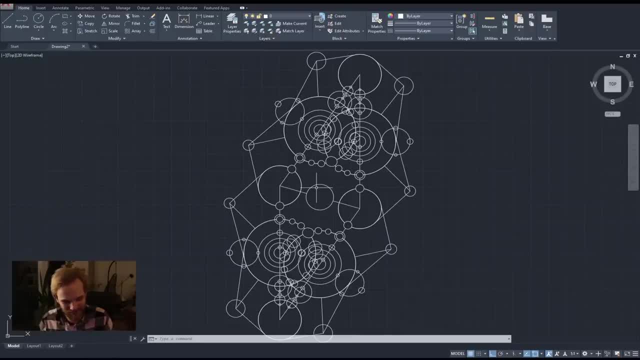 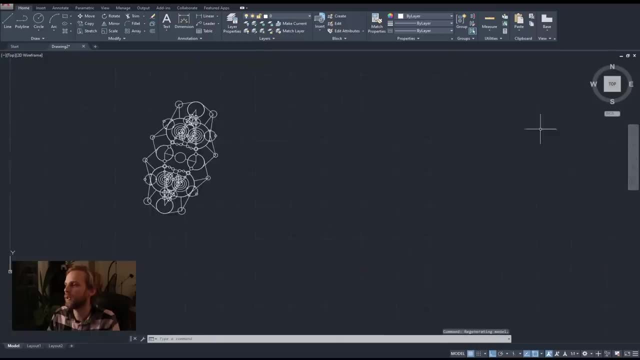 so if you're lost in your drawing, then ctrl a, z, enter, e, enter really helps. but also it's quite useful where, when you have like multiple drawings on one one sheet, then just saying, well, let me copy bam, bam, bam bam. let's say you have multiple drawings on one sheet, and just so that you don't need to zoom. 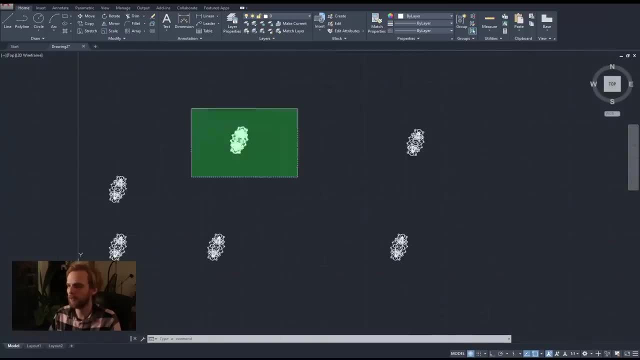 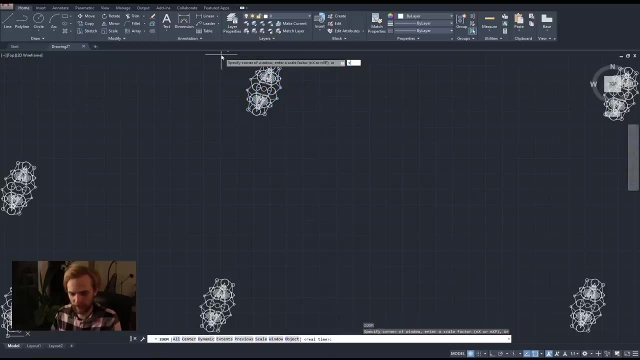 in, zoom out. uh, what you can do is you can just select z enter e enter. oh sorry, in this case it would be z enter, s enter selected. i'm a little bit rusty, apparently, yes, okay, so it's going to be selecting the object: z enter o enter. 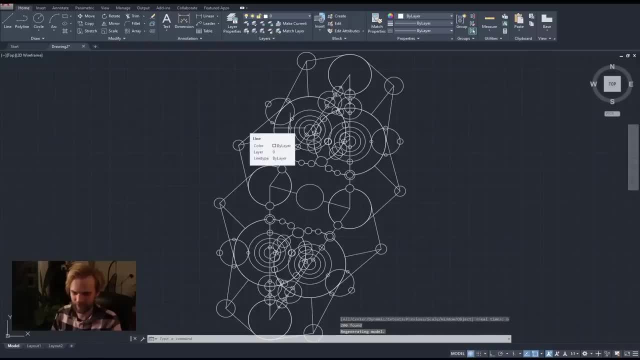 zoom to object, so zoom extends. i made a mistake during this tutorial: zoom extends. you don't need to do ctrl a, you don't need to select all of the geometry. it already recognizes the geometry. so you can just zoom in and out of the geometry and then you can just select the object and then. 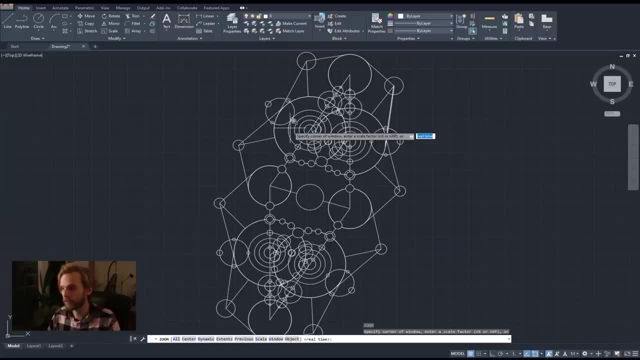 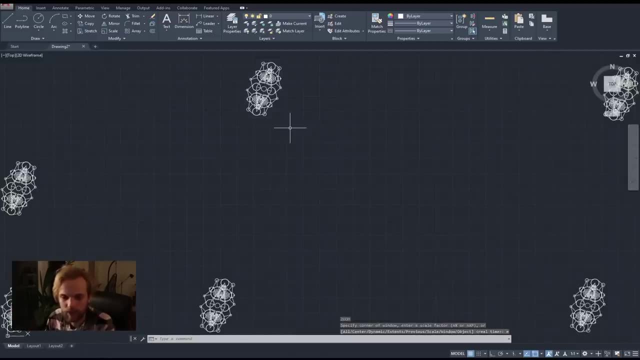 where that the geometry is, as if it's selected. so z enter e enter extends will zoom into all of the geometries on your scene in your, in your model model file, automatically. you don't need to select all of them beforehand. that's useful. uh, yeah, forgot about that one, i apologize. z enter, enter. there we go, we're zoomed in. uh, so that's that. 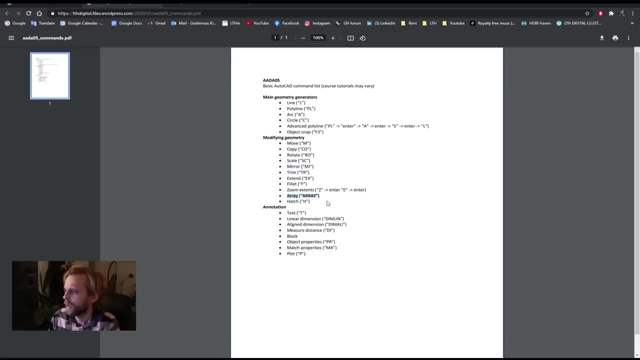 zoom extends quite useful. and then we have array and hatch. these two i will show you later. uh, once we have some geometry going on in the rhino, this is an autocad course in the autocad file. once you have some proper geometry going on, then i'll 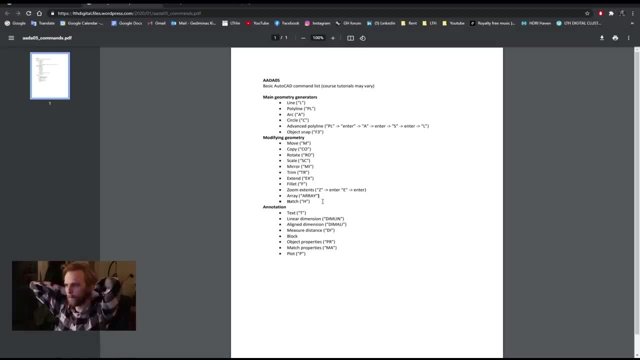 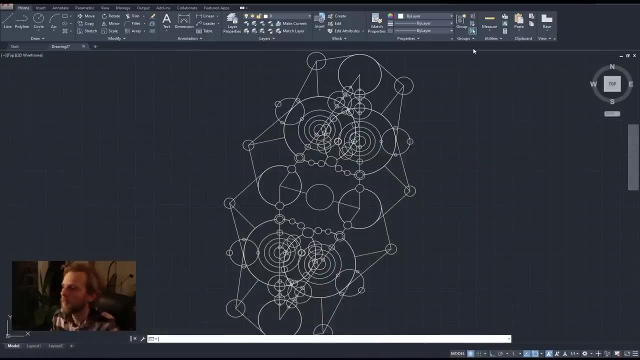 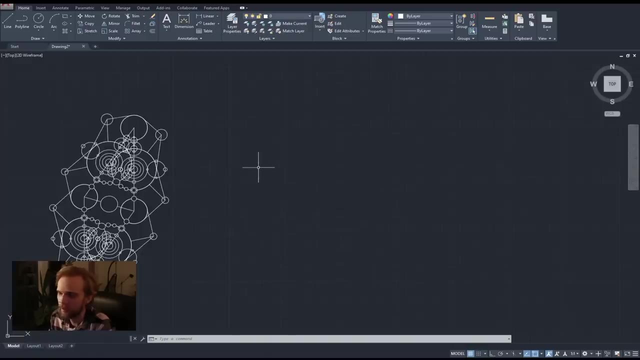 show those two. uh then, um, let's draw a building. enough of this, let's, let's draw, let's draw a plan first, right, so i will, i'll keep this, why not? i'll keep this, but here i'll start drawing my, my building, right? so the first thing that you do before you, or actually no, i, i will not keep this, i will. 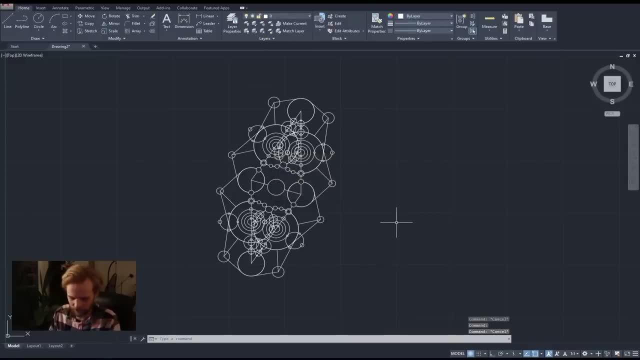 close this file all together, or we can, we can just select it. there we go: selected, deleted, clean, clean sheet. you know, to just start with, the first thing that you do before you start drawing is you check the units. we already did that, right, we are drawing in. 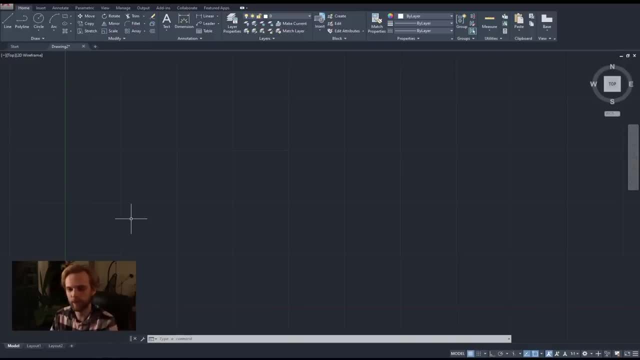 millimeters. second thing that you do when you, before you start drawing, is you create layers in which you're going to be drawing it. so up till now we will. we were drawing in a single layer right, which was the layer zero. AutoCAD works in layers and different line thicknesses different. 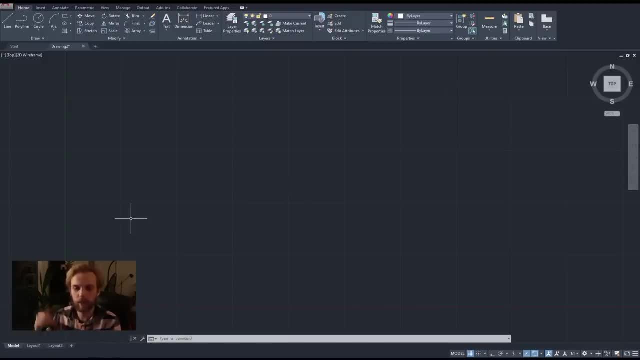 line types and line colors are described by different layers- right, and you can turn on and off those layers. it works in a similar way as as Photoshop, actually, in this regard, one more thing that I didn't know, it is that AutoCAD is vector-based rather than right-handed. 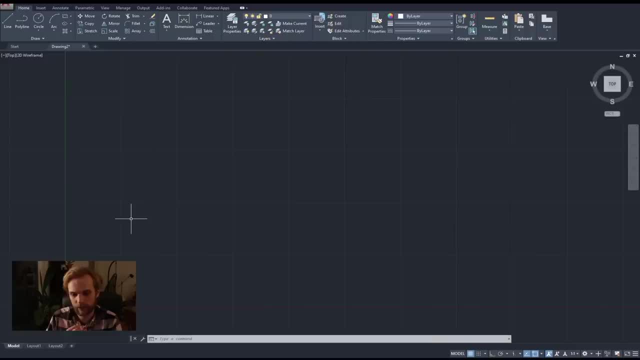 vector-based. so think of it as Photoshop versus Illustrator, right, you're used to those two by now. uh, Photoshop uses pixels while Illustrator does it, meaning that you can zoom into geometry of Illustrator infinitely and it's not going to change resolution, or it's not going to. 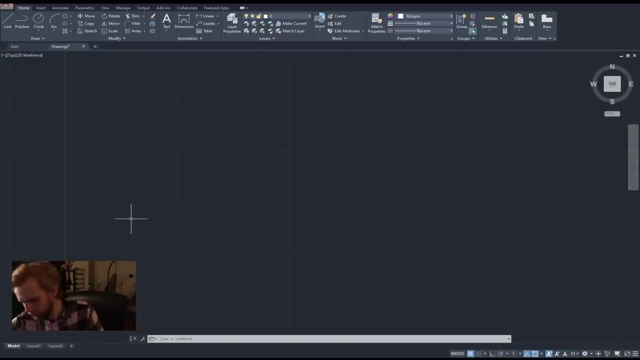 it doesn't have a finite resolution, while, um, while in Photoshop, if you zoom in too close, then you'll start seeing the pixels right. so any kind of 3d modeling or drawing software for commercial use is going to be vector based. it means that your lines are infinite in, in their resolution, in their quality. 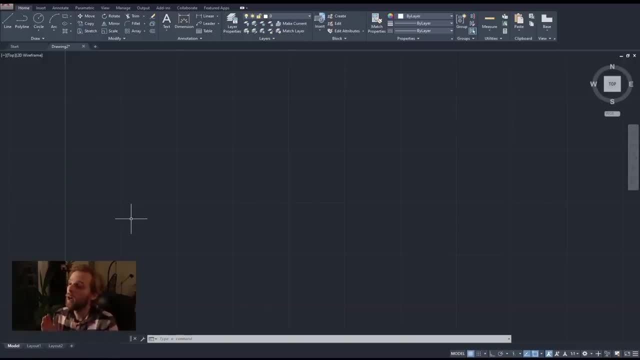 that's important to you know. okay, layers, right. so how do we access layers? well, they are located right here, the layers tab, of course, and you can see, here it's, it's our active layer, layer zero, and, if i expand this, that's the only layer that we have, layer zero, and it says. it says that: 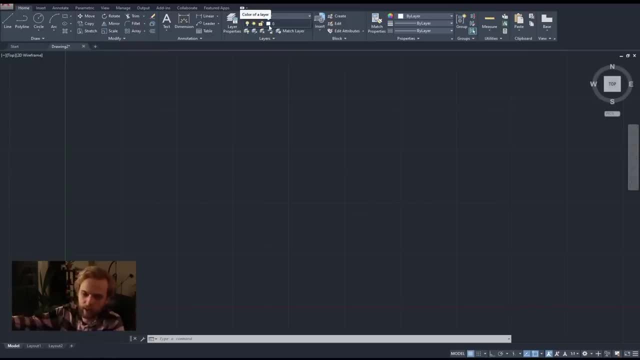 it's white but it's actually black. well, it shows white because we have a black background, but it's going to print out black. don't ask why, just go with it. i'll explain the print printing settings later. um, if you want to add more layers, we need to go to layer properties, so i'll click. 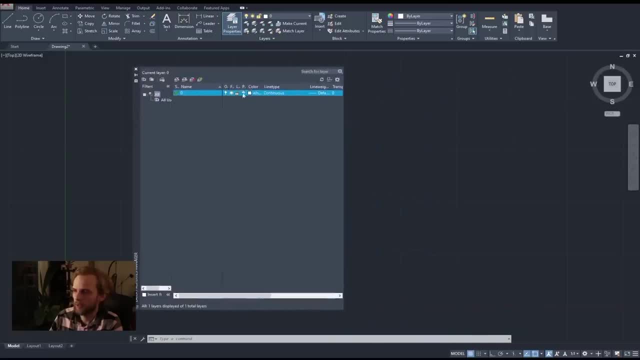 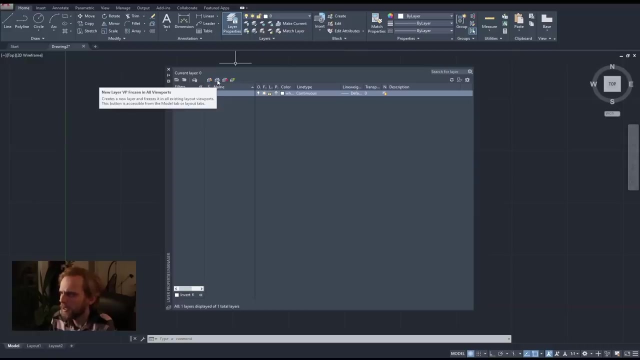 on that layer properties will open up this layer tab for us, which let me expand it and let me just make sure that you see it. there we go. so here we have these four icons: create new layer- freeze- oh wait. new layer. frozen- oh. create a new layer that's frozen- uh. delete layer and set. set a layer. 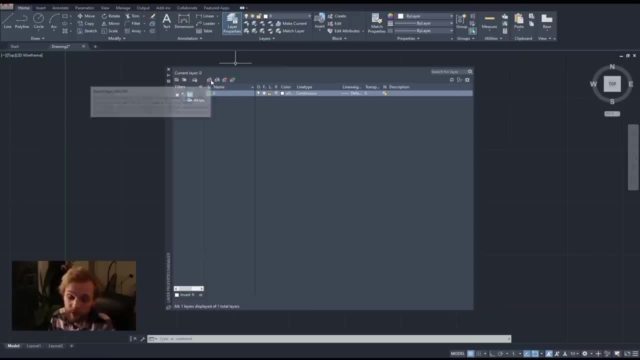 to current. we don't care about these three, we only care about creating new layers. so i'm going to be that i'll click on this create new layer tab and i'll choose and i'll say thick line or or just thick, right, so creating new layer, calling it thick. create one more layer, call it medium. 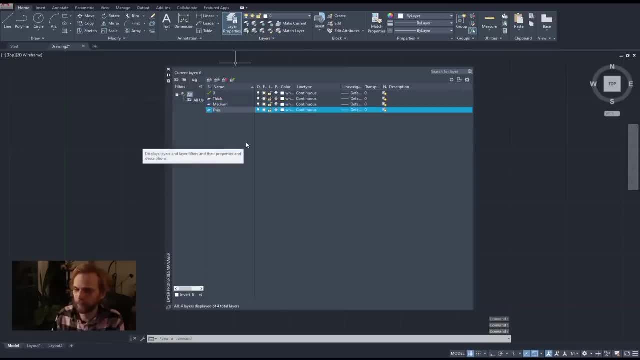 and create one more layer, call it thin, right? so we have these three layers here: thick, medium, thin. great, what can you do with them? you can turn them on or off, you can freeze them and you can lock them. for now, just ignore the freeze area, just think of it this way: if you lock them, 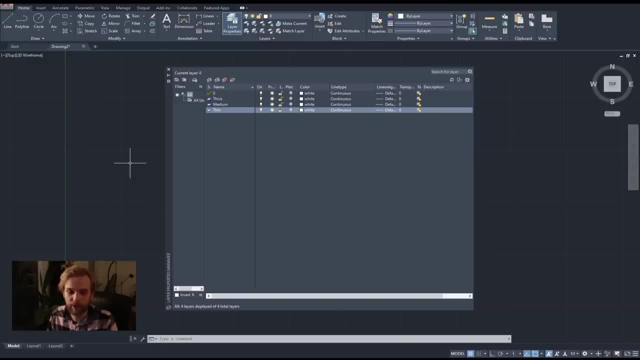 you can't select the geometry of that particular layer in the viewport, which is quite useful when you have a lot of stuff layered on top of each other. stuff that you don't want to select can be done in the viewport, which is nice. um, then, are those layers, uh, printable? can you print? so that's. 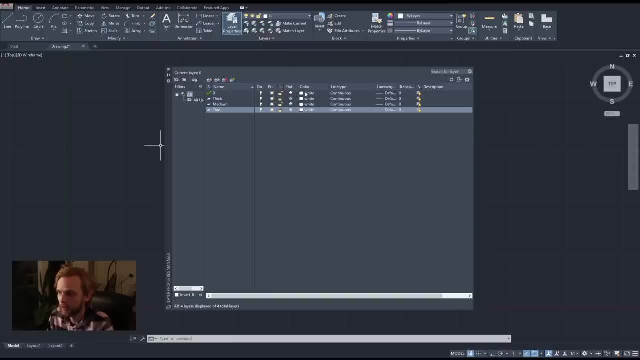 the plot area here. what kind of color do those layers have, what kind of? what's the display color and what kind of line type and line weight? so we will be changing that in just a, i guess in the next tutorial, but for now i'll just change the colors. uh, just so that we can distinguish between. 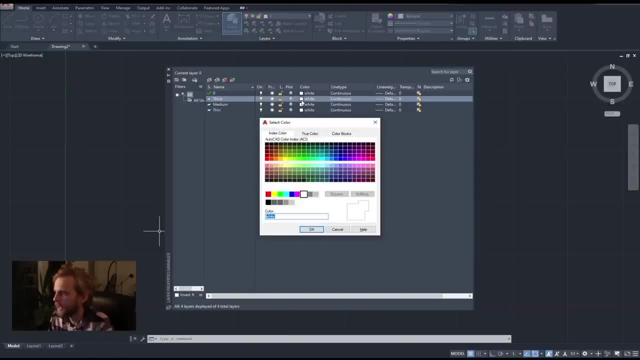 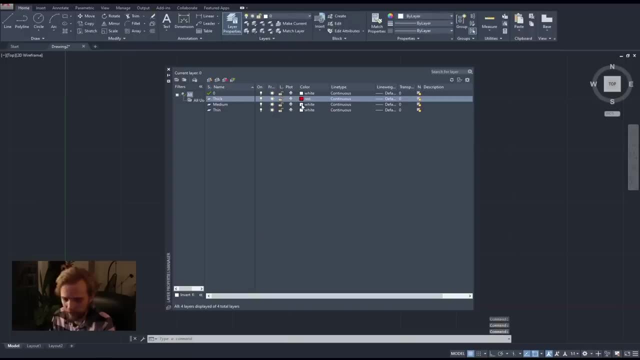 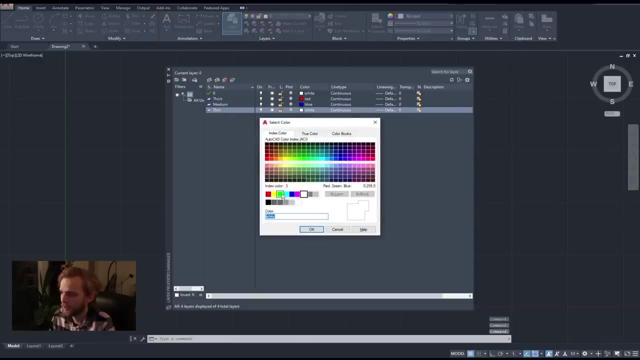 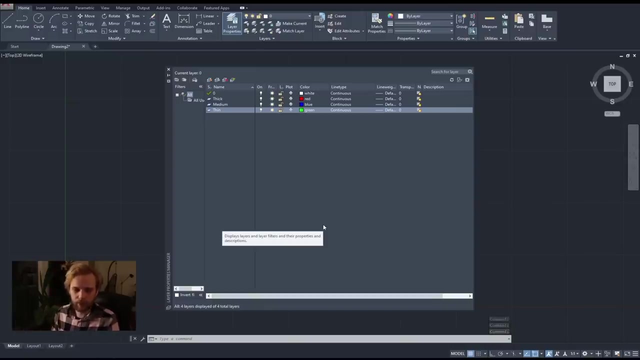 thin, right. so the thick layer. i always like to choose red from here. medium, i always like to use blue, and thin, i always like to use green, but it's absolutely up to you. this is just something that i'm used to, and, as i'm drawing, this is the way i color code my lines. that that's about it, right? so we have. 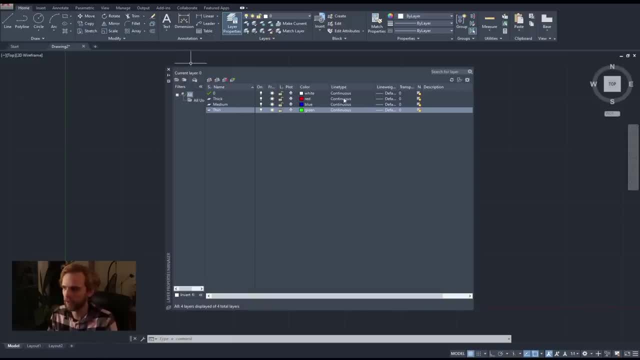 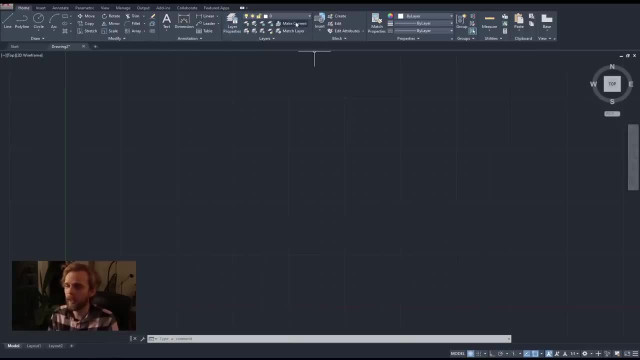 our layers set up and i'll keep the zero layer for now. that's, that's fine, that's okay. once we have them set up, i can close. and now i can uh, create or or not not create. but now i can expand this drop down list of layers and i can choose which one is going to be my active one. 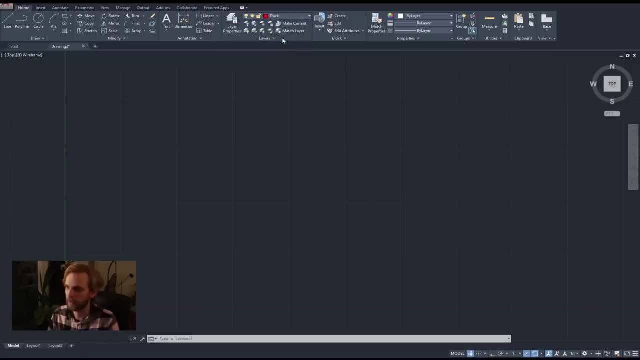 the one in which i draw. so i'll choose thick layer here. thick it's my active one, and now, as i draw a circle, for instance, it's going to be red because it lives in that layer. um, if i draw another one, it's also red, red, right, all of them are red. um, if i want to change a layer of an? 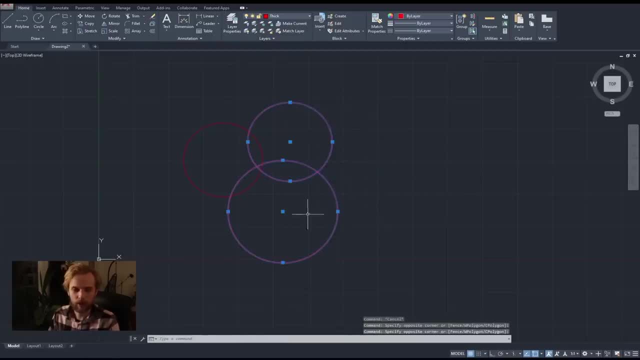 object. all i need to do- or multiple objects. all i need to do is just select them and in the drop down list i just choose the layer that i want to use, and then i can select the layer that i want to layer right once i hit escape, i'm back to my uh, to the active layer in which i'm drawing. but now the 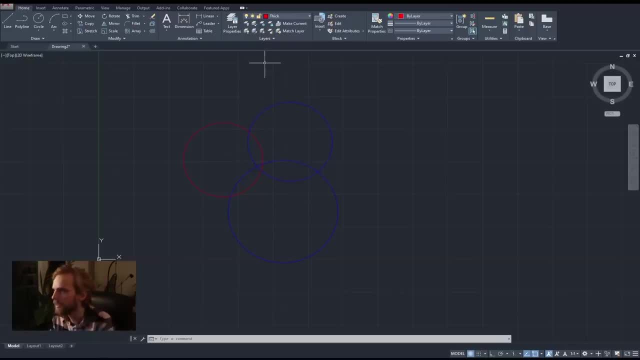 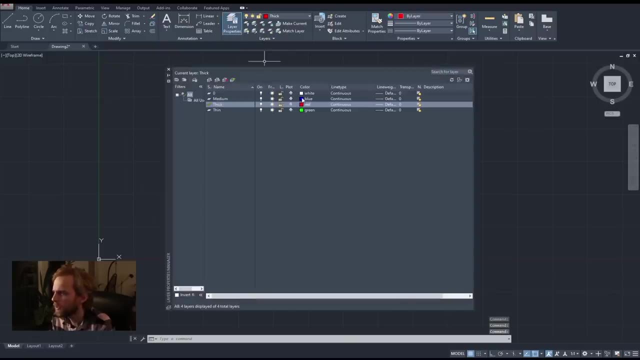 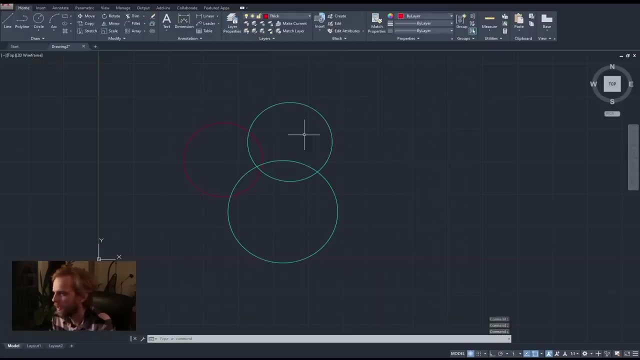 layers of these two objects have been changed and i can see that it blue might not go well with the recording, so i will go to layer properties and change this blue to cn. right to cyan, not cn cyan, uh, just so that they pop up a little bit better. there we go. so that is that's that right. uh, working with layers- really easy in. 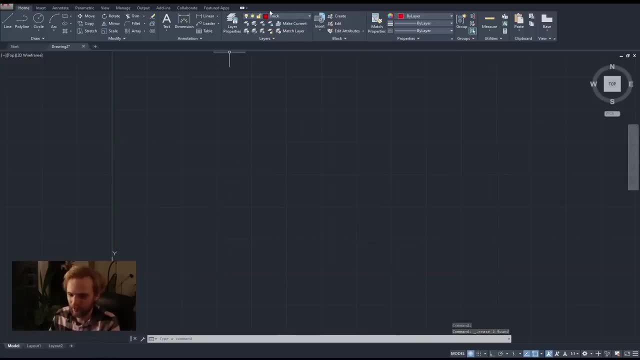 autocad, let's start drawing. so i'm gonna start drawing in thick layer, uh, with thick lines, because i'm going to be drawing a plan and i'm going to be i'll start drawing from the walls right, or rather from this section of the walls. so the plan is cut at 1.2 meters. 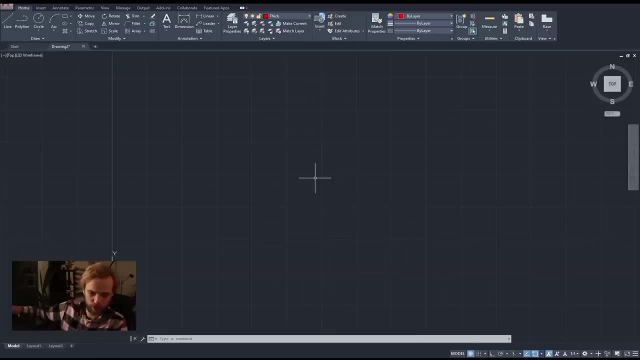 um, yeah, it's cut at 1.2 meters so that you are cutting through windows above the tables and whatnot. so it's like a locked, locked number. um, you can always kind of adjust the, the height you know for different projects if there's a need for that, but the default, you know the default. 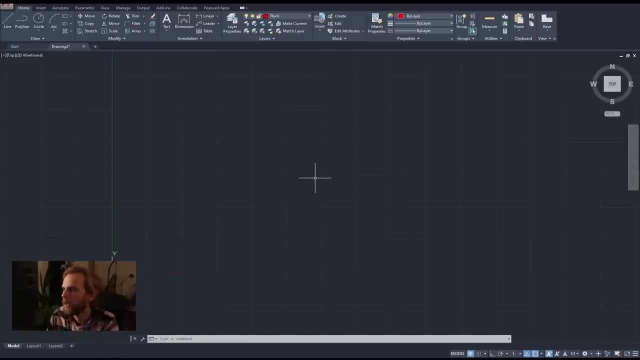 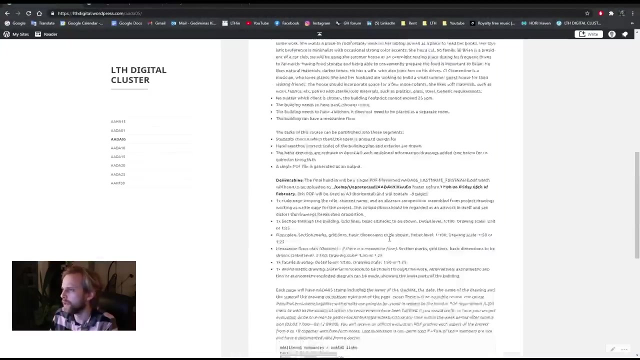 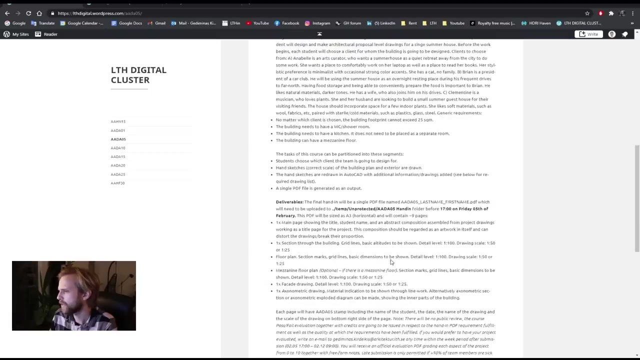 number that you should have in your head is 1.2 meters. uh, so that's how high we're gonna be cutting our, our plan or our building, and showing the plan uh through the cut. so if we go into the course website and kind of read through this, i can somewhere here that's the course description. 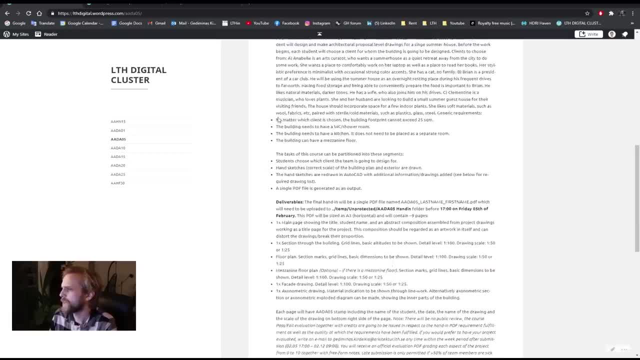 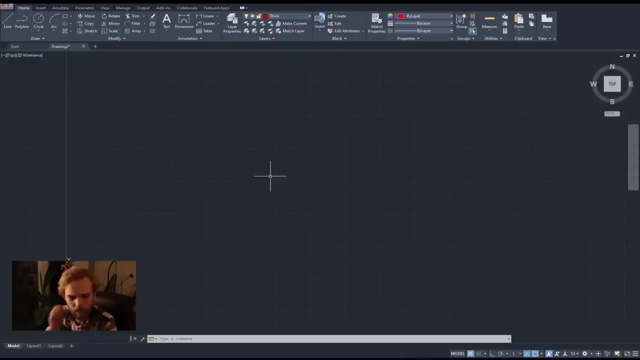 that's the deliverables. yeah, there we go. uh, no matter which client is chosen, the building footprint cannot exceed 25 square meters. okay, that's like five by five, sure, but five by five is. is not that convenient for me? i'm thinking of, uh, six by four, perhaps. 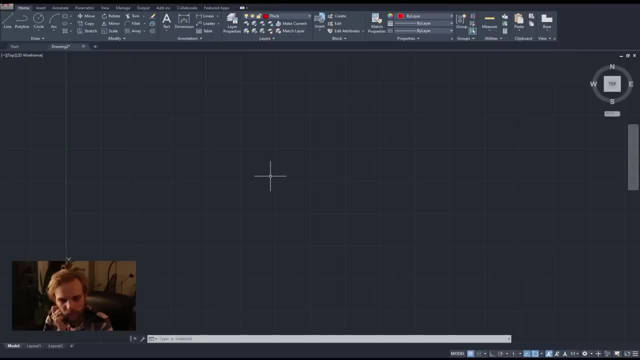 yeah sure, let's just do six by four. uh, we'll, we'll see how we can cram it in. i haven't planned it out in my head, so it it might be a very crappy, very crappy building, but this is just to showcase the way you work in autocad. um right, so 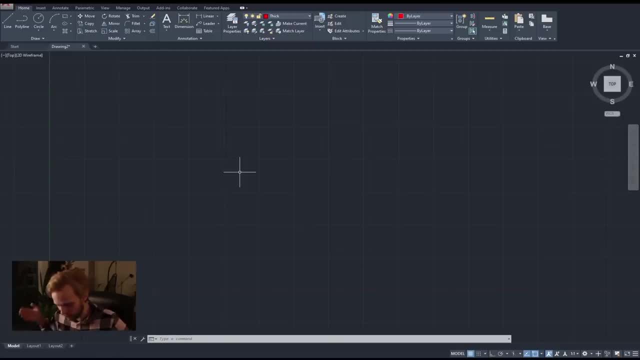 i need a. i'm going to have a building that has a footprint of six by four meters, six thousand by four thousand millimeters, so i'm going to actually create a rectangle, r-e-c-t rect. i'll start drawing it from anywhere it doesn't matter, and i will say that i'm going to draw it in dimensions rather than 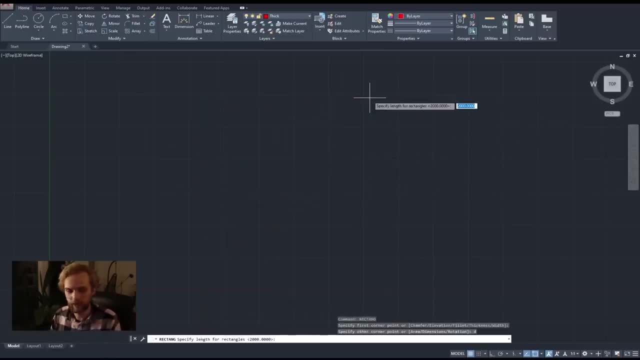 just clicking somewhere else on the screen. so d enter, right, d enter. and then i type in the length, which is six thousand. enter, did i not? yes, six thousand. and now it asks me for the width, and the width is going to be four thousand. actually i can kind of get away with 4200, but uh, for now i'll just say 24 square meters, that's fine. 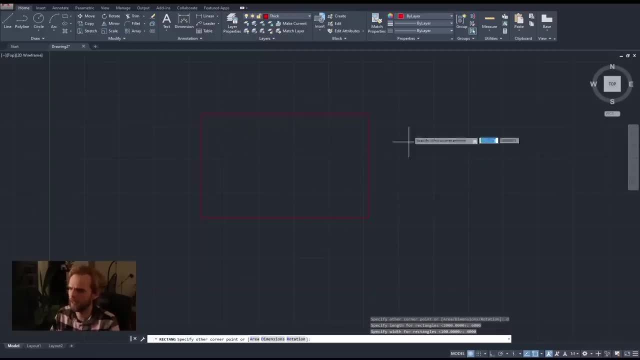 as well, four thousand so, and then i'll just choose that: yeah, here, whatever is the rectangle there, um, so that's my, that's my outer- uh, footprint, right outer footprint. my walls have thickness, of course, and for this i will say that the wall thickness is going to be. 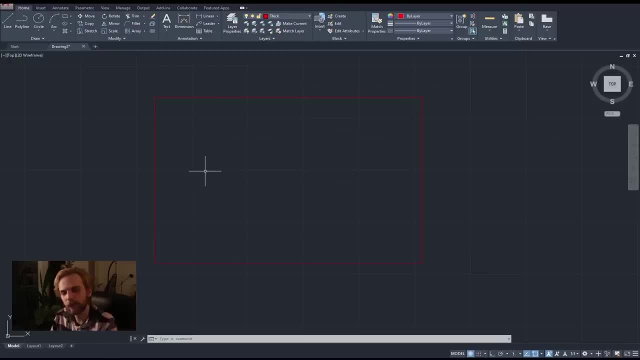 um 400 millimeters. the outer wall thickness, uh, around 400 millimeters. usually they are a little bit thicker than that, but uh, it's a summer house, it's a pretty small house, so 400 is okay, uh, so what i want to do is actually i want this rectangle to go inwards to make a copy. 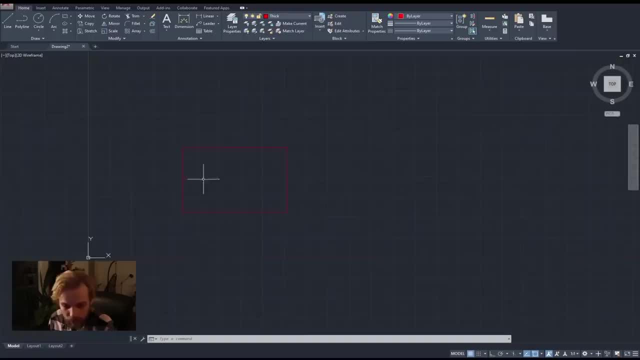 of this rectangle inwards by 400 millimeters, and there is a tool that does that. i will show it on this side here real quickly. if i have a polo line or a line segment and i use a tool that's called offset, offset, oh, i think it's, yeah, it's just, oh, enter and i type in the distance. so here i'll just 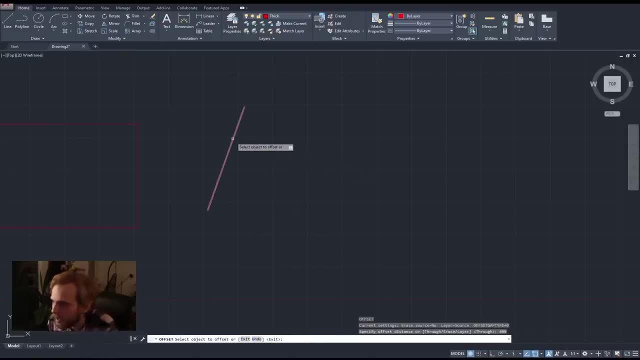 type in 400, enter, i can select the line segment here and i can offset it to either side, to here or here, doesn't matter, and click, and then i know that between these two lines the gap is indeed 400 millimeters. right, so that's offset really useful. uh, also works with polo lines. 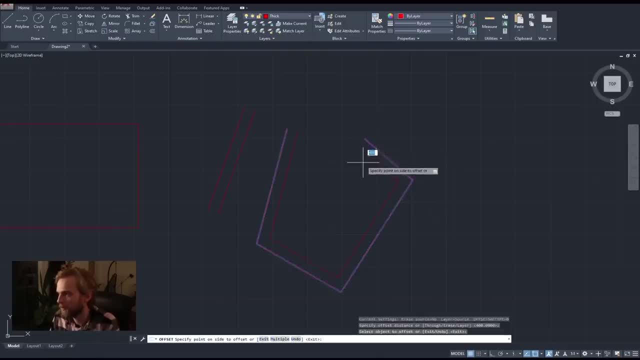 offset uh 400, like that. right, if i were to draw the same shape or similar shape, uh, with line segments though, like that. and then i did offset keyboard, come on, offset 400, then, uh, since i drew this with pole line and this with line tool, this is exploded. 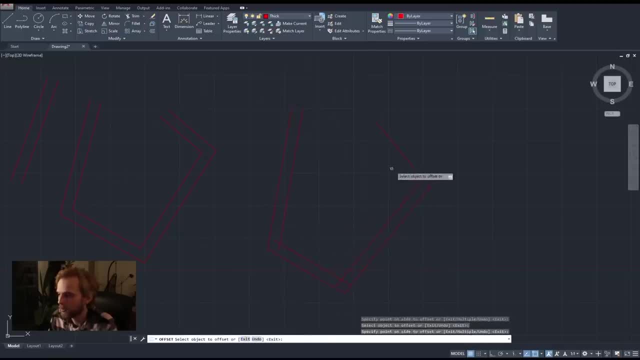 so that means that my offset is going to be a little bit more tricky, like that, right, i will need to offset every line separately, and then i will need to tr, trim, enter, enter and trim away the doodads here. right, clean it up. now they're kind of the same. the only difference is that 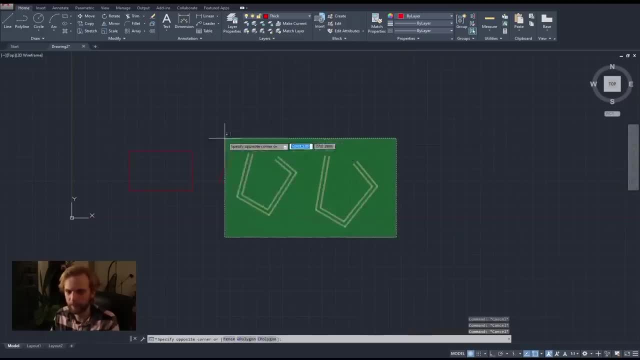 this is exploded while this is joined up, right? so back here, back to our plan. i can just do offset 400 and offset it in words by 400 inwards, because we are already at 25 square meters or 24 square meters, so i can't offset it outwards, i need to offset it inwards, right? so that's the. 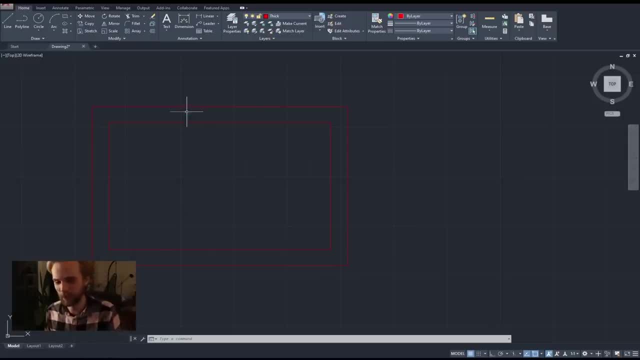 thing that we're going to be working with, right, that's our inner area, not a lot of stuff to work on, so let me just quickly plan this out. um, let's say we have some sort of a block here- toilet, shower room, entrance, kind of work okay. so let's say i want a separate. 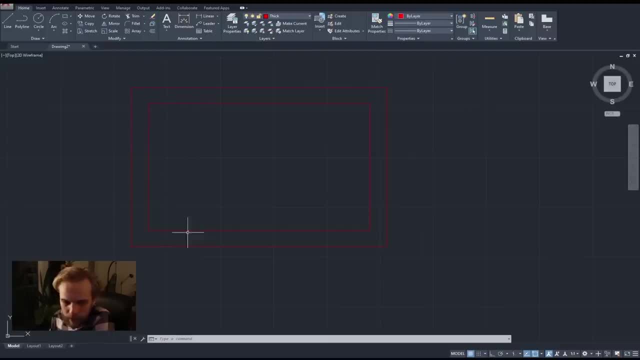 room here, right in this area, where i'm going to have my bathroom, my shower and and whatnot in in this particular room, right, um, and it's going to be a little bit of an awkward room, but that's going to work out. so i am going to create a line segment, right, and i'll just uh, kind of draw it out from. 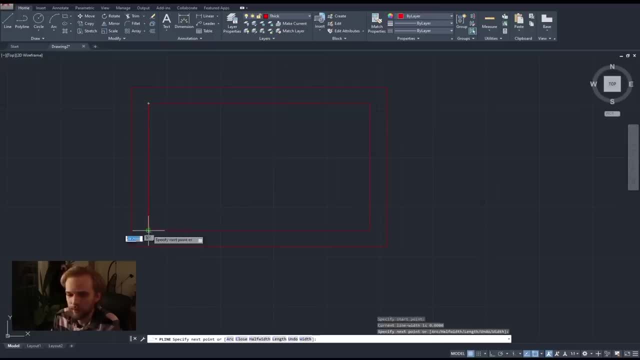 this corner point to this corner point, like so, and hit enter right. so now what i have here is i have a duplicate line right. there is this polyline here and also this line segment. the reason why i do this is because now i can take this line segment. 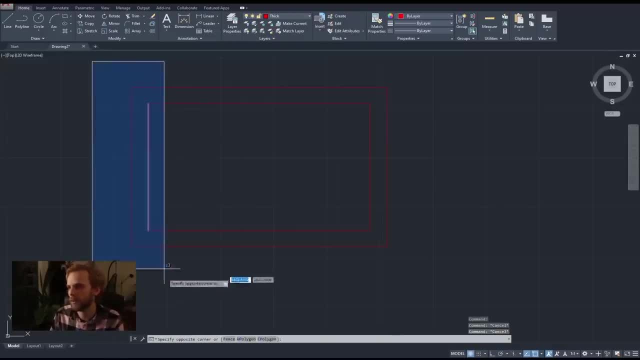 i can select it. if you have problems selecting it, you can always use the blue marking tool and just select it that way and i can type in offset and let's say how wide, how wide, so the smallest shower. that that is kind of nice, still nice to have. 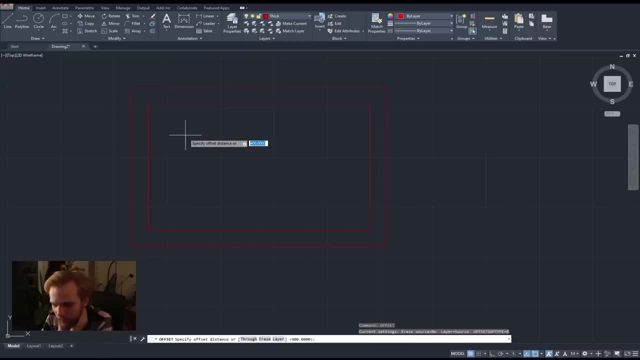 is around 900 millimeters, so we can't have it thinner like than that. so i will say 900 millimeters, instagram and choose. so okay, let's do instead of 900, i will do one meter at least. yeah, one meter. it creates an offset, right. 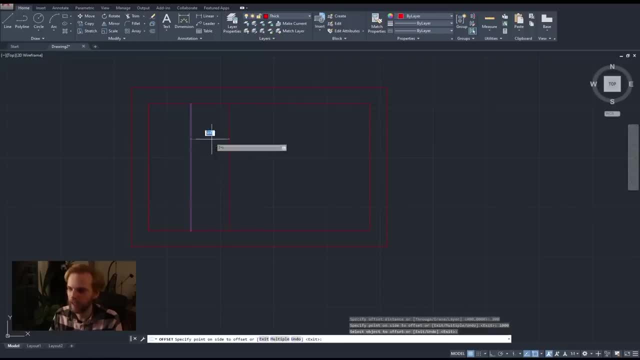 and now for this line. so this is going to be like a mark where my bathroom ends. so i want to place all my tools here in this particular space, to make this into a wall. so I will offset it again. I click on it and I'll type in 140 millimeters, 14 centimeters. that's enough for the inner walls, right? 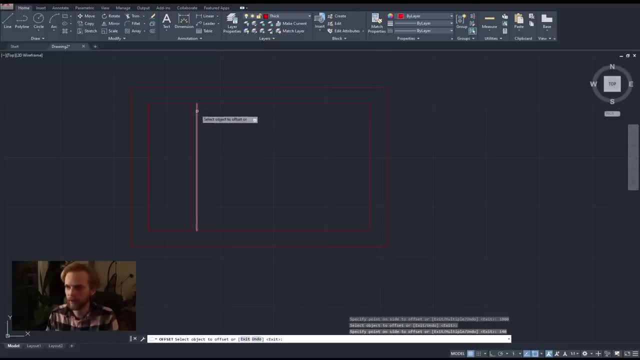 14 millimeters, and once I'm done, I just hit. escape or enter doesn't matter, and I have my my two line segments that describe an inner wall, right here. I still do have that line segment here that I used, right, but I don't need it. 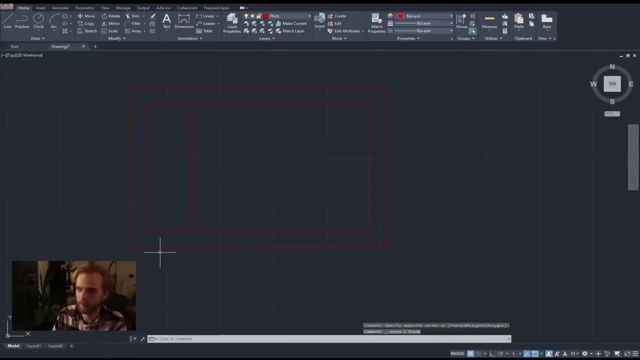 anymore. so I'll just select it and hit delete. let's get rid of it all together, right? so that's my two line segments. now what I want is: I want to get rid of this segment here and this segment here, but that is. trim right TR, enter, enter and then click. 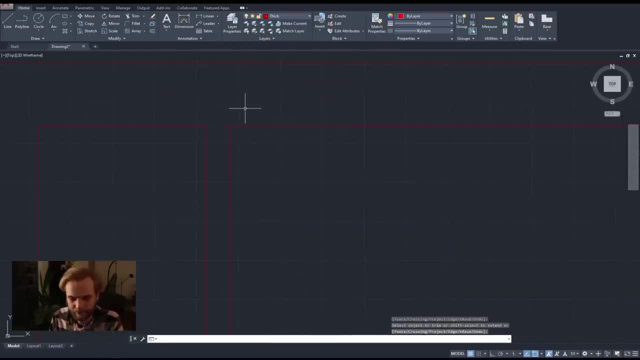 Lick, enter easy, right. I've just successfully deleted those two segments and now I have a room here and a room here. I don't have any doors or windows or anything, but I do have a room. that's one mirror here and all of the remaining areas looking like this a little bit. you can change in the default settings. so now, 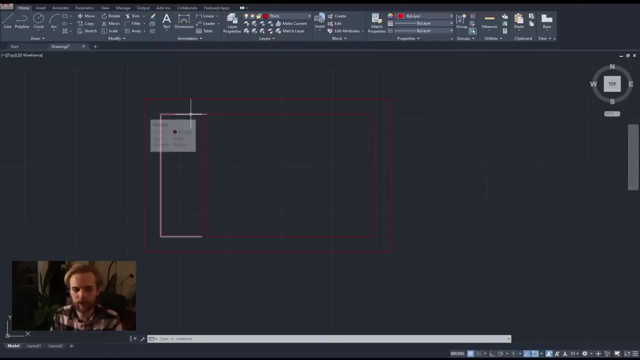 all these segments are down and I can just delete all the remaining areas, like get it here. this is not clean anymore, because this polar line and this line segment are two separate entities. I want to join everything up so that this is a rectangle, this is a rectangle and this is a rectangle, so that I have three. 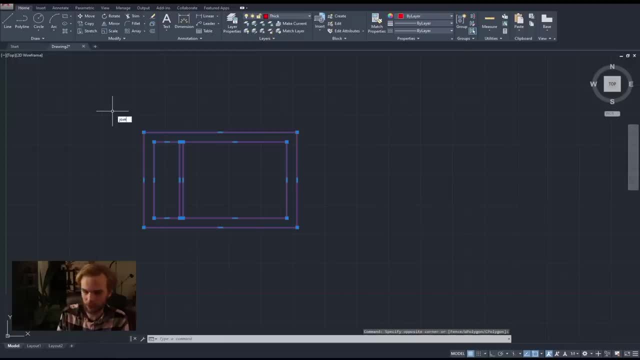 rectangles here, so I'll select all of it and type in join, hit enter and yeah, that's, it joins them up, right. so now this is a rectangle rectangle, rectangle closed. very important that they are closed, but that is that let's create an entrance doorway, right, or let's create a doorway into into the bathroom, right. so I'm going to create a 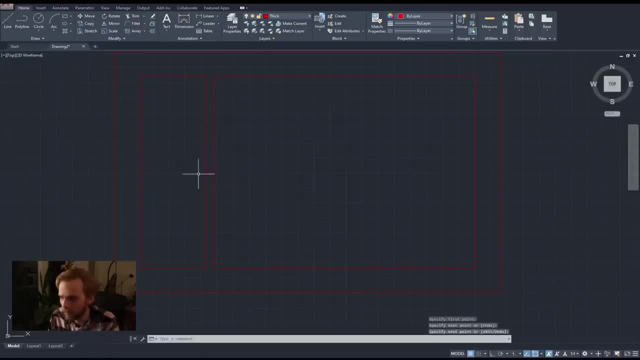 line segment, just from here to here, from the midpoint to the midpoint, because I want the door to be centered and the door is 90 centimeters, so the the door is 90 centimeters, so the door is 90 centimeters, so the the width of the door is 90 centimeters. the height of the door is usually two. point in between 2.1 meters and 2.2 depends on what kind of door you're using. but usually what I like to do is do 2.2 meter high doors and add, if I need to, then I add framing inside, so it kind of eats up a little bit a little bit. 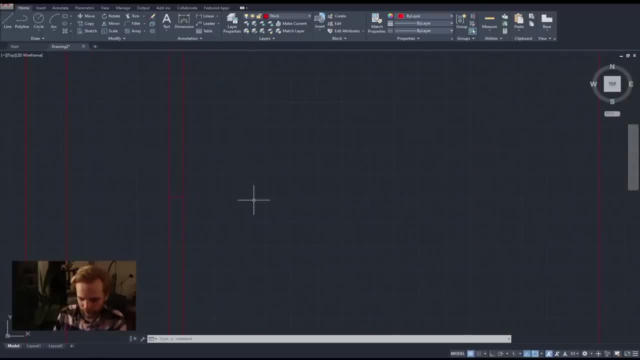 of that height. either way, we have the line segment. I will offset it. I'll specify the offset distance to be as I want to offset it to both sides. it will be 45 centimeters, so 450 millimeters. hit enter and now I can just offset it. 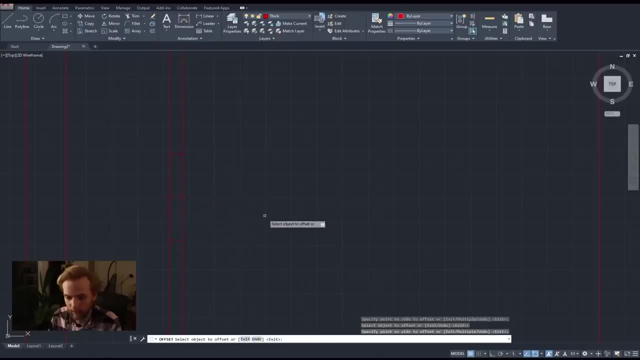 up and offset it down, like that right, stay with me. I hit enter. now I don't need the middle segment anymore, so I can just select it, delete it, all right, and I have these two segments now, so I'll say trim enter. I'll just trim away this. oops, trim enter, enter. always forget to do the double enter and 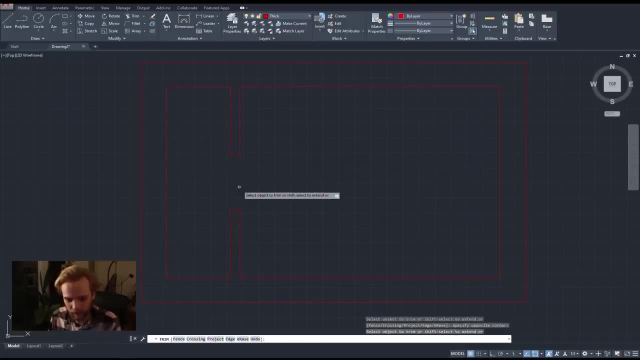 I'll just trim away these two line segments here, right. so now what I've done is I created the opening in the wall right for the door to be in and i can select all of this type in join, and now all of all of these segments are joined. so i have. 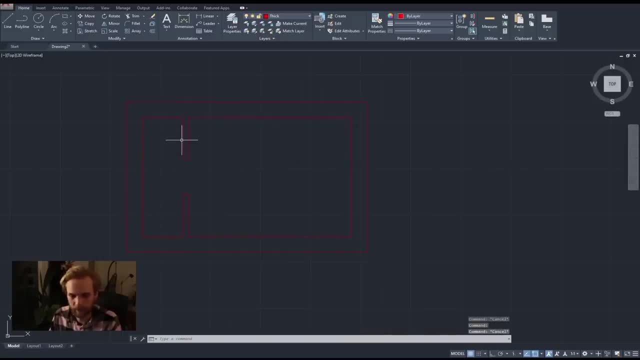 one polar line here and one polar line here. great, let's do this again. i will keep doing this, just so that you can follow along quite quite easily. so i want a door here right, and i probably want so. if there's a shower here, i do want to have a window. 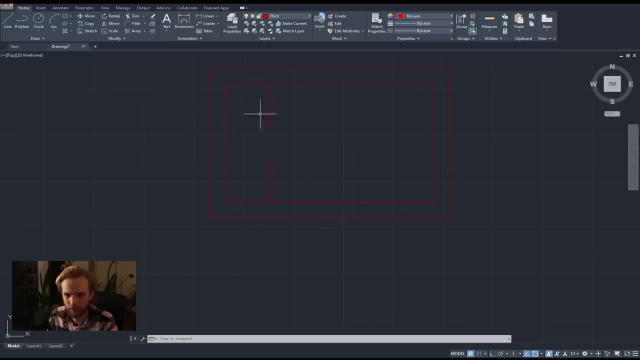 there's a toilet here. i do want to have a window here, right, um, right, so door window. okay, i will create a line segment from here to here and i will offset it, uh, by 900 millimeters to the side, like so, trim, enter, enter, enter, rather, and then the same thing here. 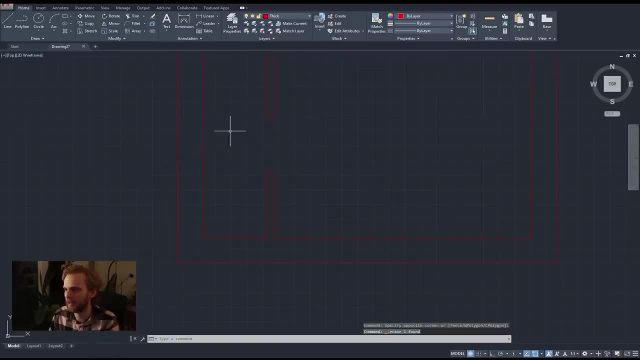 actually this one can be the the same size as the door, so i'll just kind of be cheeky about it and just start drawing from from the doorway like so trim, enter, enter, tr, not trim. god damn it. i keep forgetting getting tr for trimming and i create an opening here. so door, door, window, and it's probably going. 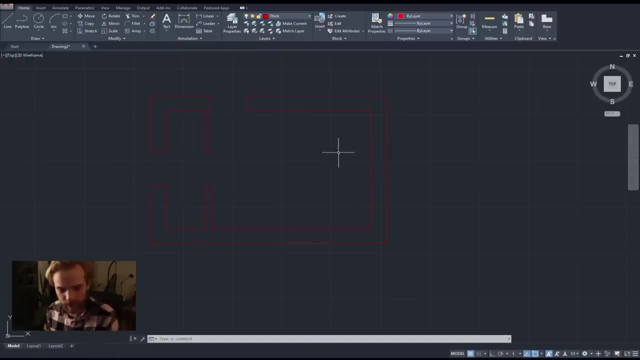 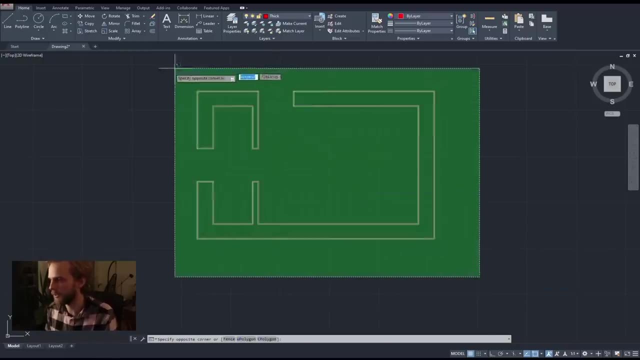 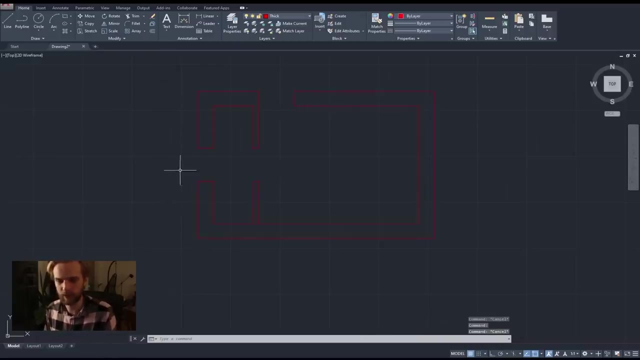 to have a window somewhere here, but we'll kind of take care of that side layer. okay, the thing is well, first of all, let's, let's clean everything up by selecting the walls and joining them up, just so that this is closed and this is closed, right so? 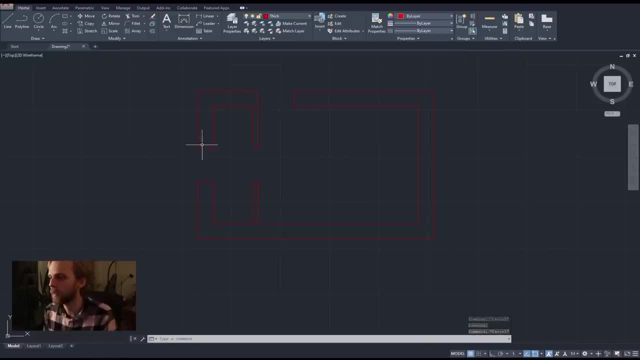 everything is kind of neat and dandy. the thing is that here, while we are cutting through the doorway here, we don't see the bottom of the doorway. all we see is just kind of floor, floor, floor, floor. but here the window probably will not reach the floor right? so that means that we will see the windowsill. 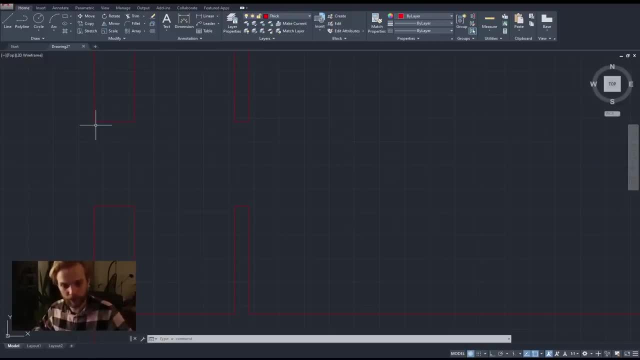 right. we will see the bottom of the window opening in the plan and i can not can. i need to show it right. so i'm going to go to the layers and i'll say that the layer in which i'm going to draw is the medium layer. so let's talk about this. just a second thick layer is used to specify all. 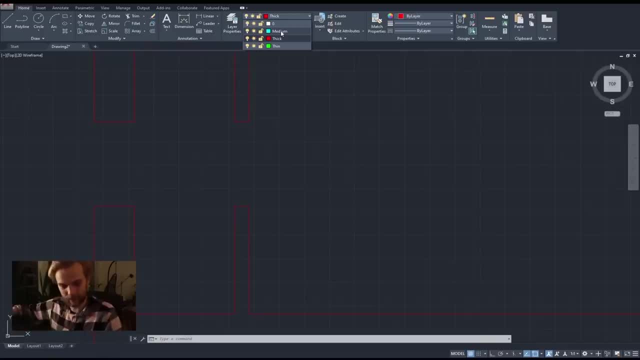 of the lines which you get from cutting something, right, so i'm cutting the walls right and i'm looking at the cut of the walls, meaning that they will be shown thick in the thick line. medium line is stuff that you see as a projection, right so you're not cutting through. 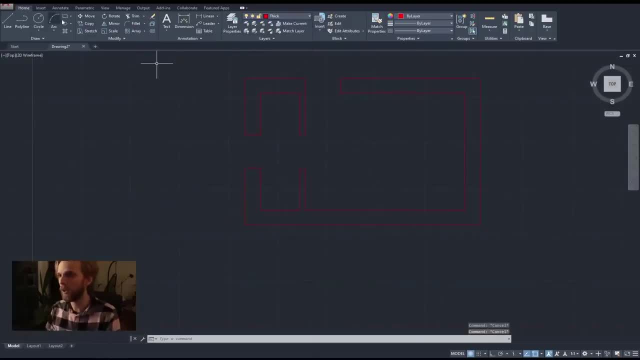 it, but you can still see it. so in this case, uh, if i have a, if i have a window- oh my god, wait, just bear with me- sure, that's fine. so let's say, i have a window. um, you know that that has some sort of partition. 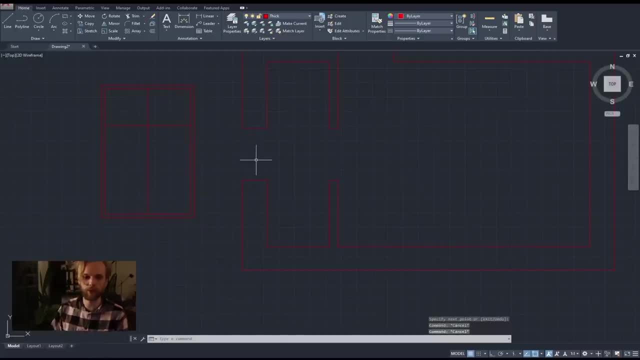 partitioning whatever is just a window right in in the, in the facade, and i am cutting through that window like so, right at this height, i'm cutting through it and i'm looking at it downwards. i'm looking at the cut, you know, straight downwards. that means. 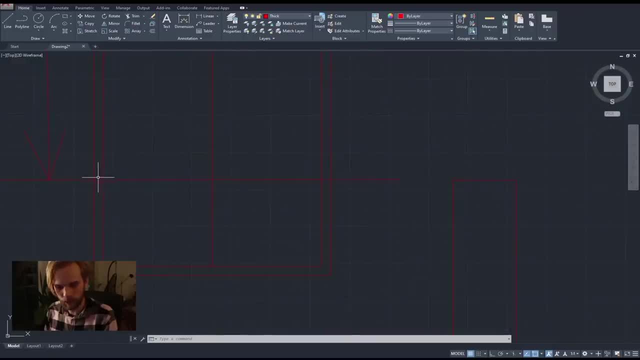 that i i will see the frame, i will be cutting through the frame, i will be cutting through the glass frame again and then wall right, so wall frame, glass frame, wall, but also i will be seeing the hole here. right, i will be seeing the windowsill, so that windowsill is not a cut rather. 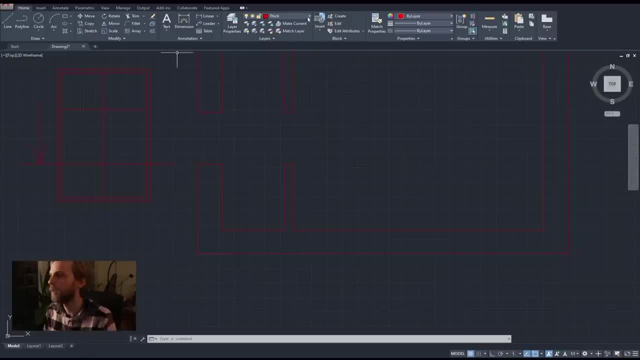 it's just a projection, it's just something that i see, meaning that i use a medium line, grab a line tool and i just draw it from here to here enter, or either let's just draw a rectangle instead, might as well follow line tool like that, that, that, that, that that's the windowsill right, and i still. i still have the red lines. um. 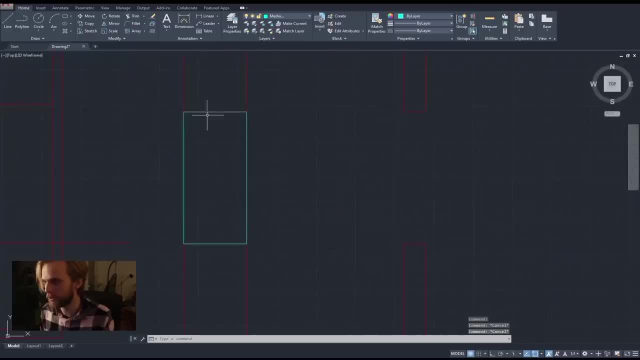 above it, i guess, like the cut above it. it's just that, visually, uh, autocad needs to choose which kind of geometry to show if there's like two geometries on top of each other. so you just choose to show the medium one. but we don't care, because we know that we have the thick line above it. 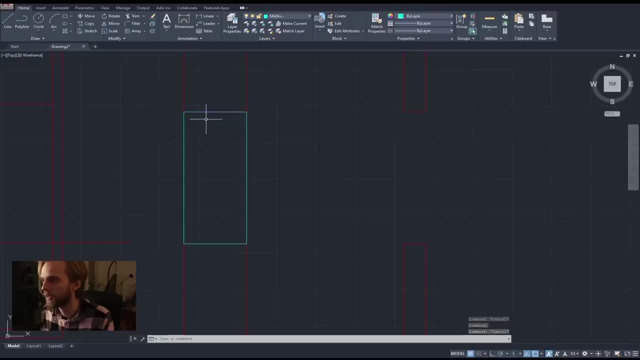 and my camera died just a second. god damn it. yeah, yeah, yeah, okay. so that's the window. windowsill right now for the frame. we'll do the frames in the next tutorial. um, for the doors as well, right? uh, as long as we have the windowsill is fine. one more thing is we have the floor slab right and then we have the. 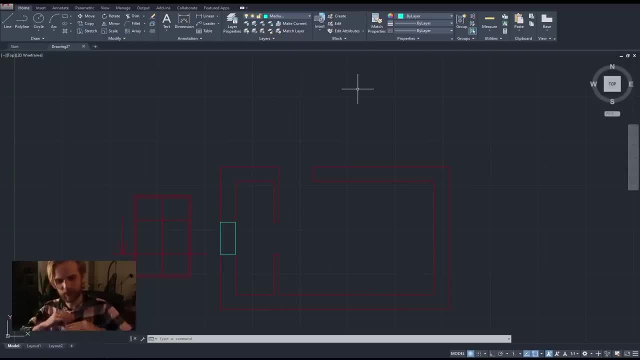 outside, you know the ground, the gravel and so on. those are things that are in two different heights and two different levels. right, because usually you have like a step or two steps near the entrance and blah blah, which means that there's a line where the floor slab ends right, where where the 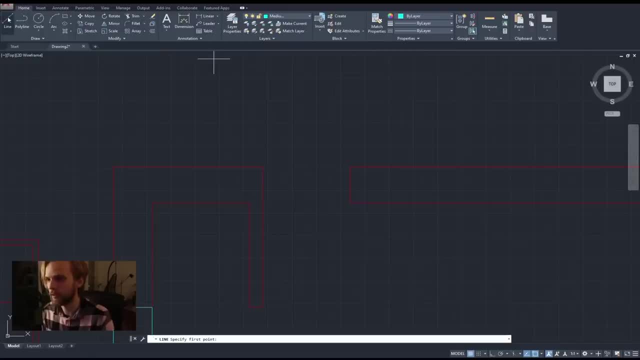 floor just ends. we need to mark that line. so i'll use the line tool and just mark it here. that's where my floor slab ends, right, so we have that going on now. nice, um, we will be adding doors here. the next tutorial: a toilet shower. it's a little bit gonna be a little bit tricky to plan out, but i will figure it. 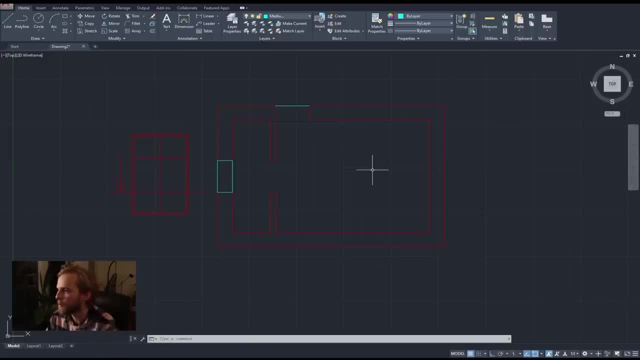 out. we will figure it out. for now, um, this is all that you will learn today, so thank you for watching. i wish you good eighty years, Cya next time. bye, bye, bye. have a nice day and i'll see you on the podcast. bye, bye. 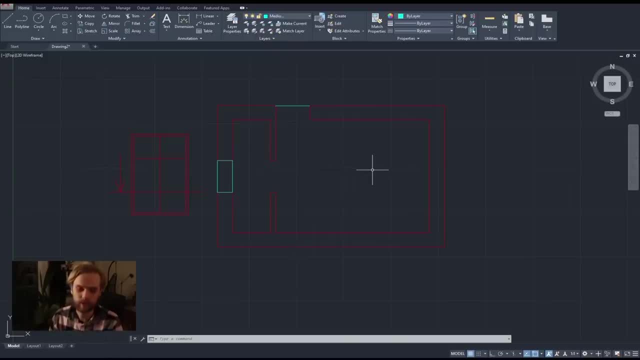 bye, bye. you need to do, uh, practice, practice the lines, practice the tools and so on, and draw out the, just the walls with the openings shown right properly. so this is that one. this is the level of detail that that you should have after the first day of tutorials. 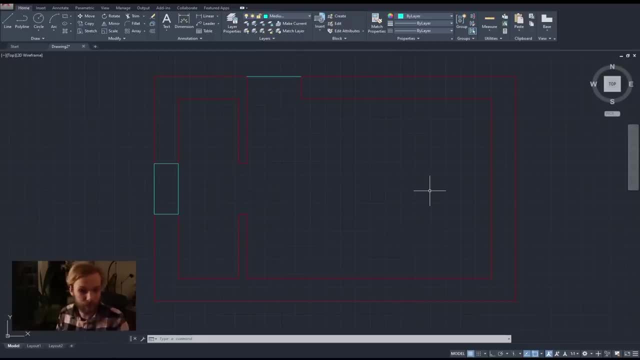 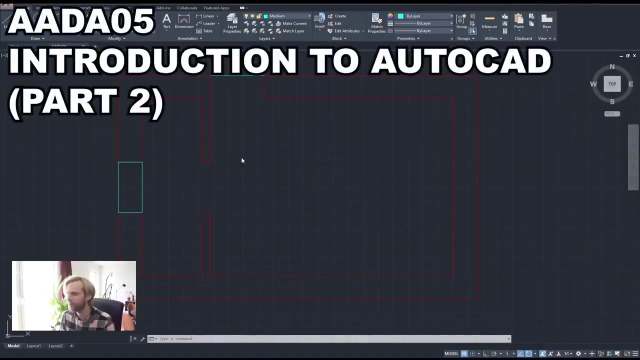 next up. i will not need to show you every tool, so we will make a lot of more progress in terms of of drawing in the next tutorial. for now, get to work and have fun. bye, all right, hello, hello, and this is going to be the second part of our tutorial series for router cat. 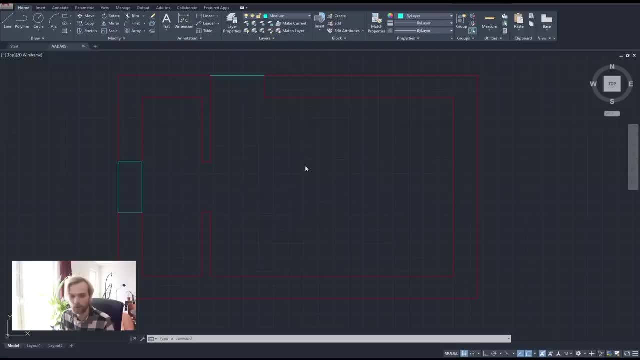 where i'm going to kind of continue on working on the plan and hopefully we'll move, move forward with the section and so on. so in the first part i've already showed you most of the most of the tools that we're going to use. so here it's just designing, right it's, it's just. 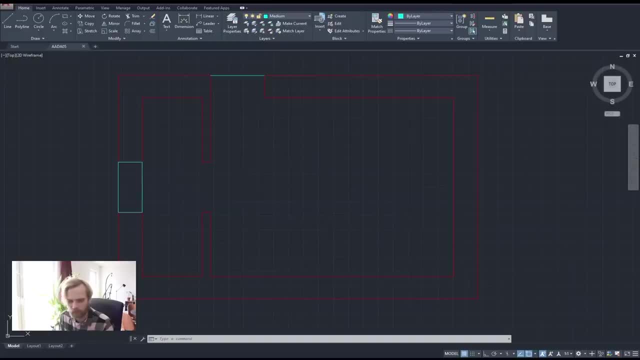 adding geometry into our plan. so let me- um, yeah, let me- keep the camera there. that's fine, should be okay, okay. so we finished off by creating openings here for the window, for the doors and whatnot, and creating a little room for our sink to be in. 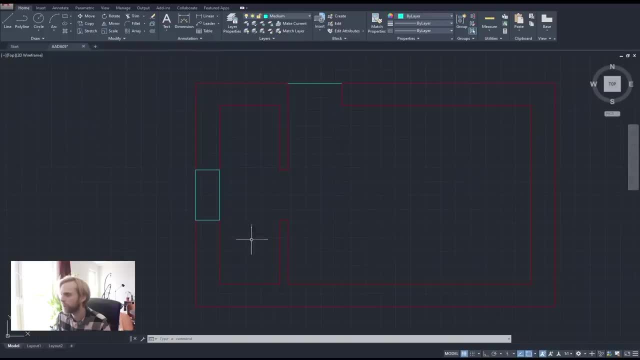 well, it's probably going to be somewhere here- the shower and the toilet, so let's continue. so the the thing that i want to do is probably add a little bit more detail into the window, a little bit more detailing to the doors and whatnot, and then continue on working with this area right here. so, first of all, i'm going to create a window. 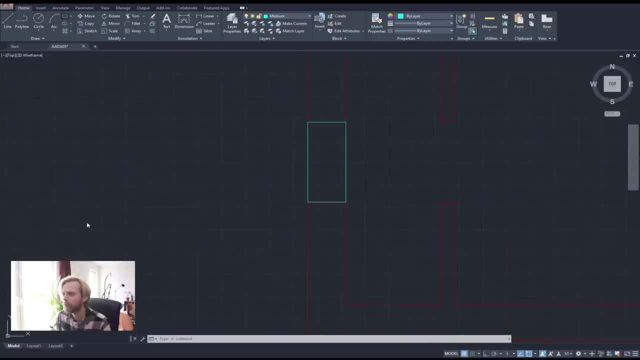 so remember where i showed you before. if you have a window like that- and i'll just draw it in 10 lines without any thicknesses- let's say you have, you know, a regular window in a facade. you want to, and it's in the hole in the wall right and you're cutting through it like so. 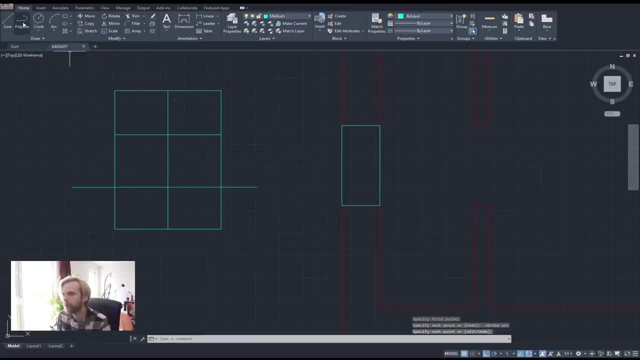 so, and you're looking down on it- right, you're looking downwards, through the cut, you're cutting through the wall. right here and right here, you're cutting through the wall, you're cutting through the glass and you're cutting through the frames of the window. so if you have divisions, you would be cutting. 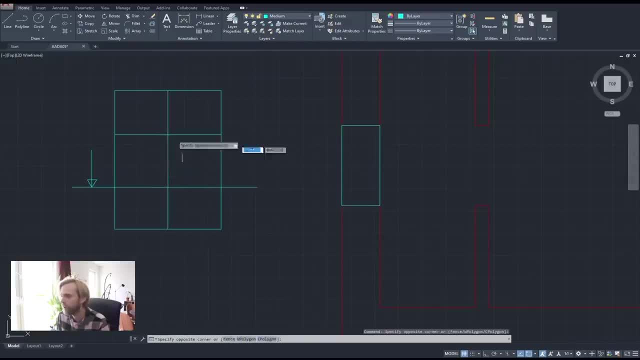 through the middle frame as well. but i think for a window this size we don't need any divisions. it's just going to be: why is it lagging? let's do 50. it's just going to be this kind of window. so we're going to cut through the frame here. 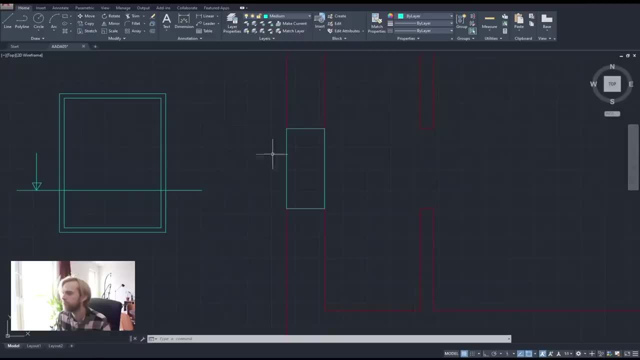 through the glass here, through the frame here- right, let's do that. uh, window frame. uh, what i prefer to use is five by five centimeters. right, it's not accurate, but that is enough for our level of detail that we're going to be using. so, since we are cutting through the frame, i'm going to be using a thick line, right, and i'm 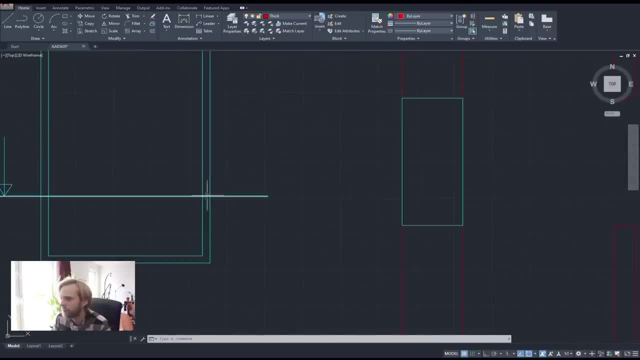 actually going to just draw the, the cut of a frame anywhere on on the screen- doesn't matter if i pull a line to it- and i'm going to enter it with a new line and i'm going to hit that white笑y circle and just hit that f8 button or ortho, ortho, snapping on um so that it's horizontal, or 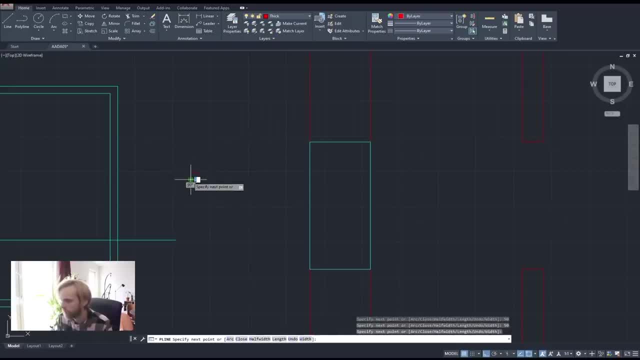 vertical and i'll just give it: 50 enter to the side, 50 enter side, 50 enter. there we go, something like that. so you could do a rectangle, but i just, i don't know, i'm used to drawing it in this frame and place it in the middle of this opening here, right on this side and on this side. 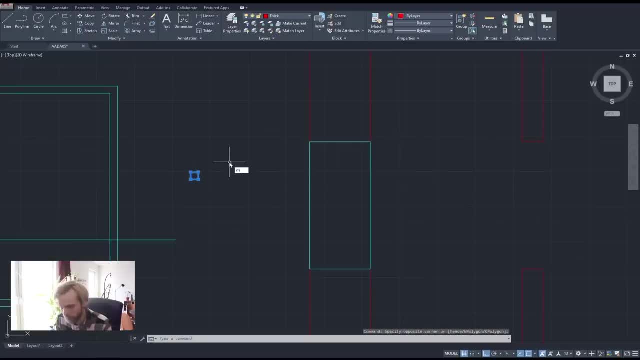 so I'm going to take the frame, I'm going to move it, M enter and I'm going to move it from its, let's say, top middle point here all the way out to the middle point right here. uh, right here. there we go. click, now it's here. then I just take it, I copy it. 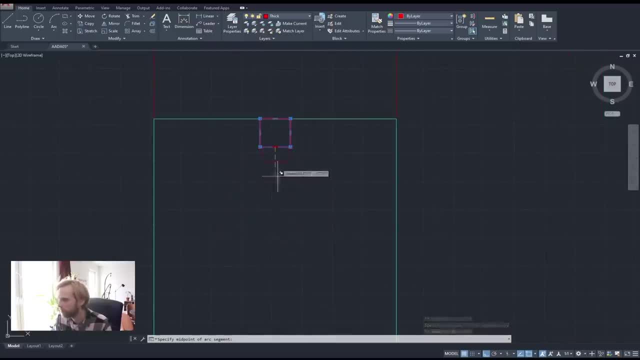 by by using the command copy. for some reason, it's not making a copy, I don't know why. let's try again. copy from here to here. here we go. now we have a cut through the frame right. so this area right here is done, and this area right here is done. now we will be cutting through the window as well. 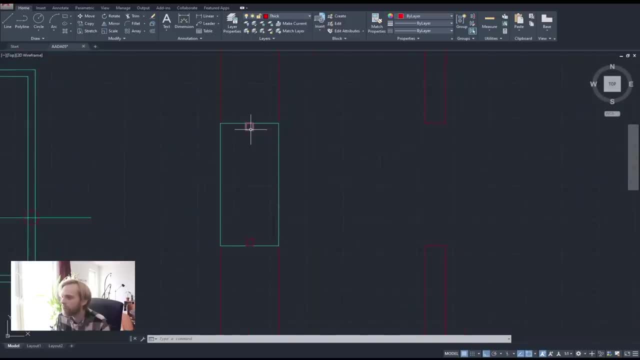 through the glass. sorry as as well. and for the glass, since it's- uh, this is just graphics, but I prefer to do it this way, since we are indeed cutting through the glass, you would think that we will be using a thick line, but since glass is inherently transparent, 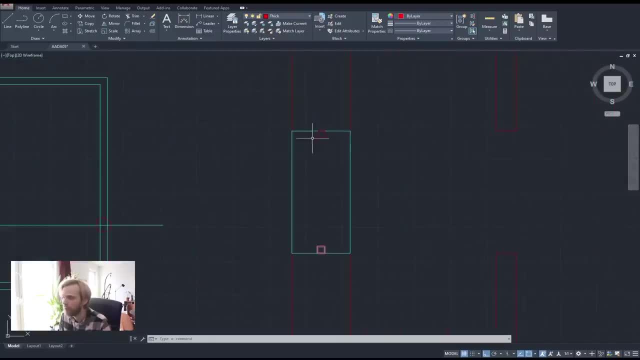 um, I prefer to use a medium line thickness for it, just so that it's not too thick, right, um? so let me jump to the medium layer and just draw a line from the midpoint here to the midpoint here. so that is our glass in the window. the thing is that if, if you think about it, we are cutting, indeed cutting through the glass. 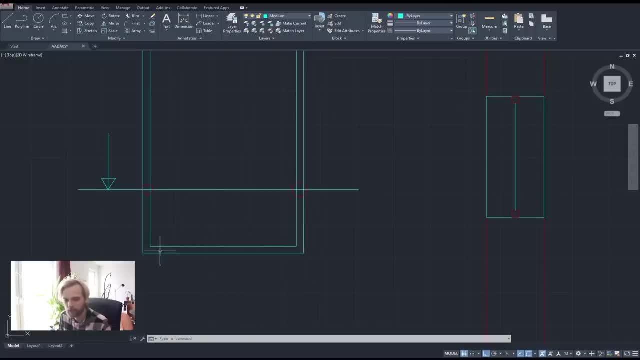 are also seeing the bottom of the frame right here, right, this, this edge, right here, will be seen right, which means that here we need two more lines to show the bottom of the frame, and for those two lines, uh, since i'm using a medium line to show the cut through the glass, i will be showing those two. 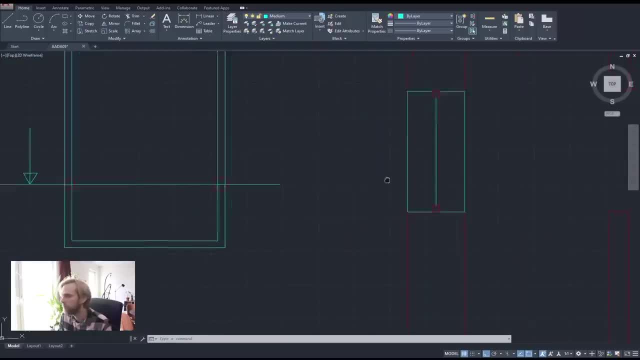 lines that we actually see at the bottom of the window. uh, as a thin line. right, i will represent it with a thin line. the reason why i'm doing this? uh, the reason why i'm doing this is because once we print it out, or plot it out as a pdf and we have it zoomed out, 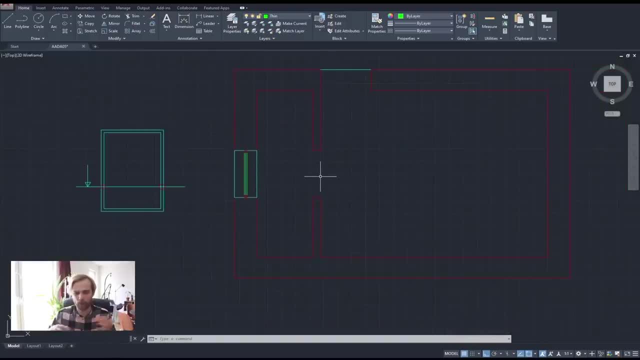 i don't want these three lines to merge into one thick, one right, just just because we are so zoomed out and the thicknesses eat each other up, right. so i have them separated into two thin lines and one medium line, rather than thick and two medium lines, which would be a little bit more accurate. but 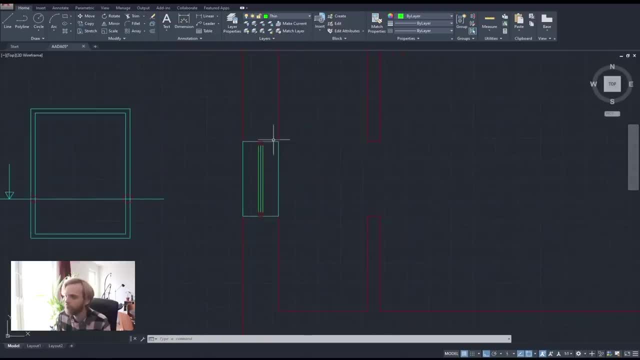 wouldn't represent the window that well, yeah, that's basically it. we. we have a window now, right, we have the glass, the bottom of the frame and the cut through the frame right here. okay, window is done. now the door. um, perhaps we should use. where do we? on which door do we start working? 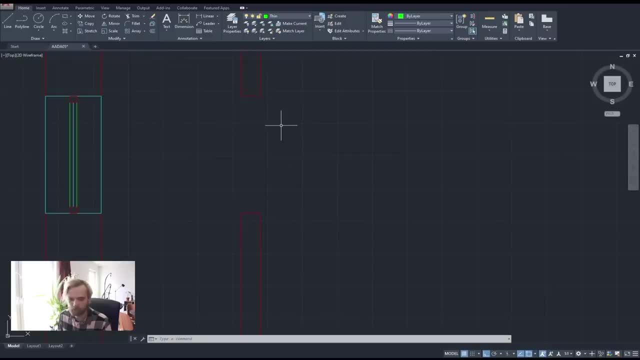 on. let's work on this one, right? so the door is, uh, it's basically drawn. um, i can show you somewhere here: the door is basically just drawn, as always being opened, unless it's, uh, re reconstruction project and you already have existing doors in the previous project, which 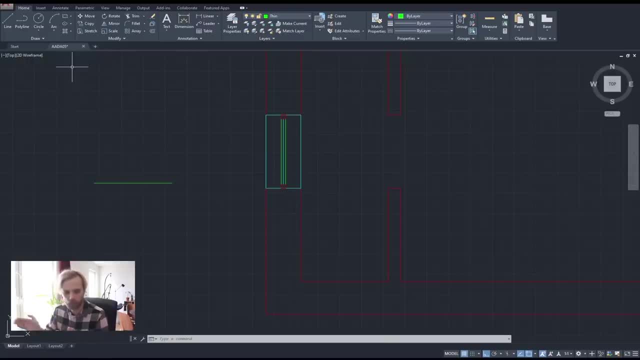 you reconstruct, then those doors are usually shown half opened at 45 degree angle, but in this case, since these are new doors, we are going to be showing them at completely opened, at 90 degrees angle from the, from the wall, and they will incorporate a door swing like so right? well, not. 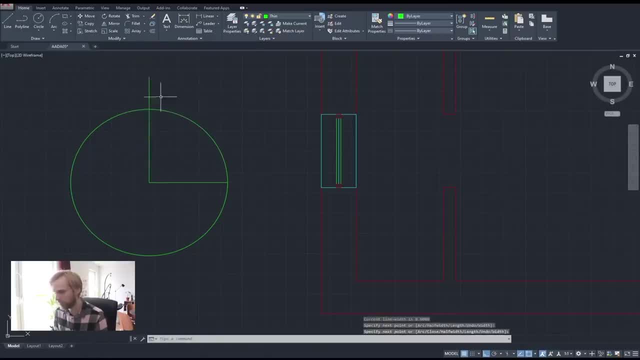 like. so actually i'm going to make this quite fast, like that. so it's going to be the door swing showing the travel of the door when you open it up, as well as the door itself being opened. the door is shown in a decline because you're cutting through the door and the 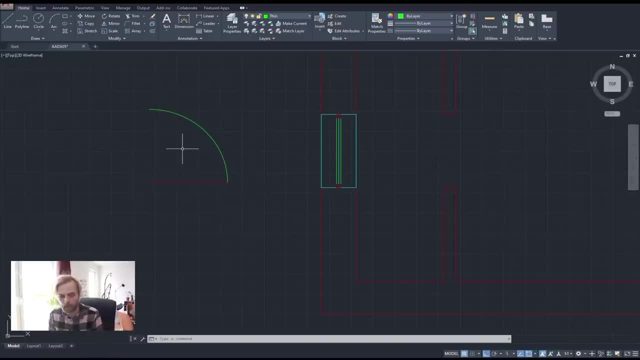 opening of the door is shown in a thin line because it's a non-existing geometry, right it's? it's something that you just use as a markup to show the travel. so you don't even need to have a medium line for that. it needs to be a thin line. so that kind of doorway needs to be here, needs to. 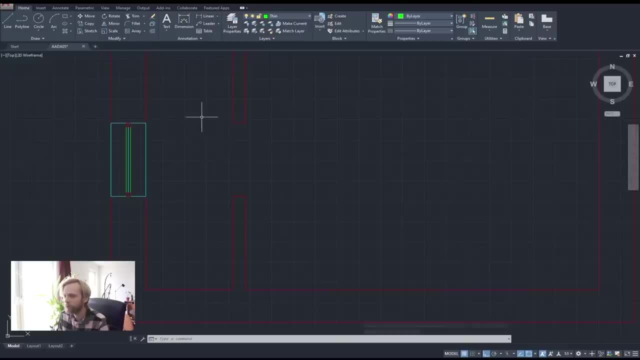 be incorporated here. so the way i i really like doing it is by creating a line line tool here. um, do we do it that way? maybe we want a little bit of an offset? okay, let's first do a little bit of an offset. so i will create a line, or or rather two lines, from here to here. 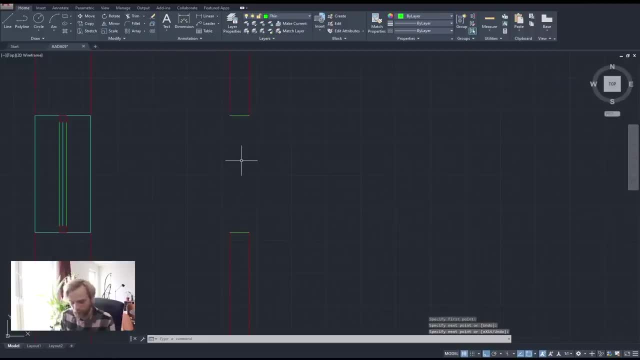 and from here to here, these two line segments and i will give them a little bit of an offset. so, for example, i will just use a five centimeters at most. we can do even less. we can do two centimeters, it's up to you, but i prefer using five. so five centimeters enter, i'll just offset. 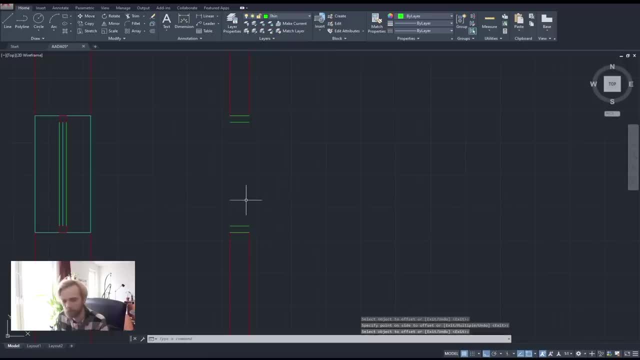 that line inwards, like so, by five centimeters, and that line inwards, like so, also 50 millimeters, five centimeters. so now we have um these two floating lines here and these two guidelines that we first had. i don't know what i call it- you can see them on the screen, but at least the 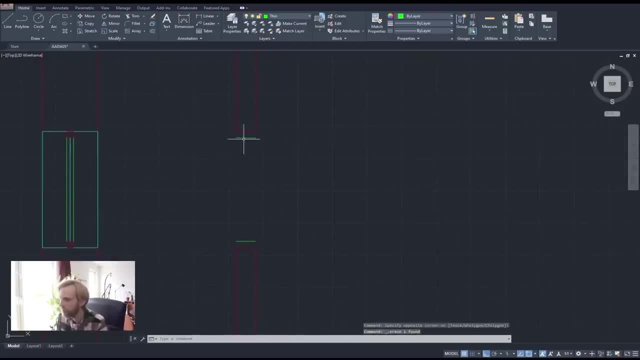 lines have been converted to be the same size and the shape of the plane, as you can see here them anymore, so i can delete them so. so this is a bracket in which our door is going to be held, and treat these two lines as your helper, helper lines. right, we will be deleting them. 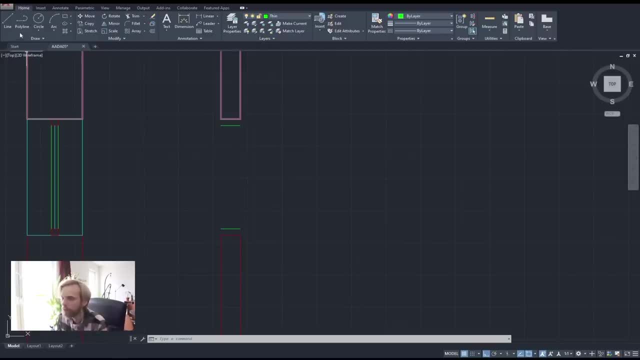 later on. so now, what i do is i create a straight line segment in a thick layer, from the midpoint here to the midpoint here, like that, right, i select it. and now i want to open up the door right, so, uh, this doorway or this door board, i want to rotate it right, so i'm going to use a tool that's called 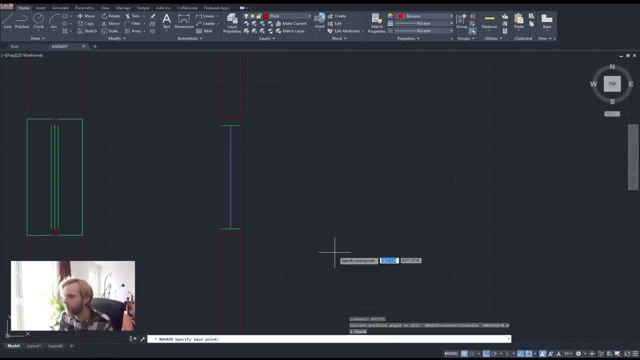 rotate, rotate, enter. it's going to ask me to for a point around which i'm going to be rotating. so let's say the door hinge is right here. that's that point, and basically then i can just either move it like so, move the mouse like so and click, or i can type in 90 degrees. 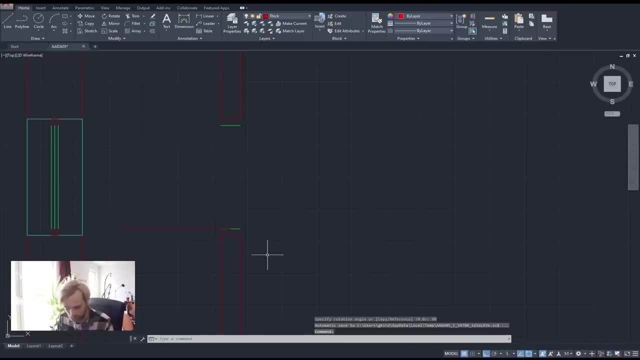 and hit enter. well, not 90, sorry, minus 90.. so apparently, if if you add positive values, it's going to rotate counterclockwise, if you had negative values it's going to rotate. oh sorry, negative values are clockwise, positive values are counterclockwise. 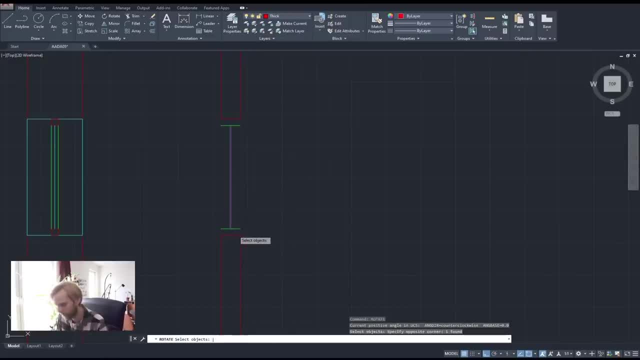 so again, rotate, select this object, enter, rotate around here, minus 90 degrees, there we go. so now it's. it has been opened and now all i need to do is just create that arc right, so i can either use a circle tool and trim away stuff from the circle tool, or i can just use arc. 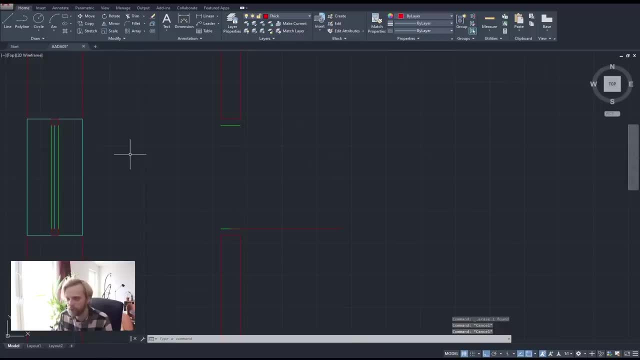 well, let me show you it then, in both ways. so let me do it with the circle tool. first, i will create a circle from here to here, from the midpoint here to the end of the door here i will create one more line: from midpoint here, midpoint here. 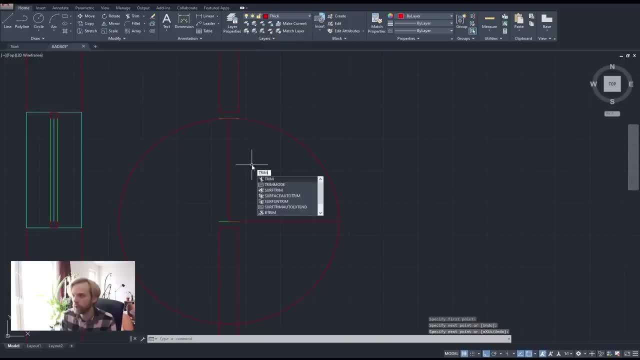 like that, and now i will trim, enter, enter again and i'll just get rid of the unnecessary parts of the circle to just get that arc there. and now i can delete all of the necessary stuff and change the arc of the the doorway right of the door swing. so that's that. um, i will show another method. 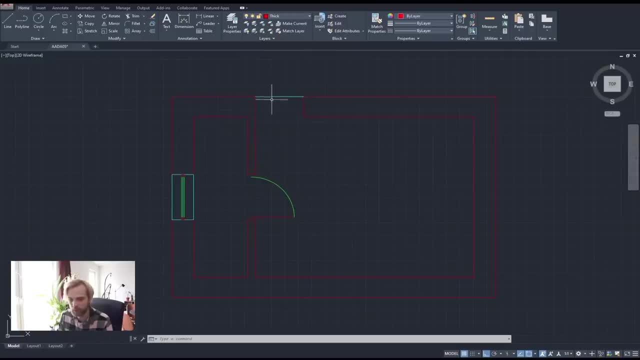 of how to create that arc in this version here, because we need a doorway here. so let me do the same thing first. from here to here, we have a line segment. from here to here, we have line segment. i offset them, uh, 50 millimeters. offset inwards. inwards, escape out, delete the trash or the. 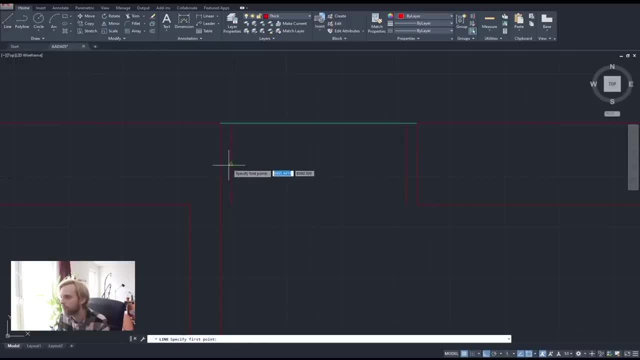 helper lines like that great align segment, bam, something like this: rotate to 될, rotate that one. and this time around it's going to be jet trace react z equal to z, log integral of z for our x field. its gonna be something like that of all these layers to take effect and get scared. so that's different. but if we don't mind connecting, we're doing the same thing first, from here to here, we have a line segment. from here to here, we have line segment. I offset them 50 millimeters. offset inwardsisión a sina. 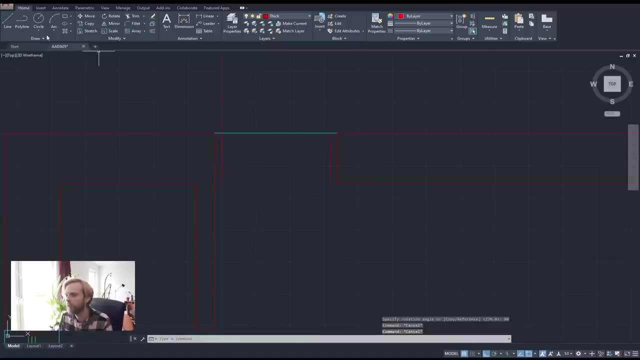 counterclockwise, so it's just going to be 90 degrees, like that. and now what I can do is I can just create an arc, let's say arc tool or a enter, and I will say that the center point of the arc, or rather I will not be using start point of an arc, but rather I will be using the center mode- 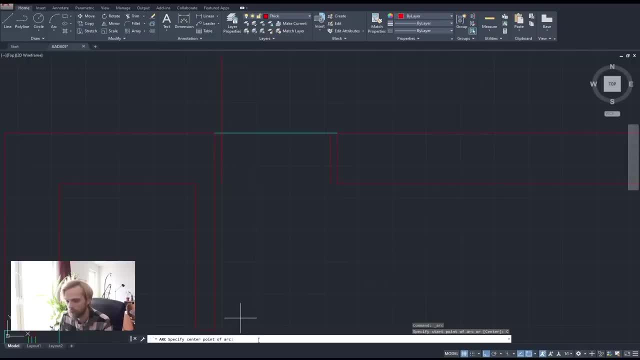 for the arc tool. so I'll click on that in the bottom, which will ask me to give it a center. so the center is going to be located right here, where the door starts, right here, and I'm just going to draw an arc from this point to this point. that's it. that's. that's an arc that has been created. 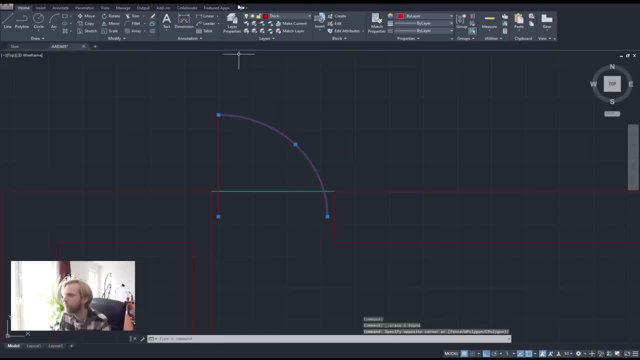 now we clean up the trash again and change the arc layer to thin. that's it, so that those are two, two different methods of how you can actually use the or how you can add the arc. sorry about this, okay, moving on. so we have two doorways. we 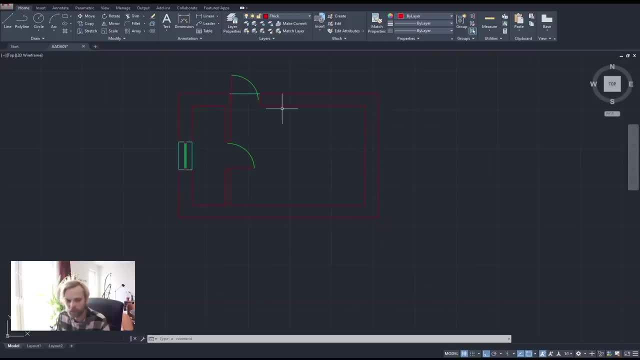 have a window. perhaps I want a window here as well, but first of all I need to plan out how my whole room is gonna look like. so let's say we enter here, we will need some place to put down our coats, and we will need some sort of a place for. 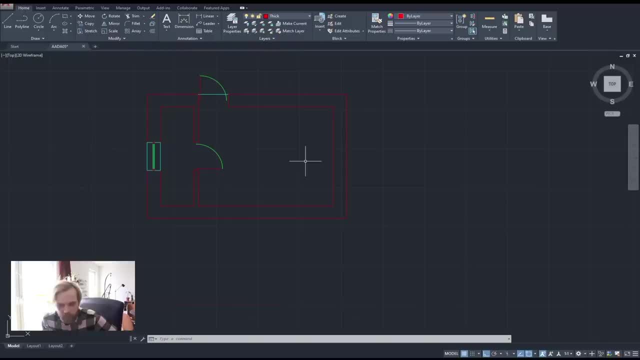 a for a bed and it's just going to be a small bed because we can't have a large bed here. so let me just create just to see the proportion of the room. let me just somewhere else on the screen, let me just create a size of a bed that that I. 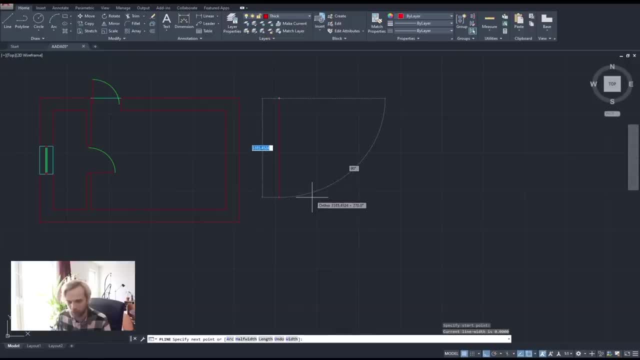 want and it's going to just be. I'm drawing it with polo line 2000, 100 millimeters long. I'll go for one mirror, 10, 1100 millimeters wide, 210 or 2100, and close off the fall line. so that's my bed and it's going to be in the 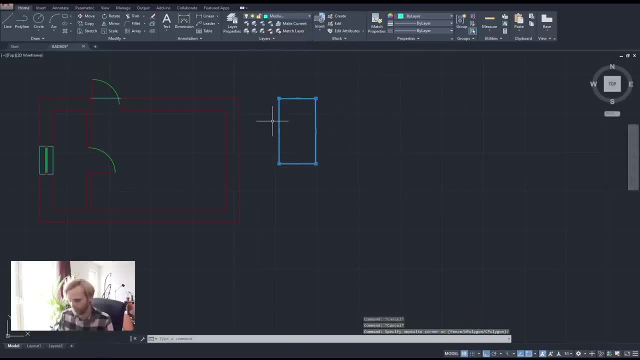 medium, medium layer. I'm just going to move it somewhere here and start planning out how, how everything is going to be kind of arranged, how everything is gonna look like. that's not great, let's see, let's see. let's see if we can make it better. I'll 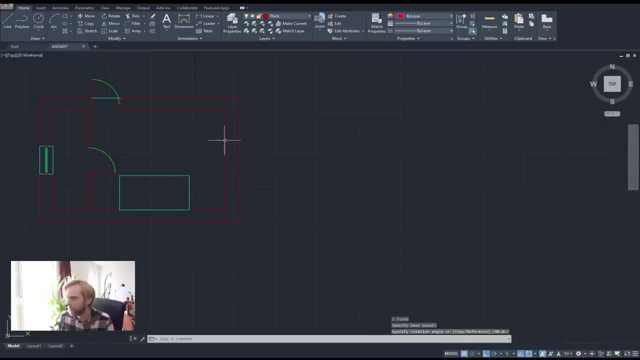 rotate this from here here. there we go. reposition this here: that's a little bit better. we can have a table here, but the door is going to be obnoxious. that's fine, we can work with it just like that. so now I can choose a place to put down my 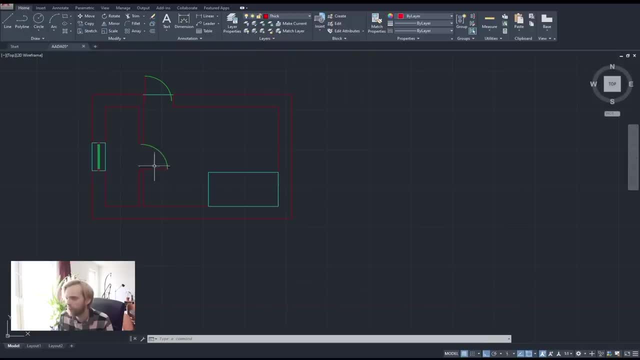 we can flip the door around. let's see how wide the table is going to be so i can check the distance here. i can measure the distance by typing in dist for distance, enter and clicking on two points. so from here to here, give me the distance, and right next to my cursor or also above my command line. 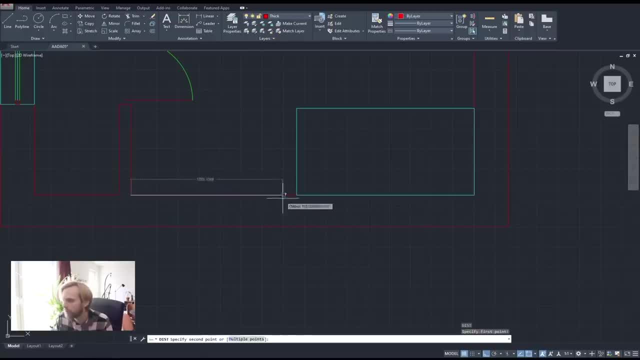 well, we can't see it anymore there. i will see the distance. so let me try that again: 1960 millimeters, 1.9 meters, that's a lot, that's, that's uh, that's quite enough, uh, for shelving and also the the table. so i'm gonna do that, i'll create a polo line. 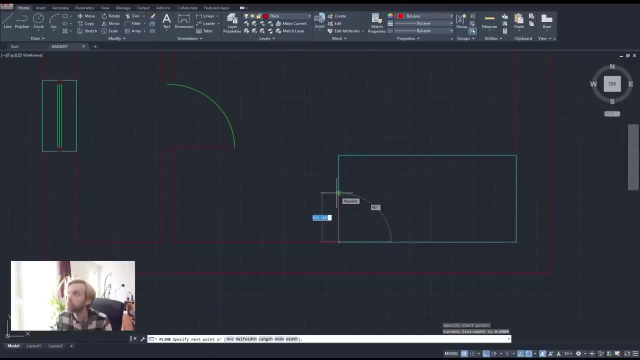 and i will say that my table is, um, let's go for a pretty thin one, let's go for 600 millimeters, years, 600, enter until here, here. here, there we go. and this block is just going to be representing my, my table, right so bed table, there's going to be a chair here and then this door is in the way, right. 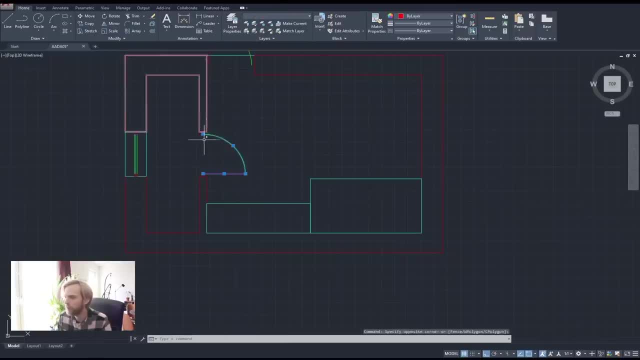 it's just messing everything up. so what i'm going to do is i will mirror this door so that it opens up here. the way i do that is just i'll create a line in the opening just to have the midpoint of the line. i will select the door, i'll type in mirror and then i will use the midpoint of that. 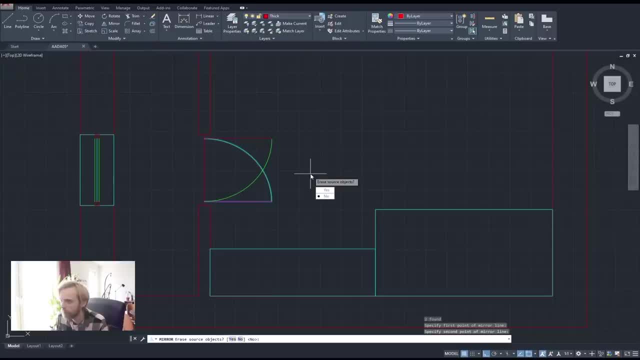 line. i'll mirror the door horizontally, like so, and when it asks me to resource objects, i'll actually say yes, right, so that it deletes the old version. that's it now. it has been mirrored, quite easy. um, as you can see, most of the time i have orthographic snapping turned on for this. 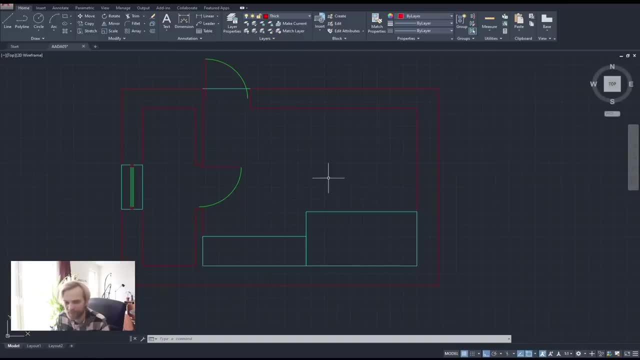 project. um, yeah, that that is how it is okay. so we enter really hate the. the entrance here, though, like the flow is really bad. i'll solve this later. i think there's there's, there are ways of how to solve this, um, but for now, let's continue. so now i 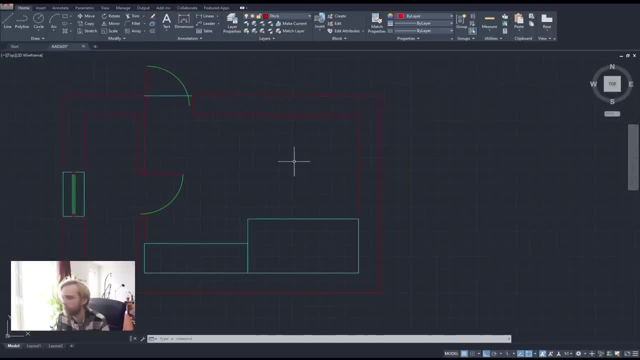 need a kitchenette, right. so kitchen cabinets are always have. kitchen cabinets always have the same module size and it's always 60 by 60 centimeters. so the refrigerator, the stove, the, the sink cabinet, all of them have 60 by 60 centimeters, so that's a lot of space for the kitchenette. 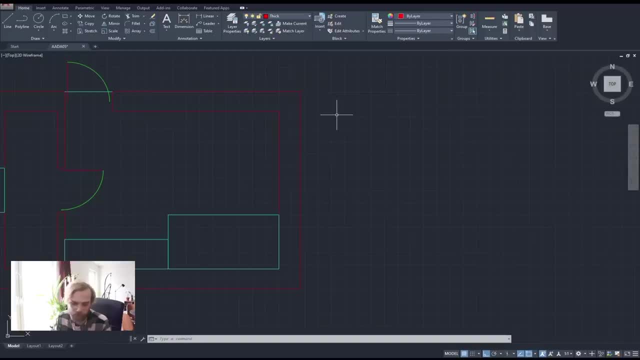 all of them are 60 by 66 by 60 centimeters. that's the not regulation, but the default value, let's see. so i'll switch to medium and i'll just create that single rectangle of 600 mill by 600 mil by 600. 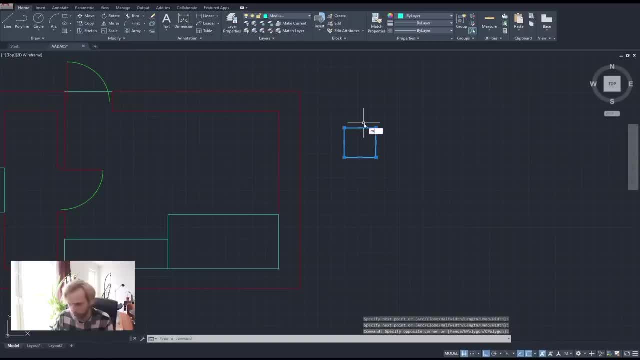 like that. that's our single segment for the kitchen, and i'm thinking of having the kitchen. So that's, let's say, that's our refrigerator copy, That's going to be our sink, our stove, and or rather maybe the stove is here, the fridge is here, the sink is here and the cutting area and food preparation area is here, right? 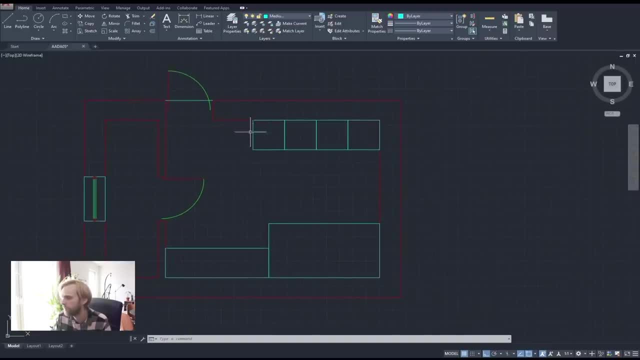 So we have that. That's good enough. I think that's good enough. And now I can add one more wall right here Just just for- how do I call it? Just a separation, you know, kitchen from the entrance. Also, it will create a little bit of a hallway here, which is fine. 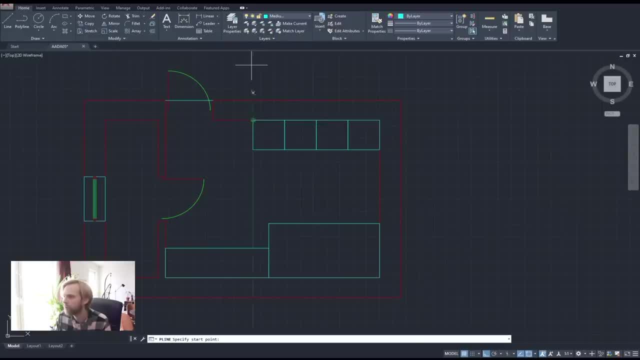 So I will create a poly, I'll just draw out- Well, let's go for thick line. I'll draw out a wall, but I don't really know how long the wall can be. So what I'm going to do is I will create an offset for the bed, offset for the bed, and I'll give it like 900 millimeters, like that, Right. So now I know that this gap right here is walkable and it's it's easy to walk. 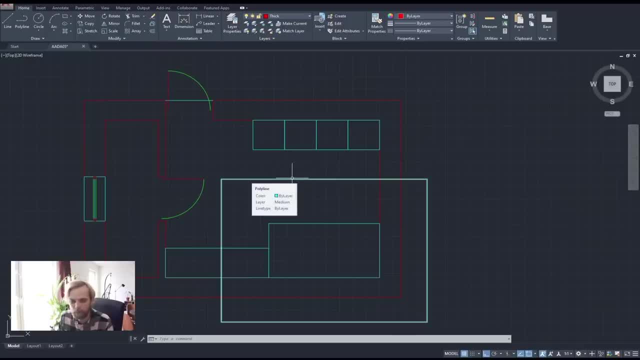 And yeah, so basically I am able to walk around it. So now I know that the longest wall that I can have is something like this: right In the gap between here, I will create a polyline now, draw it out like: so I'll give it 140 millimeters to the side and finish up here. finish it up here. 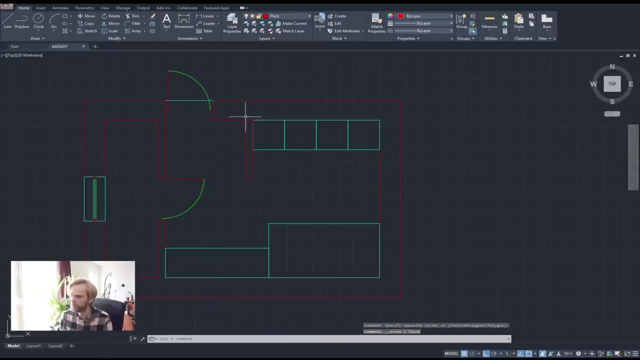 And now I don't need the helper line anymore, So I can delete it. So that is my second partition right here, which I think is fine. You enter, you put down your clothes, you can work, you can sleep, you can use the stove or you can prepare food and you eat where you work. Yeah, that's fine, That's, that's reasonable, I think. 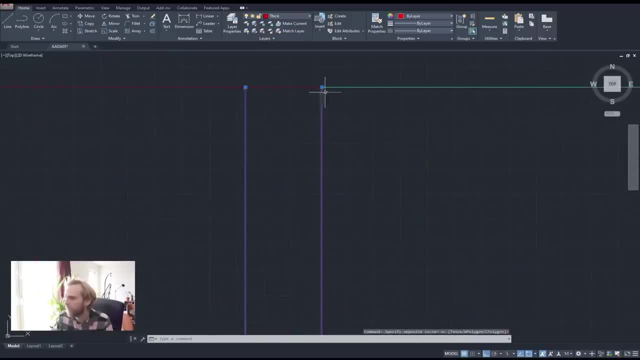 So here, right here, I have a line segment that I don't need in the wall because, you know, my wall kind of continues on here. So I will just trim it away, trim, enter, enter, get rid of that, And then I'll join up these two line, these two separate segments, this one and this one. I'll just type in join to join them up and make it a closed polyline, to just have it clean. 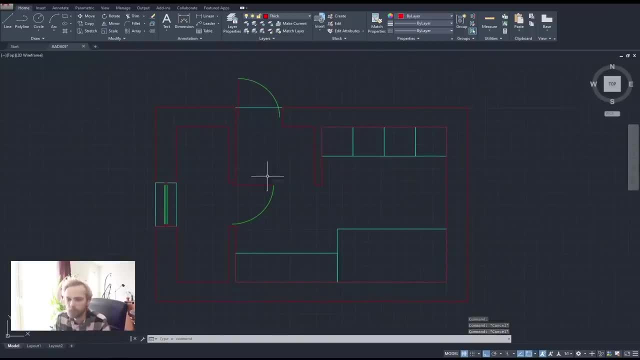 Okay, once you enter, you want to put down your clothes somewhere, So I will create a little bit of a shelf. I guess not a shelf, Let's just call it clothes storage. right, I'll create that and it's going to be. let's go for 500 millimeters, 500 mil, like that. 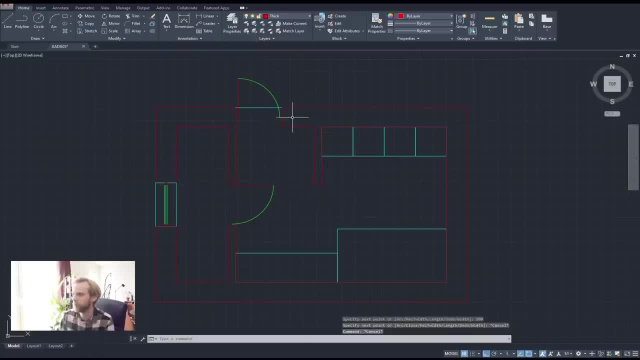 I have no idea how long this is Actually. before I create that, that area right there, I need to measure distance from here to here. 1.2 meters. We have 1.2 meters for that. Sure, 1.2 by 500 millimeters, So 1200 by 500.. Sure. 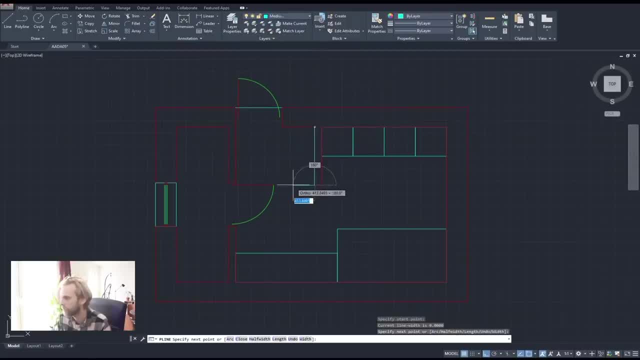 I will switch to medium line and I'll just draw it out from here: 500 to here, 500 to here to here. This is where we put our clothes right Now. I really want to solve this, because this is kind of obnoxious- that you need to close, have the door closed. Of course, you, most of the time, will have the door closed and it's going to work, but visually it's not that nice. 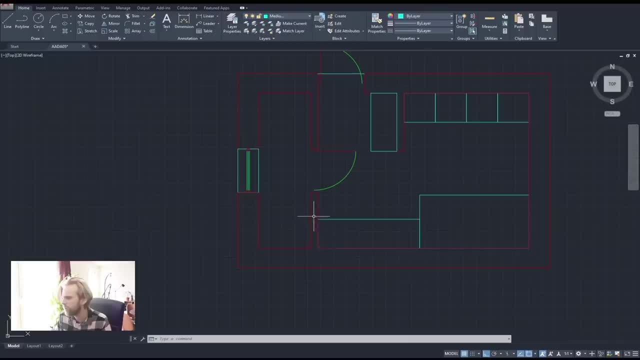 So I am going to probably create a total toilet here and see how far I can move this doorway away from the, away from the desk. So the toilet is well, actually for the toilet. you can consult Neufeld or you can just go to Google. 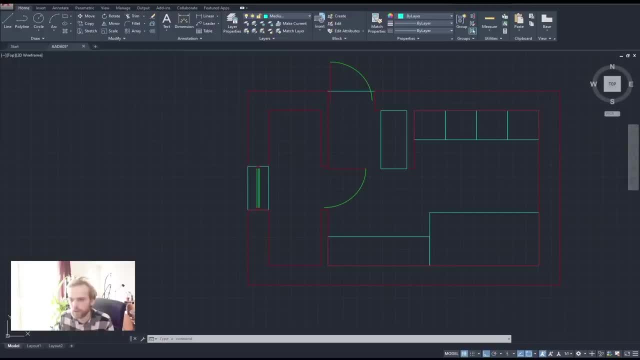 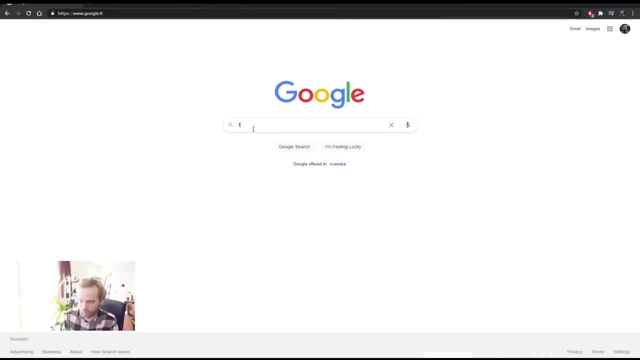 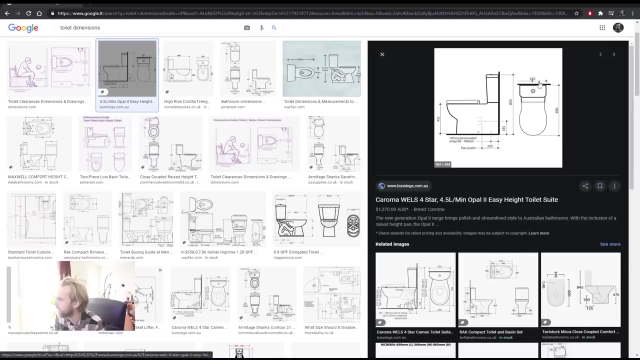 Let's just type that in real quick. Just give me a second. Just a second. There we go. Google Toilet Dimensions, Toilet Dimensions Images- sure, why not? And just find any image here, and then you can see 690 by 35.. 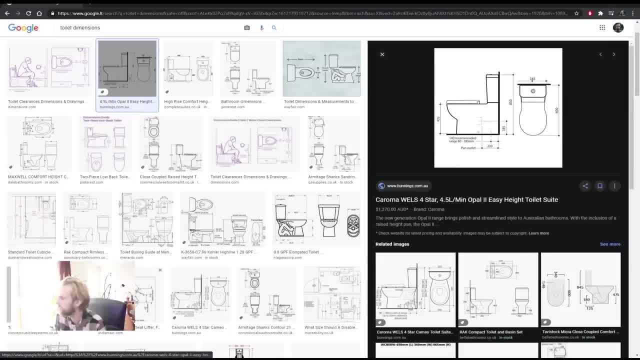 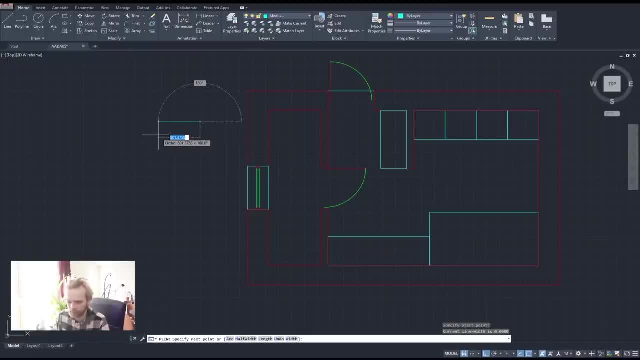 Let's see So: 69 centimeters by 35 centimeters. Sure, I'll just draw it out as a rectangle. for now, That's all I care about is just the size. We will make it nice later: 690 in well, 350 in width, 690 in length, 350, 90.. 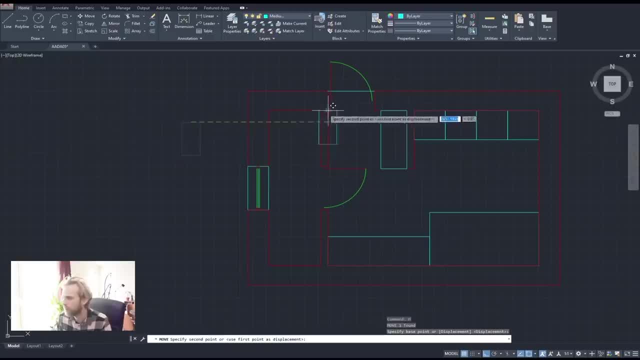 There we go, Something like that And just place it here, Which means that we do have a little bit of room for this to move out, And I think we will. We will use that. I think we will use that. Should we use that? 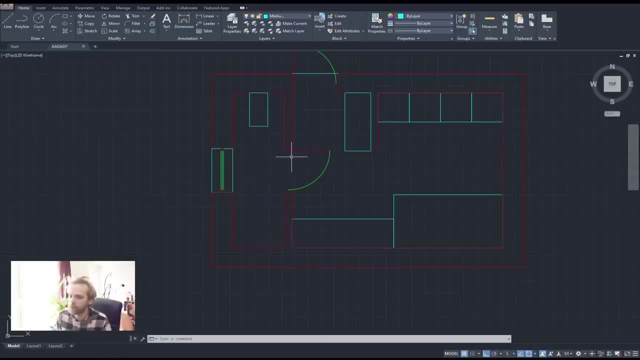 Yeah, maybe we should. So I'm just going to move everything to the side a little bit. The way you do that is well, you can just kind of select these two, these two polo lines here, And notice where we have these points here. 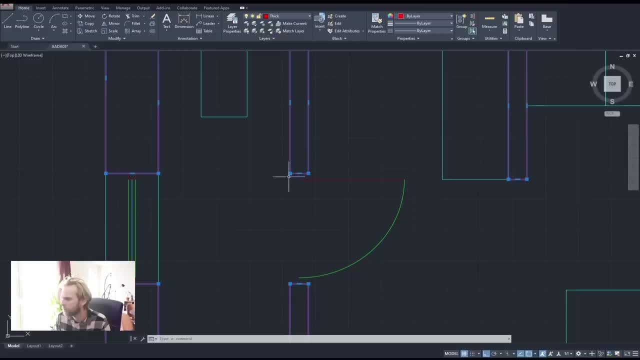 I believe we can just kind of move those points around, can't we? Let's see, Yes, we can click on those points on those corners and just move them up, And I'll just move them up by just a tiny bit. Do I want to do that? 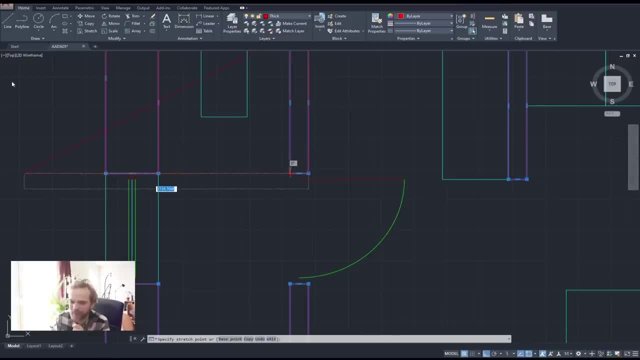 Sorry, Sorry about this. I need to design it in my head real fast. Do I want to move them? I mean, I do like the center composition here, But maybe we can break the center composition. Nah, I'll keep it. 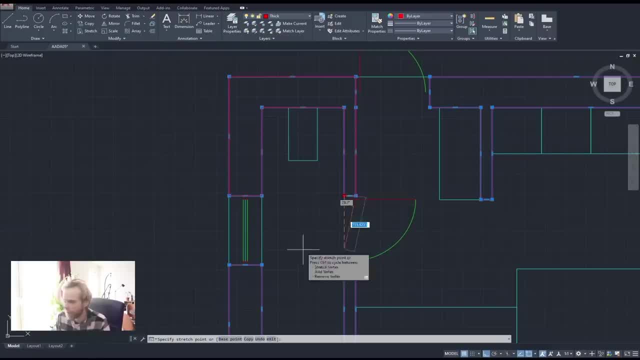 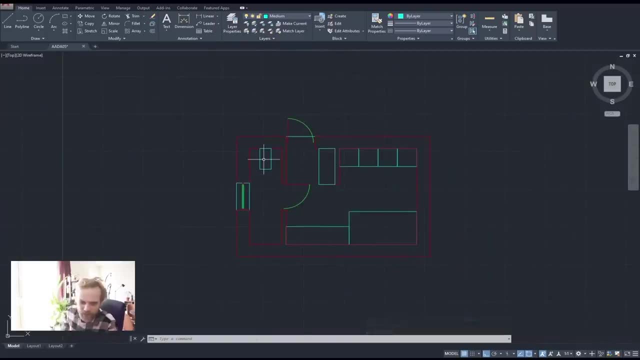 I'll keep it. So I'll escape out of this And it's lagging Escape. I'll actually keep it. That's fine. It is what it is right. The opening: When the door here is opened, you can't go through here. 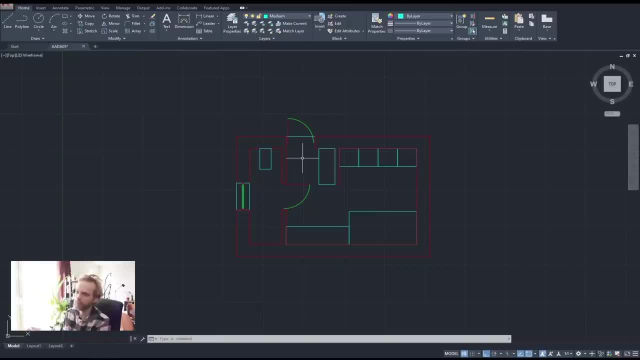 But that is, That is the bane of small houses. My thoughts were that I could move this opening towards somewhere here Until here, And then flip the door around again, Mirror it back to what it was before, And then you will have a smooth transition into the toilet, the bathroom, 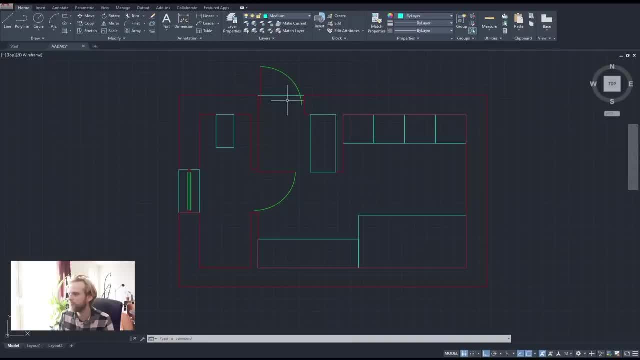 But it's not ideal. It's definitely not ideal as well, So might as well just keep it the way this is, It's fine, Let's just move on. So we have our toilet here, The shower- I don't even think we need to create like a separate shower cabinet. 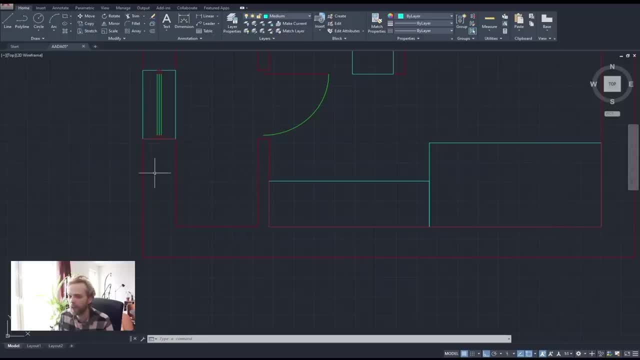 I think we can deal with this part here as a shower cabin in general. So that's fine. It will have a mark which shows that the shower ends here. And let me just measure the distance real fast. How wide is it? It's one meter wide. 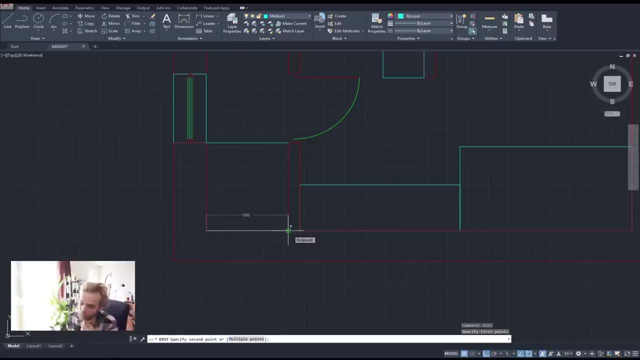 So it's a pretty damn wide shower. We can actually- We don't need it to be that wide, do we? Well, We kind of do, Because if we put a sink here, then we need a gap here. Yeah, So okay. 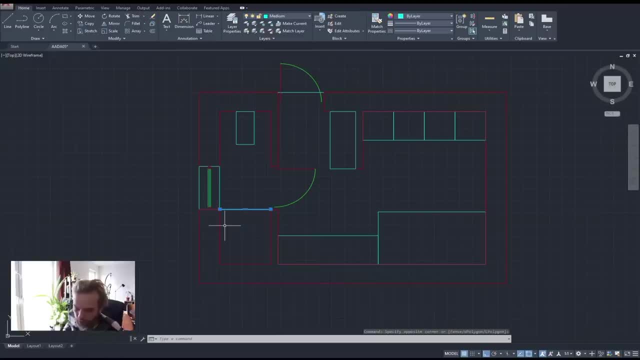 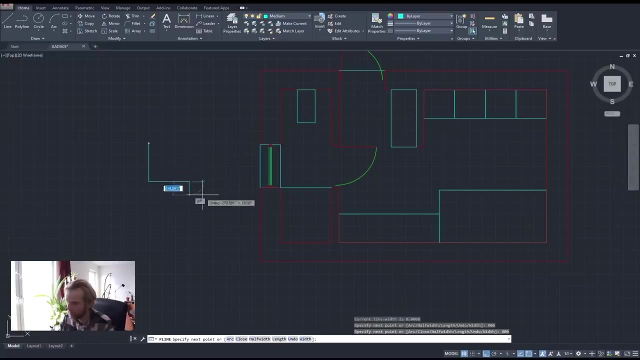 We will have a pretty large shower, But the depth of it is a little bit too big, I think. Let's see the distance: 1.15 meters. That's actually reasonable. Usually the The smallest shower that you can have is 800 by 800 by 8.. 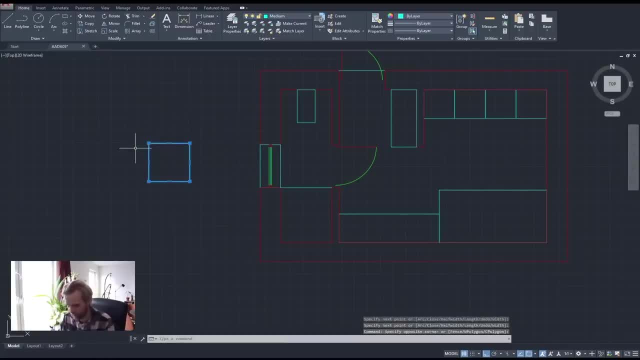 Yeah, 800 by 800 millimeters, So something like this. So here what we have is basically just a larger shower. That's fine, That's fine. Maybe I will indeed move this line back by negative Or not negative, Just 150 millimeters. 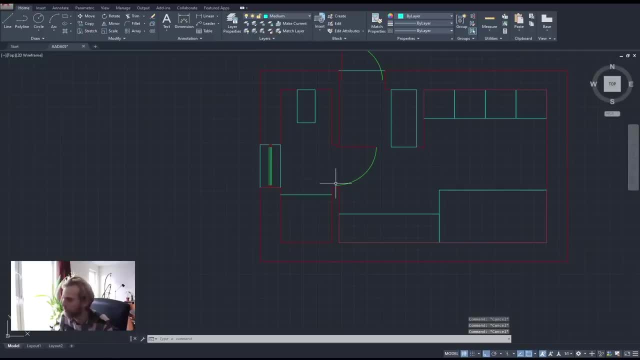 So it's, meter by a meter, A little bit cleaner, Right? So this is where our shower is. I think we have it planned out. I think that's That's good enough, Now just adding a few bits and pieces here to the walls to make it a little bit more. 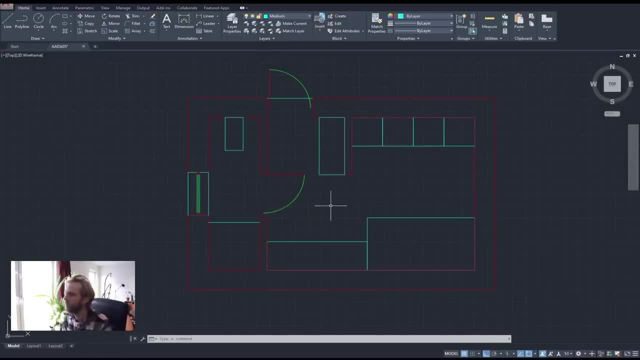 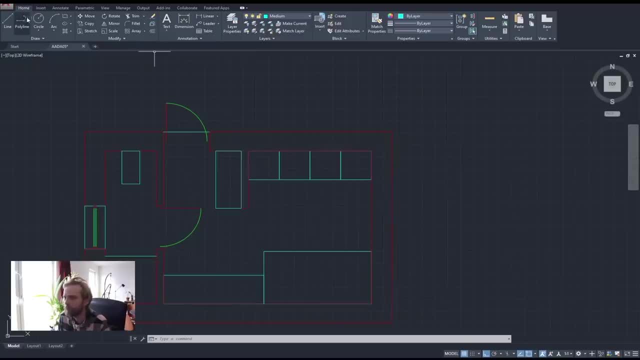 Okay, Okay, Okay, Okay, Okay, Okay, Okay. So I will create a window here. From here until here, There is going to be a window, And let me immediately make a thick line And let's draw it in a thick line. 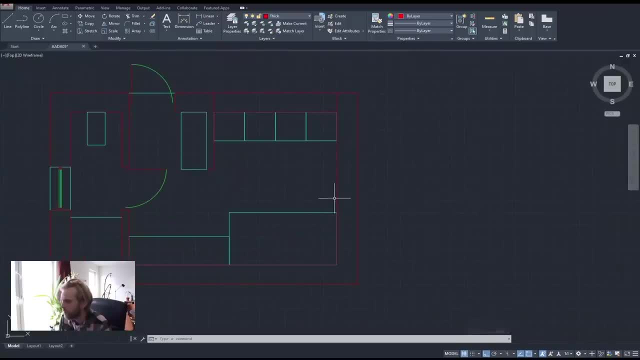 There is going to be a long, long window here, And also you want a window for the desk. depending if you're using a computer or not, Sometimes you don't want the window directly on the desk. so my thoughts are: what if we do? 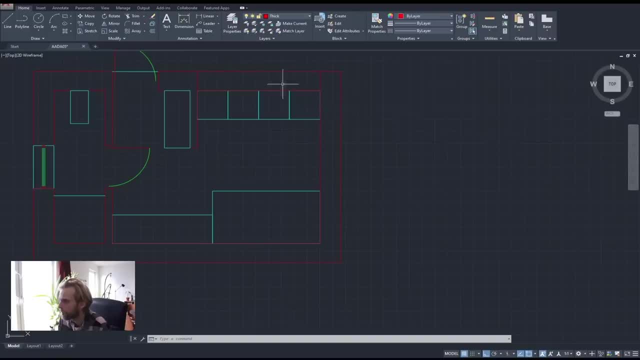 what if we do a window that is straight up a corner window, so it starts here and it's going to end here, right? so instead of that line is just going to be a window all the way around and it's going to be like a corner corner window. i think that's gonna look cool. 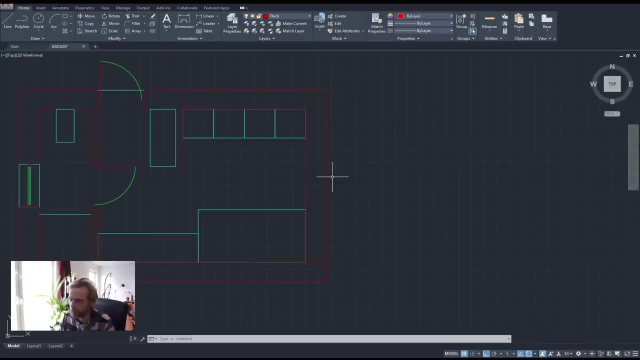 uh, so might as well do it, and also it's going to be a little bit more of a challenge for us to actually make it nice. so, window, right now i have a lot of stuff here that i don't really need to see, so i'm going to expand my layers tab and i'll hide the thin line and the medium. 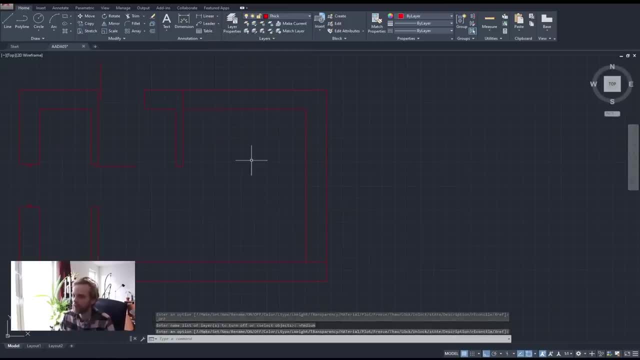 line layers by just clicking on the light bulbs here, so now they're hidden. uh, just so that it's, it's kind of easier for me to to work with this, i will trim away, trim, enter, enter, trim away this whole portion of the of the building, because that's where my window. 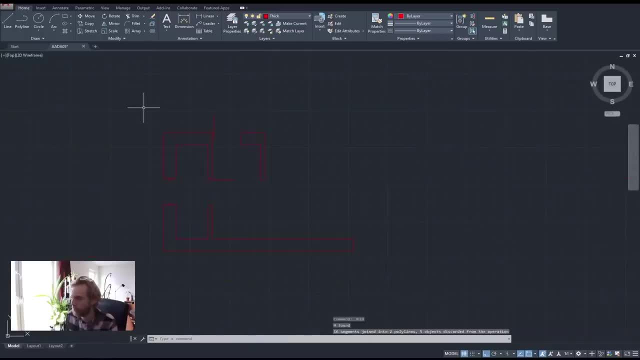 is going to be. i'll make sure to join everything up so that this is a single polyline and this is a line, sorry, and i'll turn on the medium layer again and make it my active one and now i'll draw out. from here to here i'll draw out the windowsill. it's going to be something like that. 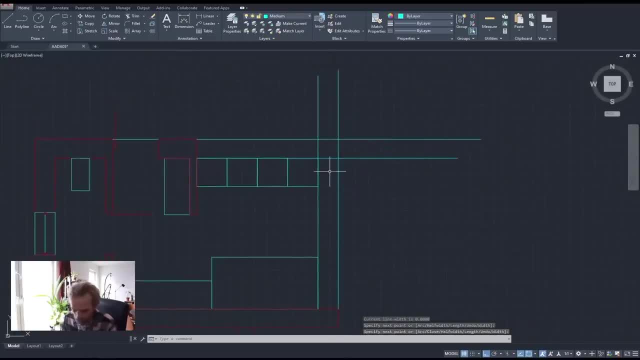 right, something like that, and now all i need to do is just fillet the window sill into a corner right, so i'll make sure that the radius is set to zero. so fillet r, enter r short for radius, enter, zero enter. so i made sure that there is no rounding and i will. 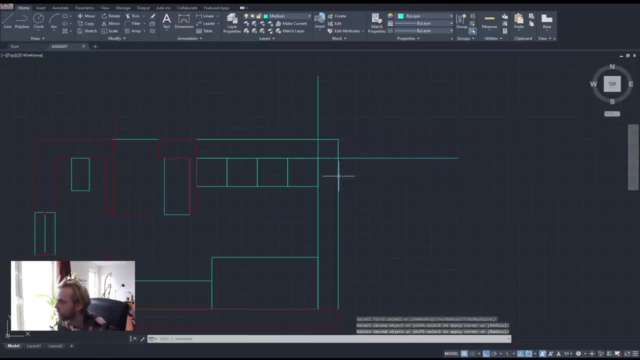 just fillet this with this. come on with this line, enter to repeat the flat command and i'll fillet this with this. there we go. so they they get kind of extended and filleted into one one area or or one pole line. uh well, they are not one pole line yet. these are two separate polylines that make a corner. 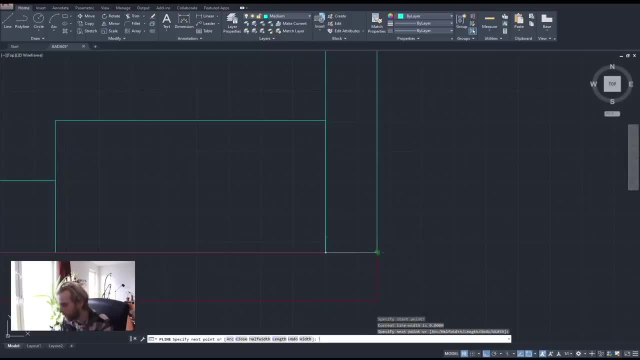 so i'll actually create a pole line here, or or a line segment, rather, here and here. i'll select all four of these lines, that and that, and i'll join them up. join, that's it. now. it's a single, single, closed polar line. great, so we have that. 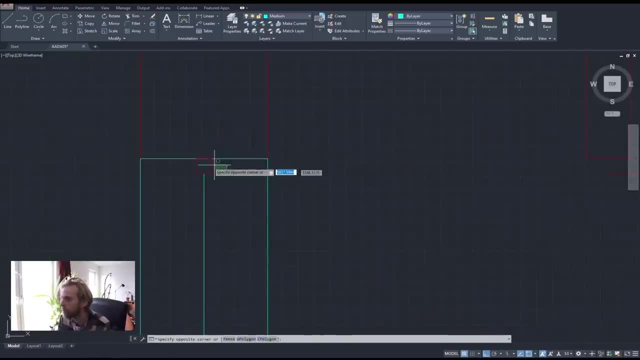 now on to creating the window frames. well, to do that, i will be using reusing this window frame here, window frame cut here, so i'll just copy it. i'll copy it from the side midpoint right here to the midpoint, right here. there we go. that's, that's one frame that's being cut. i'll also make 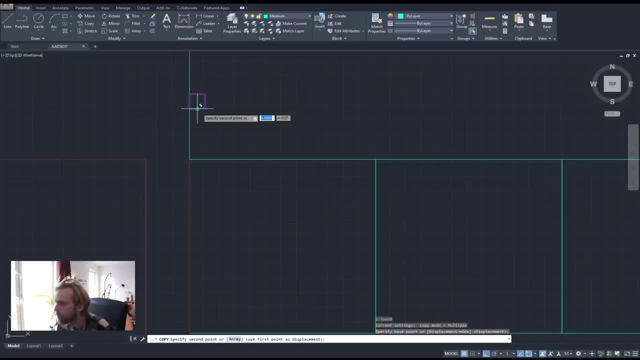 a copy to the other side of the window, from the bottom midpoint here to the midpoint here, like that. right now i need to know where exactly is the frame going to be located here in the corner, and the way i do that is i'll just draw out two helper lines. 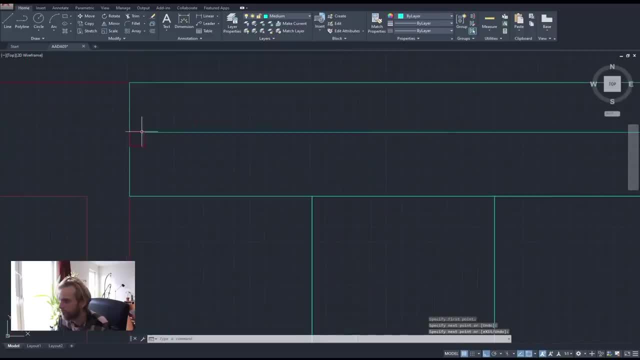 like that and like that, so it goes from uh around the outer perimeter of the frame. so from this point as well as from this point, and they meet up in this corner, meaning that now, if i take this and i copy, copy it from its corner point here, through the corner here, 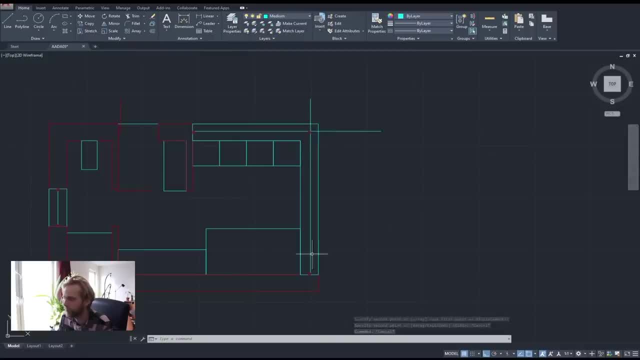 this is going to be like a clean transition: clean, 90%, 90 degree bend. so i don't need the helper lines anymore. i have the the corner frame located right here. usually the corner frames do have a little bit more of a of a thickness to them, but in this case, since we're dealing with low 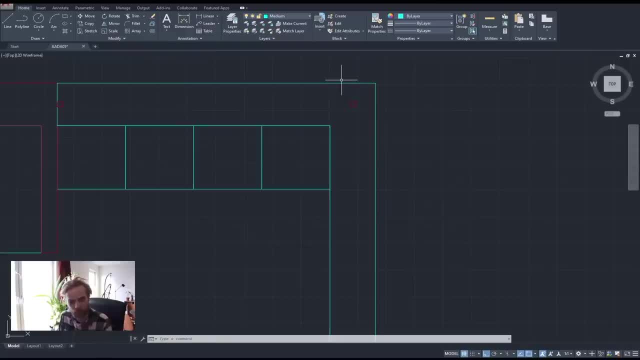 low detailing level for our plans. we don't really need to to show that. that's fine the way it is. now on to adding more frames, because this is a pretty long window, so it's going to have partitions. i'm thinking of adding two partitions here, so i will first measure the distance. 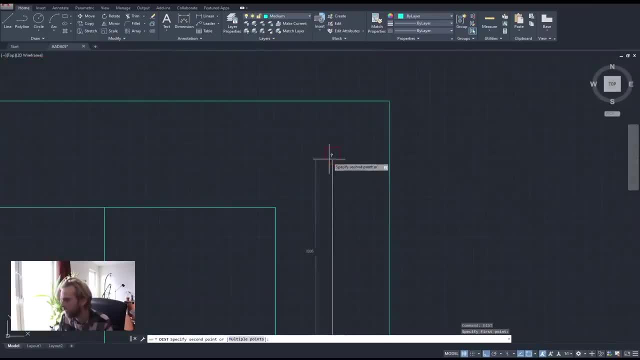 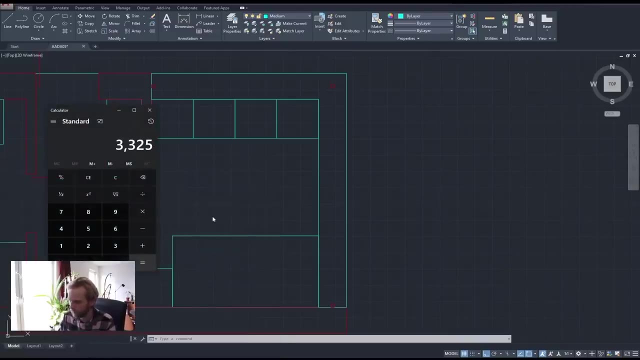 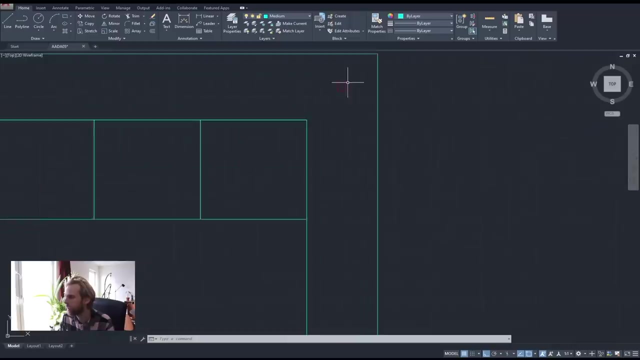 between this and this and i get 3325 millimeters, which is not great, but that's gonna do the trick. i will just run a calculator: 3325 divided by 3 is 1.1 meters approximately. so what i'm going to do is i'm just going to take this frame and i'll copy it. 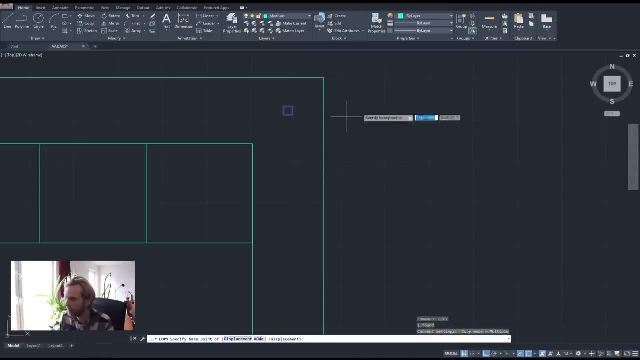 i'll copy that, that frame cut downwards by 1100, 1.1 meters like that, and i'll take the bottom frame, i'll copy it upwards by 1100- enter, escape out of the copy. so now i have like a pretty okay transition here and also i believe we do want. 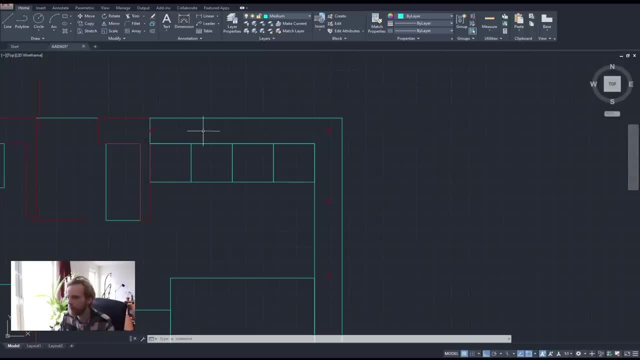 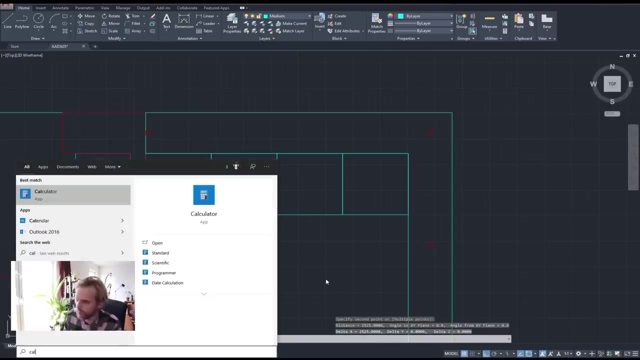 at least one window frame here in the middle. so i'll repeat the process- distance from here to here- and i'll copy it upwards by 1100. and i'll take the bottom frame. i'll copy it upwards by 1100. uh, that's two, two, two, five, two, five. so that's going to be. well, math is hard. okay, let me grab. 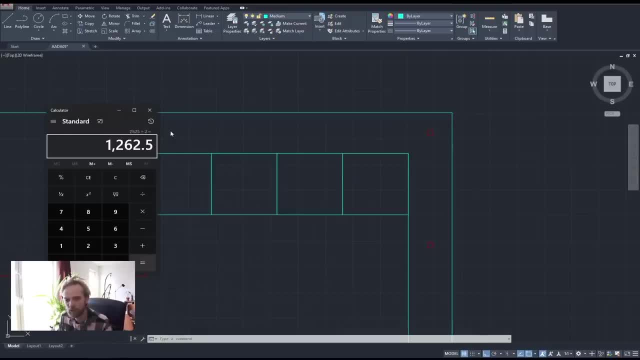 calculator: two, five, two, five, divided by two. one, two, six, five. so i'll actually do this: one, two, six, five, point five. so i'll take this, uh, this frame right here, i'll copy it to the side: two, five, six, five, i believe, poof, uh, oh, no, no, no, no, uh, one, six, two, five, point five. one, six, two, five, point five. 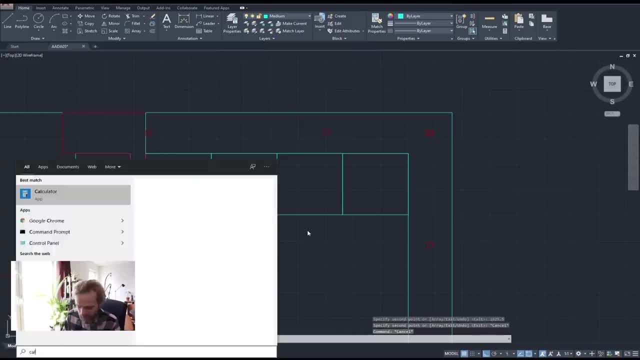 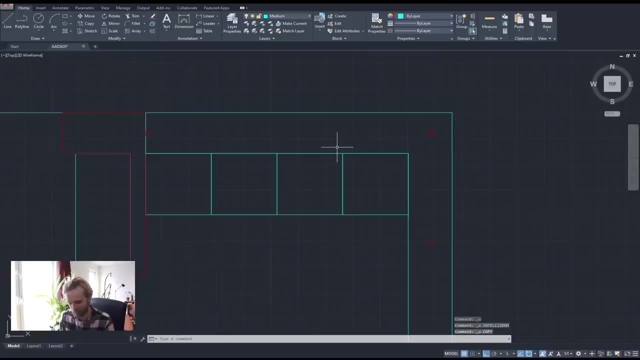 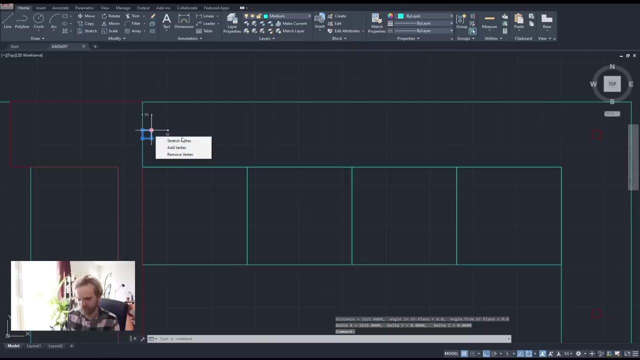 no, oh god damn it. one, two, six, five. let's do it again. i messed that up. let me measure distance again. god damn it. uh, two, five, two, five, right, yeah, two, five, two, five divided. two, one, two, six, five point five copy, c'mon copy. copy here to here: one, two, six, five point five, enter there we go in the middle. 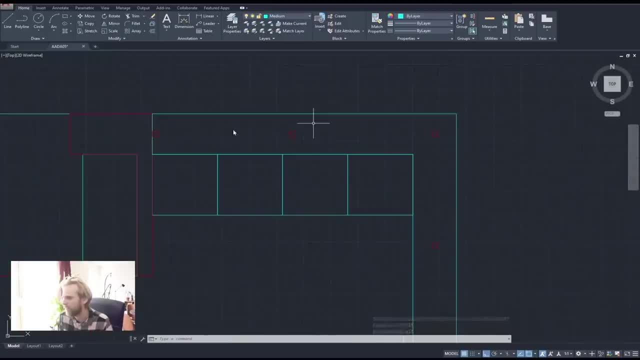 back. okay, so we have that done and actually it's not going to be in the middle right because the, the, the frame itself has a construction. so i'm going to work on this. um, i'm going to start working on this first box. i'm going to start. 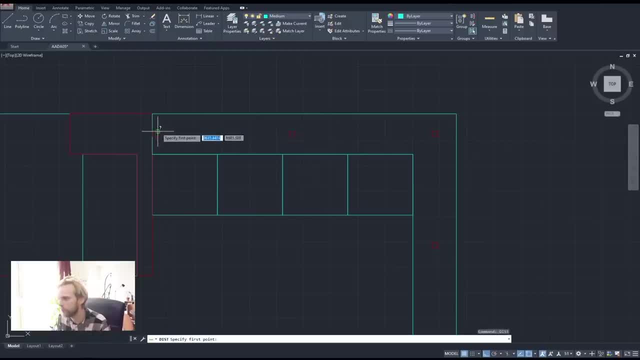 certain amount of thickness. let me just double check with measuring two distances. from here to here we have one, two, one, five point five, and from here to here we have one, two, five, nine point five. one, two, five, nine point five. one two, one, five. so that is going to be. I need to. 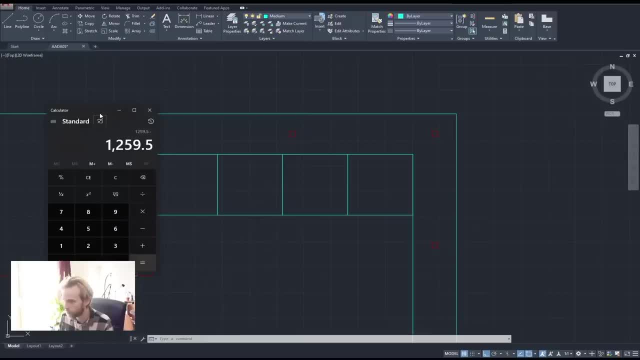 just keep calculator open. one, two, five, nine point five minus one, two, one five point five, that's going to be 44 millimeters off of an error. so I'm just going to move this further by 44 millimeters. now it's in the middle um. 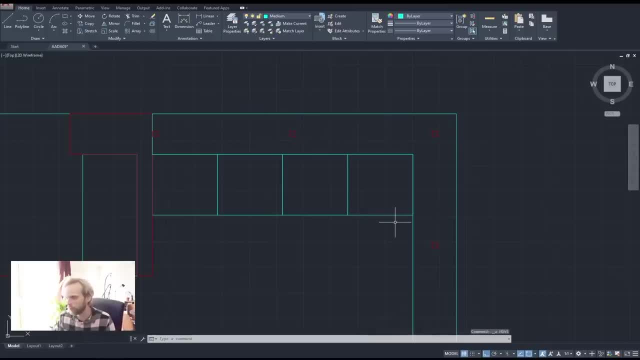 you don't really need to. well, sorry, not 44, that's going to be 22. you don't need to do this now as I'm doing it, you don't need to do this. it can be in this stage, it can be approximate. it doesn't need to be that precise, but just wanted to kind. 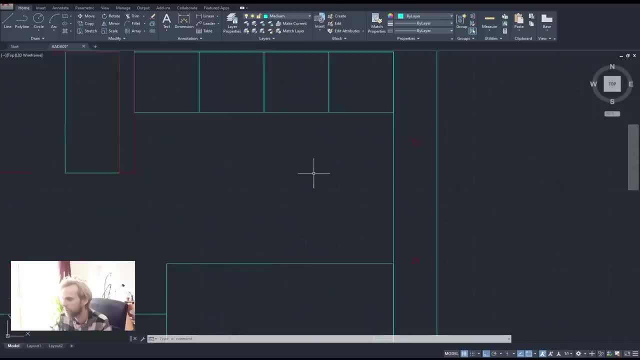 of do it just for purpose of being methodical. okay, frames are done. frames are done. now it's time for glass. so that's just line segments. from now it's time for glass. so that's just line segments. from now it's time for glass. so that's just line segments from midpoint, midpoint here, cutting. 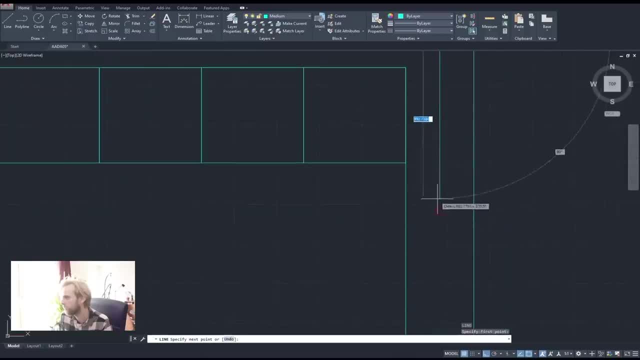 midpoint, midpoint, midpoint, here. cutting midpoint, midpoint, midpoint here, cutting through the glass, through the glass, through the glass made to mid, made, made, made to mid. that's made to mid, made, made to mid. that's made to mid, made made to mid. that's done. and now, with thin line, Oh, keep. 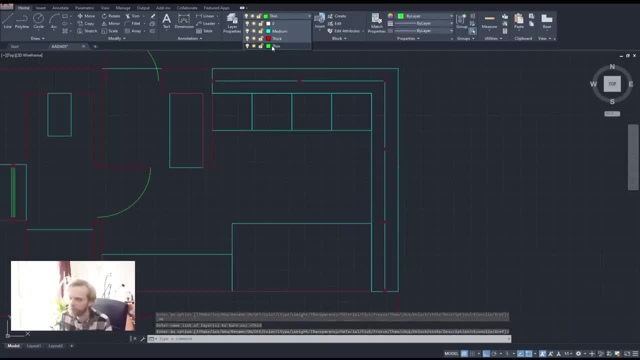 done. and now with thin line: Oh, keep done. and now with thin line, Oh, keep. later, turn on. so I had it turned off. so later, turn on. so I had it turned off. so later, turn on. so I had it turned off. so once I selected the thin line, layer it. 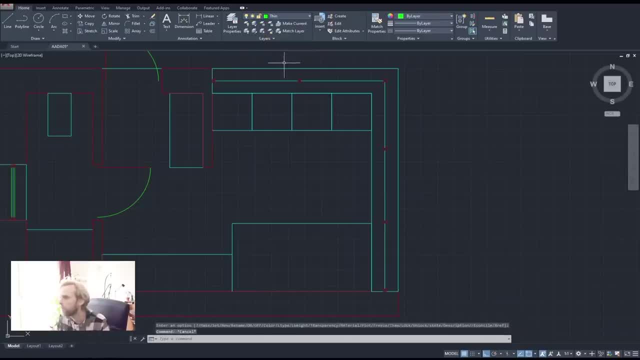 once I selected the thin line layer. it, once I selected the thin line layer, it asked me to turn it on. so I did so. with. asked me to turn it on, so I did so. with. asked me to turn it on, so I did so. with thin line layer, I will create two more. 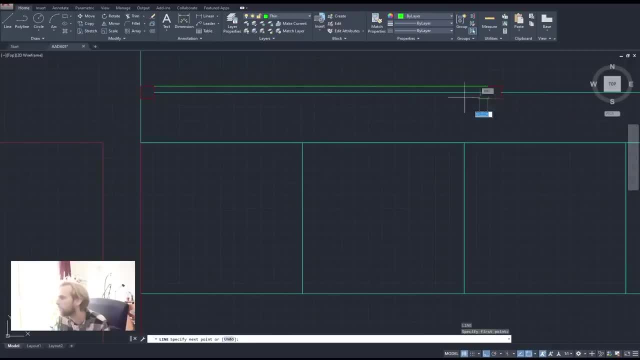 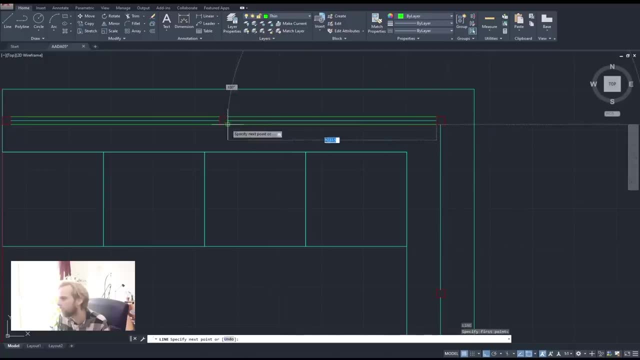 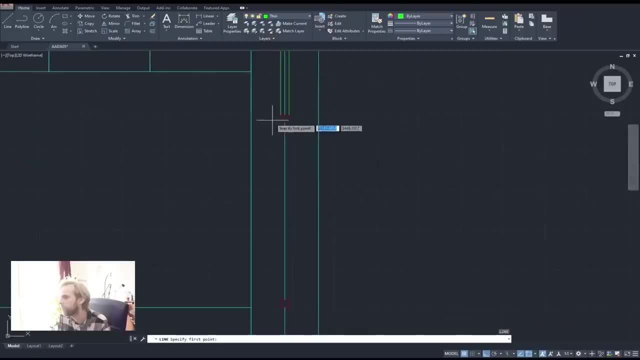 I'm just hitting enter to repeat the. I'm just hitting enter to repeat the command command command. so I'm finishing the command and then so I'm finishing the command and then so I'm finishing the command and then hitting enter to repeat the last command. hitting enter to repeat the last command. 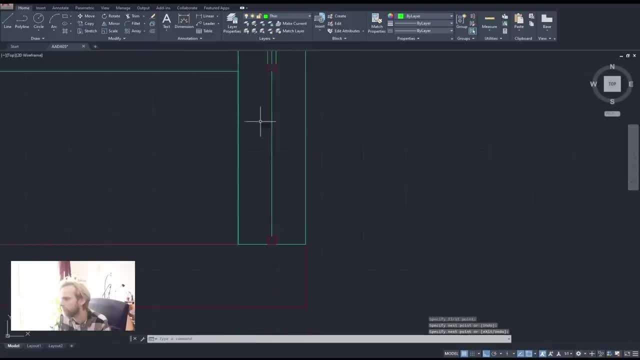 hitting enter to repeat the last command, to kind of keep drawing the line. to kind of keep drawing the line. to kind of keep drawing the line: segments: that and finally that, okay, that and finally that, okay, that and finally that. okay, we are done, we have our corner. 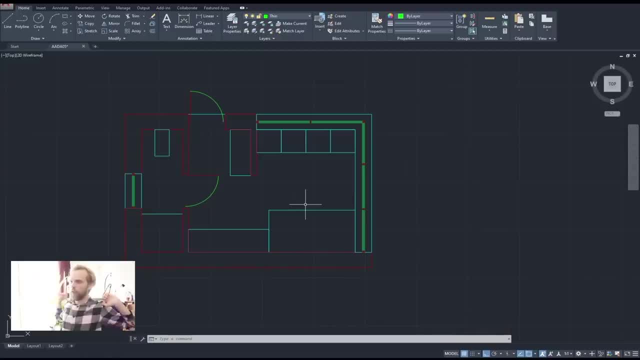 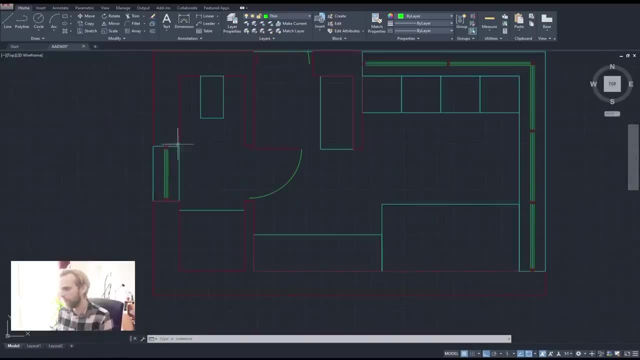 we are done, we have our corner. we are done, we have our corner corner window. that is finished. all right, so that is our initial plan. all right, so that is our initial plan. all right, so that is our initial plan, and that seems okay. there's going to be. 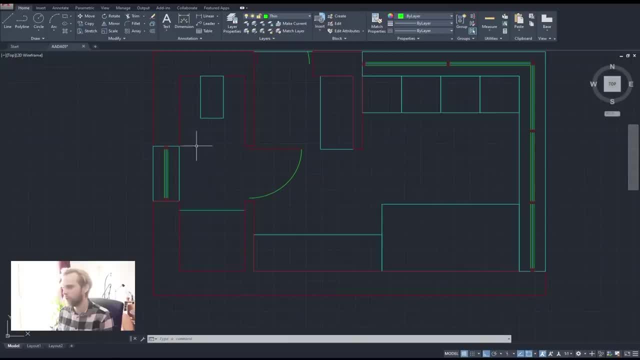 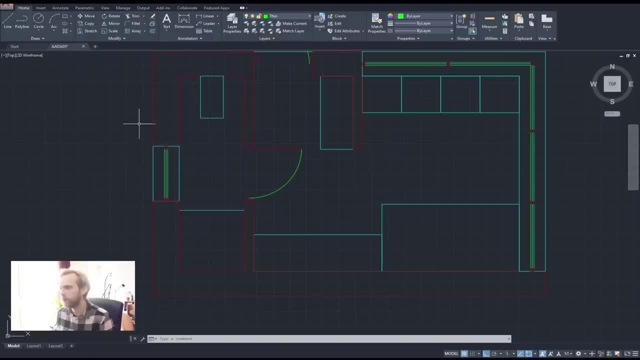 do an arc, it's going to be fine. do an arc, it's going to be fine. um, let's do an arc, so I'm going to. um, let's do an arc, so I'm going to, um, let's do an arc, so I'm going to, or rather, let's, let's just do a pole. 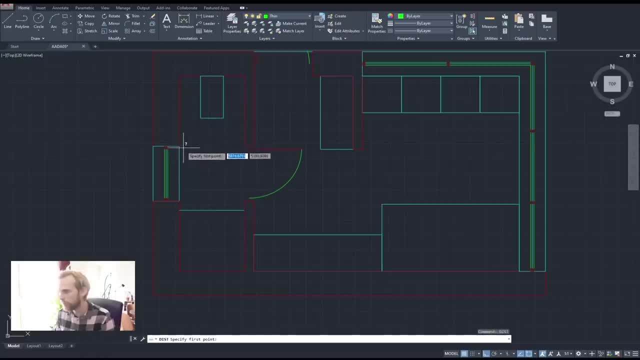 or rather, let's, let's just do a pole, or rather, let's, let's just do a pole line first. so I know that line first. so I know that line first, so I know that the distance of this window is 900. the distance of this window is 900. 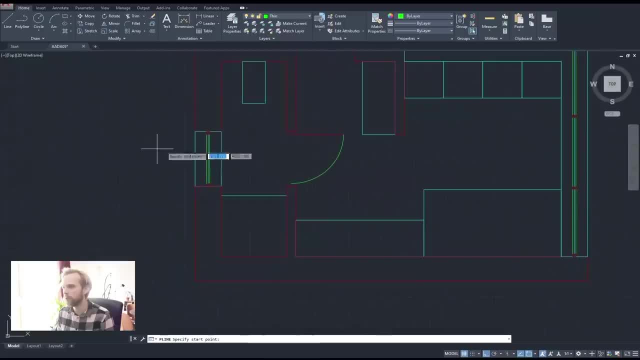 the distance of this window is 900 millimeters right, 900 millimeters wide. millimeters right, 900 millimeters wide. millimeters right, 900 millimeters wide. so I'm just going to make a sink, that's so. I'm just going to make a sink, that's. 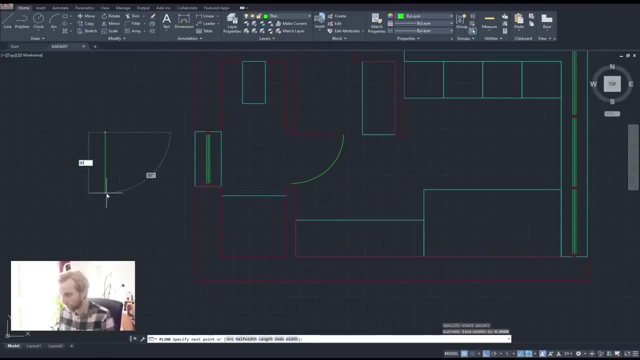 so I'm just going to make a sink that's 900, 900, 900 uh in in length, uh in in length, uh in in length, um and the width of it. I actually want to um and the width of it. I actually want to um and the width of it. I actually want to use like 400 millimeters because it's. 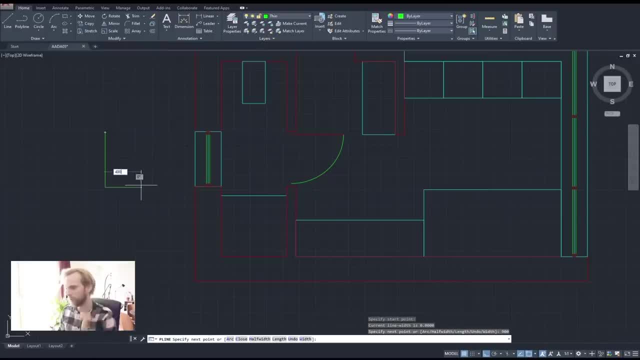 use like 400 millimeters because it's use like 400 millimeters because it's just a sink, just a sink, just a sink. um, yeah sure, let's use 400. um, yeah sure, let's use 400. um, yeah sure, let's use 400 900. 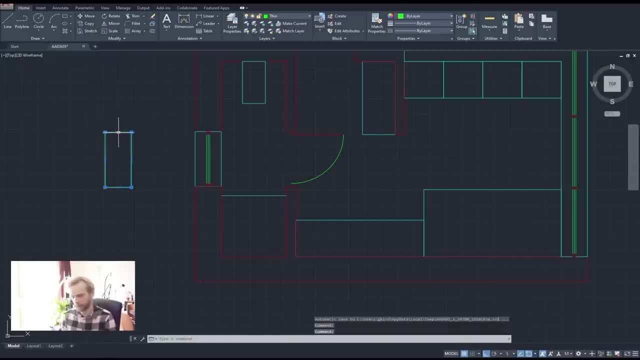 900, 900, 400, 400, 400. there we go, so we have our sink here. there we go, so we have our sink here. there we go, so we have our sink here, and I'll just, and I'll just, and I'll just move it. 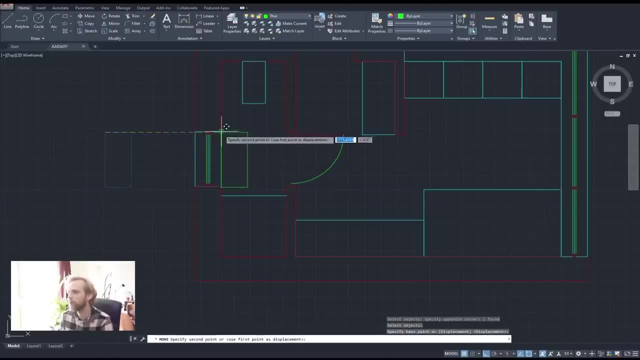 move it, move it. m enter select objects. enter from this: m enter select objects. enter from this: m enter select objects. enter from this point. to this point. right, I just point to this point, right, I just point to this point, right, I just kind of move it and I'll place it in the 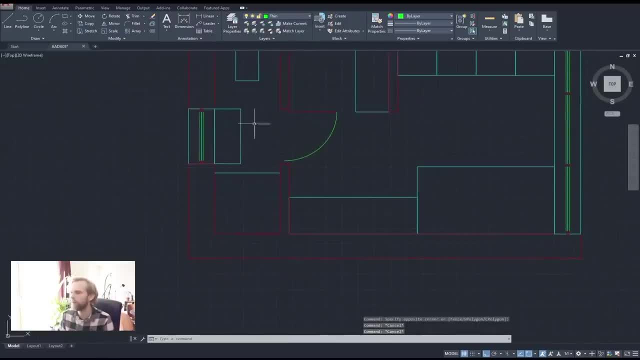 kind of move it and I'll place it in the kind of move it and I'll place it in the medium layer, medium layer, medium layer, like that, and now um like that and now um like that and now um, these corners right here are kind of, these corners right here are kind of. 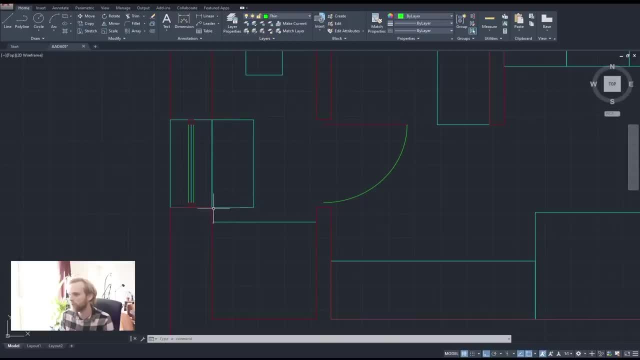 these corners right here are kind of obnoxious, obnoxious, obnoxious. so what I'm gonna do is I will. so what I'm gonna do is I will. so what I'm gonna do is I will round them off, round them off, round them off as much as I can. 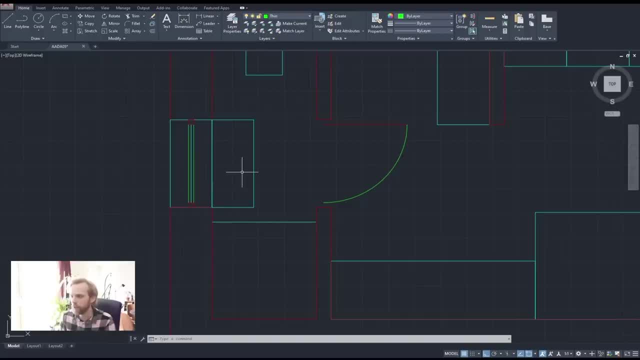 as much as I can, as much as I can, um. so my thoughts are um. so my thoughts are um. so my thoughts are: I need to use fillet right. I need to use fillet right, I need to use fillet right for this, so I will use fillet. 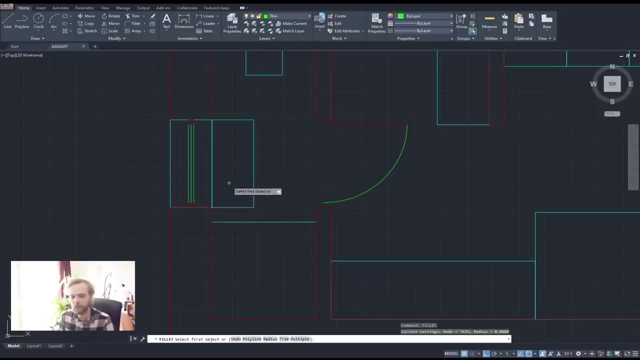 for this. so I will use fillet for this. so I will use fillet: enter, enter, enter. and I know that this is 400 millimeters, and I know that this is 400 millimeters and I know that this is 400 millimeters, so my radius cannot be larger than 400. 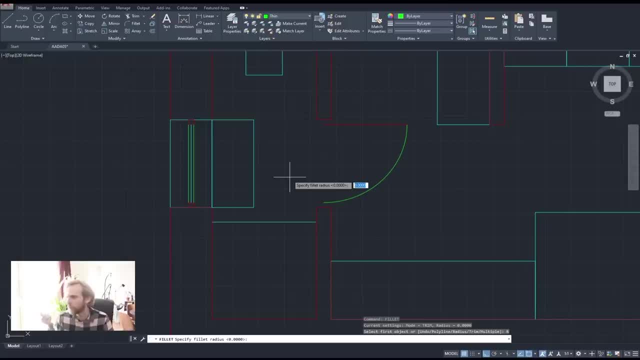 so my radius cannot be larger than 400. so my radius cannot be larger than 400 because it will just break it will not. because it will just break it will not, because it will just break, it will not work right. so I'm probably going to use 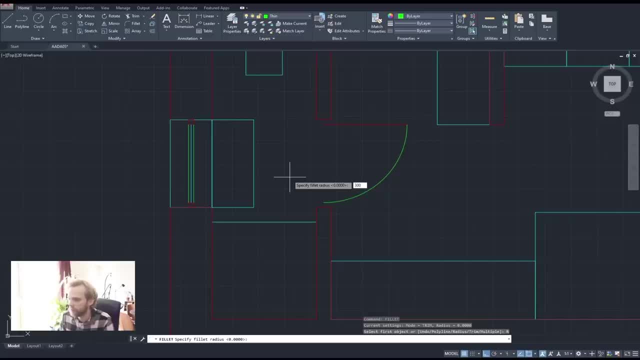 work right, so I'm probably going to use work right, so I'm probably going to use something like 300 millimeters. I think something like 300 millimeters. I think something like 300 millimeters. I think that's going to be enough, so fillet. 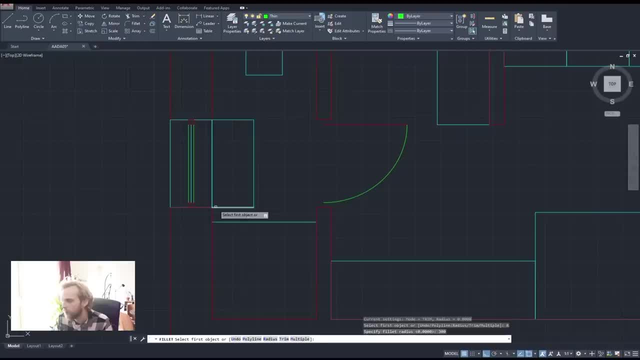 that's going to be enough, so fillet. that's going to be enough, so fillet. radius 300, enter. radius 300, enter, radius 300, enter, and then this line fillets with this line, and then this line fillets with this line, and then this line fillets with this line by 300, then enter to repeat the fillet. 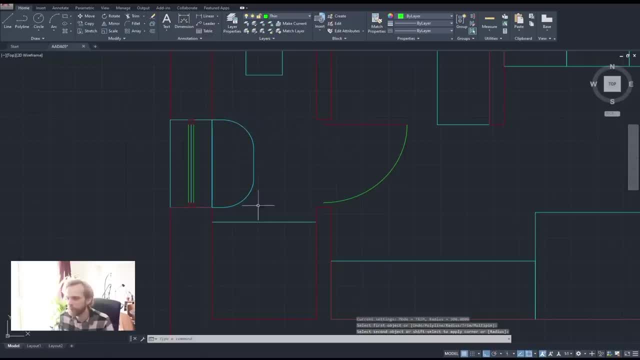 by 300, then enter to repeat the fillet by 300, then enter to repeat the fillet. this line, let's with this line by 300. this line, let's with this line by 300, this line, let's with this line by 300, that's it. 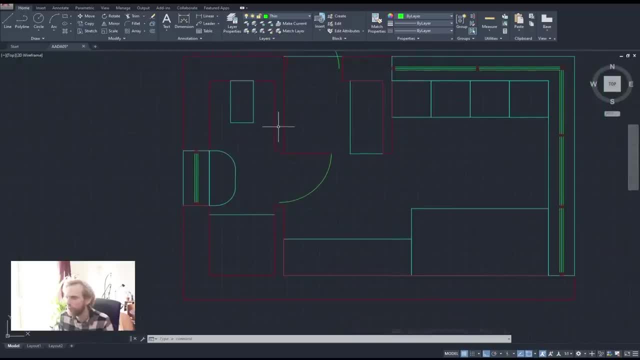 that's it. that's it. this is now a little bit better in terms. this is now a little bit better in terms. this is now a little bit better in terms of transit transition, of transit transition, of transit transition, um, what I really um, what I really um, what I really would encourage you doing in in your 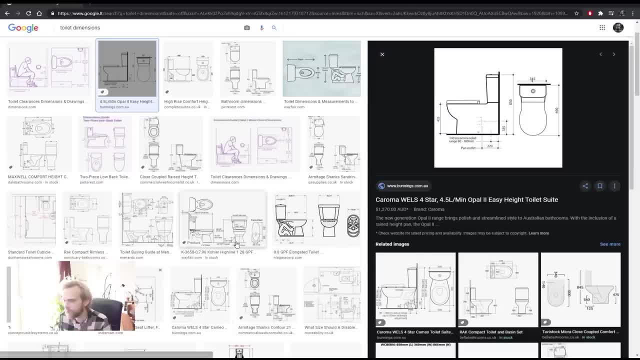 would encourage you doing in in your, would encourage you doing in in your future projects is. future projects is future projects is uh, where we have the uh, where we have the uh, where we have the toilet. we have this, this area which which toilet. we have this, this area which which. 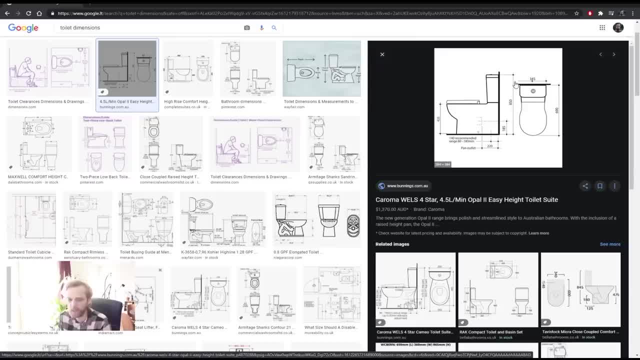 toilet. we have this, this area which which holds the water, holds the water, holds the water. this whole area right here can be hidden. this whole area right here can be hidden. this whole area right here can be hidden in the in the wall right it can be in the. in the wall right it can be. 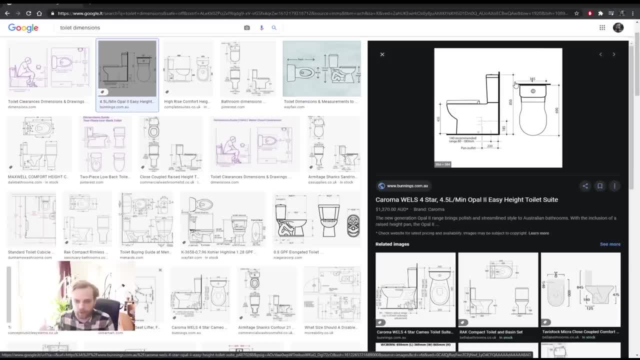 in the in the wall right. it can be placed in the wall, placed in the wall, placed in the wall, but the wall of course needs to become, but the wall of course needs to become, but the wall of course needs to become thicker. and as you place it in the wall, 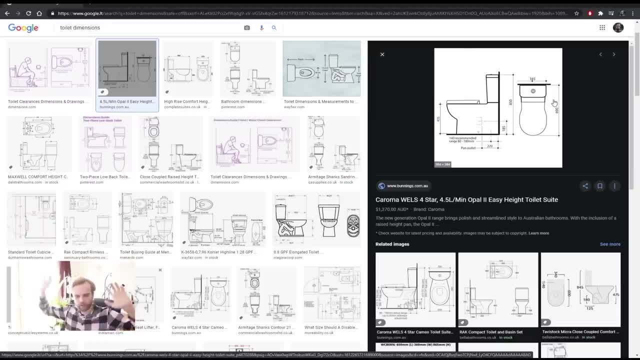 thicker and as you place it in the wall, thicker and as you place it in the wall above it. you also have um possibility above it. you also have um possibility above it. you also have um possibility for shelves and and whatnot you know, for shelves and and whatnot you know. 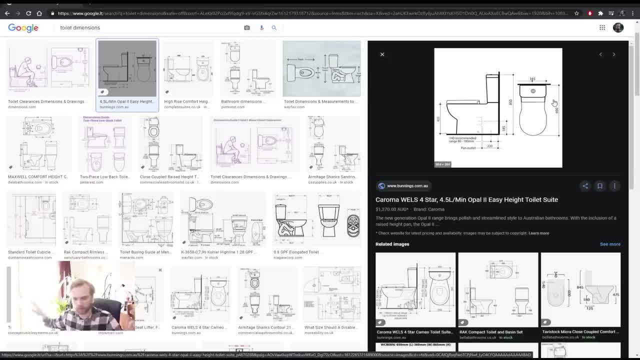 for shelves and and whatnot. you know for for all of the, for for all of the, for for all of the. you know toilet paper rolls, and and so on. you know toilet paper rolls, and and so on. you know toilet paper rolls, and and so on. so i would encourage you to. 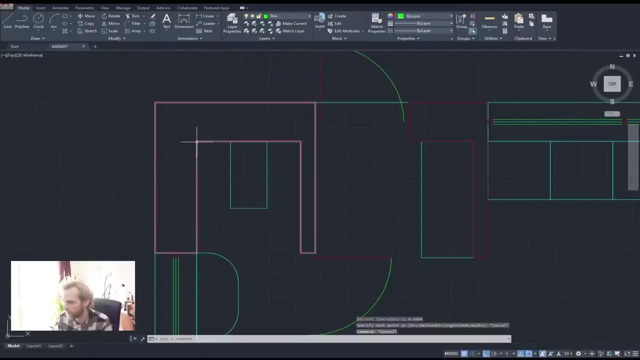 so i would encourage you to, so i would encourage you to in in your future projects, just to do in in your future projects, just to do in in your future projects, just to do something like this, um, something like this, um, something like this, um create a separate. 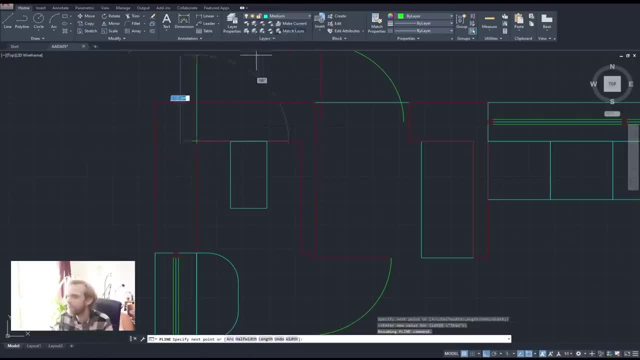 create a separate, create a separate. well, in the medium thickness. is it well in the medium thickness? is it well in the medium thickness? is it medium? yeah, let's do medium in medium medium. yeah, let's do medium in medium medium. yeah, let's do medium in medium thickness. just create a shelf. 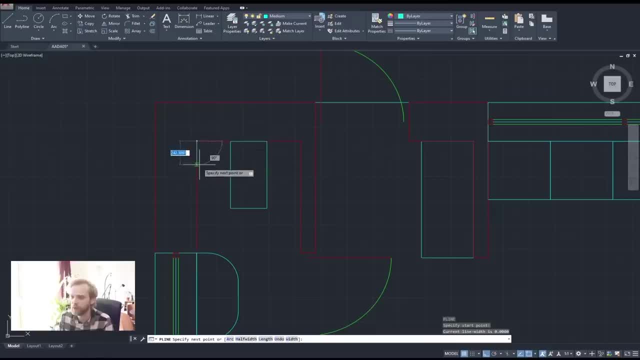 thickness. just create a shelf thickness. just create a shelf right enter. come on, let's create a shelf right enter. come on, let's create a shelf right enter. come on, let's create a shelf that is around 300 millimeters, maybe even that is around 300 millimeters, maybe even. 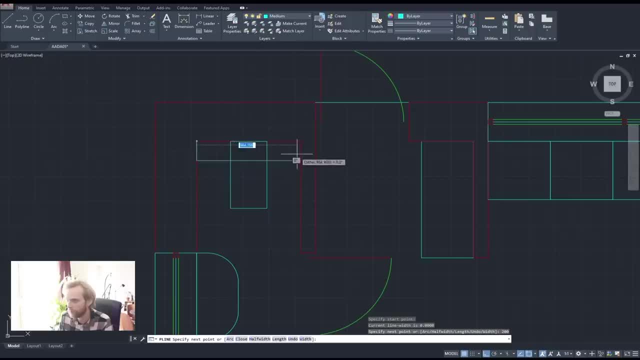 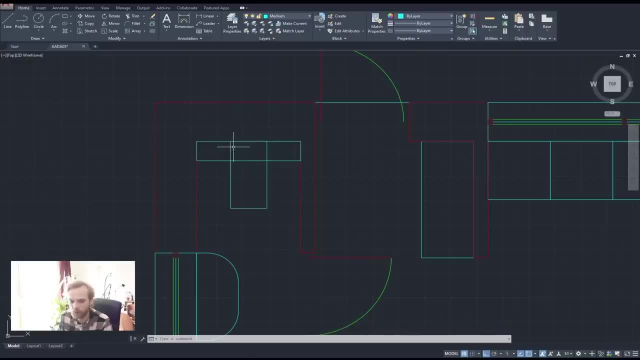 eats up the bottom or the, the last part of the, the bottom or the, the last part of the, the bottom or the the last part of the toilet, toilet, toilet, and and and the only thing that is kind of sticking, the only thing that is kind of sticking. 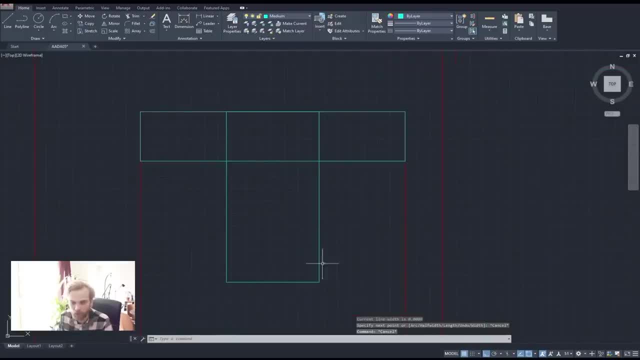 the only thing that is kind of sticking out from the shelf is the. the bowl out from the shelf is the. the bowl out from the shelf is the the bowl of of the toilet. it's just more of of the toilet. it's just more of of the toilet. it's just more aesthetic, it's just nicer right. so i'll. 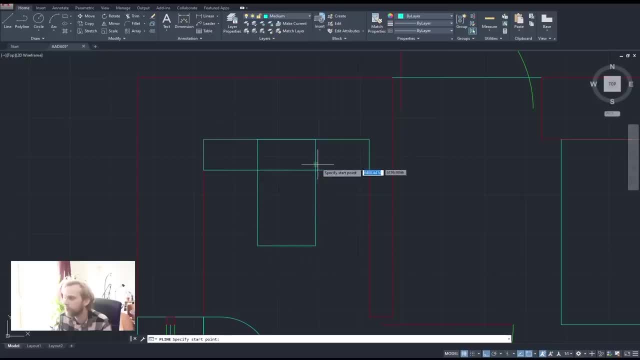 aesthetic- it's just nicer right, so i'll. aesthetic it's just nicer right, so i'll just grab the polo line tool and redraw. just grab the polo line tool and redraw. just grab the polo line tool and redraw just the bowl area of the toilet, just the bowl area of the toilet. 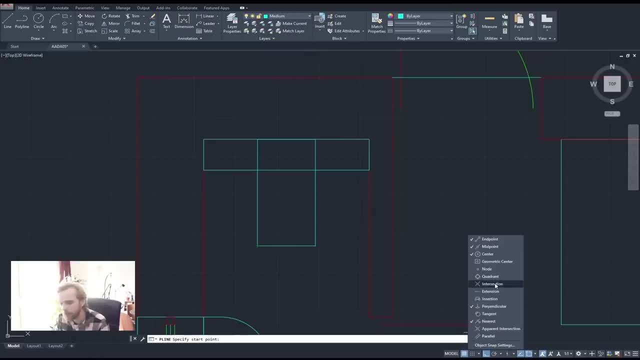 just the bowl area of the toilet. um, for that i do need to have intersection. um, for that i do need to have intersection. um, for that i do need to have intersection snapping turned on. snapping turned on, snapping turned on. enter so that i can enter, so that i can. 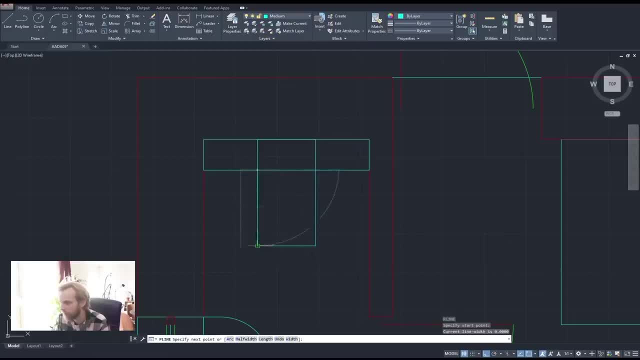 enter so that i can, so that i can start drawing from this, so that i can start drawing from this, so that i can start drawing from this intersection point here and kind of intersection point here and kind of intersection point here, and kind of draw out this: u shape here, right and now. 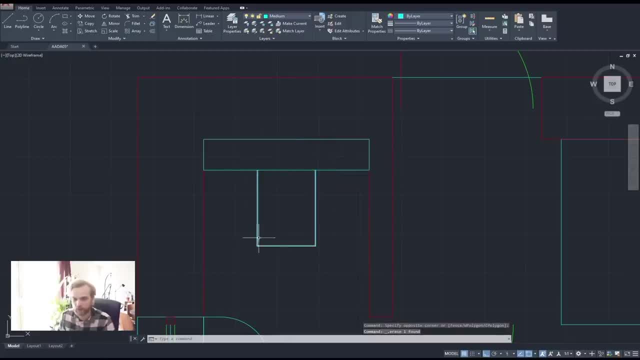 draw out this u shape here, right. and now draw out this u shape here, right, and now i can delete the old version. i can delete the old version. i can delete the old version, right. so this is just the bowl and let's right. so this is just the bowl, and let's. 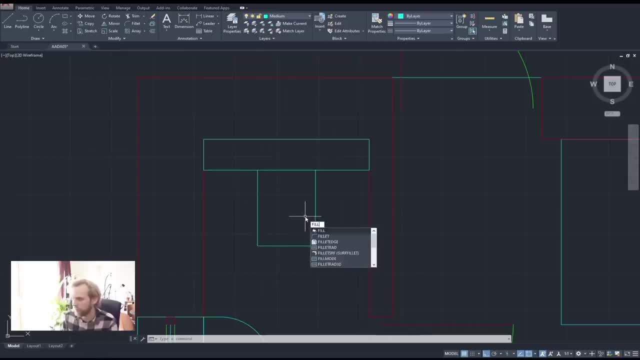 right. so this is just the bowl, and let's fillet it. let's, let's make it nicer, so fillet it. let's, let's make it nicer, so fillet it. let's, let's make it nicer, so i'll fillet. uh, first i'll measure the 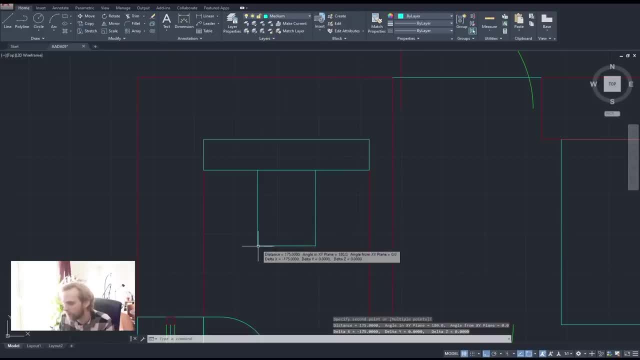 i'll fillet uh first. i'll measure the. i'll fillet uh, first. i'll measure the distance, distance, distance from here to here, from here to here, from here to here, well, or rather from here to here we, well, or rather from here to here we. 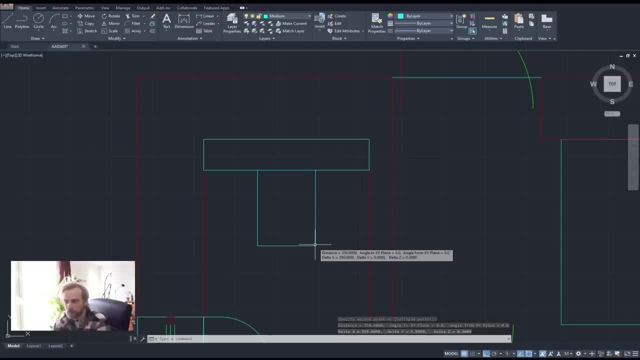 well, or rather from here to here, we have 350 millimeters, so half of that is have 350 millimeters, so half of that is have 350 millimeters, so half of that is 175 millimeters. so i'll do a fillet of 175 millimeters. so i'll do a fillet of. 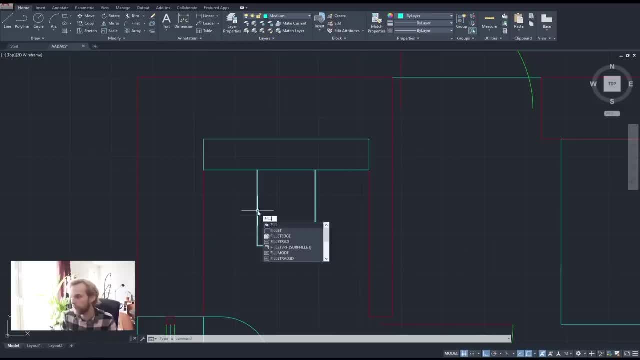 175 millimeters. so i'll do a fillet of 150 millimeters for both corners. 150 millimeters for both corners, 150 millimeters for both corners, let, let, let our r enter, our r enter, our r enter. how much did i say? 150, right, 150. 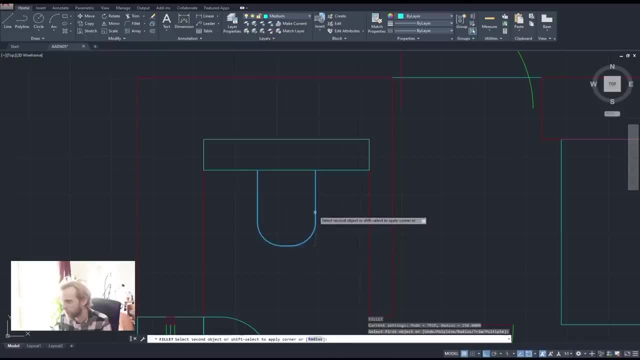 how much did i say 150 right 150? how much did i say 150 right 150? from here, from here. from here to here, 150. enter again from here to here, to here: 150.. enter again: from here to here to here: 150.. enter again from here to here: 150. 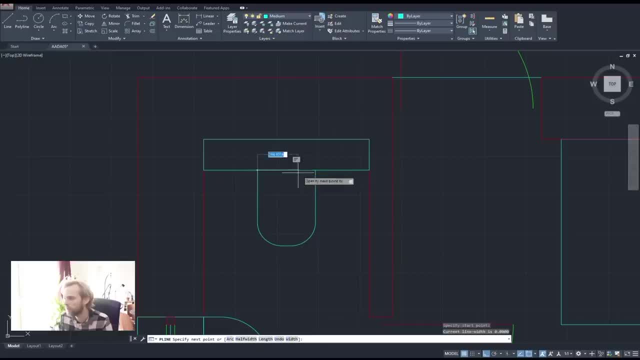 150.. 150.. so we have that. i will also close off. so we have that, i will also close off. so we have that. i will also close off the line by just creating a line segment, the line, by just creating a line segment, the line, by just creating a line segment here. 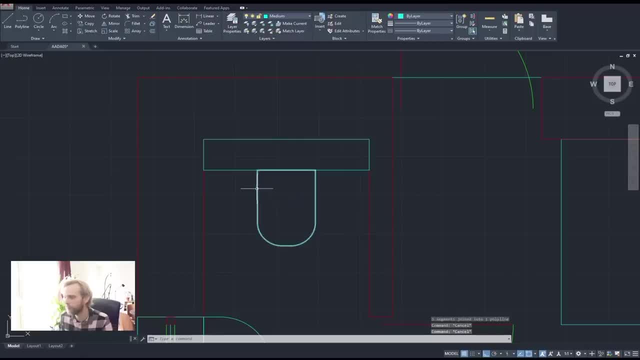 here, here, and joining it with the rest of of the and joining it with the rest of of the and joining it with the rest of of the bowl, bowl bowl, just to have it as a closed pole line, just to have it as a closed pole line, just to have it as a closed pole line and i will offset. 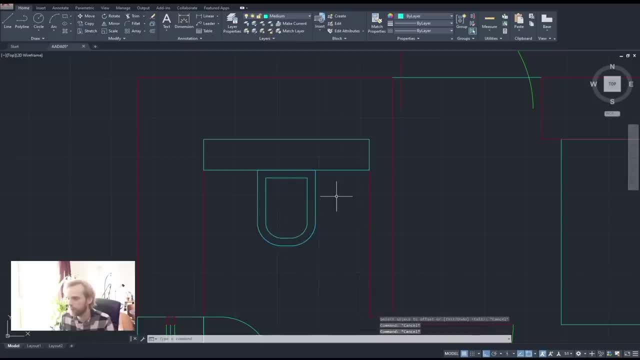 and i will offset. and i will offset the bowl inwards by 50 millimeters five. the bowl inwards by 50 millimeters five. the bowl inwards by 50 millimeters five. centimeters, just to have something like centimeters, just to have something like. 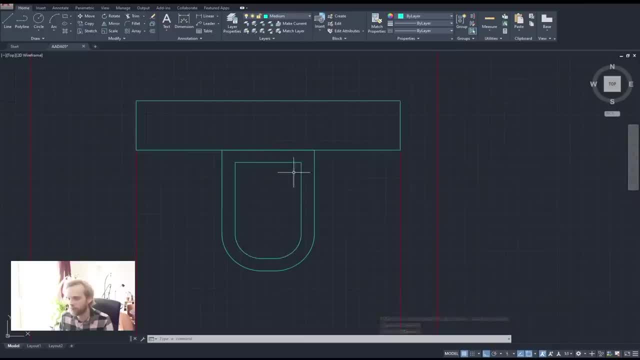 centimeters, just to have something like that, and now i will fillet that, and now i will fillet that, and now i will fillet these two corners here with a little bit. these two corners here with a little bit. these two corners here with a little bit less of a. 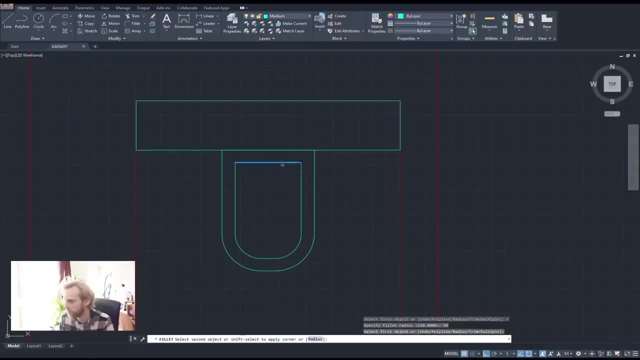 less of a, less of a of a radius. so radius is going to be like of a radius, so radius is going to be like of a radius. so radius is going to be like 50 millimeters, not more than that. 50 millimeters, not more than that. 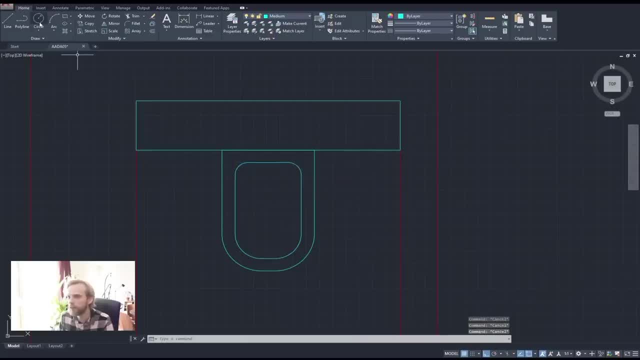 50 millimeters, not more than that, just to make it a little bit nicer, just to make it a little bit nicer, just to make it a little bit nicer. so we have that, and then just a small. so we have that, and then just a small. so we have that, and then just a small circle. 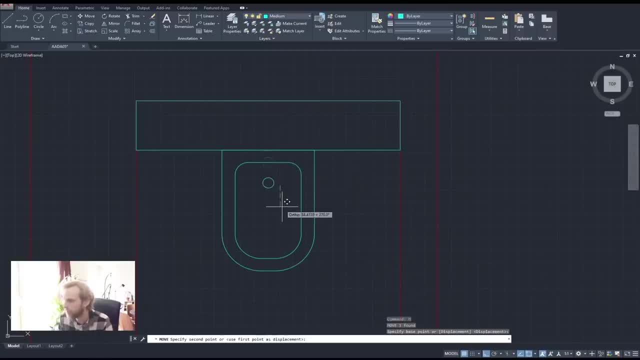 circle, circle? um the size of it doesn't matter. the? um the size of it doesn't matter. the? um the size of it doesn't matter. the positioning of it doesn't matter. positioning of it doesn't matter. positioning of it doesn't matter. um just to. to show maybe a little bit. 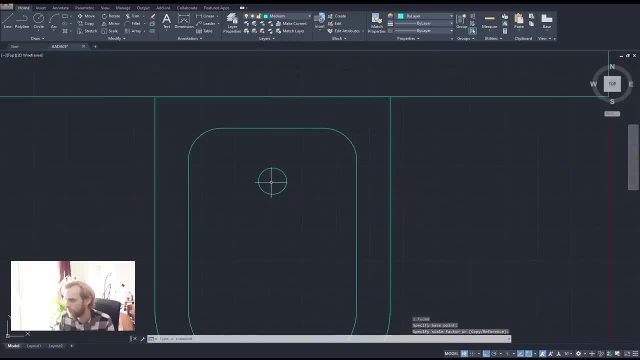 um, just to to show maybe a little bit. um, just to to show maybe a little bit bigger, just to show drainage bigger, just to show drainage, bigger, just to show drainage. come on, tail around the center point, uh, 1.5 times. tail around the center point, uh, 1.5 times. 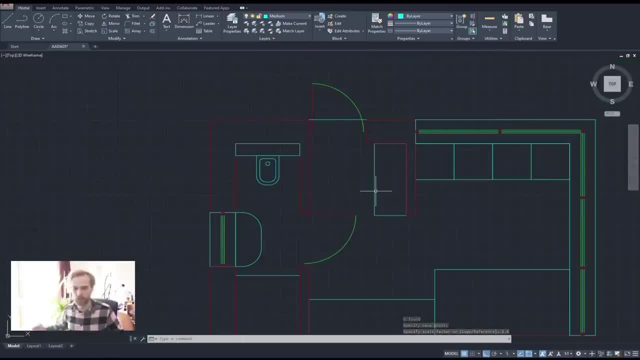 tail around the center point. uh, 1.5 times there we go, there, we go, there, we go. so we have a, so we have a, so we have a. a toilet right, a toilet right, a toilet right. i what, what, graphically, i like to do is: 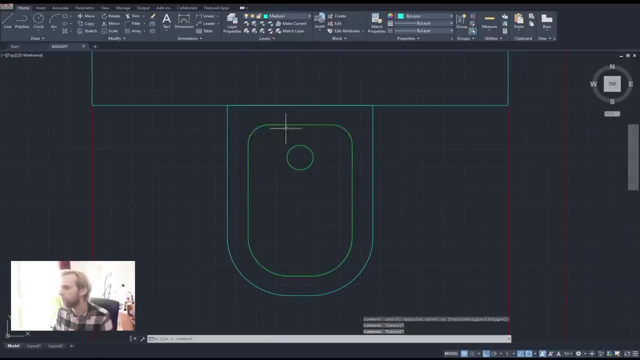 i what, what graphically i like to do? is i what, what graphically i like to do is this toilet right here, this toilet right here, this toilet right here. um, i like to, um, i like to, um, i like to make all of the inner lines thin, while 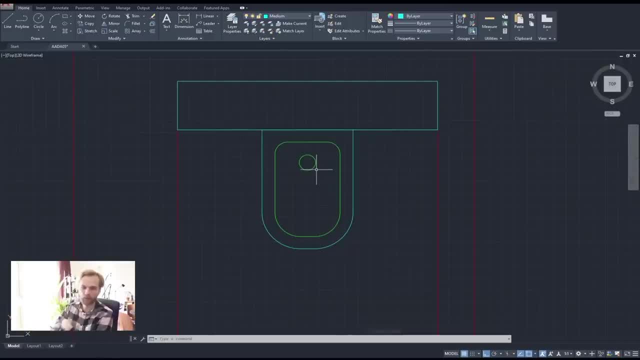 make all of the inner lines thin, while make all of the inner lines thin, while the outer line is, the outer line is medium right. we are not cutting through medium right, we are not cutting through medium right. we are not cutting through the toilet, the toilet, the toilet, um here in the shelf, in in the case of 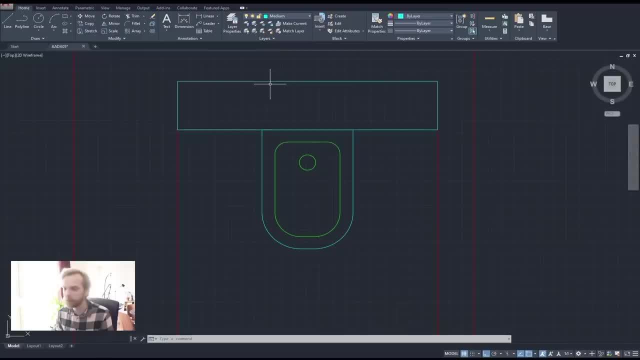 um here in the shelf in. in the case of um here in the shelf in. in the case of the shelf, we are cutting through it, but the shelf, we are cutting through it. but the shelf we are cutting through it, but it is a furniture piece, meaning that we 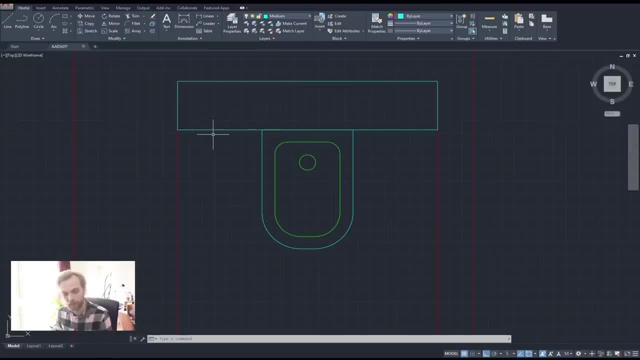 it is a furniture piece, meaning that we- it is a furniture piece, meaning that we are not going to be showing it, are not going to be showing it, are not going to be showing it. uh, in a thick line with a thick line. uh, in a thick line with a thick line. 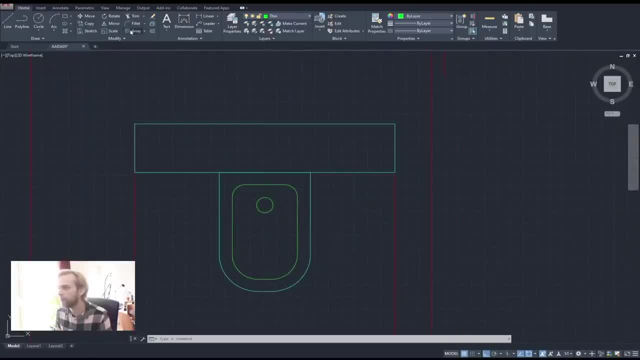 uh, in a thick line with a thick line. rather it is going to be a medium line, rather it is going to be a medium line, rather it is going to be a medium line, but it is going to have this kind of, but it is going to have this kind of. 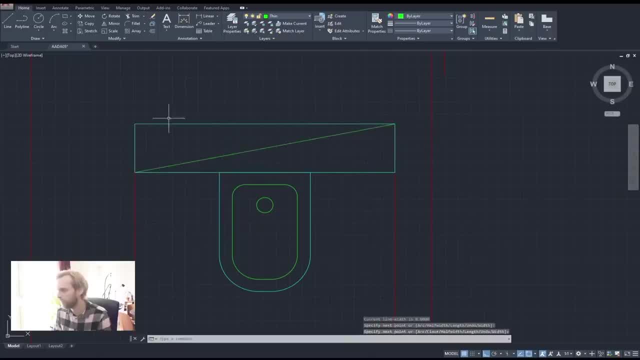 but it is going to have this kind of markup, markup, markup with a thin line, this with a thin line, this with a thin line, this, this, this, this, right, right, right. that means that this is a shelf. that means that this is a shelf. that means that this is a shelf. okay, same thing actually for this shelf. 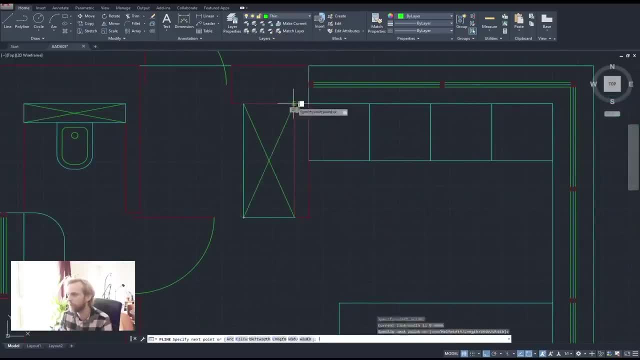 okay, same thing actually for this shelf. okay, same thing actually for this shelf as well. from here to here as well, from here to here as well. from here to here, and from here to here, and from here to here, and from here to here. right, right, right, or cabinet, i guess. 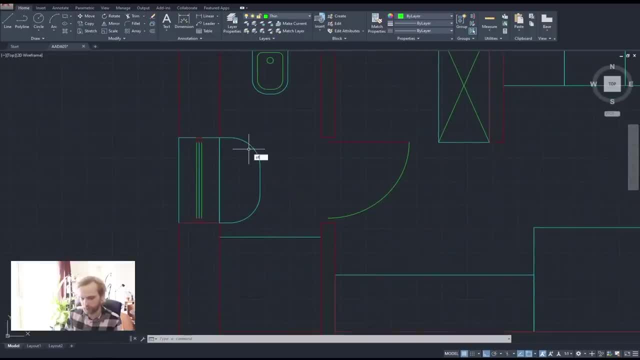 so we have that done now for the sink. so we have that done now for the sink. so we have that done now for the sink. same procedure, we offset. same procedure, we offset, same procedure, we offset, um, um, um. 50 sure, 50 is fine. 50 sure, 50 is fine. 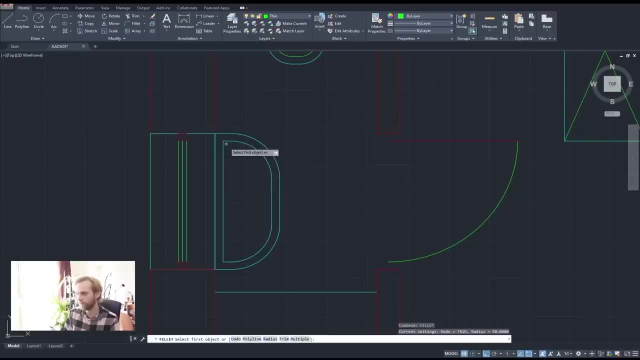 50. sure, 50 is fine. inwards, inwards, inwards, we fillet, we fillet, we fillet. radius 50.. radius 50.. radius 50.. um, i wonder if that's gonna be enough. um, i wonder if that's gonna be enough. 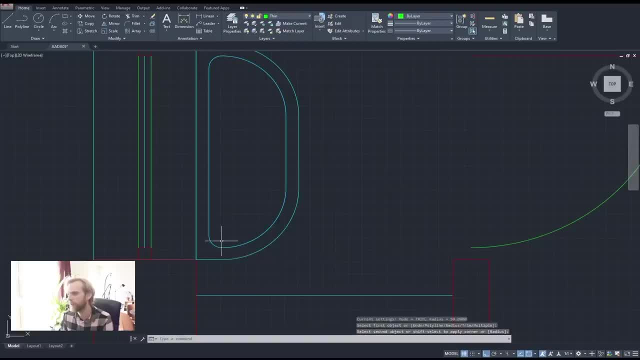 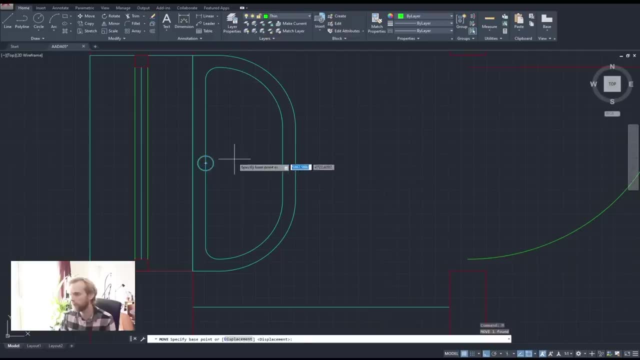 um, i wonder if that's gonna be enough. yeah, that's enough. actually. yeah, that's enough. actually, yeah, that's enough. actually, that, like that, that, like that, that, like that, i will create a drainage hole here. i will create a drainage hole here. i will create a drainage hole here. i'll just snap to the middle area. 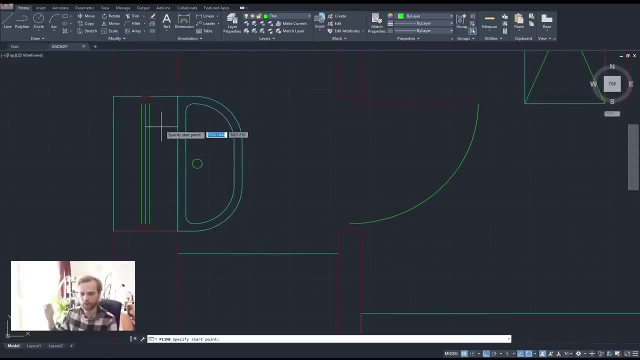 i'll just snap to the middle area. i'll just snap to the middle area. that that, that and i'll create a tap, and i'll create a tap, and i'll create a tap. you know where water flows from, so i'll. you know where water flows from, so i'll. 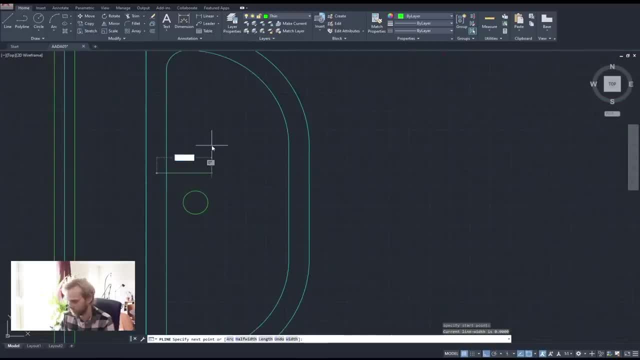 you know where water flows from, so i'll create a tap. create a tap, create a tap. uh, i don't know, 150 mil, maybe. uh, i don't know 150 mil, maybe, uh, i don't know 150 mil, maybe 50 mil or no, definitely not 50 mil. 20. 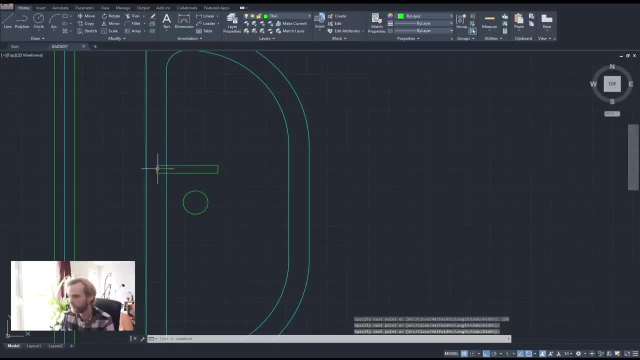 50 mil or no, definitely not 50 mil. 20, 50 mil or no, definitely not 50 mil. 20, 20 millimeters, 20 millimeters, 20 millimeters, 150, something like that, very simple, uh you. something like that, very simple, uh you. 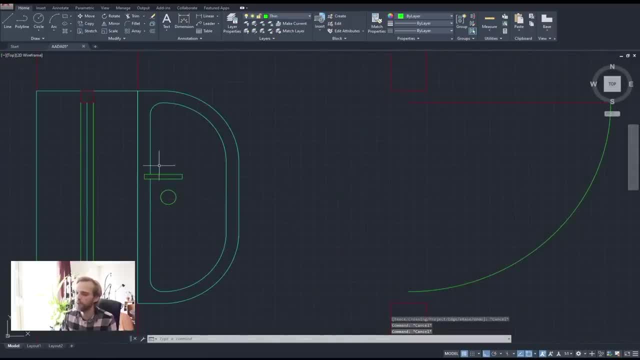 something like that, very simple. uh, you don't need to, don't need to, don't need to get rid of that. you don't need to get rid of that. you don't need to get rid of that, you don't need to have it super, super precise. 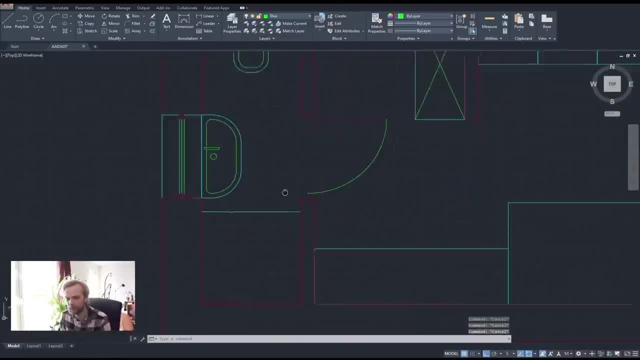 have it super, super precise, have it super, super precise, and this becomes a thin line as well. so, and this becomes a thin line as well, so, and this becomes a thin line as well. so that's our, our sink, that's our, our sink, that's our, our sink for the shower room. i think what we can. 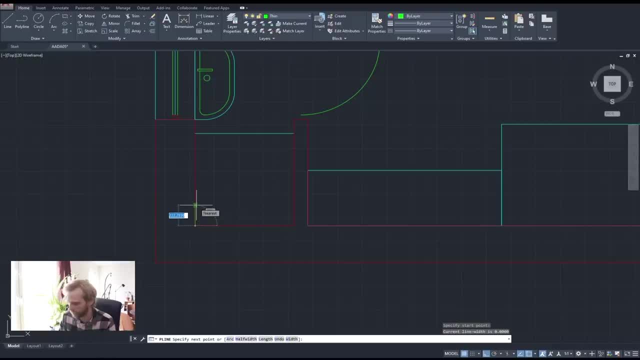 for the shower room. i think what we can for the shower room, i think what we can do, do do is add a little bit of shelving here is: add a little bit of shelving here. is: add a little bit of shelving here, just a tiny bit like 10 centimeters. 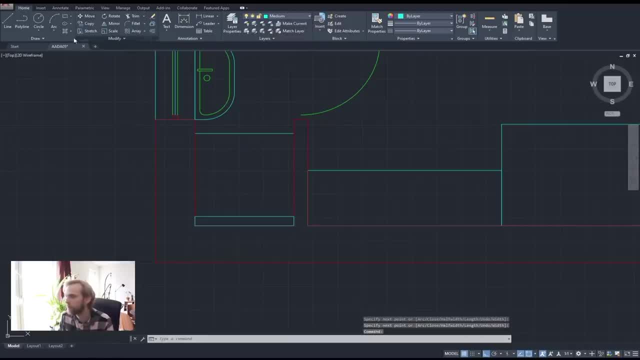 like that, like that, like that, uh well, uh well, uh well, that will need to be medium. this is for that will need to be medium. this is for that will need to be medium. this is for shampoo balls and and all of that good. shampoo balls and and all of that good. 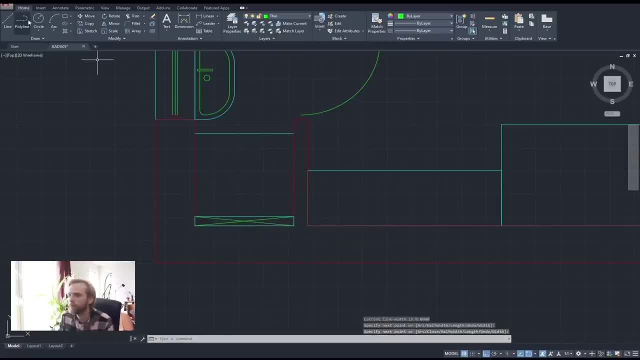 shampoo balls and and all of that good stuff, stuff, stuff. then create just a circle somewhere. then create just a circle somewhere. then create just a circle somewhere. i'll just snap to the midpoint. let's say i'll just snap to the midpoint. let's say i'll just snap to the midpoint. let's say here, and i'll say that the circle is 200. 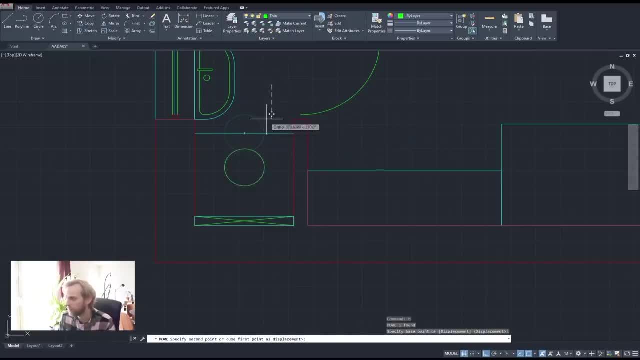 here and i'll say that the circle is 200 here, and i'll say that the circle is 200 millimeters in radius, millimeters in radius, millimeters in radius, and just move it probably somewhere here. so that's the. probably somewhere here, so that's the. 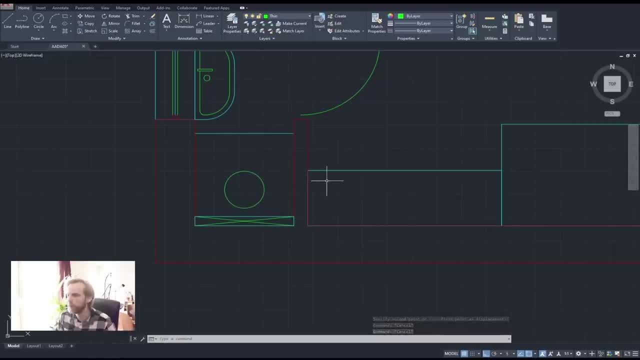 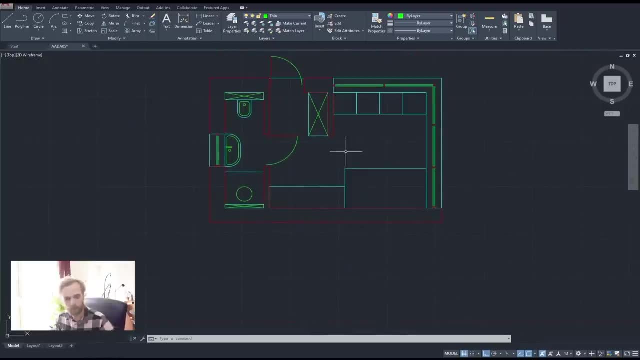 probably somewhere here. so that's the shower, shower, shower, shower head right, which will shower head right, which will shower head right, which will pour water, okay pour water, okay pour water. okay, the bathroom is done, the bathroom is done. the bathroom is done. the bathroom is indeed done. 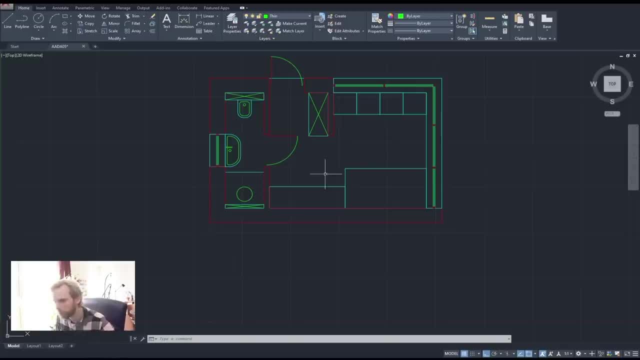 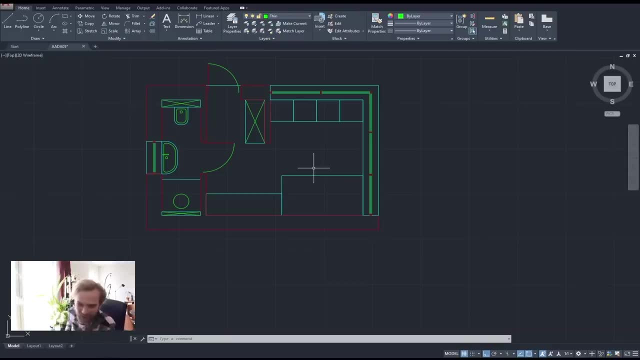 the bathroom is indeed done. the bathroom is indeed done. let's move on to the. let's move on to the. let's move on to the bedroom: slash workroom. slash kitchen. bedroom. slash workroom. slash kitchen. bedroom. slash workroom. slash kitchen. slash dining room, slash dining room. 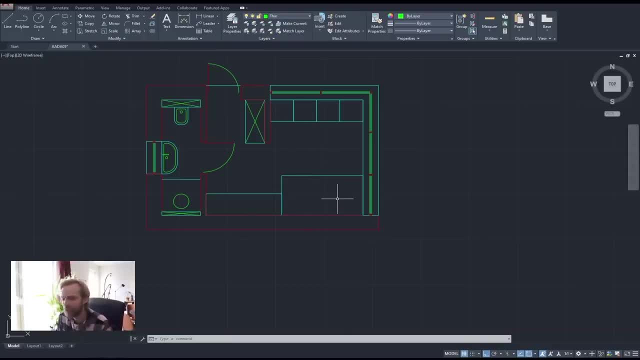 slash dining room, slash living room, slash living room, slash living room. um, um, um, to the rest of the space, to the rest of the space, to the rest of the space. um, i'll kind of work on this, uh, um, i'll kind of work on this, uh. 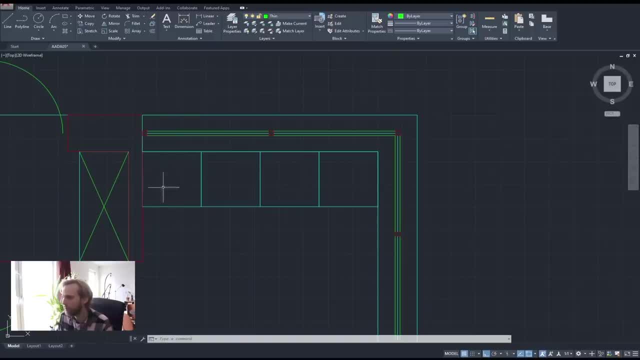 um, i'll kind of work on this, uh real quick. so i said that i want to real quick. so i said that i want to real quick, so i said that i want to have maybe refrigeration can go here. so have, maybe refrigeration can go here. so 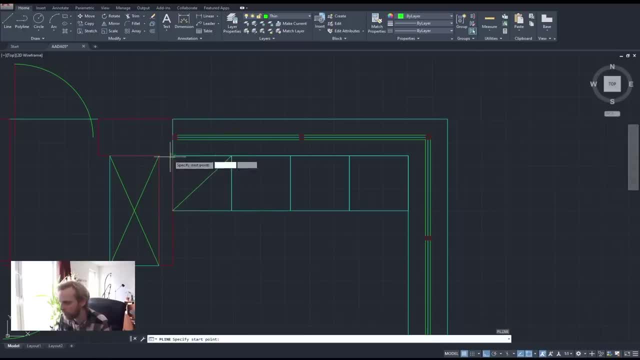 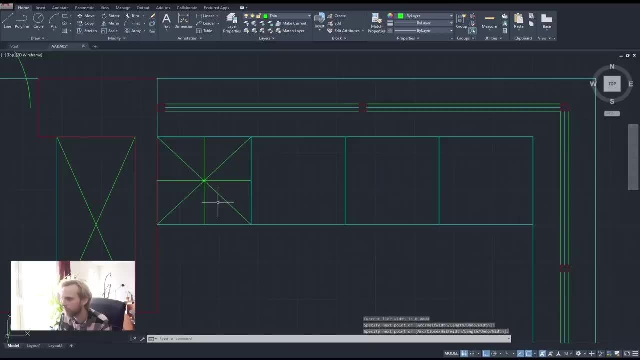 have. maybe refrigeration can go here. so refrigeration is basically just um. refrigeration is basically just um. refrigeration is basically just um. it's marked out like so, it's marked out like so, it's marked out like so, like that, like that, like that. then you take all of these lines and you 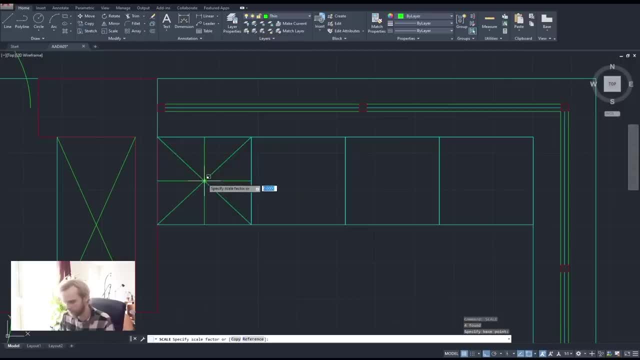 then you take all of these lines and you, then you take all of these lines and you scale them, scale them, scale them. scale to the center point by 0.3, scale to the center point by 0.3, scale to the center point by 0.3. let's see: 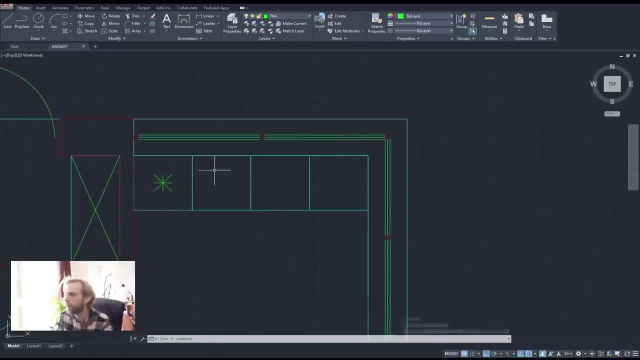 let's see, let's see like that, like that, like that that's refrigeration, that's refrigeration, that's refrigeration. uh, then you have, uh, uh, then you have uh, uh, then you have, uh, so you take your food out, you kind of. so you take your food out, you kind of. 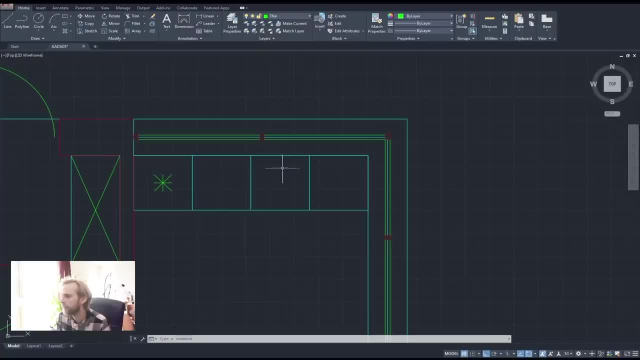 so you take your food out. you kind of want to place it, want to place it, want to place it and then, and then, and then it's a little bit cramped. okay, you take the food out, do you want? okay, you take the food out, do you want? 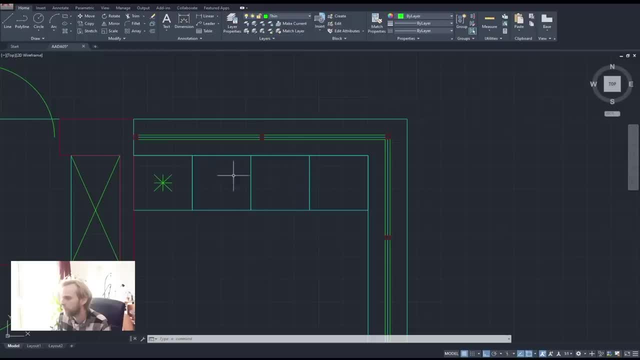 okay, you take the food out. do you want to place it immediately? to place it immediately. to place it immediately. or do you have placement here and you? or do you have placement here and you, or do you have placement here and you? cook here, cook here, cook here and then wash here, take out. 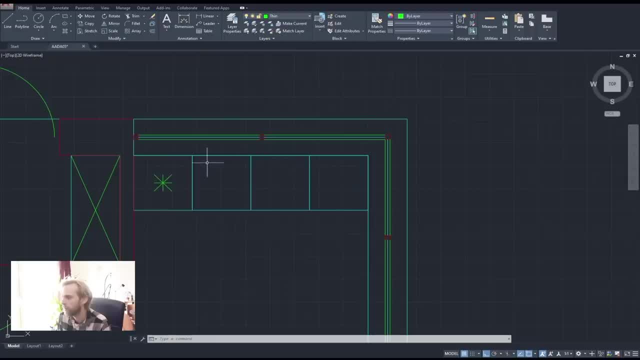 and then wash here, take out, and then wash here, take out wash, wash, wash cook place. take out wash place. cook, yeah, cook place. take out wash place. cook, yeah, cook place. take out wash place. cook, yeah, so okay, so this is going to be a sink. so okay, so this is going to be a sink. 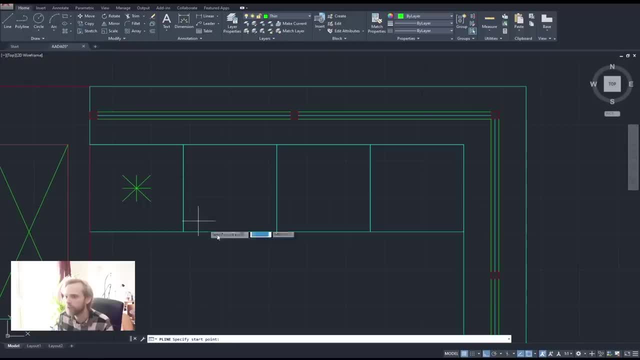 so okay. so this is going to be a sink, and for the sink, i'm just going to, and for the sink i'm just going to, and for the sink i'm just going to. um, let's, let's just draw, draw out some. um, let's, let's just draw, draw out some. 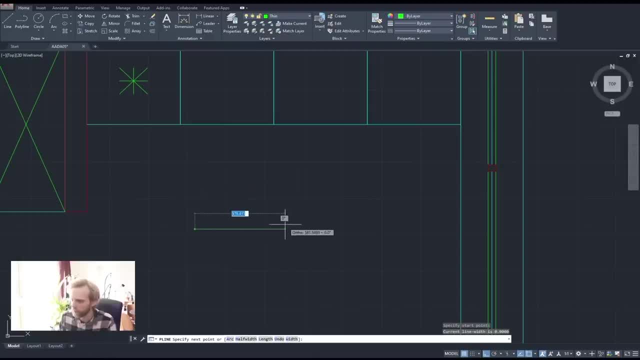 um, let's, let's just draw, draw out some sort of polo line. that's going to be sort of polo line. that's going to be sort of polo line that's going to be um the width of the sink. let's say, is um the width of the sink? let's say is. 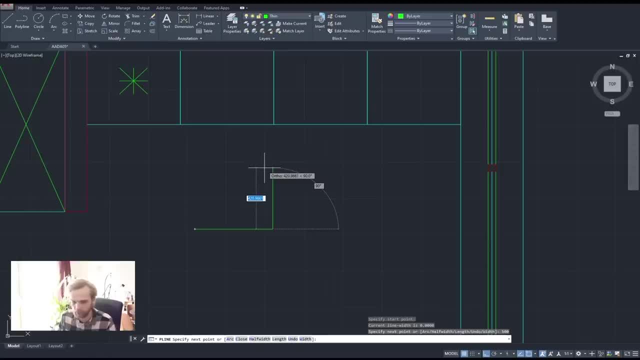 um. the width of the sink, let's say, is 500 millimeters. the length of the sink: 500 millimeters. the length of the sink: 500 millimeters. the length of the sink, or the or the or the. sorry, the length of the sink is 500. 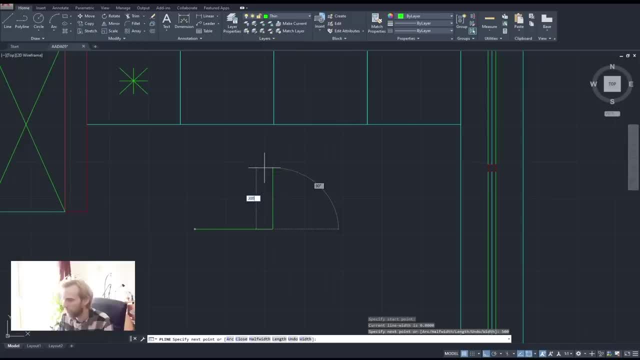 sorry, the length of the sink is 500. sorry, the length of the sink is 500 millimeters, the millimeters, the millimeters. the depth of the sink is going to be like. depth of the sink is going to be like depth of the sink is going to be like 300 millimeters, not more than that. 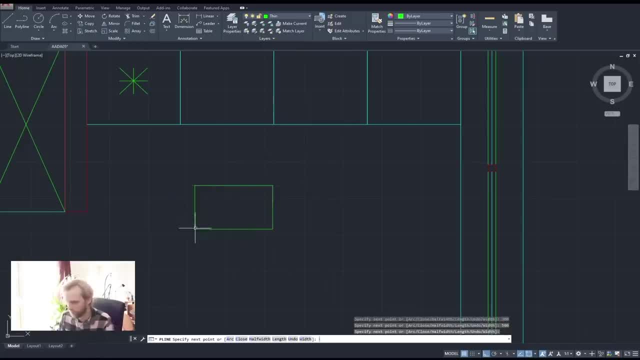 300 millimeters, not more than that. 300 millimeters, not more than that. um 500, finish up, um, 500, finish up, um, 500, finish up. fillet, fillet, fillet, um, and then we just fillet it with uh um, and then we just fillet it with uh. 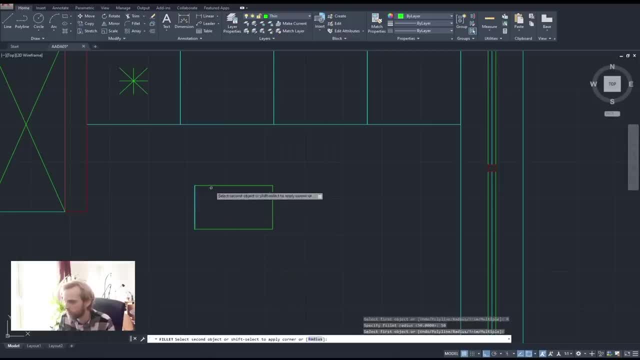 um, and then we just fillet it with: uh, just a little bit of a radius, i'll just just a little bit of a radius. i'll just just a little bit of a radius. i'll just give it like five centimeter radius, just give it like five centimeter radius, just. 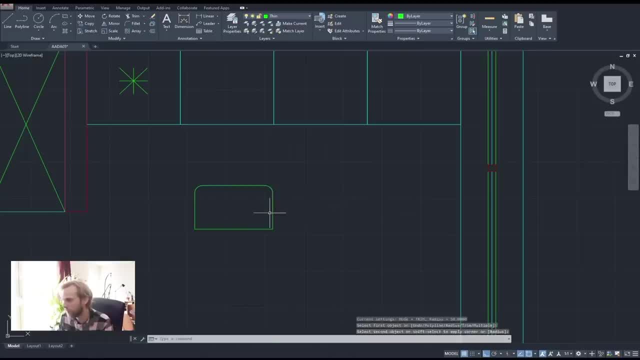 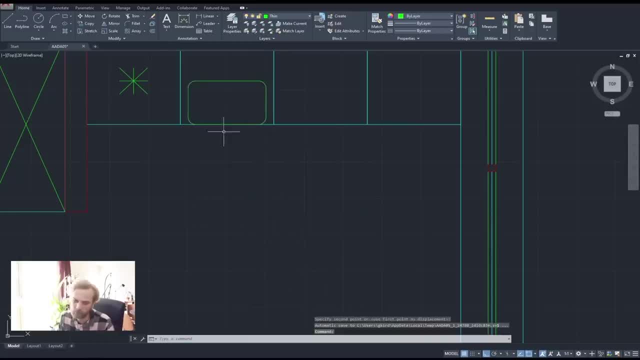 okay, i'll just take the sink then and move. okay, i'll just take the sink then and move it from the center point here, it, from the center point here, it, from the center point here to the, from the middle point there to to the, from the middle point there to. 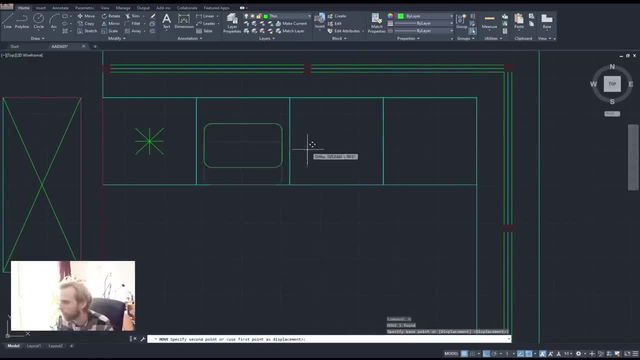 to the, from the middle point there to the middle point there and move it the middle point there, and move it the middle point there and move it inwards, inwards, inwards into the cabinet by 50 centimeters, into the cabinet by 50 centimeters. 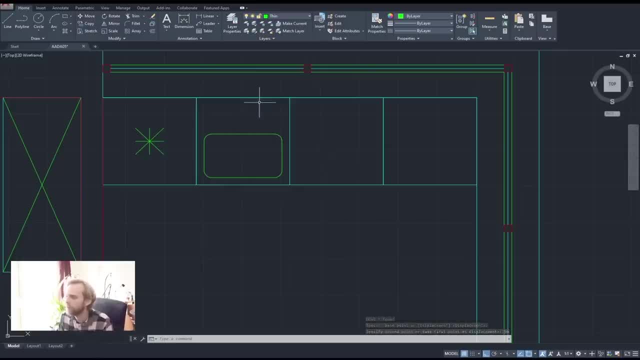 into the cabinet by 50 centimeters, something like that. oh, 50 millimeters, something like that, oh 50 millimeters, something like that, oh 50 millimeters. sorry, sorry, sorry, something like that, so that you have a, something like that, so that you have a. 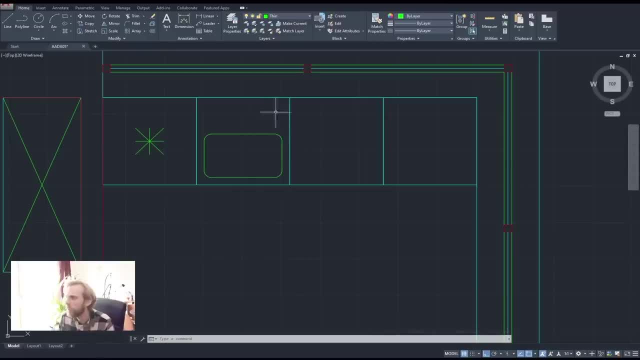 something like that, so that you have a little bit of little bit of little bit of area to to place your stuff in in here. area to to place your stuff in in here. area to to place your stuff in in here. i need a tab, so i'll just borrow the tap. 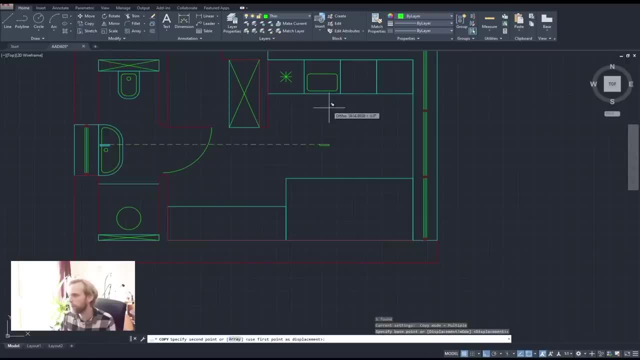 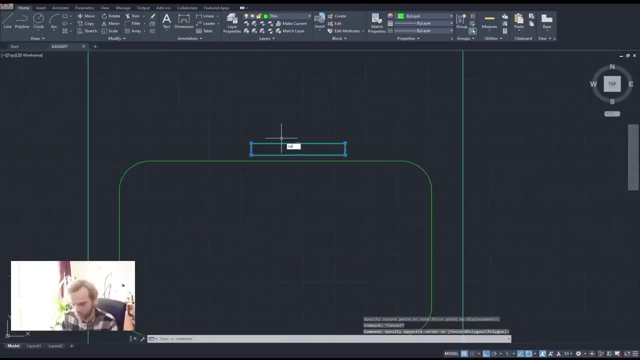 i need a tab, so i'll just borrow the tap. i need a tab, so i'll just borrow the tap from here. copy: move it here. of course it needs to be. move it here. of course it needs to be. move it here, of course it needs to be rotated. so i'll rotate it. 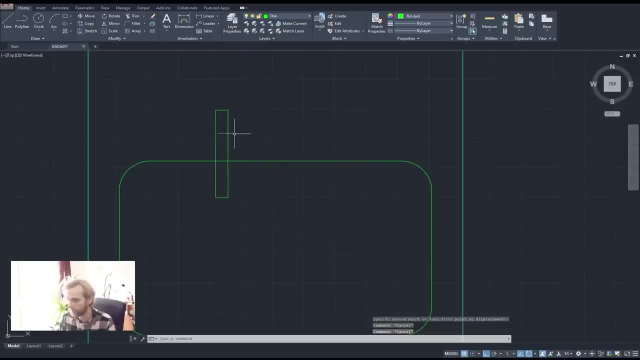 that actually fine the way it is, but i that actually fine the way it is, but i that actually fine the way it is, but i like to like to like to have them off center. have them off center. have them off center. that trim, that trim, that trim. 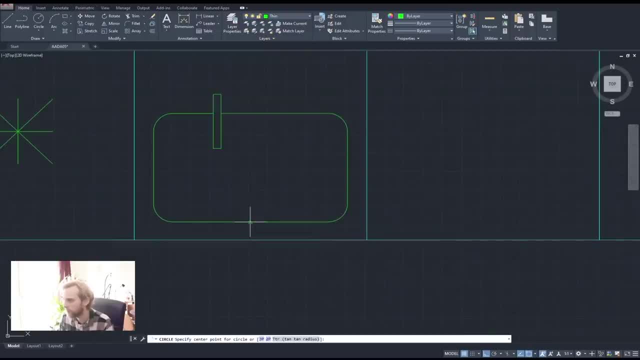 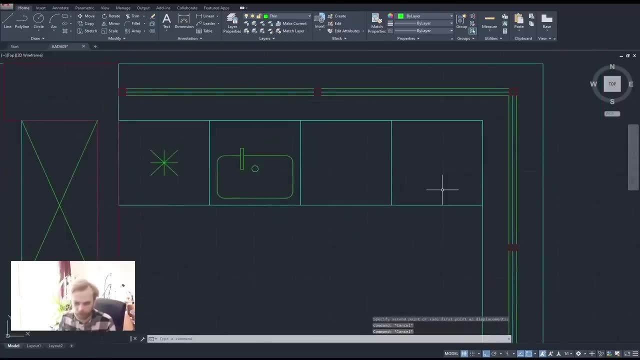 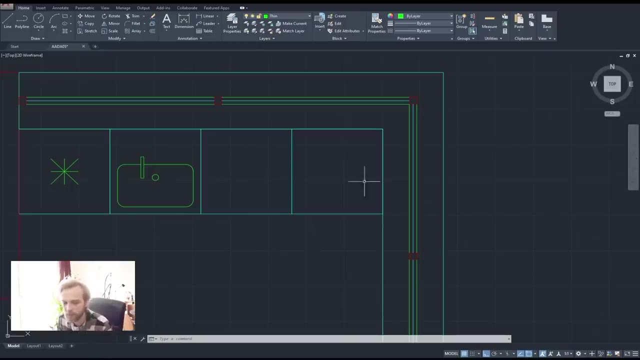 in that way. i'll create a circle here around this midpoint. the size doesn't matter. like that. that's our sink, right? nothing, nothing more than that. then this is just a cutting area, so we don't need to do anything with it. and this is our cooking area- cooking stove. so 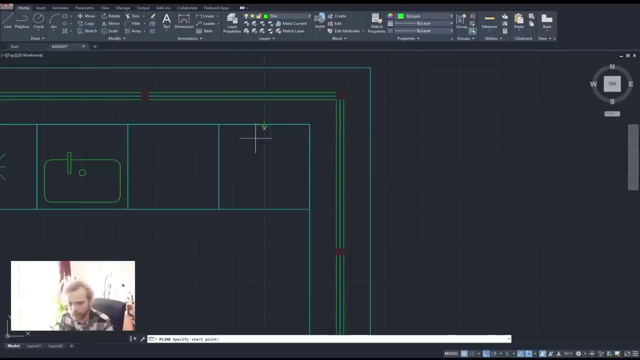 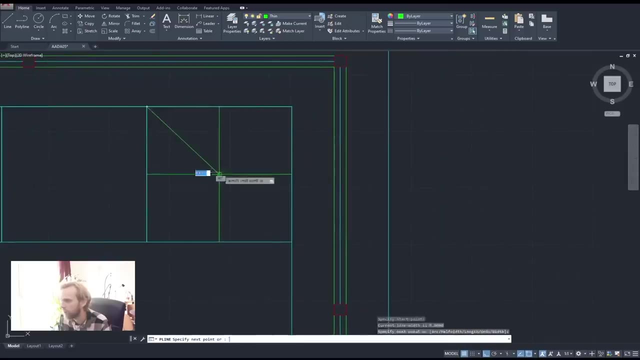 cooking stove is basically, um, it just has four, uh, heater blocks, right? so what i'm going to do is i will just be a little bit cheeky and i'll separate all of this into four, four segments, and then, for each of these four segments, i will just create this kind of a diagonal line and you'll. 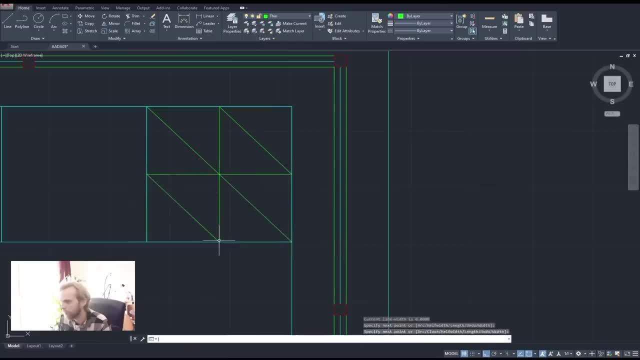 understand why i'm doing this in just a second. so i have these diagonal lines here, um, each of them have a center point right and i can use those center points to show, you know, to use as as center points for my circles which will show, show the heater blocks for the stove right. so usually you have two that are. 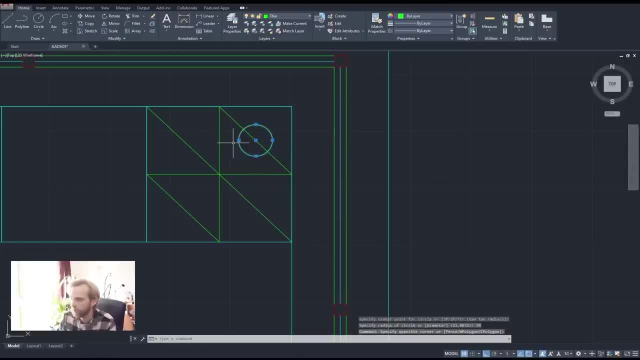 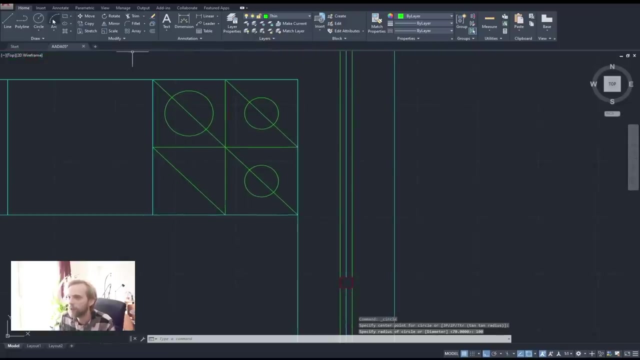 in same same size. so i'll just use 70 millimeters for this one, 70 millimeters for this one. then you have one pretty large one, uh, so this one, let's say, is going to be 100 millimeters, and you have one, a pretty like, pretty small. let's do 50, 50 millimeters. 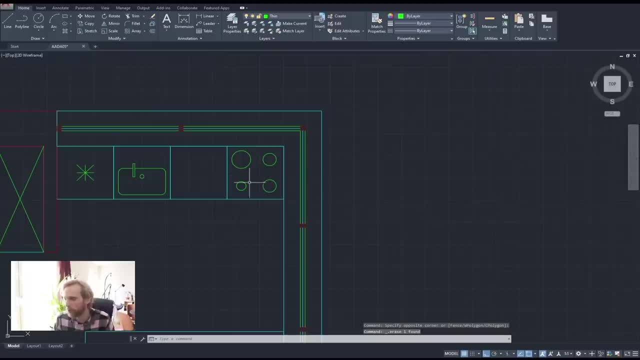 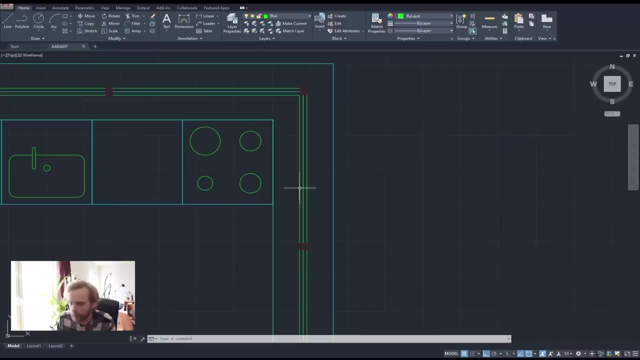 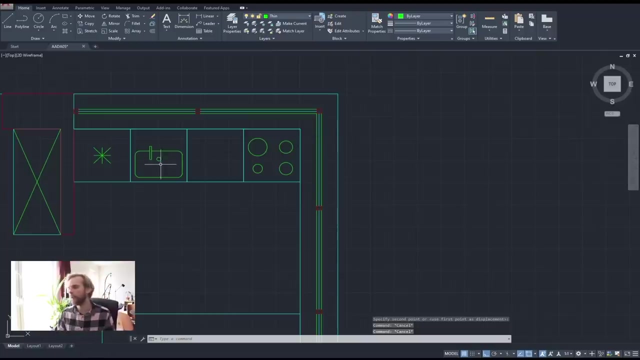 you just have to make sure you have that right. you don't need anything else. i just have those, those four heater blocks. uh, looks bad. why does it look bad? that's because it's too close to the, to the edge here. but well, maybe we can just do this and no one will know. it's better, okay, um, that's it. 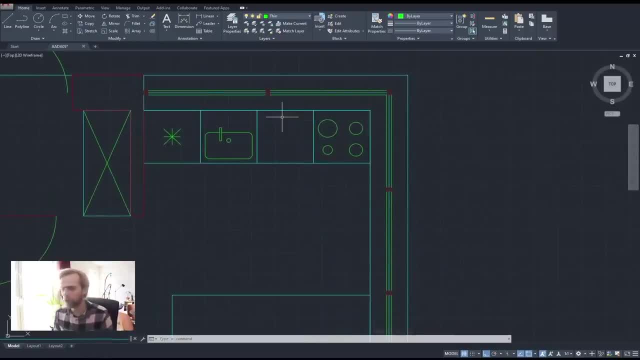 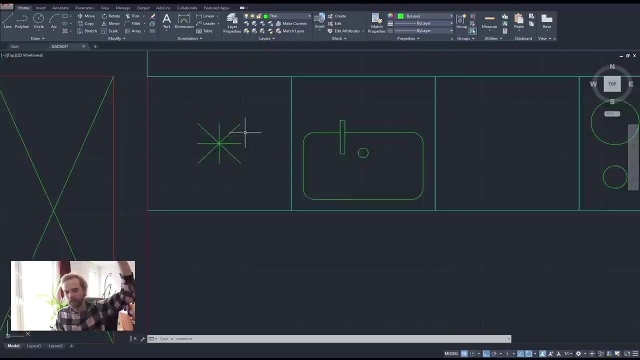 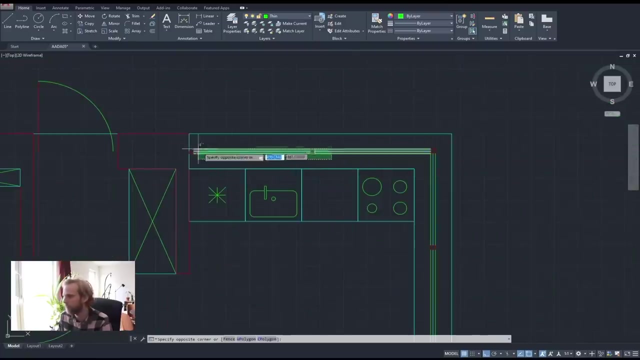 that's it with the kitchen. uh, i will want to draw a cabinet above, above the, or maybe i don't want a cabinet. I need to fix one thing: the refrigerator is high, right, and the window is going to be behind the refrigerator, so this is a bad design, right? so I'm going to remake this, this whole area, right here. 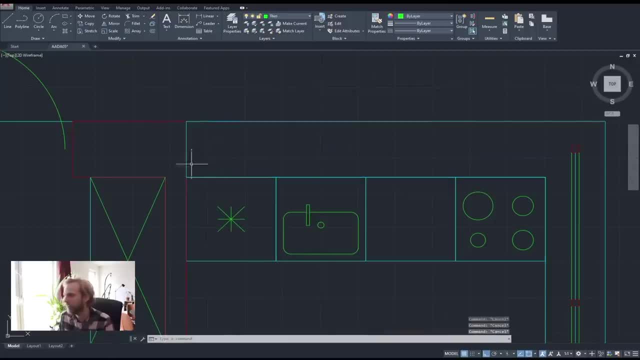 that's my bad, sorry about that. so actually, this, this wall right here, it needs to extend until the end of the refrigerator. so I'm going to: how do we do this? well, let's, let's first create that, that wall segment here. or rather, first let's, yeah, but let's create the wall segment here, like that: 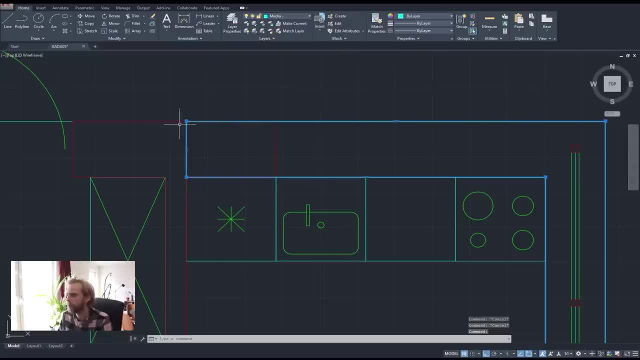 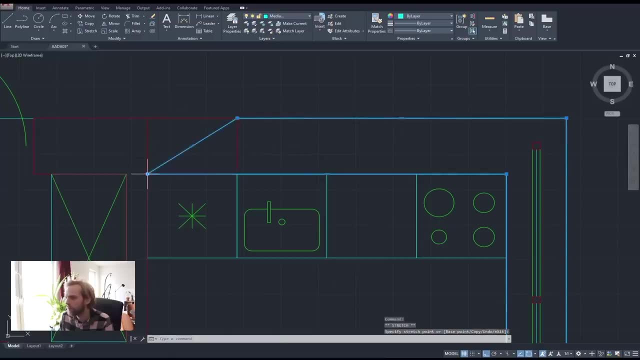 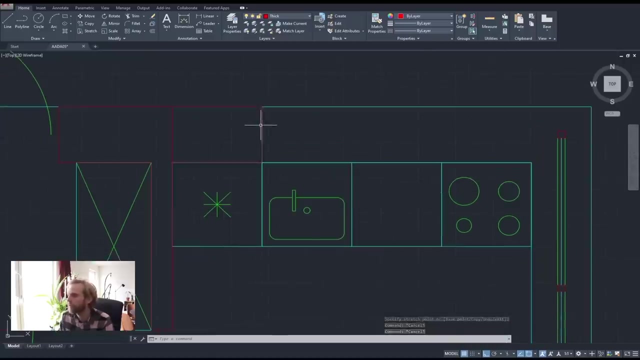 perfect, now let's actually select the blue- uh, blue- windowsill line and move its points from here to here. you can also do trimming and so on, but just moving those points around, this is fine, so we do that, then we. then we trim, enter, enter, we trim away this area right here, like so, and we join everything back up, so this is joined. 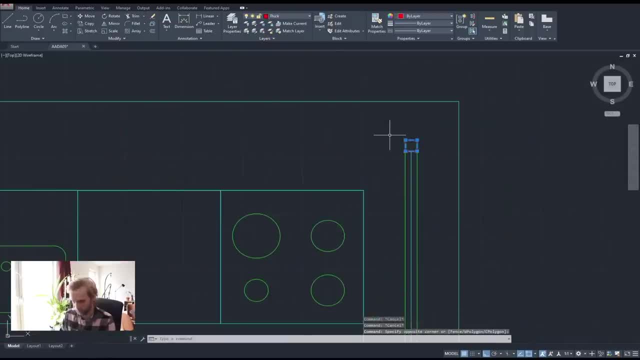 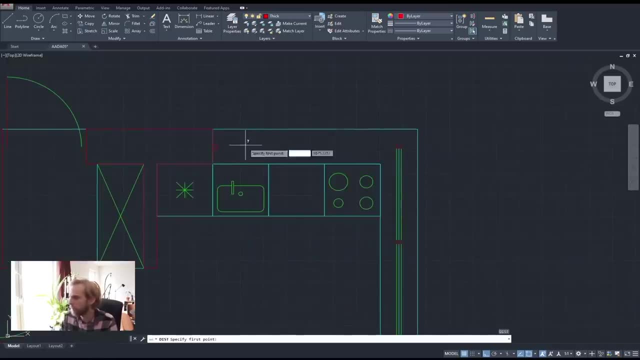 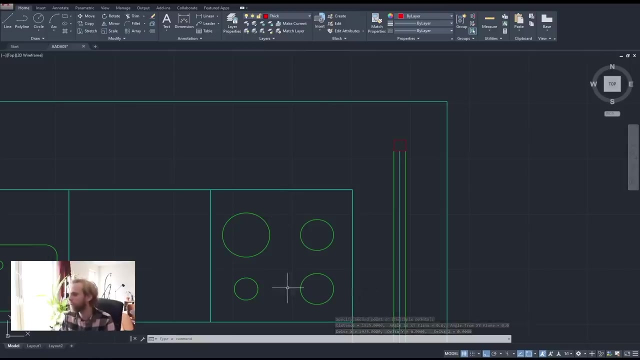 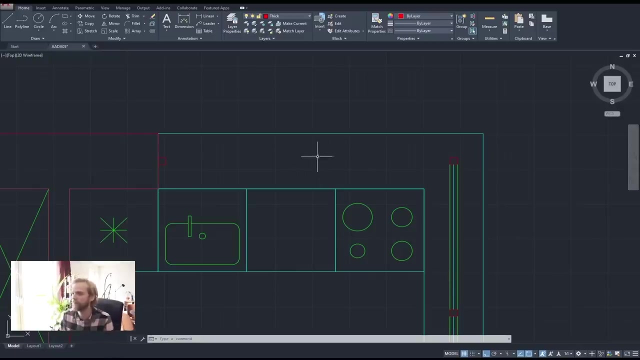 that's clean. that is also clean, okay. so now I will take the frame copy from here to here. how wide is it from here to here? we have one point: almost two meters. that's still too wide, so I'm going to: oh, it's not that wide, but no, I'll still add a division here. so if it's actually, I'll show you another way of how to do this. if you justend itsiere. 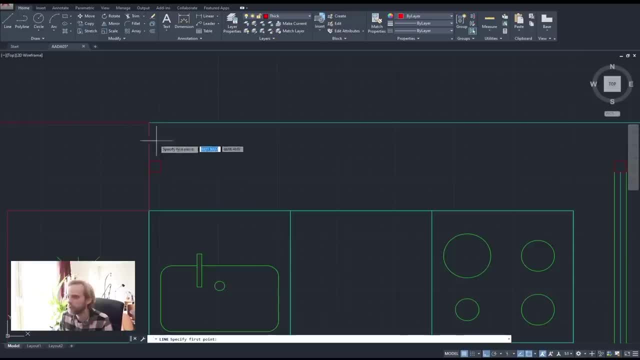 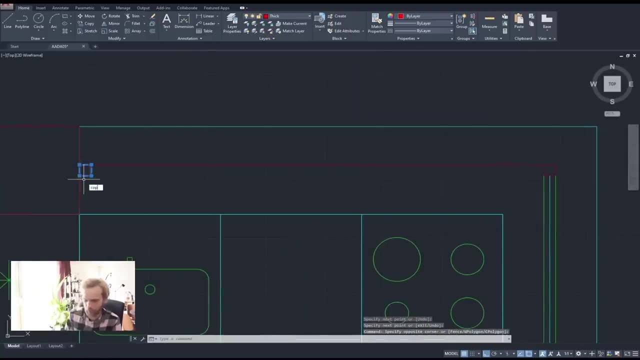 here. so if it's actually, i'll show you another way of how to do this. if you just draw a line segment here and you use the midpoint of that line as your helper, copy from the midpoint here to the midpoint here and then delete the helper, you don't really need to do any maths, it's right. 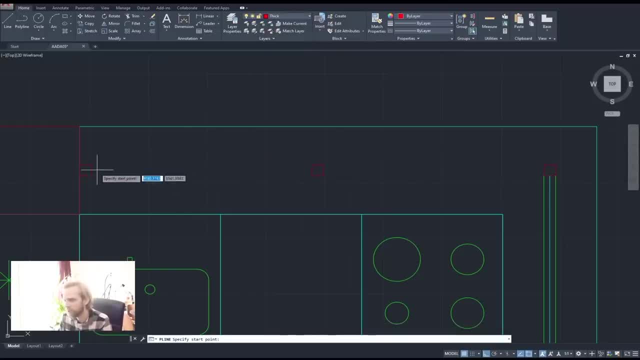 in the middle. that's kind of useful. um, actually i'll just draw out the lines in one layer and then just switch the switch the layers around of already existing lines. oh man, the sun is shining. that's not usual. you need to do this. that's not usual in sweden. 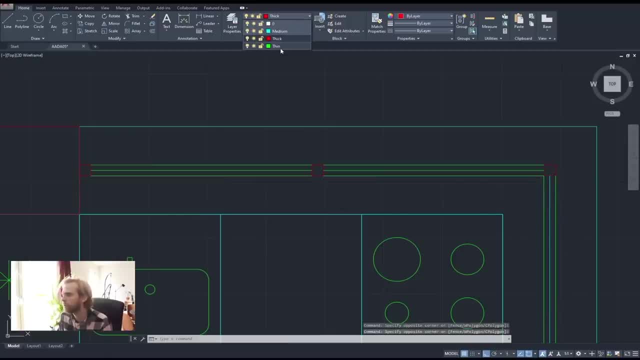 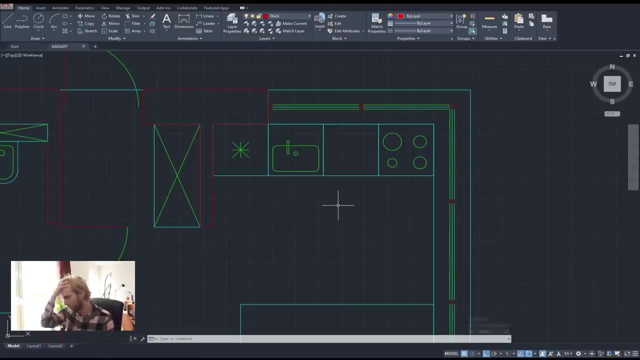 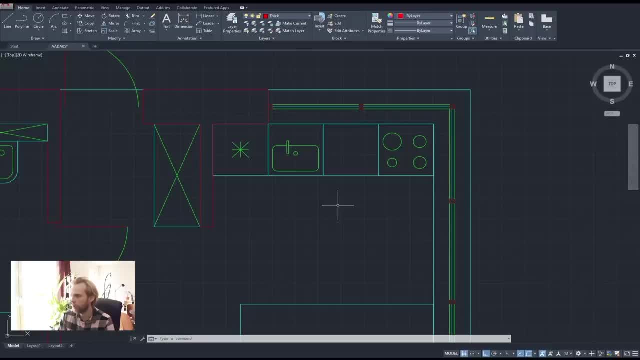 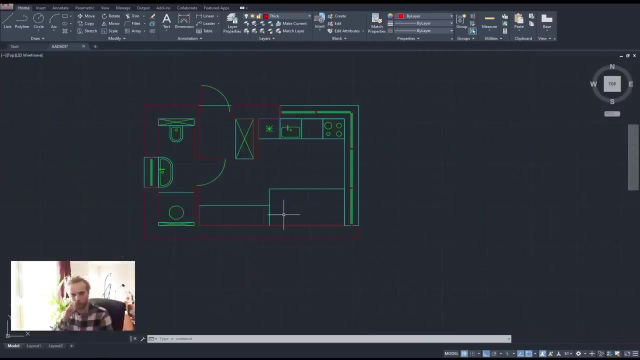 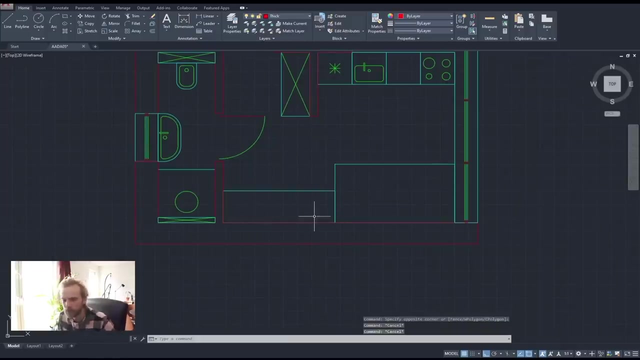 i will add a cabinet above, like near the ceiling, but i will do that later, not now. um, let's solve this and then we'll move on to um, to creating the section. so this, we have our table right. that's just a table. we don't really need to add anything to it. 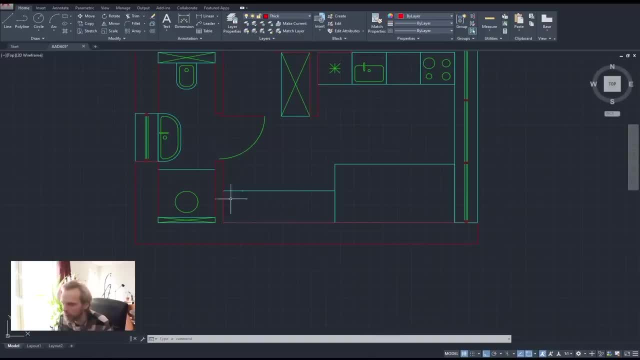 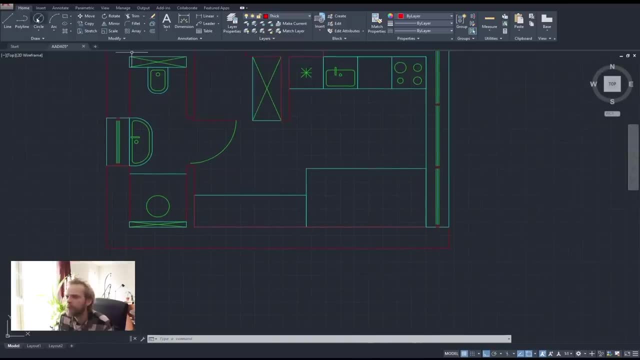 if you want, you can add a monitor or you can add some books and whatnot. you know, you can make it more lively. but it's just a table, so that's fine. and we have a bed, so for the table i need a chair. so i'll just kind of create a circle. that's uh. 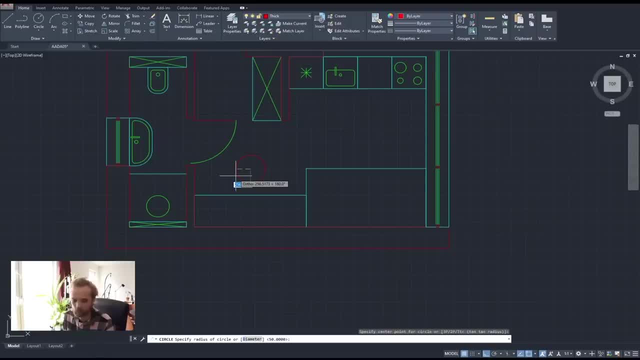 let's go for um radius of a chair. radius of a chair, let's say um 20 centimeters, so 40. 40 centimeters in time, no, that's, that's too too little circle. let's let's do 50, so 25 centimeters in radius, something like that, and my chair is going. 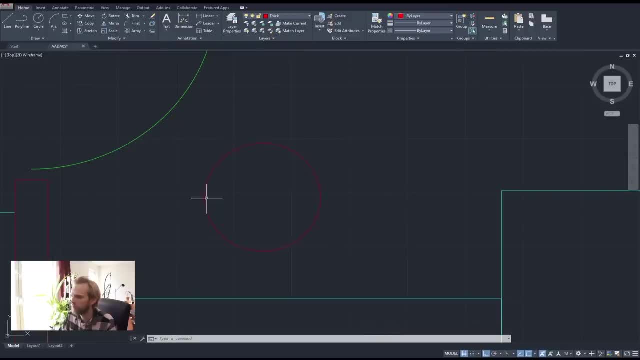 to. let's say it has a bag brace, that is an arc, so i will just offset it inwards by five centimeters. i'll just grab the, i'll just create a two line tools here, or two lines here to both sides, um, and then i'll just go to town trimming everything that i don't need. so i trim enter. 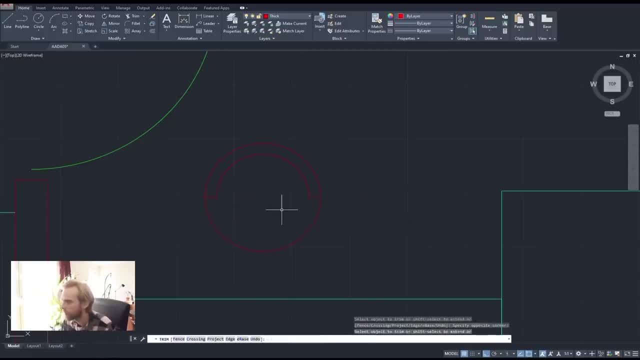 enter. i don't need this, this, this or that. that's it. um, this whole thing gets joined. so now it's it's a single pole line and this is another line, or rather a circle. so here, this guy right here is going to be medium, this guy right. 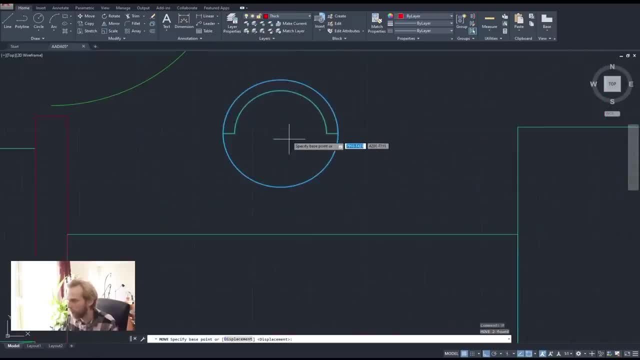 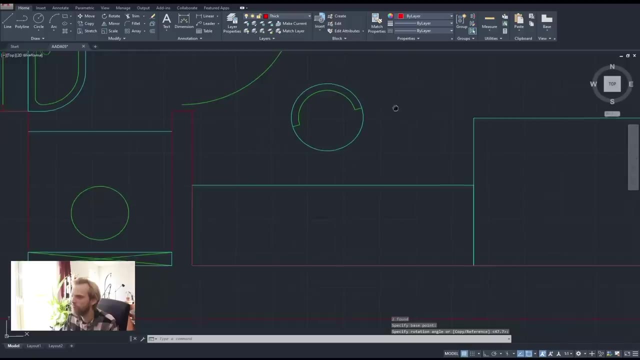 here is going to be thin and the chair is going to be. uh, what i like to do is i like to rotate, um, rotate the the chair just a tiny bit. that's not a tiny bit, so let me rotate it back, uh, just a tiny bit to make it more lively, and place it underneath the table slightly. 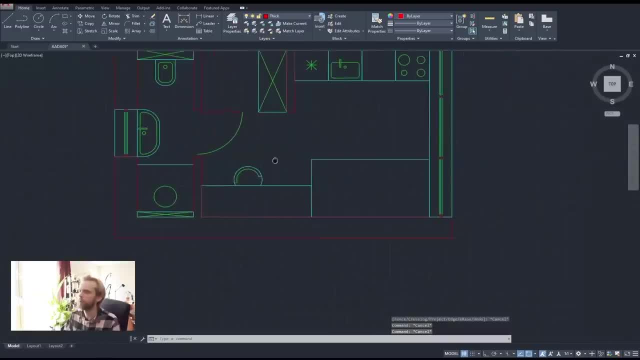 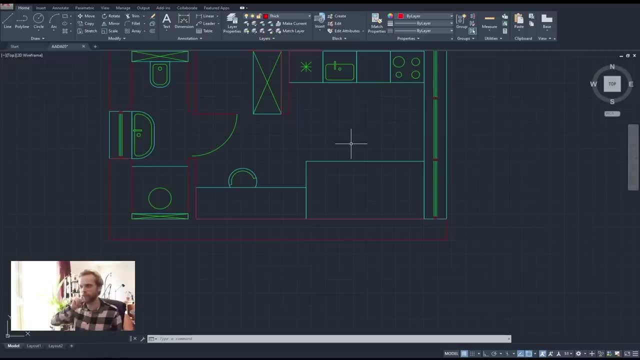 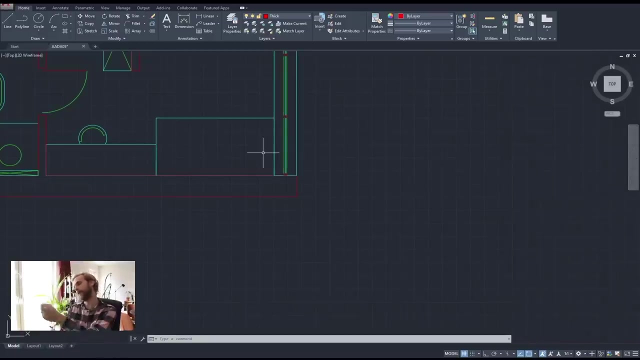 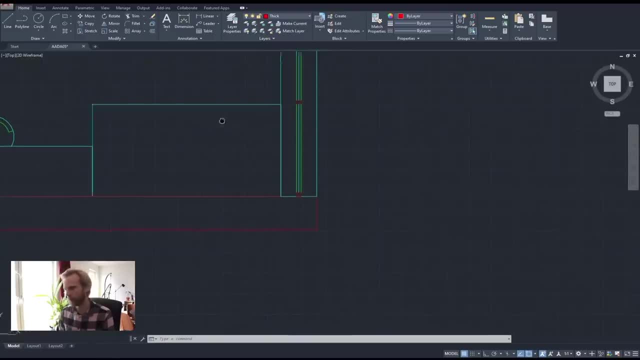 and the bed sheets right to show this as a bed. so that's not going to be tricky. i'm going to just grab a rectangle tool and i'll just make two random rectangles for the pillows. the pillows are not that accurate, so i can kind of get away in making weird ones. just for reference. i'll measure the distance. 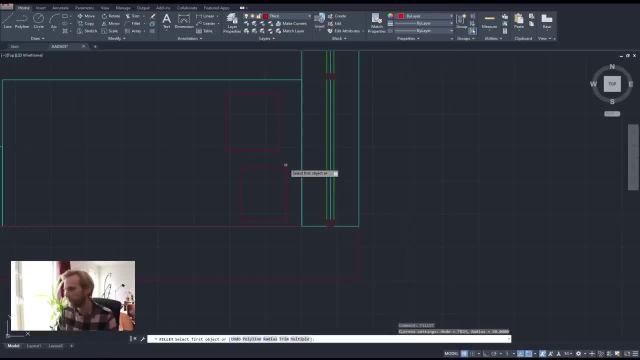 which is 300 millimeters. so i will fillet all of the pillows by um 130 millimeters or 140 millimeters, right? so all of the corners get deleted. wait, that's again. fillet, r, enter, 140, enter. ah, enter, 140, enter, fillet. 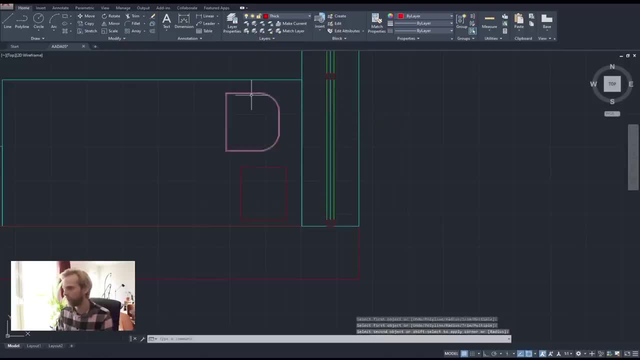 enter 140, enter, enter, 140, enter. it works okay. So just fillet, fillet, fillet, fillet. Right now I should probably I forgot to mention one thing. There's one more snapping option that you can accidentally enable, and that's called 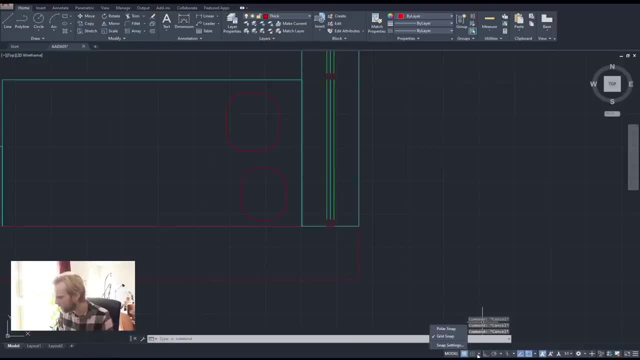 grid snapping, which I believe is- yeah, it's right here- Snapping mode grid. If you have this turned on, then your cursor, or when you're trying to draw something, it's going to snap to the grid lines like: so. That is obnoxious and I 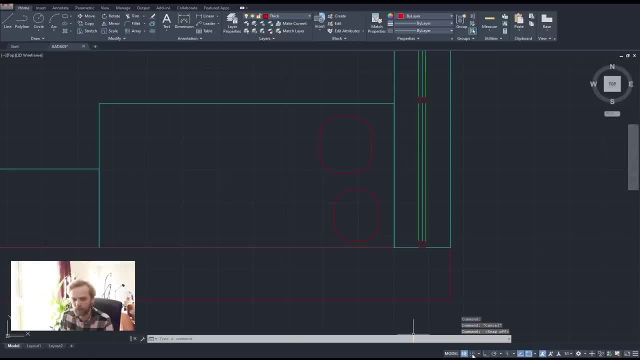 absolutely hate that. So just make sure that grid snapping right here in the bottom is turned off right. Just a tip. Okay, so we have two weird pillows here: One large one, one smaller one, that's that. So we have two weird pillows here: one large one, one smaller one, that's. 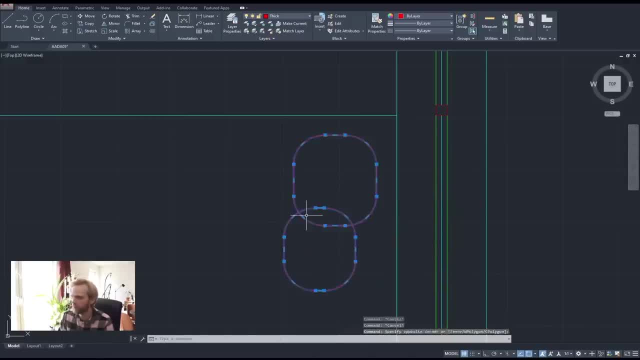 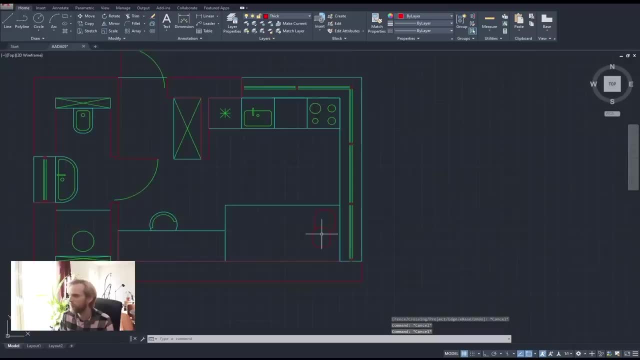 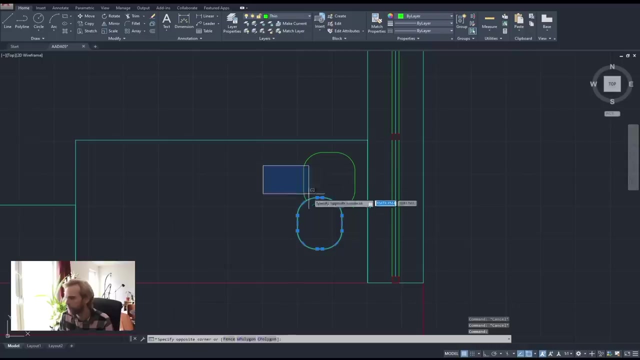 that's fine. I can actually place them together and trim the, let's say, the large one with the small one, like that, Like that I will make them thin, like so. So those are two pillows and let me just position them a little bit more centered. 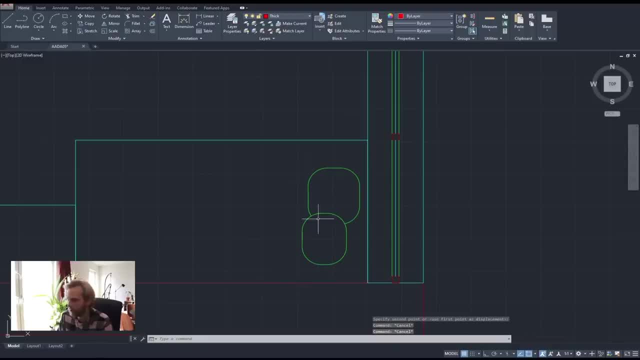 like so. Then we have a bed sheet that will go over the pillows. so I just kind of goes over them like so right, and it's trims away half of the pillows. that is the bedsheet, and the bedsheet usually that the way I. 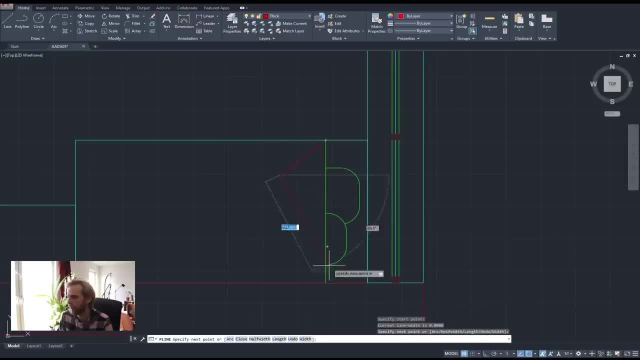 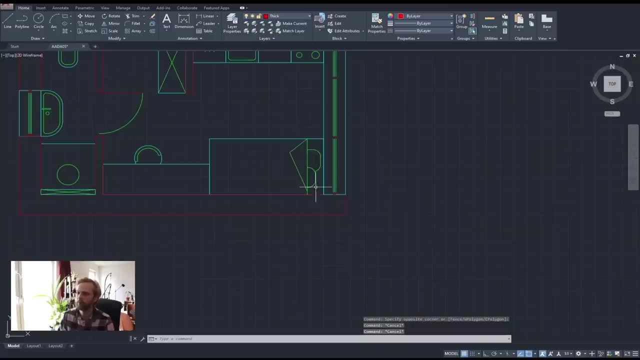 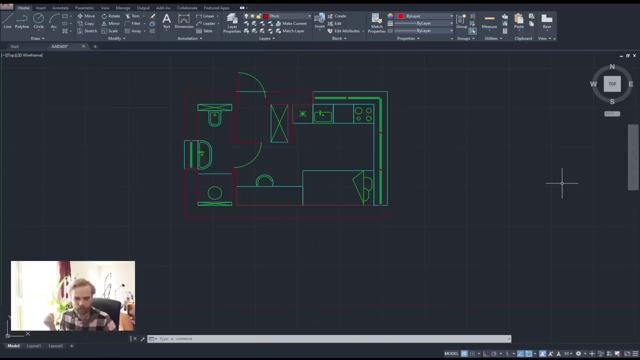 personally prefer doing it, is it? it has this kind of a fold here. all right, so it's. it's: fall that, fall that out. that's it. that's, that's the bed, with two pillows kind of tucked away behind the bedsheet. all right, we have this, this plan, then the plan. let's move on to creating a section. so 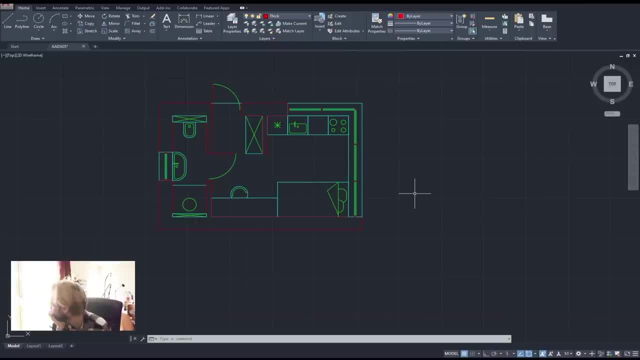 or or no, sorry, well, maybe just a second I'm gonna think. can we move into the section making? yeah, let's move into section making. so the first thing that we want to do is we want to mark out where we're going to cut the building through, right with. 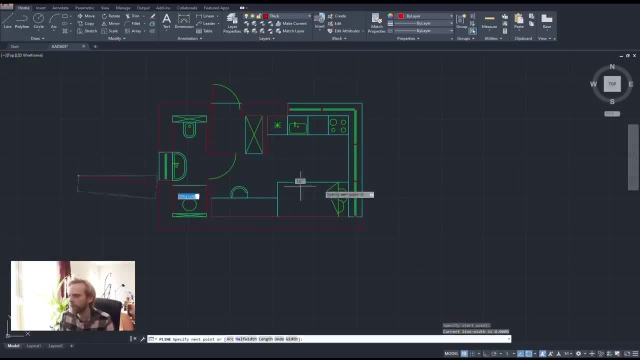 what's the cutting line. so I'm just going to create a straight line segment- it's like that- and I'm just going to see where with the move tool, where I can position it so that it cuts and shows the most things. so my thoughts are- and usually you don't want to cut through the furniture, you either. 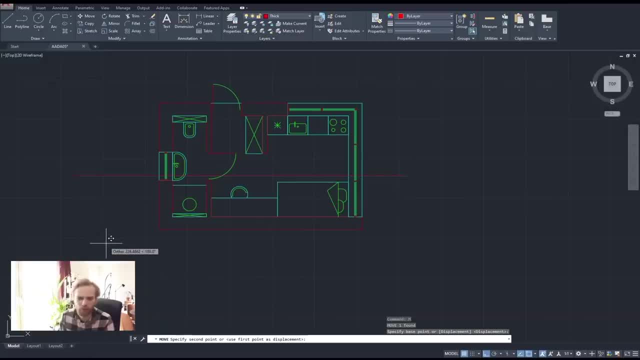 show the furniture in the projection of the cut. or you or you don't right, but you don't cut through the furniture. in this case, we are going to be cutting through the sink, but that is fine. if you are cutting through furniture, you you're not hatching it in, so you're not filling in the cut. that is important. 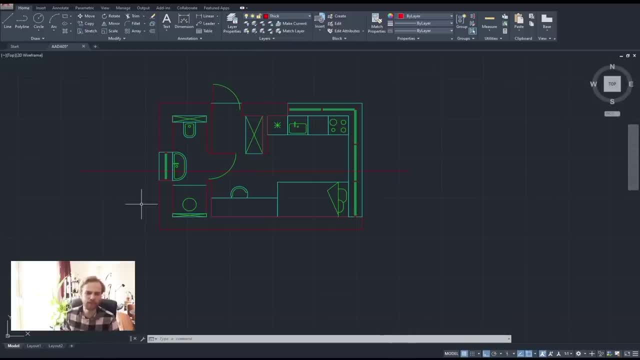 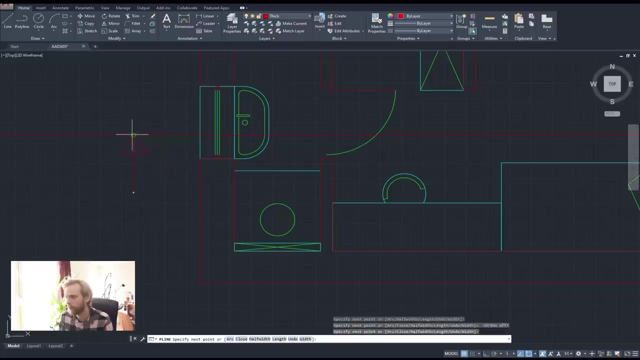 to note. You're just showing it as if it's in the projection. Let's do that. I think we can do that because we will see quite quite a bit and my viewing direction is going to be that way, Right? So I'm going to see, I'm going to be. 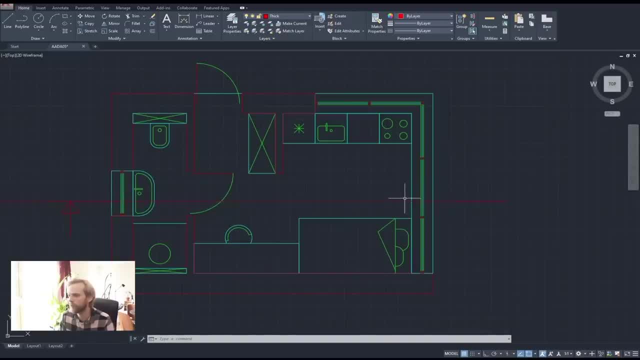 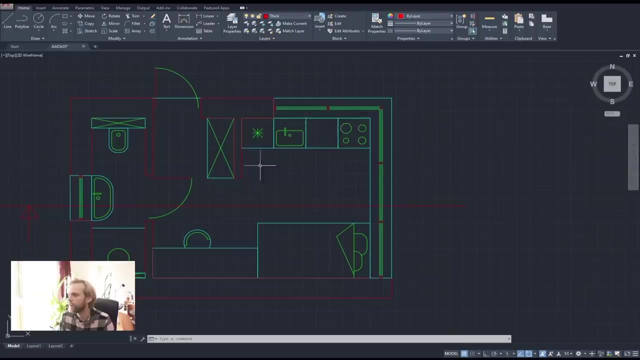 cutting through the window, through the sink, through the door, through another door, through another window. I'm going to be seeing the door, the side of the, the cabinet here, or the side of the shelf here, the kitchen area, kitchen. 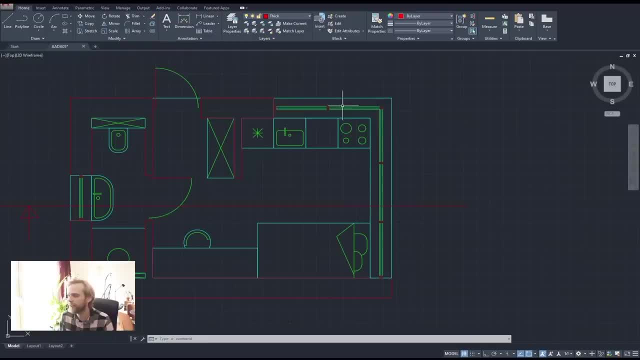 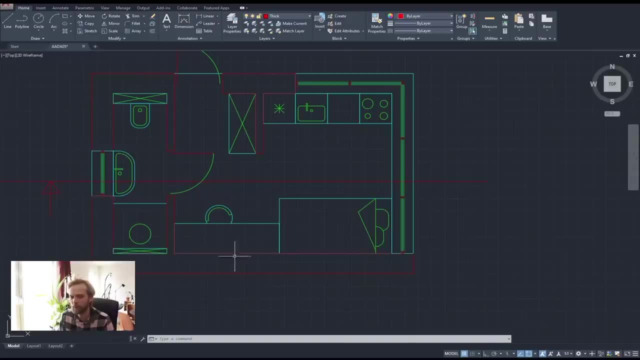 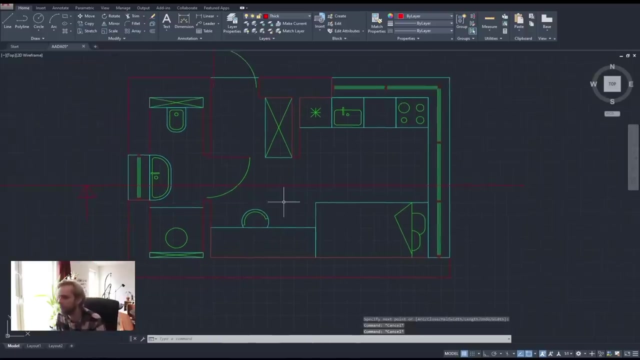 front. I'll see the side of the window and the toilet. What I won't see is the shower, the bedroom or the bed and the wardrobe. I'm going to be seeing the work table, which is fine. It's, you know, you can't add. 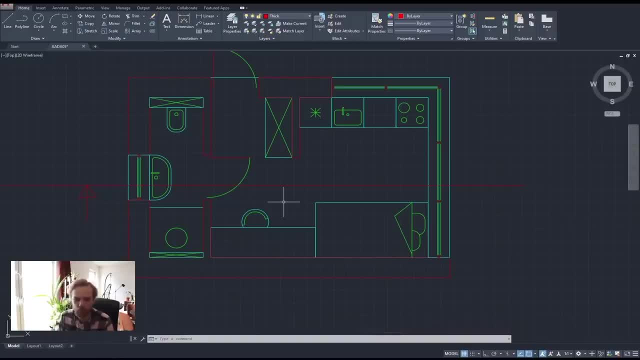 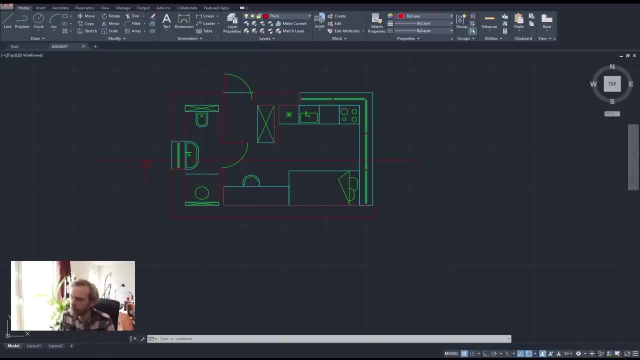 everything to a single section. Usually you need to do more than one section to show everything in the building. That's fine, So the way I really like doing this is: first I will go to layer properties here and I'll just create a new layer. 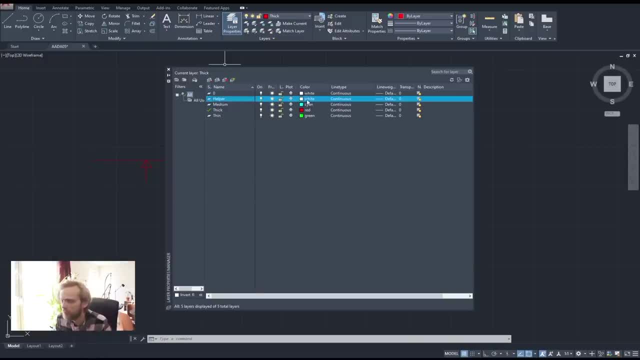 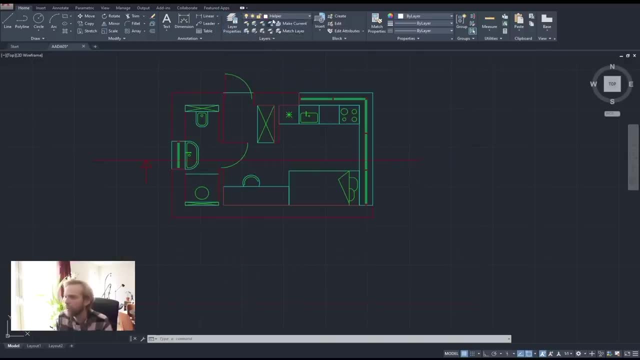 and I'll call it helper. Helper layer, and it can be white, that's fine. Just a single additional layer. I'll make it my active layer. So that's my helper, And what I want to do is basically make a cut here. So I need to have all of the correct dimensions. 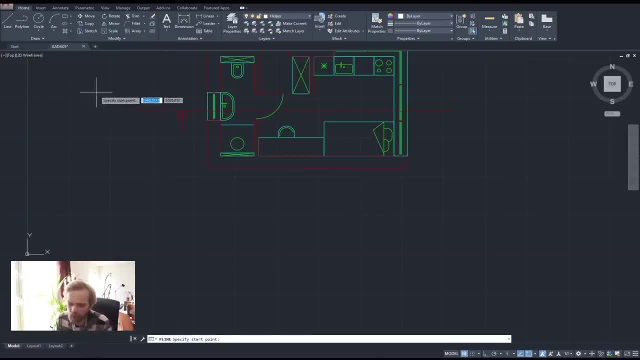 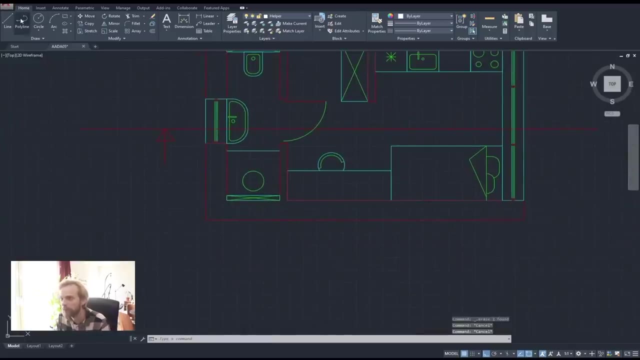 So my workflow- and it might be, I think it's a workflow of everyone who uses AutoCAD- is just dragging out, just dragging out the lines, or maybe I should draw it from here, just so that it's it's clear, more clear for you. 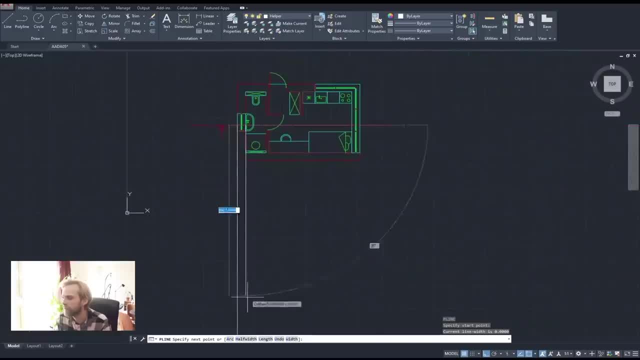 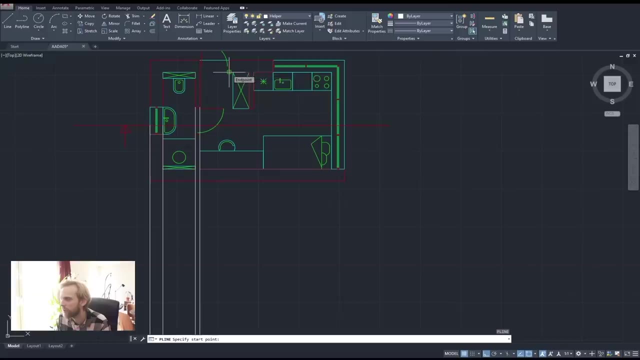 Dragging out the main lines. that that I want to. I want to keep working with right. That I will see in this section So that that can come in later. Well, no, Let's, let's do it now, Like that? Then this is going to be a line. 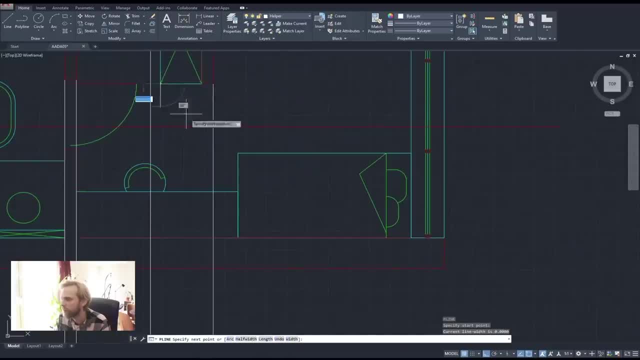 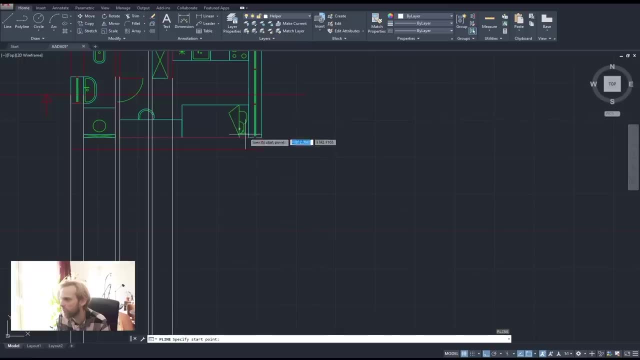 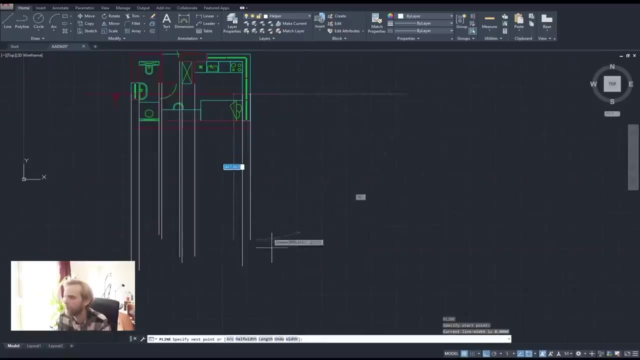 This doesn't necessarily need to be a line, but I will. I'll add it. Then we have the whole kitchen area. So this edge right here is going to be a line, And then we will have the last line here. So we have a bunch of like vertical lines extended. There's like 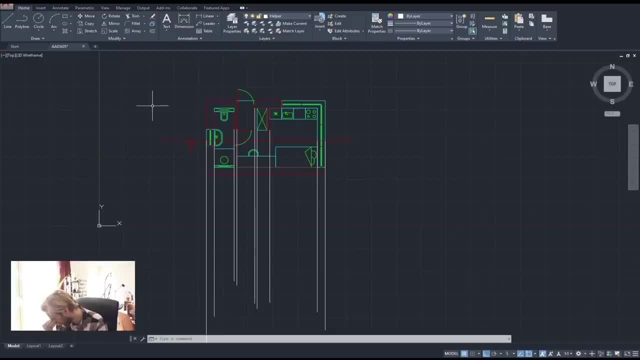 that I forgot the name of it. Just a second, Okay. Okay, How is it called Construction line? I think it's construction line. Yeah, So there is one more tool that can be used and it's called construction line. 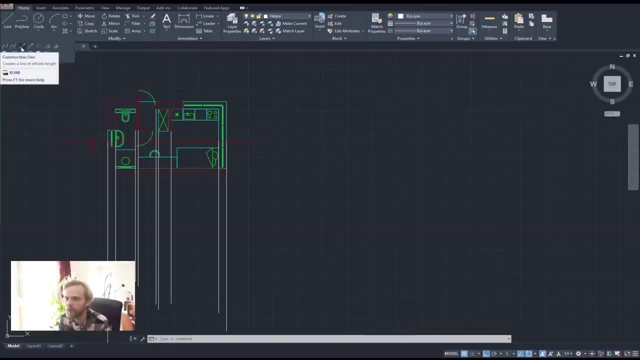 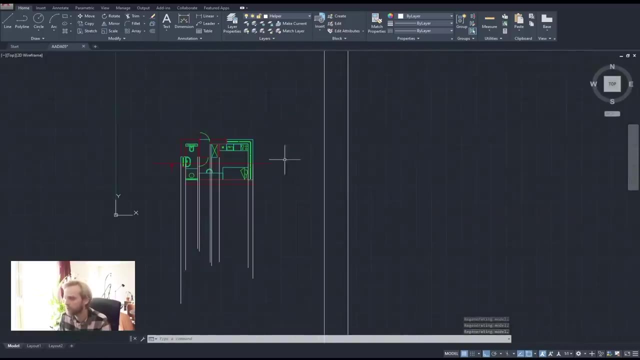 So it's, it's located right here, Or the shortcut for it is X line, And the thing about X lines is that they are X or infinite in length, right, So you can use construction lines, but this is a very simple project, So I'm not. I'm not really using them right in this case, So I'm just dragging. 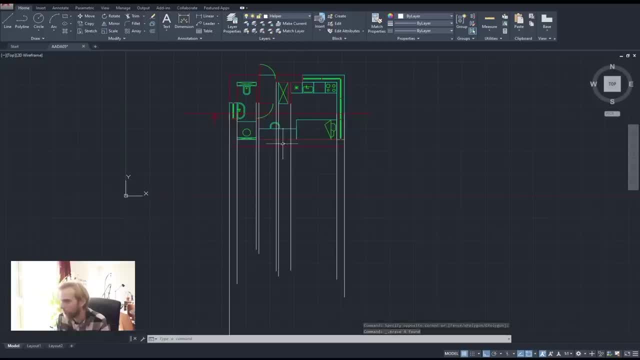 out regular ones, Right? So we have that, And now I will just start drawing. right, So I'll create. let's stick to the helper layer for now. First thing that I do is I'll just draw a horizontal line. This is going to be my ground. 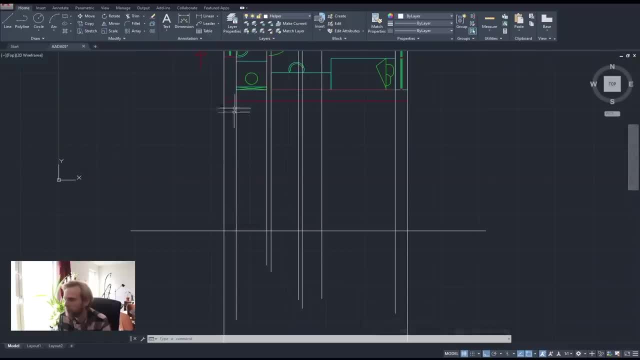 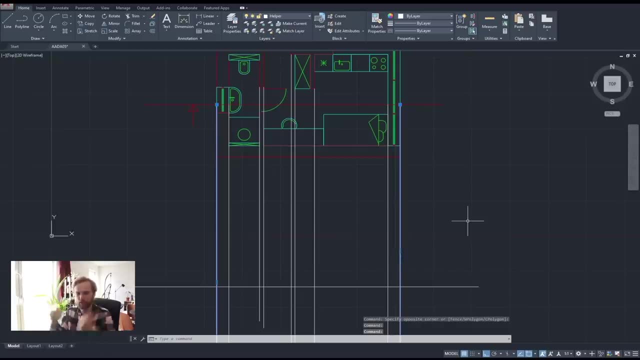 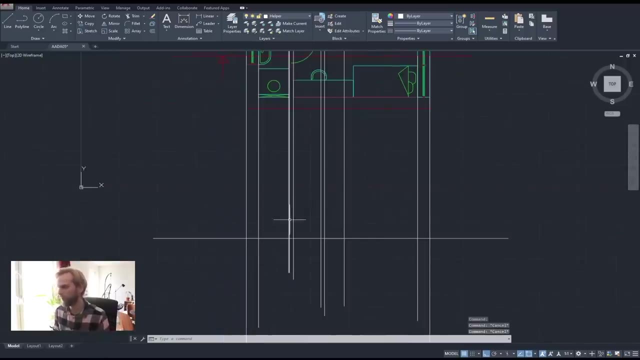 right, This is my ground line And basically my building starts here with this line and ends here with this line, right, And I'm taking that projection and looking at it, All right. So I have that going on and now, now I can actually start drawing, right. So 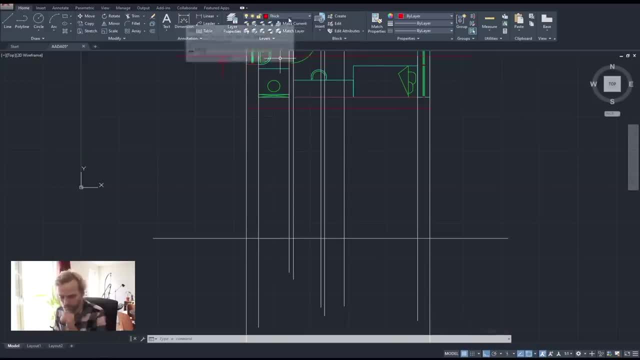 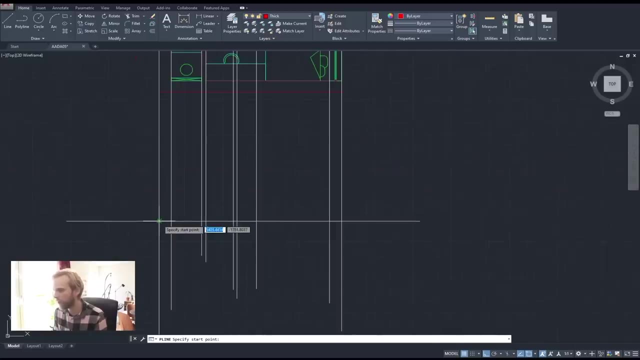 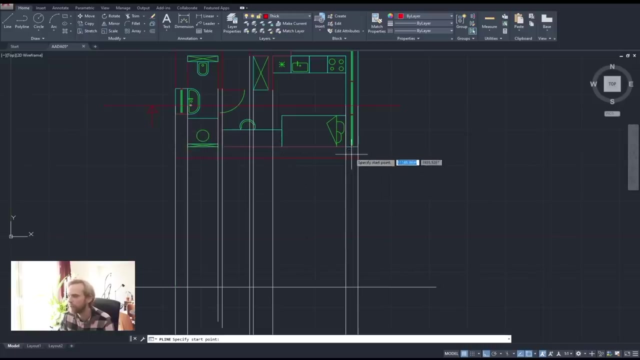 let me go and create a thick. Okay, Create a thick line here and create a polo line. Sorry, change this to thick layer and create a polo line And I'll just draw out in between the the walls. So this wall right here and this wall right here in between them, I'll. 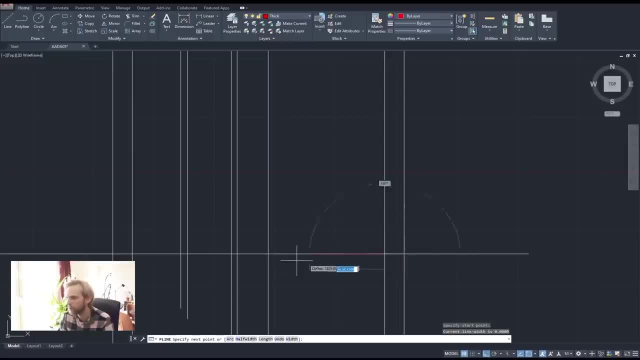 draw out the floor slab. So I know that the floor slab will start from here, will end here. Its height is going to be something around, I would say, 400 millimeters, something like that. 400 initials up here, Bam. 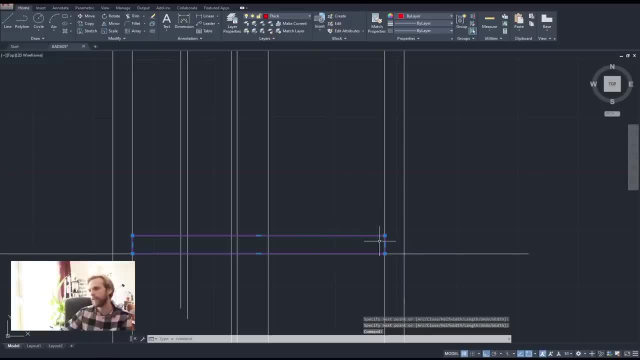 That's done. That's my floor slab And I accidentally drew it above the ground line right. So this is like our ground ground cut Okay, Where we start cutting through the earth. So this is air. This is this is air. 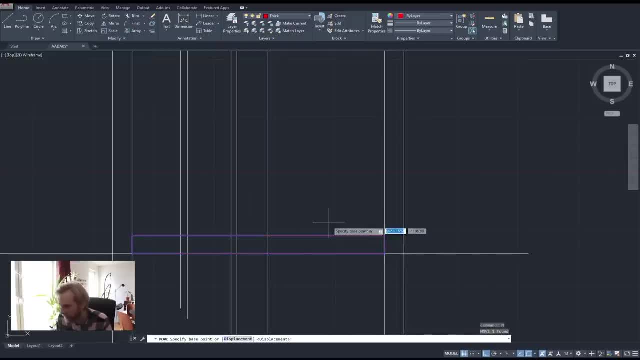 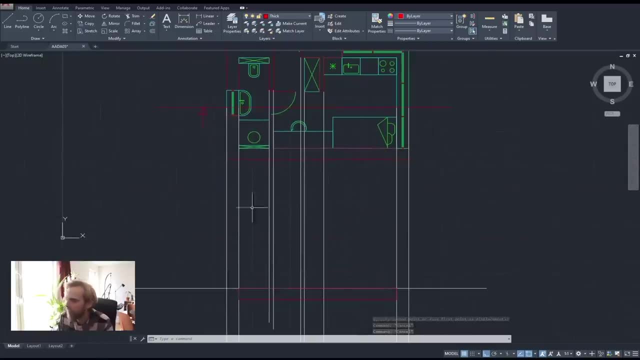 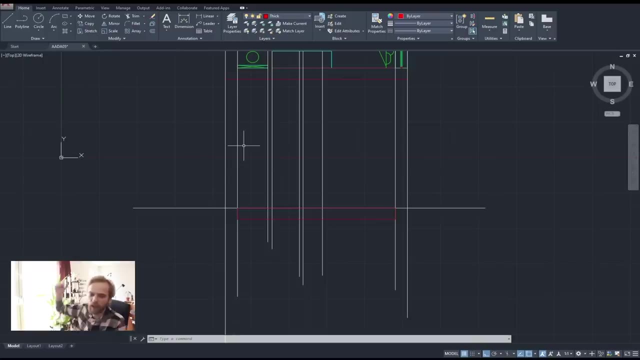 This is earth, right, So I'm going to just take this and move it into the ground like that. Okay, So that is done. Now my walls, right. I'll just kind of create the, the, the walls. So the question is: how high is the ceiling going to be and what kind of roof are we going? 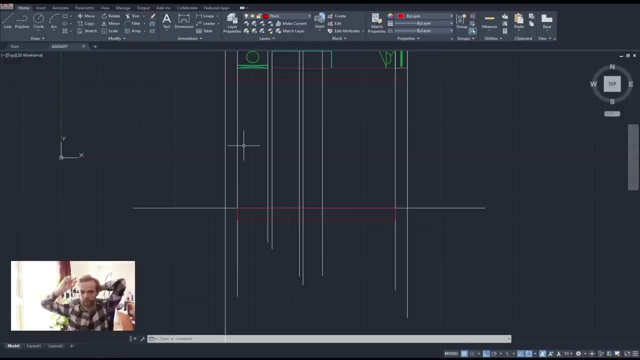 to have. Okay, That's, that's the main question, And I haven't sketched this out, So I have no idea. My thoughts are: let's have an awkward pitched roof. Why? why the heck? not Right? Let's, let's have an awkward, awkward pitched roof. 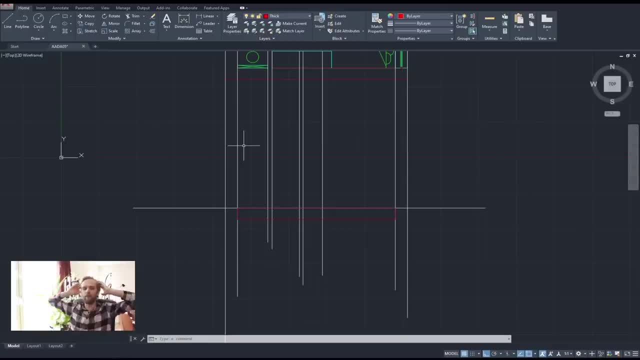 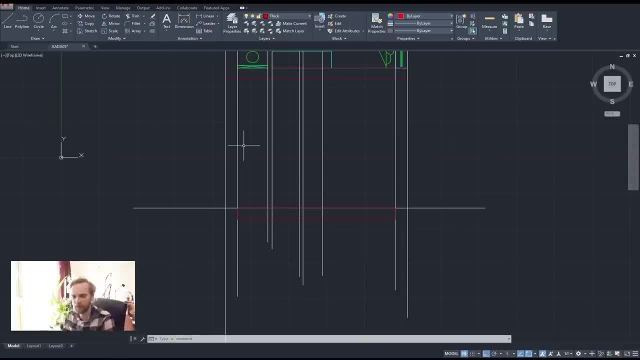 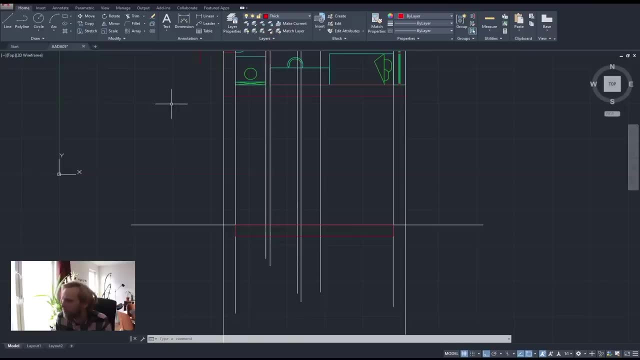 Um Or No, I will not be making a pitched roof. Instead, I'll I'll make like a, like a separated, some sort of a separated roof here, Why not? So I need the height of the ceiling right. 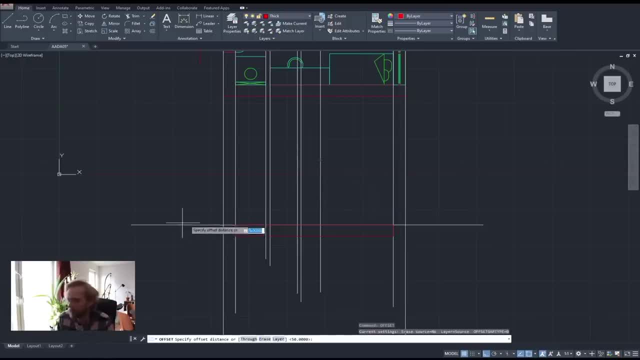 So I will offset. I will offset this ground line by by how much, by how much, by how much. i can also just copy it up as well. um, let's say the ceiling height, uh, in my shower is just going to be 2600 millimeters, 2.6 meters, which is probably going to be pretty high. yeah, that's. 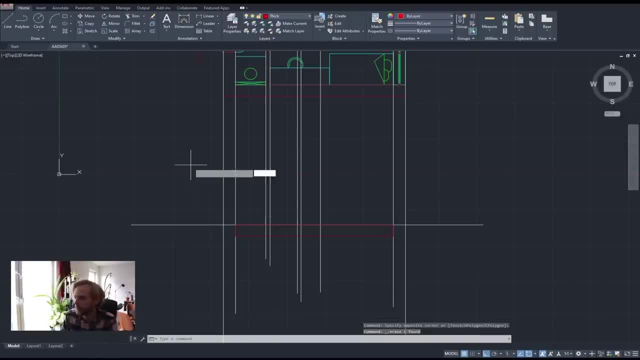 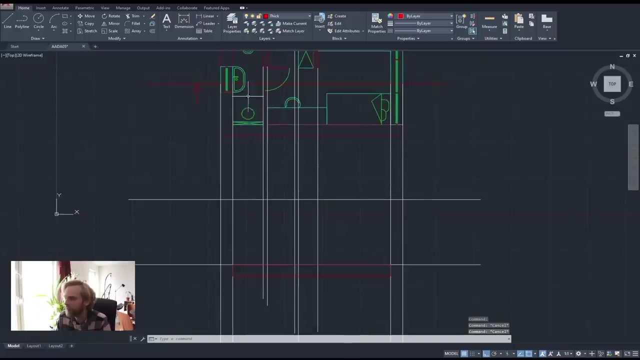 pretty high. let's do less. offset 2400 millimeters. also pretty high. go again. offset 2300 millimeters. i don't want to go lower than that, so okay, so that's my ceiling height in this area, and for this area i will want a higher ceiling. 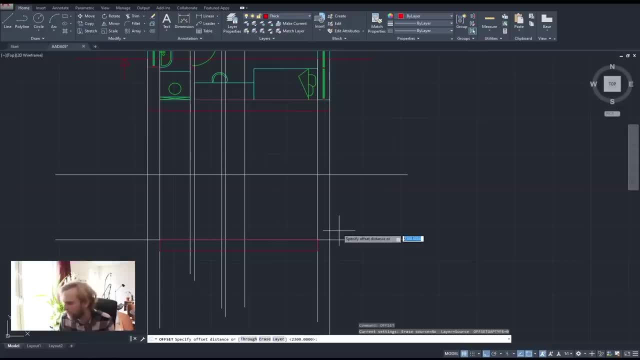 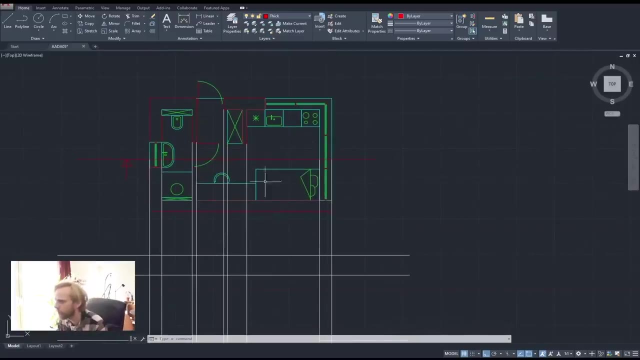 height. so let's say, offset 3000. yeah, just let's just do three meters, 3000 millimeters, something like that. so that's going to be the ceiling height in this area, right here. um, i think that's gonna work. i think that's that should work, right? yeah, that should work. 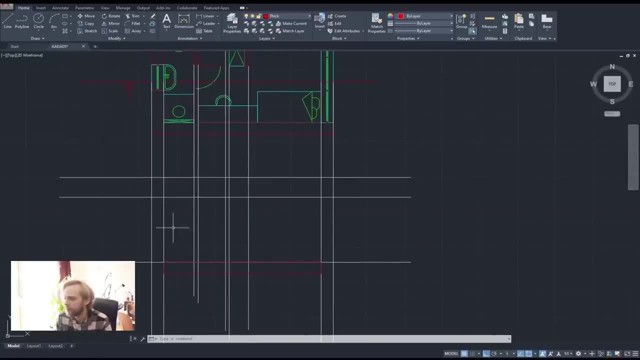 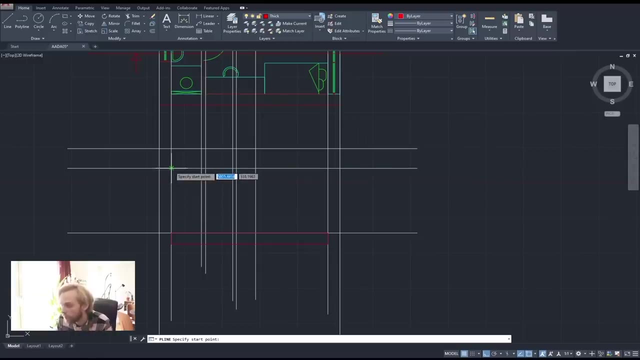 yeah, it's gonna work okay. so now, um, i have my floor slab, i need to create walls, right, so i'll just grab a polo line tool and i will just start drawing in the walls. so my wall here is going to look like that: enter right. and my wall here is going to be larger. it's going to look like that: 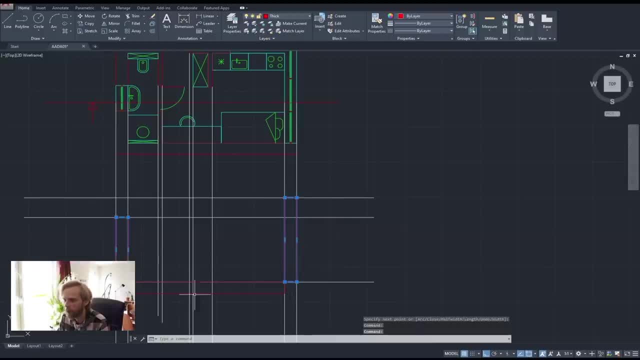 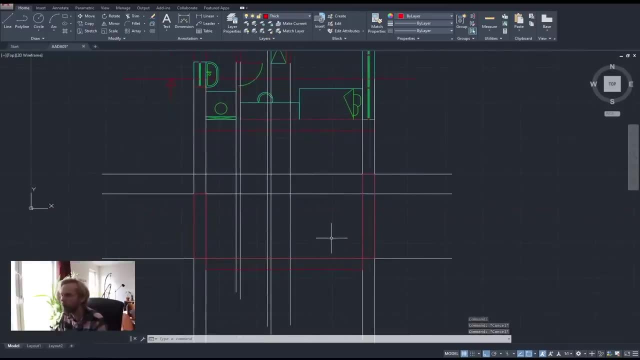 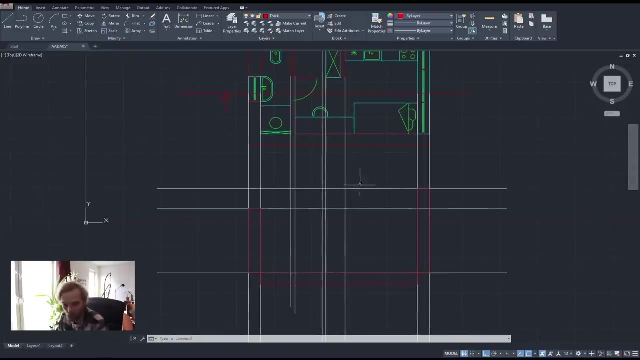 and i will just start drawing in the walls. so my wall here is going to look like that: enter, okay. so i have one wall here, one wall here and the ground slab here, or or the floor slab here, okay, so we have that done. now for the actual roof slabs. i will create more offsets here. bear with me. 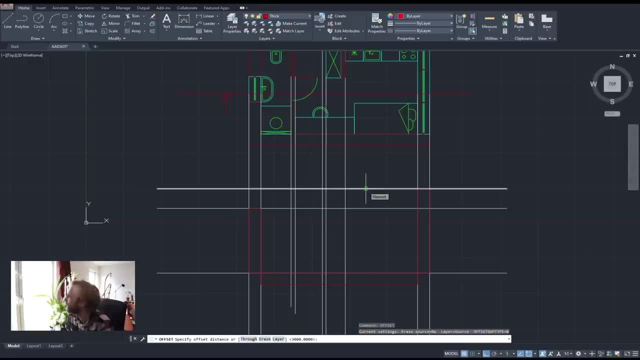 offset and the roof is usually thicker than the walls. these days, the roof is around 700 millimeters thick in, you know, in buildings, uh. but for this particular summer house, i think we can get away with, uh, 500, 400 millimeters. i'll just do 400. well, 450, let's. let's have the middle ground here, so i will. 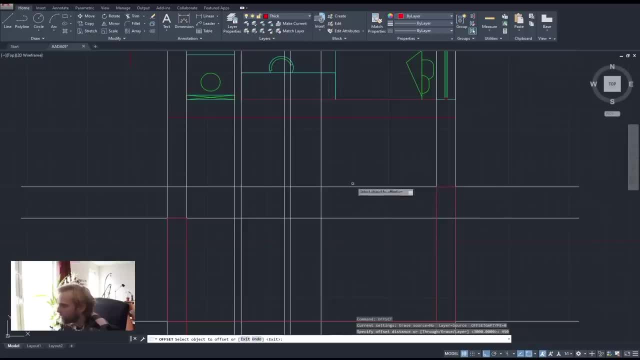 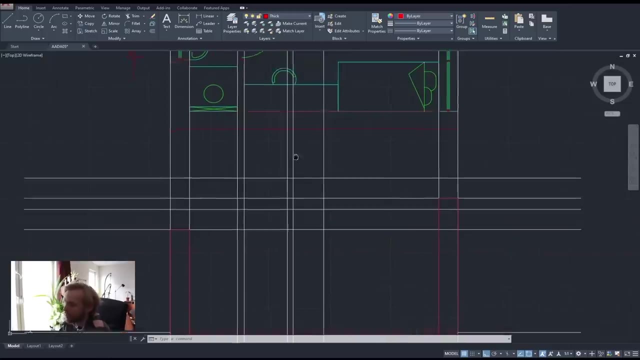 offset it by 450 and i'll offset the ceiling, the the high ceiling up by 450 and the smaller ceiling up by 450, like that. yeah, a lot of lines to to look at now, right, and you will get used to it eventually. um, now actually. 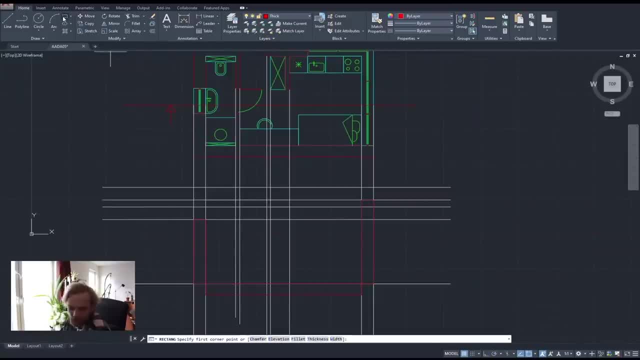 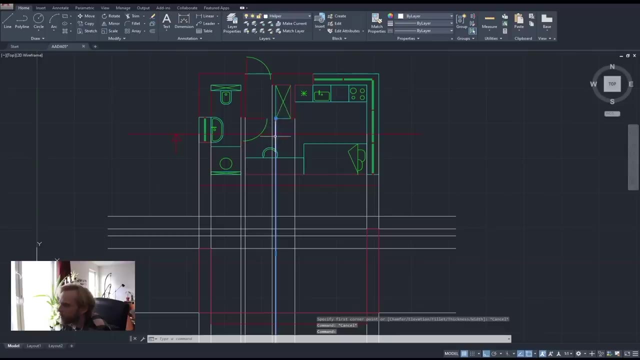 what i can just do is i can take a rectangle tool and just draw out the roof slab. let's see how far will the lower roof slab reach, probably until here, right, and then we will have the the large roof slab going on here. yeah, i think that's that's going to. 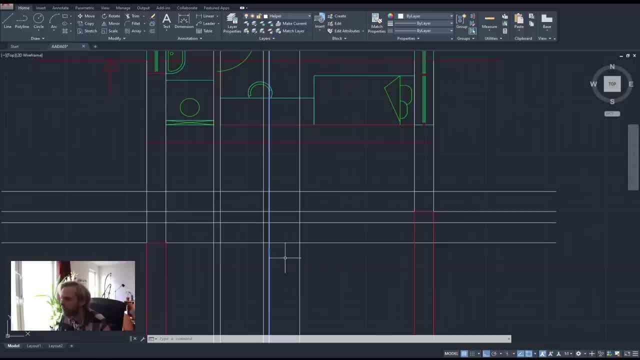 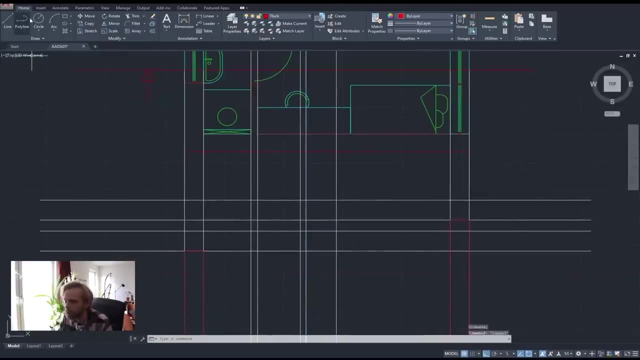 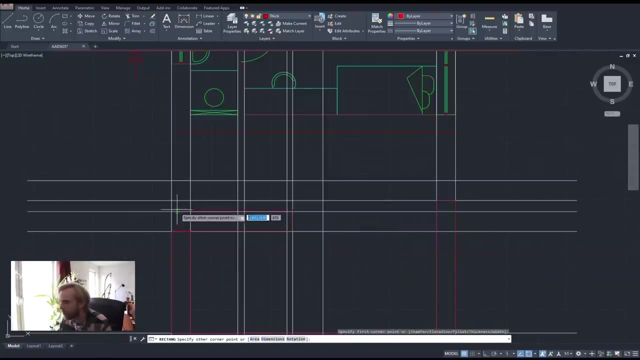 be, that's going to be the trick. so i have this line marked out and this is going to be how far the bottom roof slab reaches. so i'm just going to draw out- now i, for it's this line here. so i'm just going to draw out the bottom of the bottom roof slab. 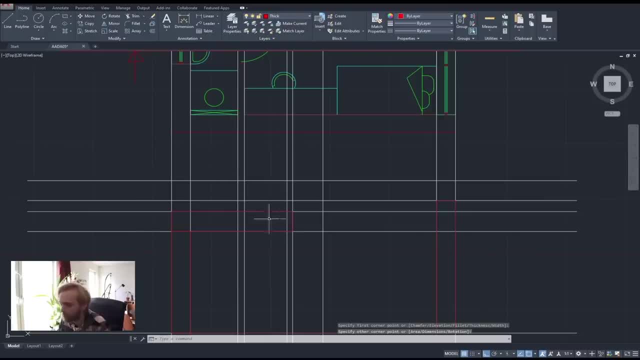 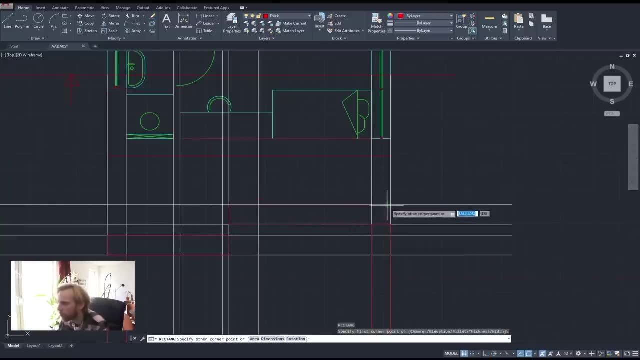 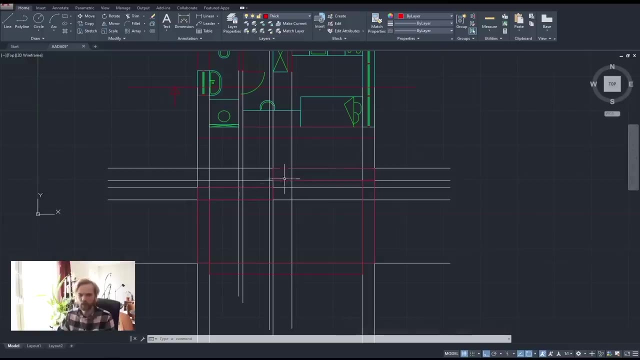 outer rectangle, like. so that's my bottom roof slab, and then for the top roof slab, of course it continues on from where the bottom roof slab ended, you know, until here. there we go, so we have roof roof, wall, wall floor. let me delete all of the horizontal lines. we don't need them anymore. we will be working with. 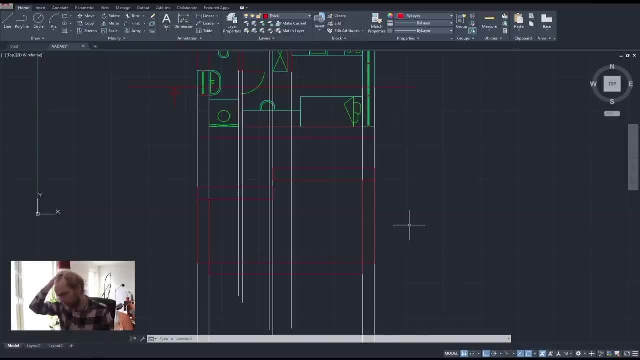 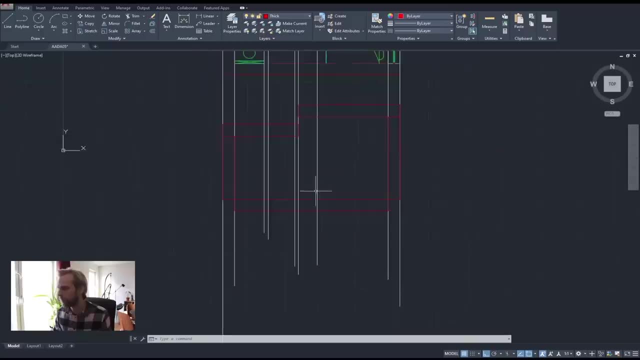 vertical lines, but we don't need the horizontal ones anymore. um, right, so we have that going on. uh, now let's create some foundation, foundation blocks, because this is a little bit, a little bit obnoxious, right, the way this, this connection, looks like, that's not a strong connection. um. 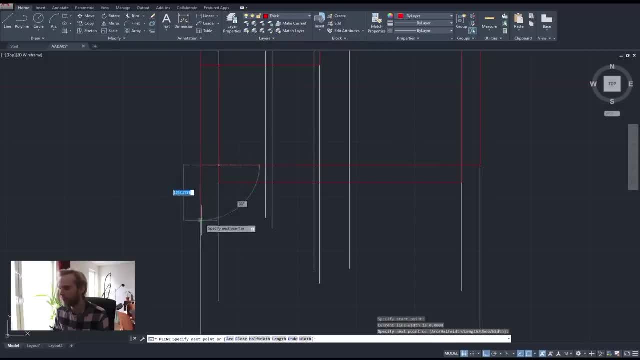 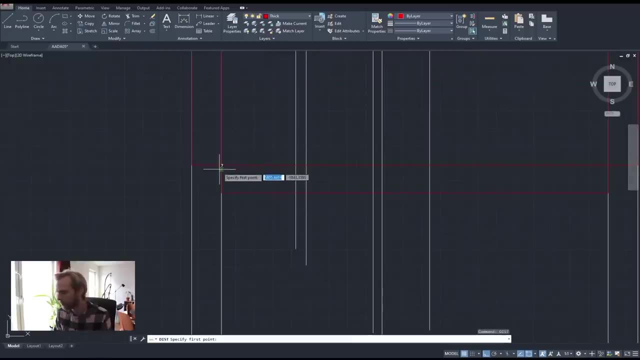 so i'll create a polo line, i'll just create a block. that- how wait? how deep is? how deep is the floor? so the floor is 400 millimeters deep, so i'll create a foundation block that is plus, let's say, plus 600 millimeters. so the foundation block is going to be one meter deep from the from the wall. 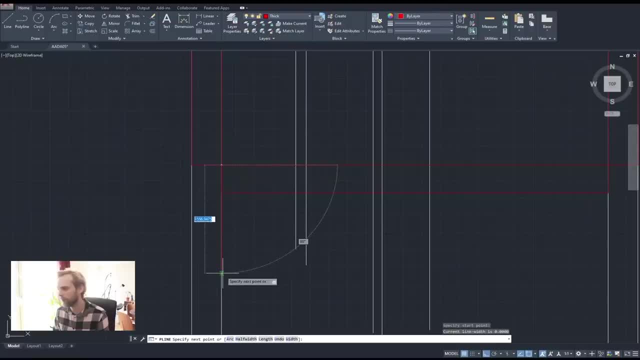 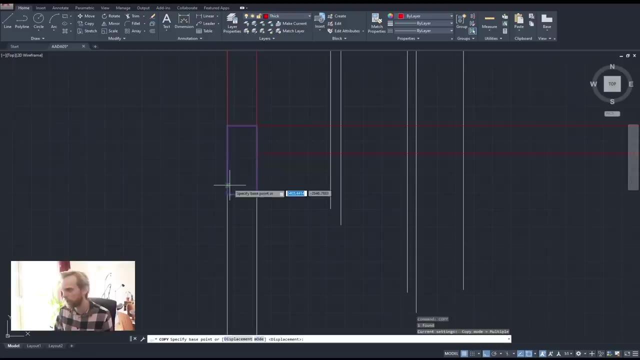 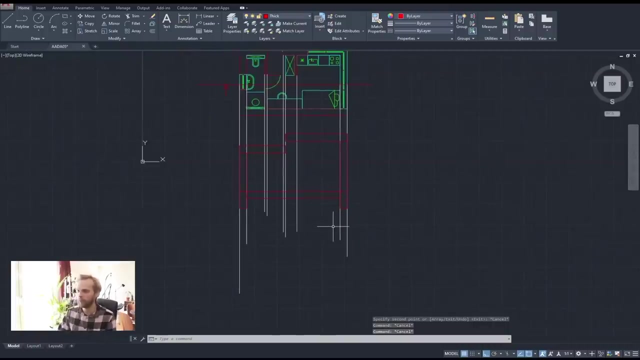 right, uh, so polo line going down 1000 millimeters, finishing up here, connecting as as a rectangle anything here. well, actually, let's just copy it. why not copy from here here? so that's the foundation that's going into the, into the ground. okay, uh, that is done now. 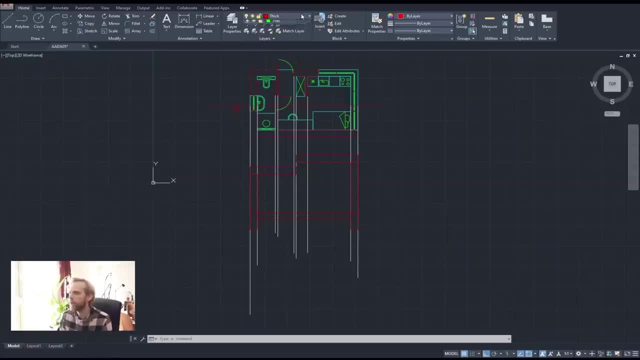 but one step. right now we need to create a new function for the construction. so this div unit, we're going to give it some space. they areErney, they are going to be bigger andburger, medium, jira and damn perfect, and we are not going to have this right at first. and now let's hand in a common jawr. 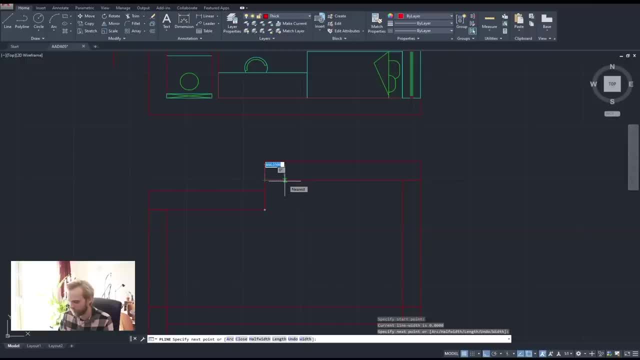 right here a little bit безза combinations, before i open the definition of that lower layer i to here and it's going to be: let's do honestly, i would want to do 400 millimeters, but in this case let's do 250, 250, and how long is it? 700 millimeters down and just close it off like that. 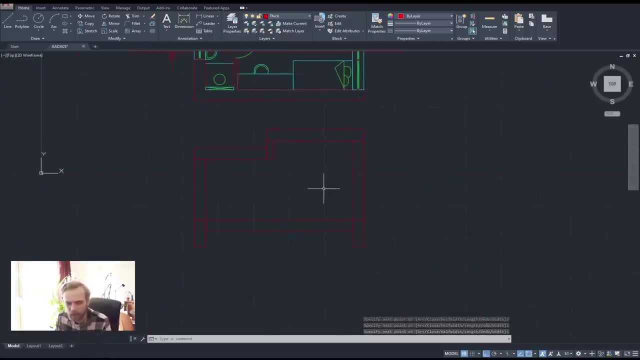 okay, so now we have our, our shape and, honestly, honestly, the way i would do this, i could start trimming and joining, but this is going to be so much faster if i just, uh, change this to medium layer, turn on thick layer, or change this to medium layer, escape out and draw, redraw everything in. 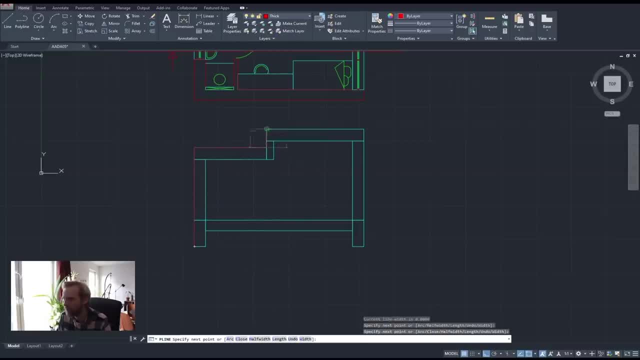 thick layer as a single or as two polo lines, like that. so just going around the perimeter? yep, messed it up there, we go so. and then going around the inner perimeter, like that, then i just hide the thick layer, uh, turn the current layer off, whatever, delete the medium layer and turn the thick layer again. and i messed it up. 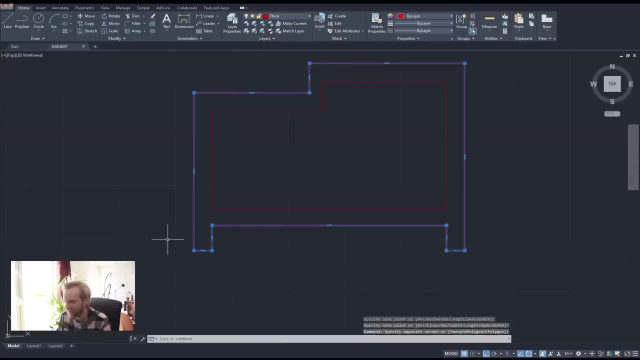 so there needs to be a line here and it needs to be joined up. there we go. you should see something like this, right? so that is the way i would do it, and then i would go around the inner perimeter of this, uh, the section of your, or rather the exterior envelope of you, of this particular 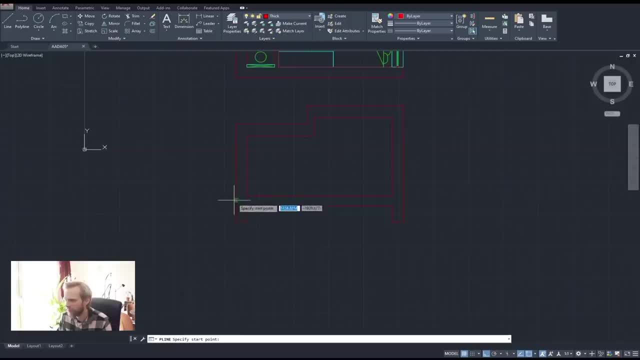 building right that i want. i also will add, just so that i don't forget, i will add ground here and here. that's the ground cut line, and i will actually take this, uh, this ground cut line, and i will move it down by five, uh, or 50 millimeters. 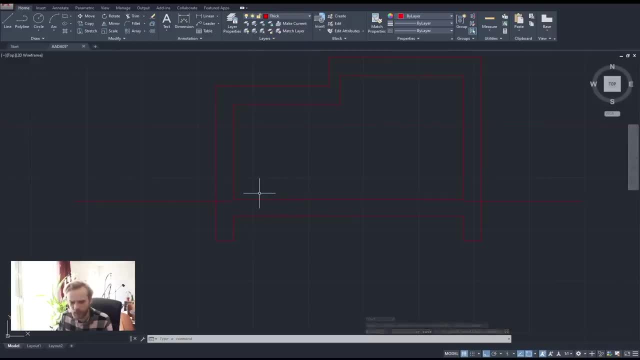 just so that the the floor slab is five centimeters higher than the ground. um, the reason for that is: when it's raining, you don't want the rain to visit your house, right? so that's the reason. that's the reason also. it's it's it's good for, for kind of brushing, uh, the dirt out of. 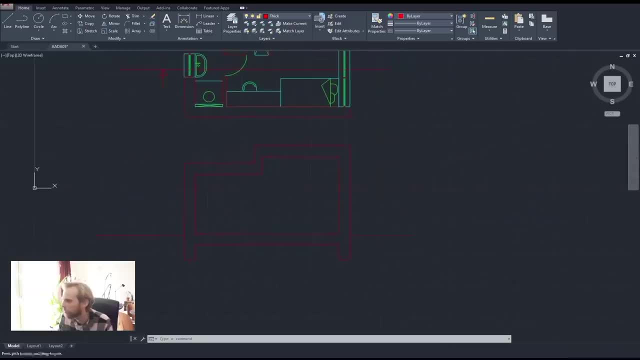 the building as well, uh, as as you leave the the building, okay, so i'm not gonna show you. so that's ground. that's, that's our little building here. let's continue on. so now I want to add partitioning walls, because I can see that there is going to be a partitioning wall here. 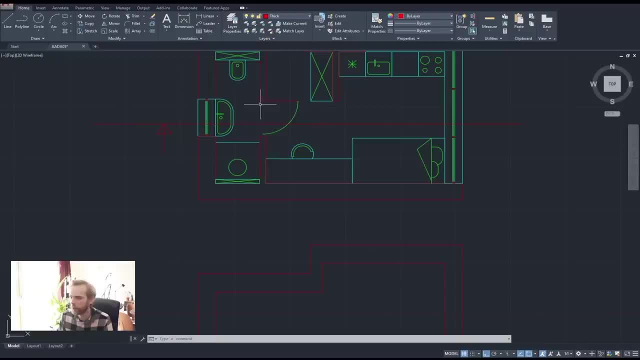 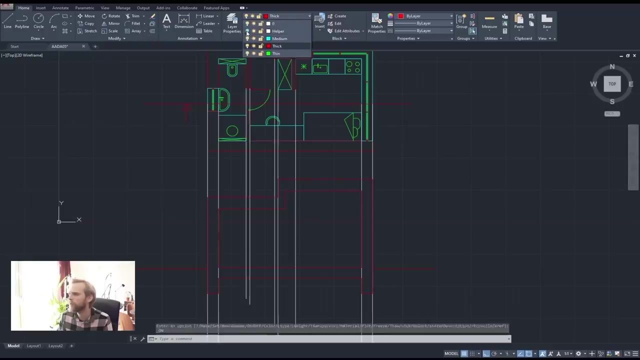 where we will also show that we are cutting through the, the doorway, and also there is going to be like a retaining or partitioning wall that we will just see in the back right. so we need that as well. let's do that. let us let us do that. so I will go into my helper. I will enable my help helper. 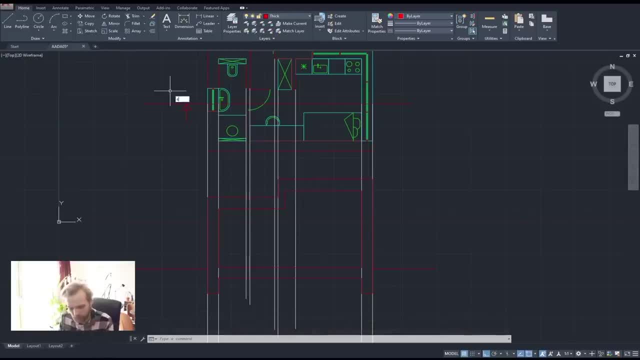 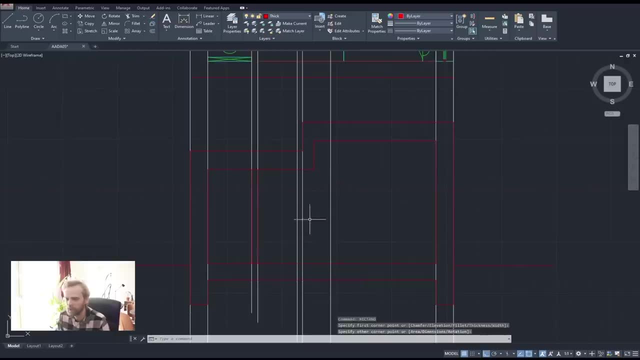 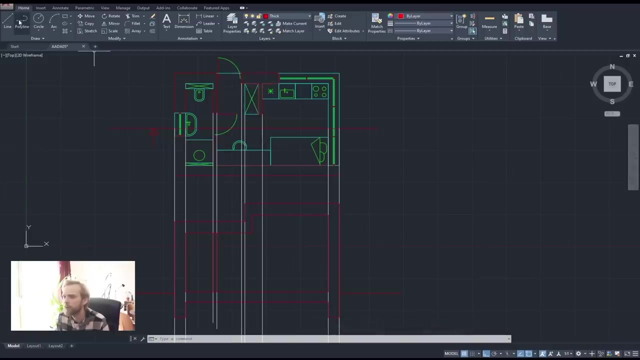 layer and I'll start drawing some rectangles, rectangle, rectangle, so partitioning wall right here. that just a rectangle. then there is no partitioning wall here, but there is going to be a partitioning wall here, but I accidentally forgot to add. do we need to add? or maybe we can use this? 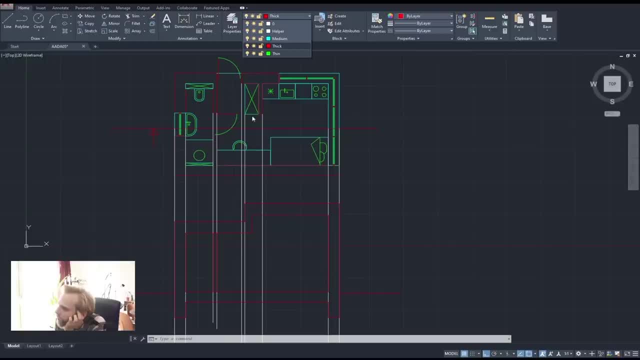 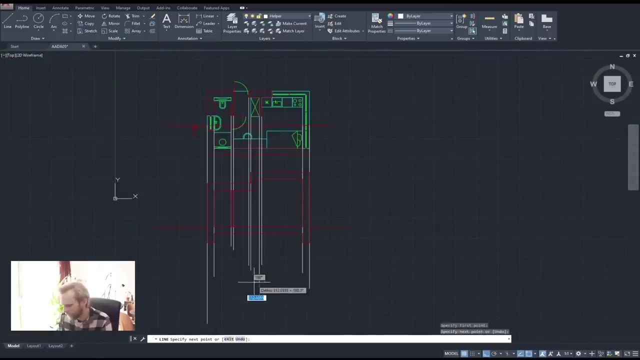 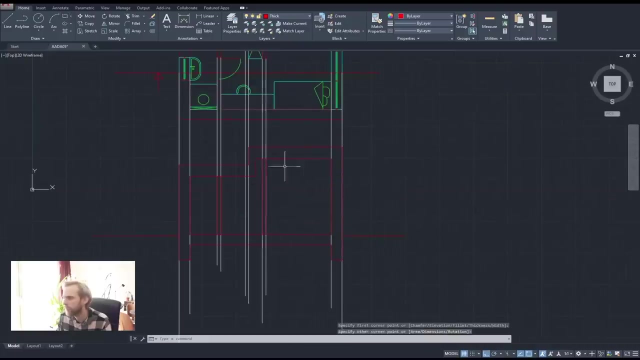 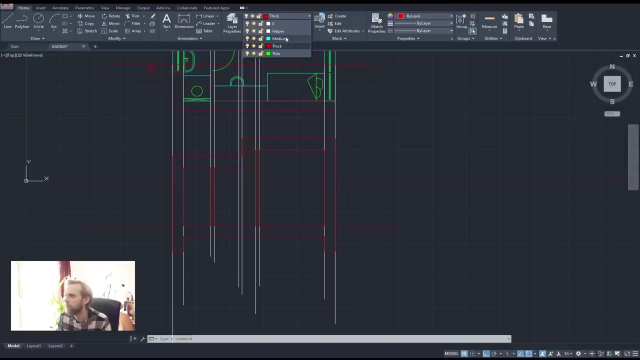 it can be kind of joined up with the shelf in a way. yeah, let's, let's do it, let's do it this way. I'll just create a one more helper line from this point here downwards. we'll create a thick line rectangle, just something like so, like that, and I will create a very weird the medium line, or either this: 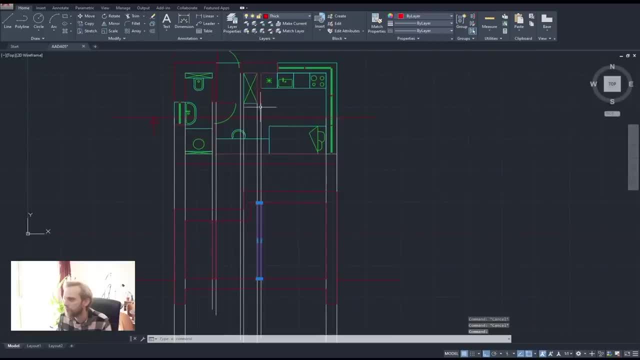 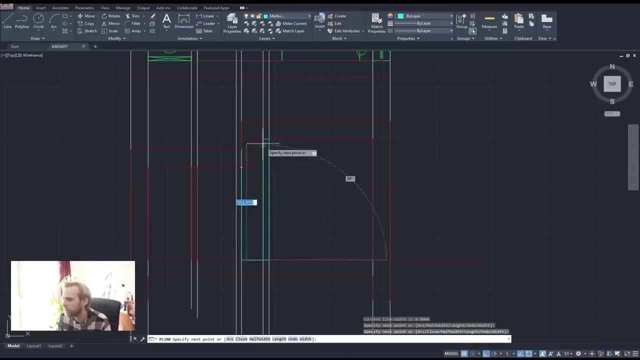 sorry, sorry, sorry, sorry. this needs to be a medium line because we are not cutting through it. of course we are not cutting, cutting through it. so it is indeed中 line thickness, and i will create one more medium line that shows the shelf at the at the side. so it's gonna. 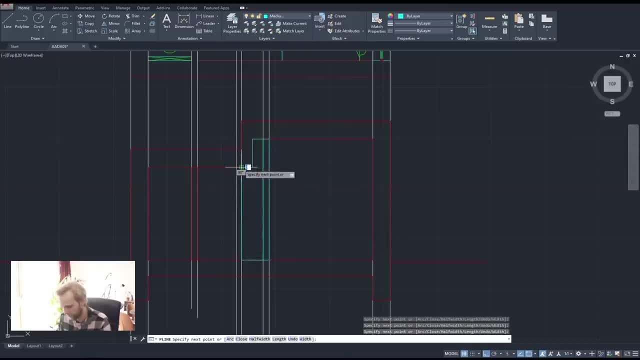 look like it's gonna look weird, but that is fine, that is okay. usually, uh, you don't have these kind of weird gaps here, but actually we can kind of, since we are, since we are here, can i just kind of fix it? yeah, let's fix it, uh, so i'll delete the two helper lines, that or four helper. 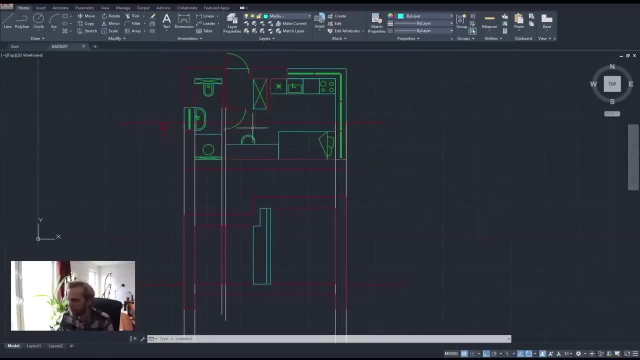 helper lines that i don't need anymore. i will kind of add them later on. i don't need these anymore as well. actually, i don't need any of these anymore. great, we can delete all of them, and i want to fix this area right here. this is an awkward. 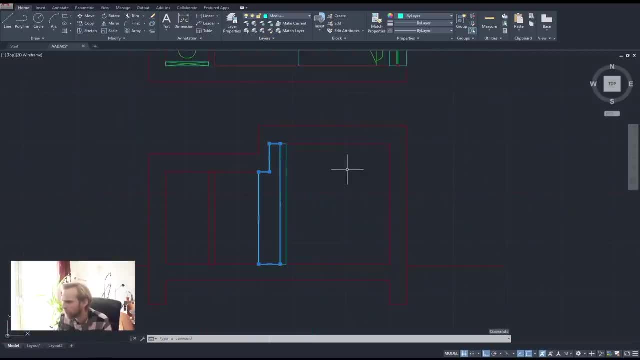 area. so what i'm going to do is i will go in here here- oh, oh, i know, i know, uh, so let me just create a line segment here, just so that i don't forget where it ends- and all i will do is just take these points and move them to. 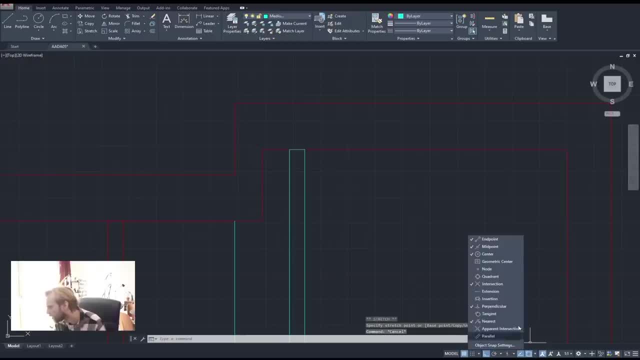 perpendicular snap. what the hell perpendicular snapping is turned on? why is this not working fine? fine, we will do it the other way around. i will trim, enter, enter, delete that segment here. i will extend this line to here or enter, extend to here. enter this line like that, and then i will create a thick line segment right here. 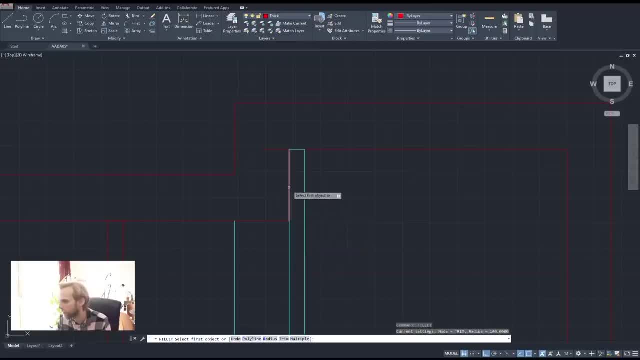 that and i will fill it. there we go: uh, fillet with radius of zero, so fillet radius zero from here to here. so that is done and now it just needs to be joined up properly. join should be good. it's going to be closed, is it's good? yes, it's good, so. 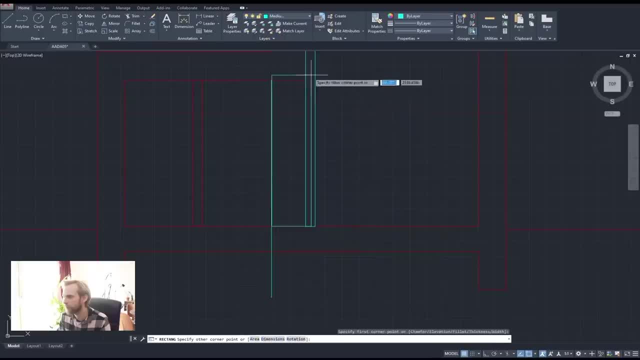 ah, right, and now just a rectangle for the shelf, like that. okay, so now it's done. sorry, i just wanted to clean it up a little bit, just to make it a bit a bit nicer. okay, so we have that done. uh, now for the let's add. 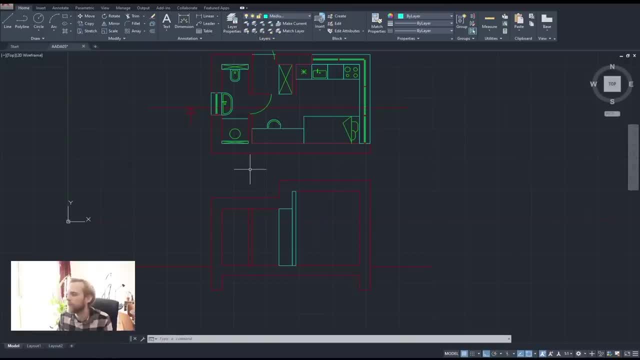 walls, right. so let's start with a window opening here on the left hand side, right. so my windowsill is going to be probably somewhere around. i'll just start drawing here from from the bottom up. it's going to be offset and i'm going to offset it: 1.1 meters, one, one, zero, zero. 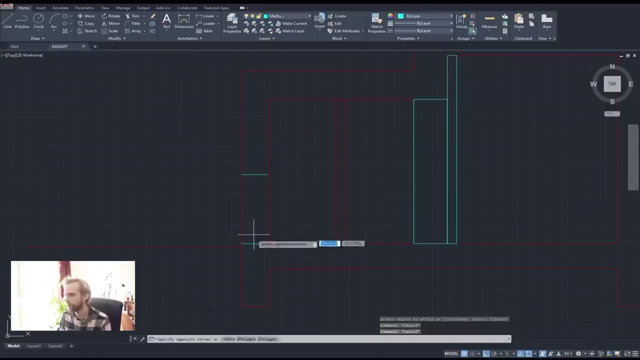 so something like that. and the height of the window is probably going to be until the, until the roof right. so i'm just going to not even measure, but just draw it like that. that's it right. uh, i will change this to the thick layer. select it. 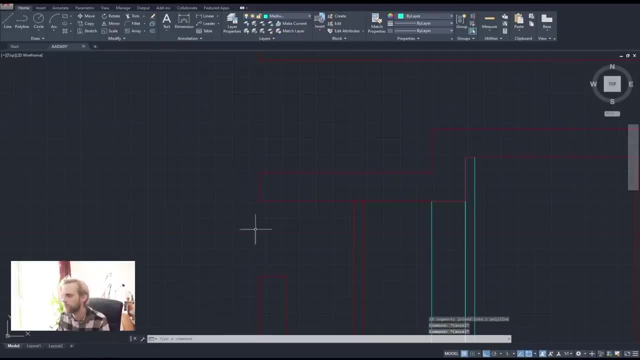 get rid of that, join everything up. that's done, right, so the, the, the window opening is done, and then it's absolutely the same procedure as what we've done in the plan. so i will not be kind of talking about it, i'll just really quickly be, uh, recreating it. i'll actually even make a shortcut. i'll just borrow the existing window here. 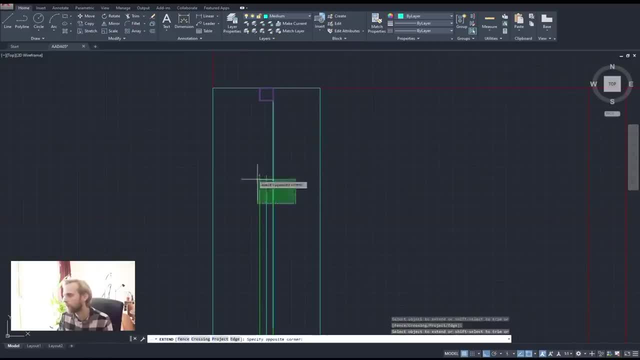 like that, there we go. so we have a window here, um doorway, uh, doorway is very simple. all we need to do is just, well, we need to know how high the doorway is, and it it is, uh, two meter, 2.1 meters high. oh, that's, that's almost nothing. that's almost nothing, okay, and i will just trim, uh, trim, enter. 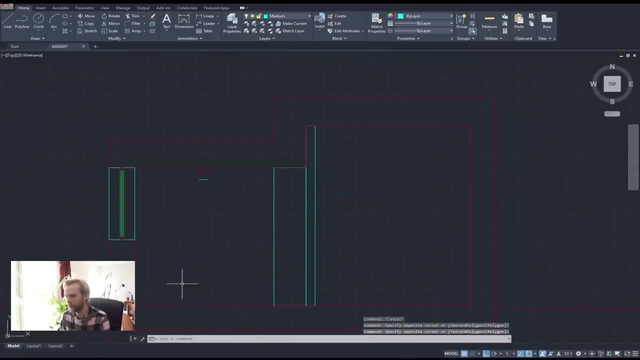 trim away everything except for, except for the top. you know there's this little area right here and actually i wanna join it in with the, with the roof, so i will trim, enter like that, join everything up. uh, it gets joined up into the incorrect layer, so i'll just switch the layers around like that. 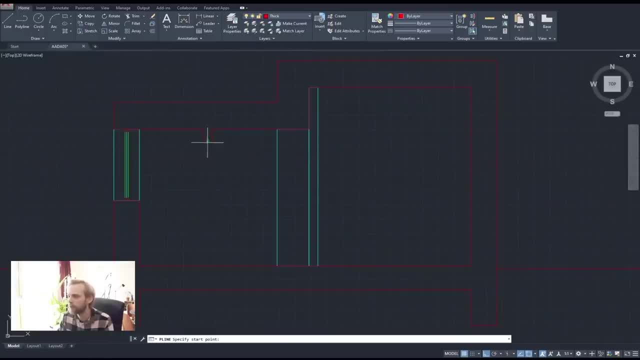 um, now let's go for the thick line, because we are going to be cutting through the doors and just add a door segment here. um, honestly, i let's make it a little bit nicer. i'll just borrow the the frame. we will just use the same frame for the door copy from here to here, like that. that's, that's the frame. 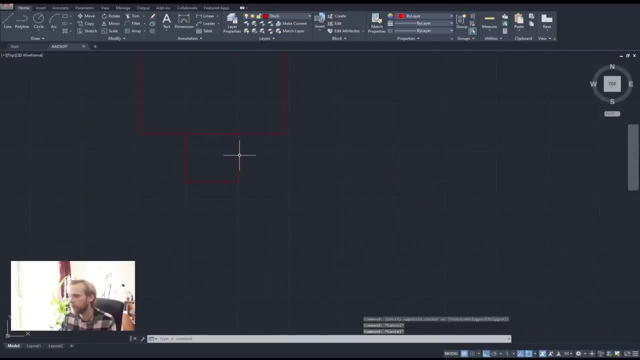 for the door and maybe we can make it a little bit nicer as well. yeah, let's just make it nice, um? so that frame is going to be all the way through and it's going to be five centimeters thick and 40 centimeters wide. it's a wide frame, right, um? and it's going to have a door going through from the middle of it, like 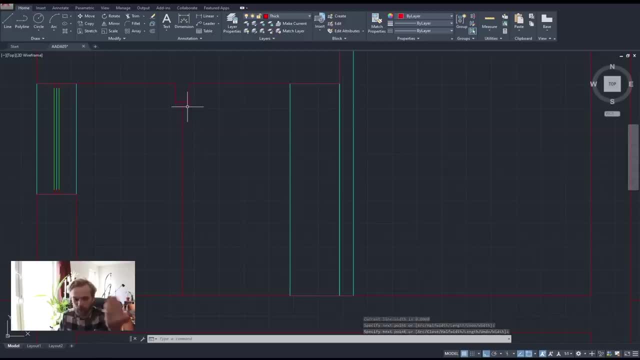 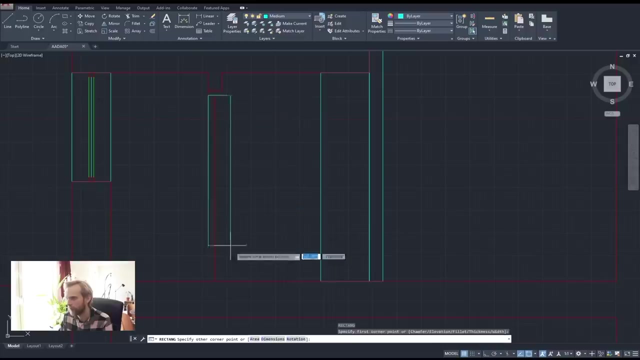 like that. so we are cutting through the door and we also see the back of the frame, as per usual. right, so we see this wall right here in our projection. so that is going to be a medium line and it's going to be a rectangle like. so i can draw a rectangle properly. let me just draw. 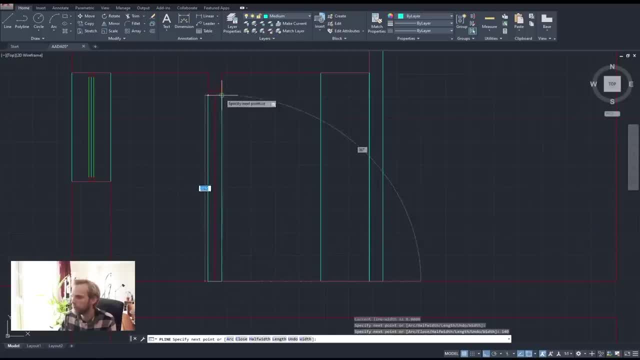 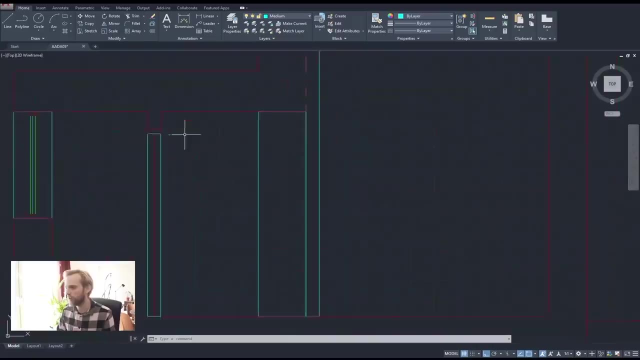 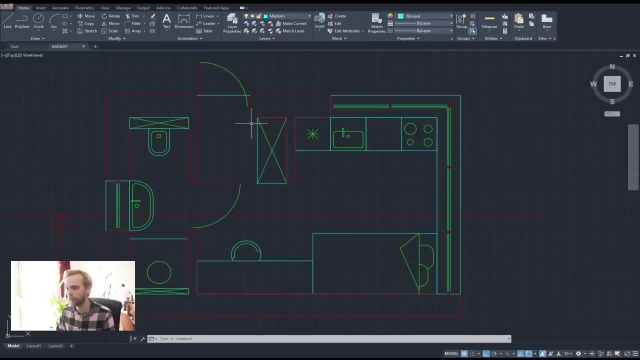 a whole line, then instead 140 millimeters width. there we go. so that's our door, doorway right and that's done. now to show a doorway in the um in the projection i already have the 2.1 meter high height here, so i don't really need to invent anything, and i know that this doorway is 90. 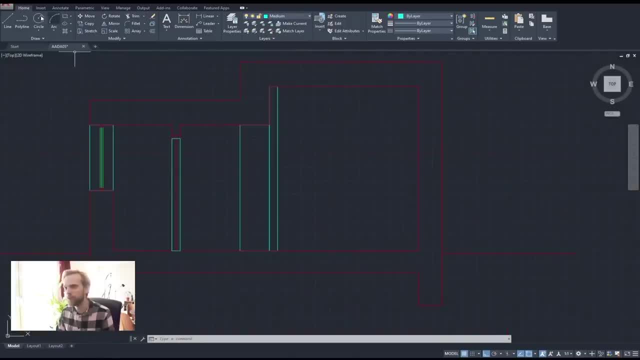 centimeters wide. uh, so i don't really need to and make any calculations. i can just do this: 900 bam, bam, bam, like that, um, and then hmm, then i kind of want to. i don't really need the bottom line, do i? okay, let me explode. 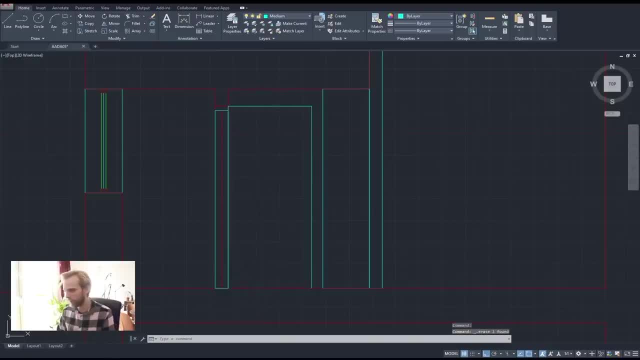 so i explode this pole line. i will delete the bottom line. i will take this, uh, these line segments that are left, again it's upside down. u now i will join them up. perfect, and i will. i will offset all of this by 50 millimeters inwards. so that's our frame for the door and for the handle. i will just where's that water tap? 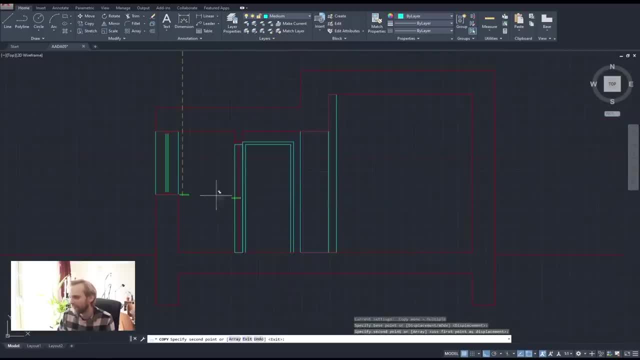 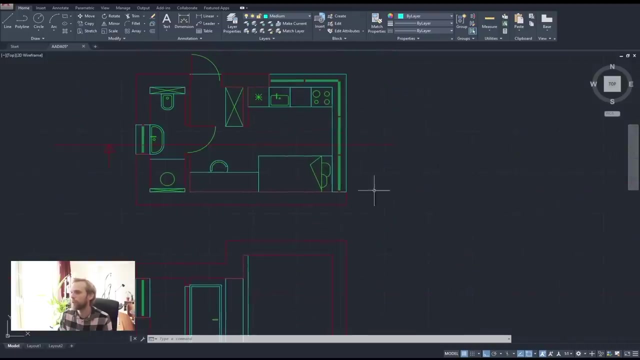 i'll just use the handle here. doesn't need to be precise, just something like that. so that's, that's the handle, um, and that's honestly, that's honestly it in terms of the doorway, that's our shelf, that's good, that's our wall, it's also good. then we have the kitchen, kitchen cabinet, and we have 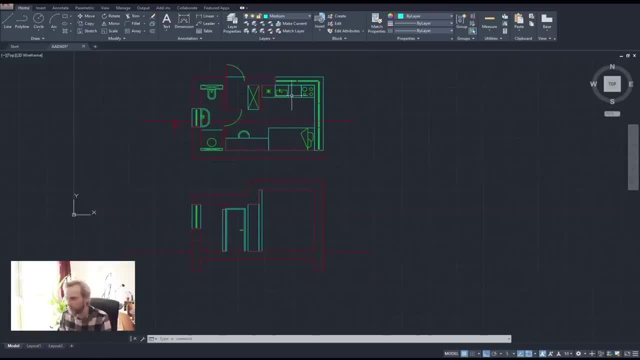 another really large window here. so for this window, i know that here i'll have a kitchen cabinet and the kitchen cabinet is always 1.1 meters high. so this window line that i i drew here kind of continues on right, and the first thing that i'm going to do is i will make 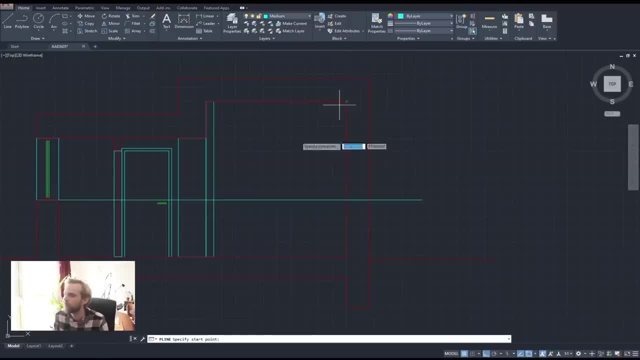 i'll probably make something like this, right, so the window is going to be located here and then i have the possibility to add shelving here in the top, i think, the storage. i think that's that's fine, so i will trim, enter, cut away that part right, because that's where the window is going to be. 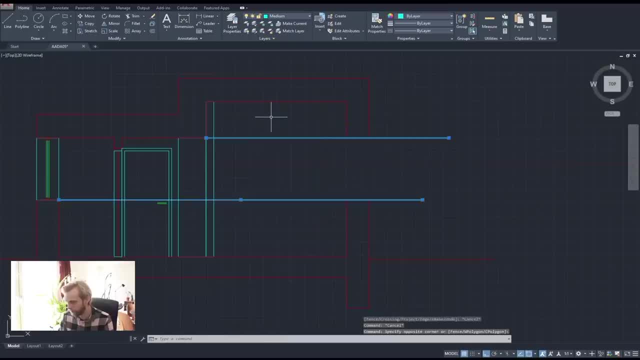 located. now it's actually going to be here and i'm going to keep it like this: delete, um, and i will draw two line segments here, as per usual. join everything up, uh, change the layer. change the layer of this one as well. there we go, and honestly i think i can just kind of cheat. 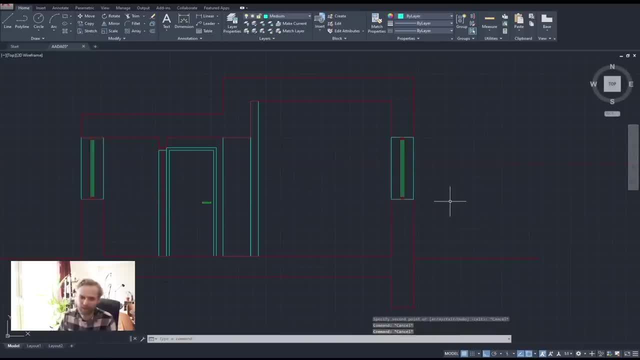 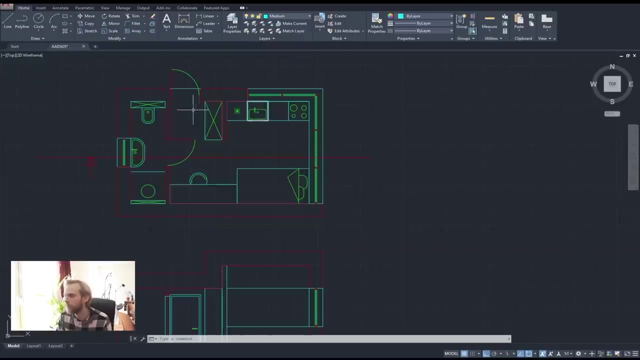 and do this. yes, i can, okay, so i'll just, uh, take that window and place it in there as well. um, so we have that, but also i have the window going until until here, right, because i see, i see this, this, this window area here it's actually not going until the the wall, it's actually stopping. 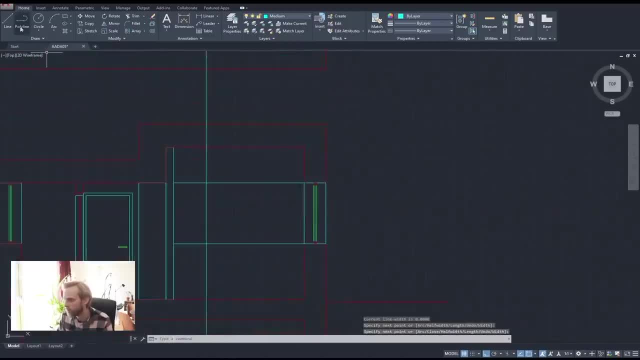 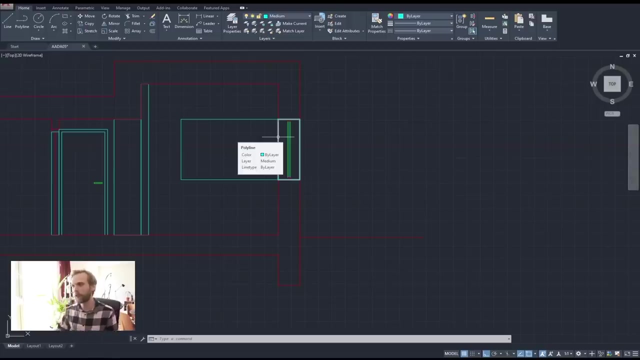 right here, right? uh, so i will have, let me draw this u shape here. i will have a window here like that, which means that now i don't see this line anymore because it's a corner window, right? so i don't don't have, um, don't have neither this nor this line anymore, so i can just delete it. 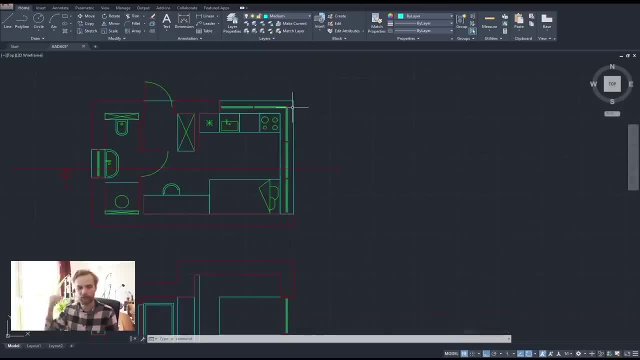 right, because i i, as i'm looking through this, i never see the. you know, here i see the the wall. here i won't see the wall. right, because i'm looking through it, i'm, i have a window that goes through the whole facade. uh, so that's done. now i will offset 50 millimeters. 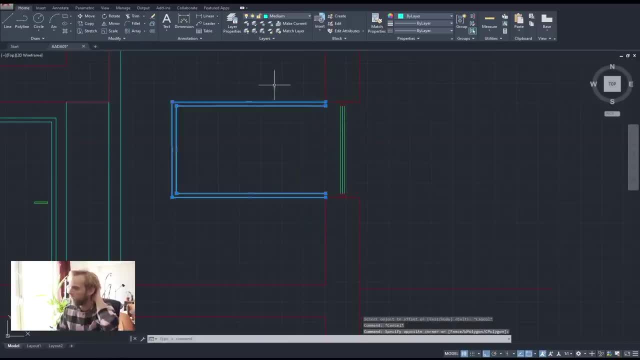 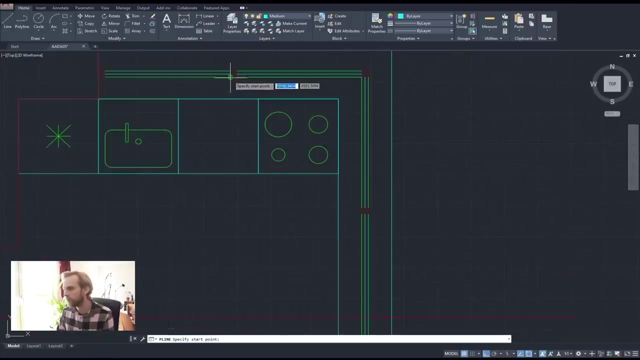 i will offset this by 50 millimeters, like that, and i will actually extend it just by grabbing the control points, or you can use extend tool. that's fine as well. i'll extend it until this window. so this is the frame that we see right. uh, now i can see that there are going to be divisions here. 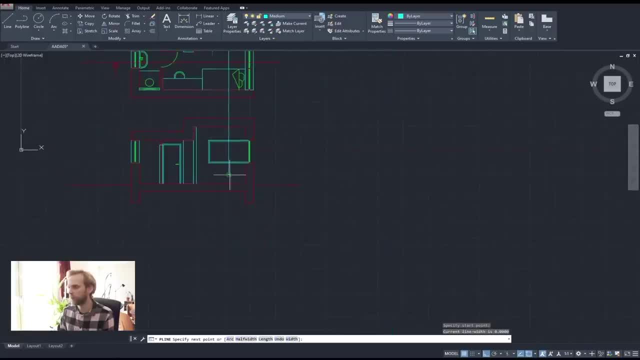 uh, well, at least one division here. so i'm just going to kind of draw out those two lines, because i'm lazy like that and i'll use trim, enter, enter to kind of clean everything up. so come on, there we go and then get rid of the rest. 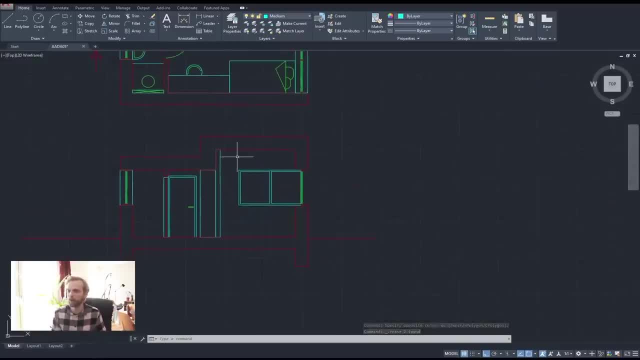 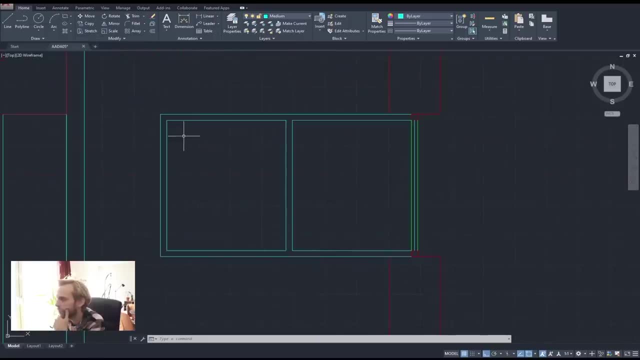 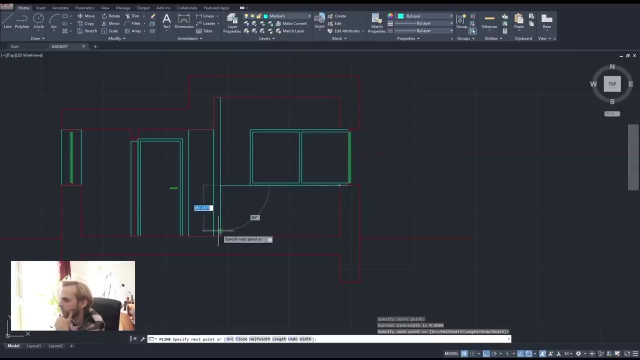 so that's, that's my window. yeah, that, that's, that's all all i need to show. um, now for the kitchen cabinets, uh, and actually maybe i want- no, i'll stick to this. for the kitchen cabinets, it's going to be, ah, just a Paul line and just a rectangle, or maybe we can do. let's do, let's do it. 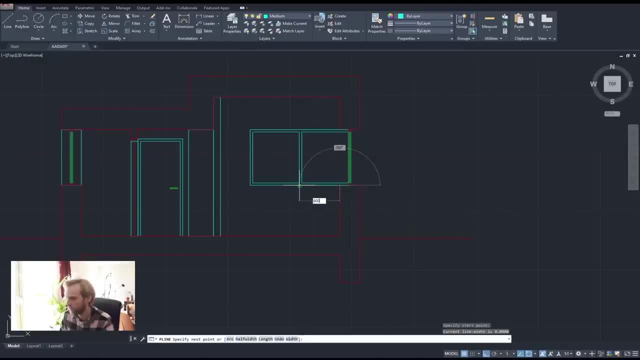 this way, from here to here, 600 millimeters down, here them. so that is like one one block. copy that, ma'am, ma'am, ma'am, that, that that is my kitchen, and my refrigerator is actually going to be larger than that. so I will, I will say: 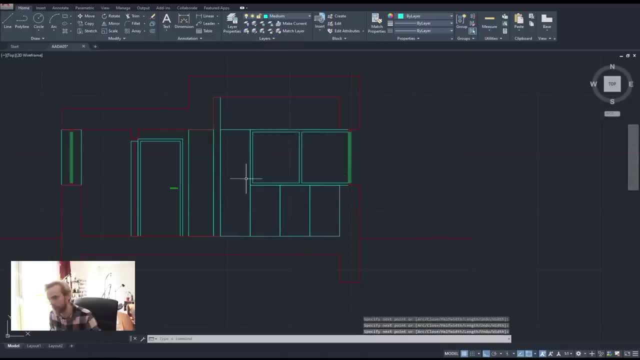 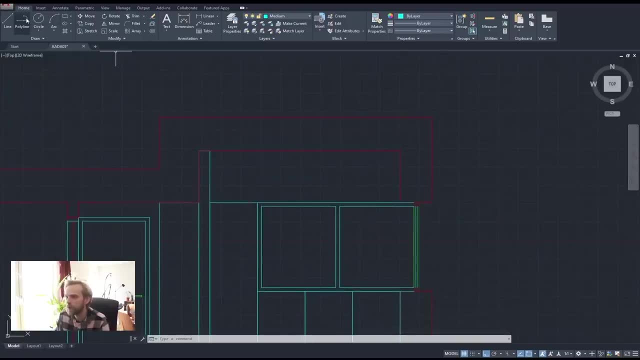 that my refrigerator is a narrow boy that just kind of fits in there like this right now for the top shelving. I actually kind of want to have shelves in the top. so I'm just going to say there's going to be like a single cabinet here and then there is going to 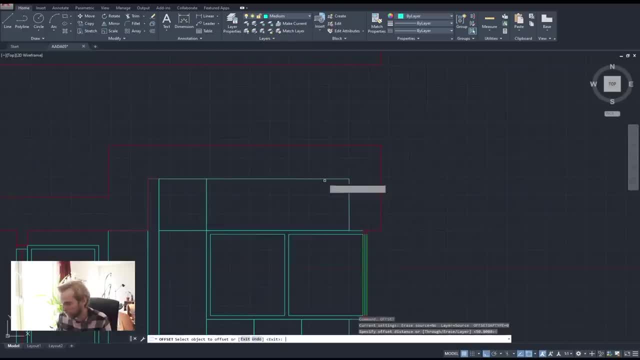 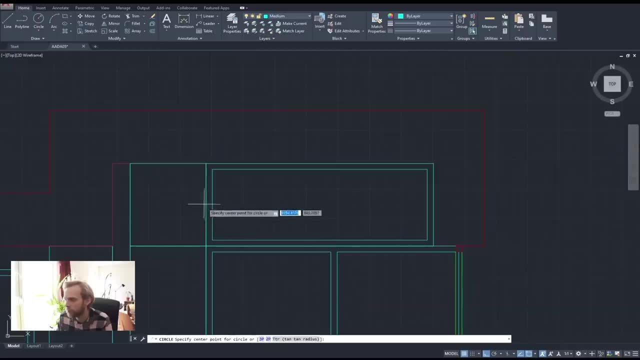 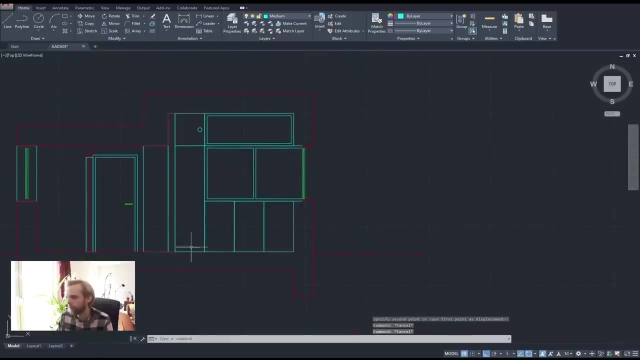 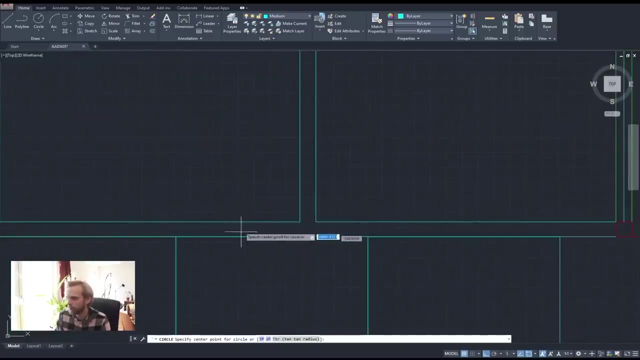 be like open shelving here, so I'll just offset it inwards by 50 millimeters. so that is open shelving, and this is like closed cabinet shelving, to which I can add a handle like that. all right, um, we can do a wire tap as well. uh, wait, where is our water? here we go, this it's. 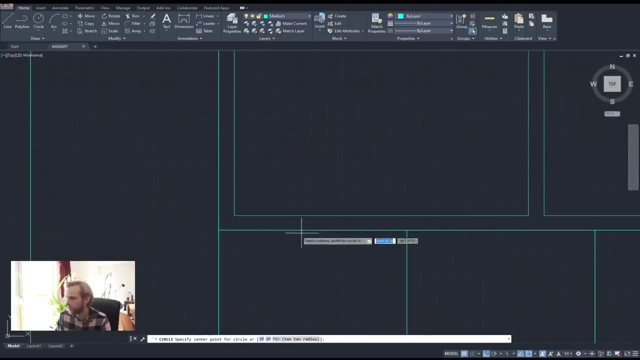 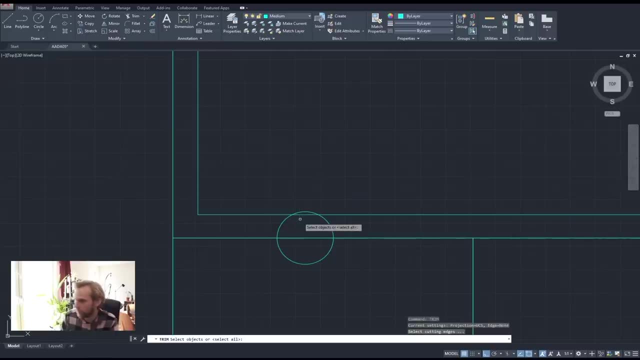 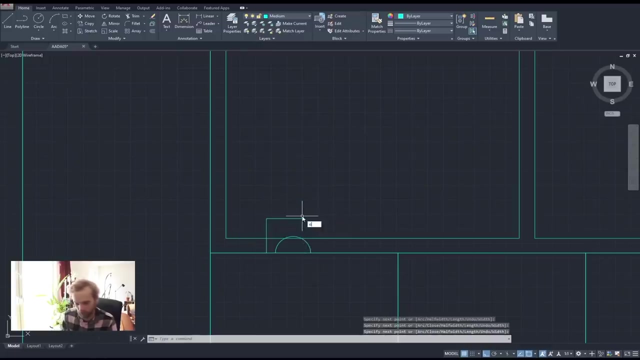 that it's, it's there, right? so I will just kind of create a a, a, a circle. trim bam, enter bam, do something like that. uh, create a polo line that does something like that: offset 20, offset it so that it's like, or rather, let's first fillet, uh, let also 20 millimeters. why does fillet? oh? 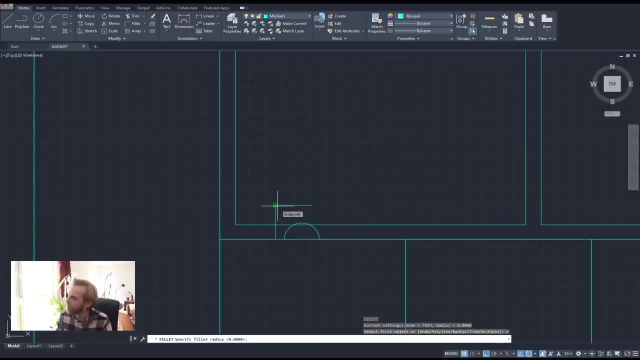 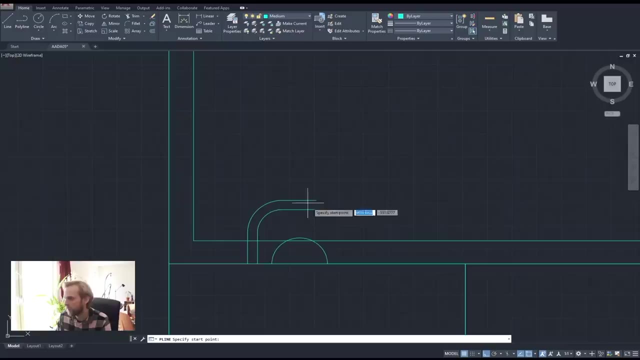 enter R. R. enter um, let's not use 20, let's use 50 millimeters between here and here, like this, and now I can offset, uh, by 20 millimeters outwards, like that just kind of close off the pole line. like so, join everything up and now do a little bit of trimming, so trim that and that. 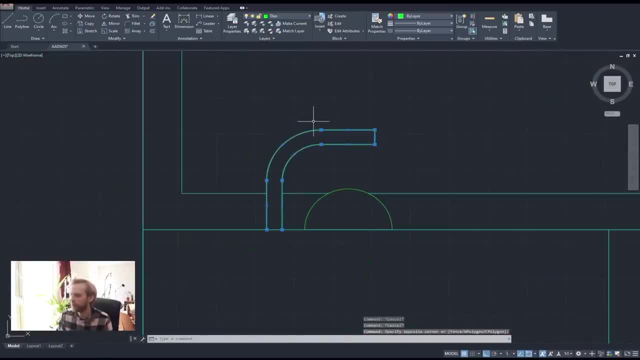 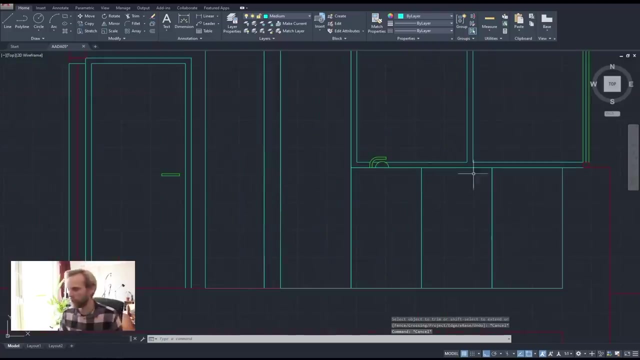 thin line. um, to go lower, trim, come on, trim, enter. there we go, and you need to be also trimmed. yeah, sorry, uh. so just you know, awkward water tap with some big, really big knob, whatever. so just you know, awkward water tap with some big, really big knob, whatever. 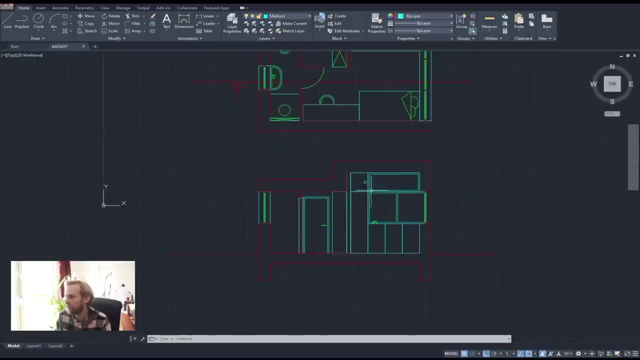 okay. so we have that that going on and that that is fine. uh, that that looks okay and there is still sink and toilet that are left to do. so I'll really quickly do it. so for the sink, I'm I'm thinking of having something like this: um, oh, how wide is the sink? I? I believe we used 400. 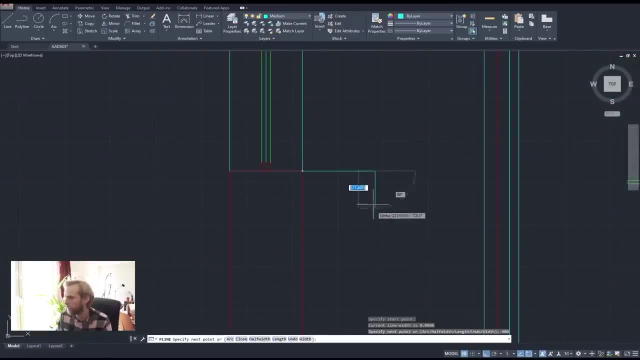 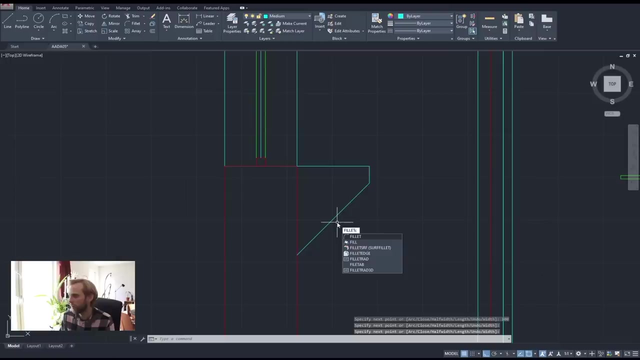 right, so it's going to be 400 mil, uh here. then it goes down by uh, let's say 300 mil, something like that, uh, and then it goes at an angle, and that angle doesn't really matter right now, so I'm just going to say something like that: right, that's it. uh, fillet, uh, select corner, or just. 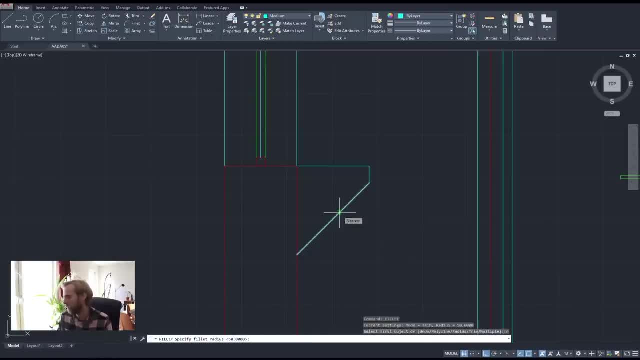 fillet radius, uh 30.. corner, or or just fillet radius, uh 30.. right, that's it, uh. fillet corner, or or just fillet radius 30.. just flip those radii like that. that's our sync. where is my trusty? 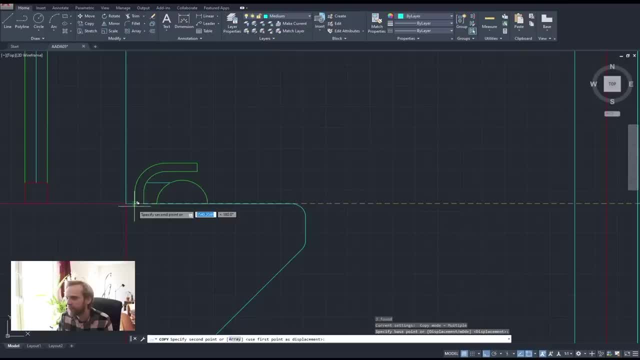 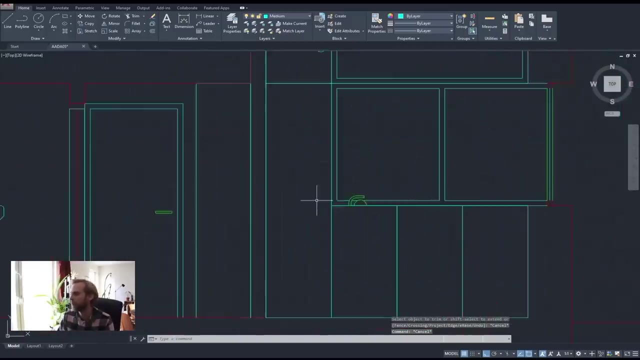 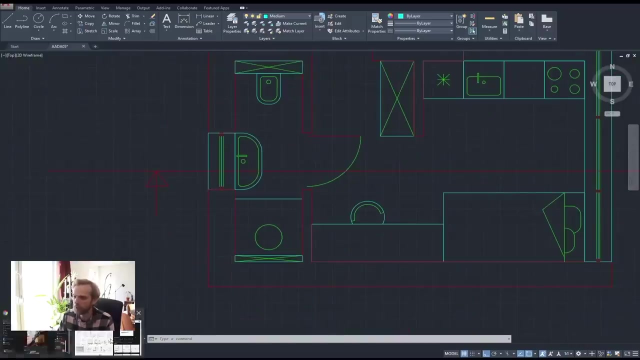 app right there, i'll just- and the rearrange, the rearrange, it scale this bad boy. 0.5, move to here and this trim, this trims away, tap, yeah, that's good. so that's our sync. and then we have the last thing as our bowl, and i will just: 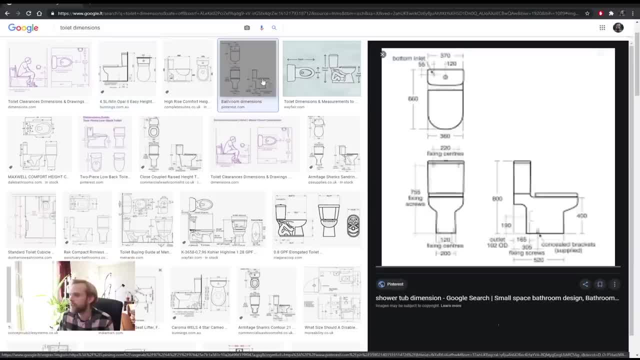 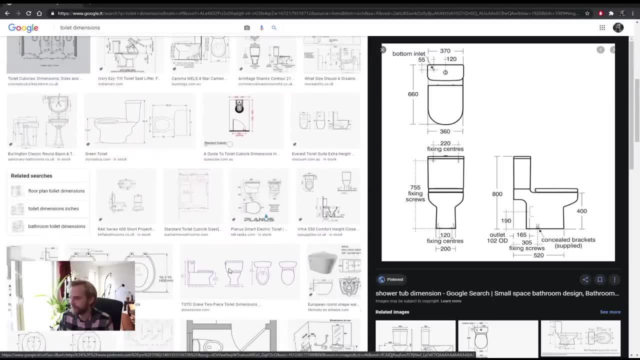 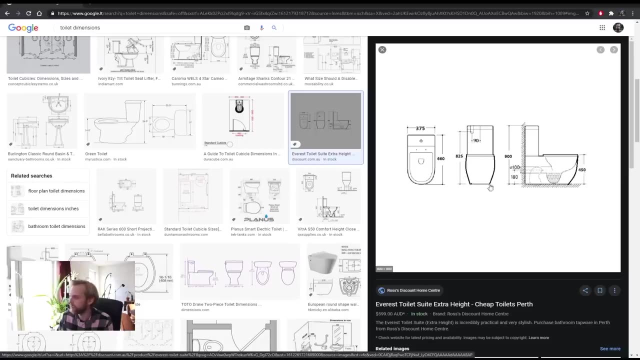 take a look at the bowl how it looks like from the front. uh, that's ugly, still like a nicer one. yeah, that's good enough. so it just goes kind of straight down. well, it does make a bend and it goes in a little bit. um, that's fine, let's do it that way. so i will create two. 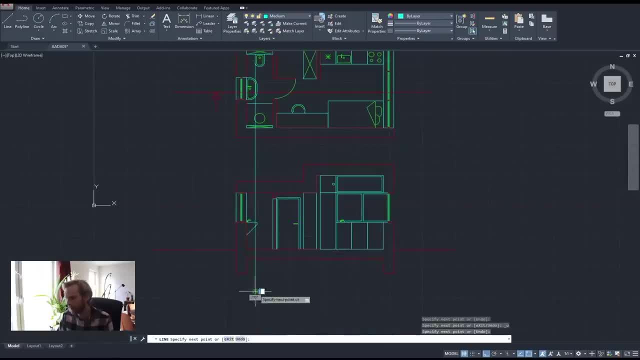 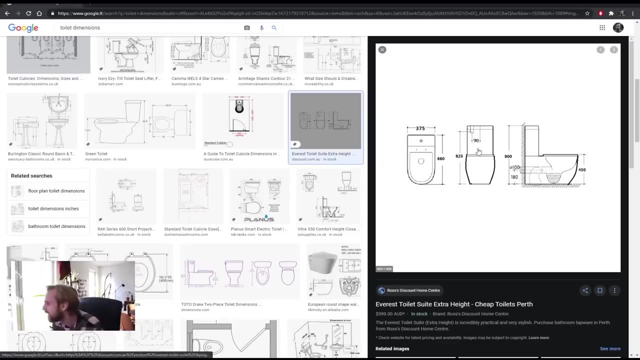 guidelines here up. that's not how you want to do it. guideline here, guideline here. how high are the bowls as well? um 450.. so they are 450 millimeters high. that's. that's good to know. where's my autocad? um a to 1. 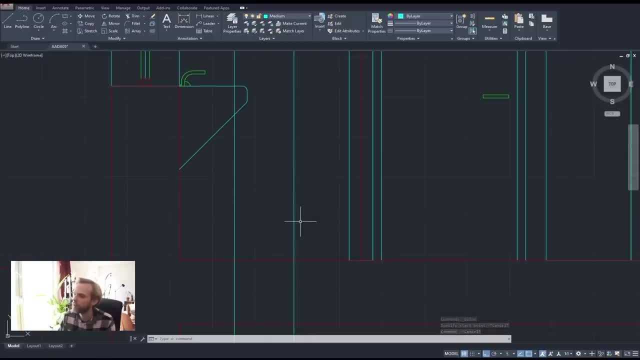 one amount, so i'll just give it a chopped away. so how do we do this? so there's gonna be a line here it needs to go down and in, okay, so let's do an offset by how much it's going to kind of go in. let's see by five centimeters. 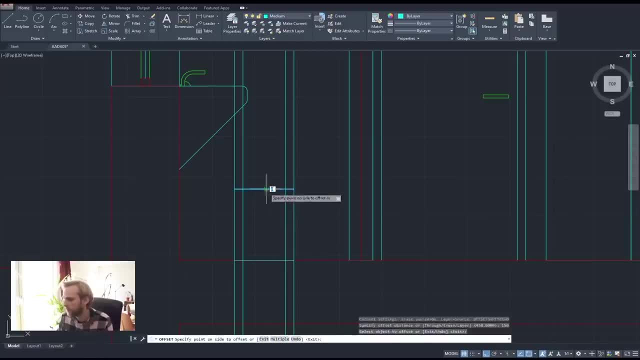 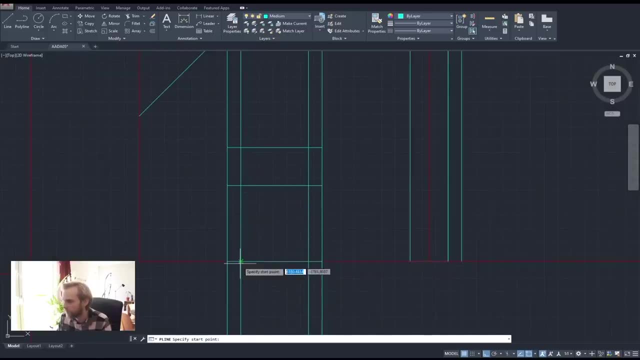 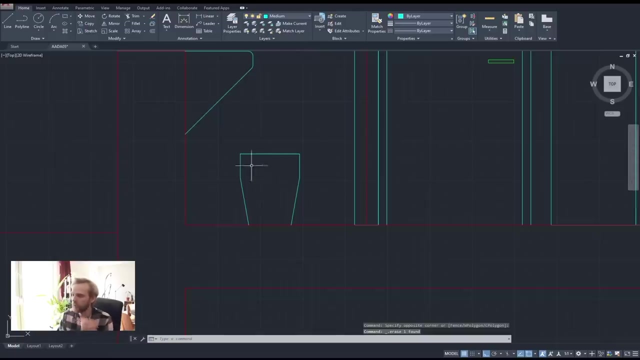 like that, like that, um, i don't know, 150 millimeters. this is from where it's going to kind of become thinner, and now i just need to trace around. so, from here to here to here, here, here, until here, enter, delete all of the guide lines. like that, that's our bowl. yeah, the proportion is fine. i'll keep it. 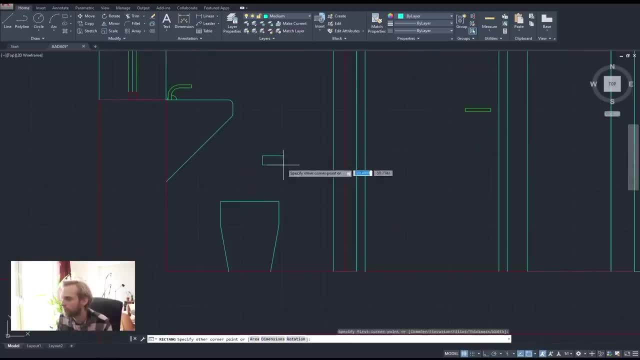 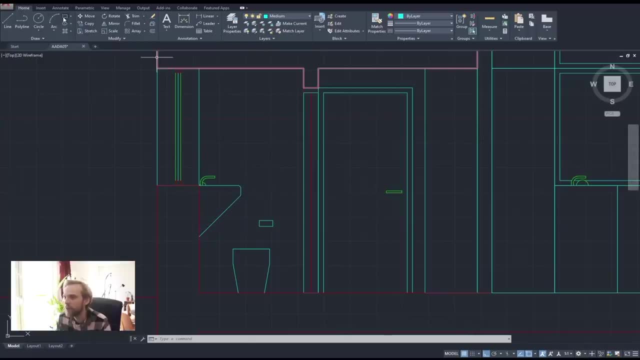 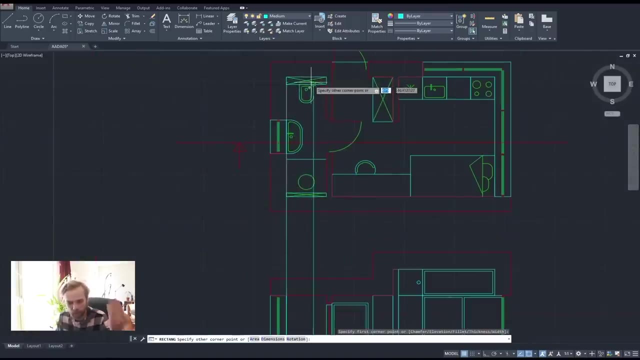 that, that's all we need to do. and the flush: uh, the flush button is located here. uh, now for the storage: uh, there is going to be- um, i, i have made that- that- that cabinet in in the back of the bathroom. so there is going to be. 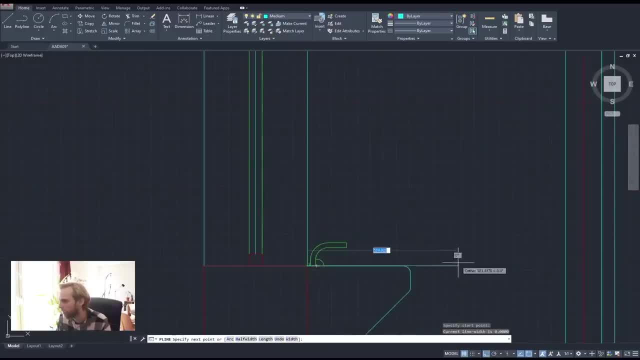 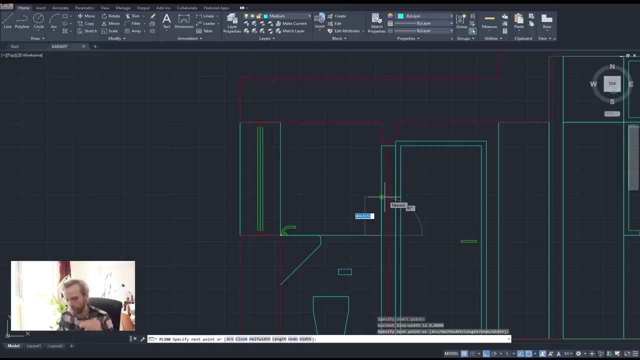 storage involved here. uh, so i'll just draw a polo line from. let's see, the storage starts at the sink level. so from here upwards, um, let's say, for the toilet rolls, the all of the you know stuff that you need at hand, uh, let's just give, give it 300 millimeters, something like that. 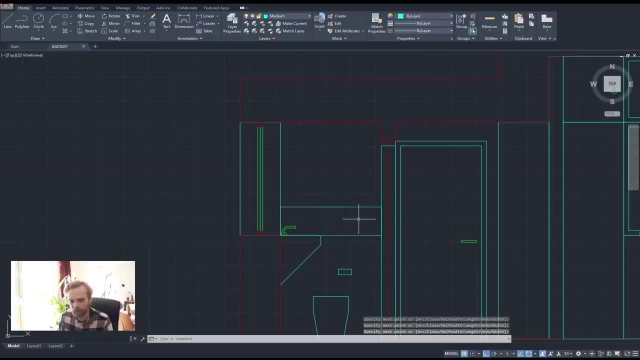 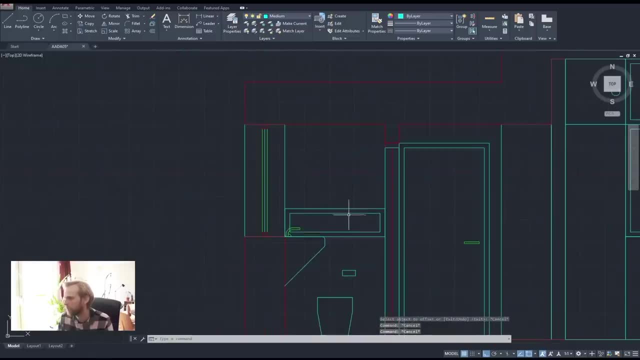 so this is going to be like open storage, right this area. so i'll just give it a frame of 50 millimeters, just to show the frame. oh, that's uh. 50 is too much. uh, this is also a problem here. 50 is too much. maybe let's not give it. no, I will give it a frame. offset 18. 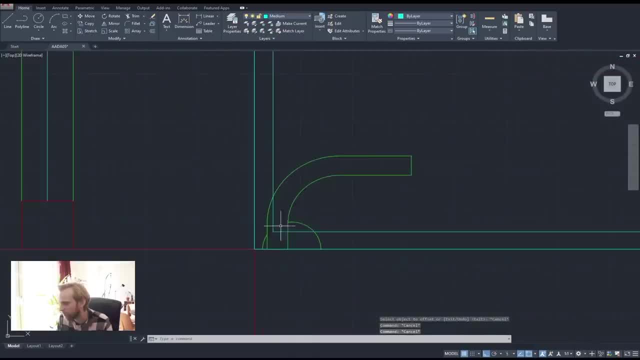 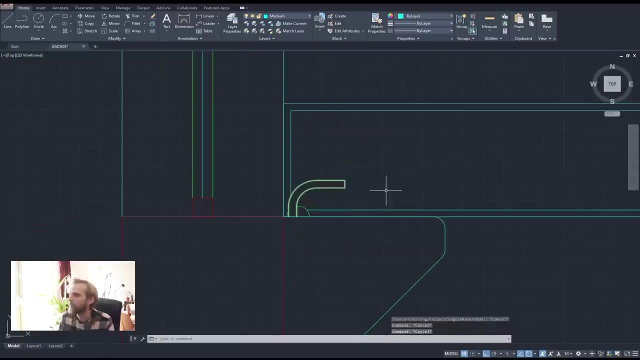 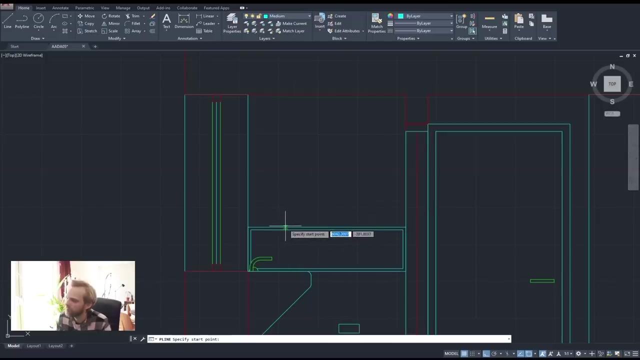 millimeters. that's the thickness of an MDF board like that. we need to clean this up a bit trim. no, no, there we go. so that's storage, and then above it we will have like three panels. I think we will have three panels. let's do three. 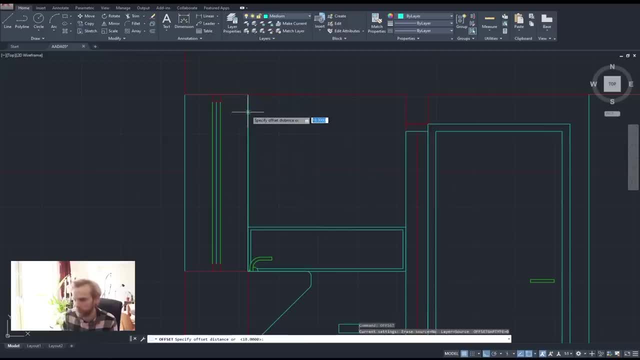 panels. so from this side we will offset by how much, by how much, by how much? if that's a mirror, then we can do 300, 300, 400. I think that's that's reasonable. so let's do an offset of 300 centimeter millimeters, or millimeters offset by 400. 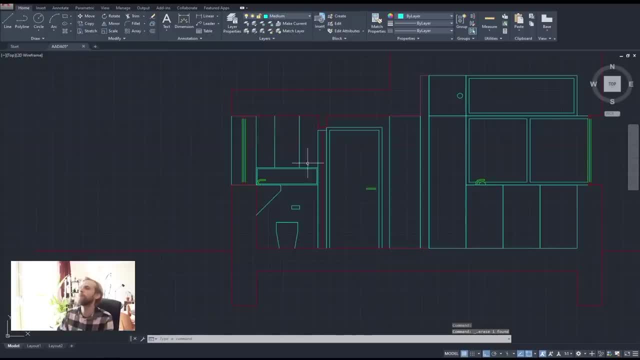 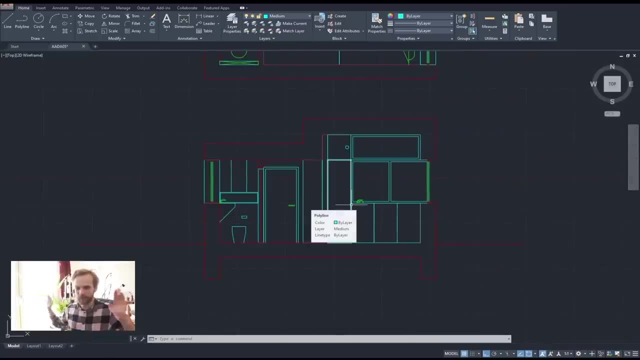 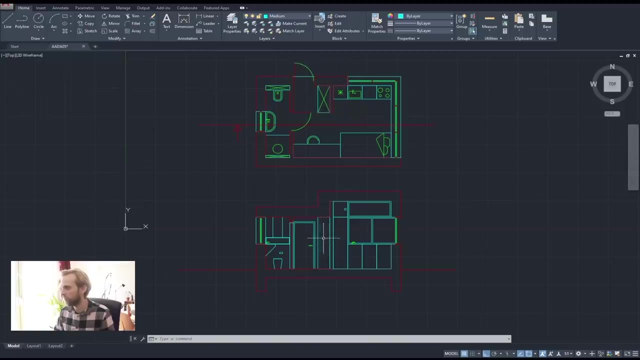 millimeters, something like that. so that is kind of storage above the above the toilet done. but that's enough. that's enough, I think we have the door, we have the door, we have the shelf here, we have the retaining wall, we have the partitioning wall window, everything that we see here, everything that we see here. 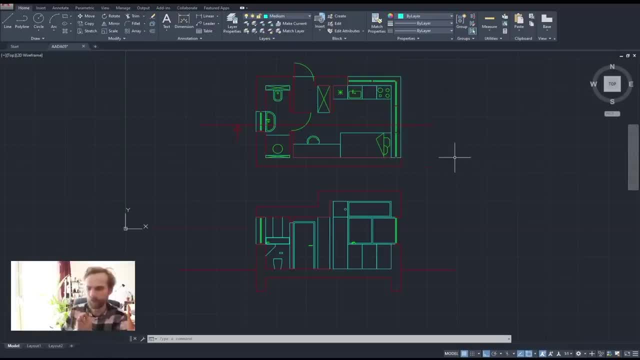 okay, section is done. let's learn one last thing, and then we will call it a day. okay, section is done. let's learn one last thing, and then we will call it a day. so one last thing is hatch. and, by the way, for this section, let's make the mark. 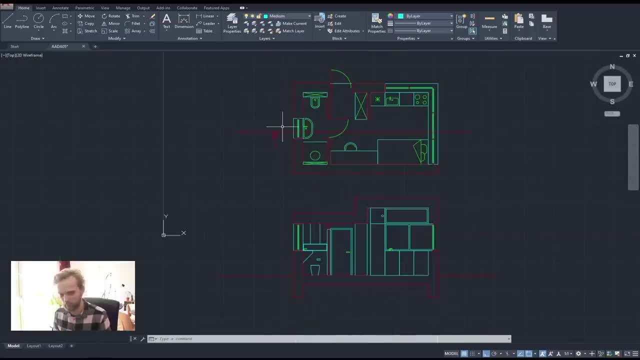 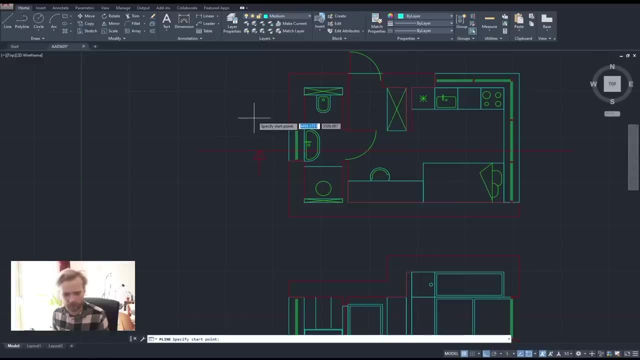 out a little bit nicer as well, because it's a little bit eh, you know. so let's make the mark out a littl e bit nicer. usually there's no kind of convention for what kind of section markups to use. uh, the ones that- the one that i really like using is, um, a line segment, that is, i don't know. 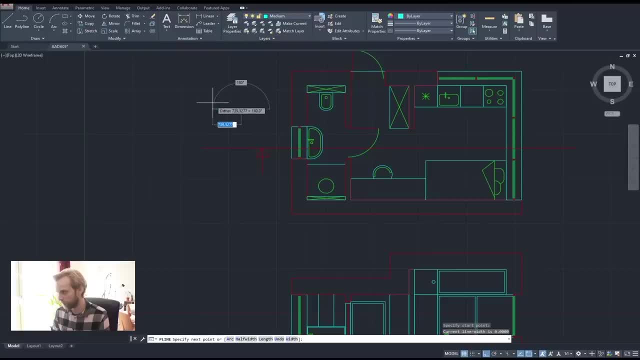 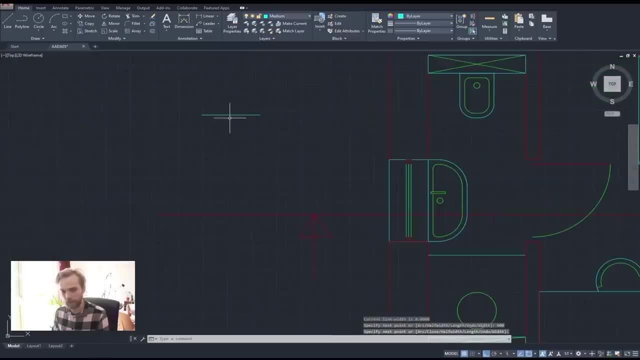 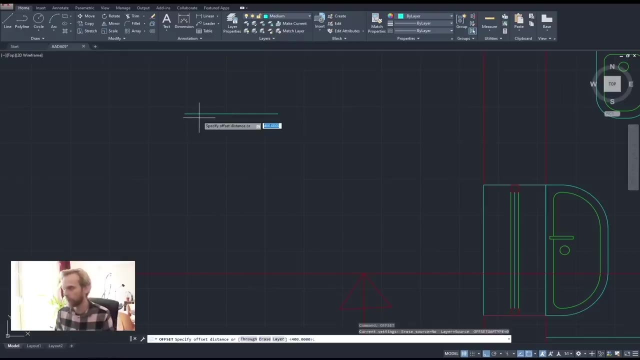 uh, in, in this case it's going to be like 600 millimeters, something like that. it's kind of a line segment here. then we have: um, then i offset it and i'll offset it by 300 millimeters. no, that is way too much, i'm sorry. i will offset it by 100 millimeters. 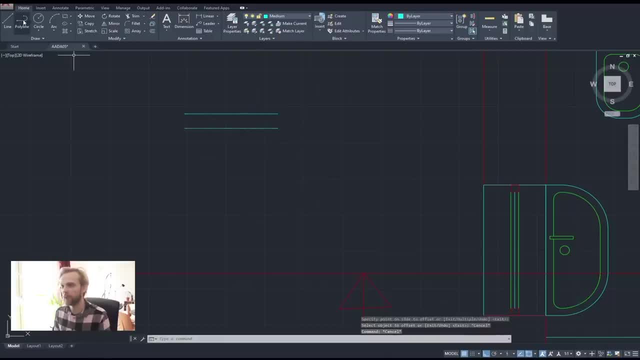 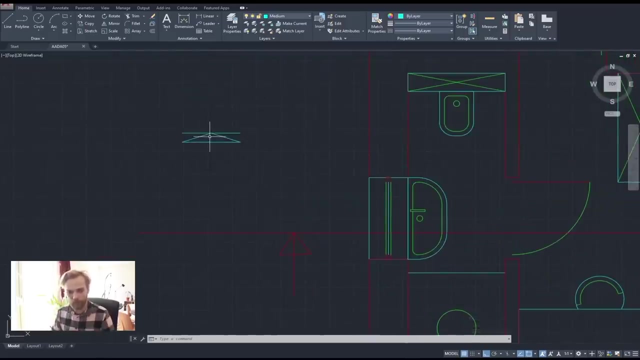 yeah, there we go. that's much better, and i will draw to the midpoint here this um, this arrow, and i'll just join up this arrow. so now i i have a line and i have an arrow, just like here: line and arrow. arrow is showing the viewing direction for this section. 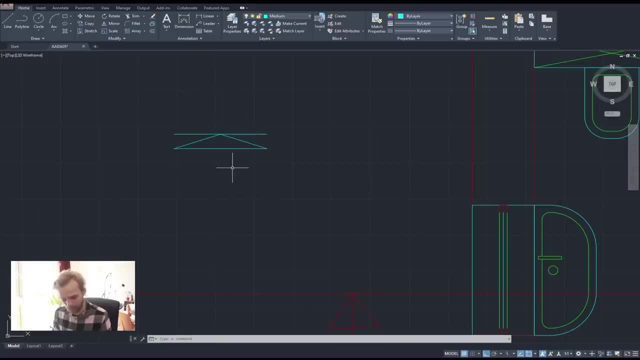 and later i will add text here or i can add texts here now. so the shortcut is text, enter: um. you specify the start point here and you type in or you specify the height of the text. so what's the height? what's the height? um, um, um. 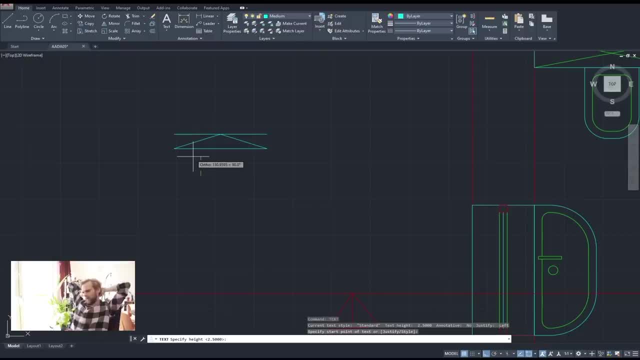 I don't know. let's do 200 for now and we will, we will switch, switch it up if it's too small. so height is 200- enter and rotation. angle of text: zero, enter. and now i can type in: finally: so x, x, x, a, that, that's it, escape. 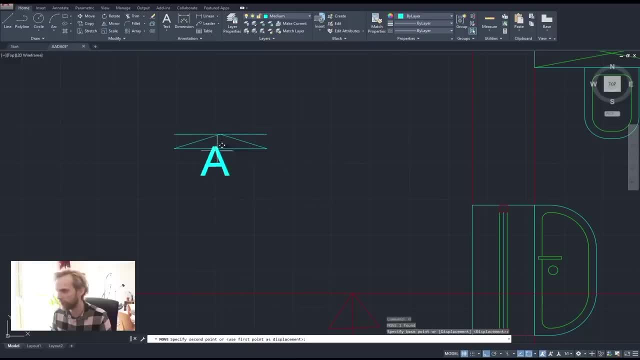 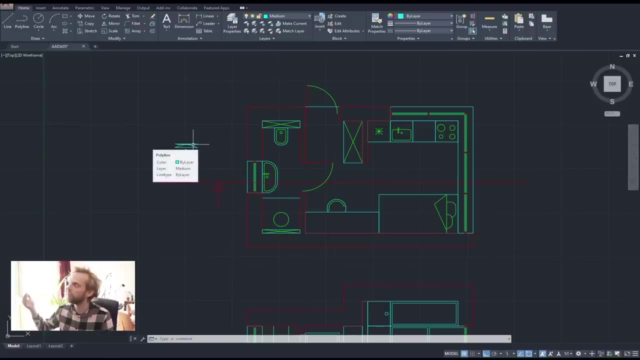 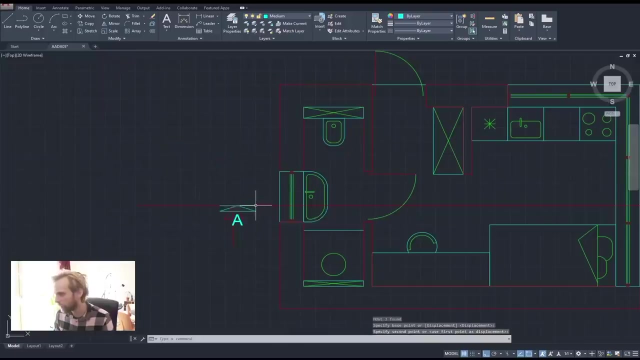 so we just drew, we just wrote a right. i'm just going to kind of center it. so once i name this section, it's going to be named section a, dash a or a, is it? the dash is probably a dash a, a section a a, and i will just place that section markup right here. make a copy of it. 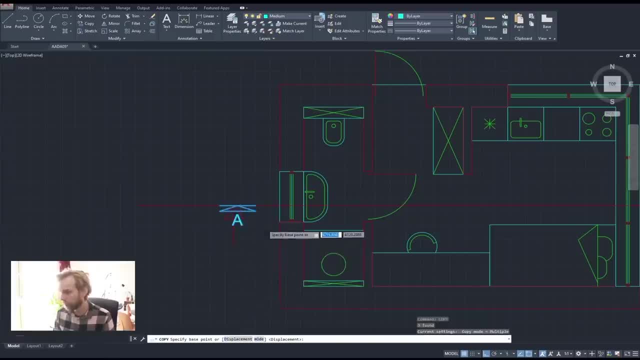 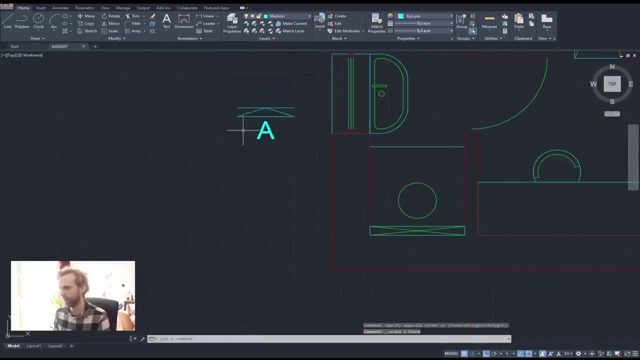 and i will just place that section markup right here. make a copy of it. and i will just place that section markup right here. make a copy of it. to the other side, to the other side of the building. very important to have section markups in your project. please do so. 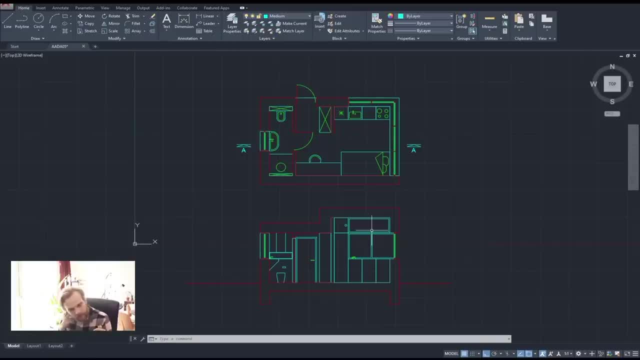 um, right, so that's text. right, adding text. that's nothing too fancy, it's just міczskiία. basically, you read what it asks, you asks of you, in the comment line and decently asked you in the command line, and you'll be good to go. 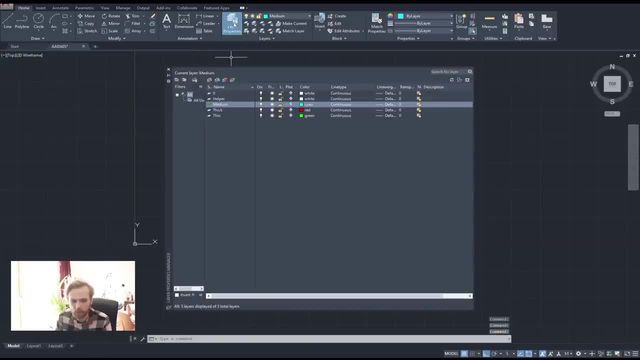 the text will need a separate layer, one in the timeline layer. so let me go to layer properties and let me create one more layer. i'll call it text, right? so that's going to be my text layer and my text is going to be yellow, sure? and then i'm going to create one more layer, even more layers, yes, one more layer and call: 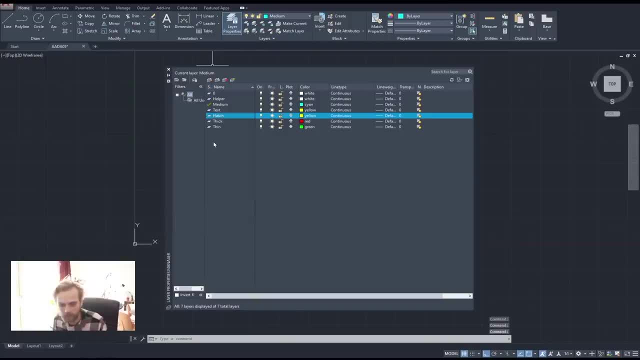 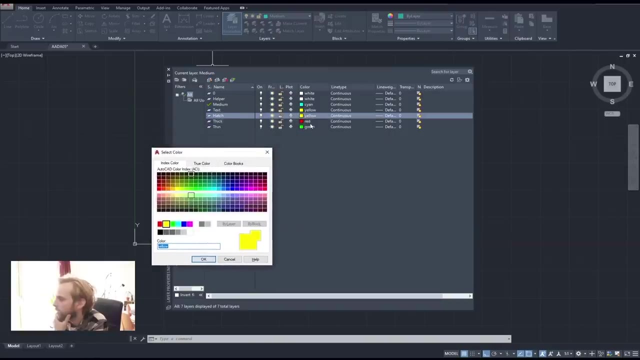 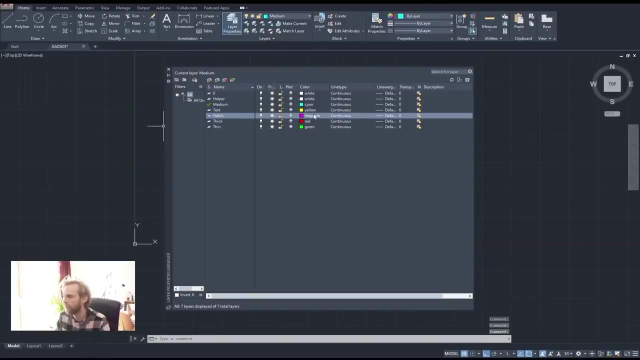 it hatch. so hatch is basically fill right in in photoshop and illustrator. you have, fill in cat software, you have hatch, uh, so hatch layer, and i'll make it uh red, green, c and yellow, pink or magenta, all right, so let's have a hatch layer with magenta. 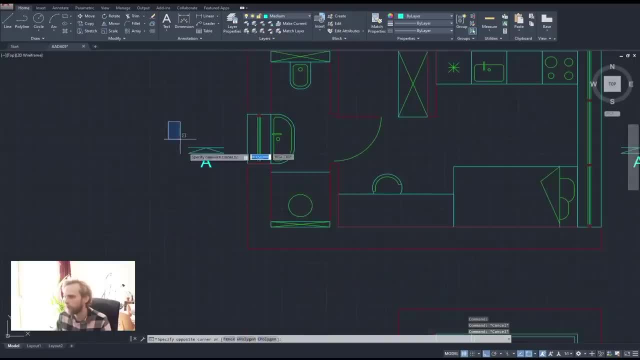 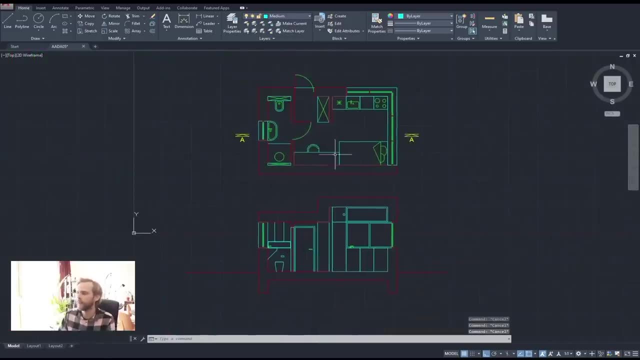 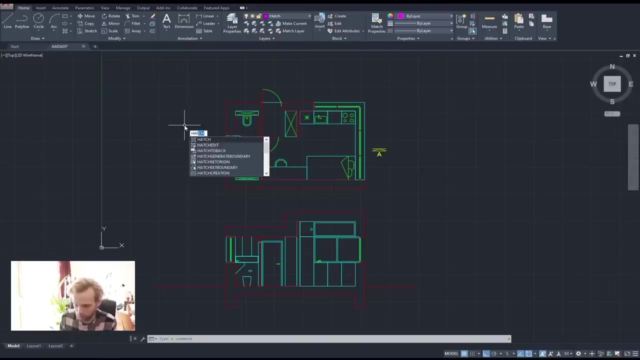 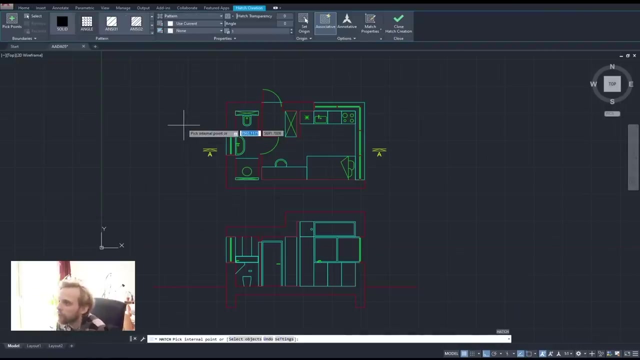 color. close that um. now i will take my markups and i'll place them in the text layer. excellent, and now i will use um hatch right to fill in the walls. so i'll go to, i'll make hatch layer my active one and i'll type in hatch or shortcut, for it is just h enter, so that's hatch. and once i have, 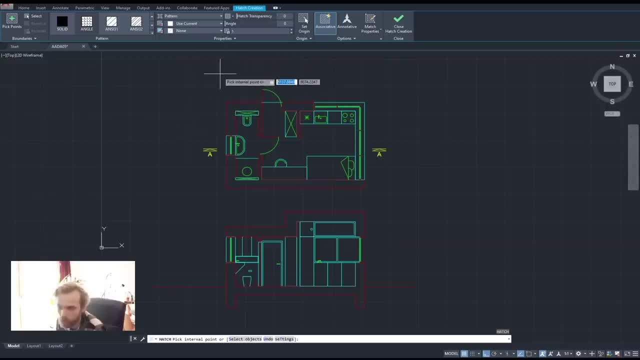 typed it in. it will give me the settings for the hatch, of course, where i can choose different um patterns- yes, the word is pattern, different patterns, right, uh? and also, like, i can change the transparency, the angle and so on. so let me, um, let's, let's do it this way. let me create a. 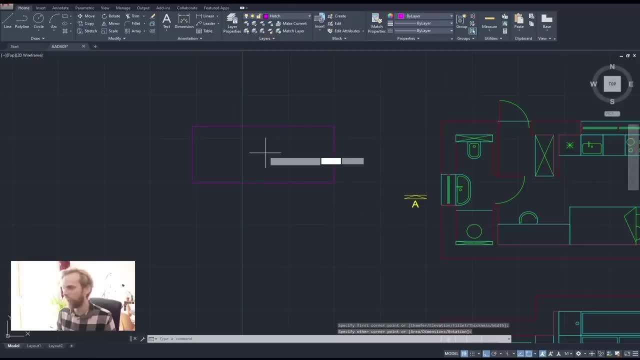 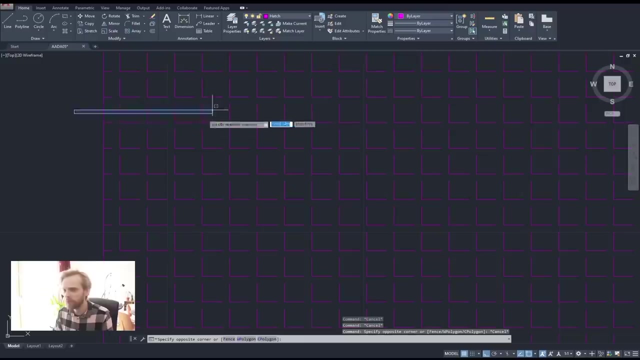 rectangle like so, and hatch it in right. so if i just click inside of the rectangle and hit enter, that's it. it's hatched in right and this is uh. it even has a pattern if i zoom in right and the pattern is super dense, so it looks kind of filled in from from when i am. 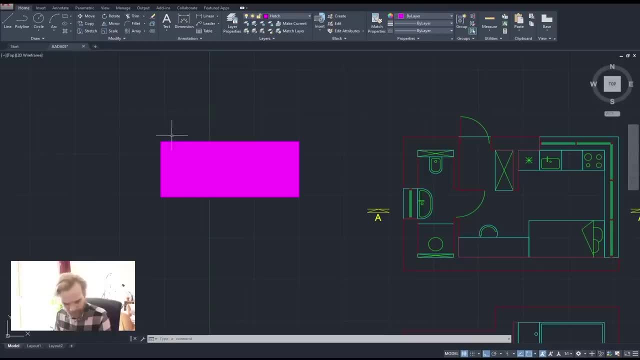 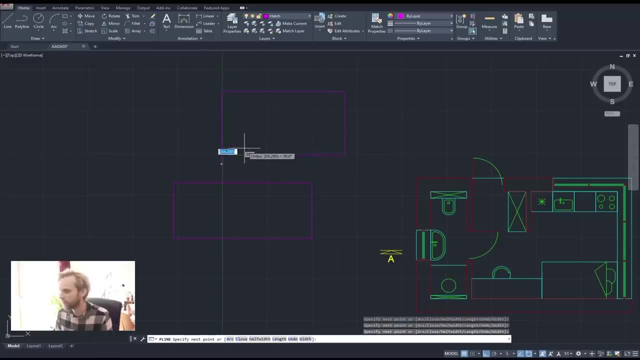 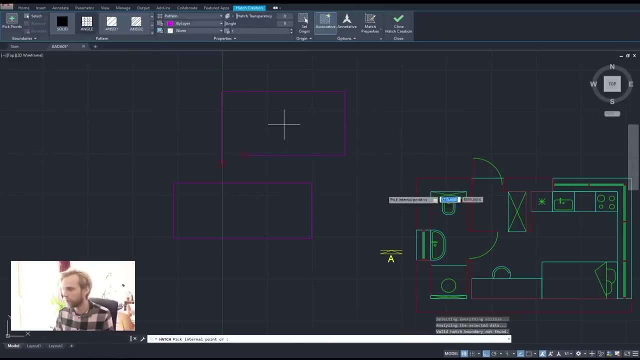 zoomed out. uh, so that's a lot of bad things happening with the hatch. let me select the hatch and delete it. uh, let me also do a rectangle that is not closed. right, there's a gap here. hatch click cannot be determined, right cannot. hatch cannot be made close. shows me even where. so it only works with stuff that is. 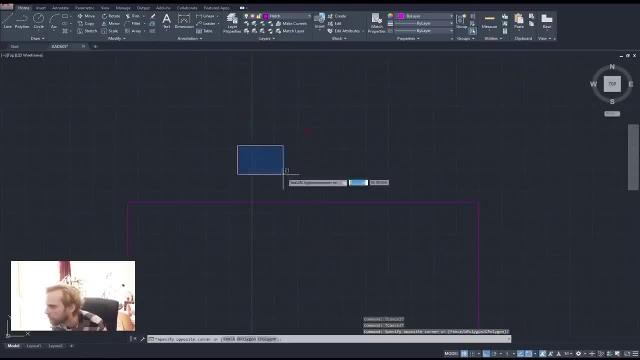 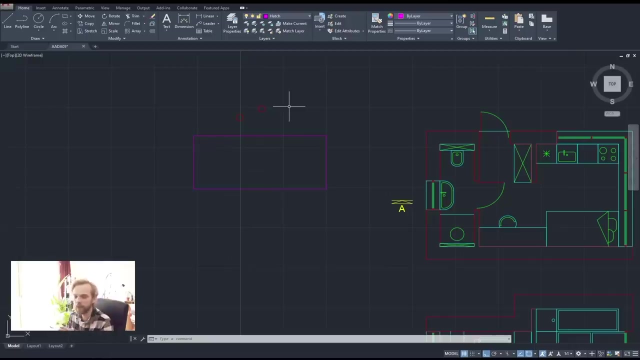 closed off, right, uh, can you go away please? oh my god, now, now i'm gonna, anyway, let's ignore those two circles here. um, so it only works with enclosed, uh boundaries. uh, that's the first thing. the second thing: it uh the scaling is very important, uh, if you want to have a pattern for the hatch, but you're scaling is so small uh that it looks. 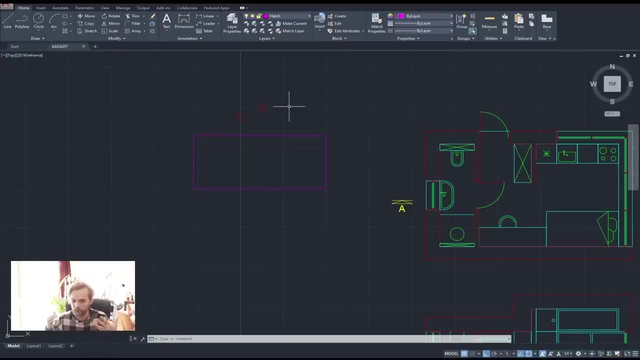 like a solid and you think that you have a solid hatch like a solid fill, but it's actually a very, very tiny pattern. your computer will get super slow because of that, so let me do hatch again, um, and here i can choose a pattern, right, so the solid pattern is just basically fill in. 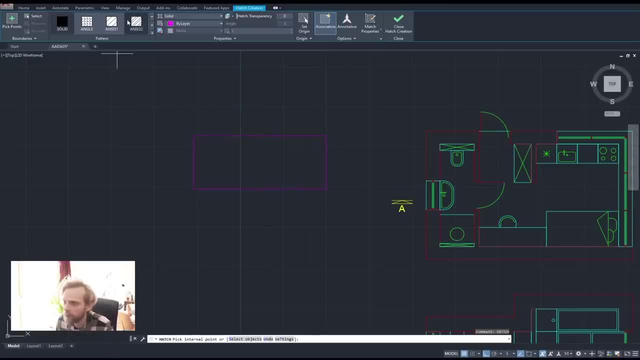 right, it's just filling in. then you have the angled patterns and you have a bunch of them. actually, is it possible for me? yeah, uh, so i can click on that small icon there and i can see all of the patterns that i can choose from. oh my god, so, so bad um. 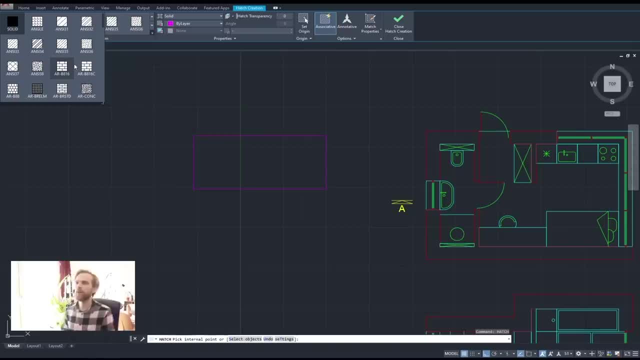 so let's not look at the bad patterns, let's just talk about these. what you have here, so hatch pattern is usually determine the material, uh, that you're cutting through, and if it's a solid hatch, it's usually uh, you're saying that, uh, don't worry about the material for now. 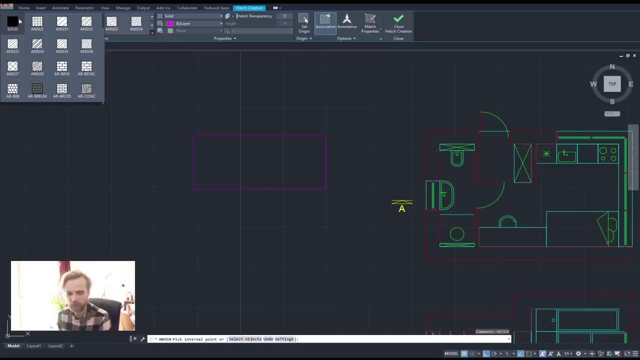 this is just a proposal, entry project, and the material doesn't matter, right. but if you later, later down the line, if you want to kind of add materiality to your drawings, explaining that, oh, this is concrete, while this is wood, while this is steel, then you use hatches, different hatches, 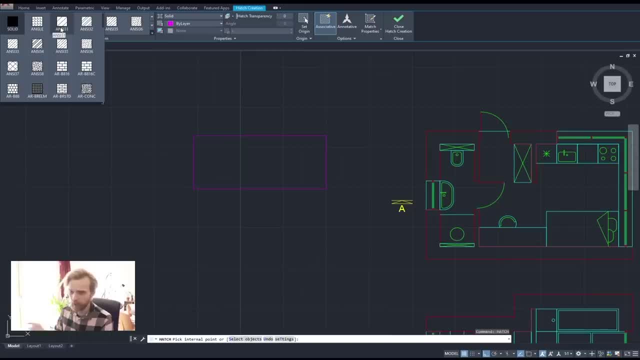 that determine it. so the regular angled hatch, uh, this one where i have my mouse is concrete. usually it's concrete. um, then the one right next to it, the one with the double line, uh, well, okay, the tricky thing is that it changes between country to country. right the the? 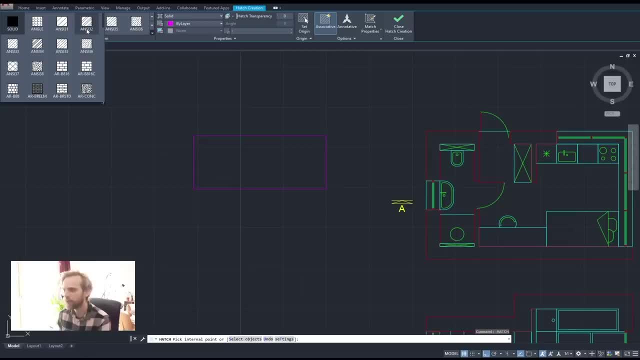 regulations, uh, change between country to country, but, um, to my knowledge, most of the countries use this as steel metal, right? so that's the hatch for metal, and the third one is hatch for wood, right? so three main hatches that you kind of go through once you introduce materiality. 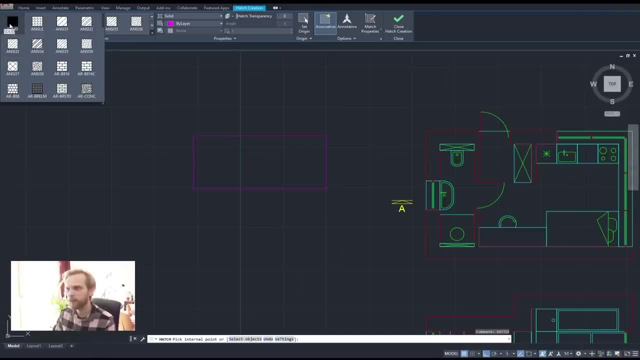 For now, I'm just going to use solid hatch. Well, actually, I do need to talk about scaling. Solid hatch doesn't have any scaling because it's solid, right, It's filled in. While these do so, you can change the density of the hatch, So let's. 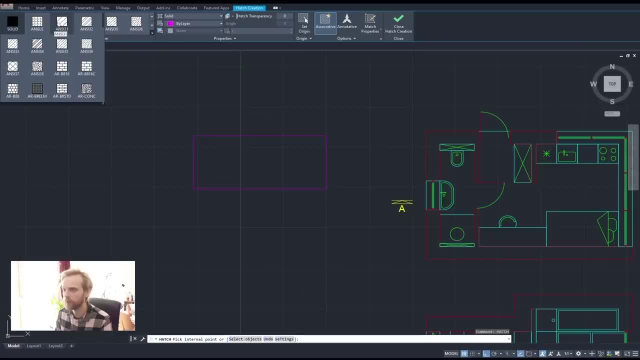 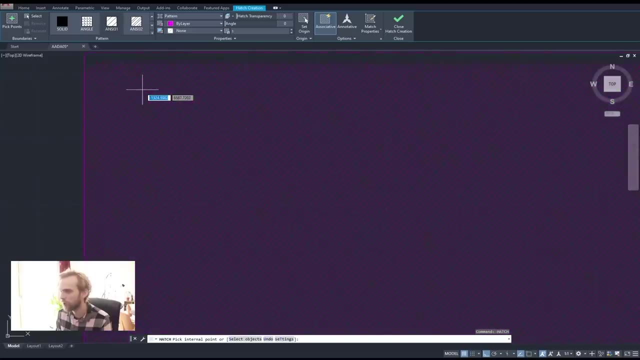 let's talk about this. Let's let's choose concrete right: The regular angled hatch. Once I have this chosen and I hover my mouse over the rectangle, I see it as solid, but if I zoom in, it is still solid. No, it's not There we go, It's all. 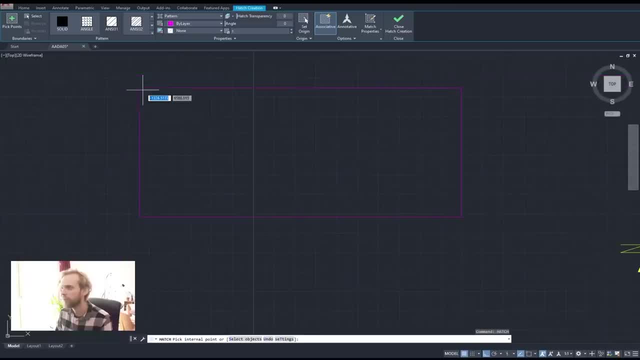 messed up right. It's super, super dense. So the first thing that I want to do is I want to change the density, and the density is changed right here. Hatch pattern scale right. If I change the scale to a hundred, enter and I have er my mouse over the. 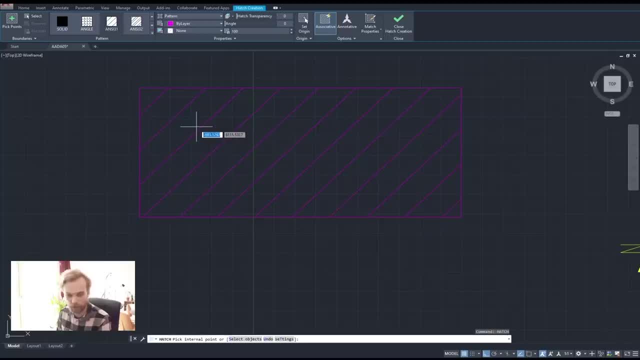 rectangle. Now you can see that the hatch has 100 times larger scale and that is actually too big. so let's do 50 and that's fine, Just to show you, you know. So that's 50. Then you have a possibility to take to change the angle. 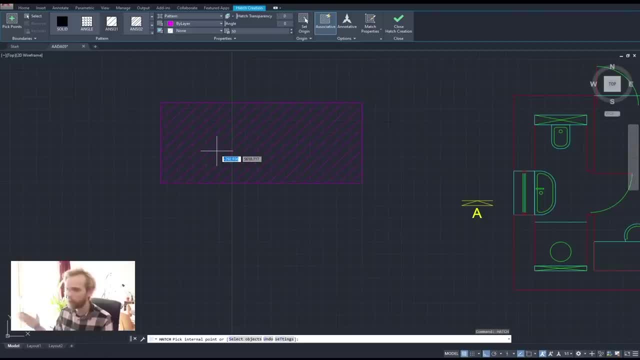 so this is, you know, the default hatch. What if I wanted just horizontal? Well, I just changed the" to 45. well, that's vertical, but you get the idea right. so minus 45 would be horizontal, right? so that is how you change the rotation of the hatch, super. 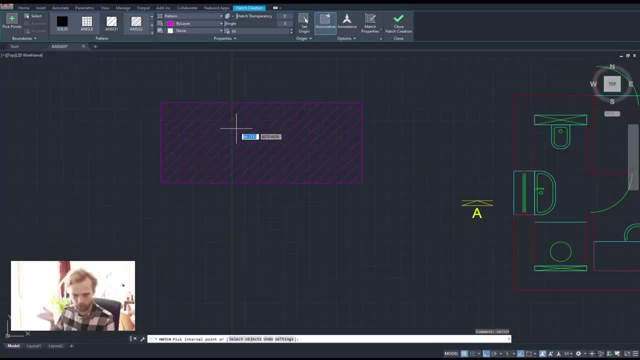 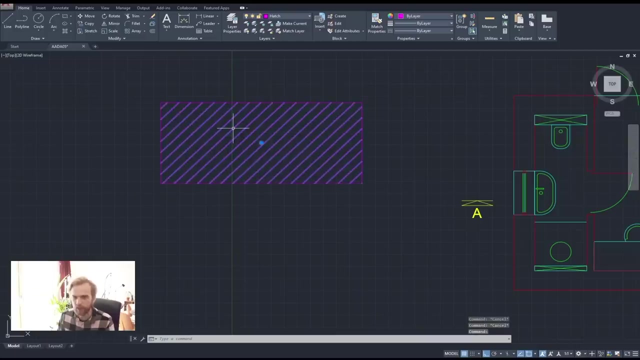 useful. for now, I will keep it at 0 and the default value for the hatch is 0 degrees. then you have transparency. don't mess around with transparency, ignore the transparency. there's one more thing, and that is one more useful thing, and that is set origin and it's basically: if I let me just create this hatch and then 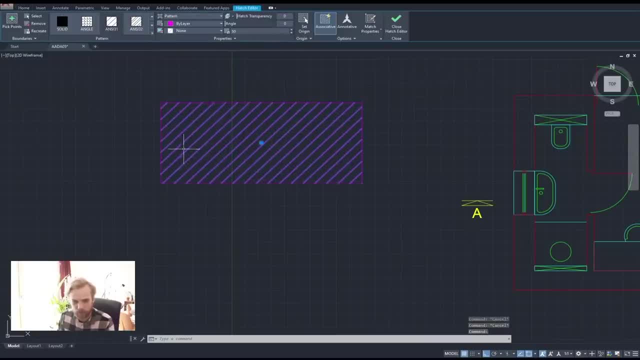 click on it once once. once it's created and I click on it, it will give me the hatch editor tab again, right, as if I was editing it, and now I can change the origin right. so you can see that I can change the origin right. so if I want to change the 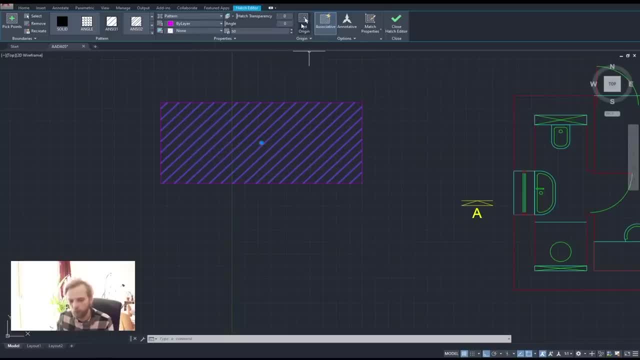 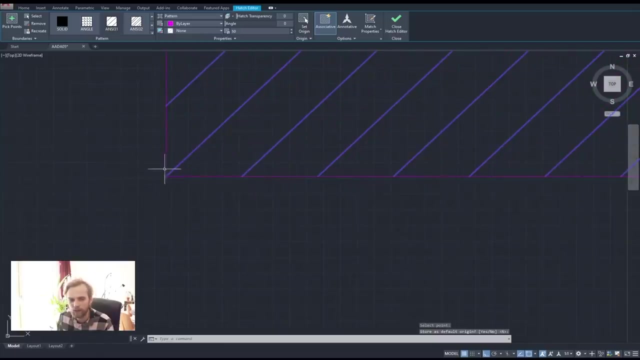 origin, right. so this is a point from which the, from which AutoCAD, starts hatching your geometry, right? so if I click on this set origin now and I choose- let's say this point right here, right, the hatch will be aligned with that particular point. so when you need, 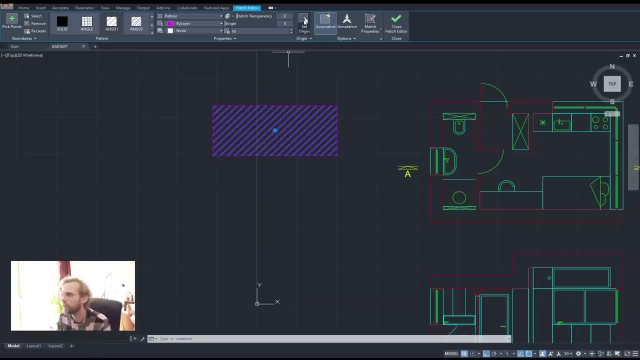 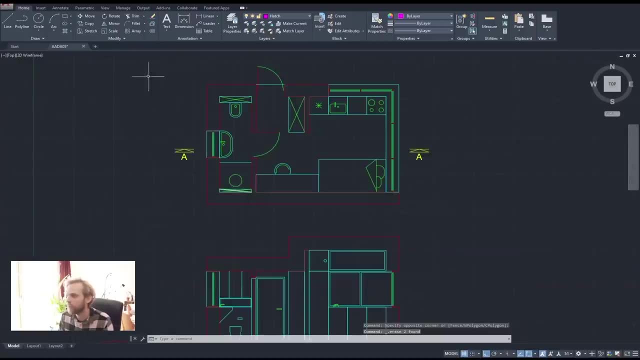 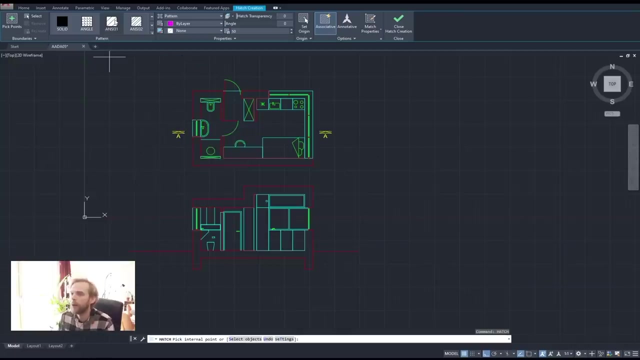 something precise in terms of how it's hatched. that set origin point is a lifesaver for sure. yeah, that's about it in terms of hatching. so now let's hatch our, our buildings, edge enter. I will actually use the angled hatch, why not? and I will just. 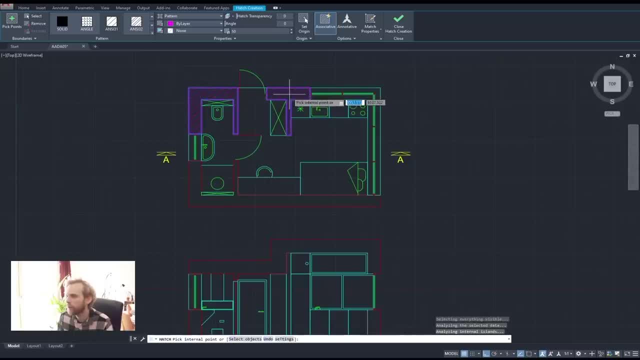 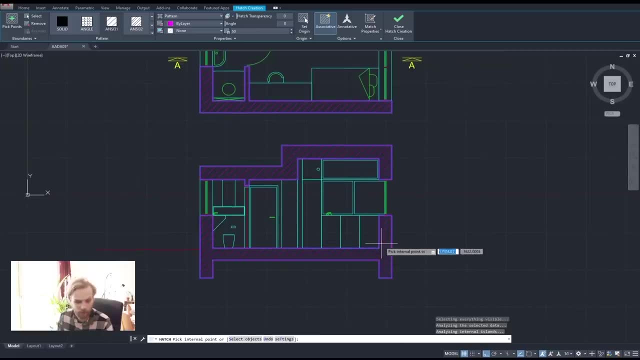 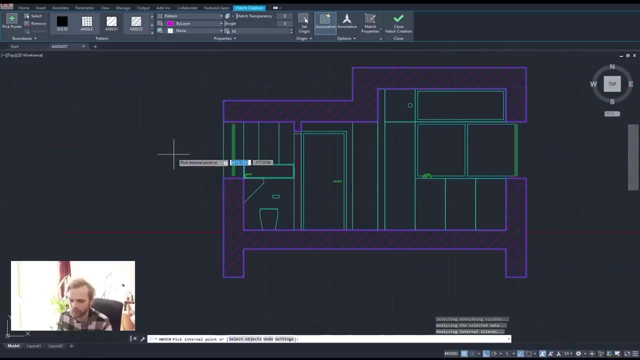 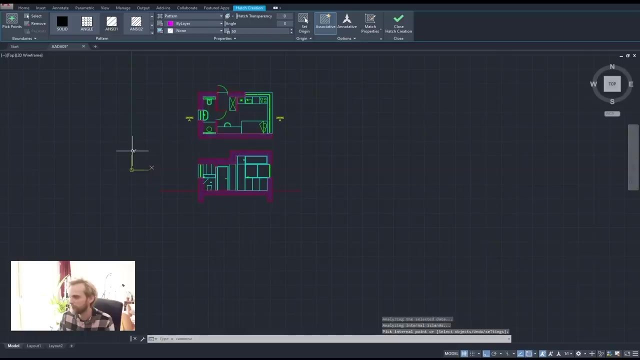 be clicking inside of the walls because that's the stuff that we cut through right. I could be hatching in the side of the frames window frames, but that's not no way too small. no need to hatch those. so that's, that's the walls that are done. enter and actually the 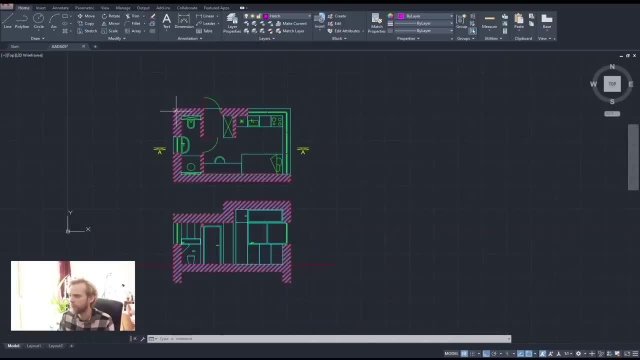 hatch is pretty big, pretty coarse, so what I can do is I can just select it, go back here to hatch editor and then just change the the density to like 20. maybe, yeah, 20 is nice. so I can just select it and then just change the the density to like 20, maybe. yeah, 20 is nice. 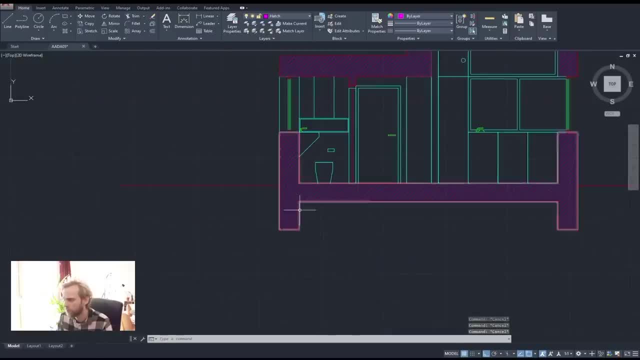 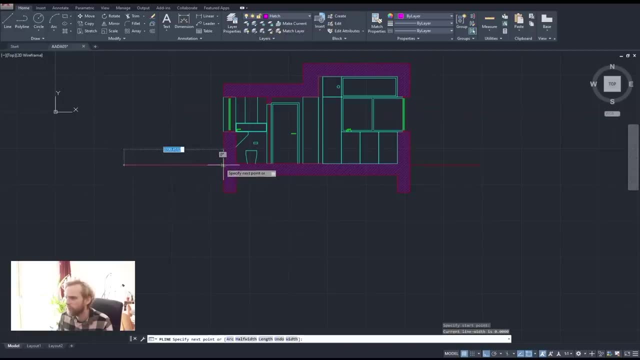 yes, 20 is nice, so I can just change the the density to like 20, maybe. yeah, 20 is nice. that is now hatch 10, and let's do the same thing with the ground, because I want the ground to be hatched in as well, so I'm just going to create a temporary. 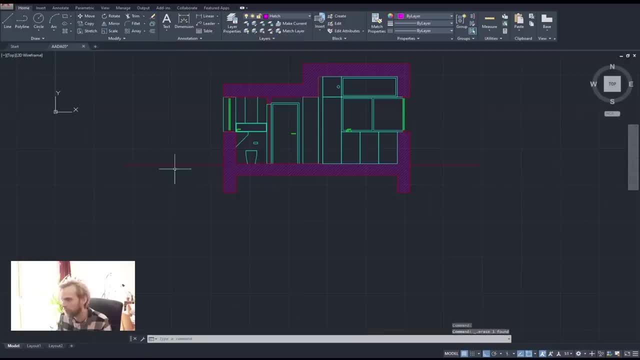 polar line here maybe a little bit smaller, maybe just goes from here to here, something like that. there, This is just. you don't need to be precise with this, just hatching in the ground. So it's something like this, and then I will start from my fall line. start there, just. 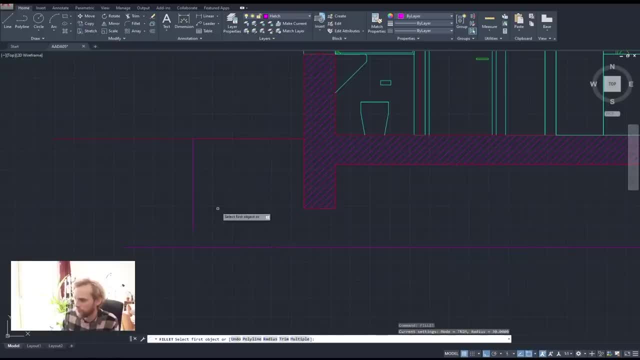 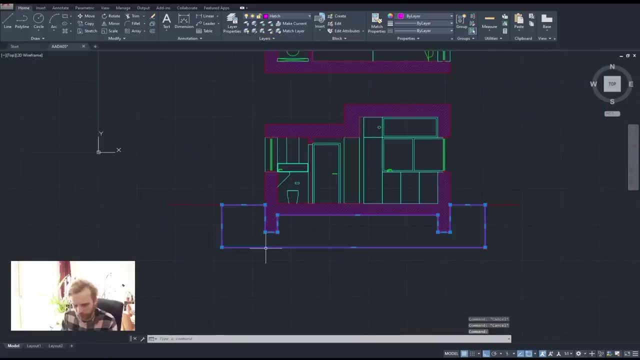 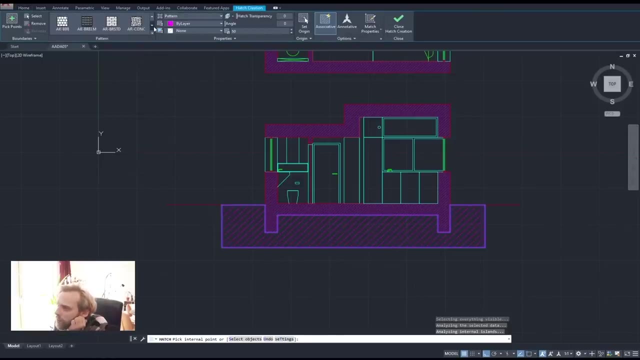 make a horizontal line and just use fillet with radius of zero to kind of fillet these two guys together. So now I have a closed fall line and I will hatch it and I will place a hatch inside and I will change it to a different kind of a pattern. I'm just thinking what? 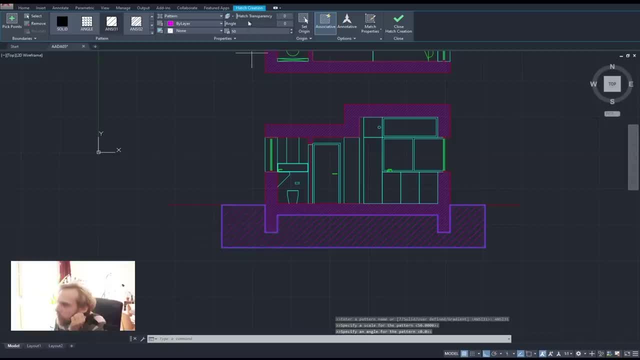 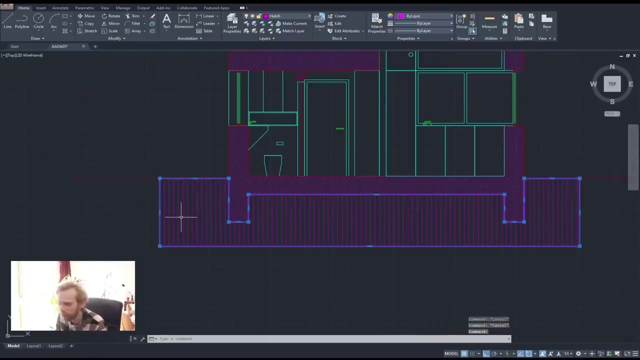 kind of pattern should I use? Maybe I'll still use the angled one, but I will change the angle to 45 degrees, something like that, and I will change the density to 30, something like that. That should be good enough, And now I don't need that border anymore, so I'll just delete it, just to have the hatch. 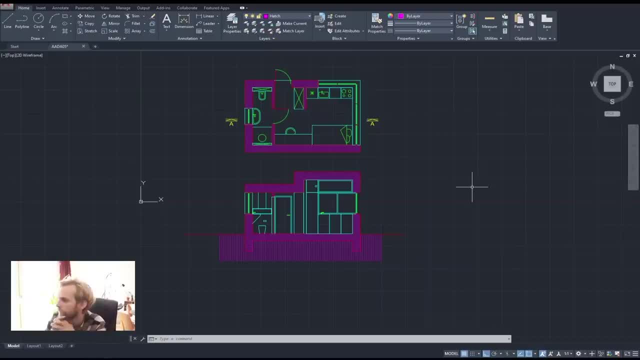 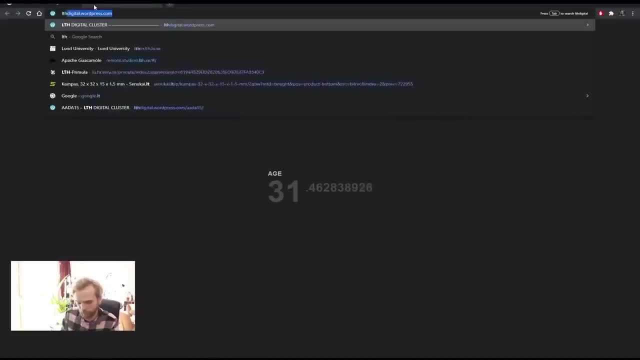 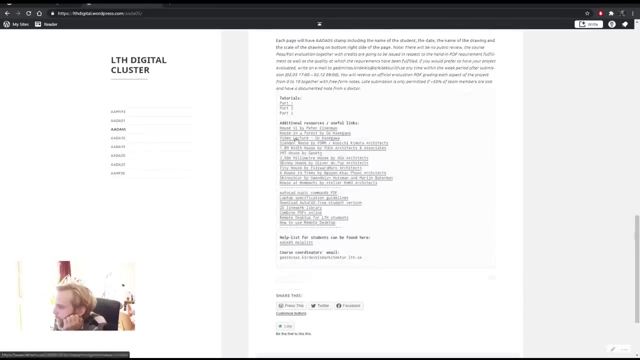 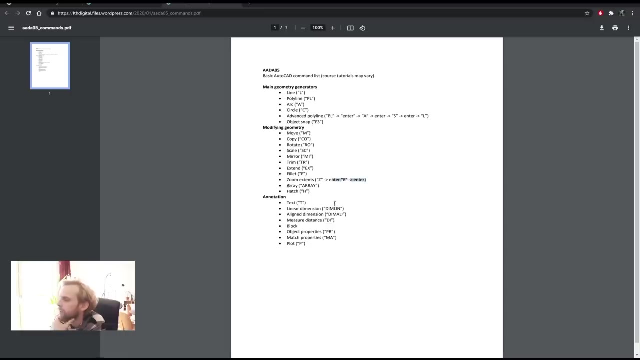 Okay, I think that is it. Can I check? I will just check the notes. Just give me a second Array. next time Arrays whatever not important Text. oh, I already showed you text, that's good. Less things to show you tomorrow, So that's fine. 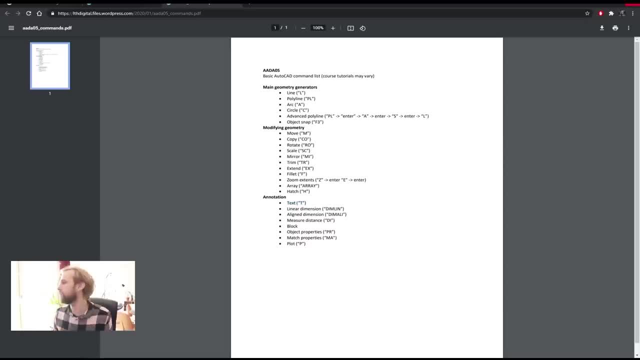 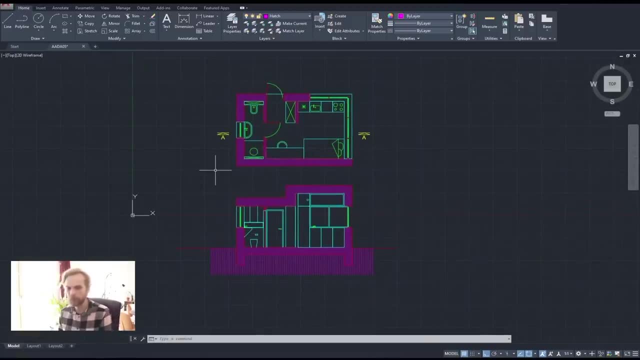 Yeah, so that's good. Everything that I wanted to show today is shown Tomorrow. we will work on the axonometry and we will finish up the project. So that's that. Go to work and enjoy the process Later. bye. 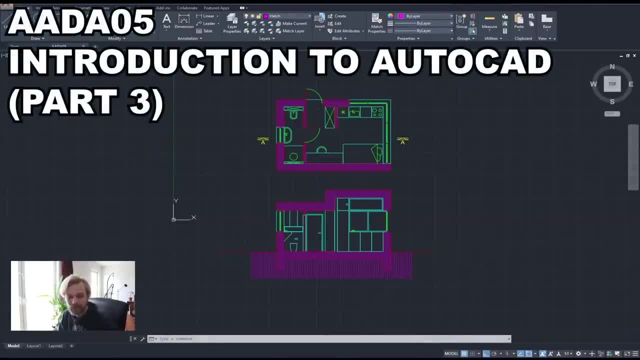 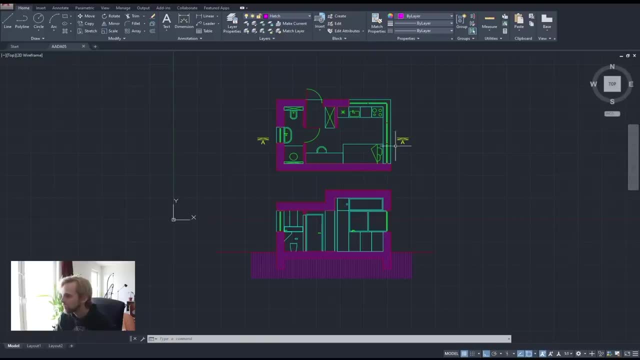 Hello, hello, hello, And welcome to the last part of the AutoCAD series, where I'm going to end and finish up this project and show you all of the remaining tools that we kind of need to use to be able to finish up. So right now we have a plan, we have a section. 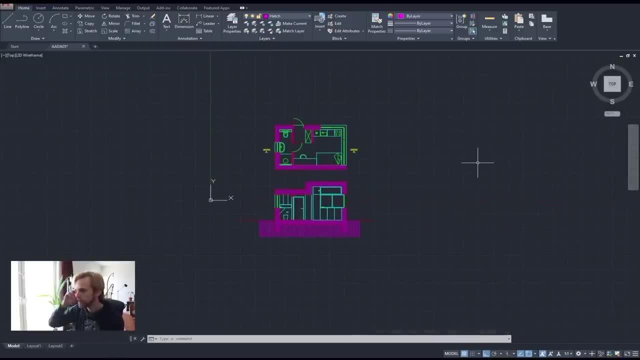 Those still need to be done. I'm going to show you how to do that. I'm going to show you how to do that, So let's get started. So we need some work and we still need some additional information, but most of the stuff. 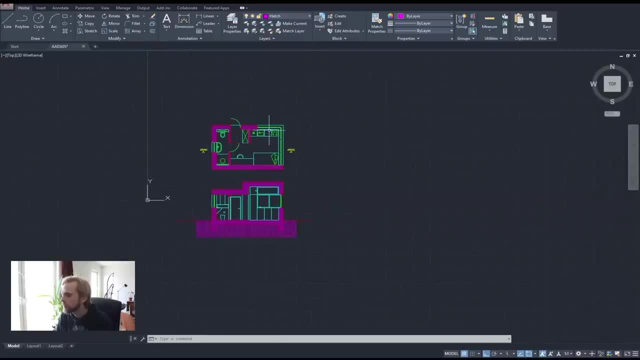 that we want is already there. The thing that's missing is the axonometry drawing. So I'm going to do exactly that right now, And then we will continue on with adding additional information and basically extracting the drawings into a PDF. So, to start off, axonometry or 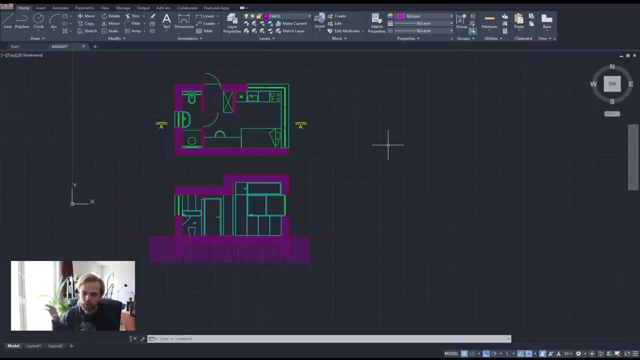 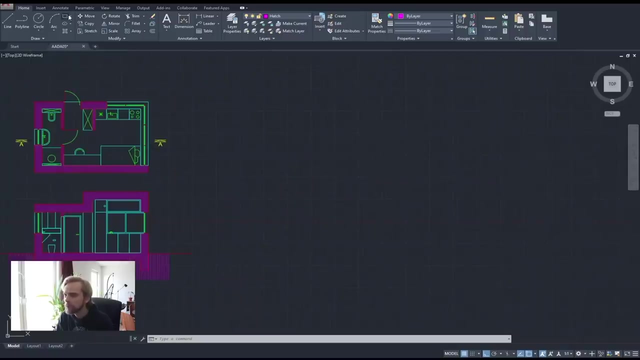 geometric view is basically a view from the top. Sometimes it's from three quarters of the top, but in this case we're just going to be using some weird angles, I guess, And a very fast example would be if I have a rectangle and I'll just draw it completely randomly. 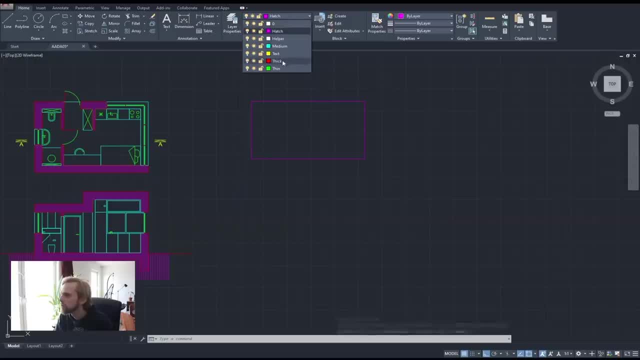 just some sort of random sized rectangle, And let me switch to thick line, just so that we're kind of consistent. Let's say, this rectangle represents the top of our shape, of our box, right? So if we look at the box from the top, it's a rectangle, right? So 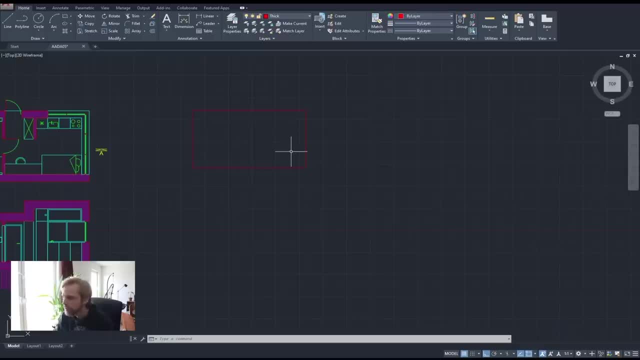 what if I want to show an axonometric view of it? Well, first thing that I do is I check what kind of angles I can use. So I can use 45 to 45 degree angles for the walls, or I can use 60 to 30 degrees. That's your view. 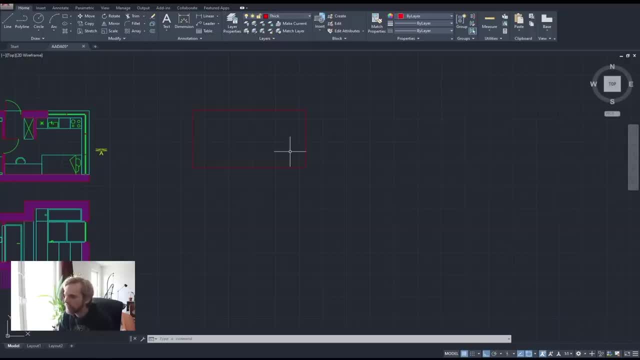 And that's usually thetypically. that's the angles that you use, So I will show you both of them. andyeah, I'll just show you both of those variations. So basically, for 45 degree angles, you can't really dolike. drawing them without any assistance is kind. 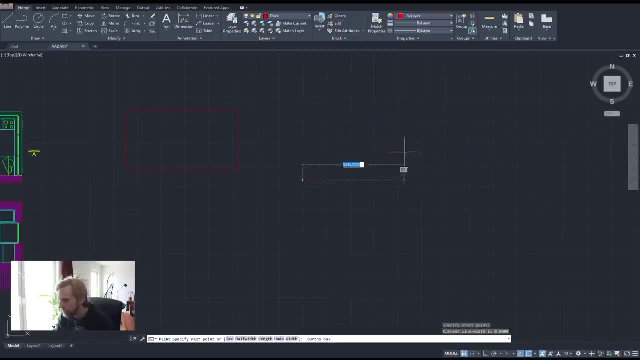 of tricky. Well, it's not tricky, It's just that you first need to draw it horizontally right, Some sort of a line, And then you need to rotate it every time by minus 45.. Well, that's the other way around. 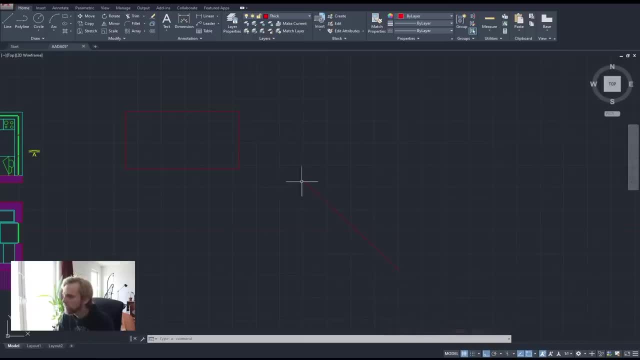 but you get what I mean. You know, to get a 45 degree angle, you just kind of draw the line horizontally and you rotate it. That's not nice. Instead, what we can do is we can use this polar tracking. This is the polar tracking widget, right here in the bottom. It's F10.. The shortcut is F10.. 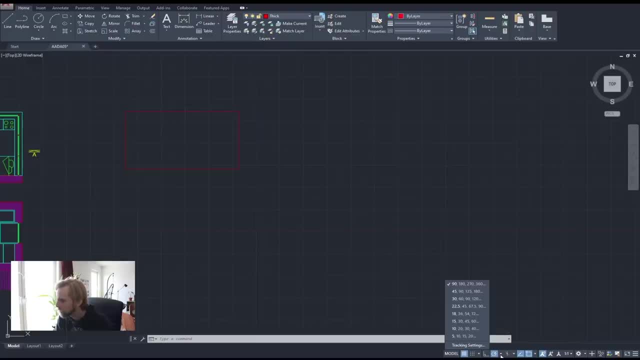 So I will enable it by clicking on it And also we can expand it And we can seeso. you can expand it by clicking this small triangular icon right here And once you expand it you can see the angles that it's going to let you choose, right. So it's basically in increments. 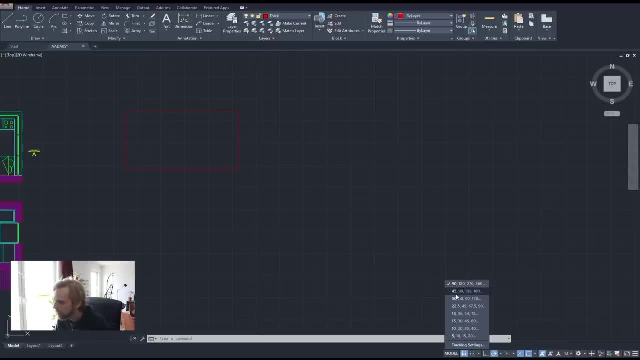 So you can have like 90-degree angles, You can have 45-degree increments, 30-degree increments, 25.5-degree increments and so on. So for an axo that is 45 to 45 degrees, I can use this 45-degree increment polar tracking. 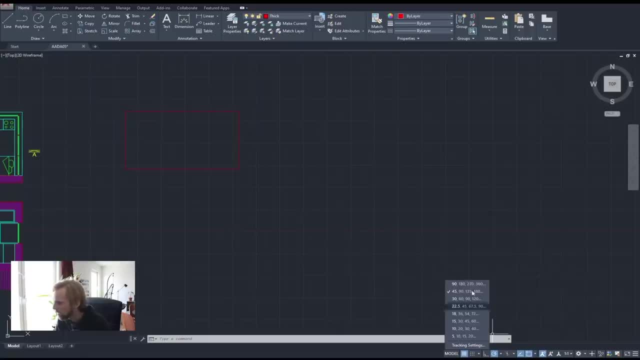 is it called? Yeah, polar tracking, So I will enable that. So now this is tick-marked, And now when I draw a line, it snaps To a direction of 45 degrees, which is great. So now let's draw this box in an axo. 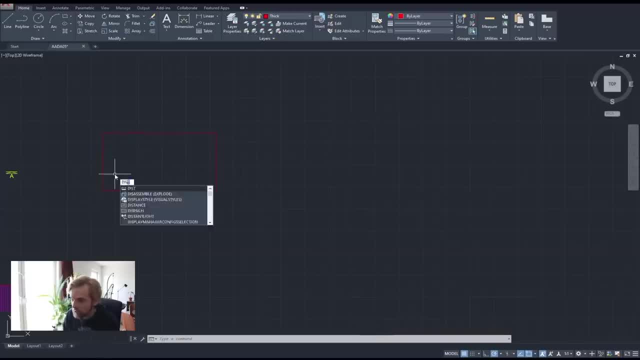 To do that I need to know these two measurements. So I'll just measure distance, Dist, Like that, And it's aroundI drew the box very randomly, So I will just say that it's around 6,000 millimeters, right. 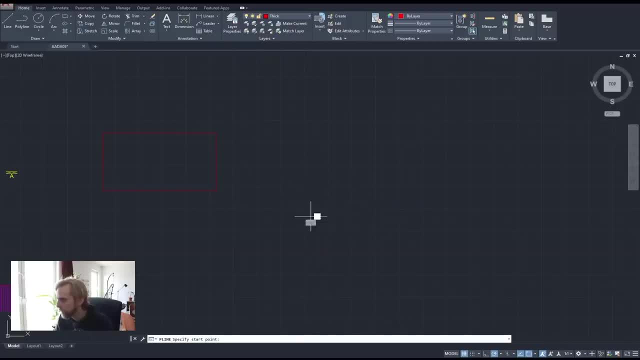 So then I just grab a polar Polar line or a line tool, doesn't matter, I'll just draw it at 45-degree angles as 6,000.. Enter, So that's my line. right, Then I will measure the other wall like so. 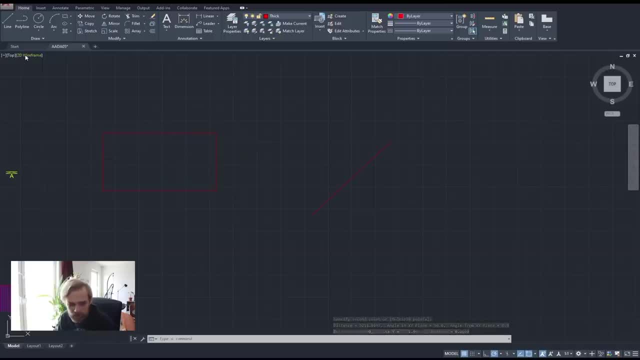 And I see that it's 3,251.. So let's say 3,250 millimeters. I'll grab a polar line tool again. I'll just draw it out like so: 3,250.. Right Enter, That's it. 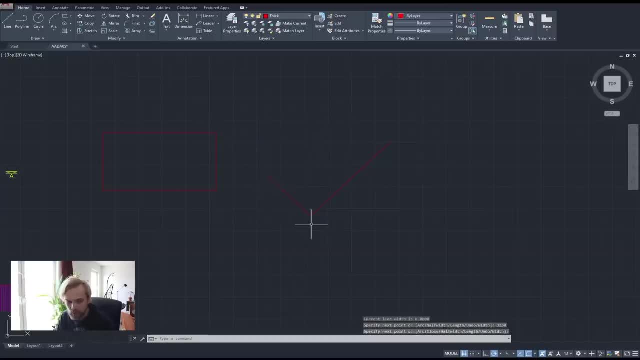 We have the two lines, and these two lines are going to be enough for me to finish up drawing this particular box, Because now what I can do is I can copy this line from its base point here to the base point here, And you can see that I missed. 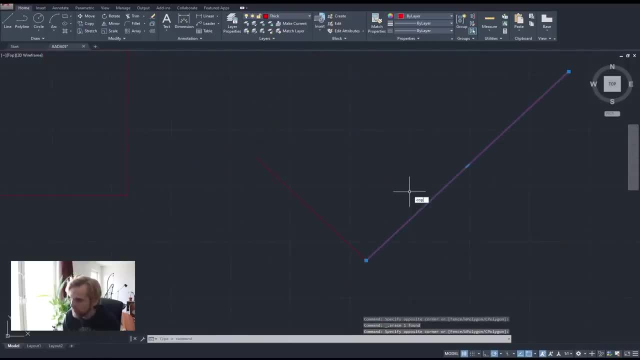 So I'll do that again: Select it, Copy From here to here. There we go. That's much better. And then I will select the other line: copy from its base point here to the base point here. That's about it, right. 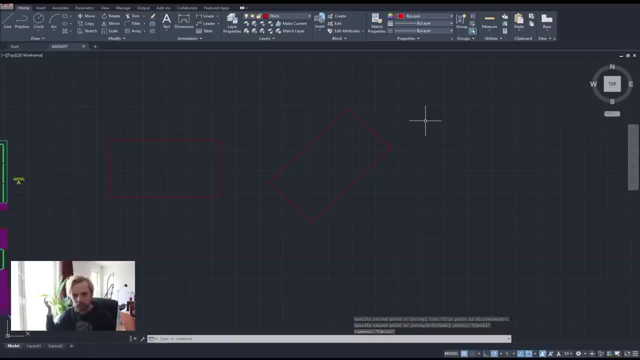 Now we have our 45-degree angle. Okay, So we have our 45-degree angle of the top of the box, But of course, in an axonometry you can see it as a three-dimensional object. So let's say, the height of this box is 3 meters. 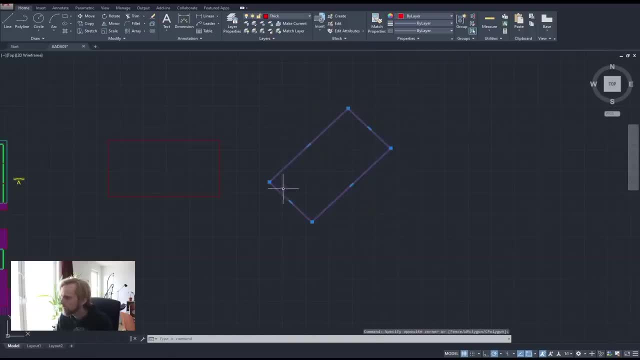 3,000 millimeters. So what I like doing is I like selecting the- Let's say, this is the roof, right. I like selecting the roof plane and copying it. Copy And I'll just copy it from top to bottom. 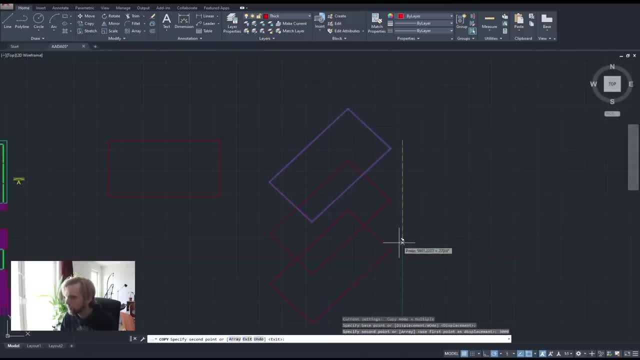 Like so, and I'll just type in 3000 millimeters right And hit escape. So then I have the bottom of the box as well. Now all I need to do is just some additional lines for verticals and clean it up right. 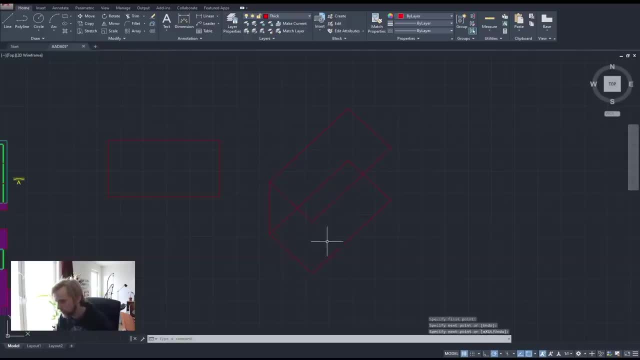 So I'll just draw those lines like so, like so and like so, And then trim, enter, enter and get rid of everything that we don't need, Don't need that, Don't need that. That's it. That's the 45 degree axle right. 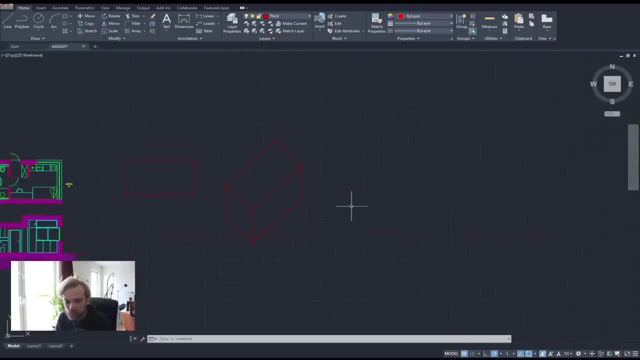 30, 60 degree axle or ISO view would look like this. Well, first of all, I need to change the polar snapping, polar tracking to 30 degree increments, of course, And then I kind of do the same thing. So I remember that this is 60 or 60. 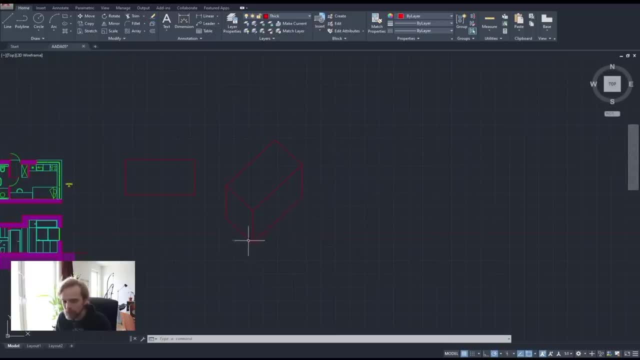 This is 6000 millimeters and this is 3250 millimeters. So let me do this: I will find a 30 degree angle right here and I'll say 6000, like, so. I will then find the 60 degree angle here and I'll say 3250, like, so. 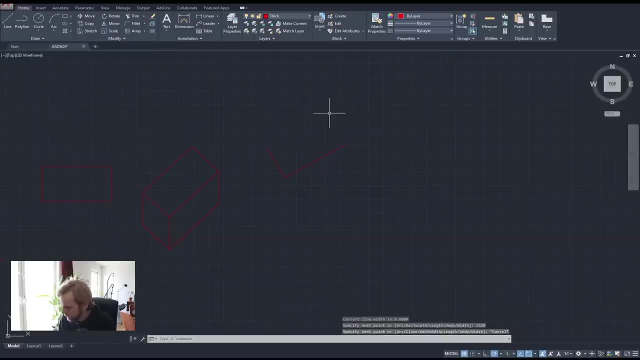 Actually, I can kind of continue drawing it this way, or let's stick to it. I'll copy right. So the procedure is exactly the same. Copy like that: The height doesn't change of course. 3000, like that. 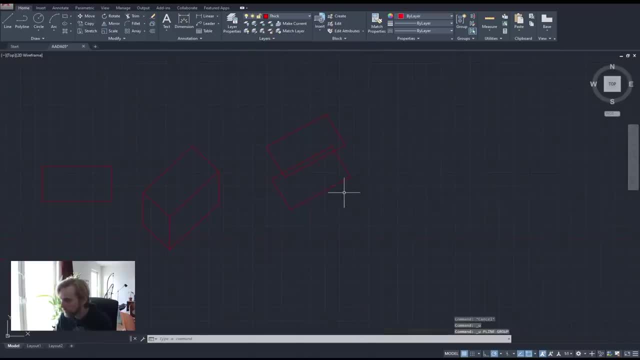 Hmm, I accidentally moved it, I guess, in the incorrect way. Copy: Please move downwards 3000, enter. Yeah, now it's good. Three lines, Bam bam bam. Those three lines are done, And now, or just trim, enter, enter. 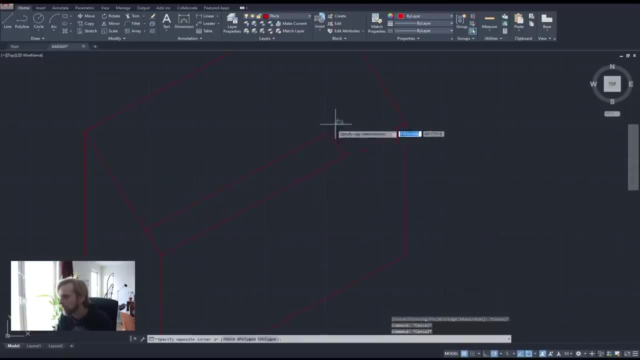 Get rid of that. Get rid of that and delete those two. There we go. So that's a 30, 60 degree angle Right, Very simple. Let's do this with our, with our uh, building um, so I will say that I want to, I want to. 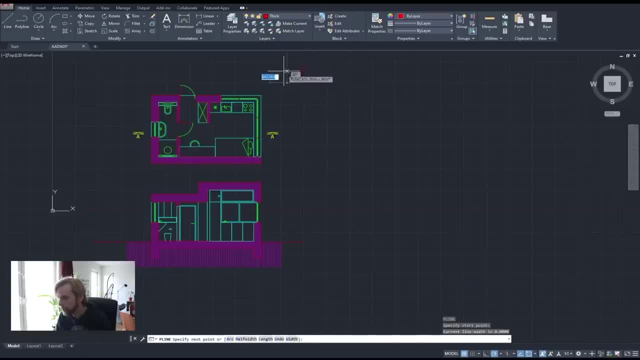 kind of look at it, maybe from this point on. I don't know. Well, if we look at it from this point on, it's it's going to be the the large roof and then the small roof. Maybe that's fine. 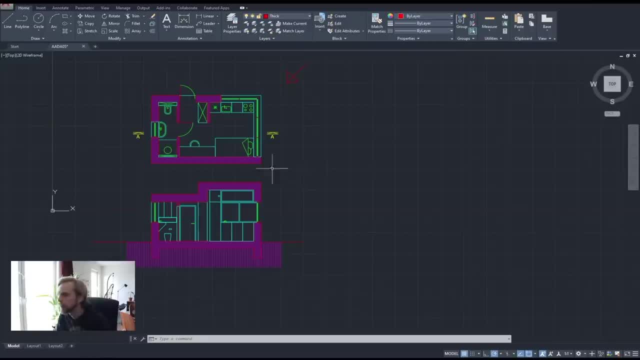 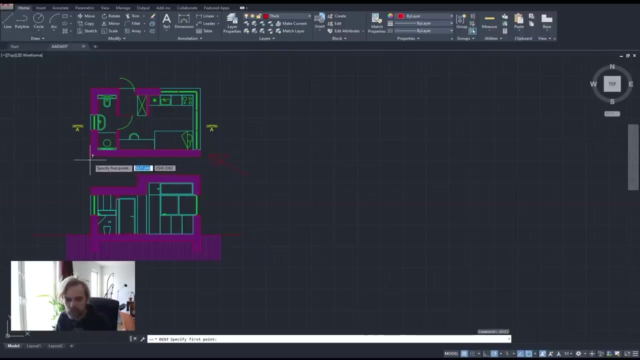 Hmm, Okay, Or maybe we can. yeah, let's look at it actually from from here, from this point, right, Like so. So I will uh measure distance and I'll do it 30,, 60, uh measure distance. 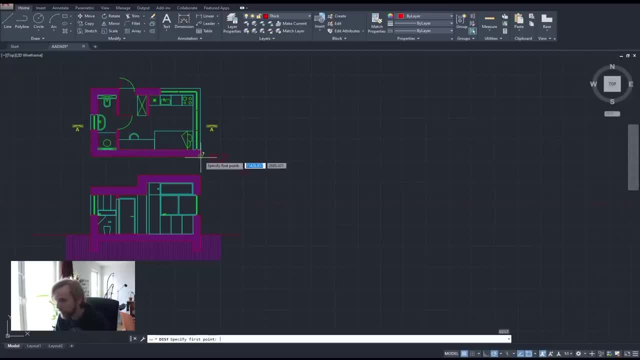 So that's 6,000 millimeters in length And of course the width is going to be 4,000 millimeters, like that, or thousand. So I will just grab a polo line tool and just draw it out like so and I'll say 6,000 in. 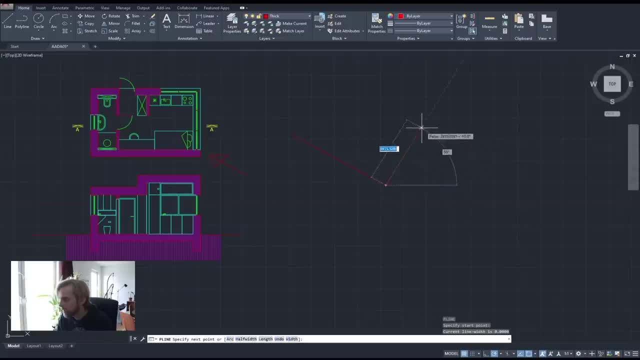 this length. Uh oh, there, we go 4,000 along this line. So, um, make a copy, Bam, Okay, Okay. So I'm going to make and then basically close it off, right? So let's say, this is like the, the footprint of of my building, right? 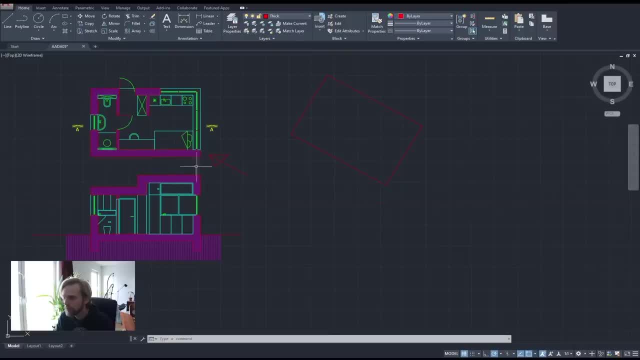 So this is uh this edge right here around my building, then I need to know the height, uh the height of it. And here I kind of have, um, how do we do this? Yeah, Let let's uh draw it from the ground. 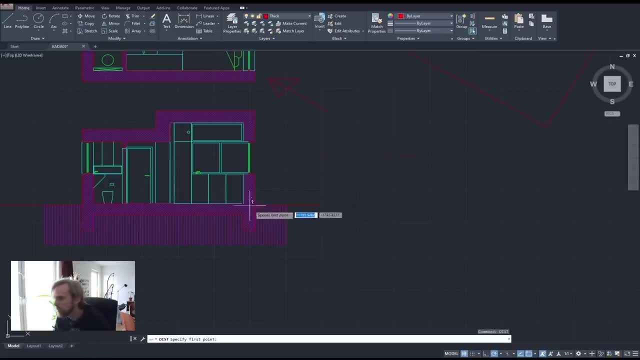 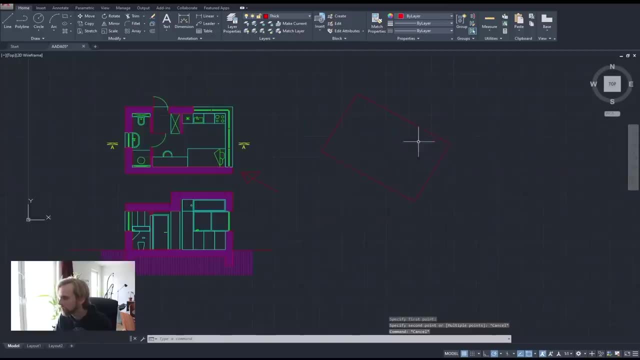 Yeah, That that makes sense, So I'll I'll do distance. Um, sorry about this. Um, I do want to actually select this, join this up right, And I want to first take the floor slab and move it up to the correct height. 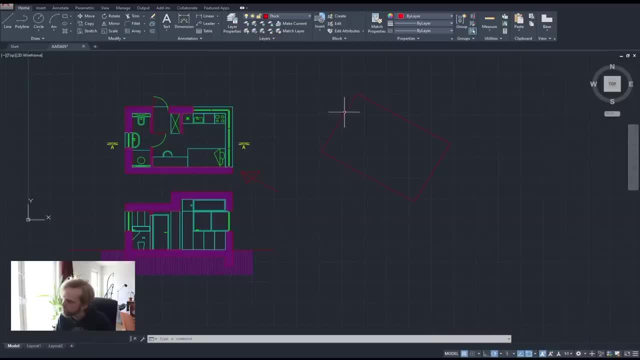 Right, Uh, just like I did with the box: In the case of the box, I moved it down. In this case, I'm moving it up. It's the same procedure, basically, So I'll just measure distance. Okay, Uh, from here to the top here. 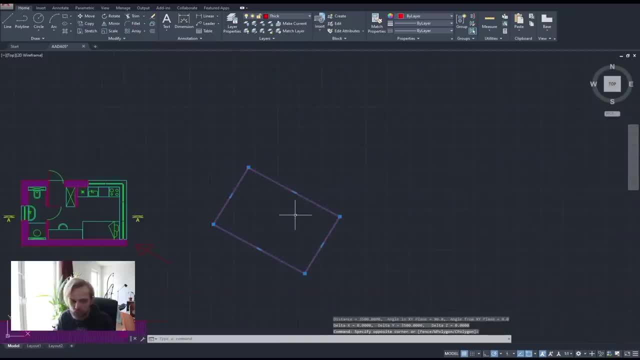 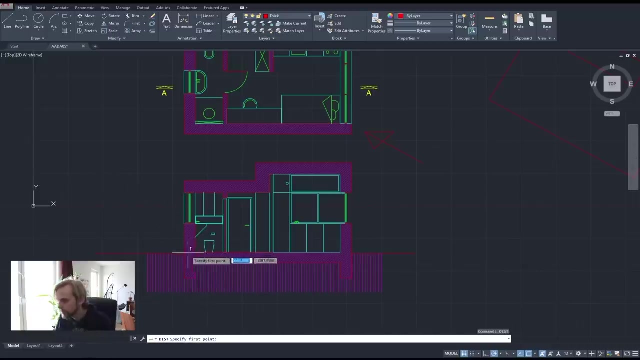 And I can see the distance is 3,500, right. So I'll just take this copy up, 3,500, like that, And then I'm going to measure distance here. Distance from here to here, That is 2,800, right. 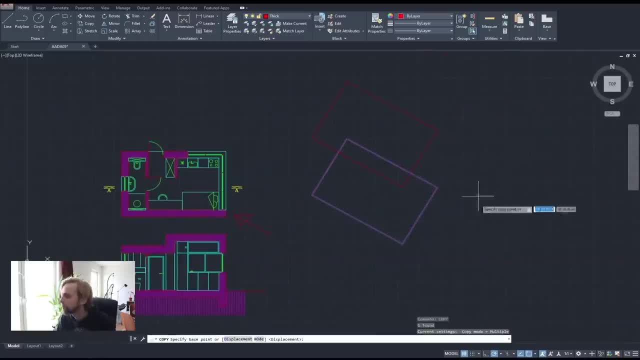 So I'm just going to measure. I was going to make another copy up 2,800.. There we go, Right, So now I have all of the levels that I that I will need for my axle and I can start connecting them. 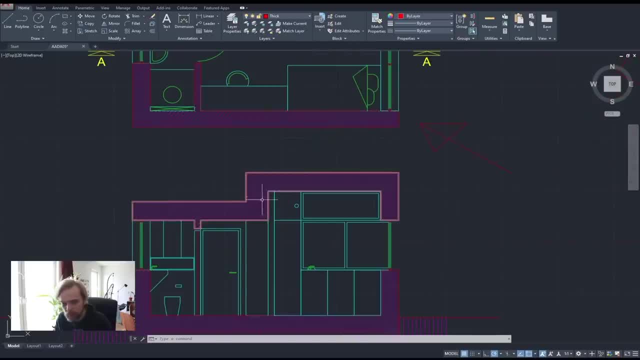 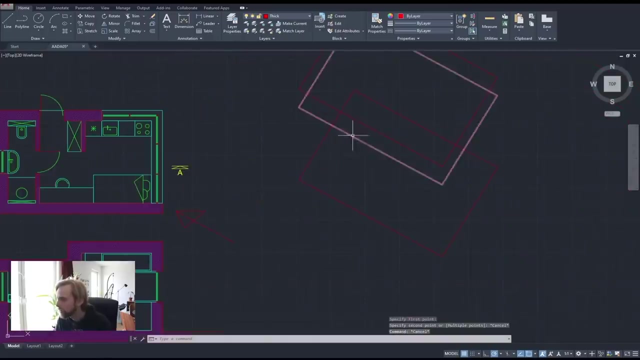 Um, before I begin that hiccup right here, I need to know where that hiccup happens. right, The change in the height. So I'll measure distance again from here to here: 2,560. Okay, Sure, So along this line, if I grab a polyline tool along this line it's going to be 2,560. 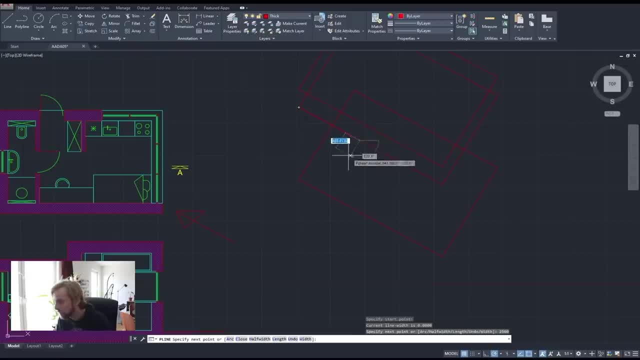 millimeters Enter. Actually, let me extend it. So I just have this polyline as a helper, and I know that this- oh, I messed it up, Let's do this again: 2,560, right, Or 2,650. 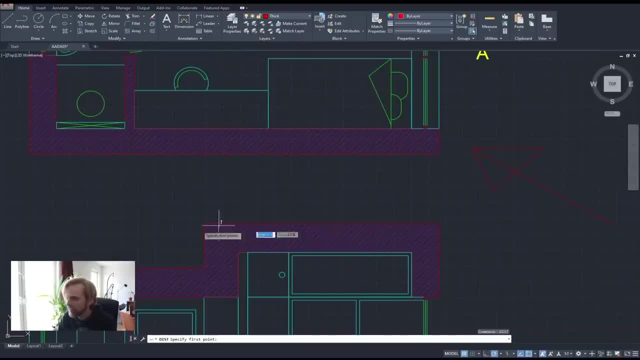 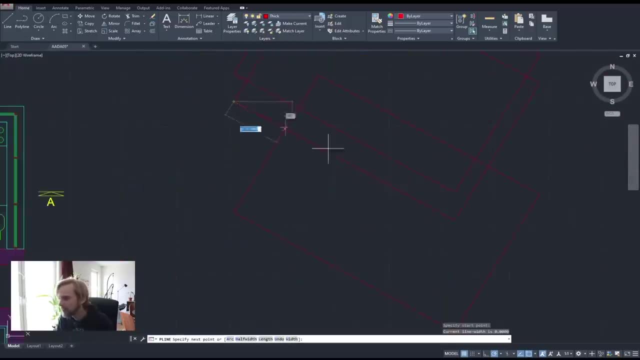 Oh my God, Distance: 2,560.. Okay, From here to here: 2,560.. Come on, Come on, Just 2,560.. Enter. Did you snap properly this time? Yes, you did, Okay, Good. 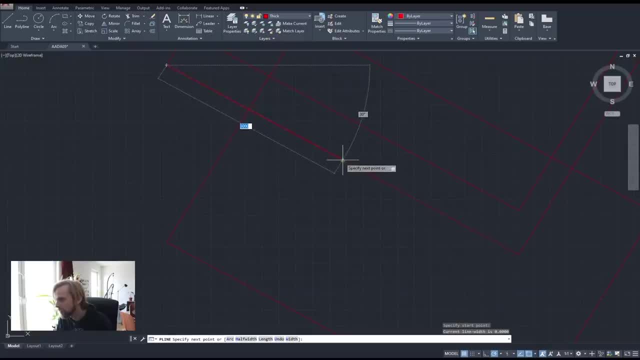 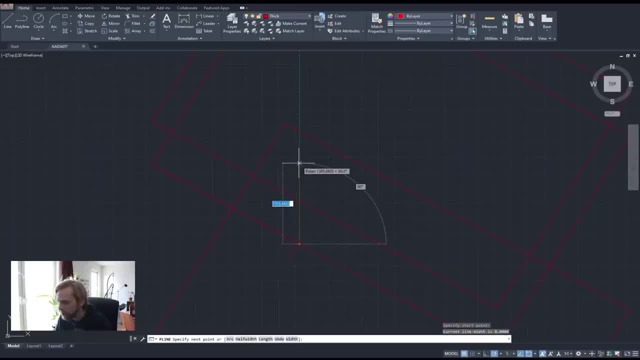 So I have that point here and now I can just draw that point up, Draw a line from that point up. The height of the line doesn't matter, because I can just always select things that I don't need. So, for instance, I don't need this anymore and I can delete it, and I can also trim enter. 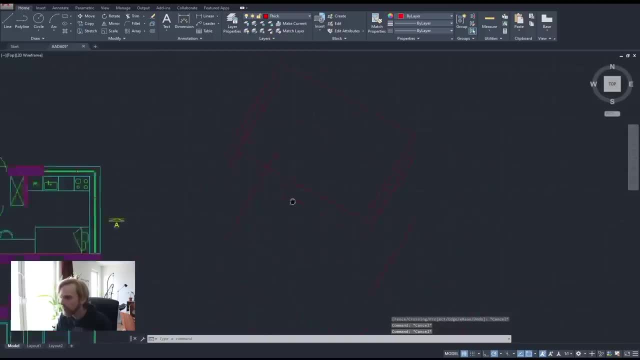 enter and trim away the excess Right. So I have basically what I've done is I created this hiccup line right here And I know that with this hiccup line, the top of the roof ends, the highest roof it ends. 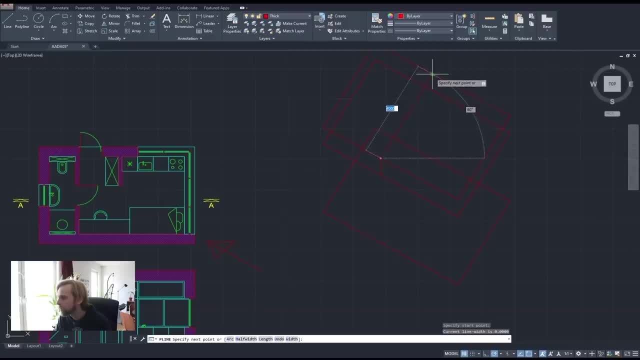 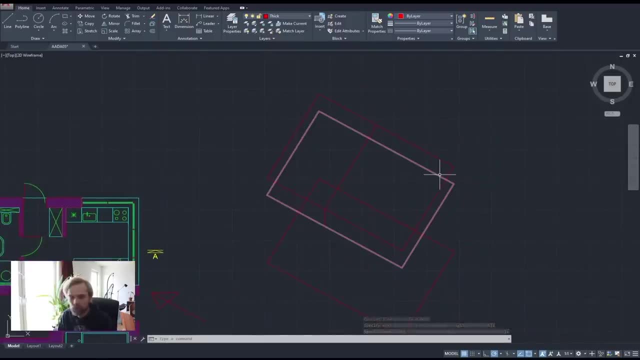 So I'll just grab a polo line tool and I'll just draw it out like so, Or I could just take this line and copy it, and that works as well. Okay, So now it doesn't look like much, but once I start cleaning it up, it will start taking. 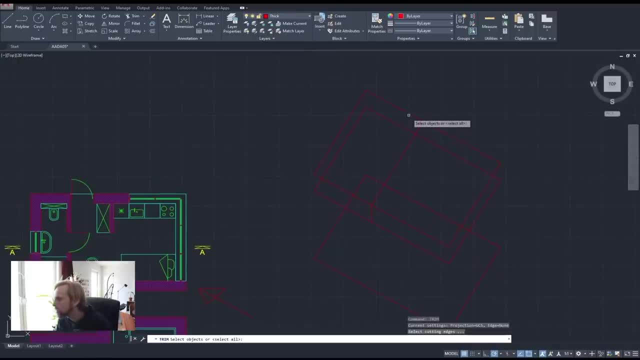 shape. So I'll do exactly that: I'll trim and I'll trim away, enter this area right here, this, this, this and also this Right. So that now is the top of my roof and that is the bottom of my roof. 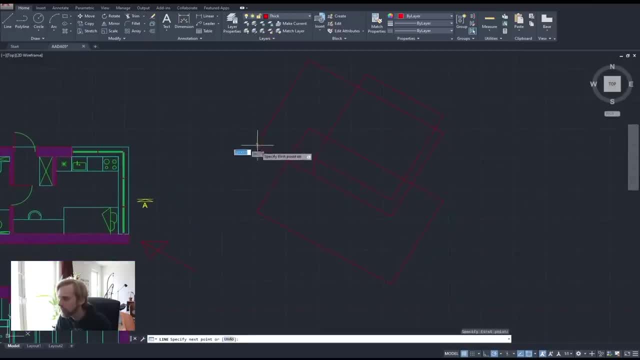 And I can basically connect everything with vertical lines. So there's going to be a vertical line here, There's going to be a vertical line here and the vertical line here. That's, that's all I need to do. And now it's just cleaning it, cleaning everything up. 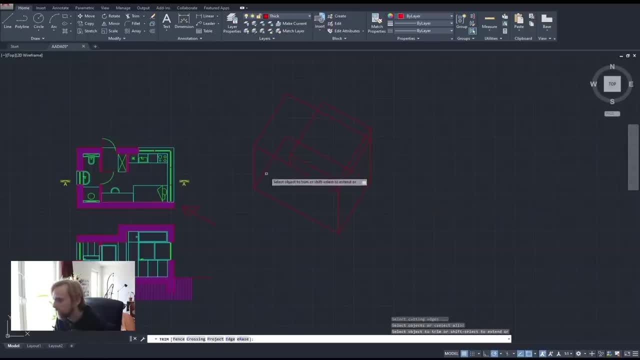 Right, So trim again, enter, enter and get rid of all of the unnecessary bits. Construction workers behind the glass Hope you don't hear them. Let's do that. All of the unnecessary bits and pieces that we don't need, we just trim away. 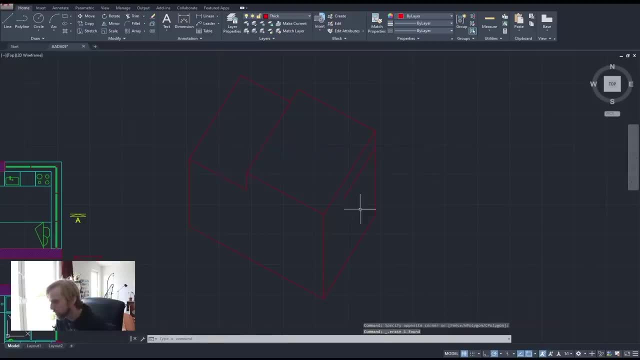 And I can see that I can just delete that zigzag here, So I'll just kind of delete it, Right? So that's the shape, That's the shape of, of, of the beautiful building, Right, Wonderful, Let's continue. 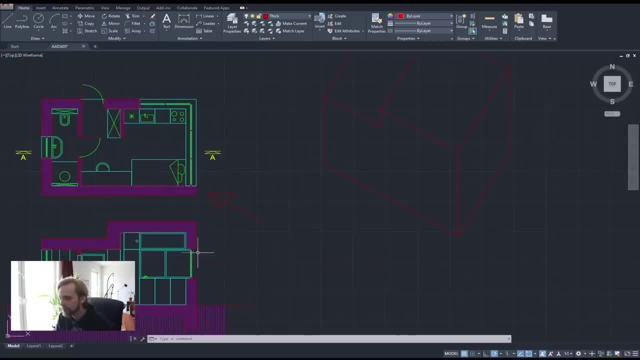 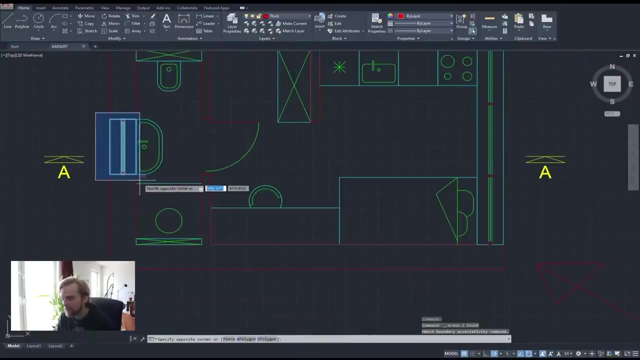 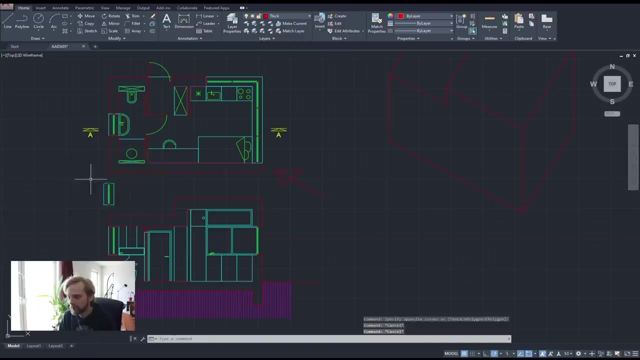 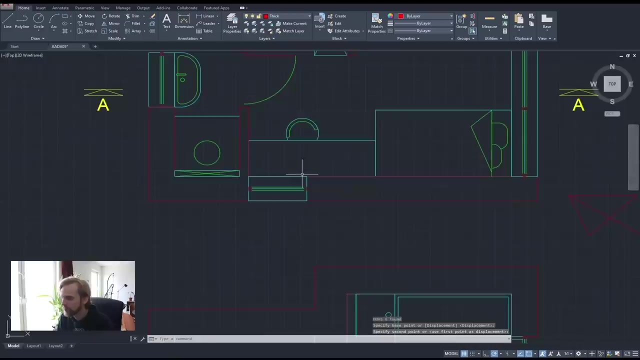 So what I want to add now is this: Well, that's actually a very boring facade. Let me do this real fast. Let's grab. grab this Copy, Rotate, Come on, Rotate And just create some sort of opening at least. 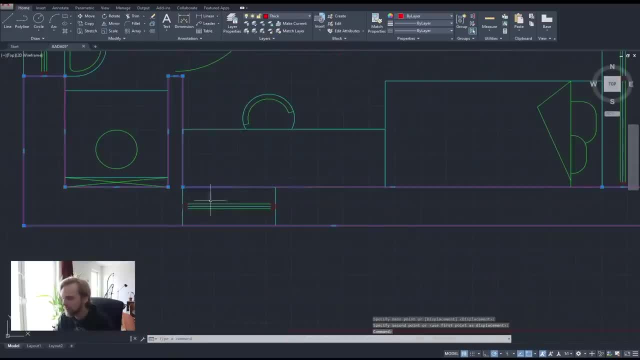 Right Somewhere here, And then, of course, I need to clean this up. So I'm just going to make, I'm just going to hide the medium lines for now, Or rather, first I'll create two thick lines here: Here and here. 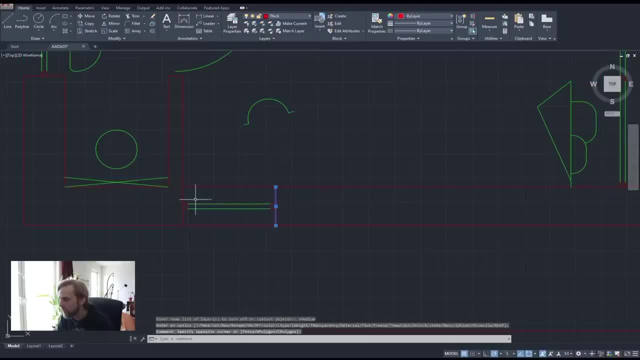 Turn off the medium layer. Select these two lines. Trim Delete, Join everything up here And also join this. Join Okay, This is closed. This is closed, Perfect, Okay. So now we can. we can actually turn on the medium layer. 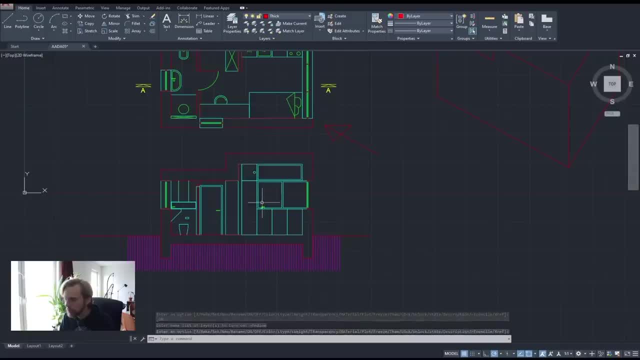 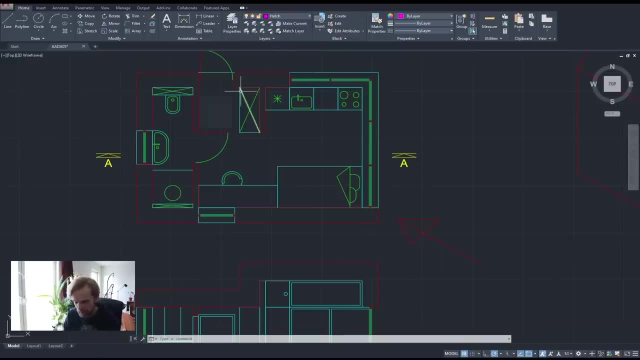 And now we have additional window here Which will not show up in the section, But we we don't care. I deleted the hatch, So I'll reinstate the hatch. That's going to be that pattern. I believe I used 20 for the scale. 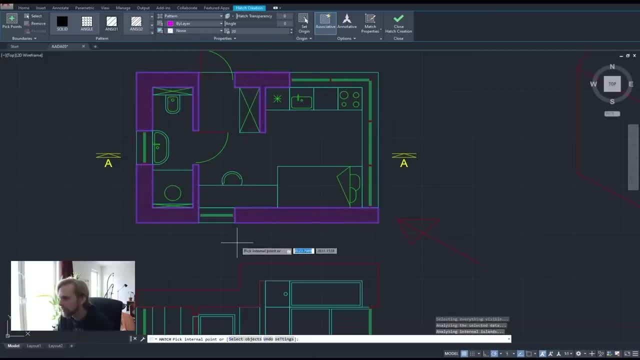 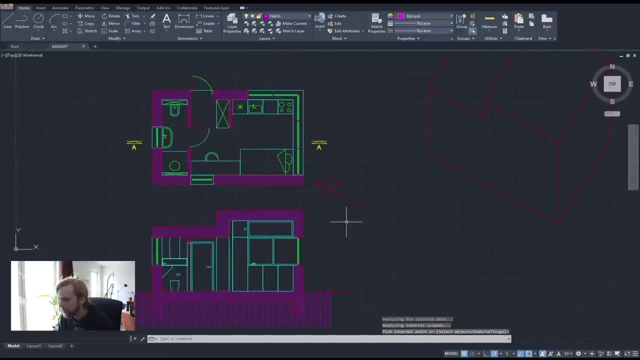 Yeah, Looks like it. I'll just click inside of the walls where I want the hatch to be. There we go. That is done. Enter: Okay, So we do have a window here now, So it's not going to be that boring. 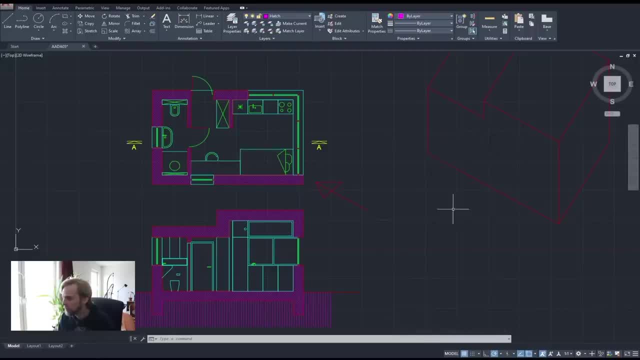 At least, I kind of want to now cut a hole, Cut a hole out for this window And also, of course, for this window. So the first thing is, I need to know what's the height at which the windows are going to be located. 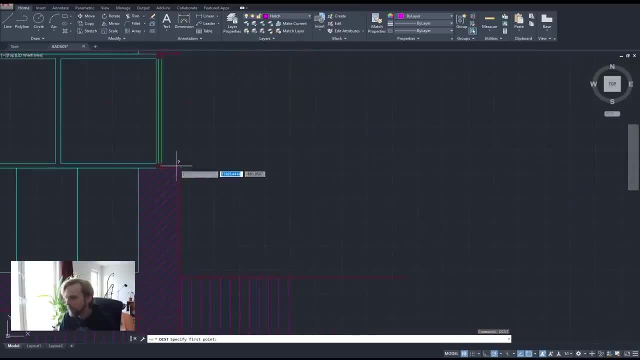 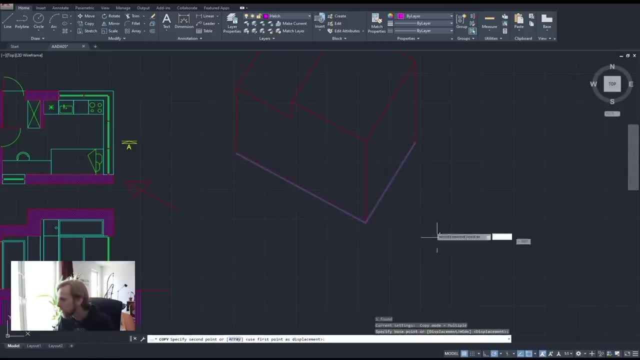 And actually both of their height is going to be the same. It's going to be 1150 millimeters above the ground line, This line right here. So I'm just going to take this polyline, I'll copy it Up By 1150.. 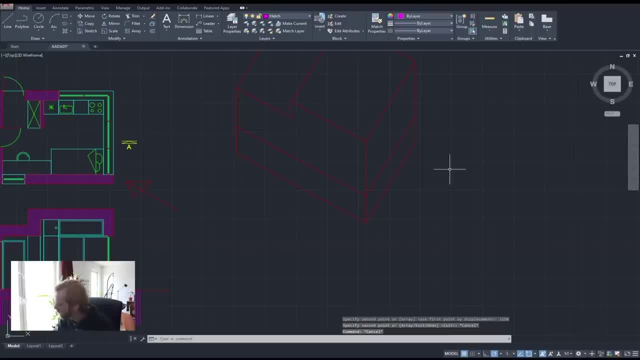 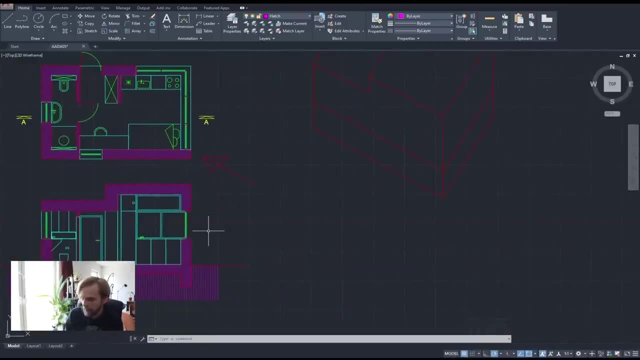 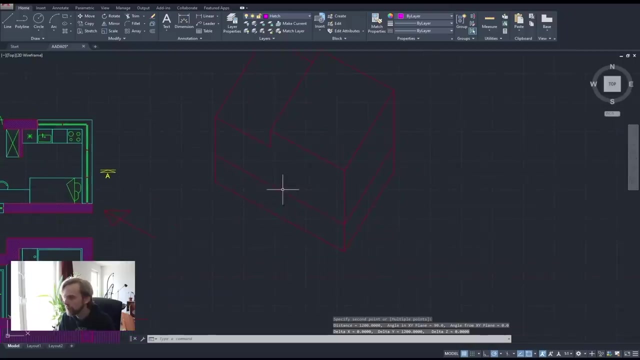 Enter. Okay, So that is the bottom of the window And the top of the window. I can just measure the distance again. So my window height is 1.2 meters. So I'll just take this line again. Copy Up. 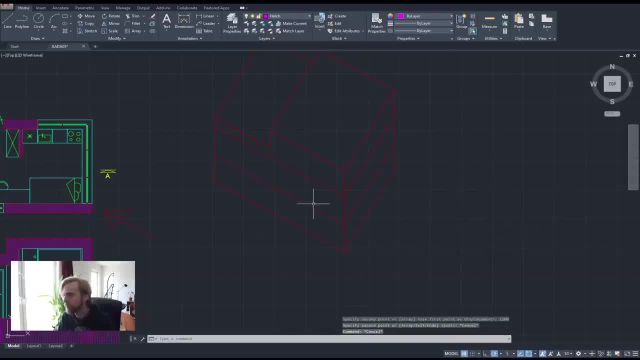 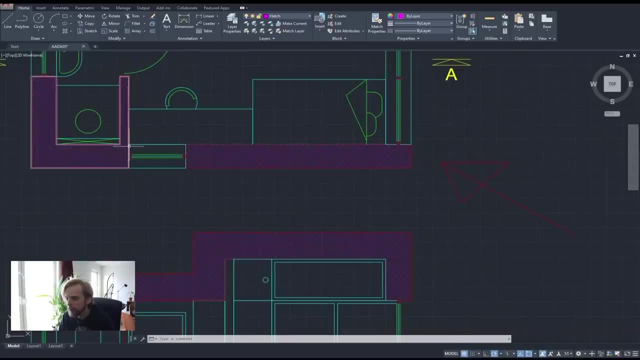 1200.. Enter, Right, That's it At the top of my windows. Now I need to know where this edge is And also where this edge is Right, So I'll just measure distance From the end of the wall. 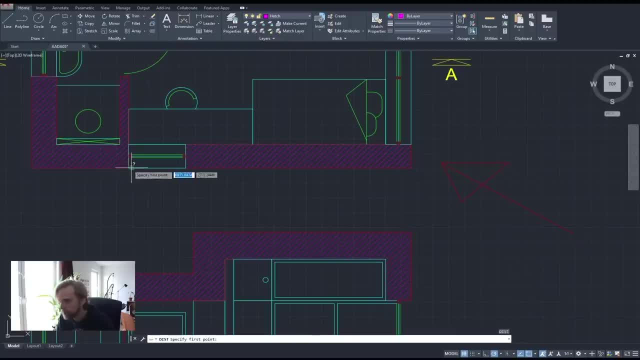 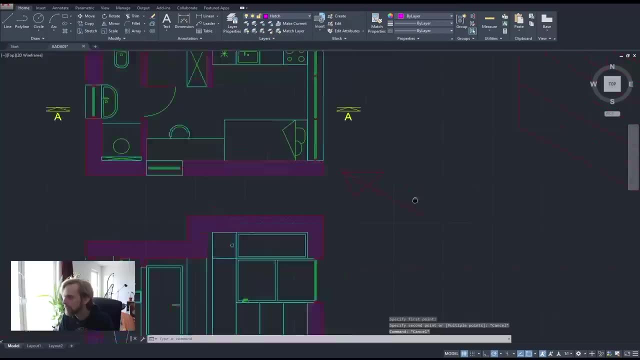 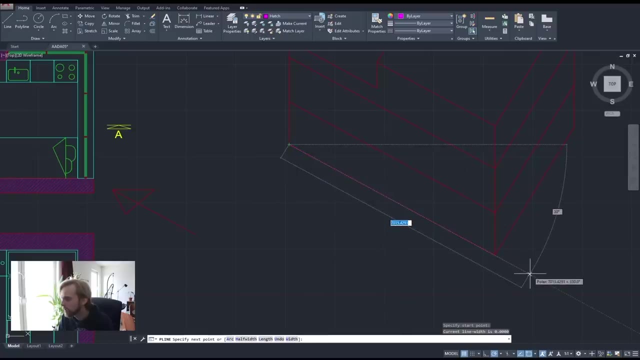 1540.. And then it's going to be another one of 900.. 1540.. 900.. Okay, Let's do it this way: Polyline, To make sure that you're just drawing a polyline In that particular direction. 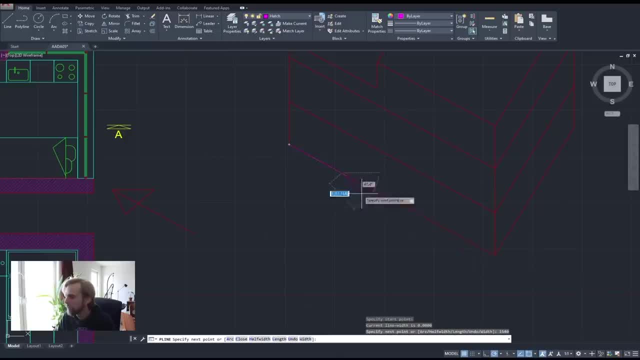 And 1540.. We're doing 1540 here And just Honestly just drag it out, Yeah. So basically we have this kind of L shape. I like using it this way As my helper lines. Actually, I should probably like have these lines. 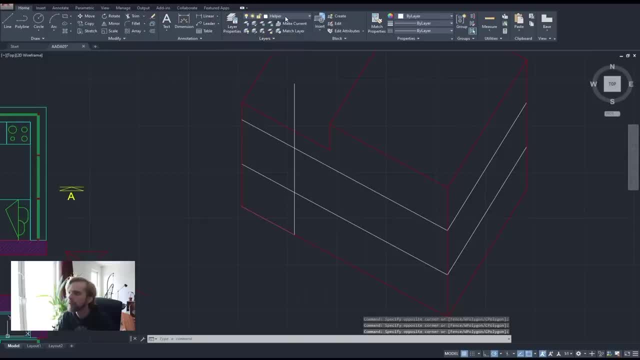 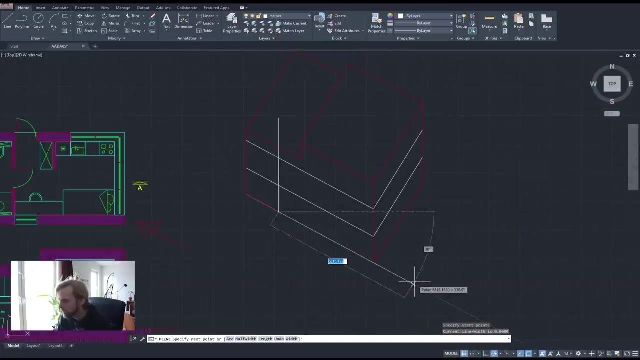 Just to be more pedagogical In the helper layer, Because these are just my Helper lines And I'll make my helper layer active as well. We continue, So I just grab this. I start drawing from this point Along this direction. 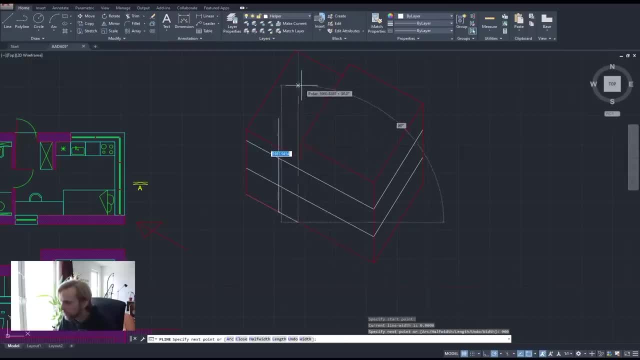 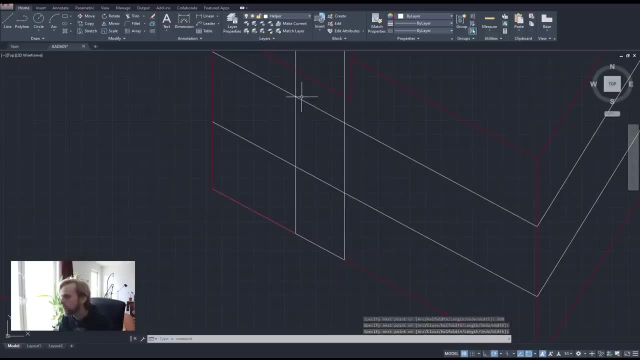 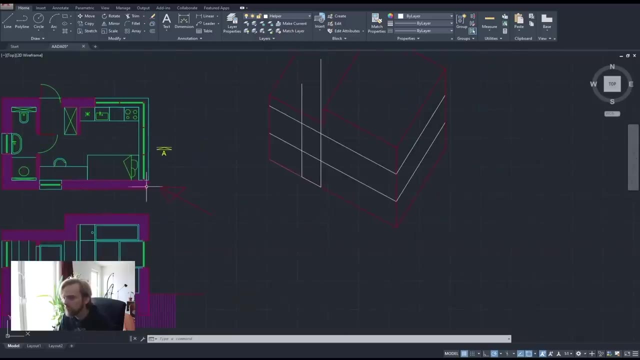 And I will say 900.. Because that's the width of my window. Like so Right, Like so So. this rectangle right here Is where my window Is going to be Located in the axle. Same thing for here, But for here it's going to be quite simple. 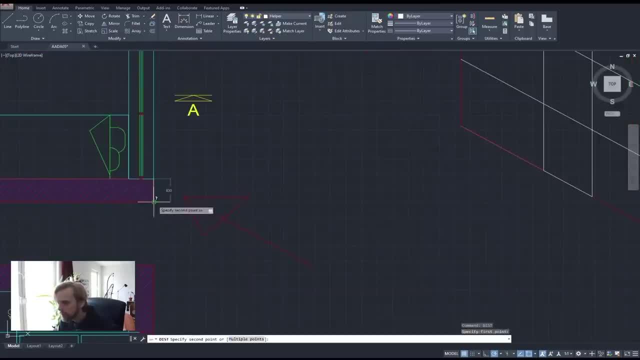 I just measure the distance From here to here. That's 400. Of course, And I can just take this Vertical line here And just make a copy of it Along this edge, So I'll just snap somewhere to this edge. 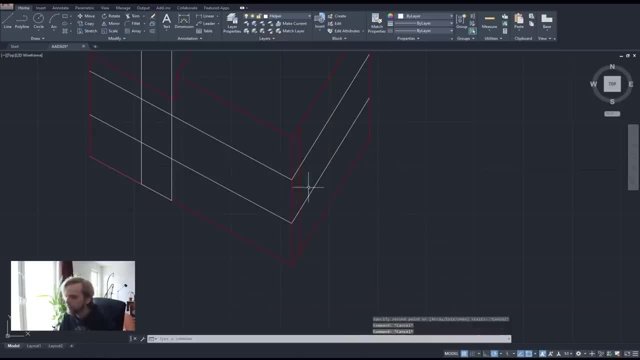 And type in 400. And that makes it into, Makes it into a copy. Okay, Let's Clean this up again, Right? So I will just grab the thick line tool And I'll just grab a polar line tool. 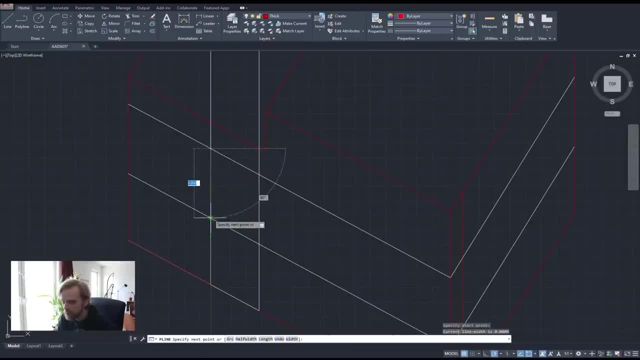 And here, Just make sure that intersection Snapping is turned on. Intersection That it's turned on, And I will, And I will just draw out this Twisted rectangle here, Or projected rectangle here. That's the hole for my window. 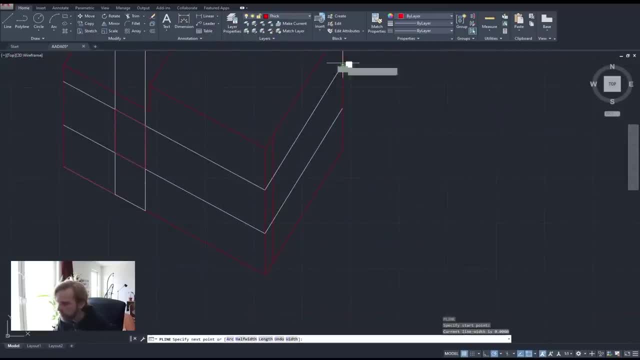 And I'll do the same thing here, Only that it's a corner window, So it's going to be a U shape Rather than a rectangle Like that. This Right And now. I don't need the helper lines anymore, So I just delete them. 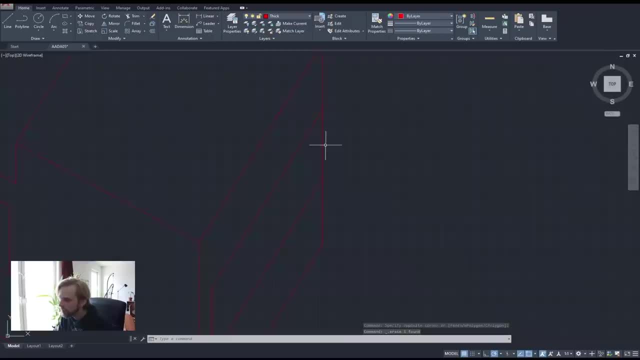 There we go, This line right here. Line segment right here Is not necessary, So I'll just trim, Enter, Enter And trim it away. Okay, So now to be Pedagogical, I need to give thickness to this. 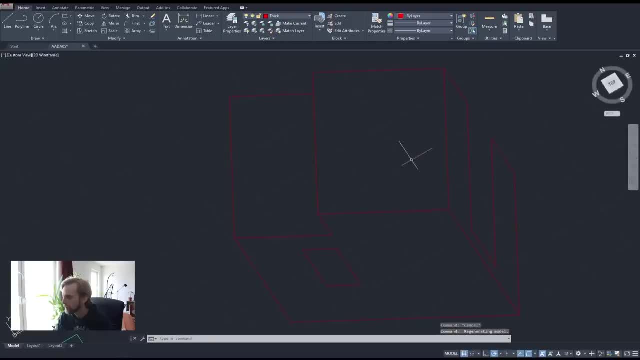 Right, Of course I need to give. By the way, If you do this Accidentally, Like if you accidentally rotate The The view, Just click on the Top Top right corner Box Right here, And then click on the arrow. 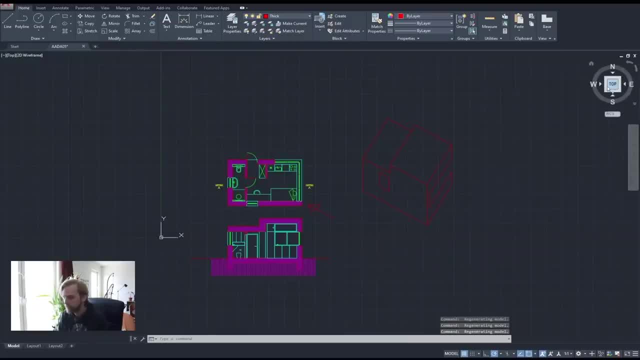 Keys, Like Here, To rotate it back. So that's top is. You know Where you want it to be, Right? Continuing on Thickness. So To give it thickness, All I need to do Is just draw out a line segment here. 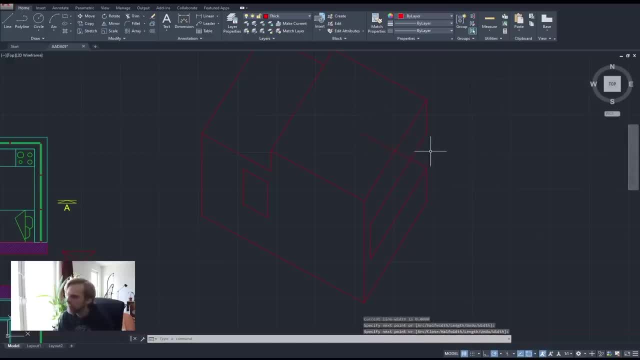 Of course, And, As you can see, I always Tend to draw out line segments That are Too thick, And then I just simply trim it, Trim them back To The thickness That I want, Right, And 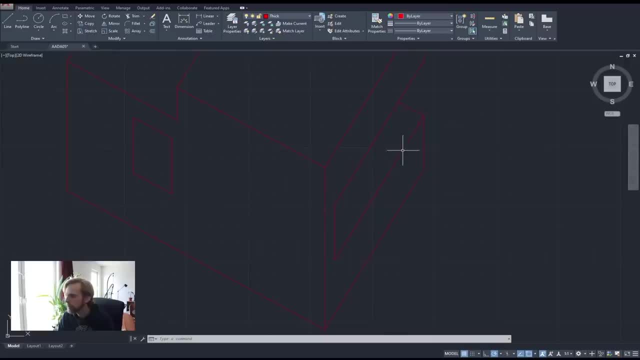 The thickness Of the wall Is 400 millimeters- I don't even need to check that- So I know that This line Will go in By 400.. Well, Actually, What we can do, Hmm. 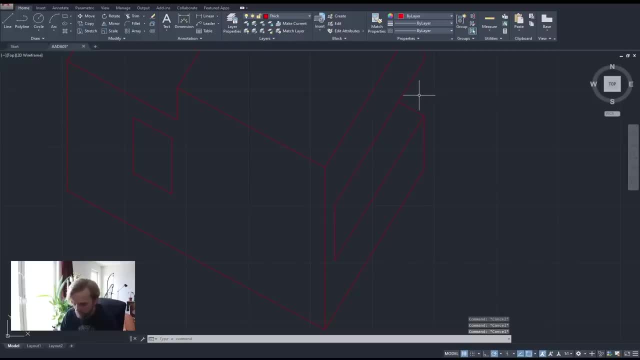 No, Let's do it The old fashioned way: Copy Or Offset. Offset Would work as well. Offset: 400.. From here To here, That's 400. And then Draw Just a line segment. 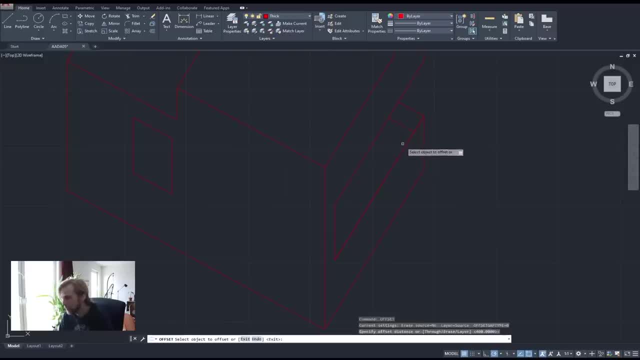 Here: Offset That line segment By 400.. In words Like So: And Delete The Original, Of course Trimming Again. Enter, There We Go. There We Go, Okay. 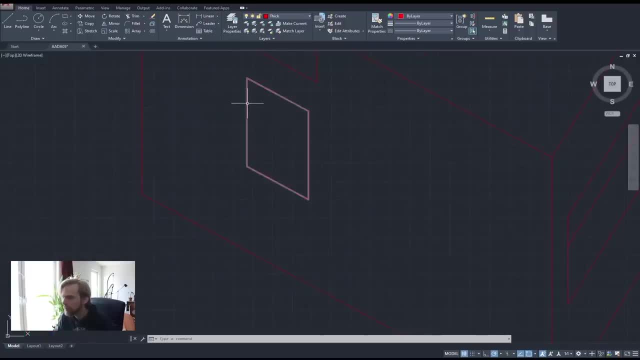 So We Have This Line Here And There's Also Going To Be Thickness Of The Wall Here. But In This Case I'm Going To Be 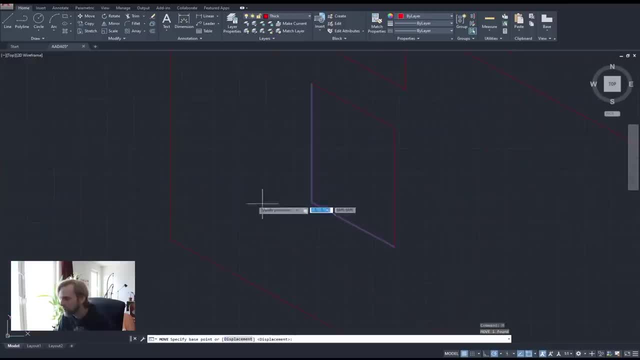 A Little. Keep Holding uh along the 30 degree direction, right by 400 millimeters, like so: trim, enter, enter, trim away the excess, grab the polar line tool, extend it. you have your opening here, right, okay, so there's no windows. uh, let's add windows, of course. so the windows are going. 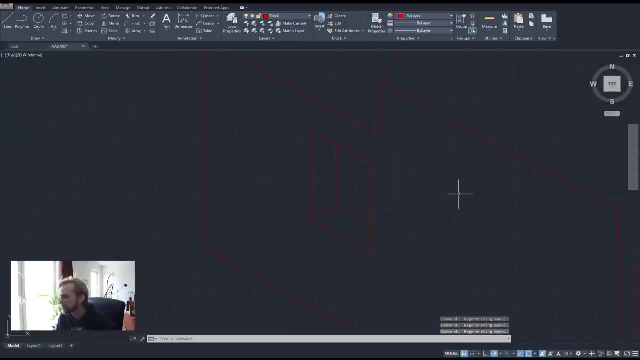 i keep doing it. um, the windows are going to be, uh, located, let's say, in the middle, or? or actually do i want them in the middle? maybe i do. let's say, the windows are going to be located kind of in the middle of the of the wall, right, so i'm. 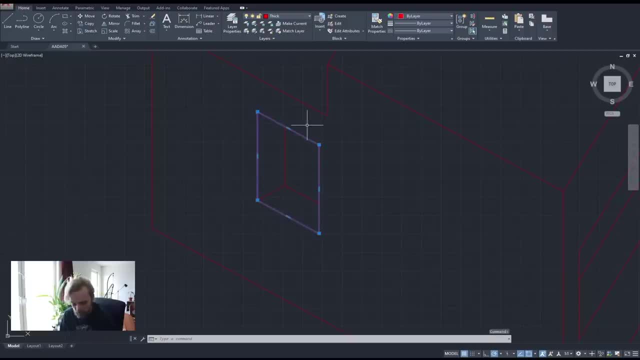 just going to take um this polar line that i already have and i'll copy it from this corner to the middle, middle corner here and that is going to be my initial window or window plane. right, Then I will offset by 50, because I remember that my thickness of the window frame is 50 millimeters. Offset it. 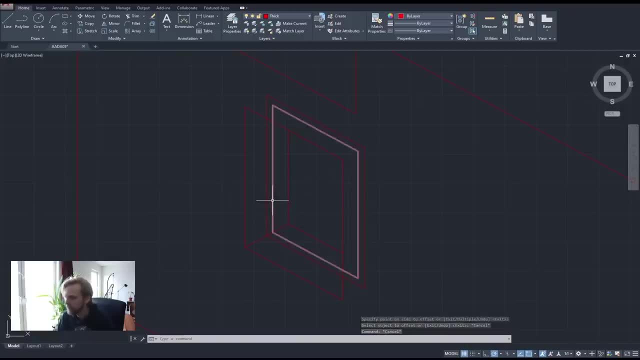 by 50 and just copy it inwards by, I don't know, 25,, 25, something like that, And now it's just a bunch of cleaning up, right? So the more curves you have, the more you need to think what you're. 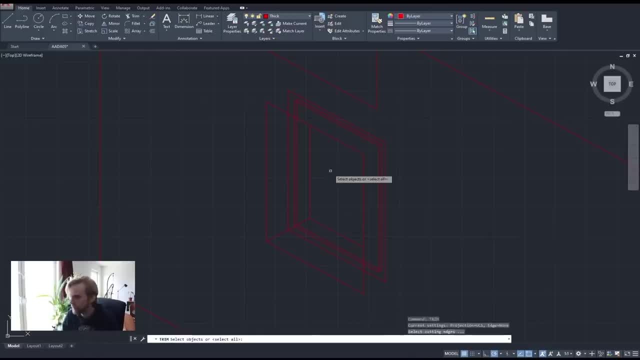 cleaning up, But it's basically going to be. if I trim enter, of course, I don't see anything. that's going on here. That's gone. I will not through the window, technically, since it's glass, you would see that. 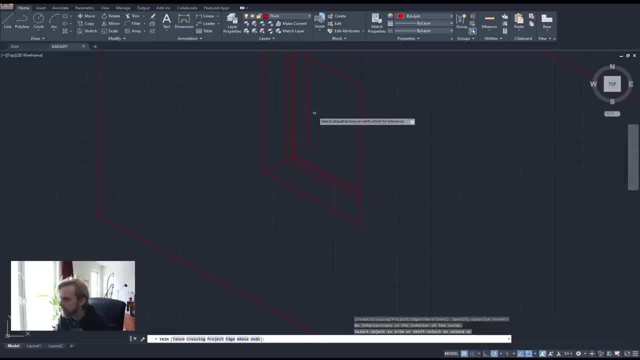 the backside of the wall. but in this case we don't want to show it, So I'm not going to be showing it, And that is basically it. Then I just delete the excess And then we have wall window frame and glass. right, So we have our window here. Same thing for this bad boy. 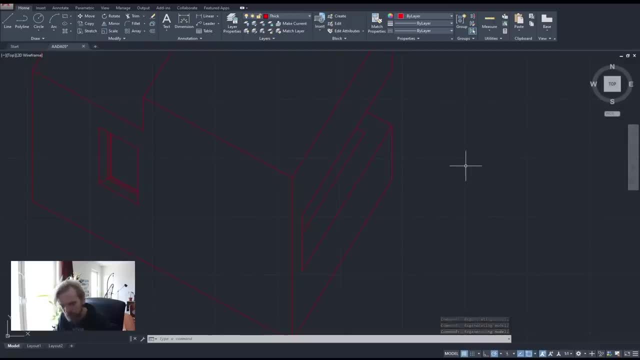 right here. Why am I doing this? I think this is because in Rhino, the shortcut is holding down the shift key to pan the view, So I think that's why I'm doing it. Anyway, In this case it's exactly exactly the same procedure, only that I'm going to draw a polo line. 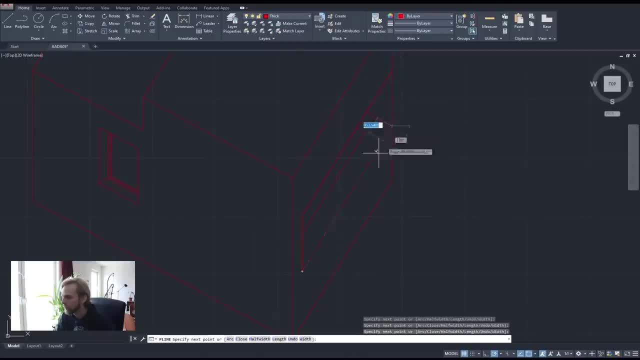 like. so Let me make it white helper line layer. So I'll just draw it as a white polo line so that it's easier for you to see. Make a polo line, copy it in. I will just make a copy of it, Or rather I can just move it, actually Move it inside of the 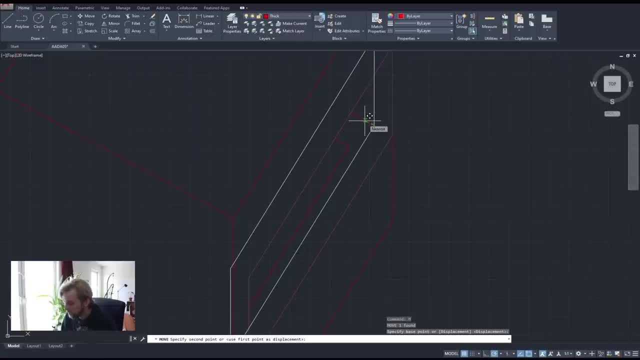 hole by. so that's going to be middle of the wall. That will need to be 400.. No, the wall thickness is 400.. So that's going to be 200 millimeters, something like that. So now it's moved in And of course it makes a bend here, right. So I can't have that line just located here. 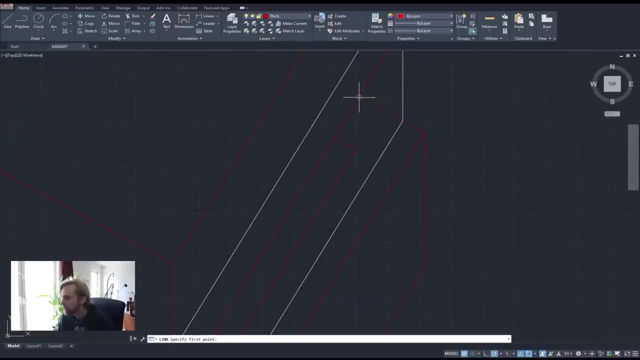 It needs to go in And the way it's going to go in, like the way I'm going to find that point, by how much this edge needs to go in. I'm talking about this corner and this frame right here. See how it's going in. It's not, you know. resting on this side of the wall. See how it's going in. It's not, you know. resting on this side of the wall. See how it's going in. It's not, you know. resting on this side of the wall. 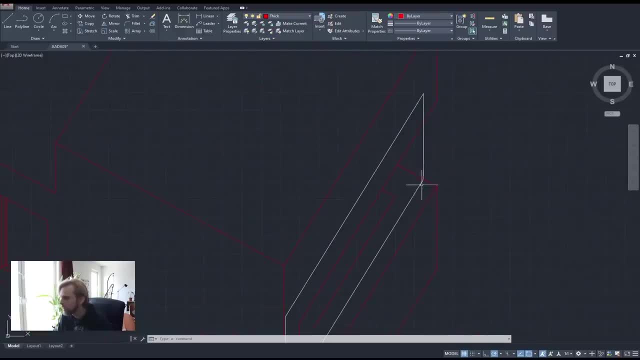 thing here. it can't rest on this side of the wall, it needs to go in. so i am going to just grab this line right here and i will make an offset of it by 200 inwards. so now i can see the the new, the new line segment that i can draw, and i'll draw it, of course. so, helper, uh, polo line from here. 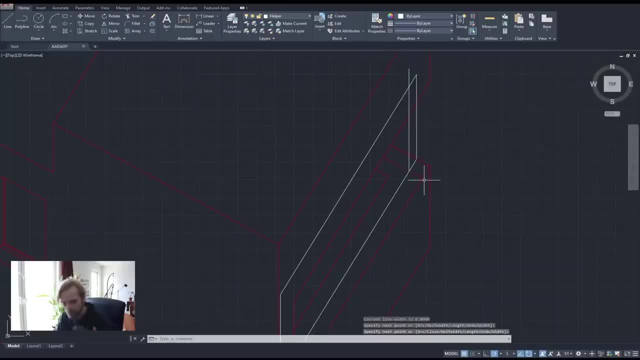 upwards. it's like that. we need to clean it up, uh, because the more again, the more curves you have, the uh, the harder it is for you to understand what the hell is going on. so i'm going to delete all of the unnecessary bits, um, and i'm going to rotate the view. as per usual, i'm going to trim. 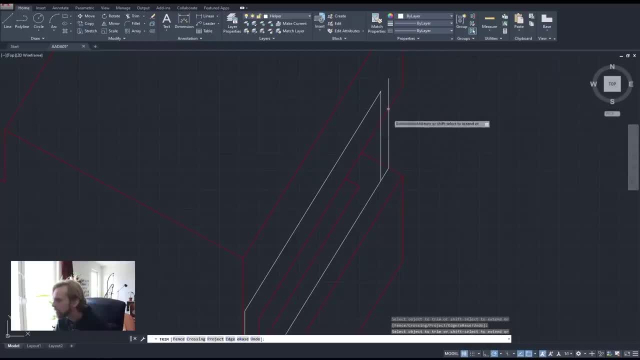 enter, enter, and i'm going to trim away the things that i don't need, so that, and i'm going to join things that i do need. it's a second, yeah, um, right, so so now i have it offset. it offset, uh, by 200 inwards, and that is great. it makes a bend, but we will never see that bend that it makes. 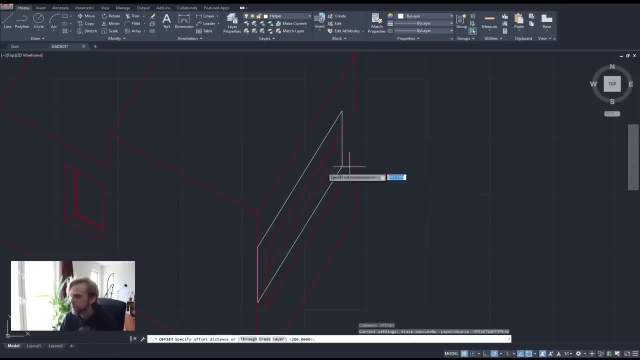 a bend, but we will never see that bend, but we will never see that bend. so we are going to do the same thing with this plane here. i will offset it now. i'm just doing the same thing as i'm i was doing here: offset 50, hello, offset 50. there we go. you go in then take this copy. 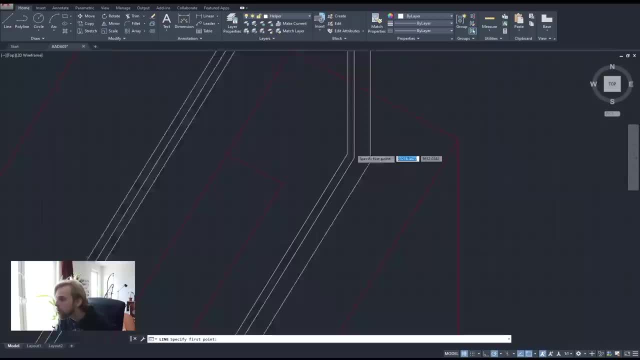 along this direction by 25, that small little line right there for the frame. um, right now we clean everything up as per usual: trim, trim bam, bam bam. no need for that. delete, okay, so that's oh. uh, forgot that part. trim bam bam. now, that's fine, okay, um, so i have this done. there's also- uh, i forgot one thing we have. 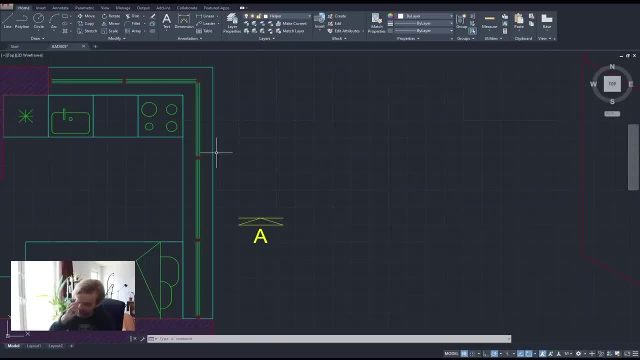 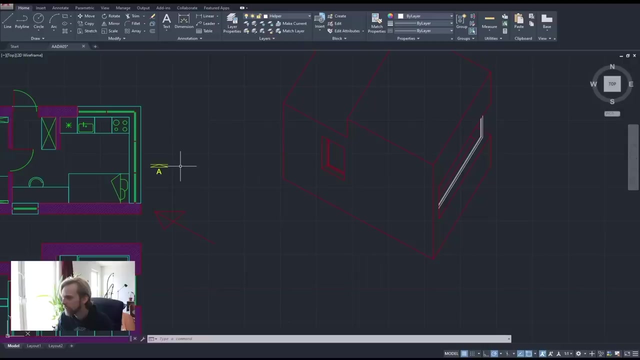 two partitions. that's oops, that's my bad. so the way i'm going to do partitions, i think, is: do we measure from the side of the wall? yeah, maybe, maybe we just measure from the side of the wall, right, or is that a stupid way to do it? 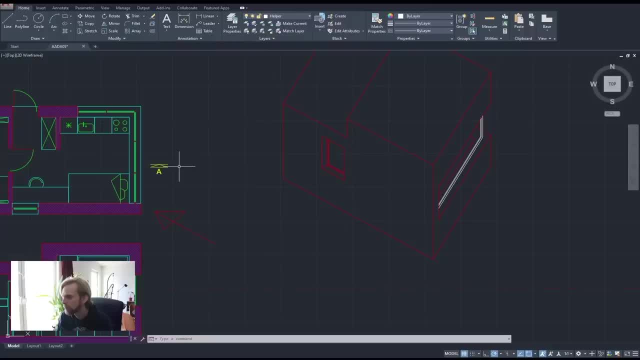 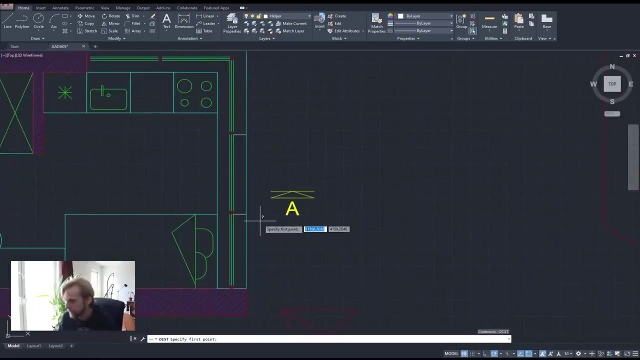 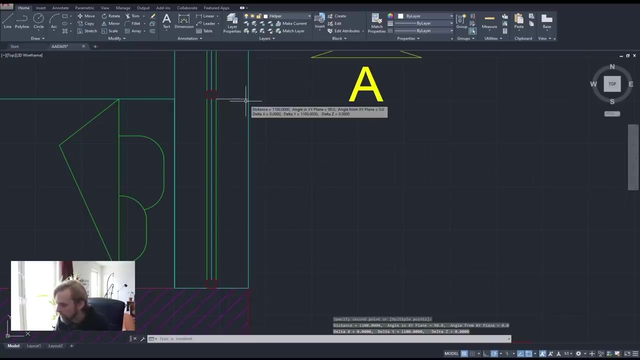 maybe it is a stupid way to do it, i know, let's do it this way. i'll draw two helper lines here, right here and right here, and i will measure their distances from this corner, from where the window starts. distance to this line is going to be one thousand one hundred, and then 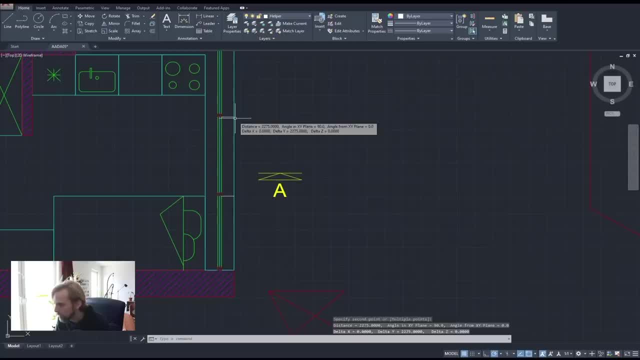 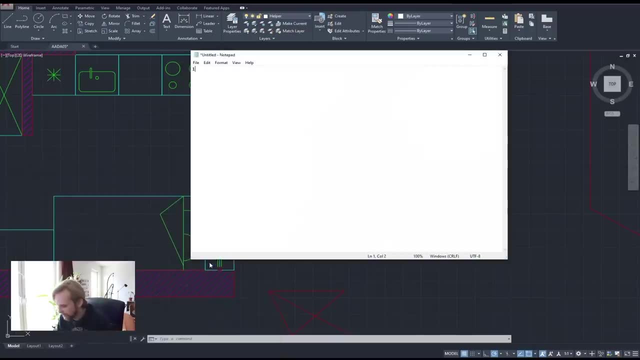 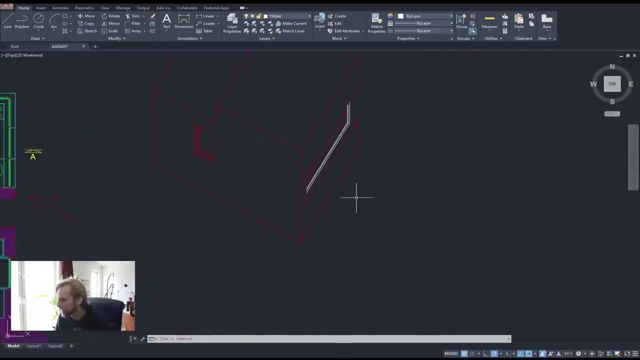 another distance is going to be 1 100.. and then another distance is going to be to be two thousand two hundred seventy five. one one zero zero, two, two, seven, five. okay, i just need to. i am sure that i will forget that. uh, so then what i can do is i can just draw a pol line from. 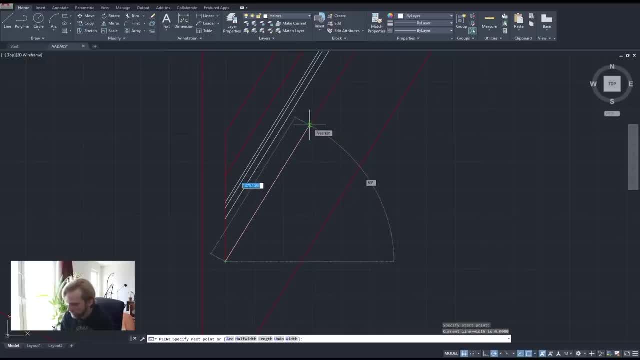 here like so, um, one one, zero, zero, like that. so that's a point right here, and let me actually mark it out just with a random line here. and then another one is going to be: uh, yep, forgot it. two, two, seven, five. there we go. two, two, seven, five. 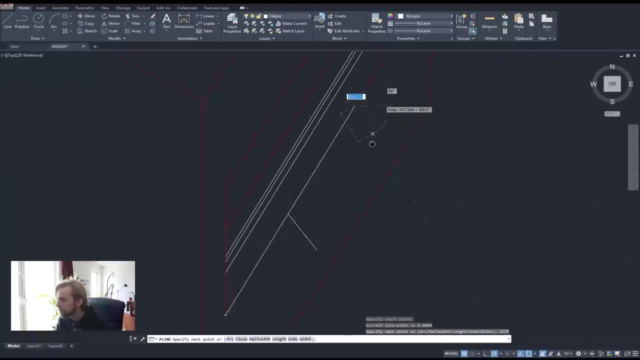 enter so it goes until here and just draw it out, like so. so i have like these two, two corner points and i know that if i were to make like an extension for the frame it would reach those two corner points. so i can kind of backtrack right, i can kind of do this. i can grab a polo line and i can draw it, uh, like so. 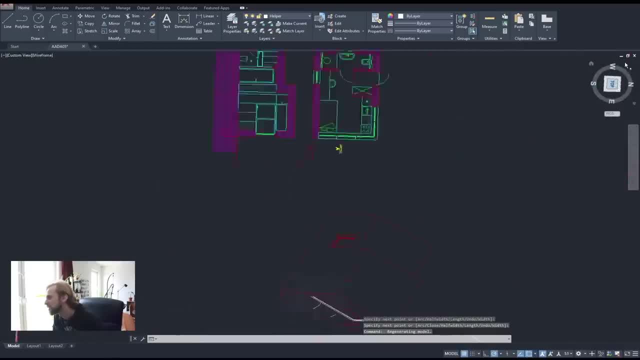 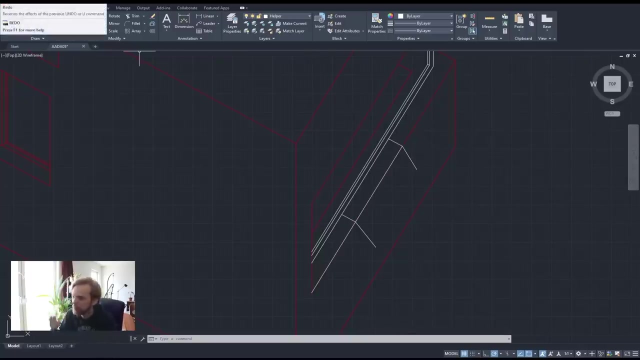 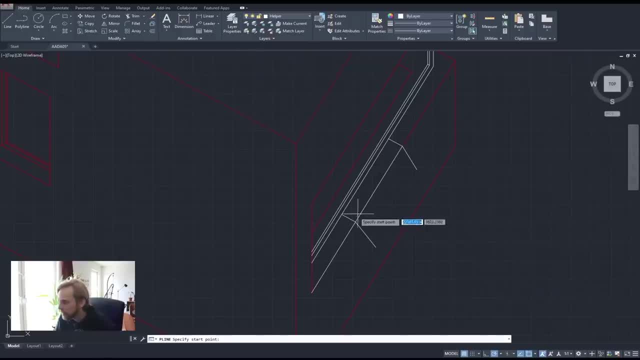 is just vertical lines, right? so i'll just grab a polo line again and i'll just draw out. i just need to make sure that i'm sticking to the correct position. yeah, there we go. i'll just draw, draw out vertical polo lines here, or vertical line segments and here. right now i don't need those. 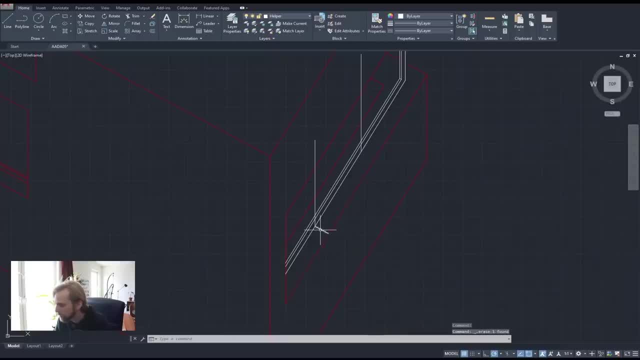 helpers anymore. so i'll just delete them so that they are not in the way anymore like that. and for these line segments, i can actually clean them up a little bit more: trim, come on, trim, enter, enter, bam, bam. i can clean them up a little bit more and i can start. 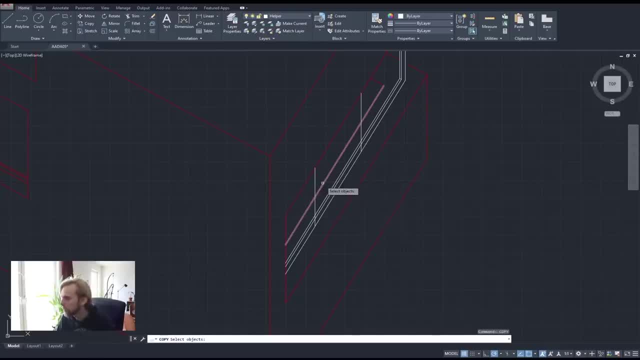 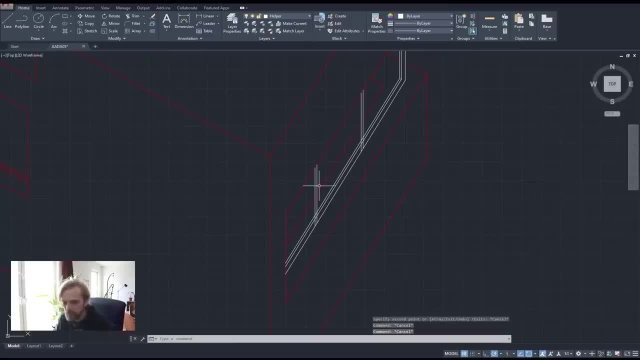 by 50 millimeters. right, because that's that's the thickness of the polo line right um, or polo line, not the pollen of of the frame. so i i drew this, this line right here and then i copied it by 50 millimeters. don't need those helpers anymore. 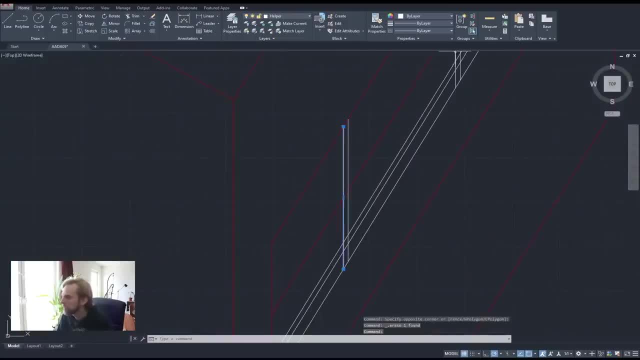 okay, so we have that done. um, and now i will just take these two line segments and i will copy them in by: uh, 25 millimeters for this thickness right here, only that we will see it on the side copy along this direction: 25 mil. that's done, okay, time to clean it up and make it actually. 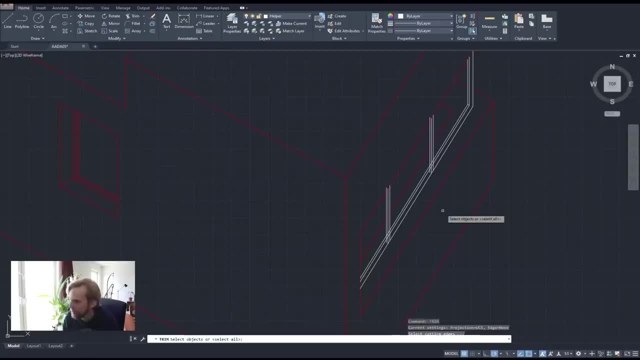 look like a proper, proper window. uh, trim, enter, enter. and now it's just a bunch of trimming here. uh, so the frame will merge. so the frame kind of does this, so the frame will merge. so the frame kind of does this right, it just merges, um like so, and of course you don't see. 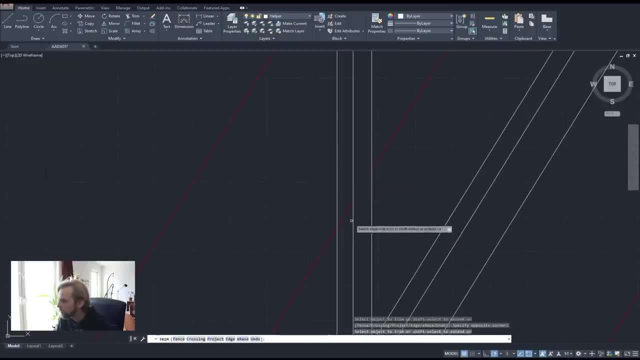 right, it just merges um like so, and of course you don't see, right, it just merges um like so, and of course you don't see anything behind the frame, anything behind the frame, anything behind the frame. here as well. you don't see anything behind. here as well, you don't see anything behind. 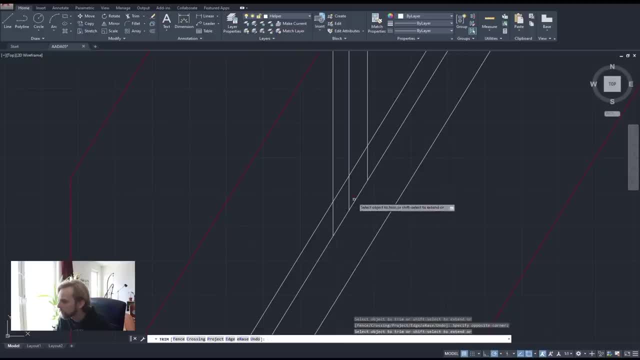 here as well. you don't see anything behind the frame, the frame. the frame merges here, um merges here, um merges here, um continues on here. like that continues on here. like that continues on here, like that. okay, that's good, and let's clean this up. okay, that's good, and let's clean this up. 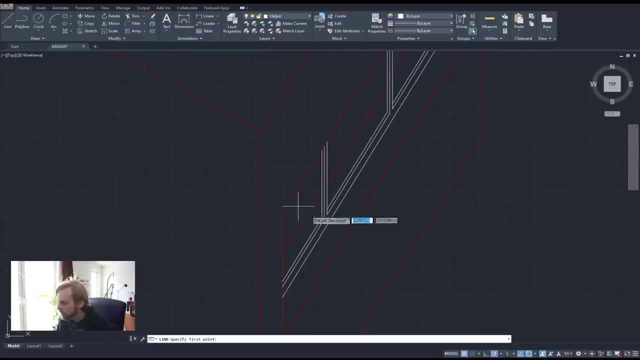 okay, that's good and let's clean this up. that's good. and there are two line segments, that's good. and there are two line segments, that's good. and there are two line segments that are missing. that are missing. that are missing where the frame bends, like here, and 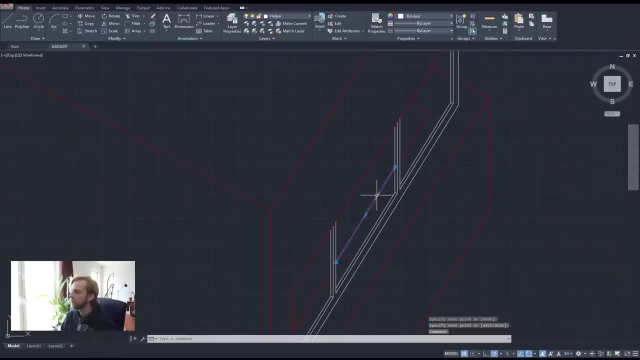 where the frame bends, like here, and where the frame bends like here and also right here, also, right here, also right here, oh yeah, and we don't need to see the oh yeah, and we don't need to see the oh yeah, and we don't need to see the inner line of the wall anymore, so we can. 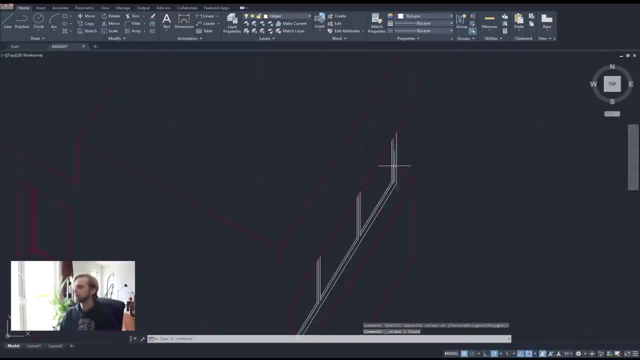 inner line of the wall anymore, so we can inner line of the wall anymore, so we can just delete that. oh that, that as well. oh that, that as well. oh that that as well. that's it, that's that is our. that's it, that's that is our. 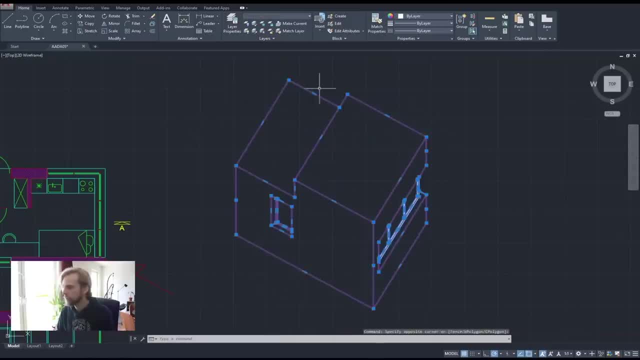 that's it, that's, that is our window in the axle right window, in the axle right window, in the axle right. um, i will change everything to medium, um, i will change everything to medium, um, i will change everything to medium. layer, uh, just because, layer, uh, just because. 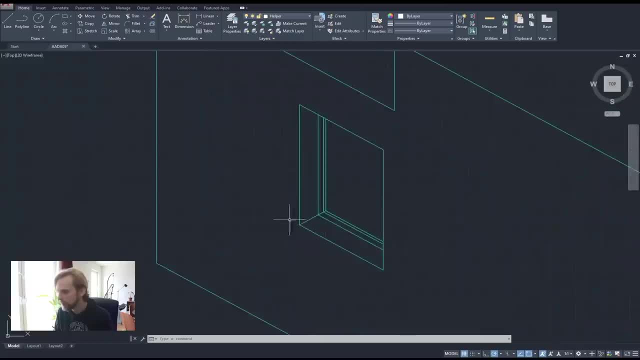 layer. uh, just because we are not cutting through anything, so we are not cutting through anything, so we are not cutting through anything. so it makes sense that it makes sense that it makes sense that it is a medium layer, except that for the it is a medium layer, except that for the. 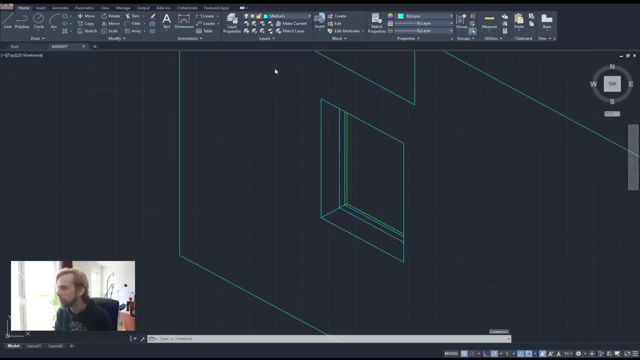 it is a medium layer, except that for the glass, glass, glass. i will change the glass to thin. i will change the glass to thin. i will change the glass to thin. thin layer, because there's too many thin layer, because there's too many thin layer, because there's too many, too many lines. 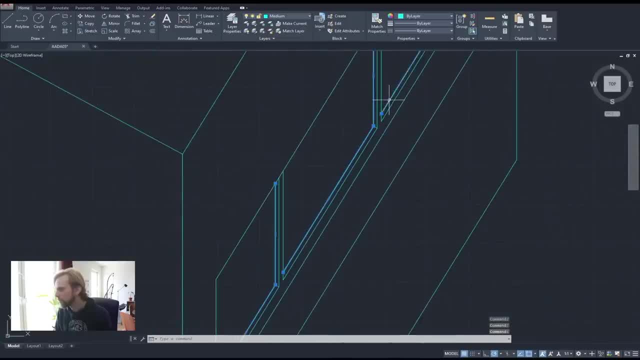 too many lines, too many lines that are concentrated, that are concentrated, that are concentrated, uh in in one spot. so i don't want them uh in in one spot. so i don't want them uh in in one spot, so i don't want them to merge, to merge. 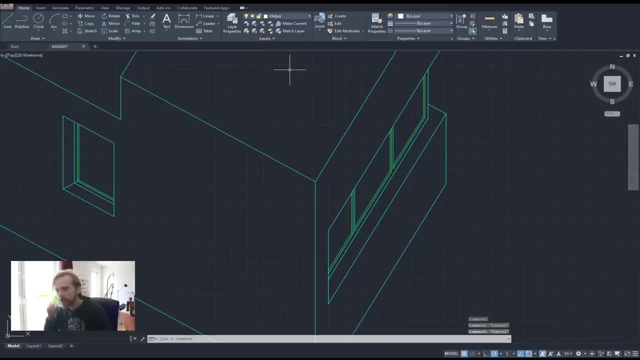 to merge, like graphically. i don't want them to like graphically, i don't want them to like graphically. i don't want them to merge into one thick line. merge into one thick line. merge into one thick line. so i'm going to make the glass. 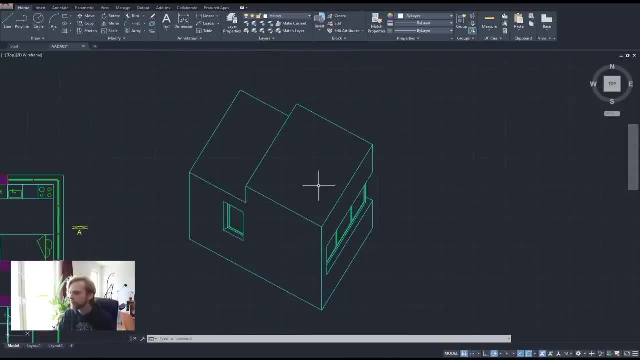 so i'm going to make the glass. so i'm going to make the glass. thin layer, okay, thin layer, okay. thin layer, okay, um, now it's all about hatching it. um, now it's all about hatching it. um, now it's all about hatching it right and and making it nicer. 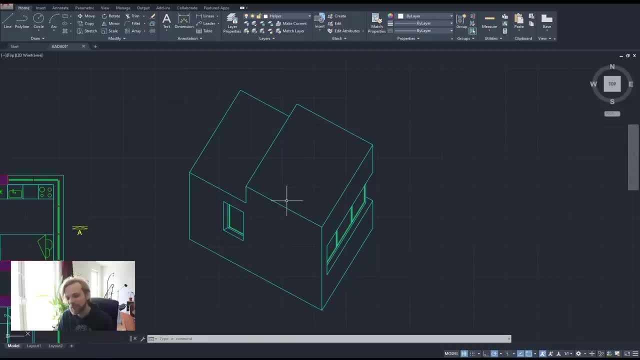 right and and making it nicer right and and making it nicer. um, it's not a very difficult building. um, it's not a very difficult building. um, it's not a very difficult building, that's for sure, that's for sure, that's for sure. um, let me just add the hatch and then 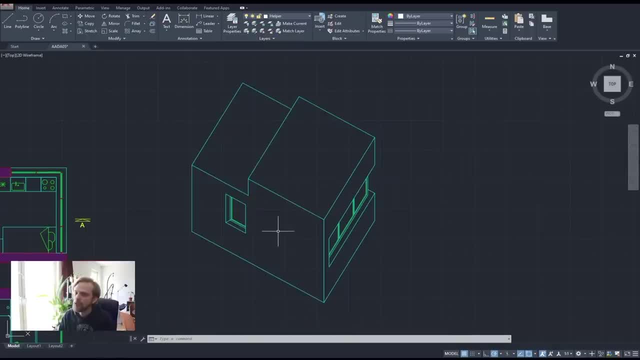 um, let me just add the hatch, and then, um, let me just add the hatch, and then we will continue. i don't want to spend, we will continue. i don't want to spend, we will continue. i don't want to spend too much time here. too much time here. 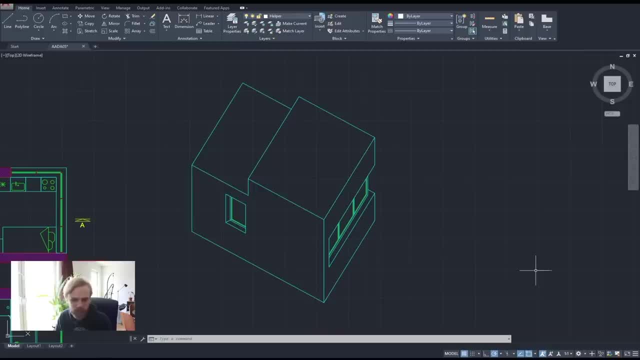 too much time here. uh, so i want to have uh planks. let's uh, so i want to have uh planks. let's uh, so i want to have uh planks. let's see, see, see, horizontal planks going around, the horizontal planks going around the. 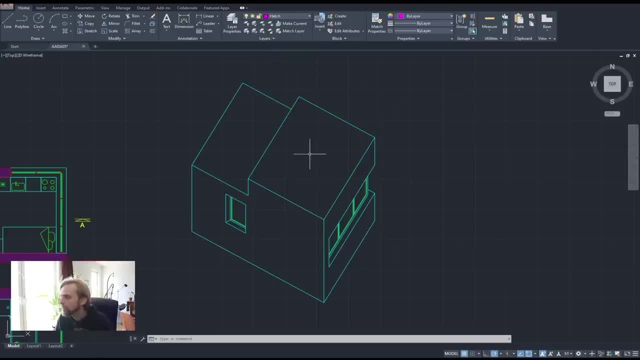 horizontal planks going around the building. so i will building, so i will building, so i will go to my hatch layer and i'll create a go to my hatch layer and i'll create a go to my hatch layer and i'll create a hatch, hatch, hatch for it, and i'll just 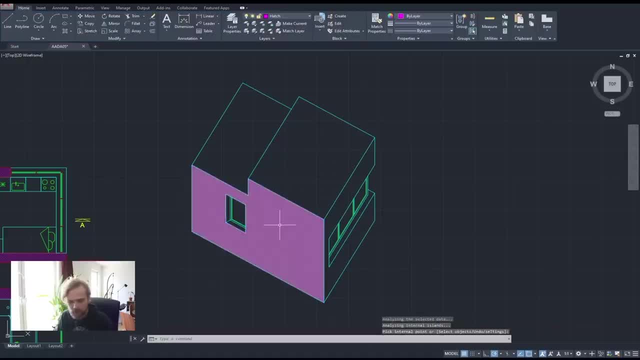 for it and i'll just for it and i'll just choose. let's say, this wall enter. so i've choose. let's say, this wall enter. so i've choose. let's say, this wall enter. so i've just created some random hatch. i'll just created some random hatch, i'll. 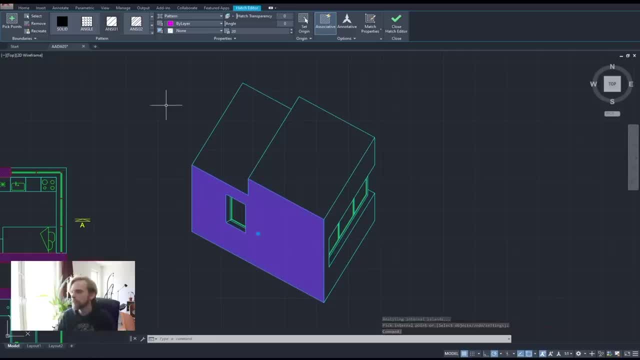 just created some random hatch. i'll select it, and now we can kind of go to select it. and now we can kind of go to select it and now we can kind of go to town here. so i know that this is town here, so i know that this is. 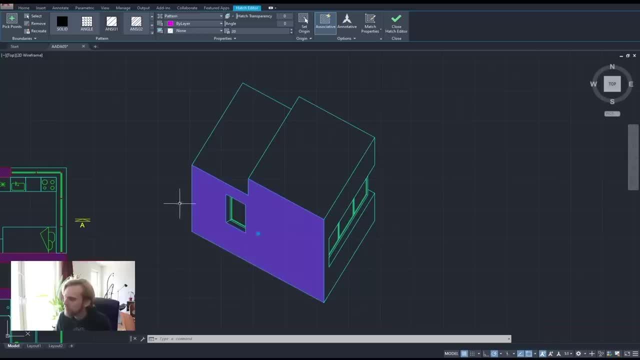 town here. so i know that this is: this is 60 degrees, this is 30 degrees, this is 60 degrees, this is 30 degrees, this is 60 degrees, this is 30 degrees, if i, if i, if i remember correctly, remember correctly, remember correctly um. 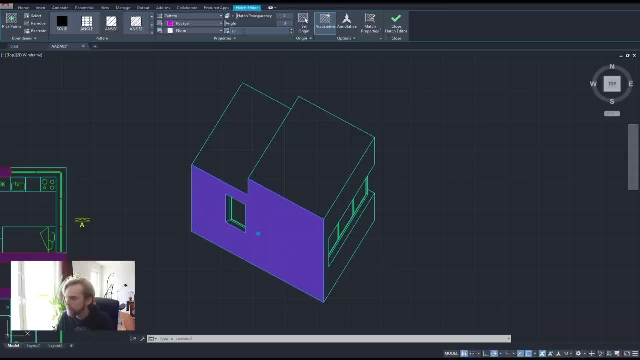 um, um. so i believe, if we do so, i believe, if we do so, i believe, if we do, if we do zero degrees here, oh sorry. if we do zero degrees here, oh sorry. if we do zero degrees here, oh sorry, sorry. where? when the angle is zero degrees. 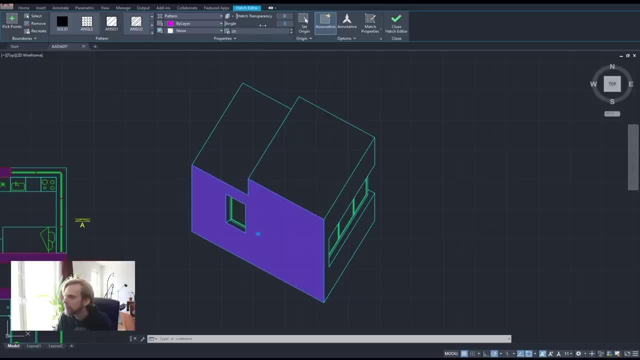 sorry where, when the angle is zero degrees, sorry where, when the angle is zero degrees, it's at 45, it's at 45, it's at 45, right? um so let me do, or actually let me right. um so let me do, or actually let me. 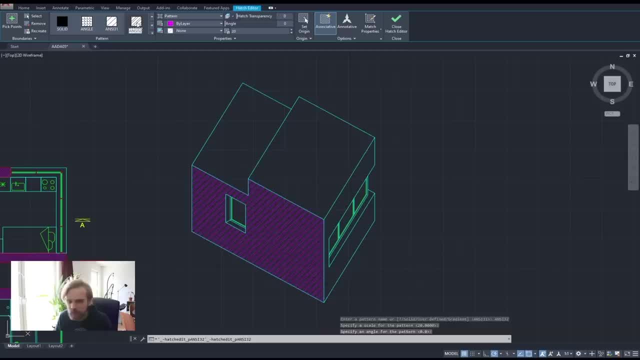 right, um, so let me do, or actually let me change the change. the change the. yeah, i'll use this uh instead the this. yeah, i'll use this uh instead the this. yeah, i'll use this uh instead the this. hatch instead for the planks. hatch instead for the planks. 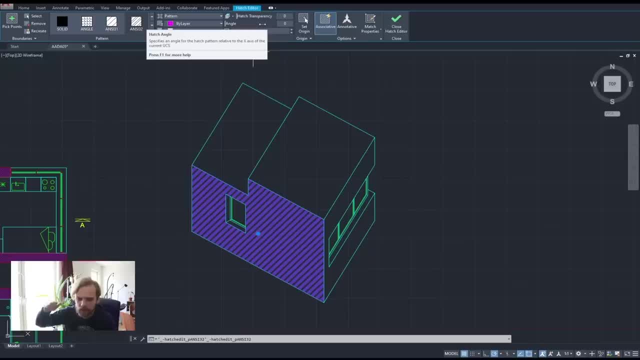 hatch instead for the planks. so instead of uh 45, we want to first. so instead of uh 45, we want to first. so instead of uh 45, we want to first start with horizontal. so let me just say start with horizontal. so let me just say: 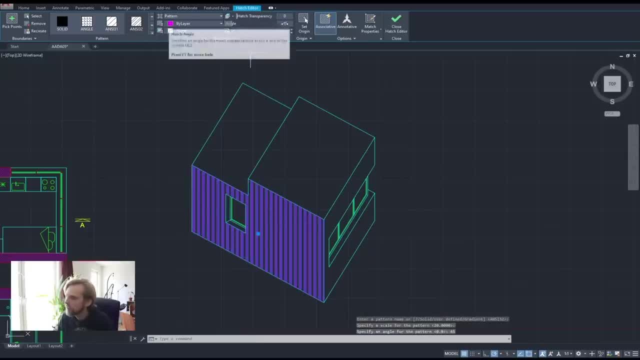 start with horizontal. so let me just say: 45 degrees, that is not horizontal. 45 degrees, that is not horizontal. 45 degrees, that is not horizontal. uh, so let's add 90 more 135. uh, so let's add 90 more 135. uh, so let's add 90 more 135. so now these are horizontal, and now i 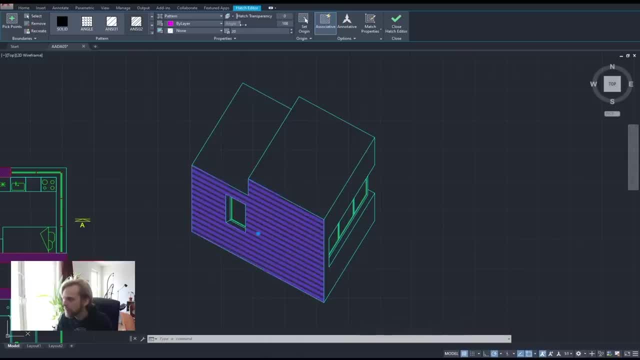 so now these are horizontal and now i. so now these are horizontal and now i can kind of rotate them, can kind of rotate them, can kind of rotate them. so i need to rotate it back. so 135 and i rotated back by 30 degrees. so 135 and i rotated back by 30 degrees. 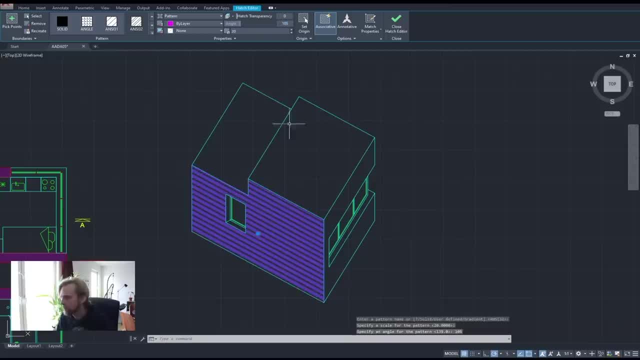 so 135, and i rotated back by 30 degrees. so that's going to be, so, that's going to be, so that's going to be: zero, 105, 105, zero, 105, 105, zero, 105, 105. there we go, and i really want the planks. 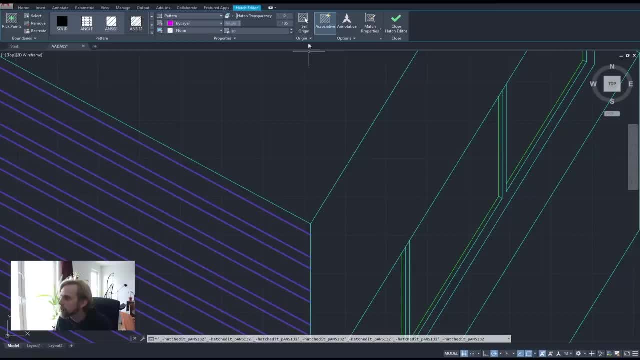 there we go and i really want the planks, there we go and i really want the planks to start from this, to start from this, to start from this point right here. so i will choose it as point right here, so i will choose it as point right here. so i will choose it as my. 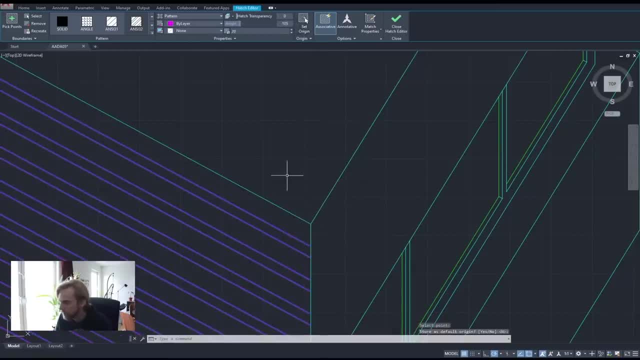 my my as my origin set origin, as my origin set origin, as my origin set origin. this point right here. so the planks, this point right here. so the planks, this point right here. so the planks start from here. start from here, start from here. okay, and now for the scale of the planks. 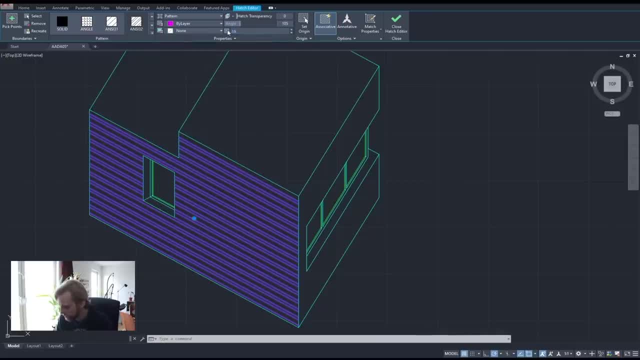 okay, and now for the scale of the planks. okay, and now for the scale of the planks. i think the scale is kind of good. i think the scale is kind of good. i think the scale is kind of good, but, um, maybe i'll do like 15. 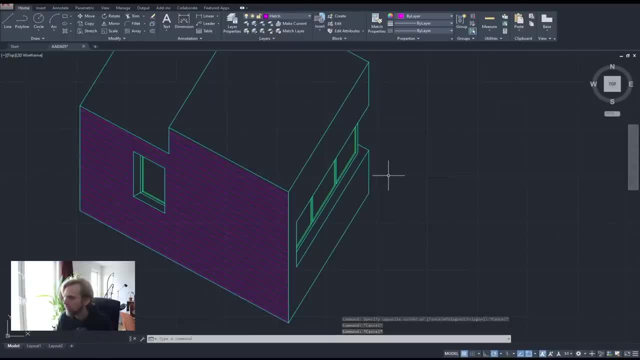 but, um, maybe i'll do like 15, but um, maybe i'll do like 15, something like that, something like that, something like that. that's it, that's it, that's it. um now for the other wall: same procedure. um now for the other wall- same procedure. 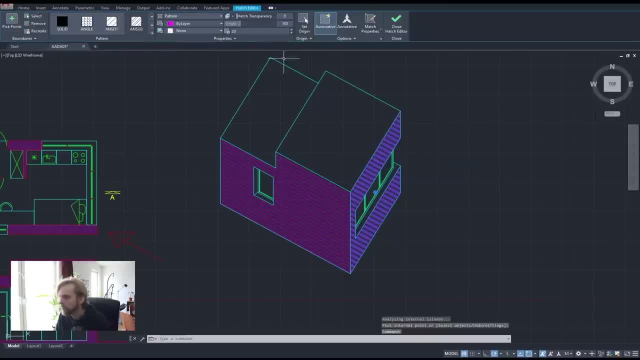 um, now for the other wall, same procedure: hatch, hatch, hatch, selected, selected, selected. angle is not going to to be 105. angle is not going to to be 105. angle is not going to to be 105. uh, it's actually going to be. that's pretty close. 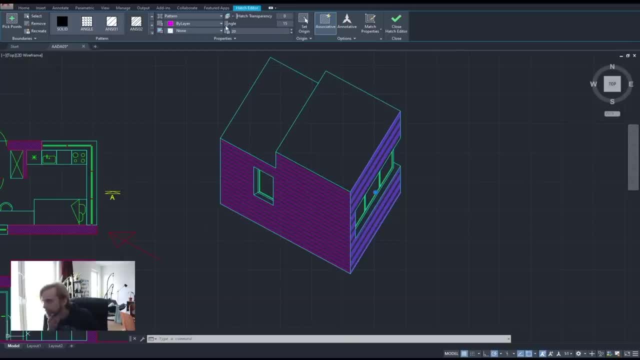 my guess is that it's going to be 15. my guess is that it's going to be 15. my guess is that it's going to be 15. right, yeah, it's going to be 15.. right, yeah, it's going to be 15.. 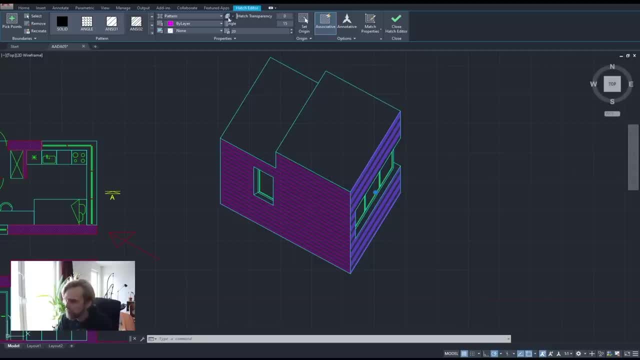 right, yeah, it's going to be 15.. um, um, um, you can, you can, you can always kind of rotate it with the, always kind of rotate it with the, always kind of rotate it with the slider here, slider here, slider here, and see what kind of values work, or you? 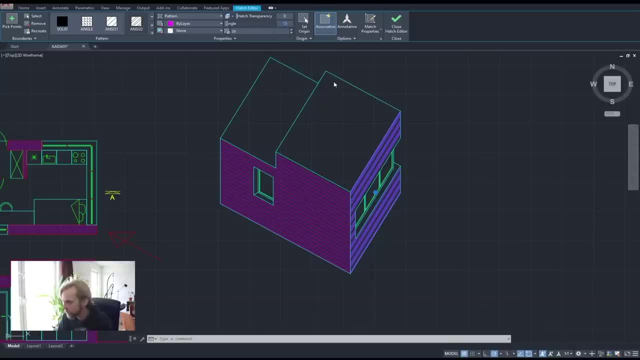 and see what kind of values work, or you and see what kind of values work, or you can do quick math in your head, can do quick math in your head, can do quick math in your head. that that works as well, so, but. but in that that works as well, so, but but in. 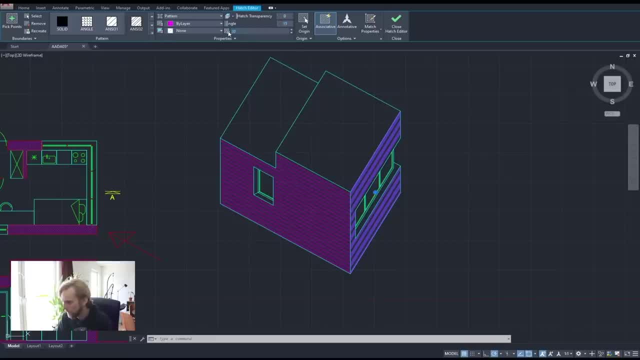 that that works as well. so, but, but in this case, this case, this case, the angle is 15.. uh, i used scale of 15. the angle is 15.. uh, i used scale of 15.. the angle is 15.. uh, i used scale of 15 as well, i believe. 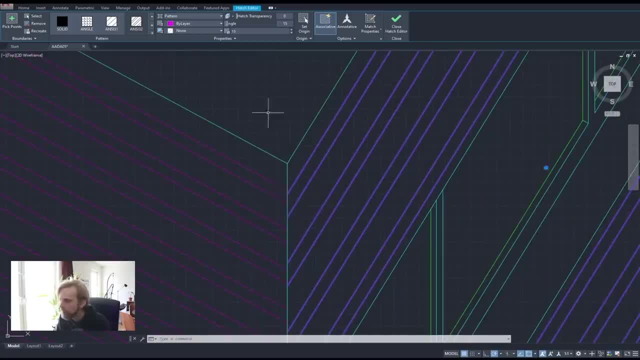 as well. i believe as well, i believe, and now i need see how these don't match. and now i need see how these don't match. and now i need see how these don't match. i need the same origin point, so i'll set. i need the same origin point, so i'll set. 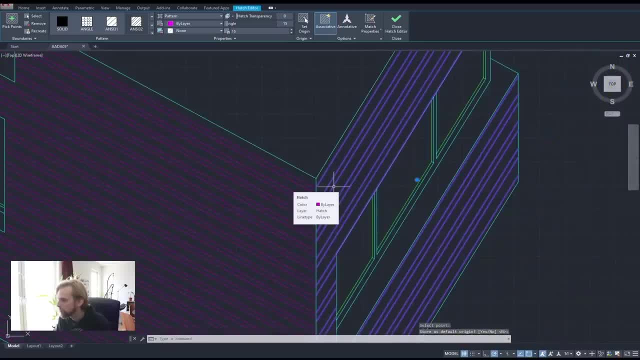 i need the same origin point, so i'll set: origin right here and these don't match. origin right here and these don't match. origin right here and these don't match. why don't they match? why don't they match? why don't they match? oh right, because the angle is different. 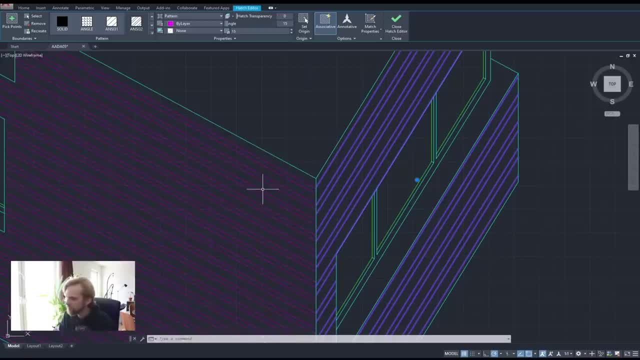 oh right, because the angle is different. oh right, because the angle is different. so of course they do so. of course they do so, of course they do. sorry apologies, of course they won't sorry apologies, of course they won't sorry apologies, of course they won't match. but also, 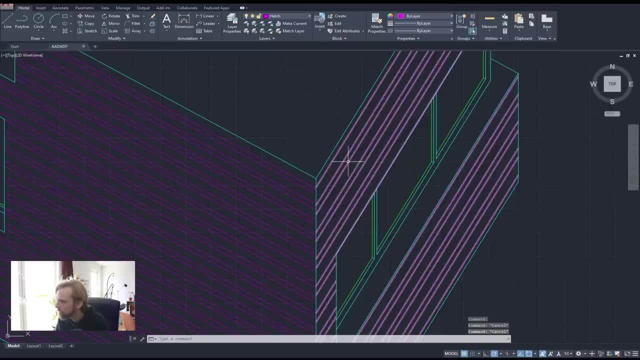 match but also match, but also that's 15 and that is also 15. they look that's 15 and that is also 15. they look that's 15 and that is also 15. they look very, very different, very, very different, very very different, both being moving 15. 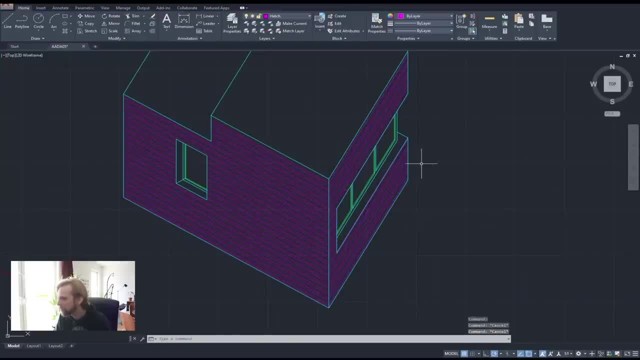 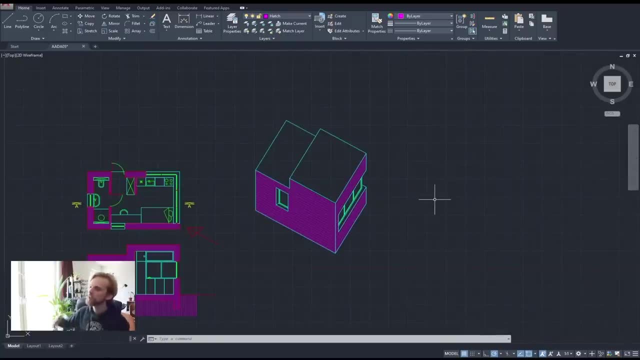 both being moving 15. both being moving 15 um a scale of 15. either way that's um a scale of 15. either way that's um a scale of 15. either way, that's good enough, doesn't matter. okay, so we have planks. 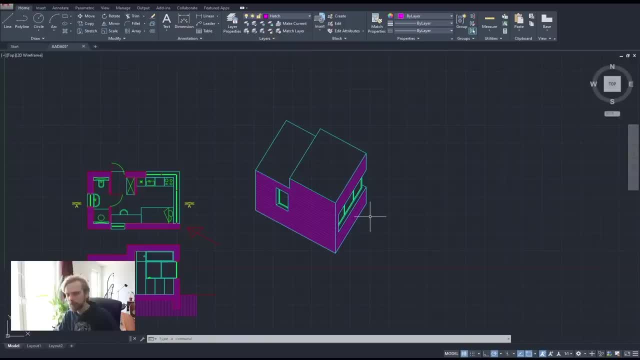 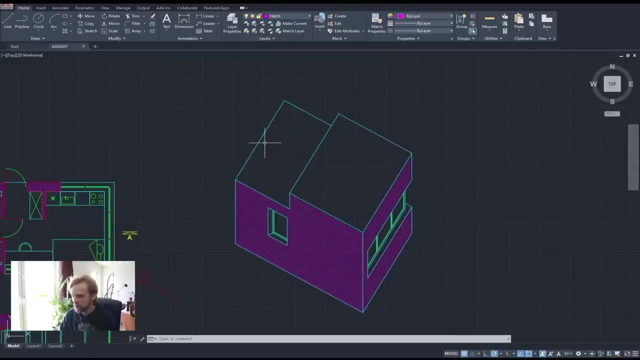 doesn't matter, okay, so we have planks. doesn't matter, okay, so we have planks here here. here, right, we, we have our our building, right. we, we have our our building, right, we, we have our our building. um, kind of want to let me just do one thing. 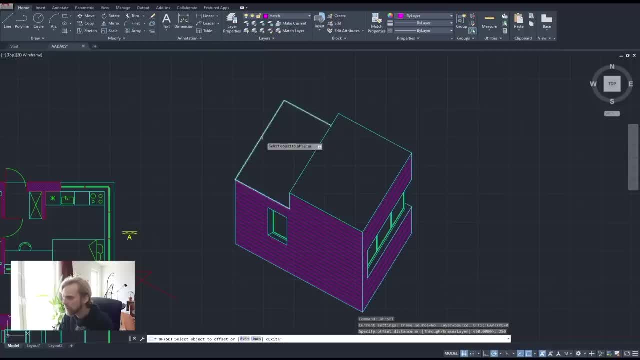 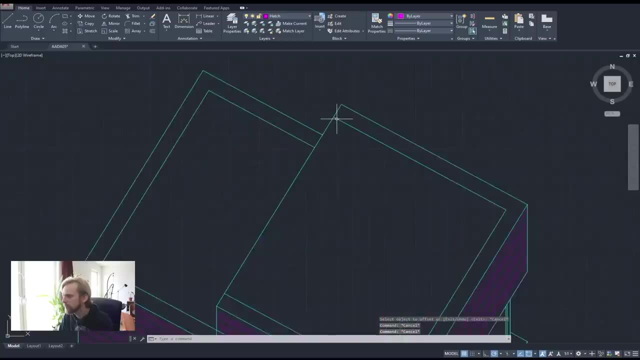 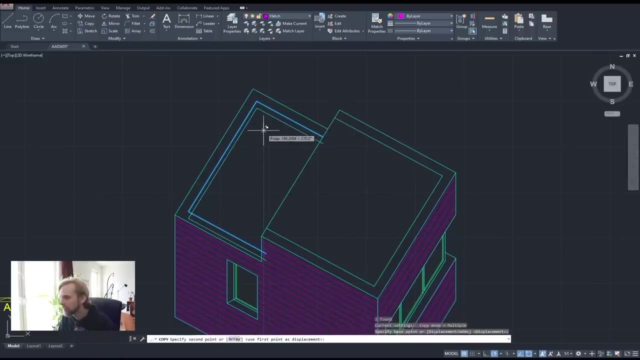 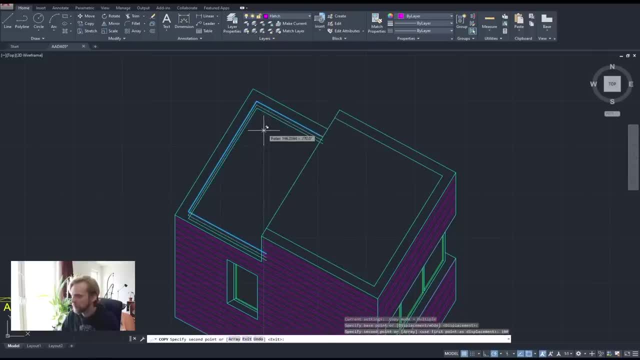 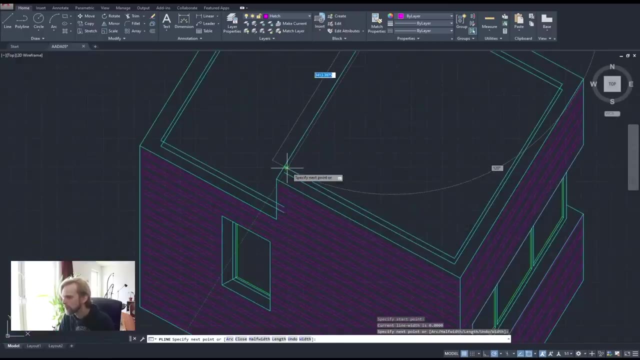 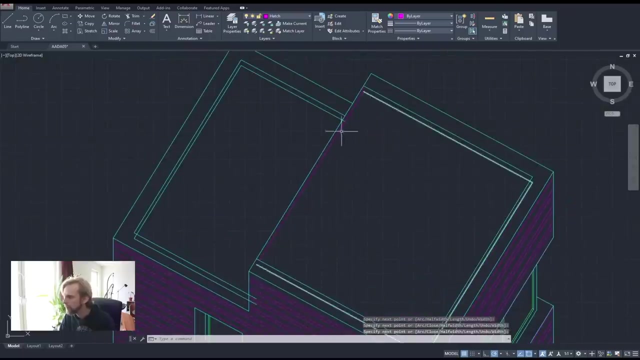 this is just me wanting to, and i have something a little bit more, and i have something a little bit more and i have something a little bit more complex in terms of the roof. complex in terms of the roof. until here, bear with me, it's not going to take too long, so that's going to be that. that, that. 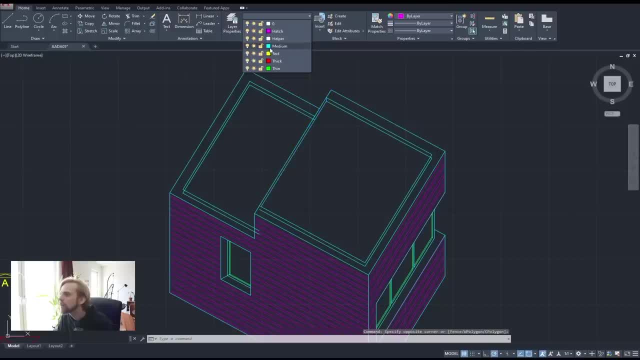 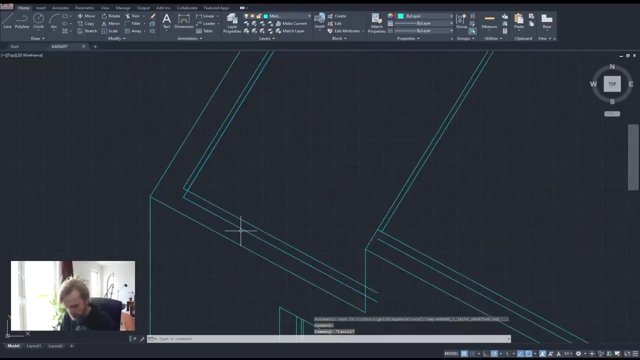 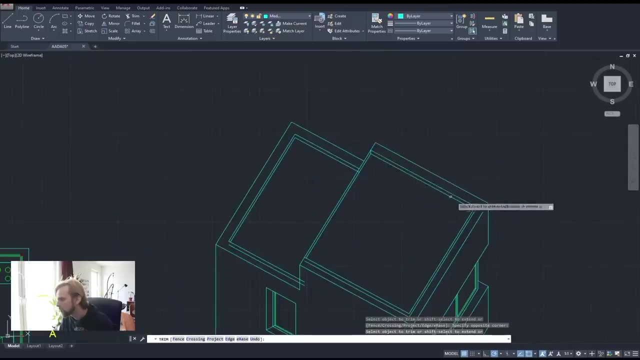 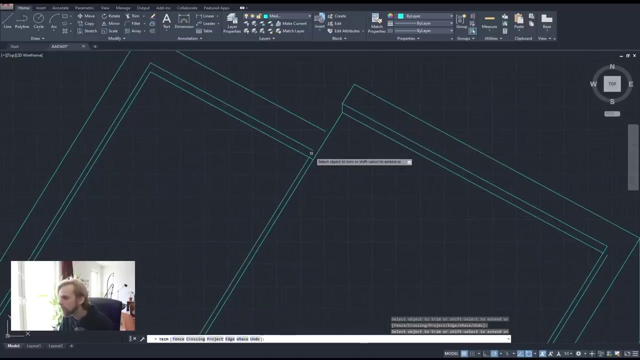 that's fine. um, can i go to medium? turn off the hatch layer. okay, medium is my active turn off the hatch layer. trim. i'll clean this up a little bit, just a little bit. trim, enter, go away. um, you are correct, but you go away and don't need that anymore. don't need that, that or that. 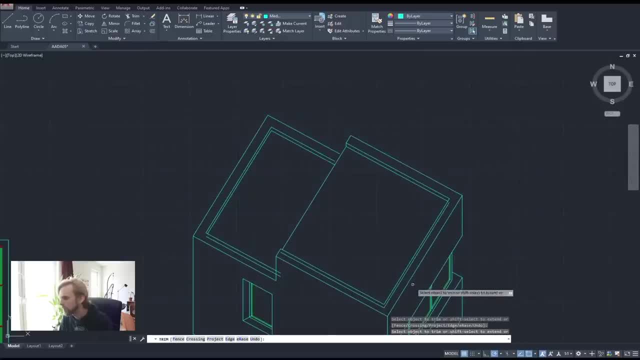 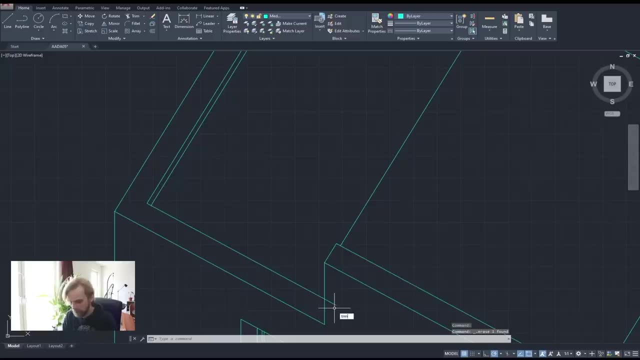 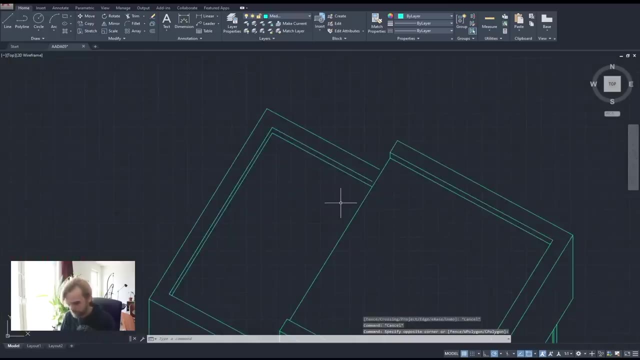 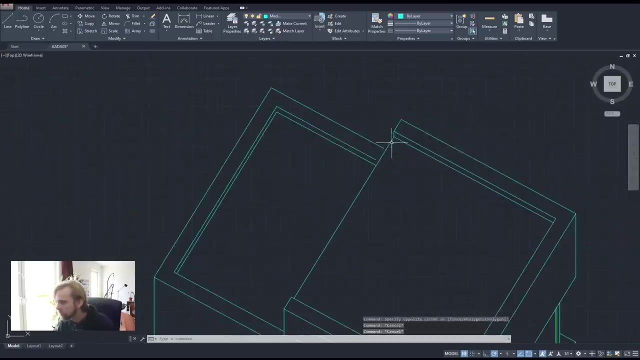 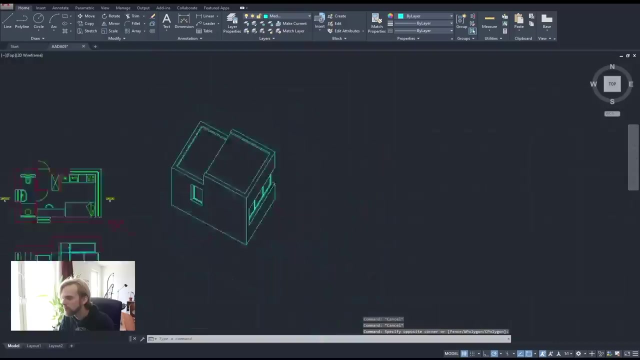 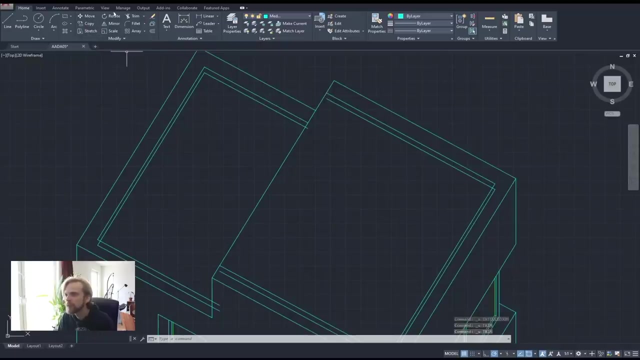 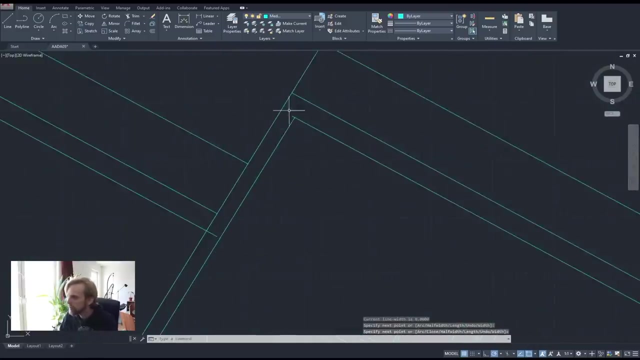 yes, it's fine. um, like that, like that, trim again forgot one, one part, this: um, what select are you locked? have i accidentally locked it? well, that's awkward. oh, undo, undo, so that was a bug. apologies for that. uh, i will need to to fix it apparently. uh, that the screen was frozen for a little bit and i didn't see that. there's, there's. 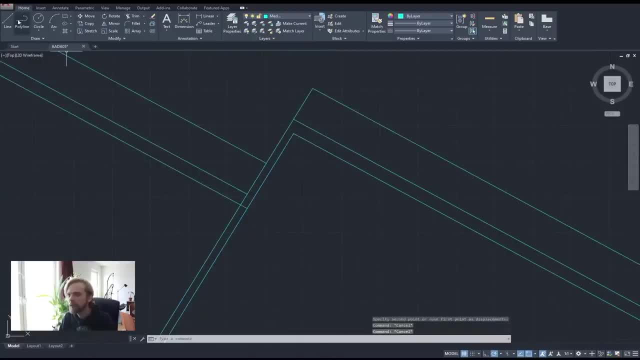 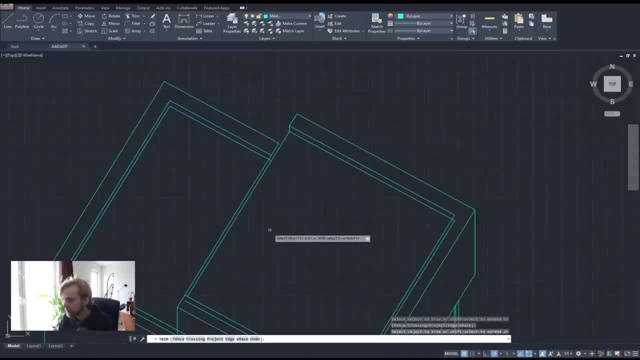 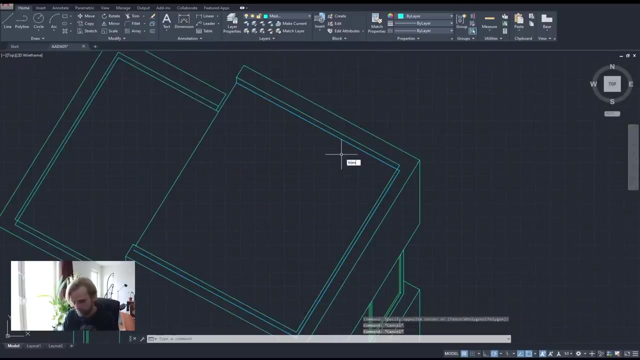 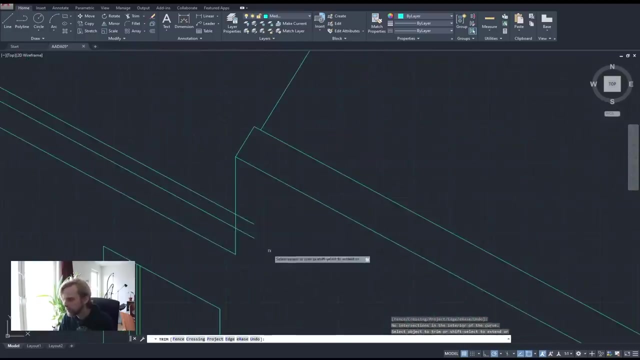 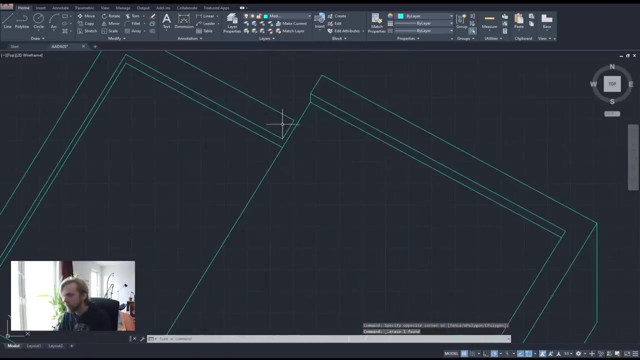 uh, there was a bug, so let's- let's clean this up real fast so that you don't need to wait too long. no need for that or that or that every time when you want to do something nice, you just need to deal with crap. ton of bugs. okay, so that's done. 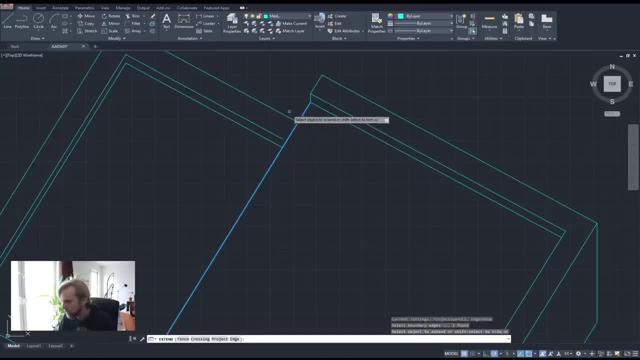 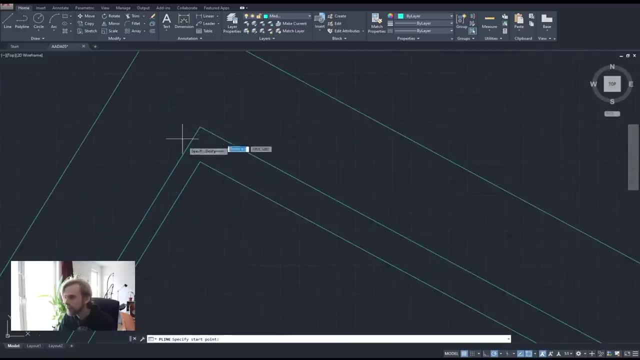 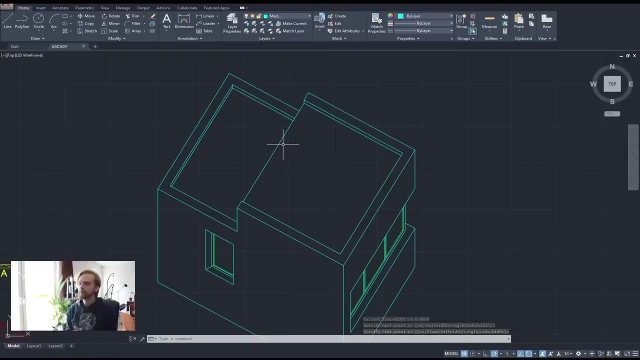 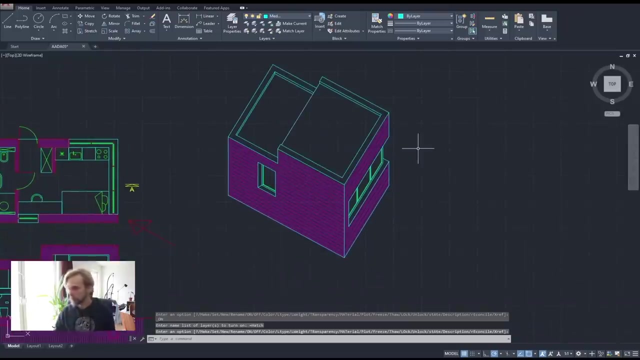 just fine, no need for that. this gets extended. um, you and you get extended, that all is fine and that just needs a line segment here. okay, a little bit more detail on on, on the roof, just just. you have something there, okay, let's, let's, uh, let's move on, uh. so we have our our axle, we have our plan, we have our section. 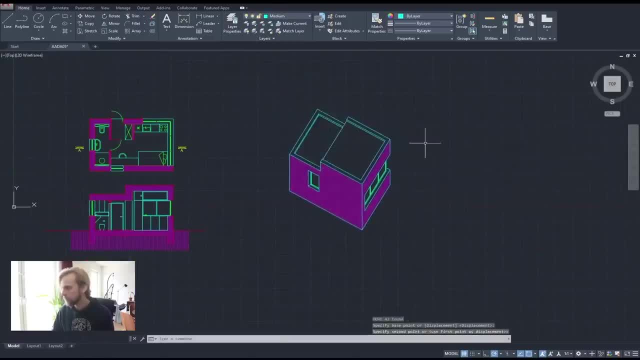 um, if i want to, maybe now it's the time to uh, to create layouts for, for plotting. yeah, i think it's it's time. i think it's time. so what we're going to do- sorry, what we're going to do- is I'm going to explain you what. what layout is, first of all, I guess. 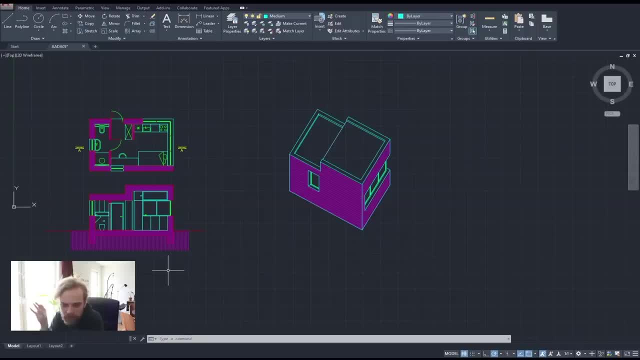 so this is your model space. this is a space in which you work. it's not the space in which you prepare the the project to be printed out, and where you work with additional information on the project. well, adding dimensions will be done here, but everything else will be done separately in the layout. so a 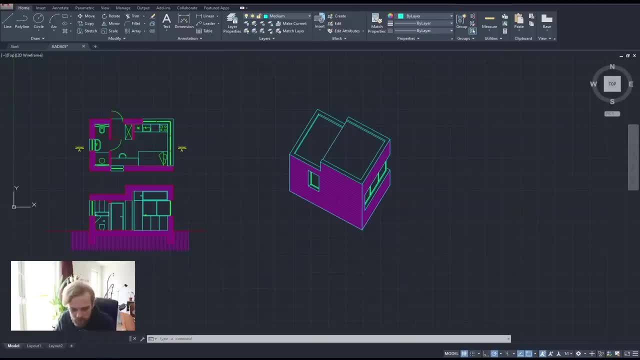 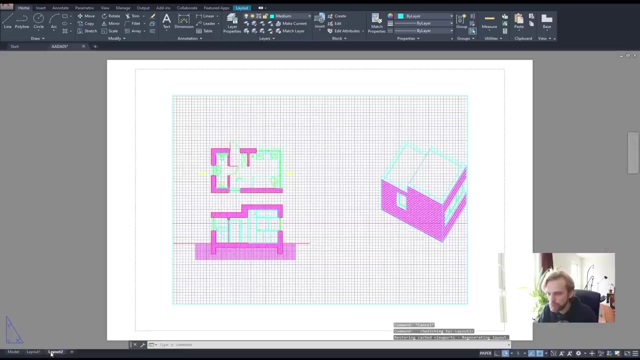 layout is here in the bottom of this. here in the bottom of the screen, you can see layout, layout one, layout two, and these are kind of just just. they're just doing their thing and we don't really need them. we will be creating our own, so I'll just delete. okay, you just right. 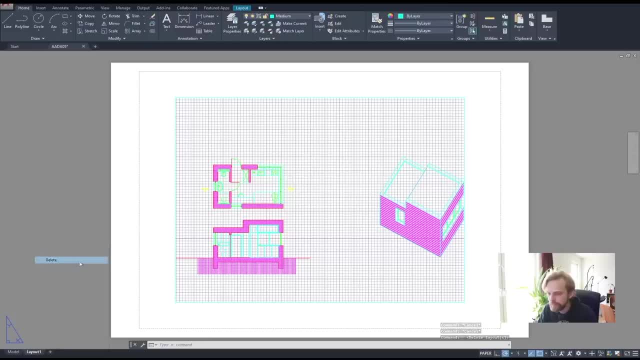 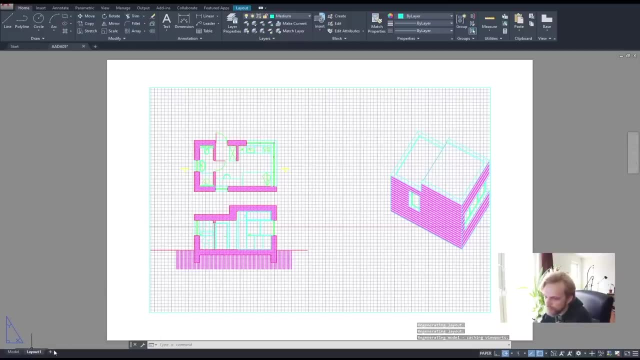 click on this and then you can see that the layout is already printed out. and you can see that the layout is already printed out and you just delete them, and you just delete them, you just delete them, delete. yeah, oh, this one doesn't delete. you need at least one layout, that's fine. 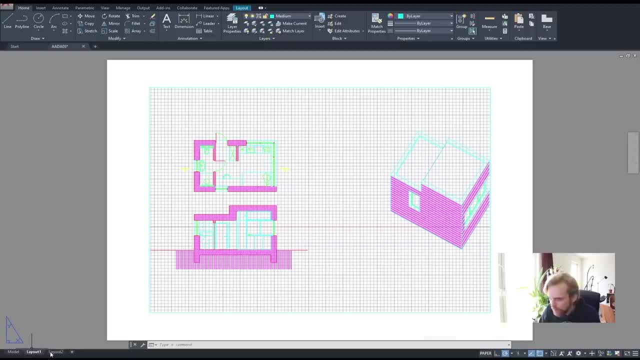 we will create our own and we will ignore this one. so new layout: you just click that plus sign, you right-click on it and you choose to do page setup manager. well, first let's rename it. I guess. first let's rename it and then let's name it plan. 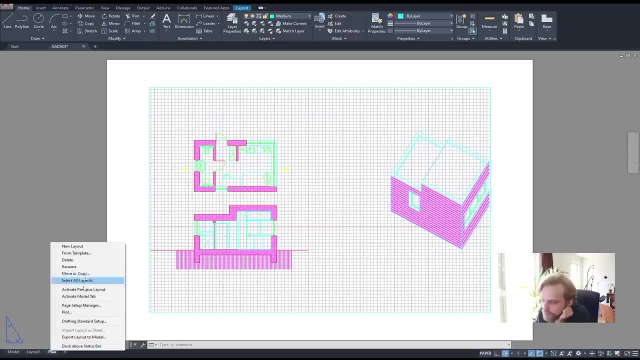 enter usually you. the convention for naming them is zero, zero dash plan, and then zero one dash section, zero two dash axle, and so on, so that all of them are kind of laid out properly. but in this case we just have three drawings, or whatever I name. name it, whatever you. 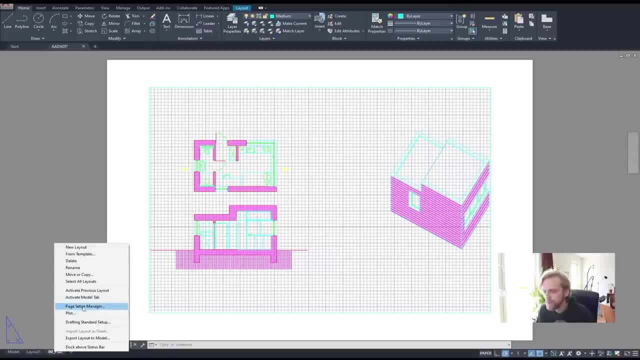 want. name it whatever you want. so that's our plan. we go to page setup manager. we, so that's our plan. we go to page setup manager. we, so that's our plan. we go to page setup manager. we right-click on the layout name. right-click on the layout name. 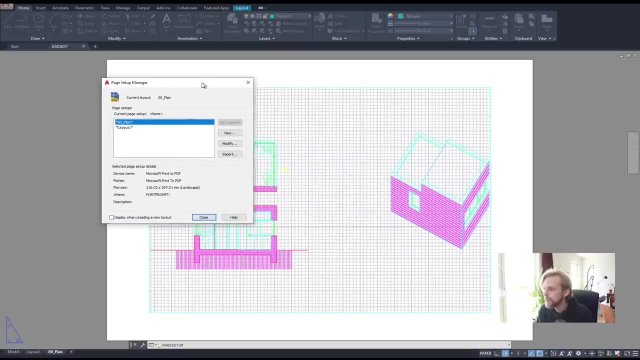 right-click on the layout name, we go to page setup manager right here. and we go to page setup manager right here. and we go to page setup manager right here and we modify it, we modify it, we modify it. so here in the page setup manager, you can. 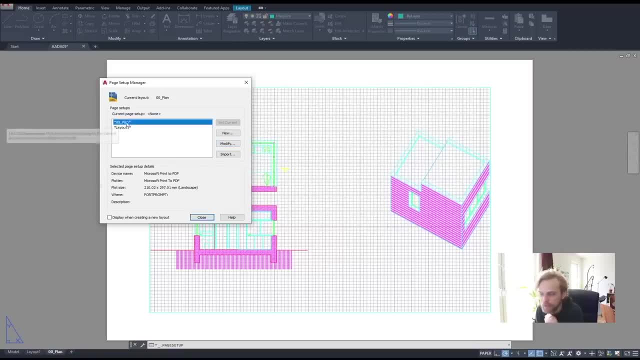 so here in the page setup manager you can. so here in the page setup manager you can see your layout one and the new one. see your layout one and the new one. see your layout one and the new one that you've created. so you select it and you 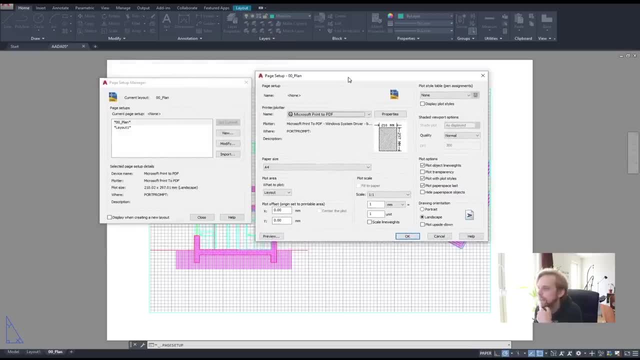 that you've created, so you select it, and you that you've created, so you select it and you click modify, click modify, click modify. okay. so this is where you kind of set up okay. so this is where you kind of set up okay. so this is where you kind of set up everything about the layout and all of 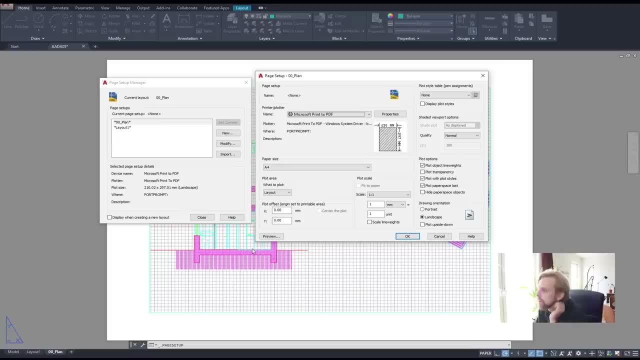 everything about the layout and all of everything about the layout and all of the settings on what kind of drawing you the settings on what kind of drawing you the settings on what kind of drawing you want to export right. so let's start from. want to export right, so let's start from. 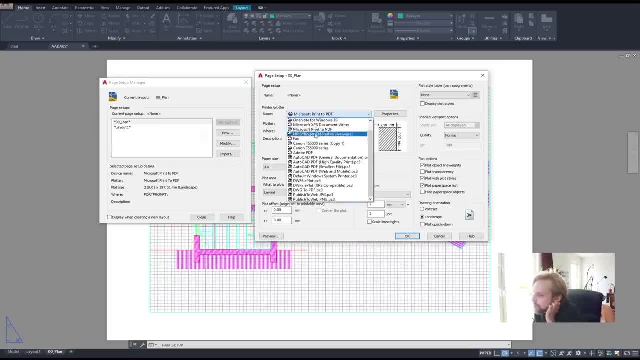 want to export right. so let's start from the. from the start: Microsoft print to the. from the start. Microsoft print to the. from the start: Microsoft print to PDF is fine. I prefer using Adobe PDF. DWG PDF is fine. I prefer using Adobe PDF. DWG PDF is fine. I prefer using Adobe PDF. DWG to PDF is also fine, but anything that. 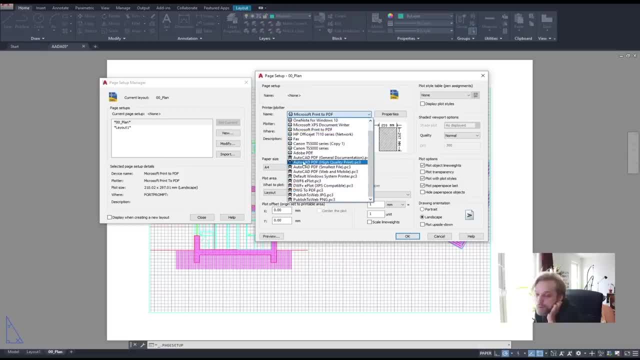 to PDF is also fine, but anything that to PDF is also fine. but anything that can kind of generate PDF you choose can kind of generate PDF you choose can kind of generate PDF you choose. you don't choose a printer because you will. you don't choose a printer because you will. 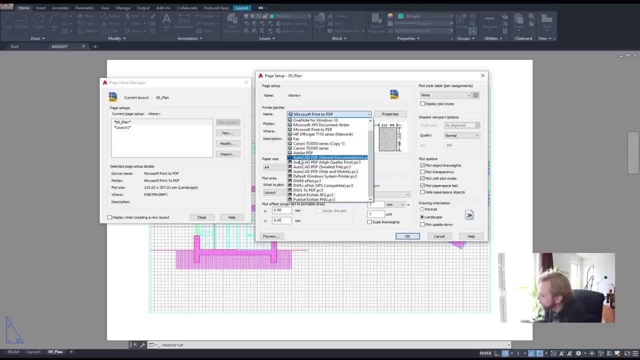 you don't choose a printer because you will be exporting it as PDF, right. so be exporting it as PDF, right, so be exporting it as PDF, right. so printing is not just printing on a sheet. printing is not just printing on a sheet. printing is not just printing on a sheet of paper or plotting. plotting is the. 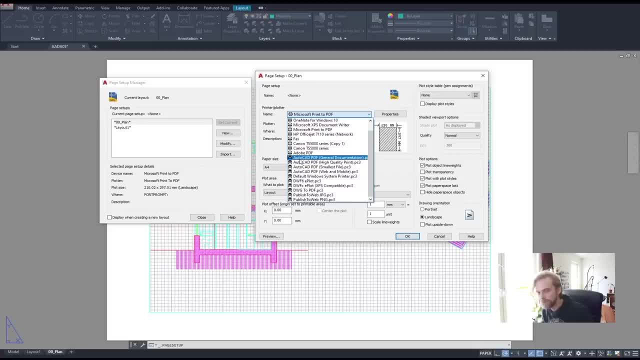 of paper or plotting. plotting is the of paper or plotting. plotting is the same thing as printing, by the way. it's same thing as printing. by the way, it's same thing as printing. by the way, it's not printing on a sheet necessarily on a, not printing on a sheet necessarily on a. 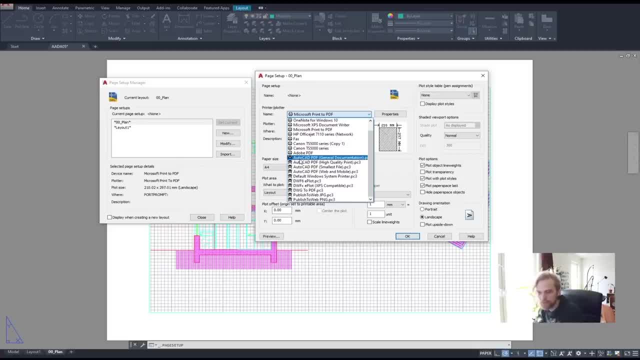 not printing on a sheet, necessarily on a sheet of paper. it can be printing to a sheet of paper. it can be printing to a sheet of paper. it can be printing to a file, right. so so to a PDF. so in this file, right? so? so to a PDF. so in this. 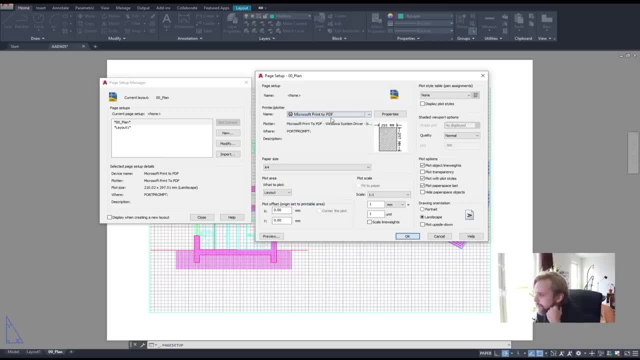 file right, so so to a PDF. so in this case, I'm going to choose: yeah, let's just case I'm going to choose. yeah, let's just case I'm going to choose. yeah, let's just go with Microsoft print to PDF. if you go with Microsoft print to PDF, if you. 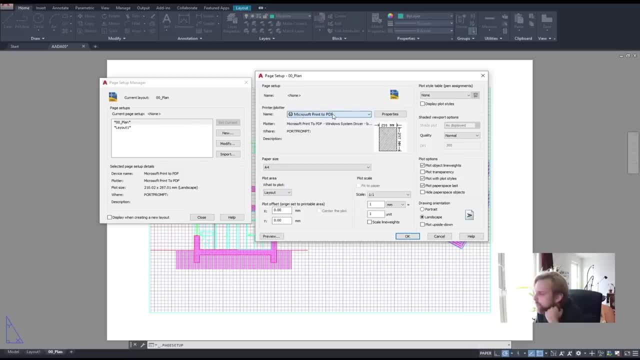 go with Microsoft print to PDF. if you want, you can use Adobe PDF. you can use want you can use Adobe PDF. you can use want you can use Adobe PDF. you can use DWG to PDF. whichever is to PDF, use so DWG to PDF. whichever is to PDF, use so. 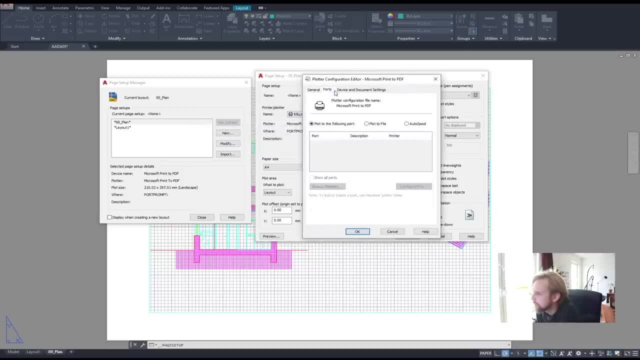 DWG to PDF, whichever is to PDF use. so that's done. let me just hit properties. that's done. let me just hit properties. that's done. let me just hit properties here and just double-check here, and just double-check here and just double-check. that's fine, that's whatever. I'll keep it. 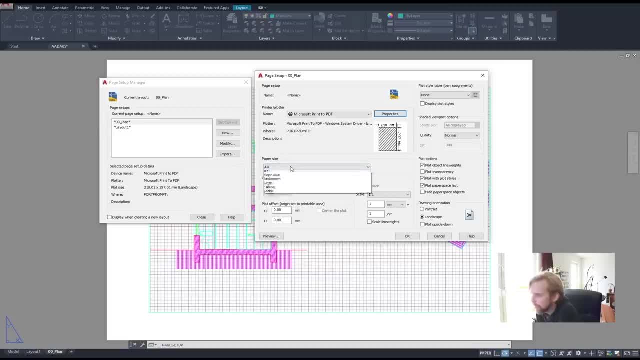 that's fine, that's whatever I'll keep it. that's fine, that's whatever I'll keep it. with the properties: paper size: here we with the properties paper size: here we with the properties paper size: here we will find a 3 will find a 3. 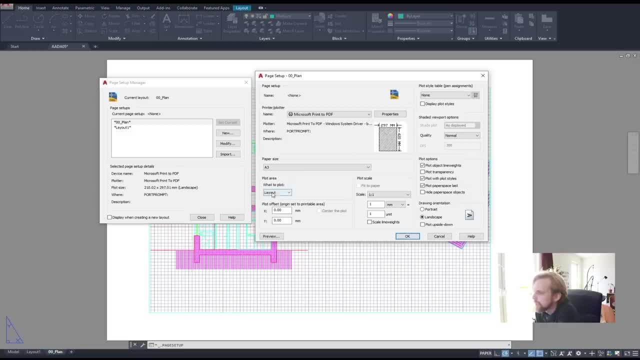 will find a 3. that's the size of the paper that we're. that's the size of the paper that we're. that's the size of the paper that we're gonna be using what to plot layout. yes, gonna be using what to plot layout. yes, 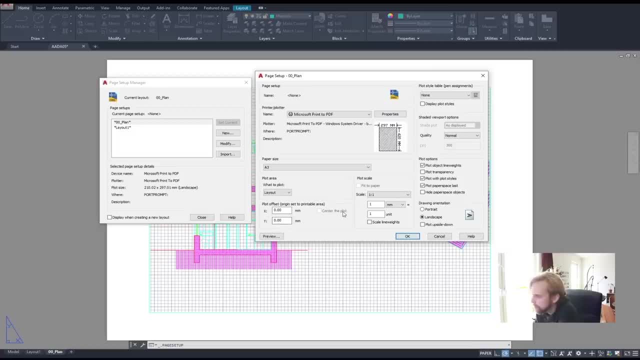 gonna be using what to plot layout? yes, plot offset. keep it at 0: 0, that's fine. plot offset. keep it at 0: 0, that's fine. plot offset. keep it at 0: 0, that's fine. scale 1 to 1: yes, so here the scale is. 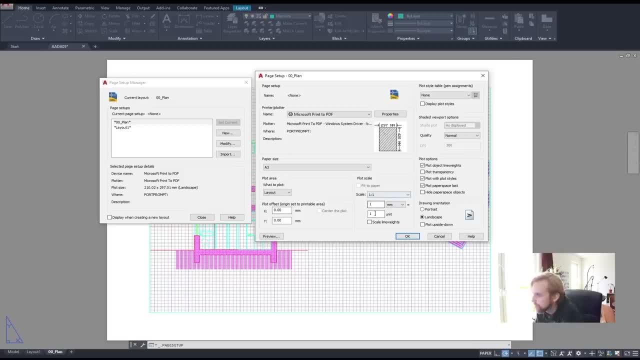 scale 1 to 1. yes, so here the scale is scale 1 to 1. yes, so here the scale is of the page, of the page of the page, not of your model. so the scale needs to, not of your model. so the scale needs to. 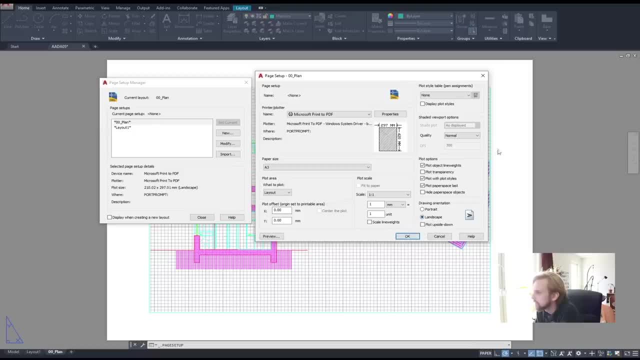 not of your model. so the scale needs to be one-to-one landscape. yes, be one-to-one landscape. yes, be one-to-one landscape. yes. and plot style and plot style and plot style. I use none. or plot style, I use none. that's important, that's it. no need for. 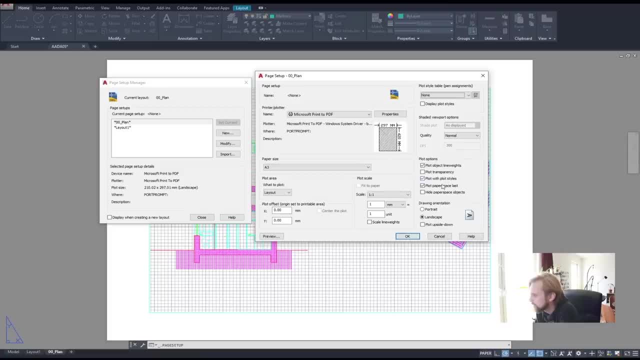 that's important. that's it. no need for. that's important. that's it. no need for anything else, anything else, anything else. yeah, no need for anything else. let's- yeah, no need for anything else. let's yeah, no need for anything else. let's, is it okay? 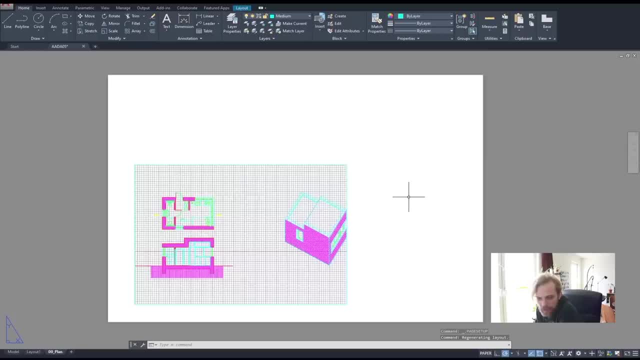 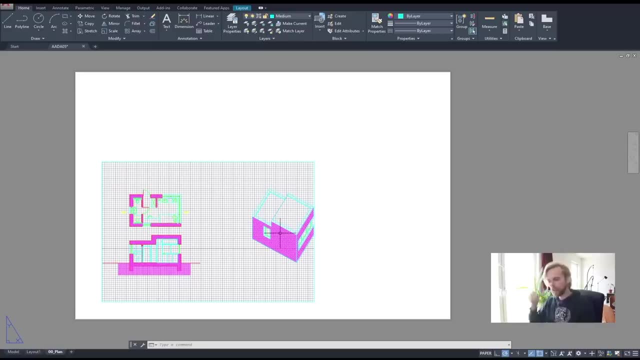 is it okay? is it okay? it closed, and now you can see that the it closed, and now you can see that the it closed and now you can see that the page became bigger right, and this is page became bigger right, and this is page became bigger right, and this is basically. this is like a window showing. 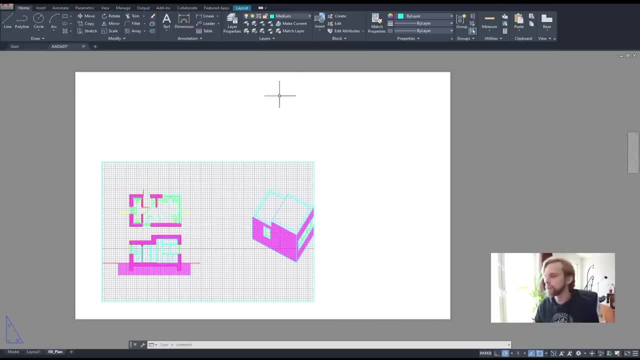 basically, this is like a window showing. basically, this is like a window showing us our model, and we will position our us, our model, and we will position our us, our model, and we will position our, our geometry in this in this page. so our geometry in this in this page. so 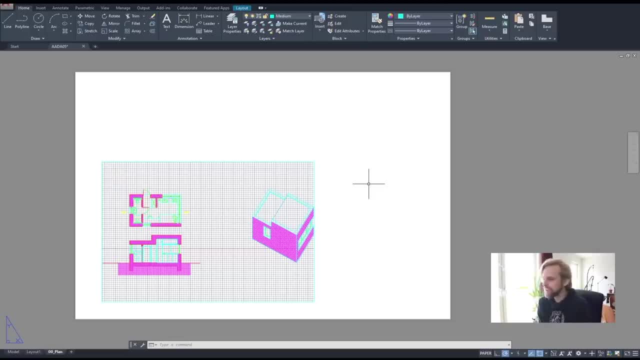 our geometry in this, in this page. so how do you do that? how do you do that? how do you do that? well, the thing is, first of all, you need. well, the thing is, first of all, you need. well, the thing is, first of all, you need to understand the philosophy of layout. 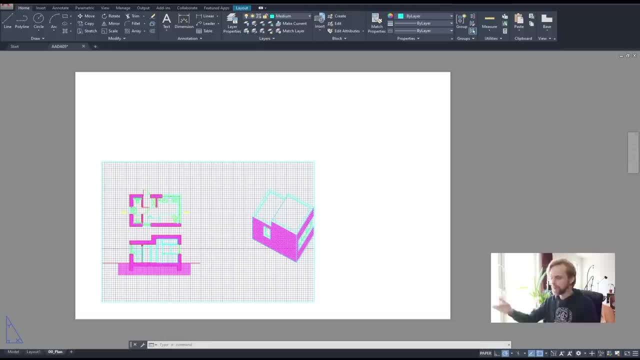 to understand the philosophy of layout. to understand the philosophy of layout, so a layout is a digital a in this case. so a layout is a digital a in this case. so a layout is a digital a- in this case, a3 sheet of paper which has a window in. 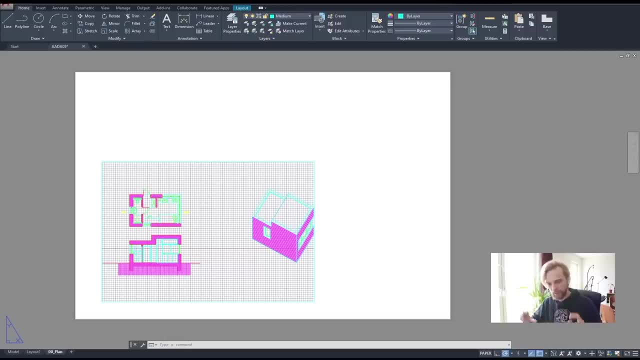 a3 sheet of paper which has a window in. a3 sheet of paper which has a window in it. right, it has like a hole in it and it right, it has like a hole in it and it right, it has like a hole in it. and through that hole you see, you see stuff. 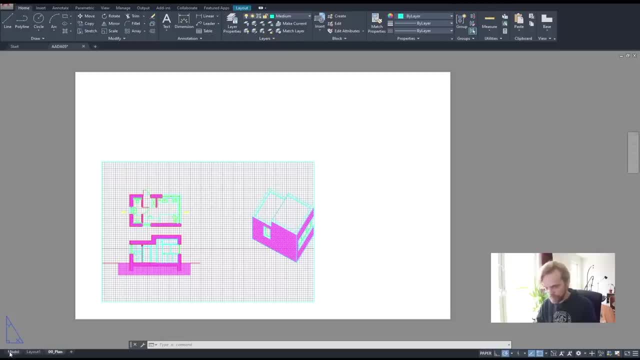 through that hole. you see, you see stuff through that hole. you see, you see stuff that you drew in your model space, right, that you drew in your model space, right, that you drew in your model space, right? so you see this stuff in your layout. so you see this stuff in your layout. 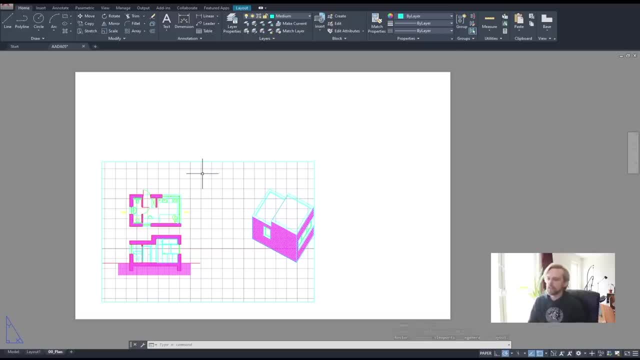 so you see this stuff in your layout, important note, right that this important note right that this important note right that this rectangle right here, rectangle right here, rectangle right here, is the frame of that particular hole, or is the frame of that particular hole or is the frame of that particular hole or that particular window right. so you need. 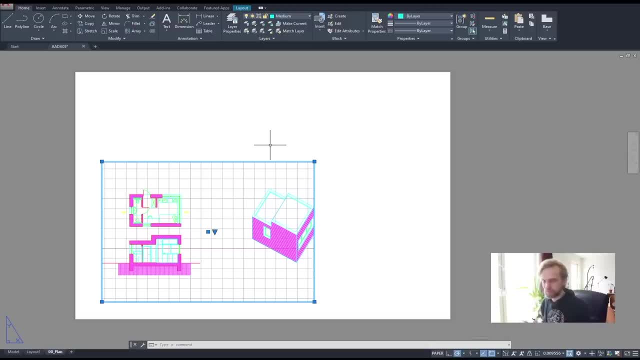 that particular window right. so you need that particular window right. so you need that rectangle to be first of all that rectangle, to be first of all that rectangle, to be first of all properly sized. you know to fill the properly sized. you know to fill the properly sized. you know to fill the the page. 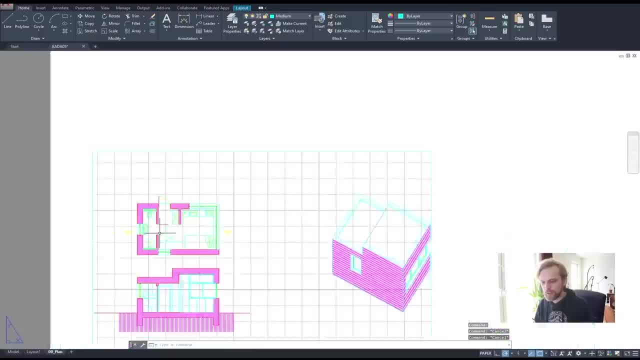 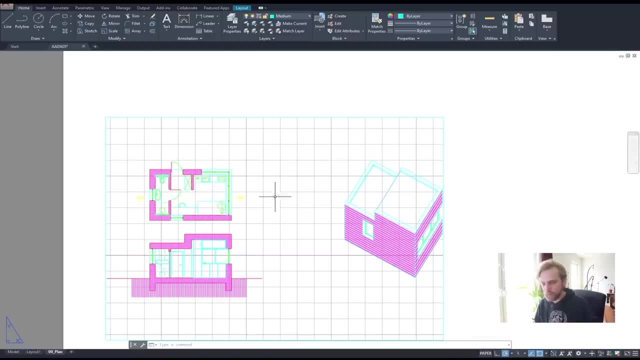 the page, the page, and, second of all, you kind of want to, and, second of all, you kind of want to, and, second of all, you kind of want to understand what's the, what's the scale of understand, what's the, what's the scale of understand, what's the what's the scale of of these elements. because right now, 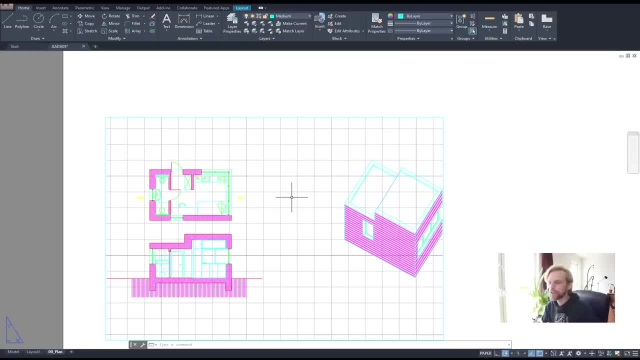 of these elements, because right now of these elements, because right now they're just kind of randomly zoomed in. they're just kind of randomly zoomed in. they're just kind of randomly zoomed in. there's no scale right, so you want to. there's no scale right, so you want to. 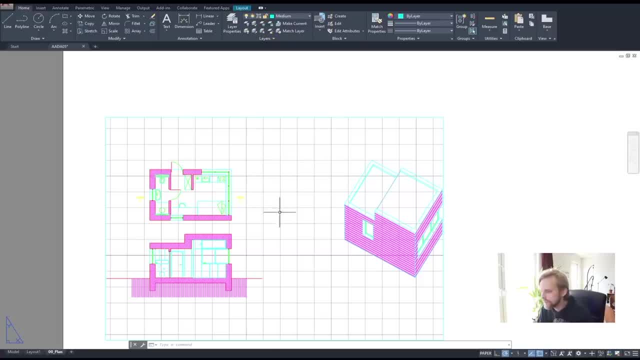 there's no scale right, so you want to have the scale. one more thing that I'm have the scale. one more thing that I'm have the scale. one more thing that I'm gonna do is I am going to before I kind gonna do is I am going to before I kind. 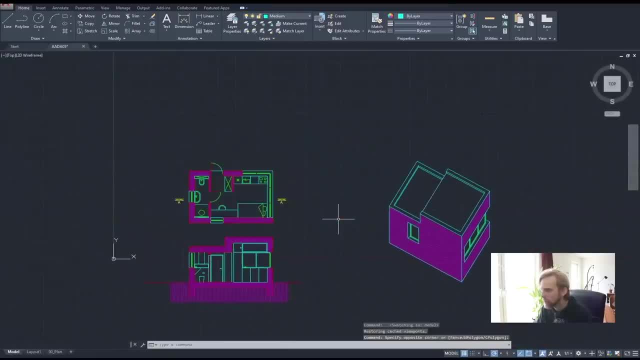 gonna do is I am going to before I kind of continue with the layouts. I'll go to of continue with the layouts. I'll go to of continue with the layouts. I'll go to the model space and I will create some. the model space and I will create some. 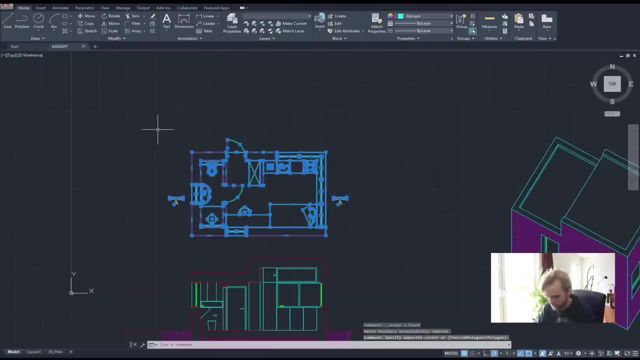 the model space and I will create some room here and of course my hatches will room here and of course my hatches will room here and of course my hatches will not let me, so I'll kind of delete the. not let me, so I'll kind of delete the. 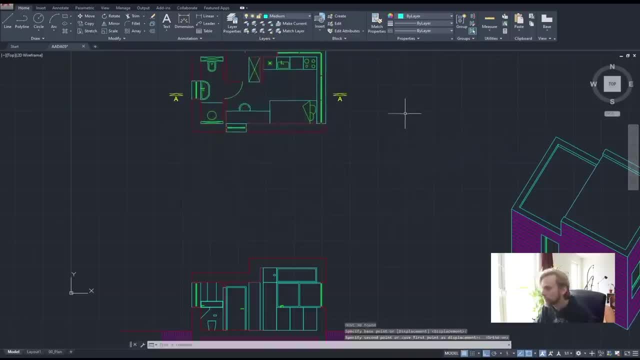 not let me, so I'll kind of delete the hatches for a bit. hatches for a bit. hatches for a bit 8. I'll just create a little bit of 8. I'll just create a little bit of 8. I'll just create a little bit of space between these, just so that when I grab 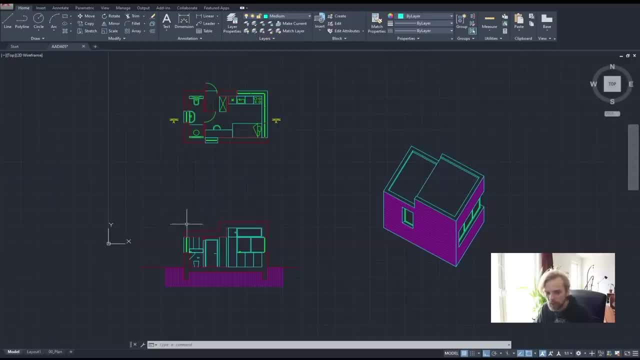 space between these, just so that when I grab space between these, just so that when I grab the view of the plan, it doesn't kind the view of the plan, it doesn't kind the view of the plan, it doesn't kind of grab a little bit of this section. I'll. 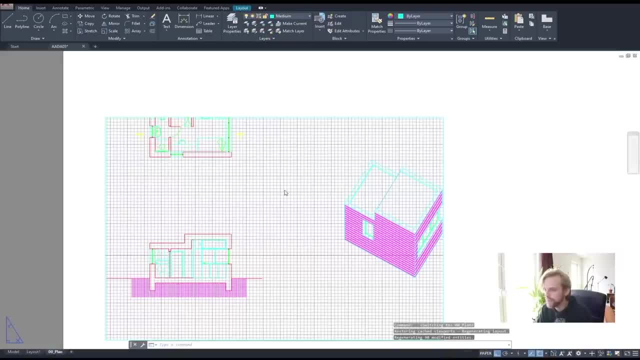 of grab a little bit of this section. I'll of grab a little bit of this section. I'll create the sections of sections. the create the sections of sections. the create the sections of sections. the hatch in just a second for now. let's hatch in just a second for now, let's. 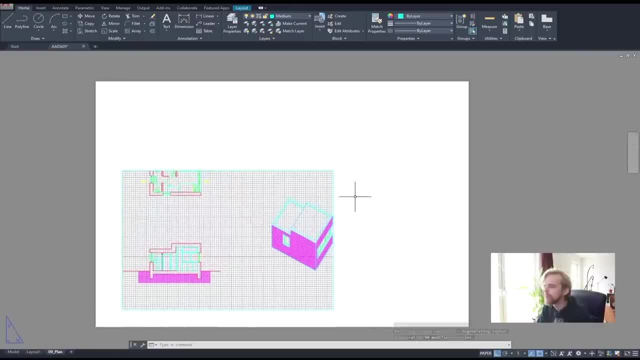 hatch in just a second. for now, let's just keep it, and you can see that it by just keep it, and you can see that it by just keep it, and you can see that it by the way updates here: okay, so first thing. the way updates here: okay, so first thing. 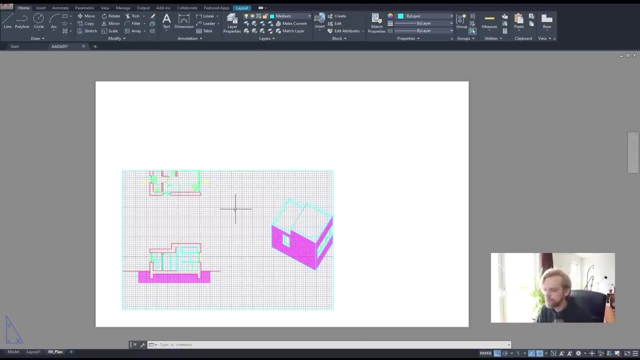 the way updates here. okay, so first thing is understanding that this is a page and is understanding that this is a page and is understanding that this is a page and this is a window into your model space. this is a window into your model space. this is a window into your model space and you had a look. look at your model. 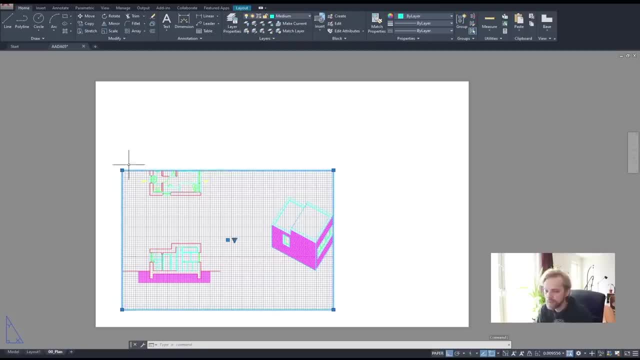 and you had a look look at your model and you had a look look at your model through that window. second, this is this through that window. second, this is this through that window. second, this is this frame, this frame. I kind of want it to frame, this frame. I kind of want it to. 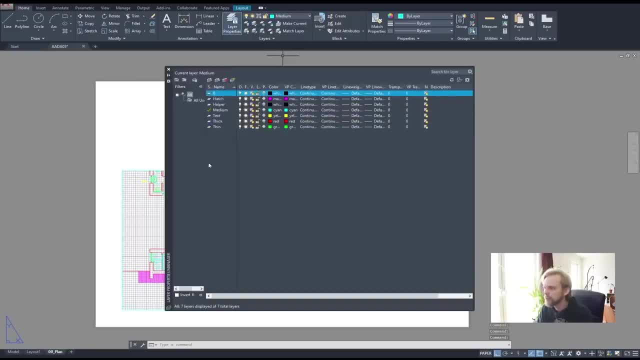 frame, this frame, this frame. I kind of want it to be. let's go to layer be. let's go to layer be. let's go to layer properties. I want it to be in a properties, I want it to be in a properties. I want it to be in a separate, as a separate entity. so I'll 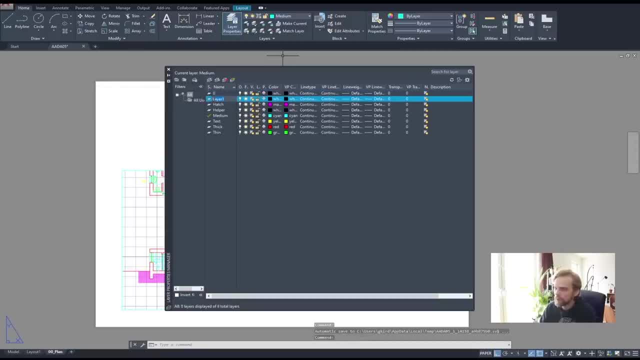 separate as a separate entity. so I'll separate as a separate entity. so I'll create a new layer. I'll call it. I'll create a new layer. I'll call it. I'll create a new layer. I'll call it. I'll call this layer. no print. do not print. 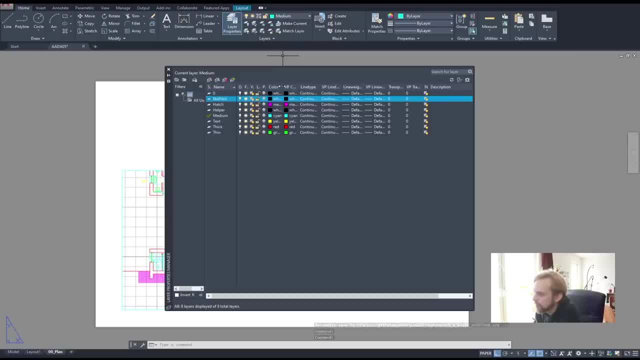 call this layer: no print, do not print. call this layer: no print, do not print. layer and I'll keep it. oh, by the way, layer and I'll keep it. oh, by the way, layer and I'll keep it. oh, by the way, here you can see it says white even. 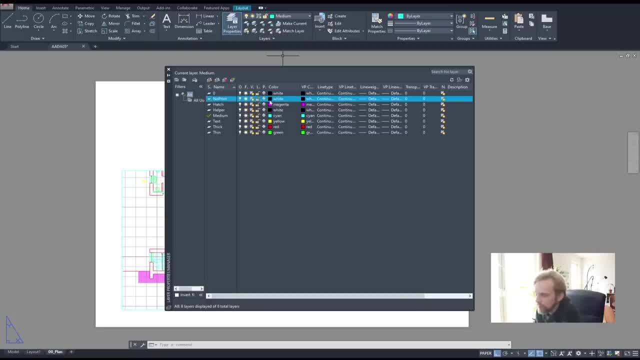 here you can see it says white. even here you can see it says white, even though it shows black. that that is not a though it shows black. that that is not a though it shows black. that that is not a bug. that is how it works, right, so it. 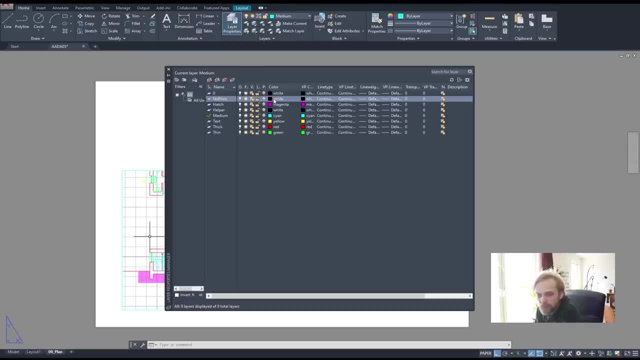 bug. that is how it works right. so it bug. that is how it works right. so it will show up white in the model space, will show up white in the model space, will show up white in the model space, but it will be black as it's printed out. 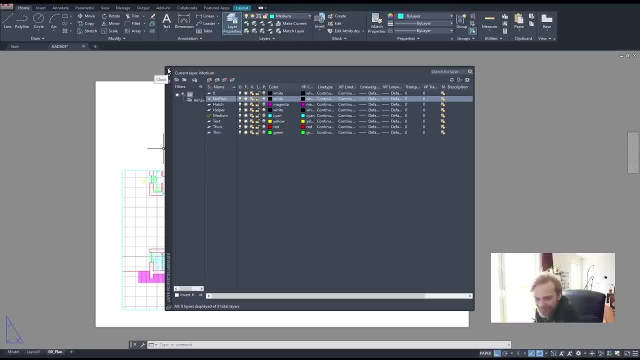 but it will be black as it's printed out. but it will be black as it's printed out. just something that just your AutoCAD. just something that just your AutoCAD. just something that just your AutoCAD. things okay, so this frame right here I. things okay, so this frame right here, I. 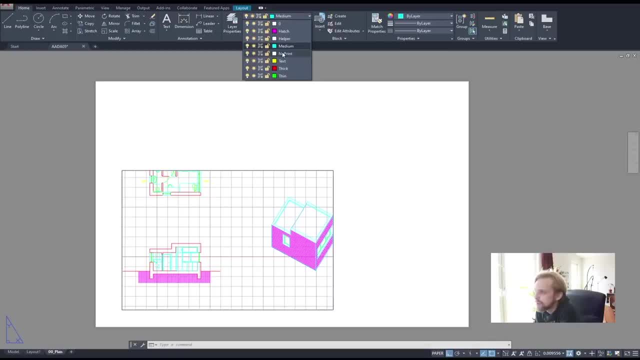 things okay. so this frame right here, I will select it and I will move it to the. will select it and I will move it to the. will select it and I will move it to the. no print layer and the reason why I'm no print layer and the reason why I'm. 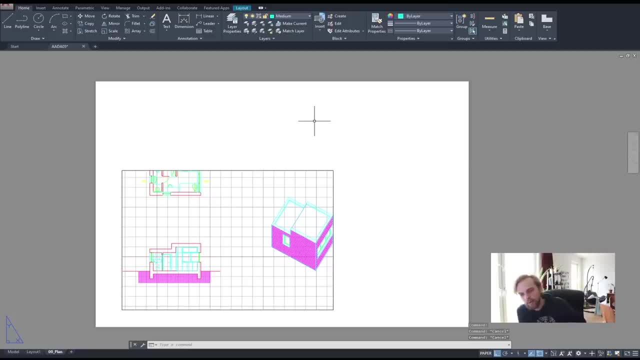 no print layer. and the reason why I'm doing is is because when we are going to doing is is because when we are going to doing is is because when we are going to be printing out the layout, I don't want be printing out the layout. I don't want. 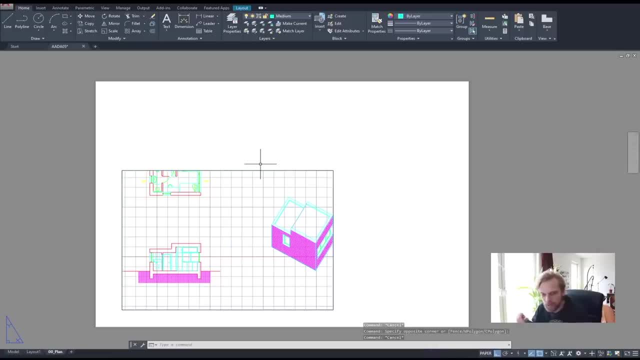 be printing out the layout. I don't want this frame to be visible by the way, this frame to be visible by the way, this frame to be visible by the way, those of you who are thinking, will the those of you who are thinking, will the those of you who are thinking, will the grid be visible? no, no, the grid will not. 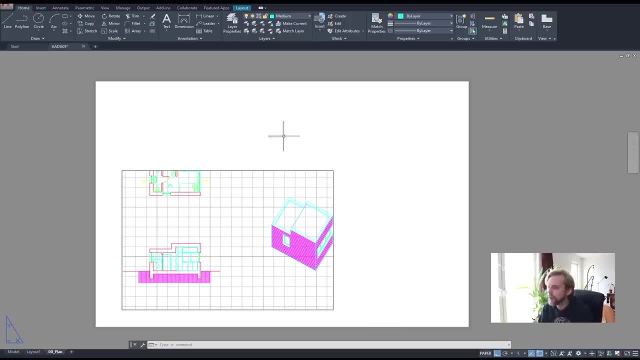 grid be visible. no, no, the grid will not. grid be visible. no, no, the grid will not be visible in the final print. be visible in the final print. be visible in the final print. but I also don't want the frame to be. but I also don't want the frame to be. 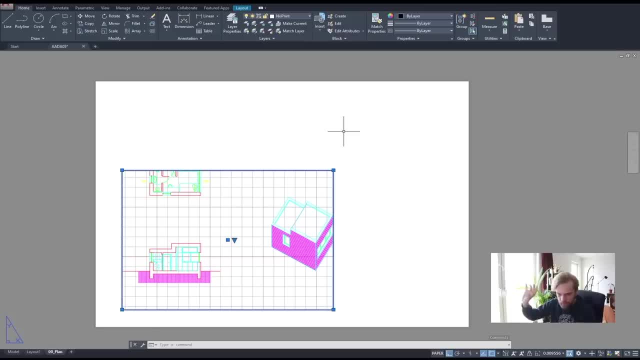 but I also don't want the frame to be visible, so that's why I'm putting it in visible. so that's why I'm putting it in visible, so that's why I'm putting it in the separate layer, and then we will just the separate layer, and then we will just. 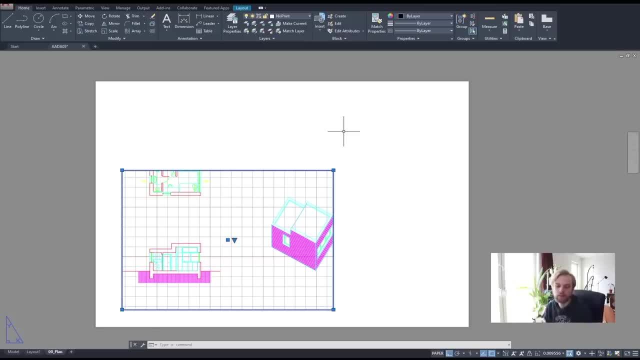 the separate layer, and then we will just make sure that that layer is not being, make sure that that layer is not being, make sure that that layer is not being printed during the printing process, then printed during the printing process, then printed during the printing process. then the next thing is: 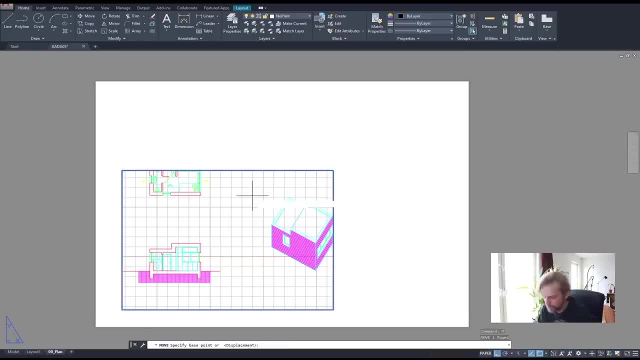 the next thing is. the next thing is: well, let's position this to the center. well, let's position this to the center. well, let's position this to the center so I can just kind of move it around. so I can just kind of move it around. so I can just kind of move it around right, f8 and just move it anywhere. I. 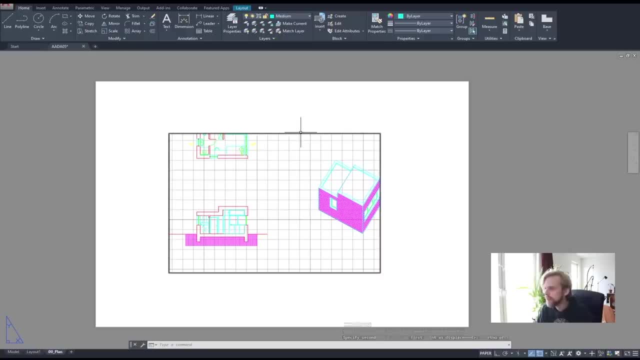 right f8 and just move it anywhere. I right f8 and just move it anywhere. I want this window and now let's make sure want this window and now let's make sure want this window, and now let's make sure that the scale- or not the scale- that we 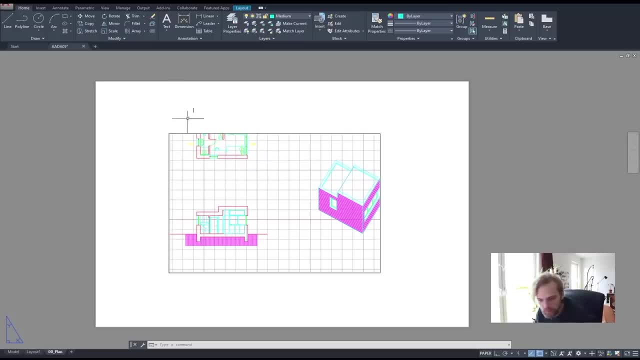 that the scale or not the scale, that we, that the scale or not the scale that we are focused on the plan view are focused on the plan view, are focused on the plan view right in this particular, in this particular right, in this particular, in this particular right, in this particular, in this particular layout. so I'm going to double. 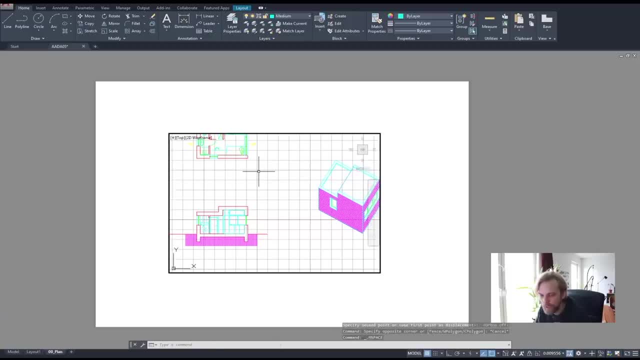 layout. so I'm going to double layout, so I'm going to double click inside of it, double click. and now we are click inside of it, double click, and now we are click inside of it, double click, and now we are not. we can't move around here in. 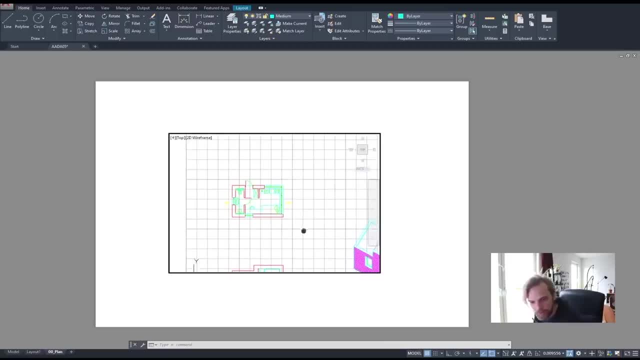 not, we can't move around here in, not, we can't move around here in the layout, but rather we are moving around the layout, but rather we are moving around the layout, but rather we are moving around in the window. so when you double in the window, so when you double, 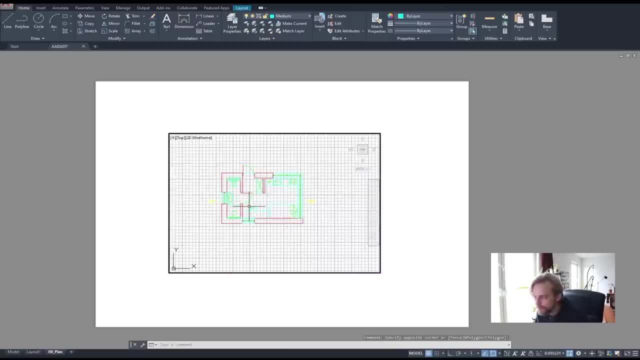 in the window. so when you double click inside, you are then working within the click inside. you are then working within the click inside, you are then working within the window and you can zoom in, zoom out window and you can zoom in, zoom out window and you can zoom in, zoom out, so you can control the positioning here. 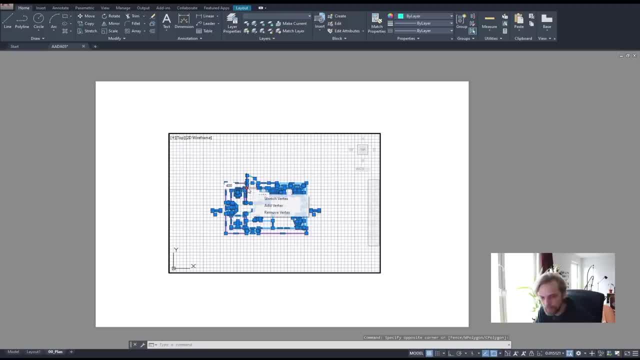 so you can control the positioning here. so you can control the positioning here, right. so what I'm going to do is I will, right. so what I'm going to do is I will, right. so what I'm going to do is I will select my plan and I will type in Z or 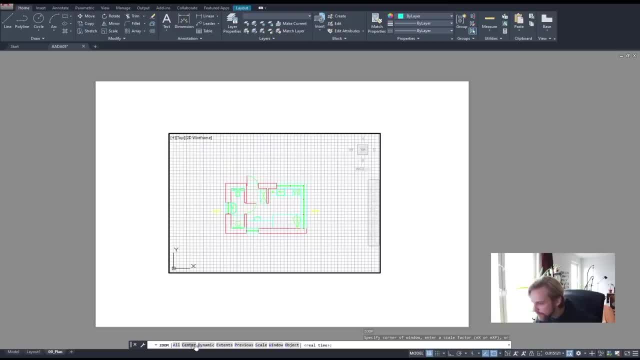 select my plan and I will type in Z or select my plan and I will type in Z or zoom, and then I will here in the bottom zoom, and then I will here in the bottom zoom, and then I will here in the bottom I'll choose object. 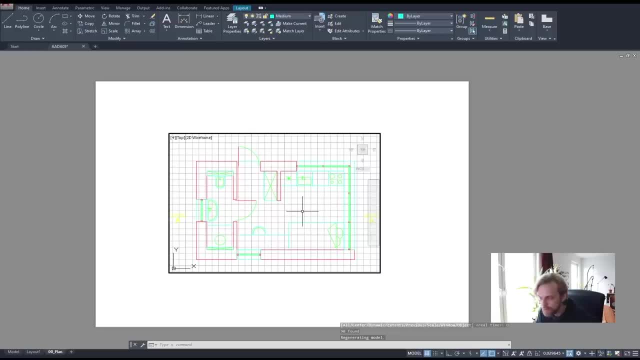 I'll choose object. I'll choose object. so I've just zoomed in to this object. so I've just zoomed in to this object. so I've just zoomed in to this object. right once I've done that, I just double. right, once I've done that, I just double. 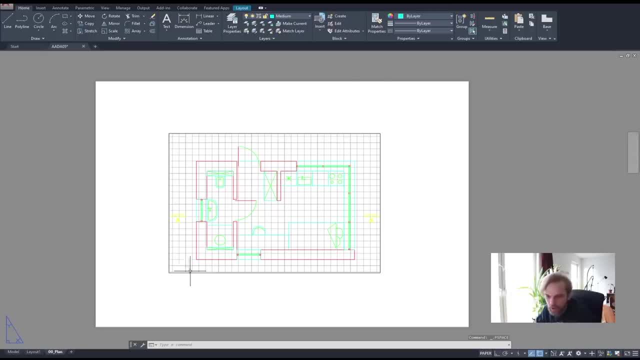 right. once I've done that, I just double click anywhere else- right, it's not click anywhere else. right, it's not click anywhere else. right, it's not inside. and now my layout is focused on inside, and now my layout is focused on inside, and now my layout is focused on this particular or this window, this: 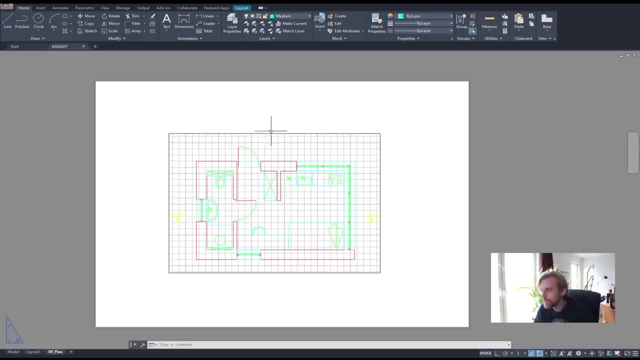 this particular or this window, this, this particular or this window, this layout window is focused on. this layout window is focused on. this layout window is focused on this particular drawing right. that's important. particular drawing right. that's important. particular drawing right. that's important. I will now need to make sure that the 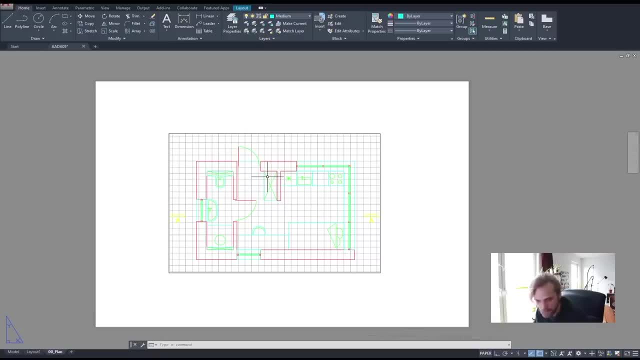 I will now need to make sure that the I will now need to make sure that the scale of this drawing in an a3 page is a scale of this drawing in an a3 page is a scale of this drawing in an a3 page is a correct scale. it's 1 to 100. 1 to 50. 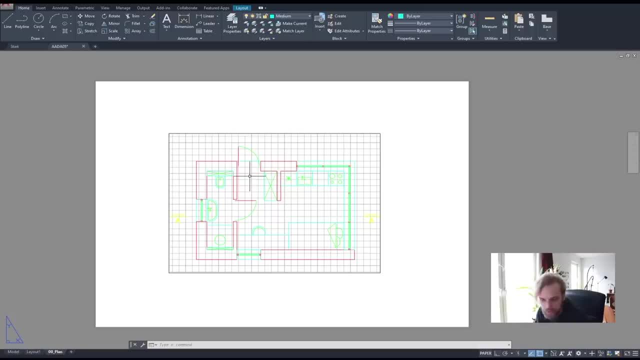 correct scale: it's 1 to 100. 1 to 50. correct scale: it's 1 to 100. 1 to 50. whatever scale, I want it to be right. so, whatever scale, I want it to be right. so, whatever scale, I want it to be right. so how do you change the scale? well, for. 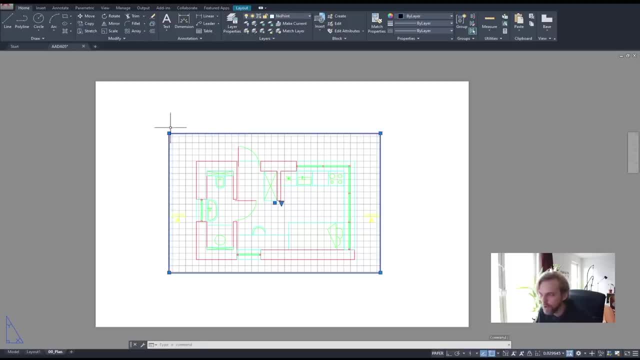 how do you change the scale? well, for how do you change the scale? well, for that you will need to access the. that you will need to access the. that you will need to access the properties of this window frame, so I: properties of this window frame, so I. 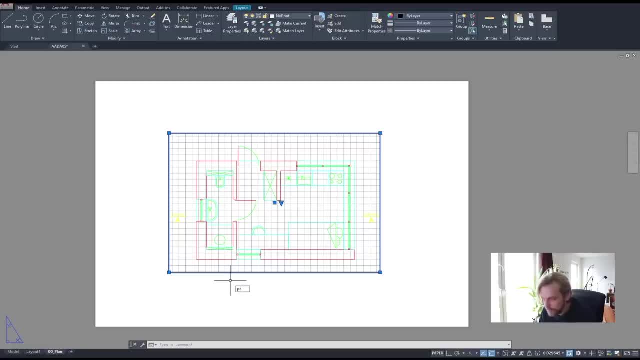 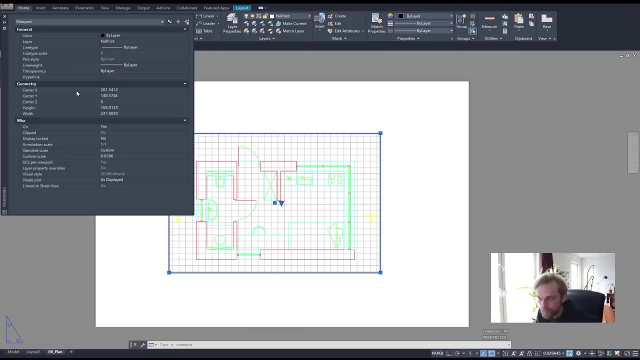 properties of this window frame. so I select this window frame and I type in select this window frame and I type in select this window frame and I type in PR short for properties and hit enter PR short for properties and hit enter PR short for properties and hit enter, it will open up this page for me, or or? 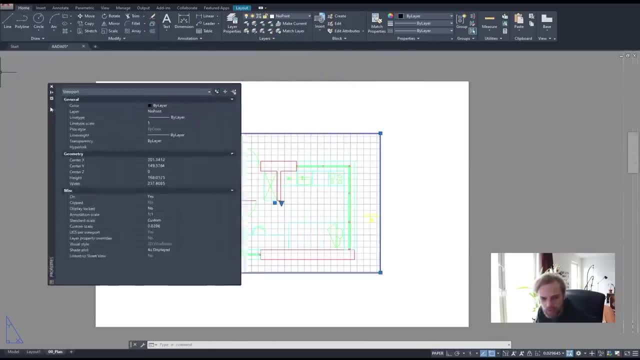 it will open up this page for me, or. or. it will open up this page for me, or or not. page this menu box for me and I'll not page this menu box for me. and I'll not page this menu box for me and I'll position it here and here in the. 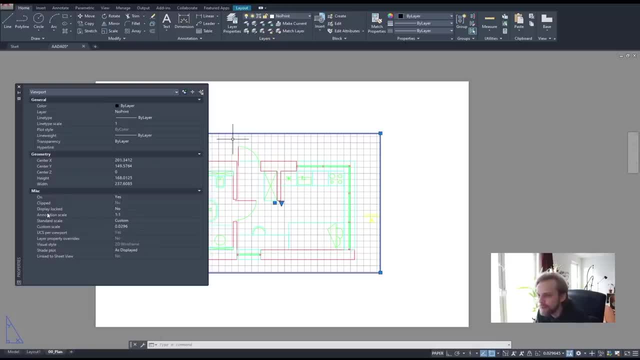 position it here and here. in the position it here and here in the properties: I can see that there is under properties. I can see that there is under properties. I can see that there is under MISC: right here there's standard scale. MISC: right here, there's standard scale. 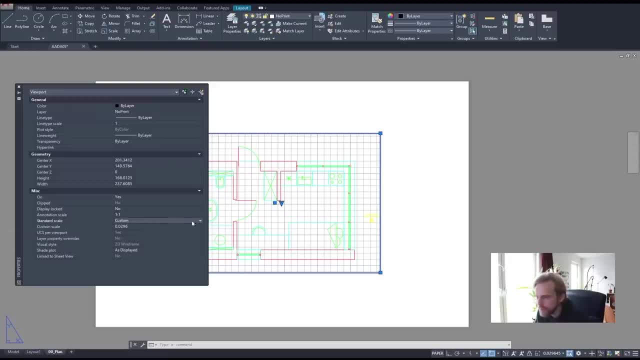 MISC. right here there's standard scale and custom scale, so I'll not be using a and custom scale. so I'll not be using a and custom scale. so I'll not be using a custom scale, rather, I will just expand custom scale. rather, I will just expand. 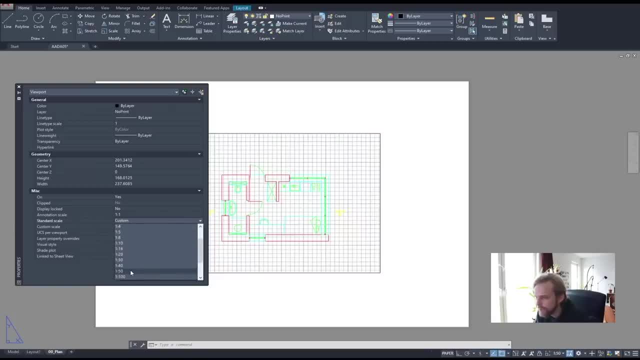 custom scale. rather, I will just expand the standard skill and I'll find the the standard skill and I'll find the the standard skill and I'll find the scale that I want- in this case, probably scale that I want- in this case, probably scale that I want, in this case, probably want to. honestly, 1 to 50 is enough for. 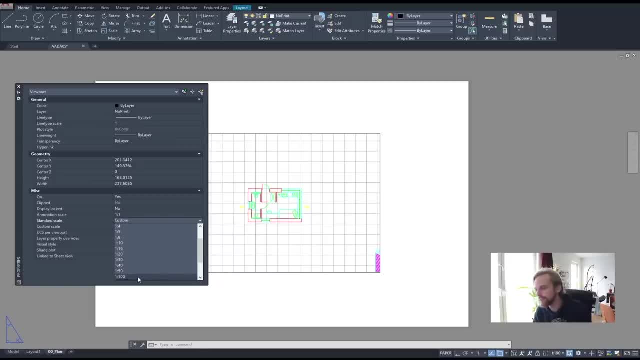 want to, honestly 1 to 50 is enough for want to, honestly 1 to 50 is enough for this kind of a project, like even 1 to a. this kind of a project like even 1 to a, this kind of a project like even 1 to a hundred would be enough, but that's way. 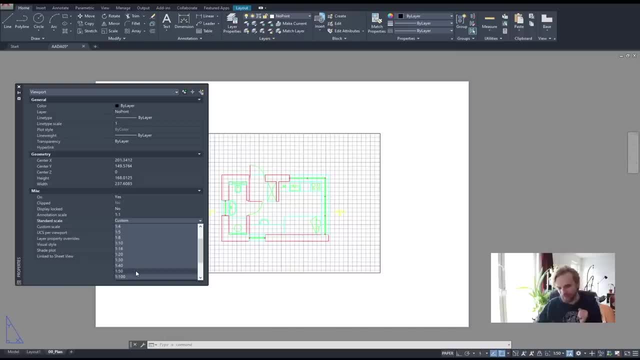 hundred would be enough, but that's way. hundred would be enough, but that's way too small. so instead I'll just use 1 to too small. so instead I'll just use 1 to too small. so instead I'll just use 1 to 50. right for for my scale you could use. 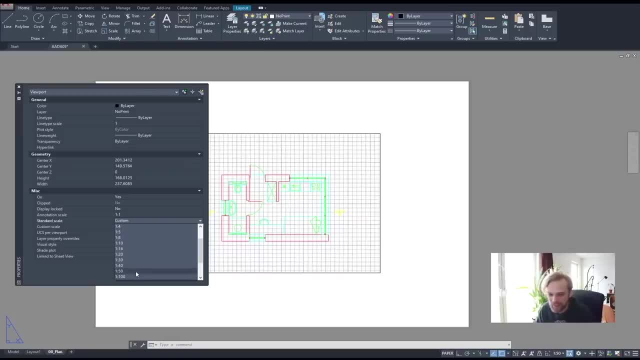 50 right for for my scale. you could use 50 right for for my scale. you could use 1 to 25. that's fine as well, but I'll use 1 to 25. that's fine as well, but I'll use 1 to 25. that's fine as well, but I'll use 1 to 50. 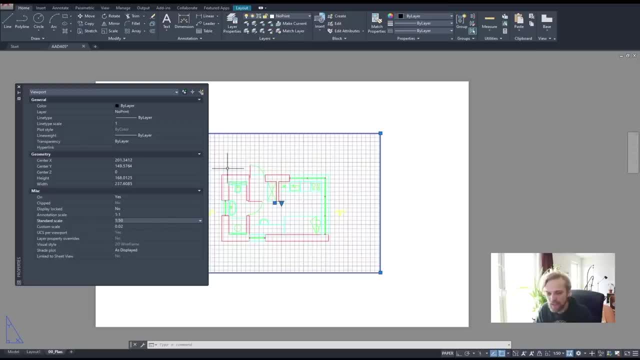 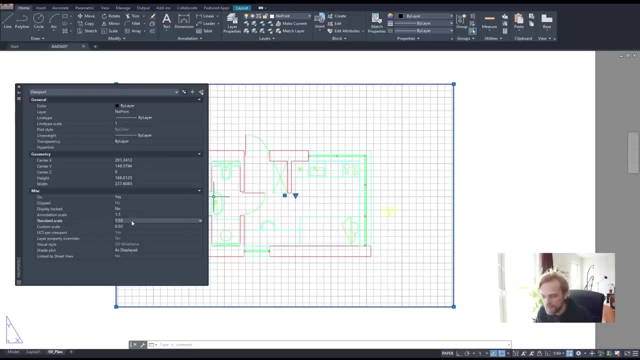 1 to 50. 1 to 50 like that, and now my this particular like that, and now my this particular like that and now my this particular drawing. this drawing right here is at 1 drawing. this drawing right here is at 1 drawing. this drawing right here is at 1 to 50 scale right. 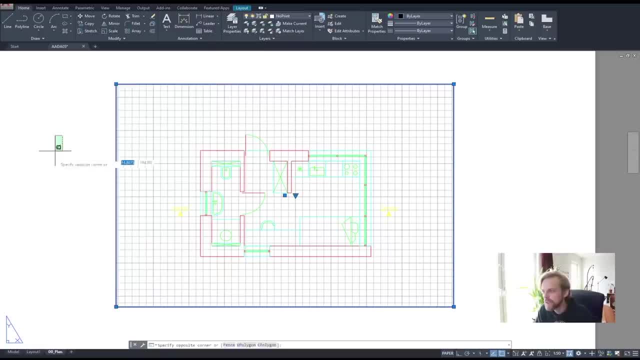 to 50 scale right. to 50 scale right, I will close my properties tab. I will close my properties tab. I will close my properties tab. escape to unselect and from now on I escape to unselect and from now on I escape to unselect and from now on I will not be messing, messing around with. 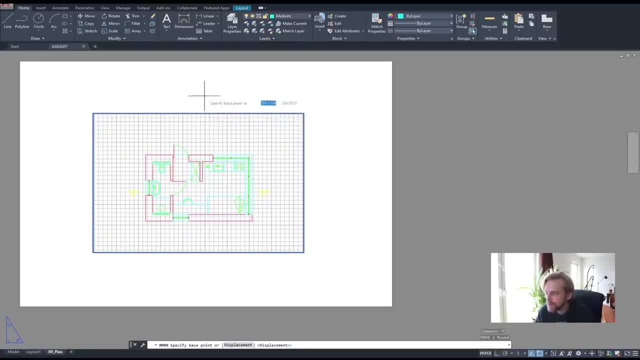 will not be messing messing around with will not be messing messing around with this particular layout. I can still move this particular layout. I can still move this particular layout. I can still move it around. and then, and whatnot right it around, and then, and whatnot right. 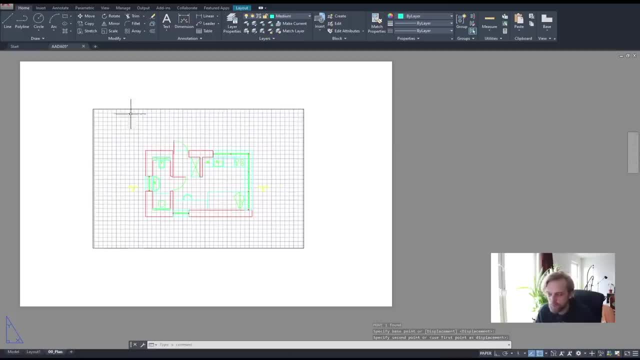 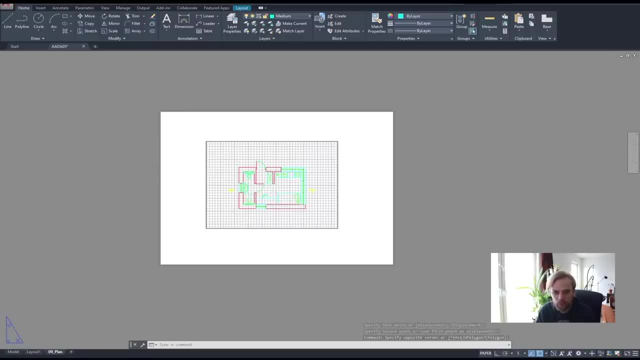 it around and then, and whatnot? right, but I will not be, but I will not be, but I will not be messing around with it now here. if I were messing around with it now here, if I were messing around with it now here, if I were to. 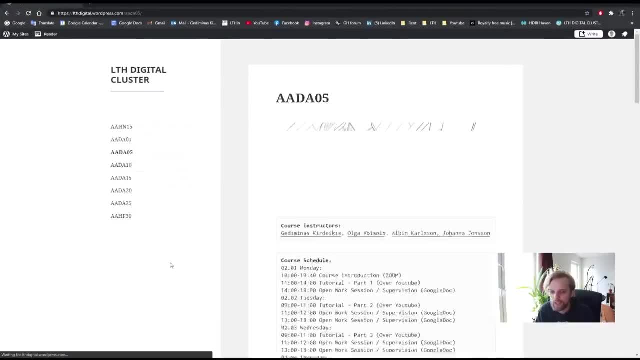 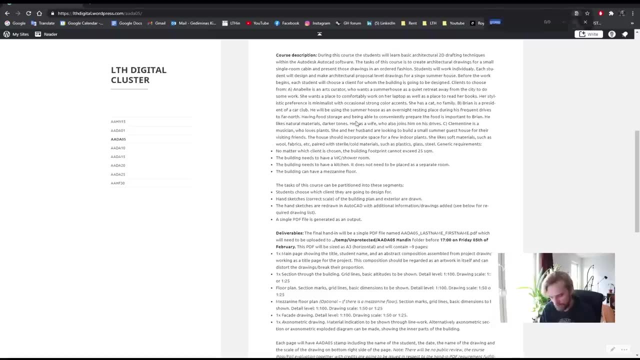 now. if I were to now, if I were to now, if I were to check a d05 requirements of stamp. each page will have a da05 stamp stamp. each page will have a da05 stamp stamp. each page will have a da05 stamp including the name of the student, the. 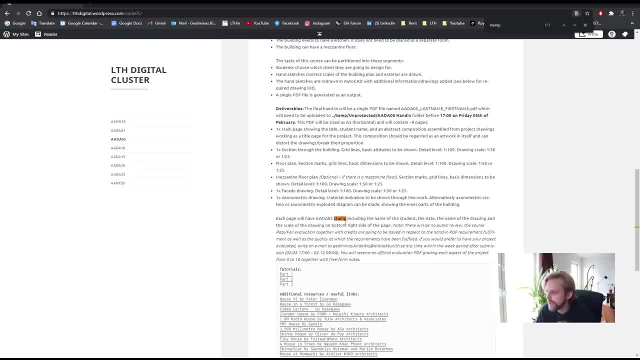 including the name of the student, the including the name of the student, the date, the name of the date, the name of the date, the name of the drawing and the scale of the drawing on bottom right drawing. and the scale of the drawing on bottom right drawing and the scale of the drawing on bottom right side of the page. okay, bottom right side of. 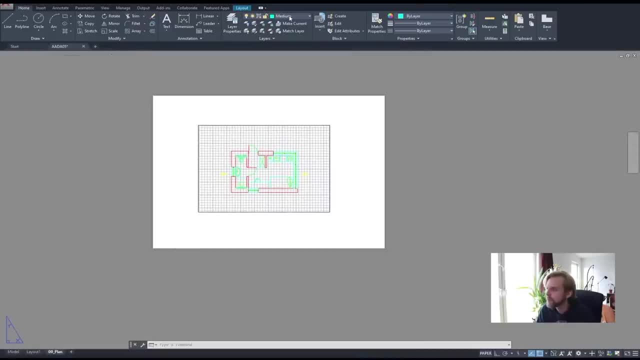 side of the page. okay, bottom right side of side of the page: okay, bottom right side of the page, we need a stamp. so what I'm the page, we need a stamp. so what I'm the page, we need a stamp. so what I'm going to do is I will create, do we? 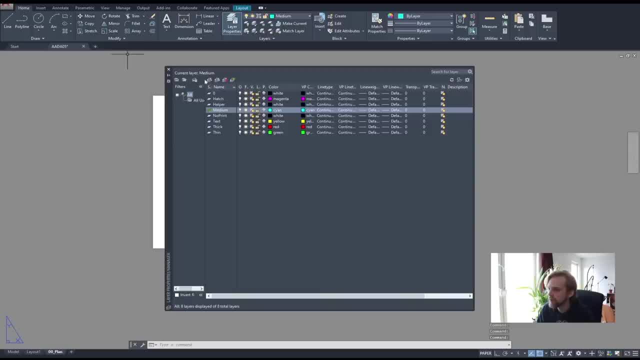 going to do is I will create. do we going to do is I will create? do we create one more layer? yeah, let's create. create one more layer. yeah, let's create. create one more layer. yeah, let's create one more layer and I'll call it layout. 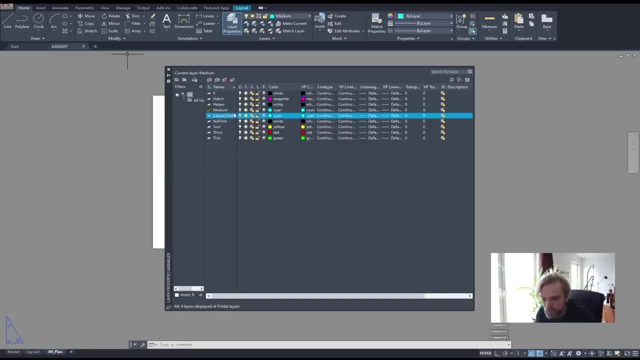 one more layer and I'll call it layout. one more layer and I'll call it layout, text, layout text, and I'll make it just text, layout text, and I'll make it just text, layout text, and I'll make it just white color. by the way, there are two. 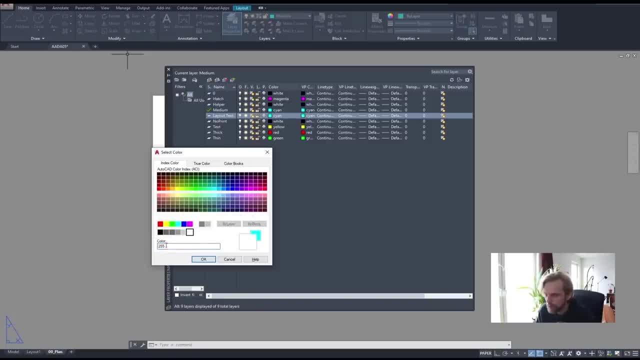 white color. by the way, there are two white color, by the way, there are two white colors. this one right here, which white colors. this one right here, which white colors. this one right here, which is 255- it's gonna say 255 here- and is 255, it's gonna say 255 here. and 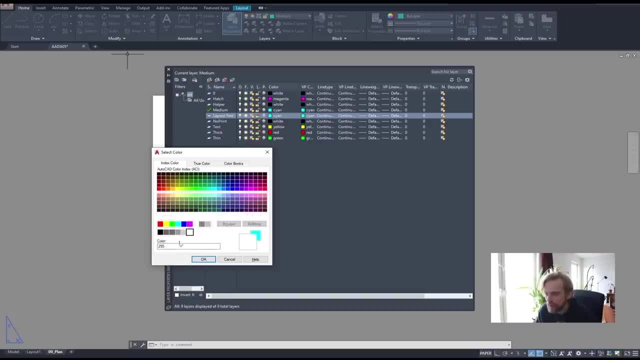 is 255, it's gonna say 255 here. and there's this one here that's gonna say: there's this one here that's gonna say: there's this one here that's gonna say white, this one, the 255 one, is going to white, this one, the 255 one, is going to. 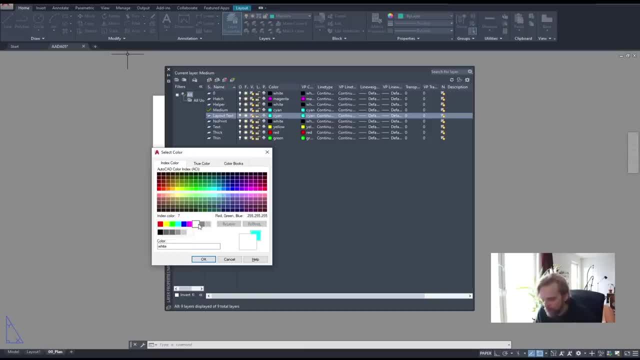 white. this one, the 255 one, is going to be printed out white. this one the one be printed out white. this one, the one, be printed out white. this one, the one that says white, will be printed out. that says white will be printed out. that says white will be printed out black. okay, 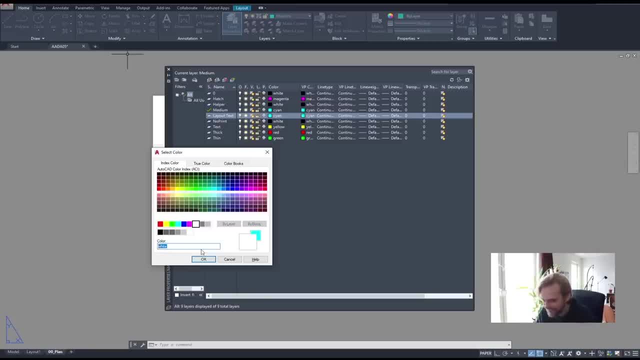 rewind if you need it, if you need to rewind, if you need it, if you need to rewind, if you need it, if you need to, and then listen to this again, I'll just, and then listen to this again. I'll just, and then listen to this again. I'll just say: okay, so we're using the white, that's. 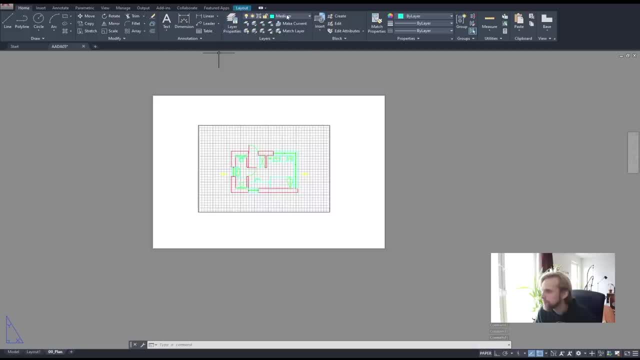 say okay, so we're using the white. that's say okay, so we're using the white. that's going to be printed out as black escape. going to be printed out as black escape. going to be printed out as black escape, and I'll just choose this layout text as: 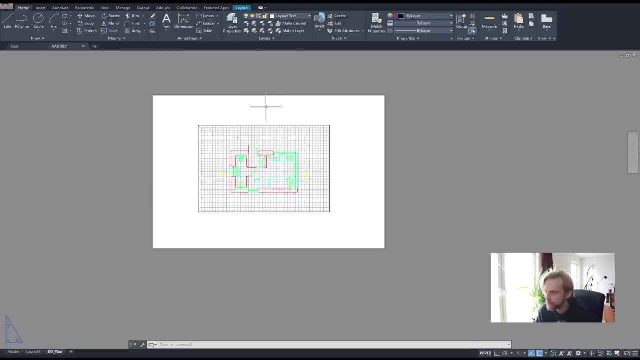 and I'll just choose this layout text as- and I'll just choose this layout text as my current layer, current current layer, my current layer, current current layer, my current layer, current, current layer, in which I draw and I'll kind of start, in which I draw and I'll kind of start. 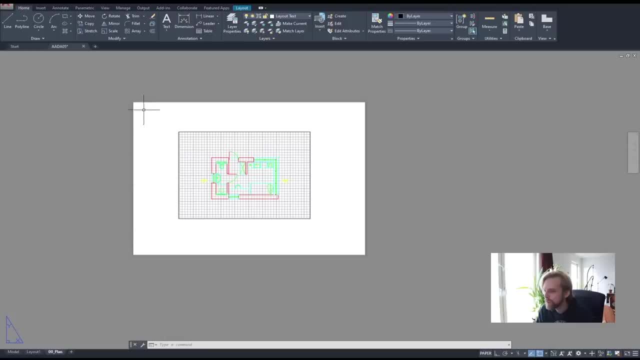 in which I draw and I'll kind of start going to town on this. so the first thing going to town on this, so the first thing going to town on this, so the first thing of the page, so I'm just going to first of the page, so I'm just going to first. 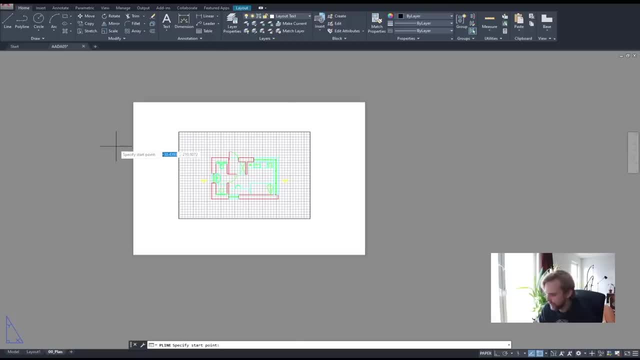 of the page. so I'm just going to first draw out an a3 page- well, that's not zero. draw out an a3 page: well, that's not zero. draw out an a3 page: well, that's not zero. zero coordinates. that's weird. why zero coordinates? that's weird, why. 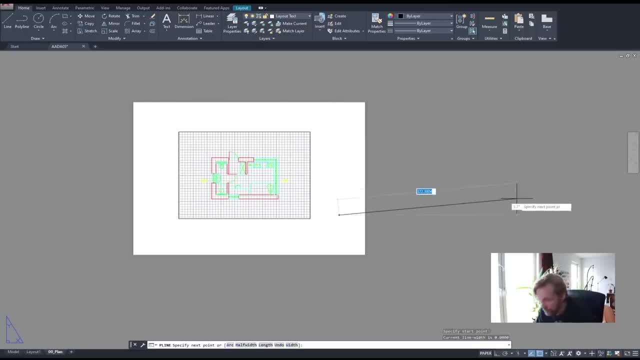 zero coordinates. that's weird. why, whatever doesn't matter, I'll just draw. whatever doesn't matter, I'll just draw whatever doesn't matter. I'll just draw out an a3 page and it's drawn at one to out an a3 page and it's drawn at one. to 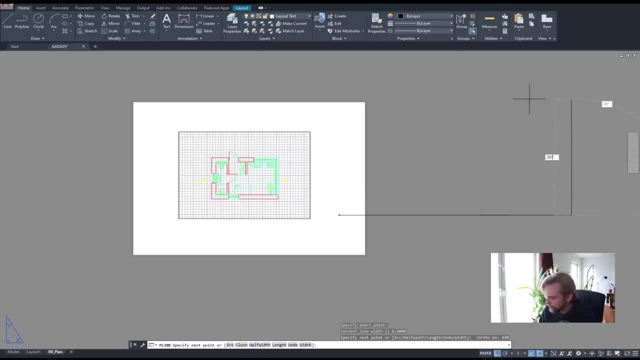 out an a3 page and it's drawn at one to one scale, by the way. so it's 420 one scale, by the way. so it's 420 one scale, by the way. so it's 420 millimeters by 297 millimeters by 420, by. 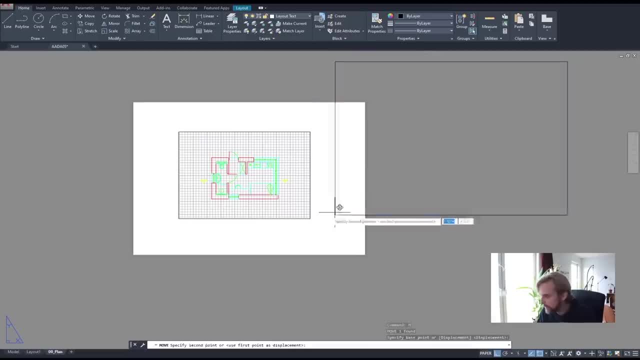 millimeters by 297 millimeters by 420 by millimeters by 297. millimeters by 420 by 297. right like that, I'll just move it 297. right like that, I'll just move it 297. right like that, I'll just move it kind of close, close to the bottom left. 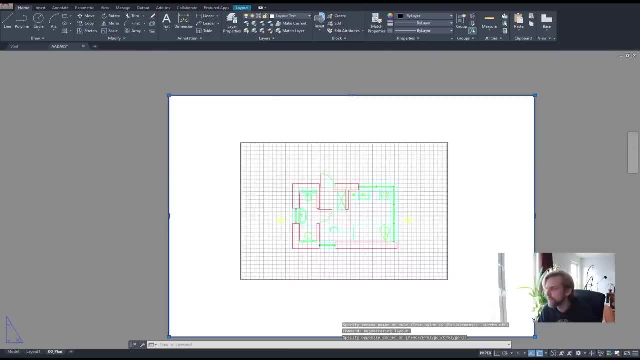 kind of close, close to the bottom left, kind of close, close to the bottom left corner, like so so that it it fits with corner, like so so that it it fits with corner, like so so that it it fits with the page that we have here. doesn't need 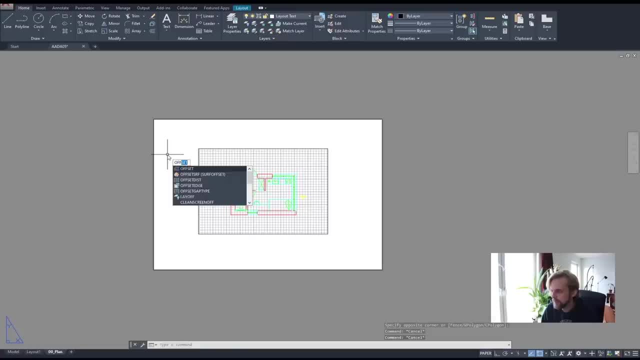 the page that we have here doesn't need the page that we have here doesn't need to be perfect. that's fine, and now I will to be perfect. that's fine, and now I will to be perfect. that's fine, and now I will offset this, this line here, by 10. 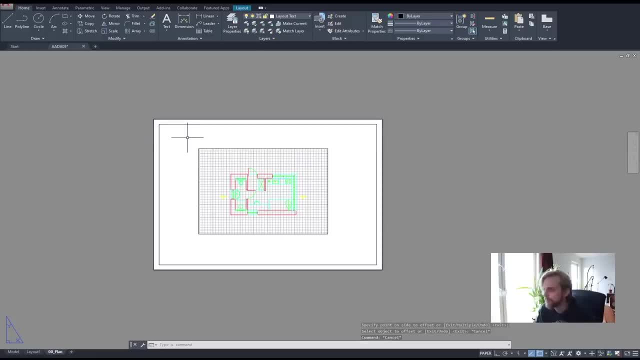 offset this, this line here, by 10. offset this, this line here, by 10 millimeters. yes, that's gonna be one millimeters. yes, that's gonna be one millimeters. yes, that's gonna be one centimeter. that's enough by one centimeter. that's enough by one. 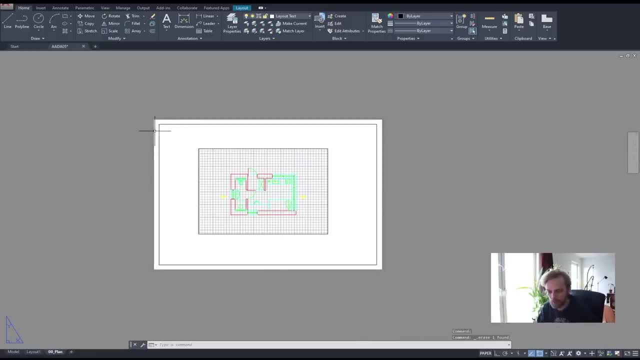 centimeter. that's enough by one centimeter. so now I have the inner centimeter. so now I have the inner centimeter. so now I have the inner bracket and I don't need an old one of bracket and I don't need an old one of. 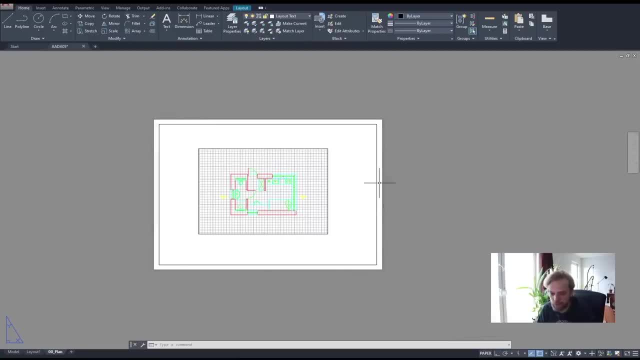 bracket, and I don't need an old one of like this. this gap is always one like this. this gap is always one like this. this gap is always one centimeter from the side of the page and centimeter from the side of the page and centimeter from the side of the page, and I can use it for placing of my, of my. 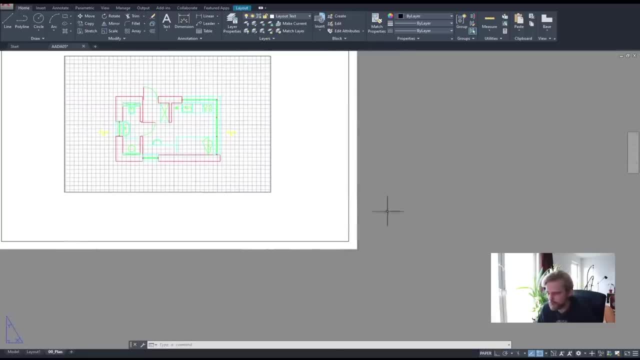 I can use it for placing of my, of my. I can use it for placing of my, of my stamp. so the stamp is basically just a stamp. so the stamp is basically just a stamp. so the stamp is basically just a bunch of information about the project. bunch of information about the project. 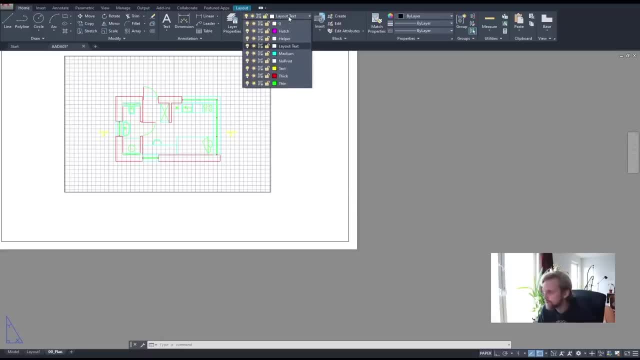 bunch of information about the project, about the drawing, and I'm going to be about the drawing and I'm going to be about the drawing and I'm going to be quite quick about this because there's quite quick about this, because there's quite quick about this because there's nothing smart right? so I'm still in the 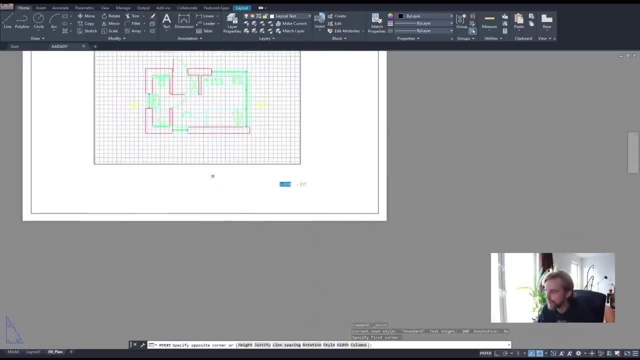 nothing smart, right? so I'm still in the nothing smart, right? so I'm still in the layout text and I'm going to write, write layout text and I'm going to write, write layout text and I'm going to write, write some text actually, right? so I'm gonna. 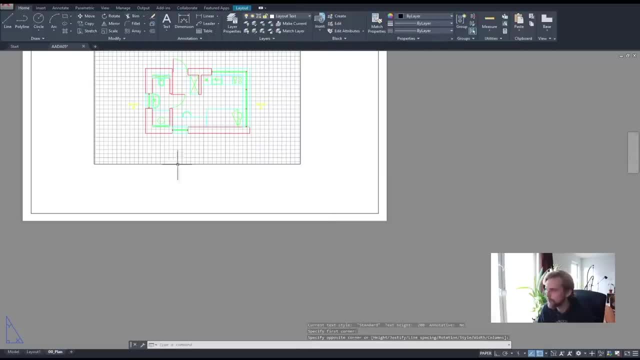 some text actually right, so I'm gonna some text actually right, so I'm gonna start writing here. maybe that's a little start writing here. maybe that's a little start writing here. maybe that's a little bit too fast. T enter short for text. bit too fast. T enter short for text. 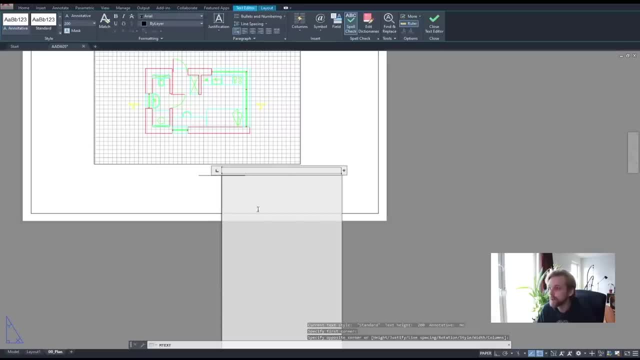 bit too fast. T enter short for text. specify first corner. specify second. specify first corner. specify second. specify first corner. specify second corner. probably change the height of it corner. probably change the height of it corner. probably change the height of it from 200 millimeters to something a. 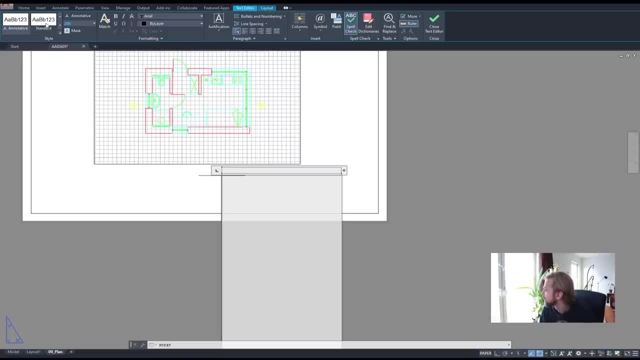 from 200 millimeters to something a, from 200 millimeters to something a little bit less, little bit less, little bit less. so things that are less than three, so things that are less than three, so things that are less than three millimeters, depending on the font- are: 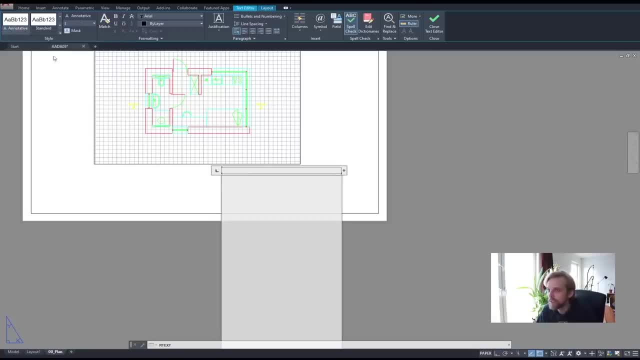 millimeters, depending on the font, are millimeters, depending on the font, are becoming harder and harder to read, so becoming harder and harder to read, so becoming harder and harder to read. so I'm gonna say three millimeters. why is I'm gonna say three millimeters? why is? 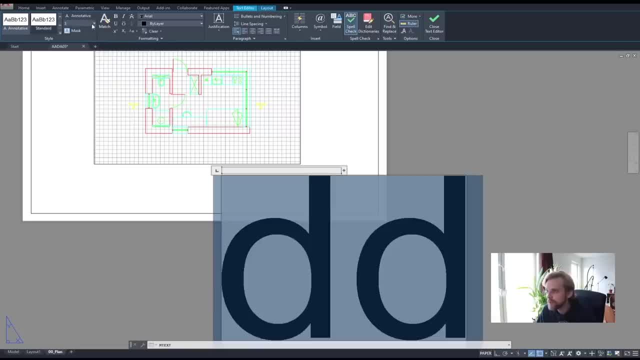 I'm gonna say three millimeters. why is this not updating DD, this not updating DD, this not updating DD? you are user, are not updating at all. you are user are not updating at all. you are user are not updating at all. that's that is strange, okay. 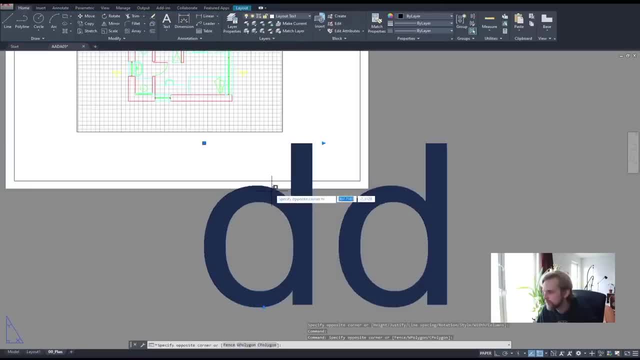 that's, that is strange. okay, that's, that is strange. okay, let me try again, select this text, and I let me try again select this text and I let me try again select this text and I double-click you now. I can't. double-click you now, I can't. 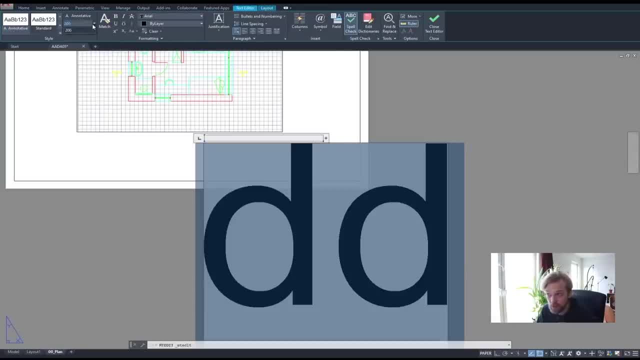 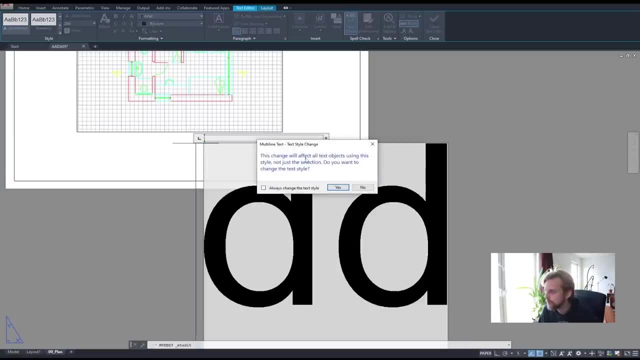 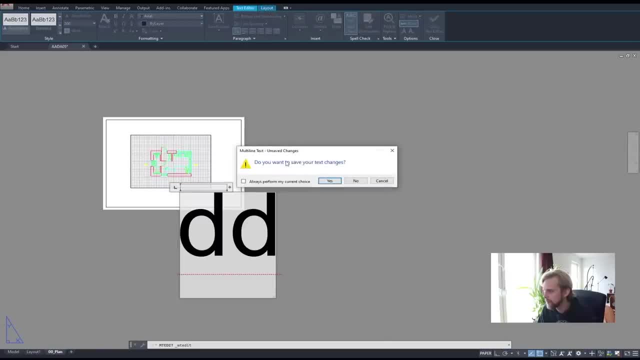 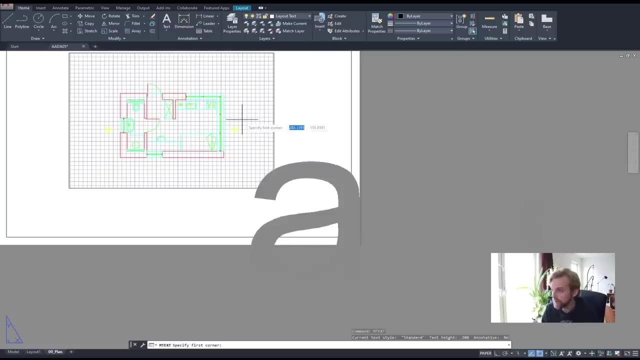 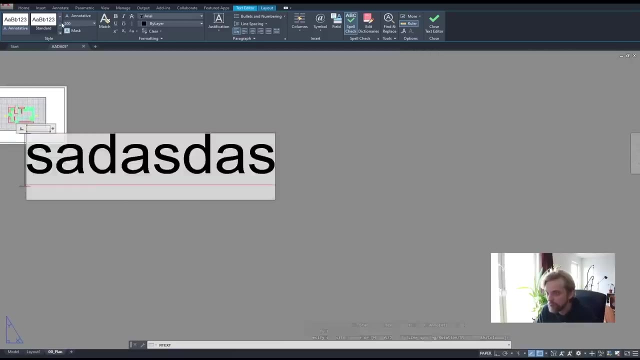 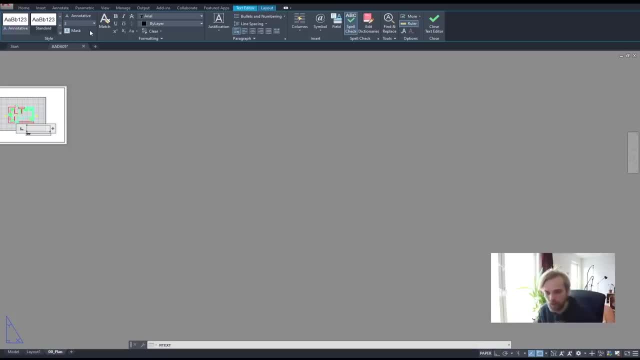 this is a little bit too big, isn't it? this is a little bit too big, isn't it? but for some reason, it oh it, well, but for some reason, it oh it, oh it, oh, but for some reason it oh it, oh well. there's some, some issues here and there. 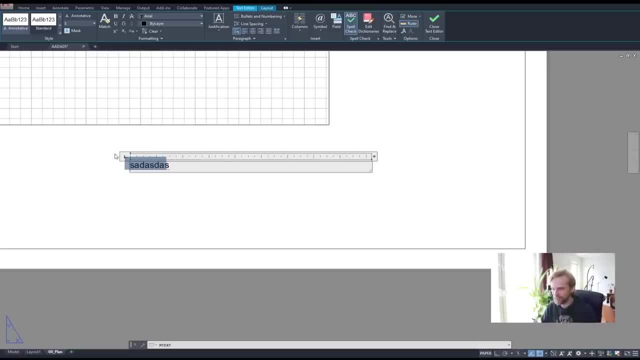 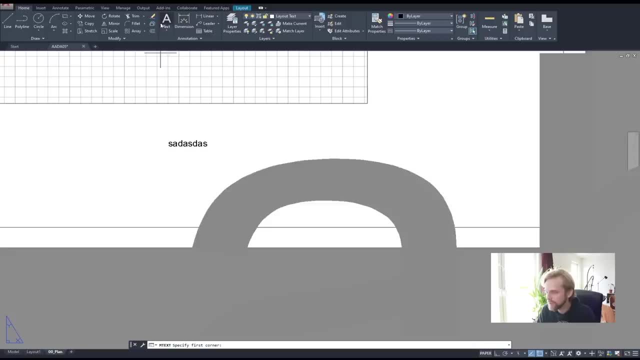 well, there's some some issues here and there. well, there's some some issues here and there with with that, with with that, with with that, without together, I guess, so now it works without together. I guess, so now it works without together. I guess, so now it works. let me just just to make sure that this: 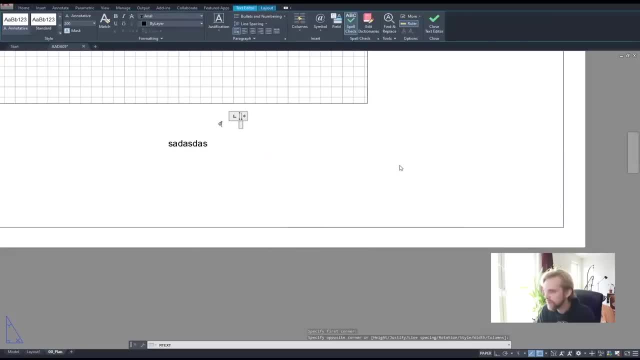 let me just just to make sure that this, let me just just to make sure that this will work as well, let me try. will work as well. let me try, will work as well. let me try. now it says 200. now it says 200. now it says 200. I change this to 3. 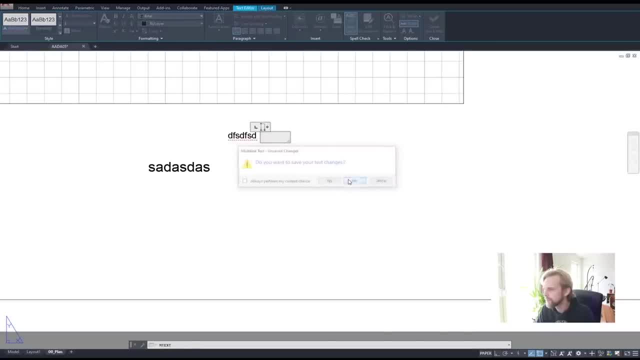 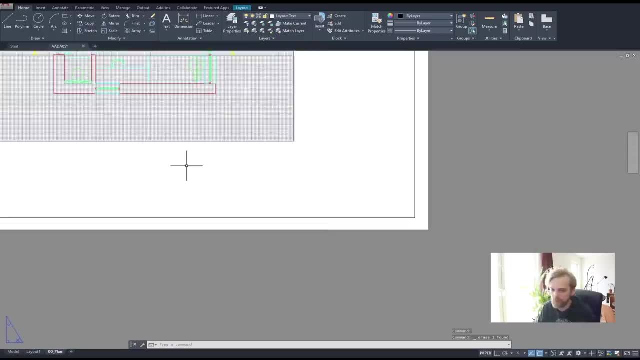 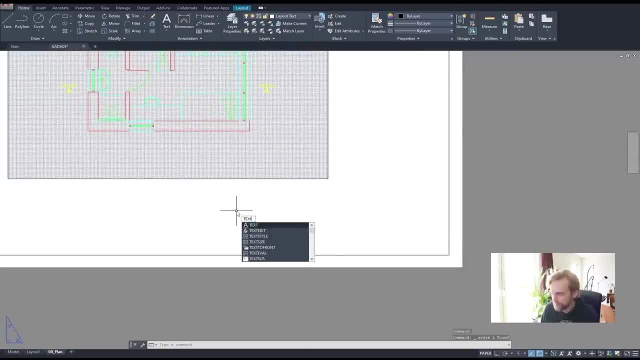 let's do this again and now let's do. let's do this again and now let's do this, this, this cleanly, I guess text text specify cleanly. I guess text text specify cleanly. I guess text text specify start point of text. let's see from here: start point of text. let's see from here. 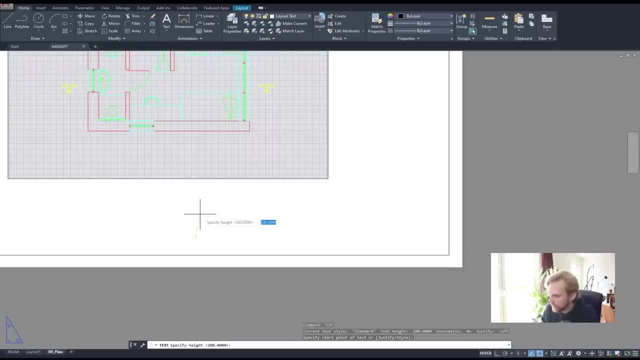 start point of text. let's see from here. specify height, so I will specify 5. specify height, so I will specify 5. specify height, so I will specify 5 millimeters in height. specify rotation millimeters in height. specify rotation millimeters in height. specify rotation angle 0. 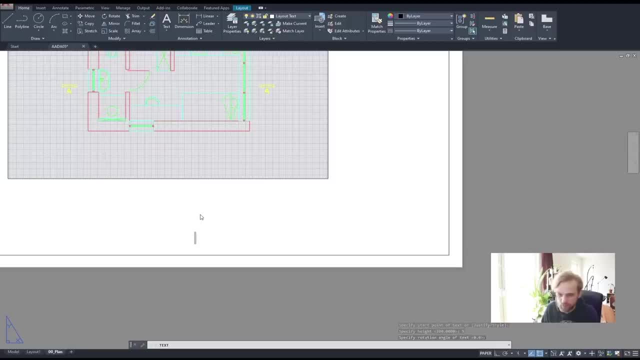 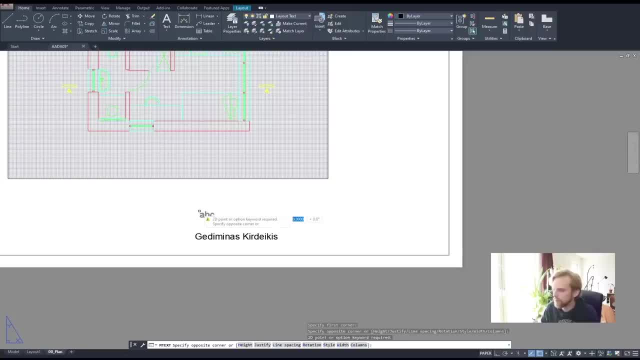 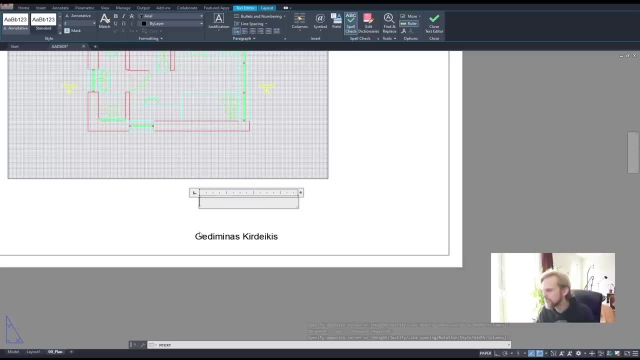 key enter first corner, um, and I will here: key enter first corner, um. and I will here. I'll just say: and here it's doing another thing, and here it's doing another thing, and here it's doing another thing, whatever name that's, that's going to be. 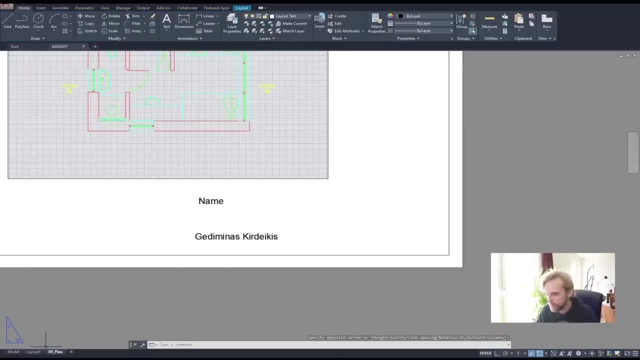 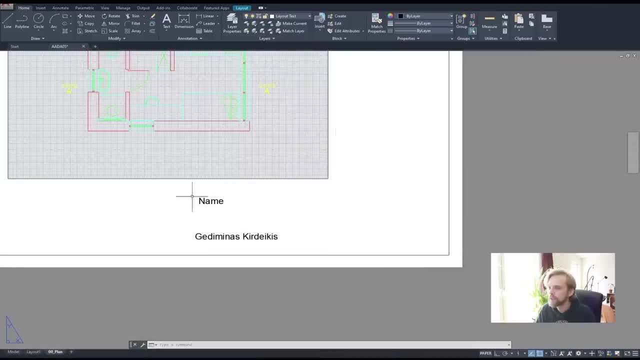 the date, the name of the drawing and the: the date, the name of the drawing and the. the date, the name of the drawing and the scale of the drawing: okay, scale of the drawing. okay, scale of the drawing. okay, so I, I still need some things, and so I I still need some things, and 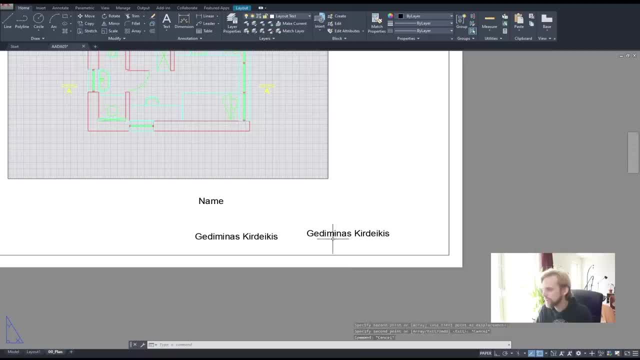 so I I still need some things and, honestly, once I have one text object, I, honestly, once I have one text object, I, honestly, once I have one text object, I just kind of like to make copies of it, just kind of like to make copies of it, just kind of like to make copies of it and just like double click on it and 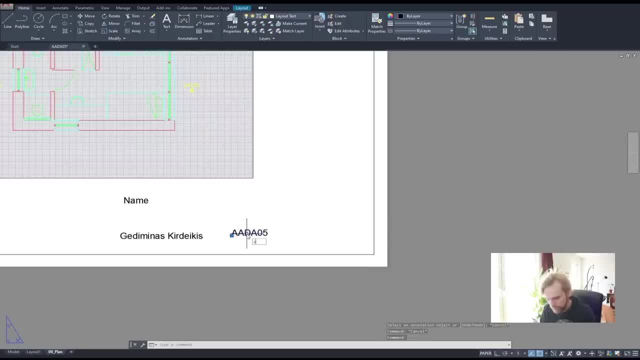 and just like double click on it and and just like double click on it and write what I need to write, so ad05. we write what I need to write, so ad05- we write what I need to write, so ad05- we will have, will have, will have the date, and I know this is not the 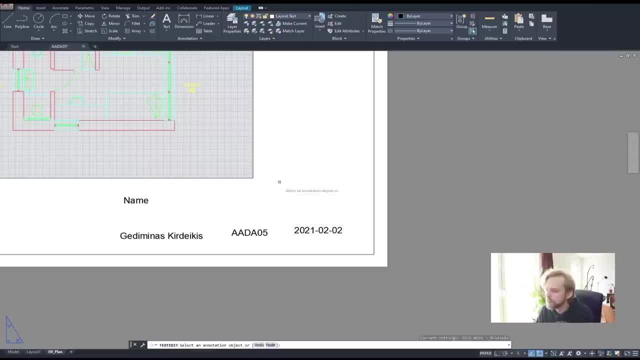 the date and I know this is not the. the date and I know this is not the: 2021-02-02: 2021-02-02, 2021-02-02- um. I know that this is not the cleanest, um, I know that this is not the cleanest. 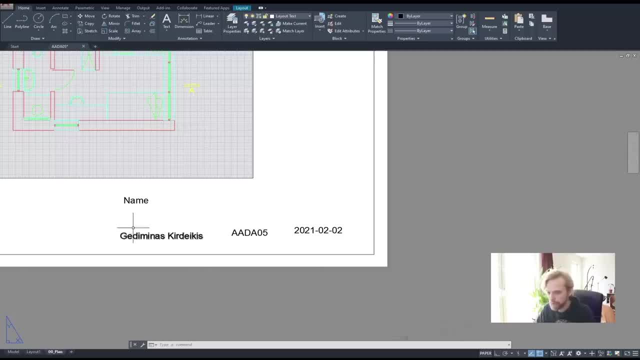 um, I know that this is not the cleanest way of how to do it, way of how to do it, way of how to do it, but whatever works for you, there's. but whatever works for you, there's. but whatever works for you there's. there's no rule in how you need to. 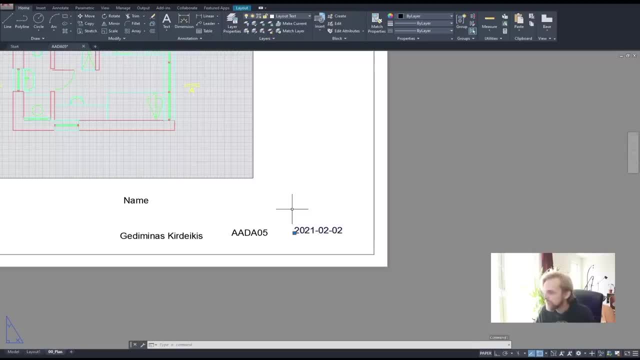 there's no rule in how you need to, there's no rule in how you need to draw it, draw it, draw it, um, um, um, and then there's going to be, and then there's going to be, and then there's going to be title, and yeah, whatever. 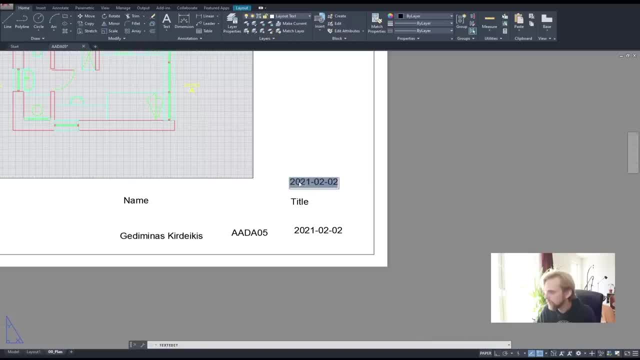 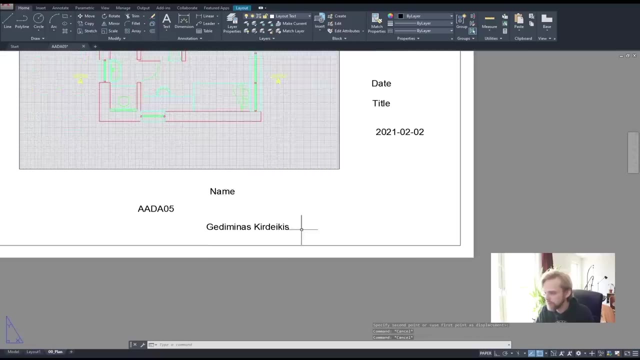 title, and yeah, whatever title, and yeah, whatever title, and date and date and date, okay, okay, okay. so now let's make some. so now let's make some. so now let's make some some adjustments, right, we need to put some adjustments right. we need to put some adjustments right. we need to put all of this information into, into this. 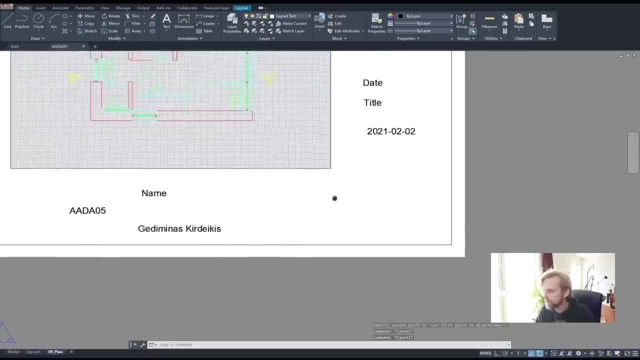 all of this information into into this. all of this information into into this corner right here, in a kind of corner, right here, in a kind of corner right here, in a kind of nice, nice way. so I'm going to draw, nice, nice way, so I'm going to draw. 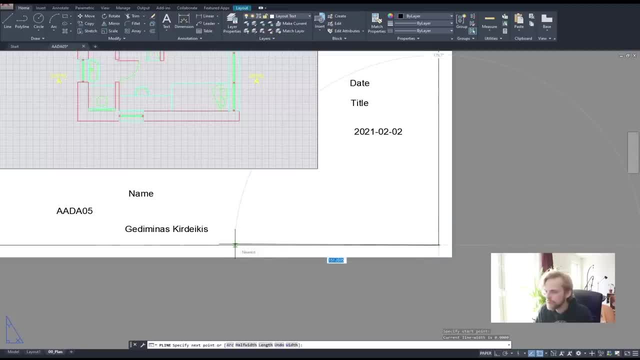 nice, nice way. so I'm going to draw with a polyline. I'm just going to draw with a polyline. I'm just going to draw with a polyline. I'm just going to draw out a table that is, let's say, going to, out a table that is, let's say, going to. 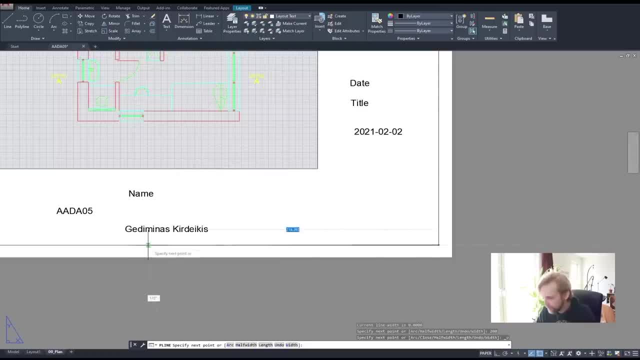 out a table that is, let's say, going to be 200 mil uh long, and it's not be 200 mil uh long and it's not be 200 mil uh long and it's not horizontal f8, horizontal f8, horizontal f8, 200 millimeters by. 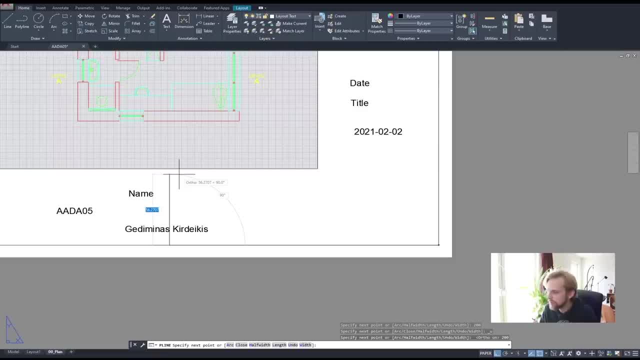 200 millimeters by 200 millimeters. by um. let's say um. let's say um. let's say by by by by 40, 40, 40 millimeters, millimeters, millimeters by 200, by 200 by 200. close it off. if we need to, we'll, we'll. 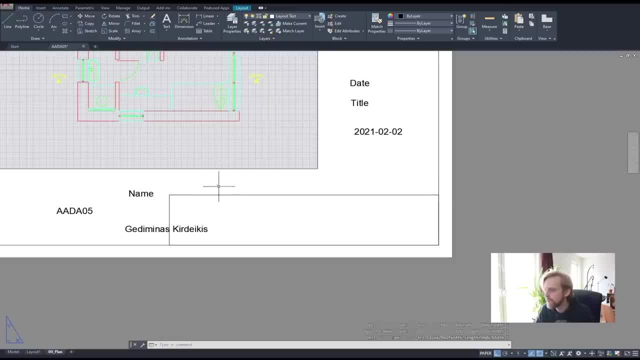 close it off. if we need to we'll, we'll close it off. if we need to we'll, we'll trim away some some stuff from it. trim away some some stuff from it, trim away some some stuff from it. um, and then I'm actually I'm going to. 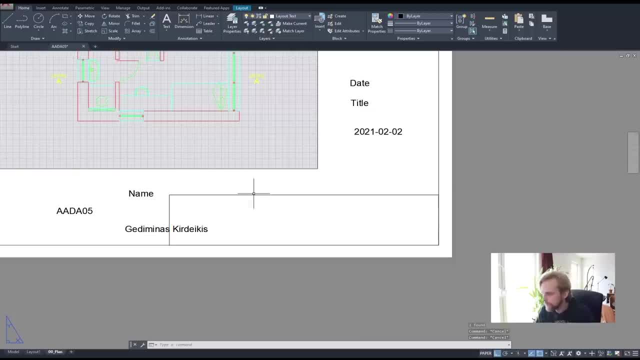 um, and then I'm actually I'm going to um, and then I'm actually I'm going to just select this and explode it. just select this and explode it. just select this and explode it so that I can work with each individual, so that I can work with each individual. 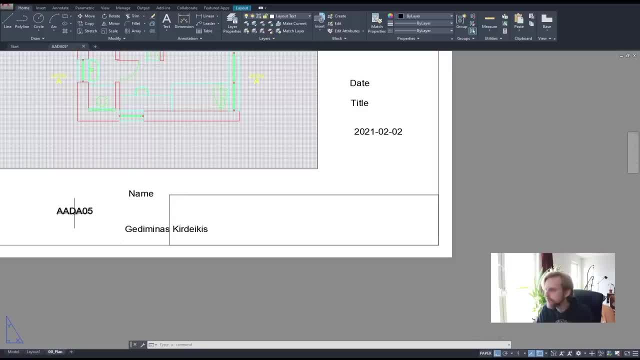 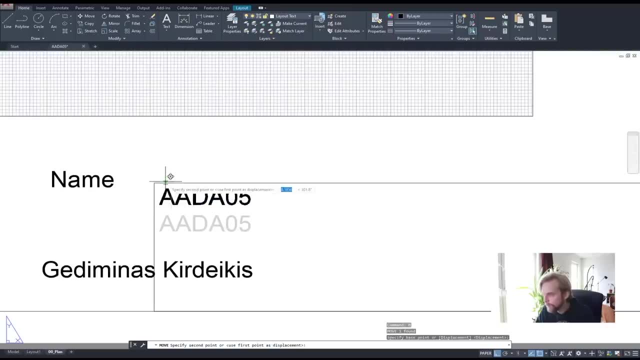 so that I can work with each individual edge separately, or each individual line edge separately, or each individual line edge separately, or each individual line separately, separately, separately, and I will see that aada05 and I will see that aada05 and I will see that aada05 is going to be located right here. 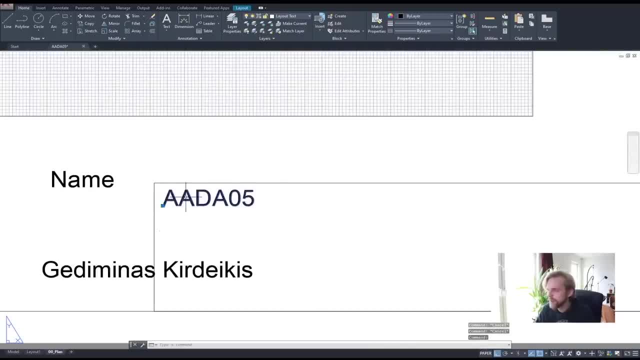 is going to be located right here, is going to be located right here, somewhere here, and it actually is going to be scaled, and it actually is going to be scaled and it actually is going to be scaled. it's going to be twice the size to all. it's going to be twice the size to all. 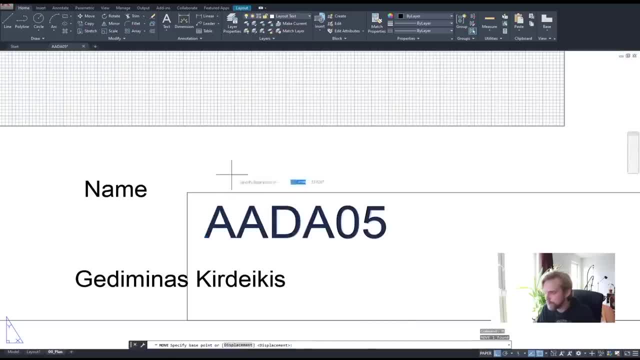 it's going to be twice the size to all other other other, all other information. so I'm just all other information. so I'm just all other information. so I'm just scaling it to by two, scaling it to by two, scaling it to by two. position it. 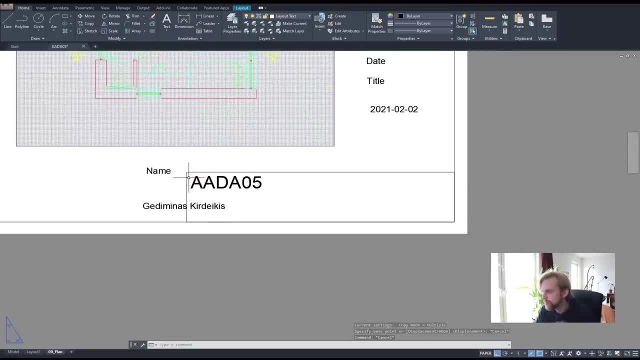 position it. position it there. we go there, we go there, we go make a copy of it or make a copy of make a copy of it, or make a copy of make a copy of it or make a copy of this. uh, probably some something like so. uh, probably some something like so. 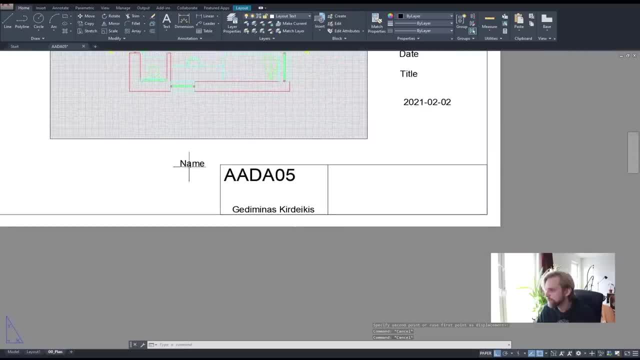 uh, probably some something like: so move this, move this, move this, my name is gonna go here, my name is gonna go here, my name is gonna go here. um, um, um, you can just kind of position it like. you can just kind of position it like. you can just kind of position it like so. 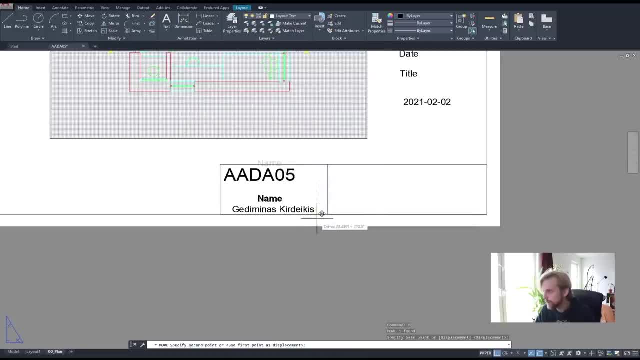 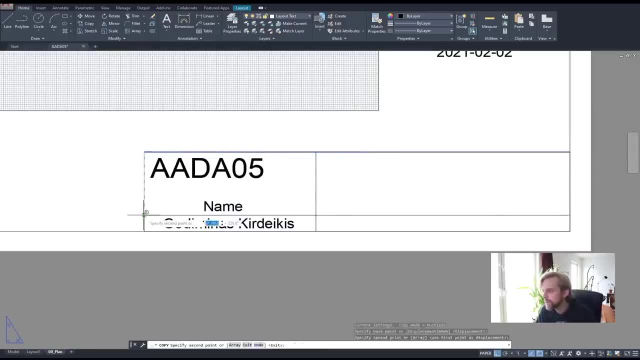 so you can just kind of position it like so, like that, and now i'm just going to kind of build, and now i'm just going to kind of build, and now i'm just going to kind of build a table, a table, a table, build a table around it. 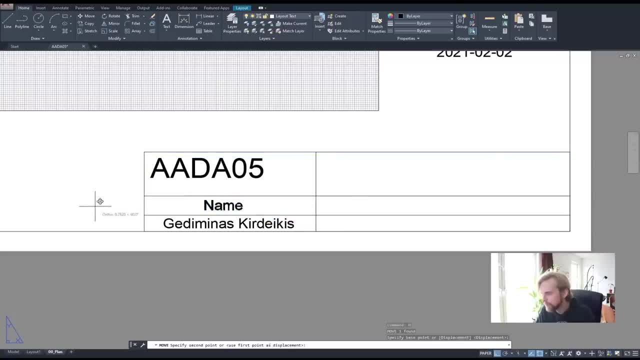 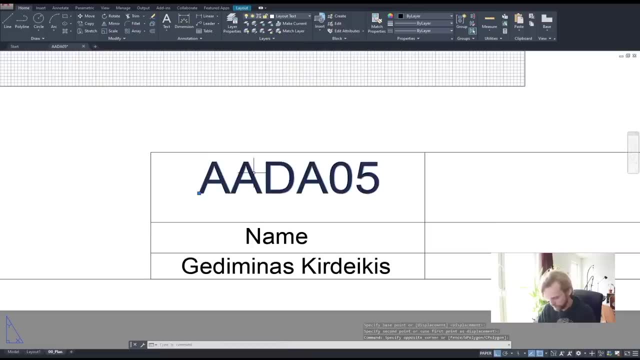 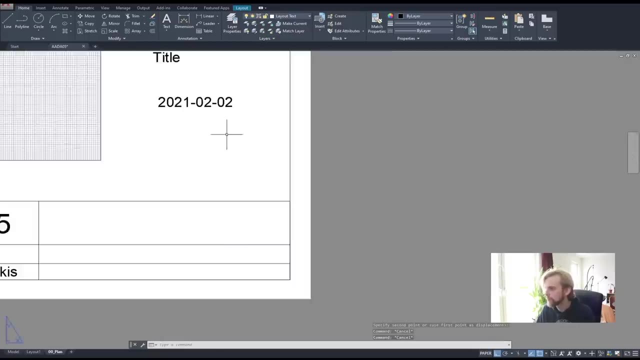 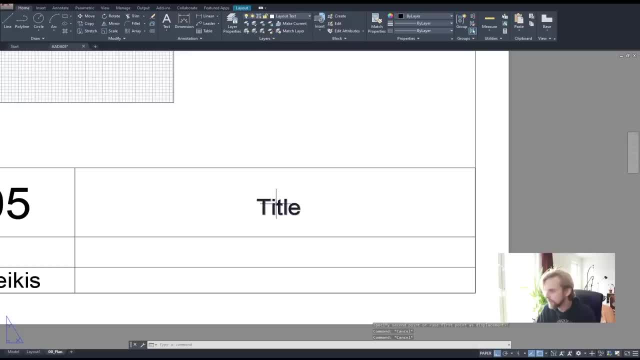 uh now for the date and the title. uh, the uh now for the date and the title. uh, the title will go in here. title will go in here. title will go in here. so i'm just going to move the title here. so i'm just going to move the title here. 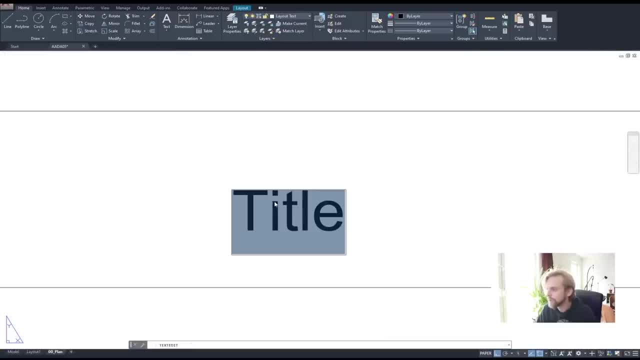 so i'm just going to move the title here and i'm going to kind of double click on and i'm going to kind of double click on and i'm going to kind of double click on it and change this it and change this it and change this- um, it's ground floor plan, so it's going. 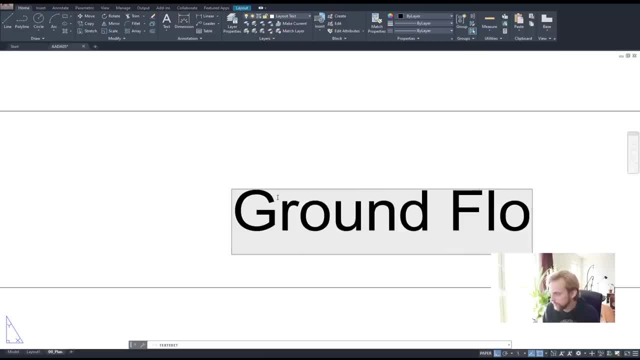 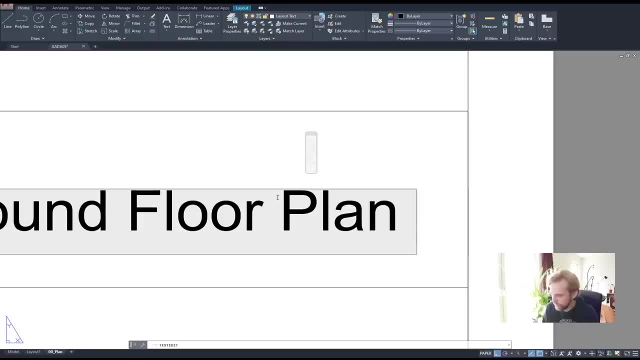 um, it's ground floor plan, so it's going um, it's ground floor plan, so it's going to be ground to be, ground to be ground floor floor floor plan. um, um, um, um, m, um, um, um, um, or, or scale, or or scale, or or scale one to. 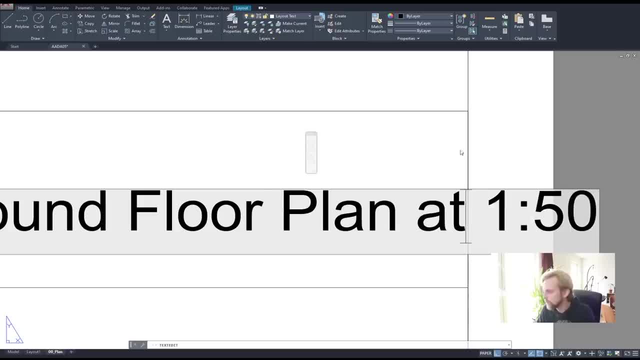 one to one to 50.. 50., 50. now we can say at 1 to 50. now we can say at 1 to 50. now we can say at 1 to 50.. usually at is: at what height are you? 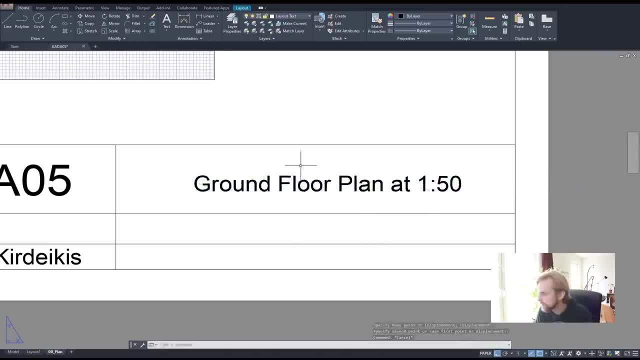 usually at is. at what height are you usually at is. at what height are you cutting, cutting, cutting, but here we don't really care, so we'll. but here we don't really care, so we'll, but here we don't really care. so we'll just say 1 to 50.. 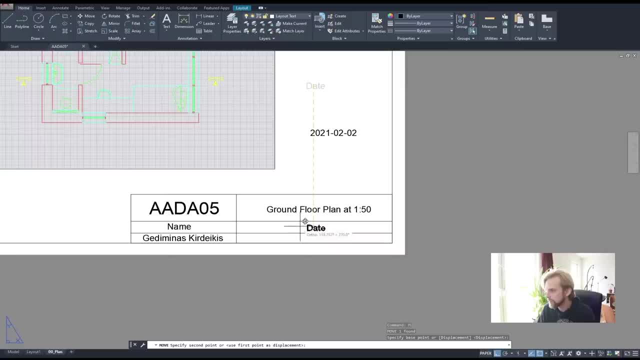 just say 1 to 50.. just say 1 to 50.. so that's ground floor plan. and then we so that's ground floor plan, and then we so that's ground floor plan, and then we have the date 2021, 2021. 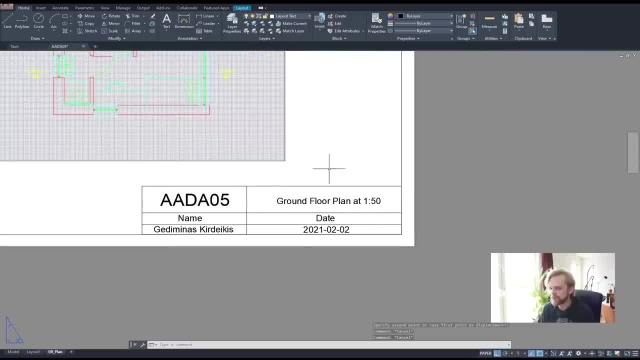 and position it properly. that's it, uh. and position it properly. that's it, uh. and position it properly, that's it, uh. that that's all you need to do, uh right? that that's all you need to do, uh right, that that's all you need to do, uh right. so you have your um. 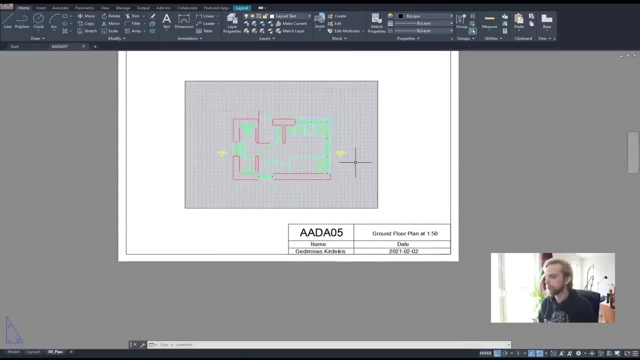 so you have your um. so you have your um. your stamp here, right. um. your stamp here right, um. your stamp here, right, um. usually the stamp is it does have much. usually the stamp is it does have much. usually the stamp is it does have much more information in it. but this is just. 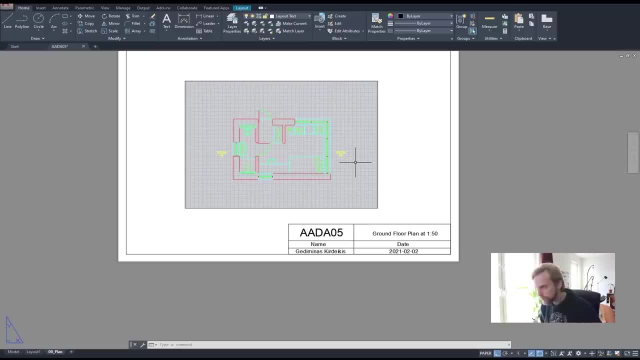 more information in it, but this is just more information in it. but this is just like first practice, like first practice, like first practice. okay, so that is done. we have our plan. we okay, so that is done. we have our plan. we okay, so that is done. we have our plan, we have our layout, everything is correct. 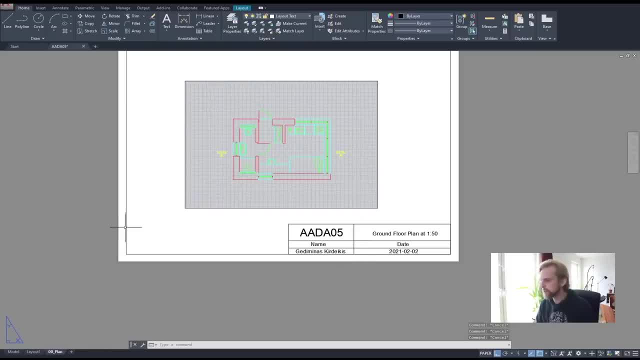 have our layout, everything is correct. have our layout, everything is correct. let's do two more layouts, right so the let's do two more layouts, right so the let's do two more layouts, right. so the way we will do other two layouts, it's way we will do other two layouts, it's. 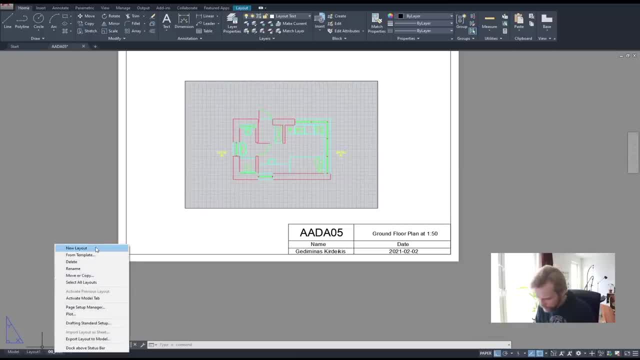 way we will do other two layouts. it's now by right clicking and choosing to now by right clicking, and choosing to now by right clicking and choosing to uh uh, uh, move or copy, move or copy, move or copy. so we right click our existing layout. so we right click our existing layout. 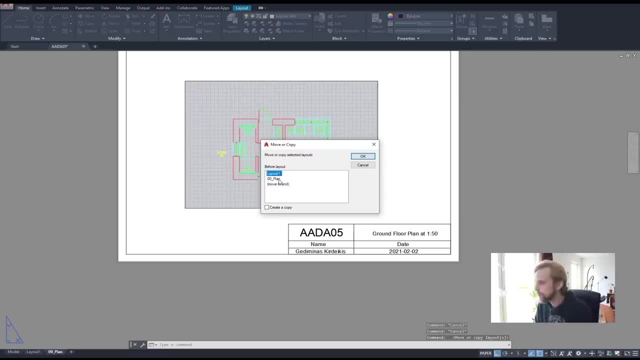 so we right click our existing layout: zero zero plan. move or copy zero zero plan. move or copy zero zero plan. move or copy um and we choose um and we choose um and we choose move to end. move to end. move to end, create, copy. right, so there's going to be a. 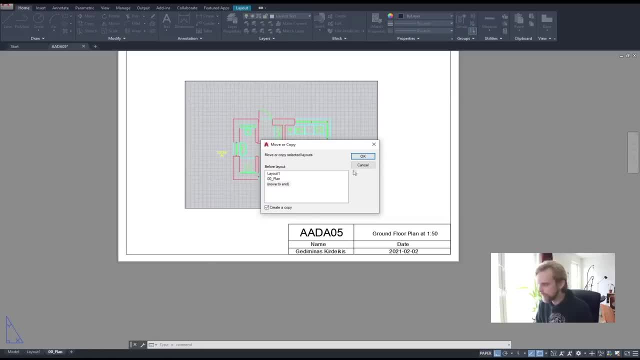 create copy. right, so there's going to be a create copy, right, so there's going to be a copy created at the end of the layout copy created at the end of the layout. copy created at the end of the layout line. i hit ok, so we have this one. 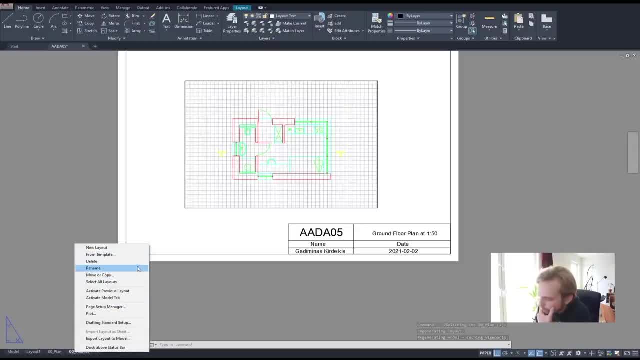 line. i hit ok, so we have this one line. i hit ok, so we have this one. we will right click it and choose to. we will right click it and choose to. we will right click it and choose to. uh, we will choose to rename it. uh, we will choose to rename it. 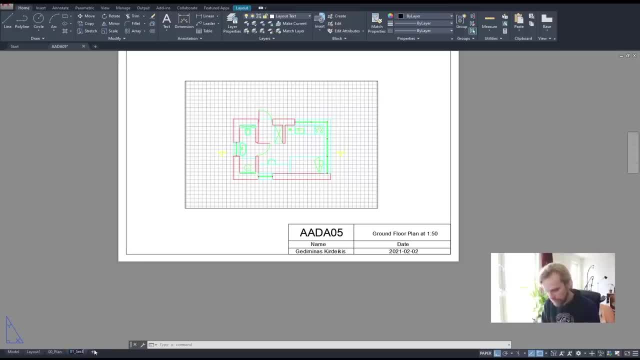 uh, we will choose to rename it to to to zero one dash, zero one dash, zero one dash section section section right zero one dash section right zero one dash section right, zero one dash section. uh, that is done, and then, uh, i'm gonna. uh, that is done, and then, uh, i'm gonna. 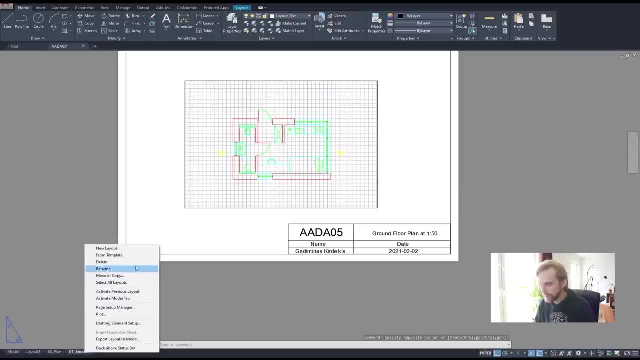 uh, that is done. and then, uh, i'm gonna, while i'm at it, i'm just going to right, while i'm at it, i'm just going to right, while i'm at it, i'm just going to right, click, click, click. uh, uh, uh, move and or copy. 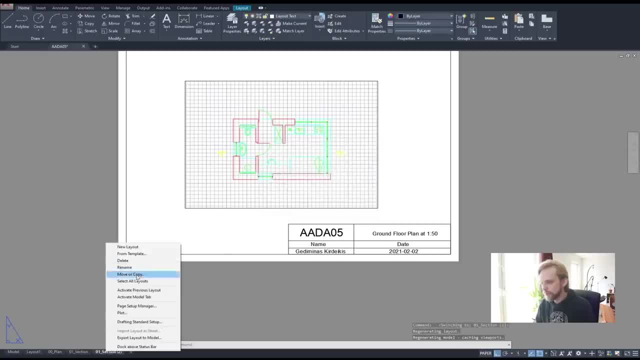 move and or copy, move and or copy, move to end. create copy. okay, uh, rename, rename, rename to uh rename, rename, rename to uh rename, rename, rename to zero two, zero two, zero, two. axle, axle, axle right. so we have section xo and plan. right, so we have section xo and plan. 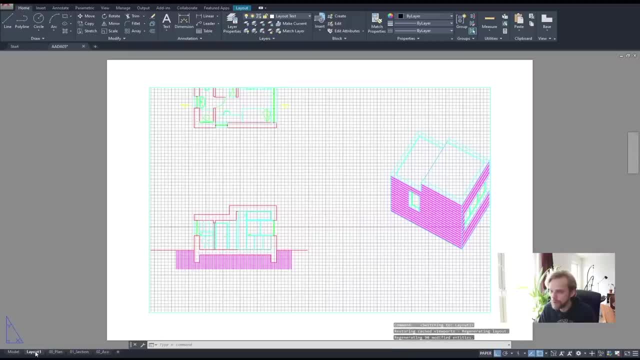 right, so we have section xo and plan, and now layout one is just, and now layout one is just, and now layout one is just randomly there. so i'm just gonna delete randomly there. so i'm just gonna delete randomly there. so i'm just gonna delete it. 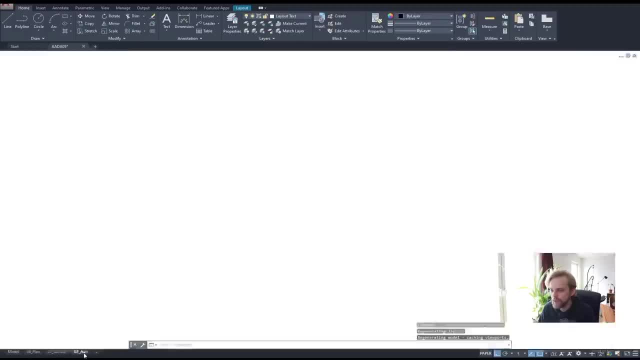 it. it no need for that, no need for that, no need for that. there we go. the only layouts that we need- there we go, the only layouts that we need. there we go. the only layouts that we need are these three: are these three? are these three? okay, so we have that? uh, now for the 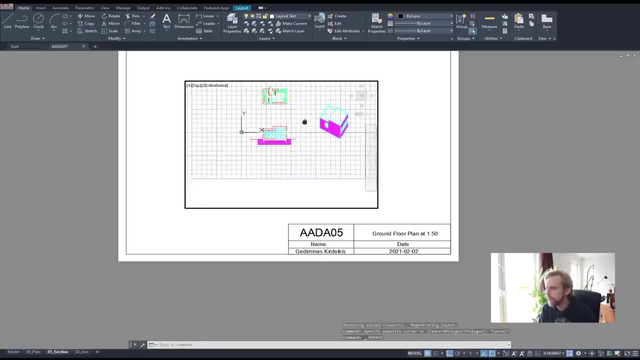 okay, so we have that, uh, now for the. okay, so we have that, uh, now for the section. i will double click inside of section. i will double click inside of section. i will double click inside of this, this window, this, this window, this, this window, uh, find the section. 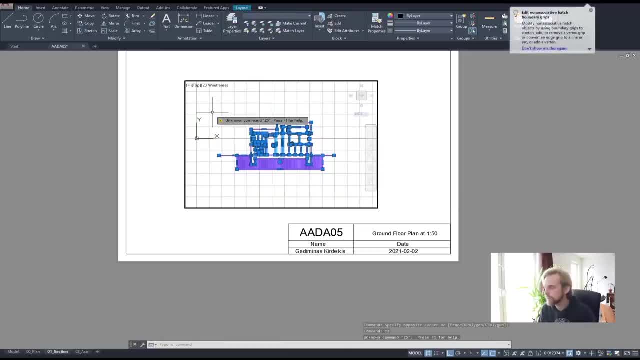 uh find the section. uh find the section. zoom into it, zoom into it, zoom into it. zs enter, zs enter, zs enter, or, or, or. that's, that's, that's, that is not. that is not. that is not. uh, an autocad command, that is rhino. uh, an autocad command, that is rhino. 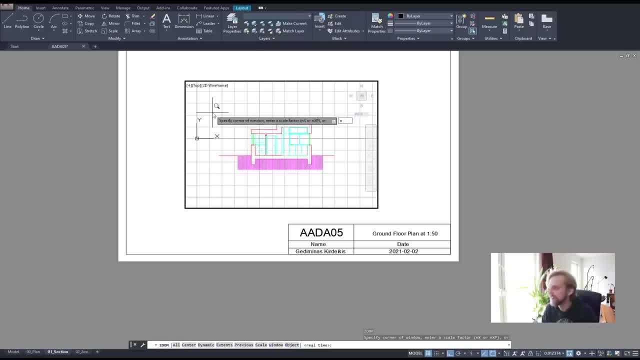 uh, an autocad command. that is rhino command z enter, command, z, enter, command z enter o, o, o, enter, there we go. that is enter, there we go. that is enter, there we go. that is autocad command, double click out. autocad command, double click out. 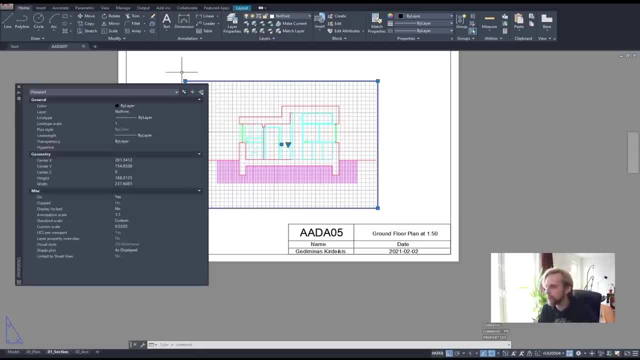 autocad command. double click out, select the frame. select the frame. select the frame. pr for properties. pr for properties. pr for properties. annotation scale: no, not annotation annotation scale: no, not annotation annotation scale. no, not annotation custom scale: uh, custom scale: uh, custom scale. uh. that standard scale 1 250. 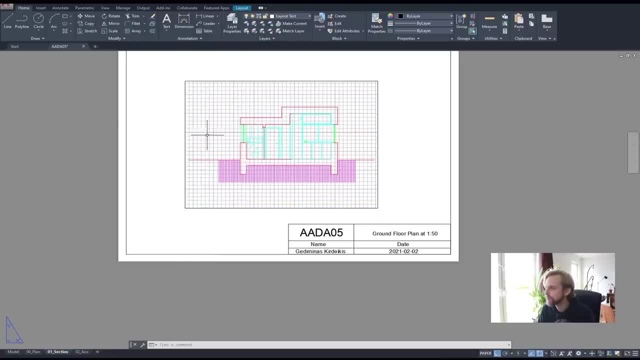 that standard scale 1 250, that standard scale 1 250, like that, like that. like that, close it off, close it off, close it off. that's done, that's done, that's done. um, and i will just change um and i will just change um and i will just change the. 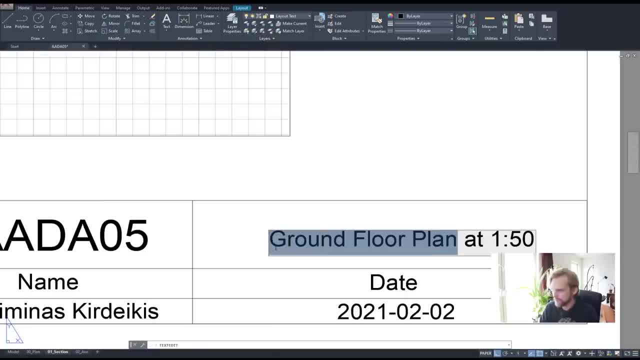 the, the, this as well, this as well, this as well, so, so, so this is section, this is section, this is section a-a at 1 250. that's all we need to change here, and that's all we need to change here, and that's all we need to change here, and that is done. and now, 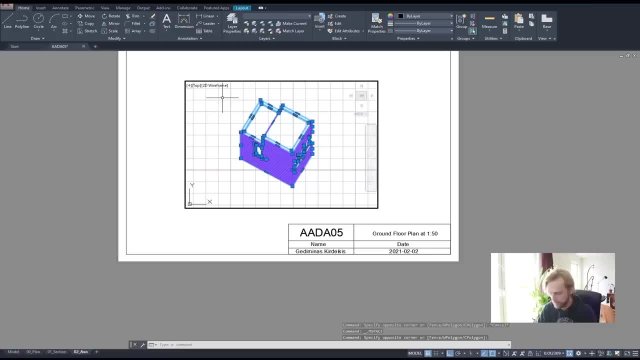 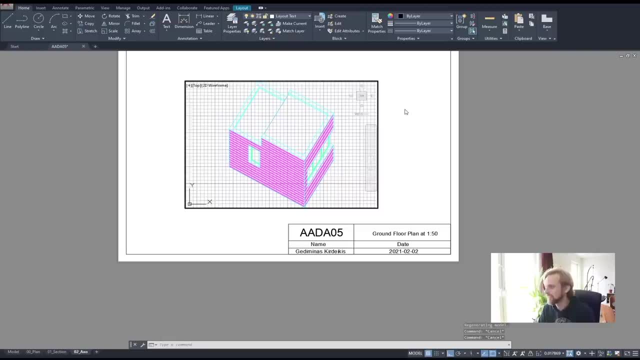 that is done. and now that is done. and now axo: double click inside. find the axo. axo. double click inside. find the axo. axo. double click inside. find the axo. zoom selected: zoom selected: zoom selected: z. enter. oh, enter not zoom selected. z enter. oh, enter not zoom selected. 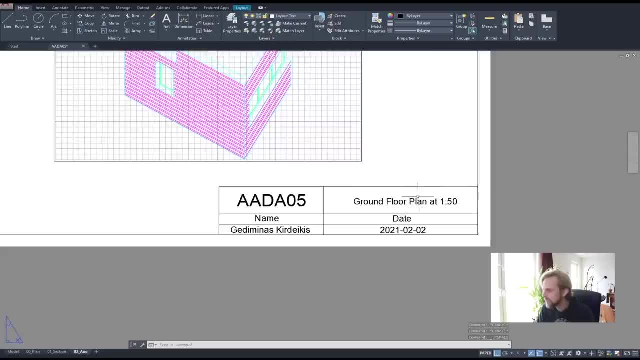 z enter. oh, enter, not zoom selected. and this guy right here, we don't really. and this guy right here, we don't really. and this guy right here, we don't really have a have a, have a scale for it. so this is just going to be scale for it. so this is just going to be. 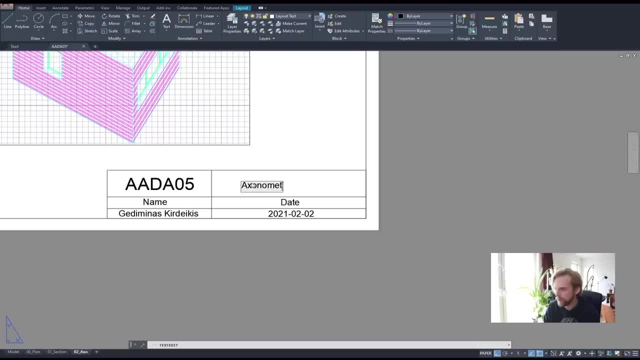 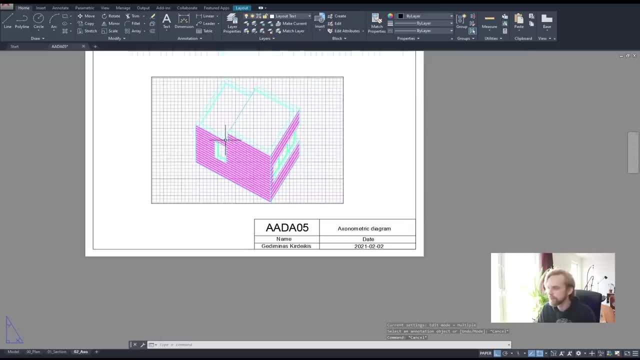 scale for it. so this is just going to be axon axon, axon axon, nometric axon, nometric axon, nometric diagram, something like that, and actually if you something like that, and actually if you something like that, and actually if you want to, by the way, if you want to, 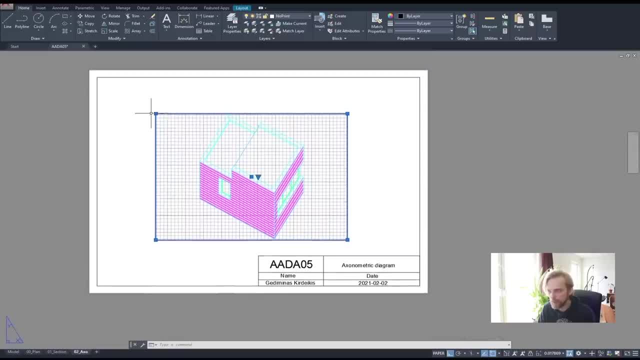 want to. by the way, if you want to want to, by the way, if you want to resize your, resize your, resize your, uh your window, you can. you can just uh your window, you can. you can just uh your window, you can. you can just click on these. 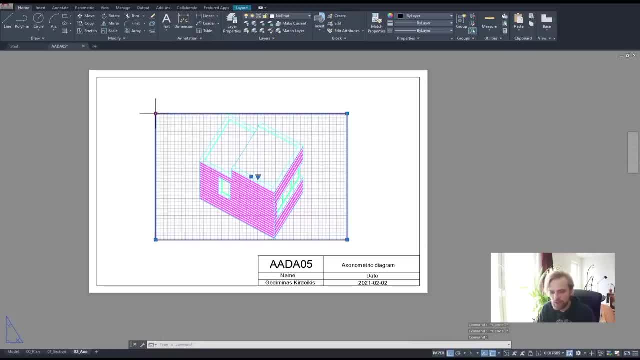 click on these, click on these doodads- these, you select the frame. you doodads these: you select the frame. you doodads these: you select the frame, you click on this, click on this, click on this corner point here and you can just corner point here and you can just. 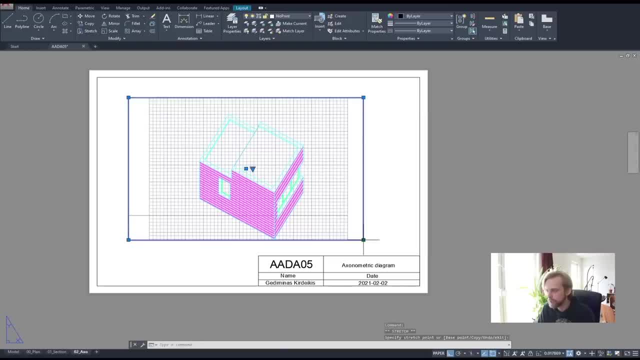 corner point here and you can just resize it any way you want right. resize it any way you want right. resize it any way you want right. that that that works as well. uh axo, that that that works as well. uh axo. that that that works as well, uh axo. doesn't have a scale, so i will not be. 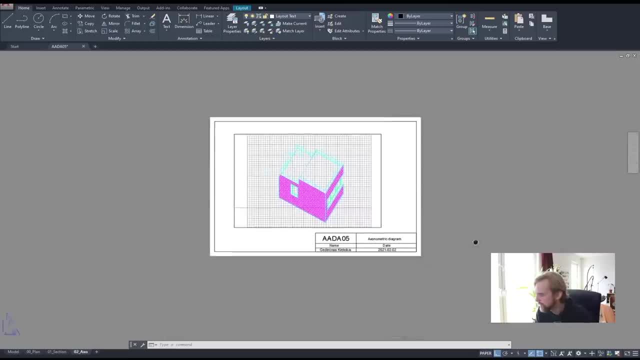 doesn't have a scale, so i will not be. doesn't have a scale, so i will not be messing around with it too much. messing around with it too much, messing around with it too much. i'll just keep it as it is okay, so we. i'll just keep it as it is okay, so we. 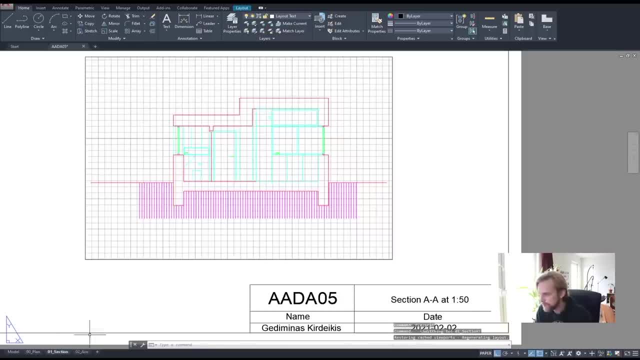 i'll just keep it as it is okay. so we have that done. have that done. have that done. uh, we have axonometric diagram. we have. uh, we have axonometric diagram. we have. uh, we have axonometric diagram. we have section. we have plan. 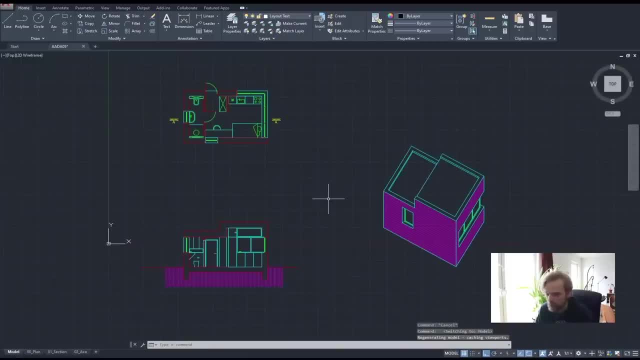 okay, i think we're good. so now in the. okay, i think we're good. so now in the okay, i think we're good. so now in the model space, model space, model space- um, we actually need to. um, we actually need to. um, we actually need to, or rather not in the model space. let's 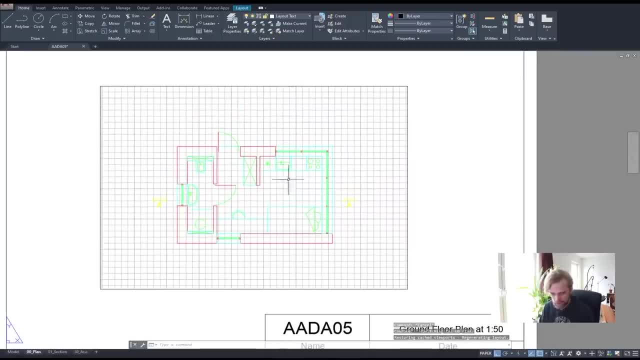 or rather not in the model space. let's- or rather not in the model space, let's- go back to layout space. go back to layout space. go back to layout space. let's change the colors. let's change the colors. let's change the colors. i. i think that's that's important to to. 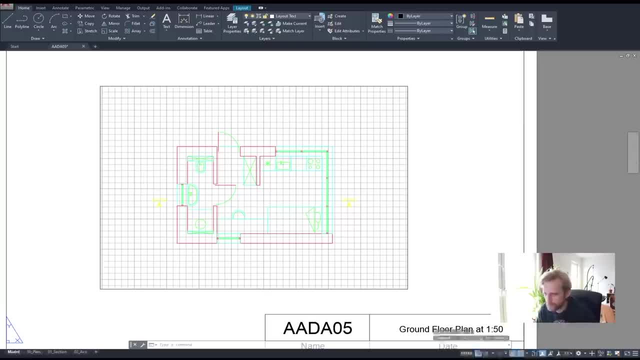 i- i think that's that's important to to. i- i think that's that's important to- to kind of change the colors, kind of change the colors, kind of change the colors. before we do that, of course we need to, before we do that, of course we need to. 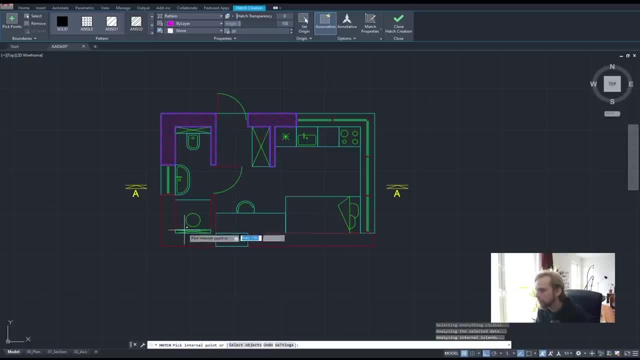 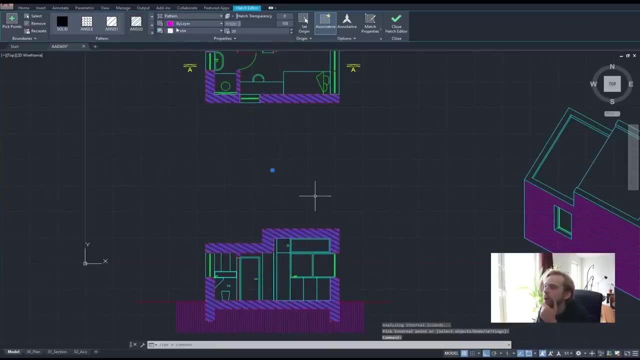 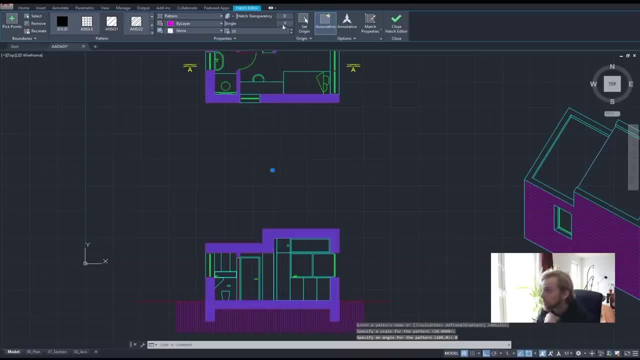 and you enter, select the hatch. and you enter, select the hatch. uh, angled angle is gonna be zero. uh, angled angle is gonna be zero. uh, angled angle is gonna be zero. and scale is 20. that's perfect, that's. and scale is 20. that's perfect, that's. 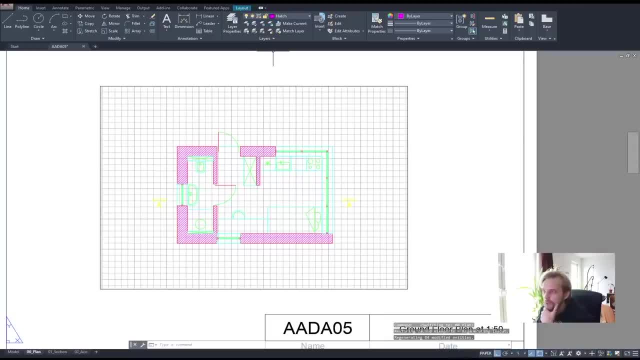 and scale is 20. that's perfect, that's it. it it. okay, let's go back to the plan. so okay, let's go back to the plan. so okay, let's go back to the plan. so that's how it looks like right now. that's how it looks like right now. 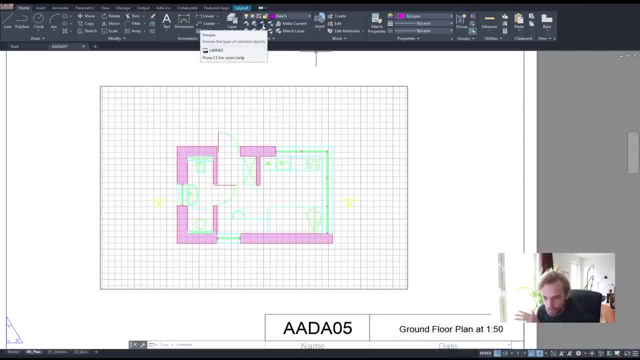 that's how it looks like right now. and to change the colors, you change the and. to change the colors, you change the and. to change the colors, you change the layer properties- right, you change the layer properties- right, you change the layer properties- right. you change the- the properties of the layers. 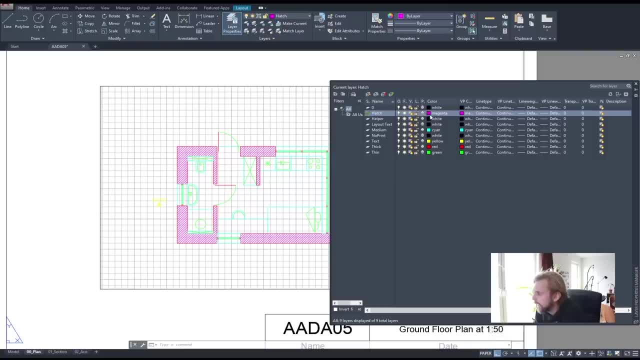 the properties of the layers, the properties of the layers for the colors, so for the colors, so for the colors. so, hatch, let's start with the hatch right. hatch, let's start with the hatch right. hatch, let's start with the hatch right. it's gonna be the easiest one, or rather, 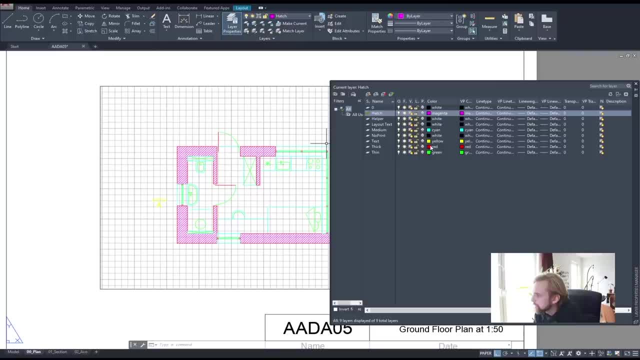 it's gonna be the easiest one, or rather, it's gonna be the easiest one, or rather, let's, let's leave the hatch for the last. let's, let's leave the hatch for the last. let's, let's leave the hatch for the last, one, one, one. um, rather, let's start with the thick line. 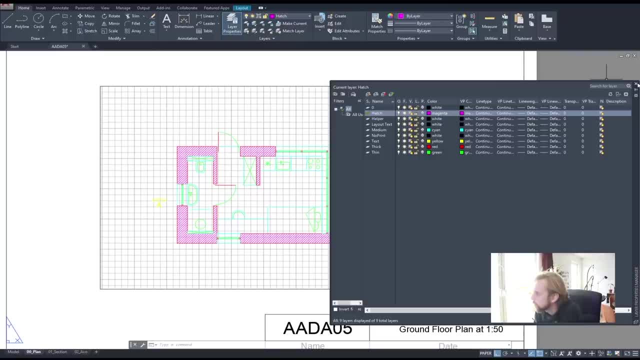 um, rather, let's start with the thick line. um, rather, let's start with the thick line, the red line right, the red line right, the red line right. so here, um well, when i am in the model, so here, um well, when i am in the model, so here, um well, when i am in the model space. 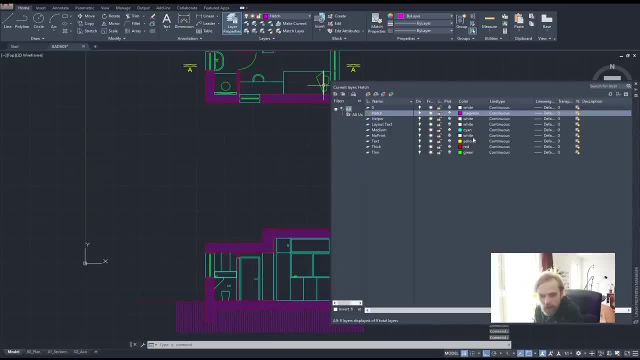 space, space, and i look at layer properties. i can only, and i look at layer properties. i can only, and i look at layer properties. i can only see one color right. see one color right. see one color right. it's, it's just uh, magenta, red, yellow. 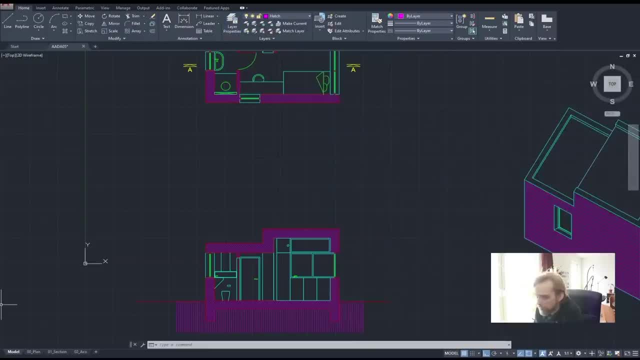 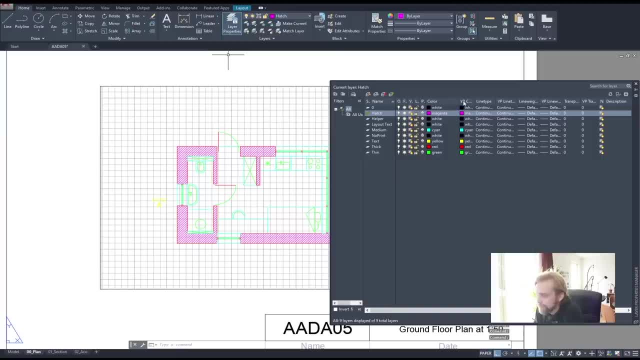 my plan right here, my plan right here to my layout and i go to layer to my layout and i go to layer to my layout and i go to layer properties. i can see two colors. that is important. i can see two colors. that is important. i can see two colors. that is important because this is the color of the model. 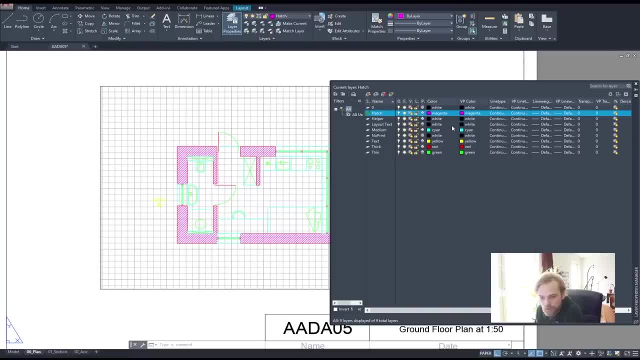 because this is the color of the model, because this is the color of the model space, this is the color space, this is the color space, this is the color in which it's going to be plotted out, or in which it's going to be plotted out, or. 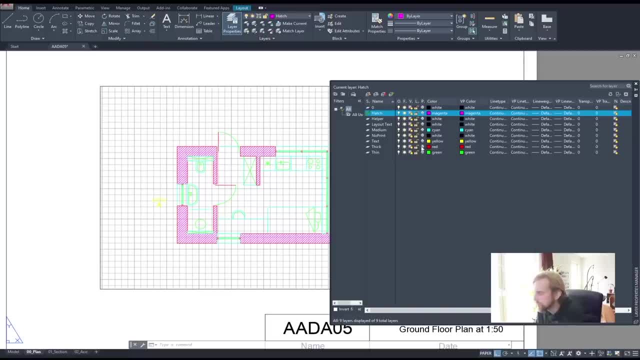 in which it's going to be plotted out, or exported, exported, exported, very big difference. so i am going to in very big difference. so i am going to in very big difference. so i am going to in the the, the um, um, um. is it called white space? no, it's, it's. 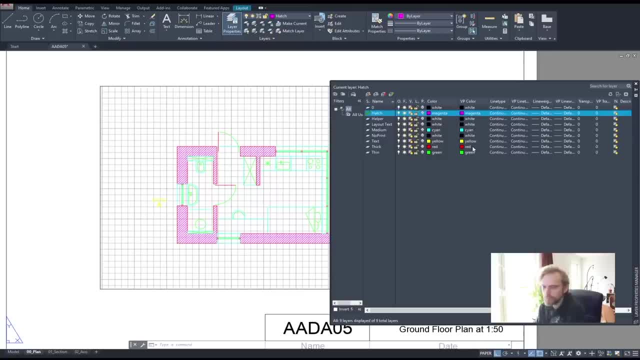 is it called white space? no, it's, it's. is it called white space? no, it's, it's something else, um, something else, um, something else, um in this column. sorry, sorry, sorry about that um in this column. i'm about that um in this column i'm. 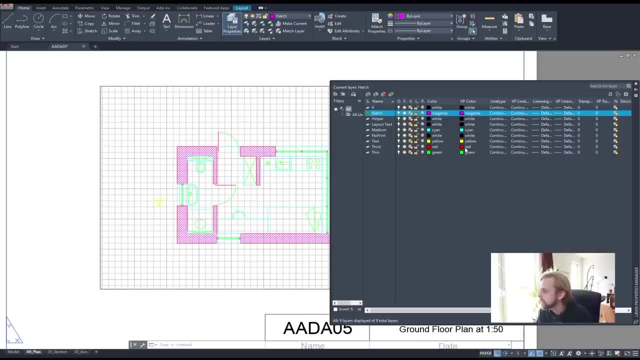 about that. um, in this column i'm going to change, going to change, going to change. start changing the colors first right. start changing the colors first right. start changing the colors first right. so the thick, so the thick, so the thick, thick line- uh, i'll change. thick line: uh, i'll change. 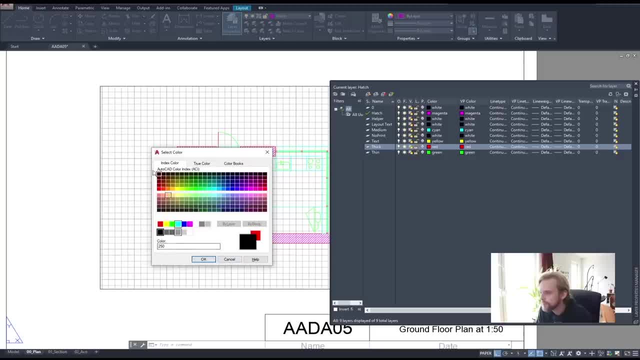 thick line. uh, i'll change from the red color to black, from the red color to black, from the red color to black, right here or right here or right here, or to white actually, to white, actually, to white, actually. i know it's, it's, it's confusing, but 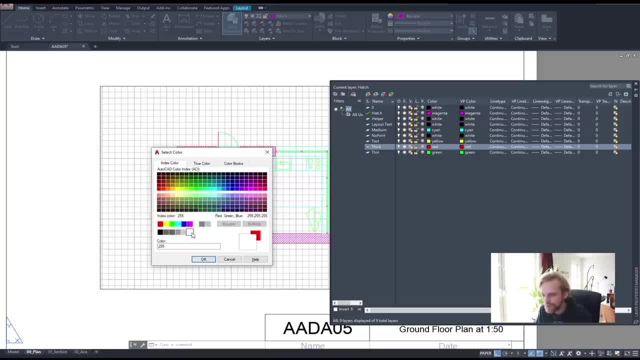 i know it's it's it's confusing, but i know it's it's it's confusing, but you'll get used to it, so i'll change it. you'll get used to it, so i'll change it. you'll get used to it, so i'll change it to this white color, not this white color. 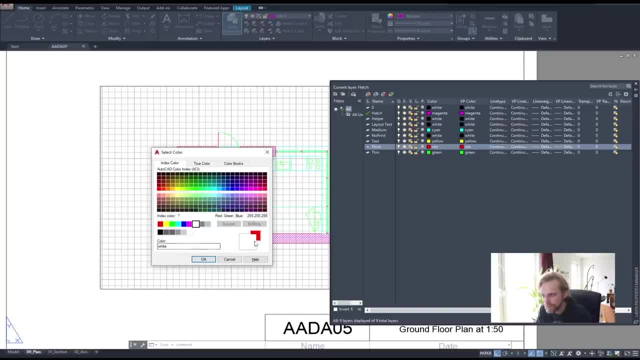 to this white color, not this white color. to this white color, not this white color. this is this white is going to be. this is this white is going to be. this is this white is going to be printed out as white. printed out as white. printed out as white. this white is going to be printed out as 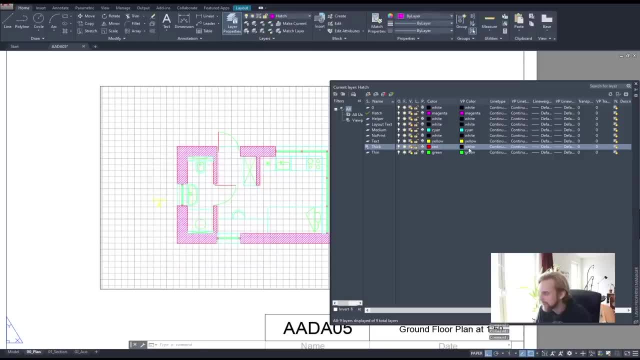 this white is going to be printed out as this white is going to be printed out as black, right. so it needs to say white, black right. so it needs to say white, black right. so it needs to say white- here, i'll change it to white. here, i'll change it to white. 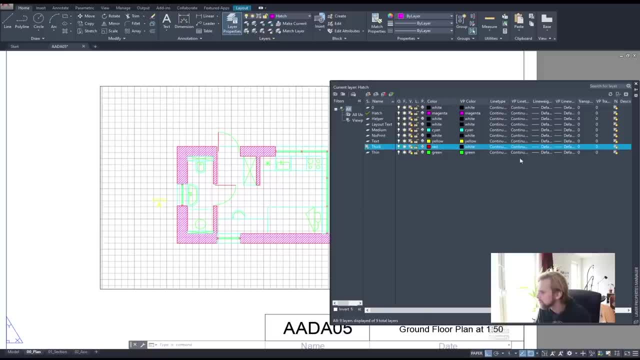 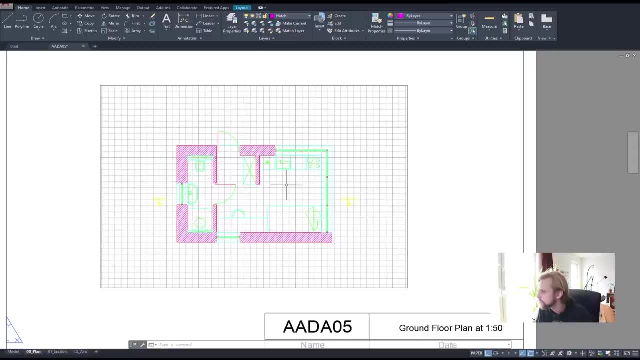 here, i'll change it to white. and now if i and now if i and now if i doesn't doesn't doesn't. so wait a minute, wait a minute, wait a minute. yep, that was that was my bad, sorry i. yep, that was that was my bad, sorry i. 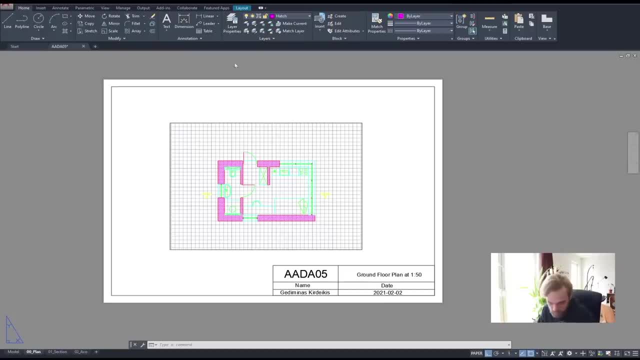 yep, that was, that was my bad, sorry. i figured it out. so apparently in the paper. figured it out, so apparently in the paper. figured it out, so apparently in the paper. space, space, space, right here. um, this is what's called the right here, um, this is what's called the. 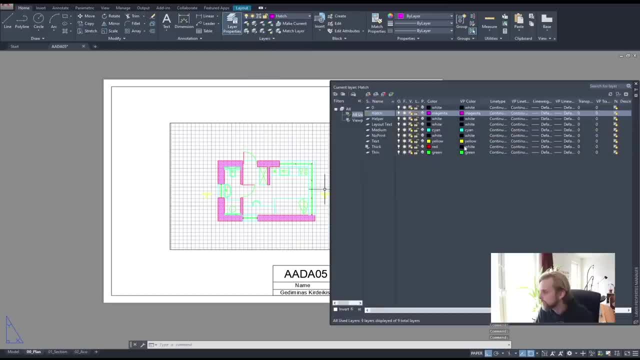 right here. um, this is what's called the paper space, paper space, paper space. you can't really override the the color. you can't really override the the color. you can't really override the the color this way, so i'll turn this back to red this way, so i'll turn this back to red. 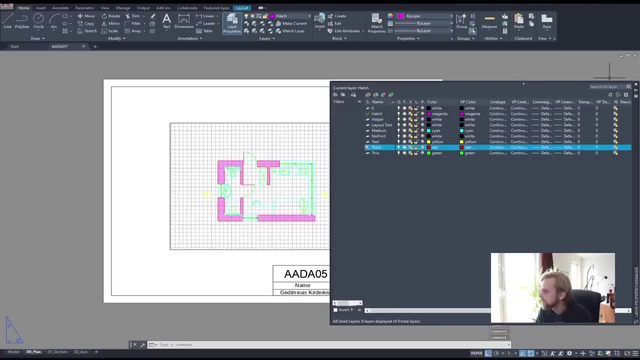 this way. so i'll turn this back to red. sorry about that. that's a little bit of sorry about that. that's a little bit of sorry about that. that's a little bit of a hiccup. a hiccup, a hiccup. uh instead instead. uh instead instead. 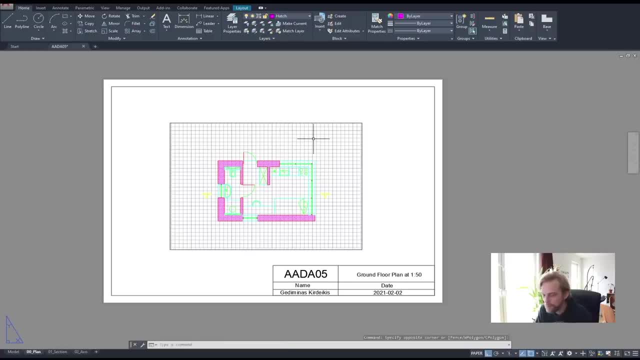 uh, instead, instead, i need to go into the model space, so i need to go into the model space, so i need to go into the model space, so i need to double click, i need to double click, i need to double click to go into this view and here, 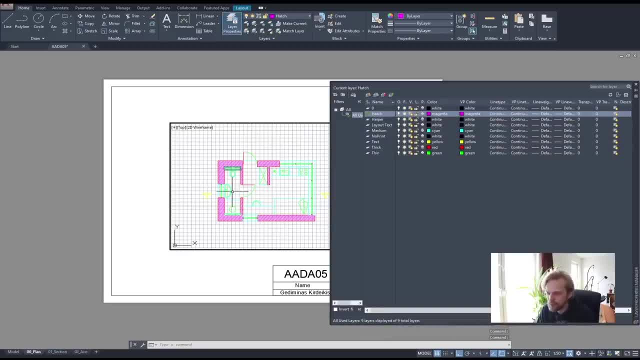 to go into this view and here to go into this view and here i can go to. then i can go to layer i can go to, then i can go to layer i can go to, then i can go to layer properties. just make sure that you don't. 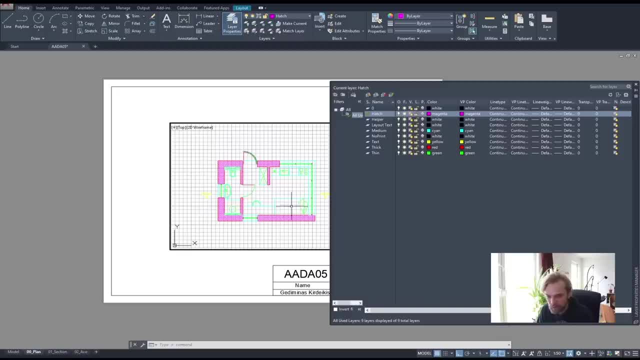 properties. just make sure that you don't properties. just make sure that you don't accidentally scroll your mouse wheel or accidentally scroll your mouse wheel or accidentally scroll your mouse wheel or anything like that. you don't mess up the, anything like that. you don't mess up the. 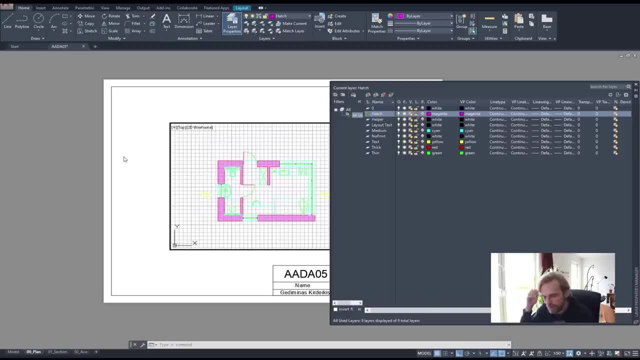 anything like that. you don't mess up the scale, scale scale i mean, if you mess up the scale you can. i mean if you mess up the scale you can. i mean if you mess up the scale you can always kind of repeat the steps and always kind of repeat the steps and 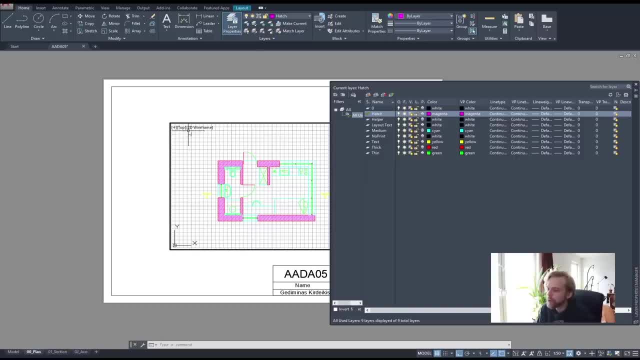 always kind of repeat the steps and get the scale back. either way, get the scale back, either way, get the scale back, either way. uh, once i am inside of this view, uh, once i am inside of this view, uh, once i am inside of this view that this is super important, once i'm. 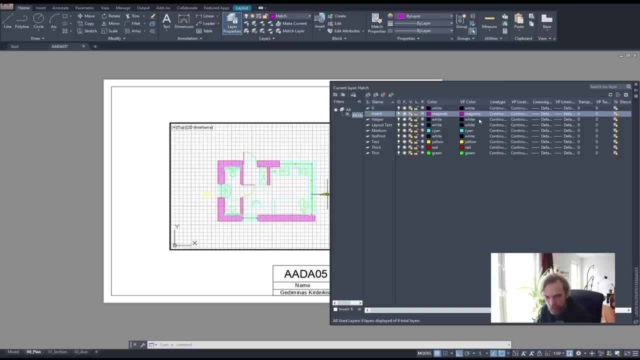 that this is super important. once i'm that this is super important, once i'm inside of this view, inside of this view, inside of this view, then i can override the color how it's. then i can override the color how it's. then i can override the color how it's going to be. 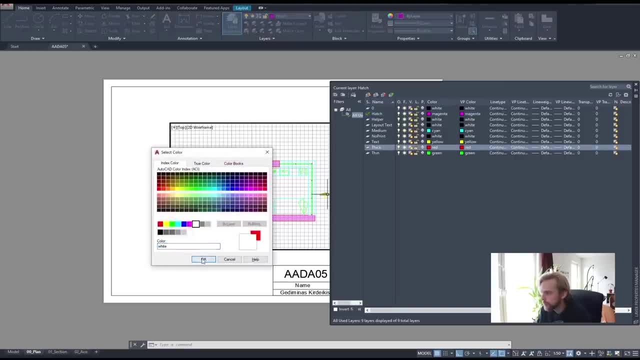 going to be going to be printed out. so thick line, it's gonna be printed out. so thick line, it's gonna be printed out. so thick line, it's gonna be white, white, white, blue in my case, or maybe red- yeah, let's go blue in my case. or maybe red- yeah, let's go. 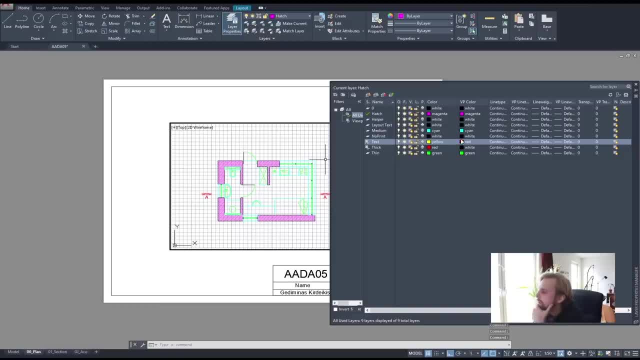 blue in my case, or maybe red. yeah, let's go for red. oh, i'll say: text is red for red. oh, i'll say text is red for red. oh, i'll say: text is red, sure, uh, no, print is whatever a medium, sure, uh, no, print is whatever a medium. 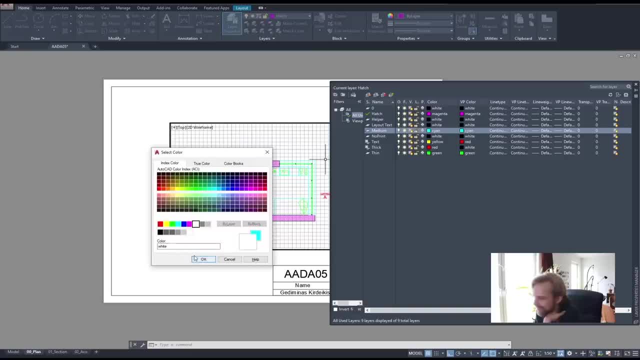 sure, uh, no, print is whatever. a medium line is going to be also black, so line is going to be also black, so line is going to be also black, so white i need. i need naming conventions- white i need. i need naming conventions- white i need. i need naming conventions for this. 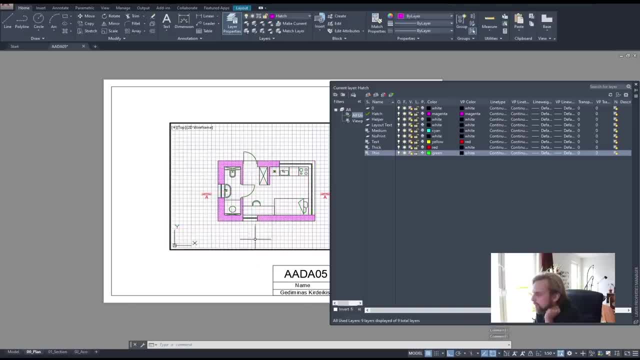 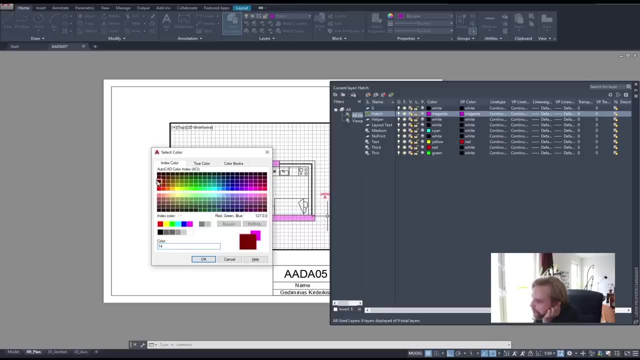 for this, for this: uh thin line white, uh, thin line white, uh thin line white. and hatch and hatch and hatch. for hatch, i will say um. for hatch, i will say um. for hatch, i will say um dark, dark, dark, dark red, red red, something like color, color 14. 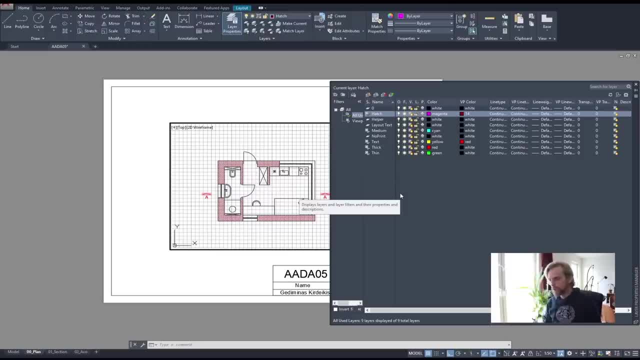 something like color color 14, something like color color 14, something like that, something like that, something like that. right, right, right. so i have this, so i have this, so i have this: uh once i've done that, i will just. uh. once i've done that, i will just. 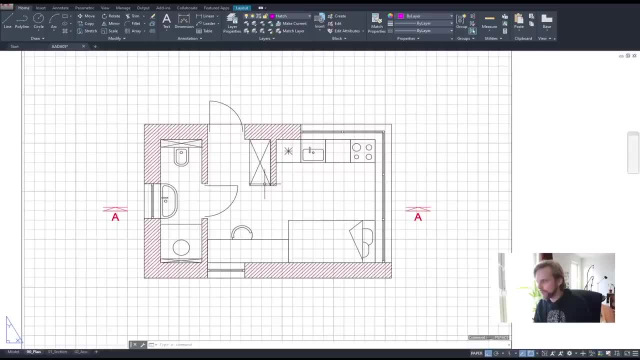 uh, once i've done that, i will just escape out. double click outside of the escape out. double click outside of the escape out. double click outside of the model space. and now you can see the- the model space. and now you can see the- the model space. and now you can see the. the colors have changed and 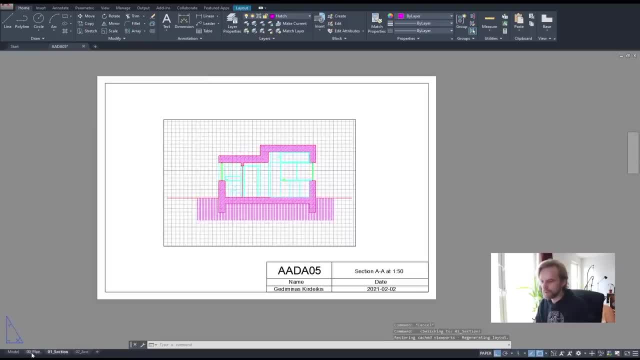 colors have changed, and colors have changed, and i will just need to do this for every. i will just need to do this for every. i will just need to do this for every, every layout here, every layout here, every layout here. um, um, um. a trick on how to do it for all of them. 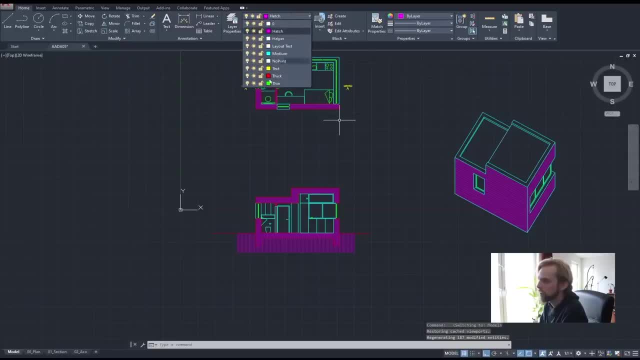 a trick on how to do it for all of them. a trick on how to do it for all of them would be just to go into model space. would be just to go into model space, would be just to go into model space and change every and change every. 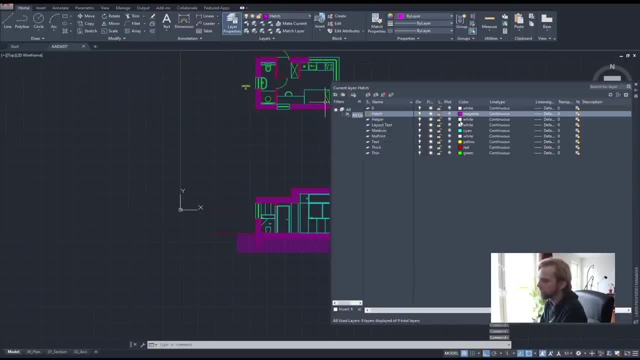 and change every like in the layer properties. come on in like in the layer properties. come on in like in the layer properties. come on in the layer properties. change the colors. the layer properties change the colors. the layer properties change the colors here and then it will update for all of. 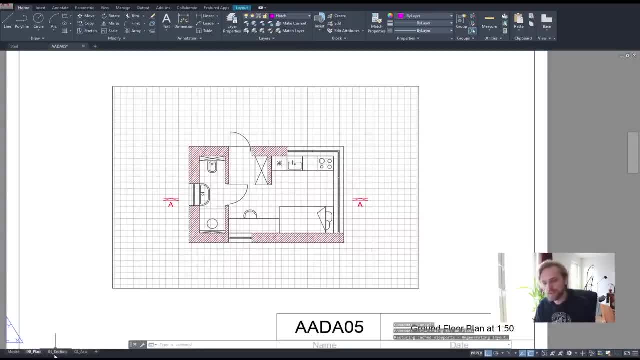 here, and then it will update for all of here and then it will update for all of the, the, the layouts, but sometimes in different layouts, but sometimes in different layouts, but sometimes in different layouts. you want different colors layouts, you want different colors layouts, you want different colors, um, so so this is a little bit better. 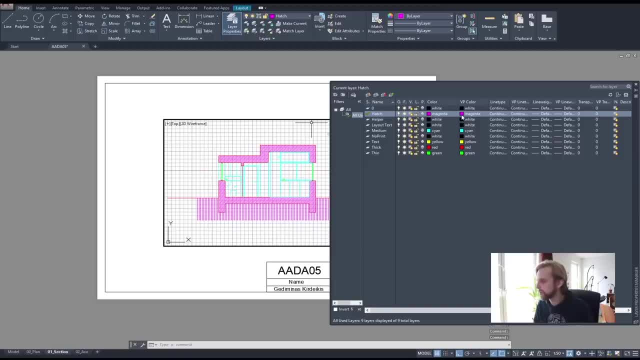 um so, so this is a little bit better. um so, so this is a little bit better to do so. double click inside layer to do so, double click inside layer to do so, double click inside layer. properties and properties and properties. and i will just really quickly go through: 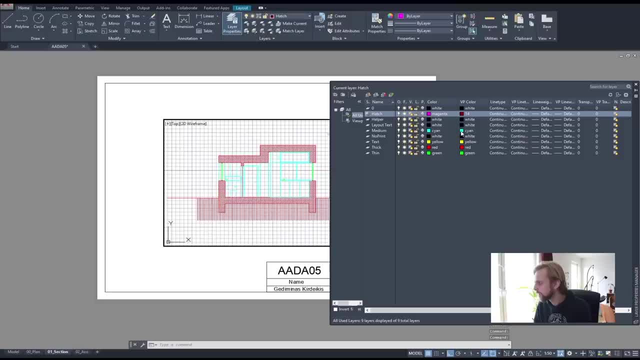 i will just really quickly go through. i will just really quickly go through this: so that was 14. this, so that was 14. this, so that was 14. um, that is gonna be white, it's gonna be white, it's gonna be white, it's gonna be white. i wonder if there's like a fast way of. 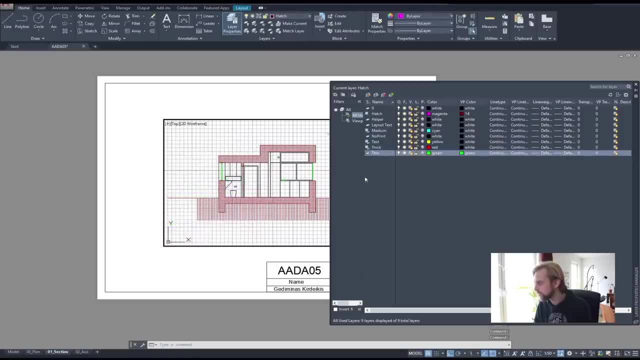 i wonder if there's like a fast way of. i wonder if there's like a fast way of how to do this, how to do this, how to do this, like setting everything to white. oh, the text needs to be red, sorry. oh, the text needs to be red, sorry. 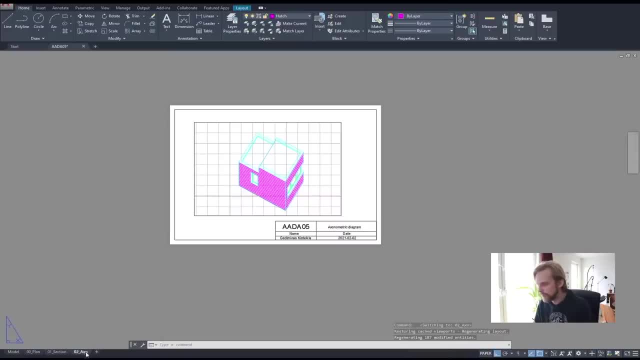 oh, the text needs to be red. sorry, like that, like that, like that double click. and for exo, double click. and for exo, double click. and for exo, uh, for instance, in the xo, i don't want. uh, for instance, in the xo, i don't want. 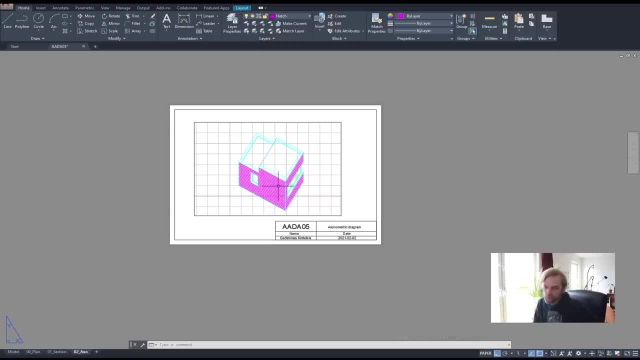 uh, for instance, in the xo, i don't want the hatch to be the hatch to be, the hatch to be uh, to, to, to be, uh, to, to, to be, uh, to, to to be dark red color. i just want it to be like dark red color. i just want it to be like: 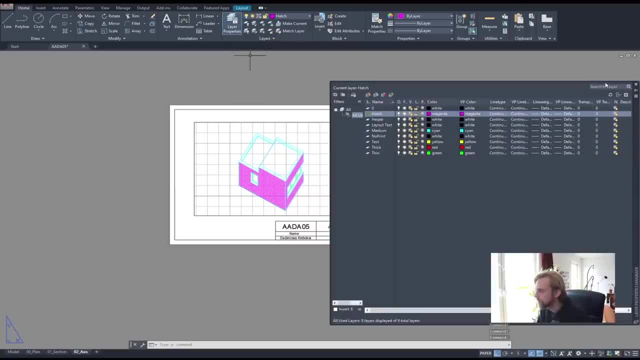 dark, red color. i just want it to be like gray, gray, gray. so here i can change. uh, i can change up, so here i can change. uh, i can change up, so here i can change. uh, i can change up. the overrides, the overrides, the overrides. just make sure that you have double. 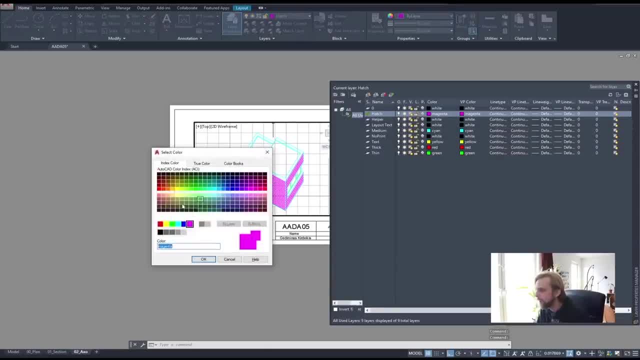 just make sure that you have double, just make sure that you have double clicked, clicked, clicked, layer properties hatch. i will just say layer properties hatch. i will just say layer properties hatch. i will just say: darkish gray, like that darkish gray, like that darkish gray, like that medium line, i'll just go for. 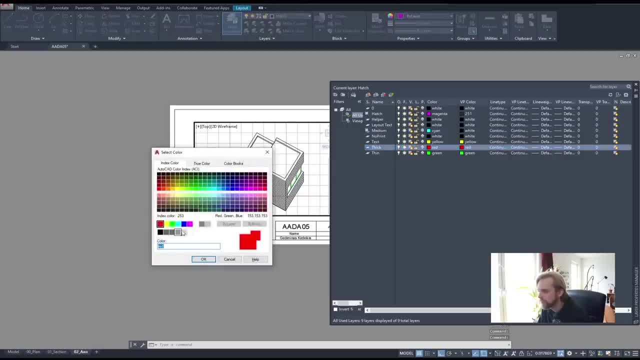 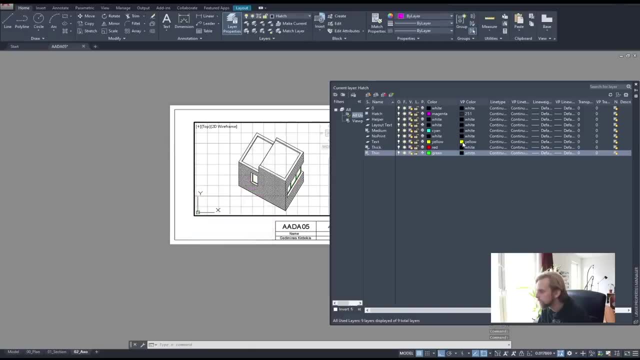 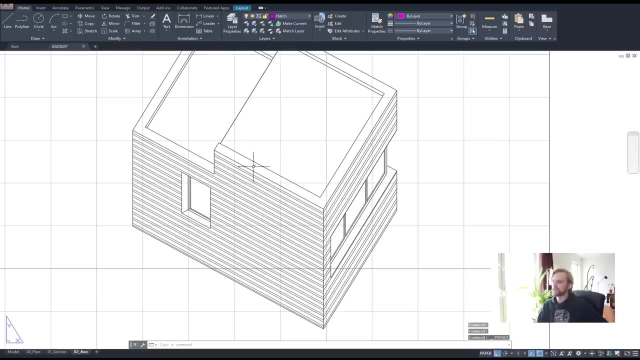 medium line. i'll just go for medium line. i'll just go for black decline, black decline, black decline, black, black, black, thin line, thin line: thin line: uh black, uh black, uh black. text text text: red, red, red, okay, something like that. okay, something like that, okay, something like that. and now you can see. 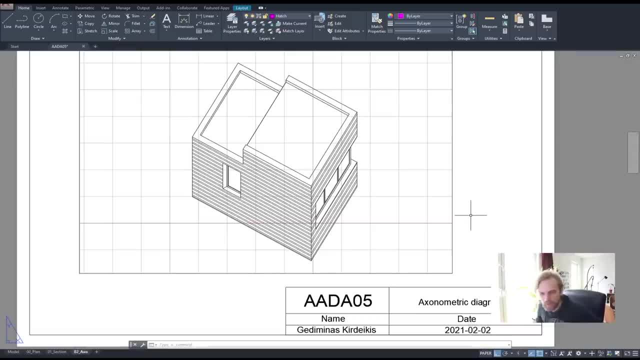 and now you can see. and now you can see um, um, and now you can see um. here the hatch is shown in in in a. here the hatch is shown in in in a. here the hatch is shown in in in a different way, different way, different way, right from from all other layouts. so 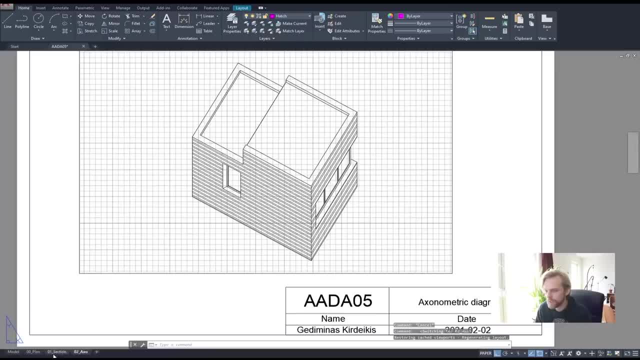 right from from all other layouts, so right from from all other layouts. so that is my, that is my, that is my um. that's my initial setup and that is um. that's my initial setup and that is um. that's my initial setup and that is uh. basically, what, what, what i'm dealing? 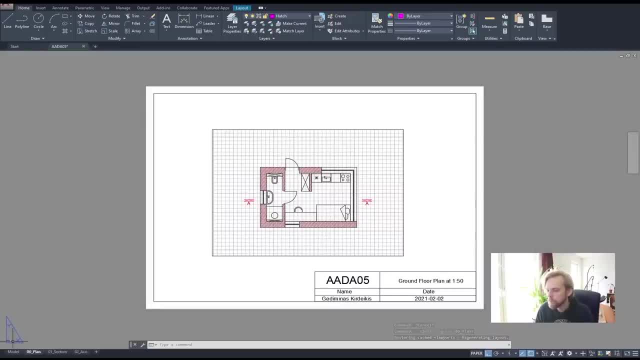 uh, basically what, what what i'm dealing? uh, basically what, what what i'm dealing with with with right now? um, right, so we can go to model space, and right, so we can go to model space, and right, so we can go to model space. and let's see. 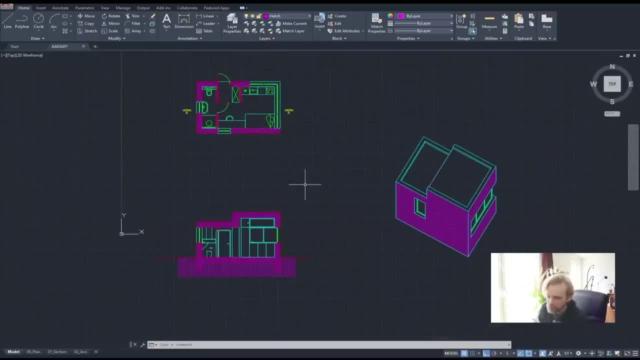 let's see. let's see, what other things do we need to add here? what other things do we need to add here? what other things do we need to add here, right? what kind of other things do, right? what kind of other things do, right? what kind of other things do do we want to add for this particular? 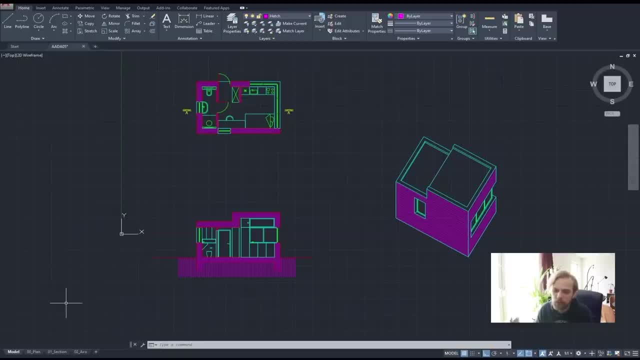 do we want to add for this particular? do we want to add for this particular project, project, project. so let's see how we can import stuff. so let's see how we can import stuff. so let's see how we can import stuff. right, let's see how we can import. 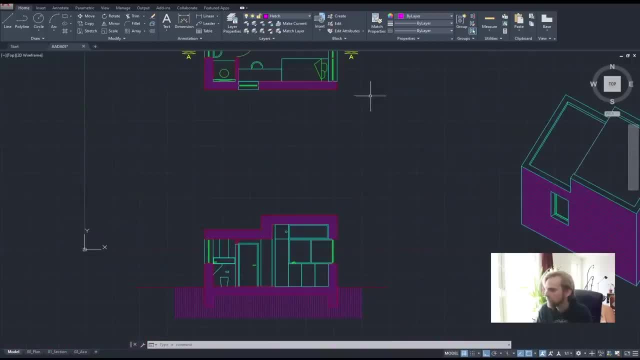 right, let's see how we can import, right, let's see how we can import objects into our scene, such as a person. objects into our scene, such as a person. objects into our scene, such as a person, a tree maybe, maybe a tree for the, a tree, maybe, maybe a tree for the. 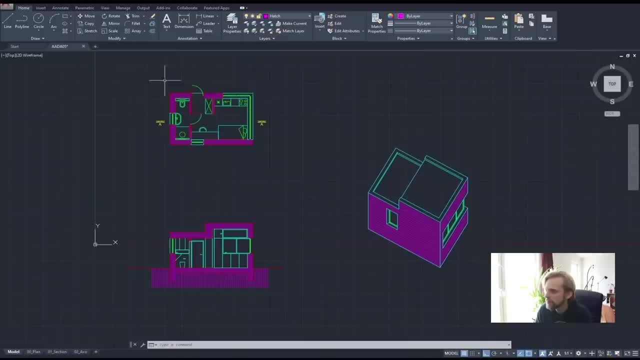 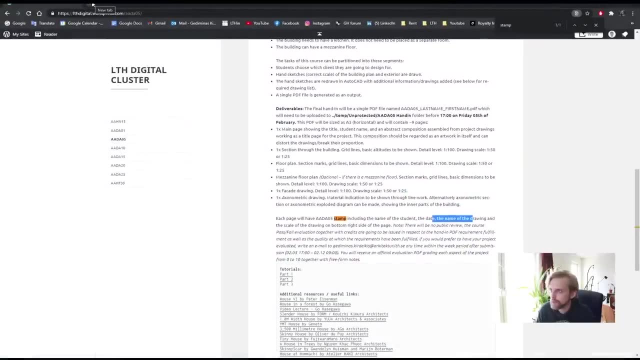 a tree, maybe maybe a tree for the axle, axle, axle, i don't know, i don't know, i don't know. maybe nothing for the plan um. so, maybe nothing for the plan um. so. maybe nothing for the plan um. so, importing, if we go to, importing if we go to 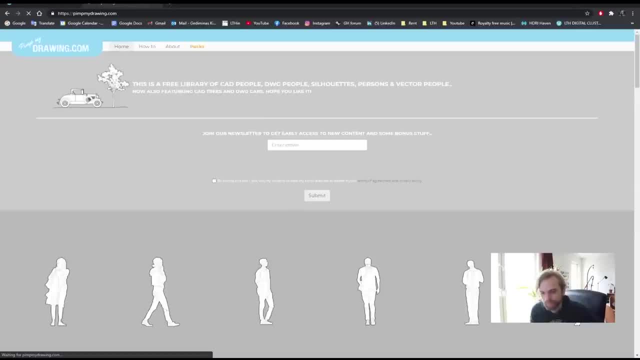 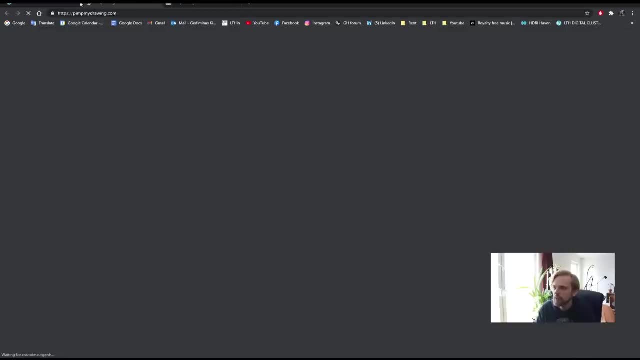 importing if we go to pimp my pimp, my pimp, my drawingcom, drawingcom, drawingcom. the link is right here. the link is right here. the link is right here to the linework library, to the linework library, to the linework library. this link right here. 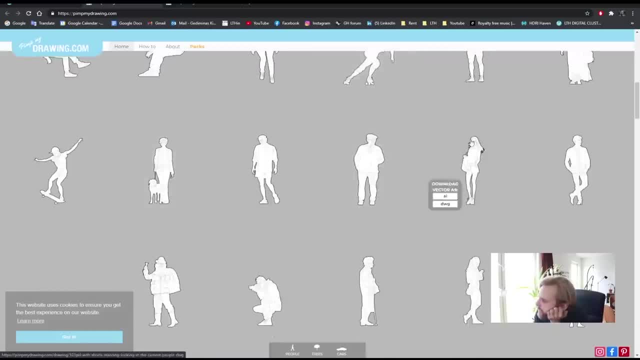 this link right here. this link right here: if we go here, uh, we can find the person. if we go here, uh, we can find the person. if we go here, uh, we can find the person. uh, which which we can use, so i will just uh, which which we can use, so i will just. 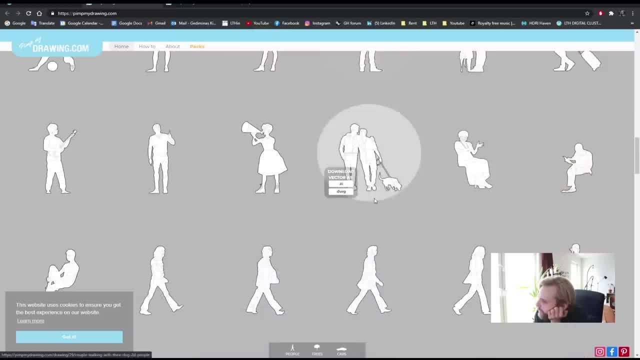 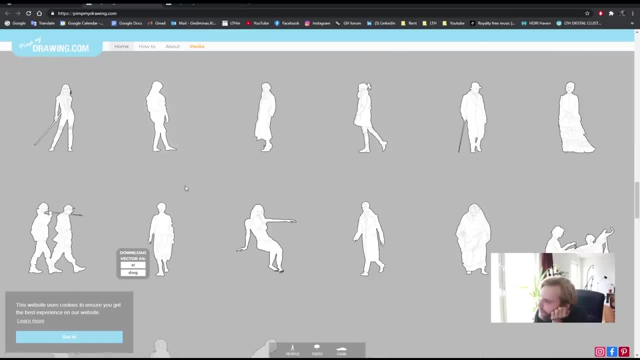 uh, which which we can use. so i will just kind of use a random kind of use. a random kind of use, a random. why are there? why are there? why are there? and that's fine, that's a good one. everyone's kind of posing. i don't want. 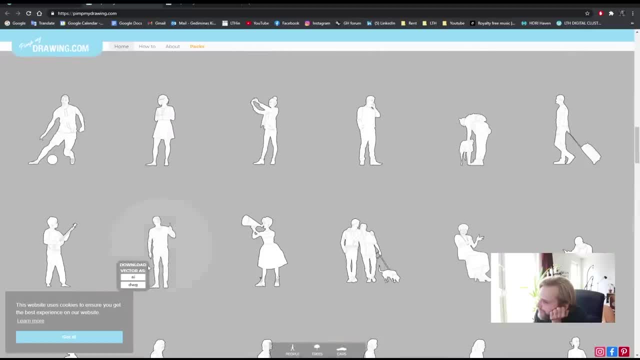 everyone's kind of posing. i don't want everyone's kind of posing. i don't want them to be posing. i'll just get this guy. so i'll just get this guy, so i'll just get this guy. so here we have this person and i can click. 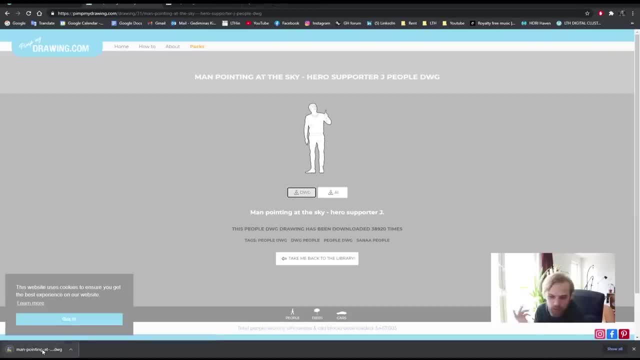 here we have this person and i can click. here we have this person and i can click on on on download the dwg and it just kind of download the dwg and it just kind of download the dwg and it just kind of downloads it right. 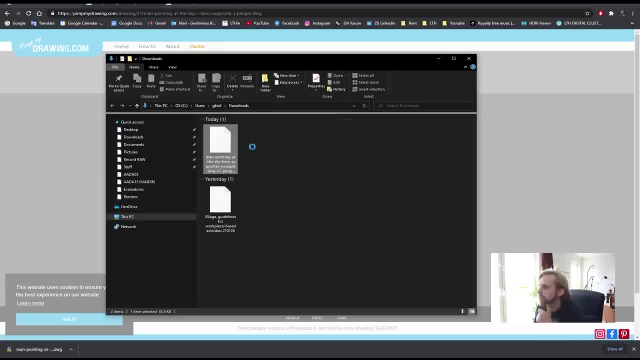 downloads it right, downloads it right and downloads the dwg file, so i'll show. and downloads the dwg file, so i'll show. and downloads the dwg file, so i'll show in folder, in folder, in folder: um, that's uh, that's the. um, that's uh, that's the. 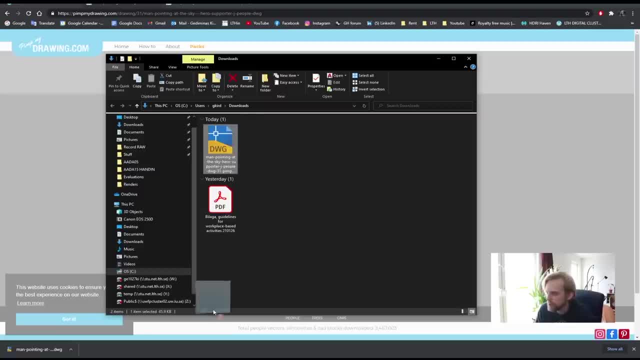 um, that's, uh, that's the dwg file, and all i need to do is just dwg file, and all i need to do is just dwg file, and all i need to do is just click and drag, drag it into. click and drag, drag it into. 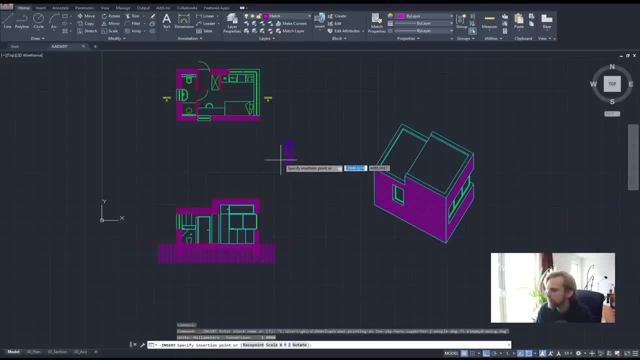 click and drag, drag it into autocad release, autocad release, autocad release. and click and click and click and then just hit enter, enter, enter, and then just hit enter, enter, enter, and then just hit enter, enter, enter. right for for all of the questions. right for for all of the questions. 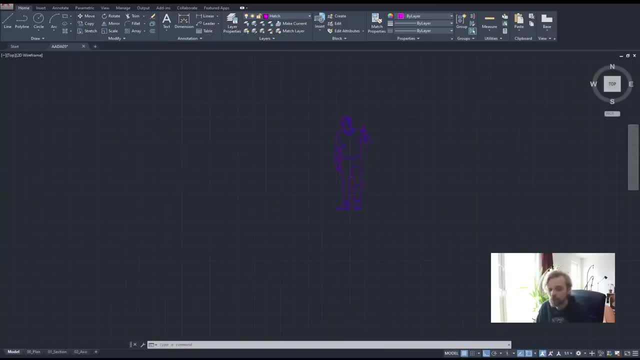 right for for all of the questions: basically, now i have it in autocad. basically, now i have it in autocad. basically, now i have it in autocad. right, that is super simple. right, that is super simple. right, that is super simple. uh, super simple to do. 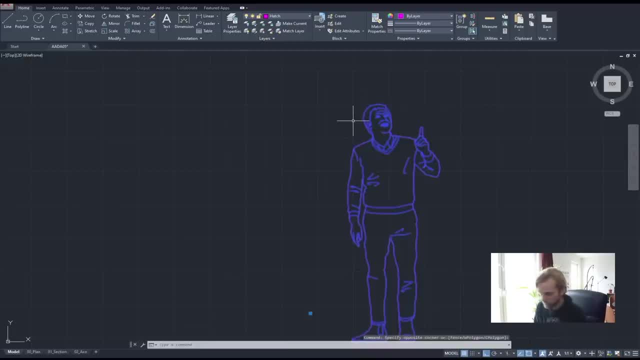 uh, super simple to do. uh, super simple to do, and it is what's called the block, and it is what's called the block, and it is what's called the block, right? so, um, you can see that all of right. so, um, you can see that, all of. 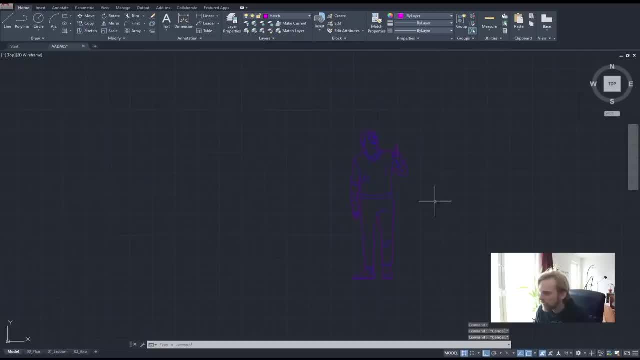 right? so, um, you can see that all of this, this, this selects at the same time and i selects at the same time, and i selects at the same time, and i perhaps i don't want it because this is, perhaps i don't want it because this is. 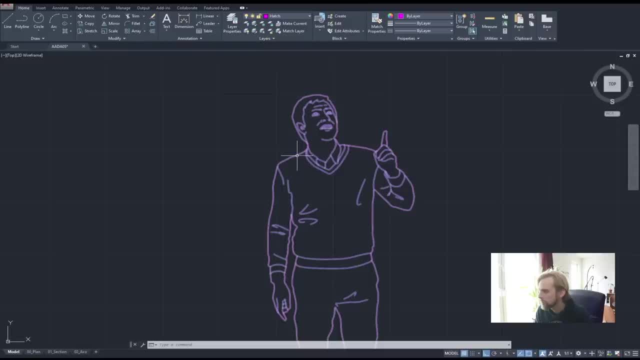 perhaps i don't want it, because this is a little bit too much detail for my type. a little bit too much detail for my type, a little bit too much detail for my type of project, of project, of project. so i will um and on. so i will um and on. 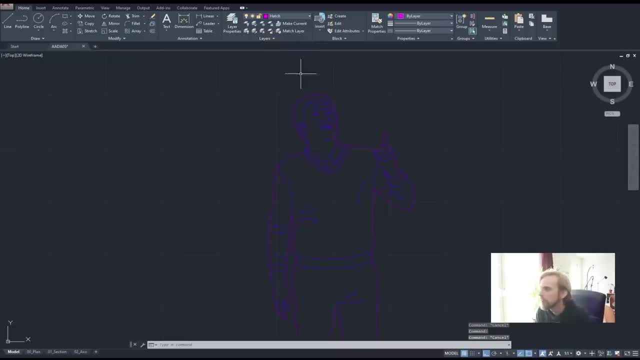 so i will, um and on, sorry one more thing before we kind of sorry one more thing before we kind of sorry one more thing before we kind of look into what a block is it also look into what a block is it also. look into what a block is it also imports with more. 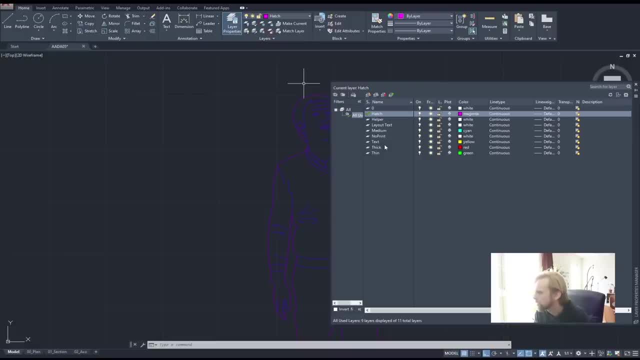 layers, or i guess it doesn't. oh it does, oh it does, oh it does it just lagged, it just lagged, it just lagged. if, if the layers lag, just switch between. if, if the layers lag, just switch between. if, if the layers lag, just switch between all and all used. right, and it's going to. 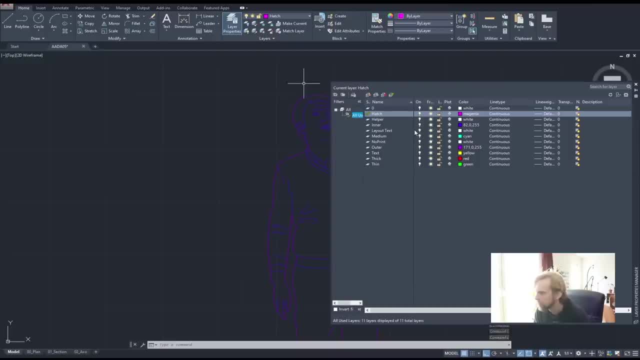 all and all used right, and it's going to all and all used right, and it's going to update autocad. come on, autocad. come on, autocad. come on, um so it, um, so, it, um so it doesn't, um so it doesn't import, with these two layers in our 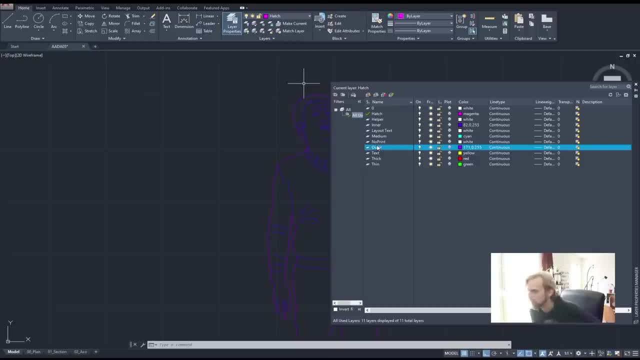 import with these two layers in our import, with these two layers in our outer, which we can just change like any outer, which we can just change like any outer, which we can just change like any other layer right in in the layout, other layer right in in the layout. 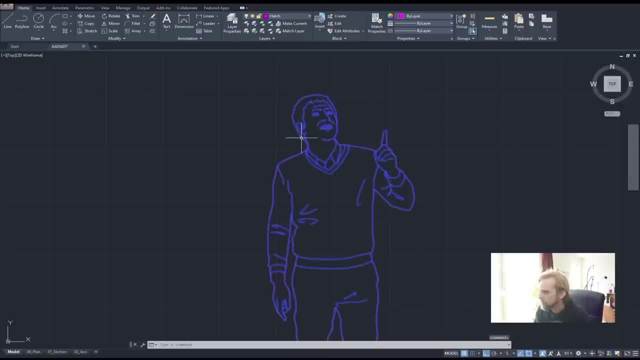 other layer right in in the layout. um, so that's that's good so for this. um, so that's that's good so for this. um, so that's that's good so for this person right here. i will person, right here, i will, person, right here, i will, uh, look at the. 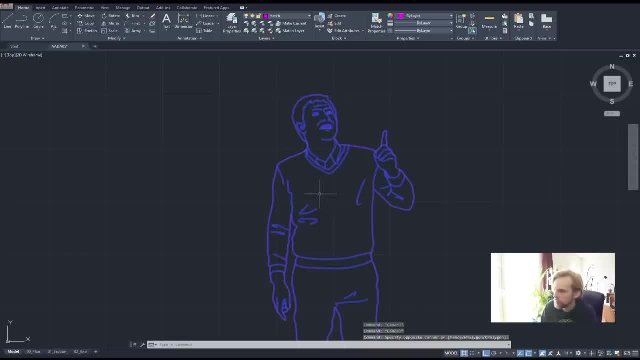 for this, for this, for this: import- right here i will type in import. right here i will type in import. right here i will type in properties, properties, properties, and i can see that it's imported into, and i can see that it's imported into and i can see that it's imported into the hash layer. but that's whatever. but 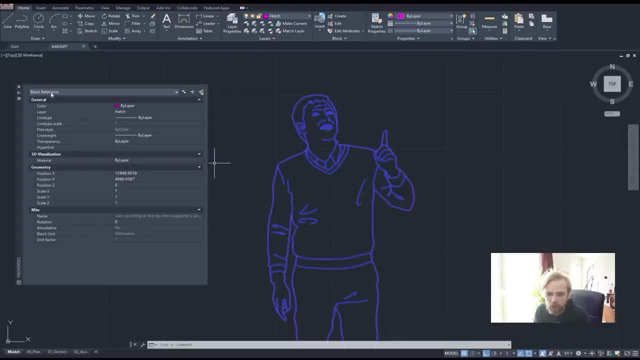 the hash layer, but that's whatever. but the hash layer, but that's whatever. but it's basically well. it doesn't say here: it's basically well. it doesn't say here: it's basically well. it doesn't say here: oh yeah, it does block reference, right. so 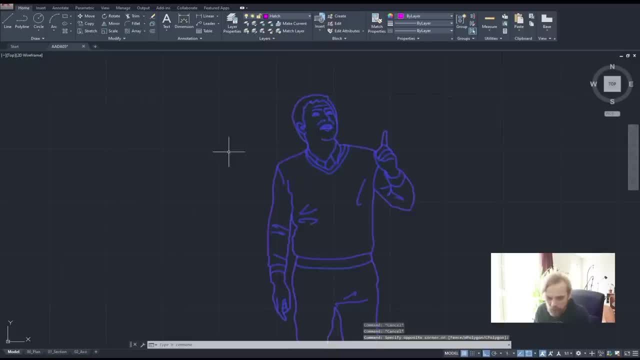 oh yeah, it does block reference right. so, oh yeah, it does block reference right. so this is a block. i don't want it as a. this is a block. i don't want it as a. this is a block. i don't want it as a block. so how do you get rid of it? i want. 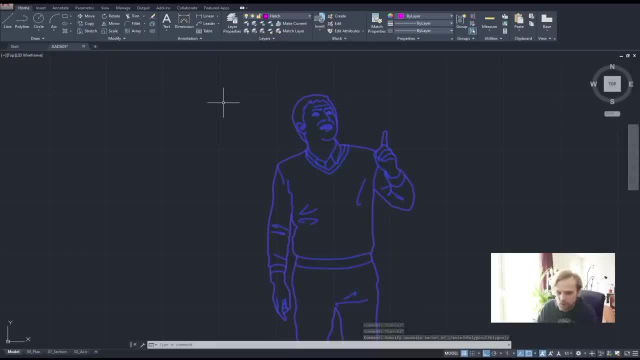 block, so how do you get rid of it? i want block, so how do you get rid of it? i want to use the line separately. how do you to use the line separately? how do you to use the line separately? how do you get rid of it? get rid of it. 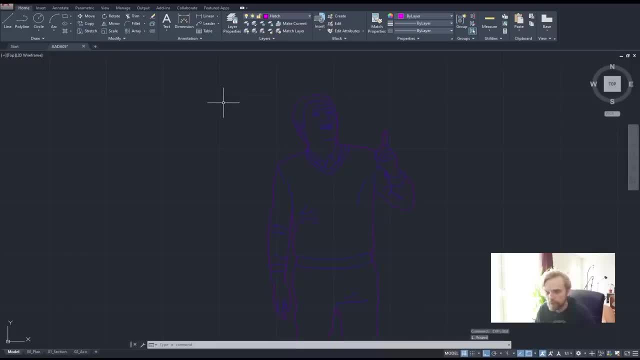 get rid of it from from being a block, you just explode. from from being a block, you just explode. from from being a block. you just explode it. so you select it, you explode it and now so you select it, you explode it and now so you select it, you explode it, and now you have all of the lines. 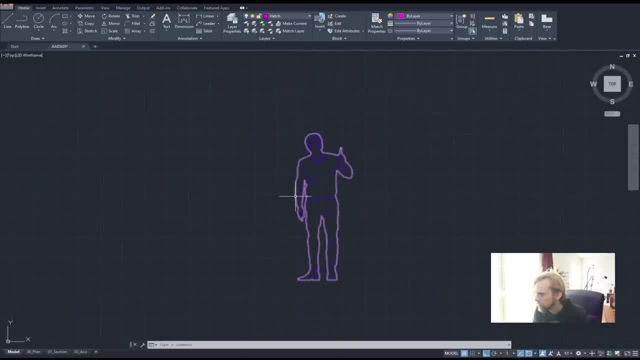 you have all of the lines. you have all of the lines separated right. so i only want the separated right, so i only want the separated right, so i only want the outline of this dude. outline of this dude, outline of this dude. so i'll take the outline and i'll just 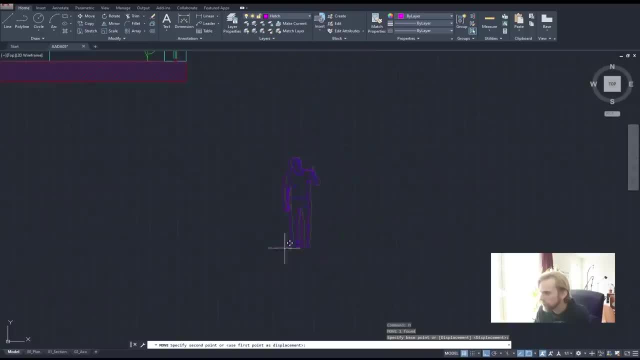 so i'll take the outline and i'll just so i'll take the outline and i'll just move it, move it. move it from let's see the bottom of the the shoe from let's see the bottom of the the shoe from let's see the bottom of the the shoe to somewhere. 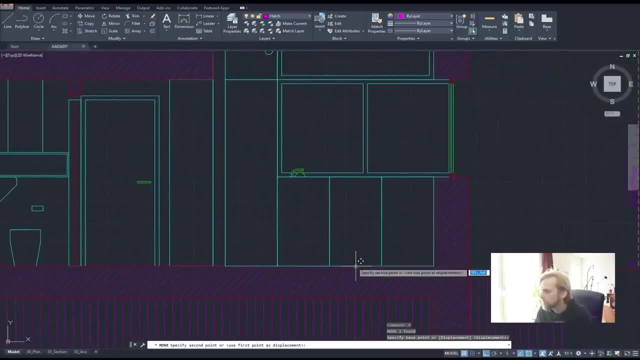 to somewhere, to somewhere, uh, i don't know, uh, i don't know, uh, i don't know- maybe near the window, somewhere here, somewhere here, somewhere here, maybe here, maybe here, maybe here. yeah, somewhere here, so i'll just place. yeah, somewhere here, so i'll just place. 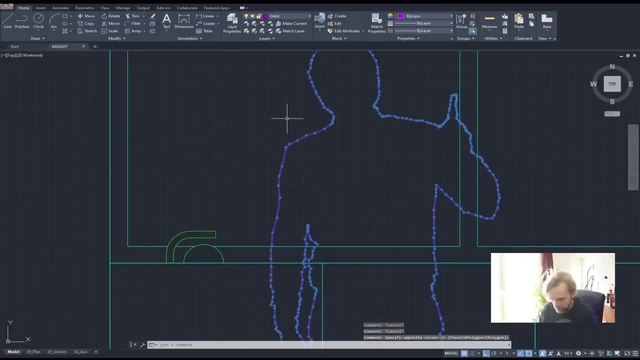 yeah, somewhere here, so i'll just place. place him here right, and then i can just place him here right, and then i can just place him here right, and then i can just use him to trim, use him to trim, use him to trim, uh, trim away the necessary bits. 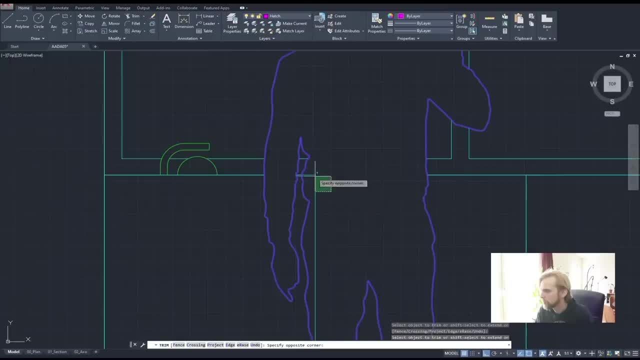 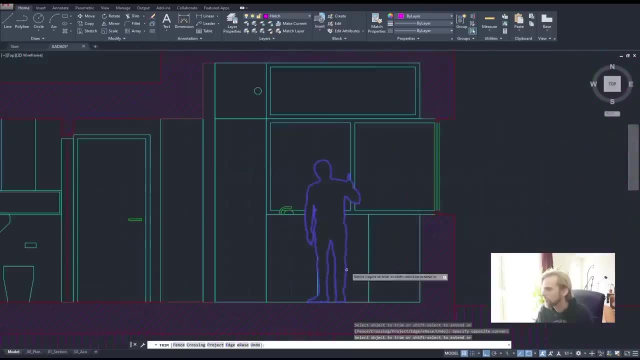 uh, trim away the necessary bits. uh, trim away the necessary bits. um, um, um, you know which, you know which. you know which he's standing in front of. he's standing in front of, he's standing in front of that. that. that like that. okay, that's it. i have my 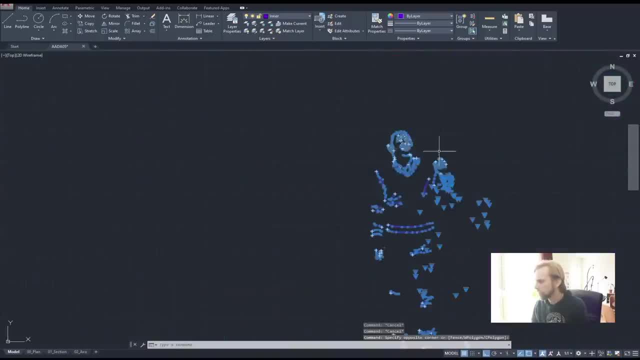 like that. okay, that's it. i have my. like that- okay, that's it. i have my, my silhouette of a person and i don't need my silhouette of a person and i don't need my silhouette of a person and i don't need all of the other lines, so i'll just 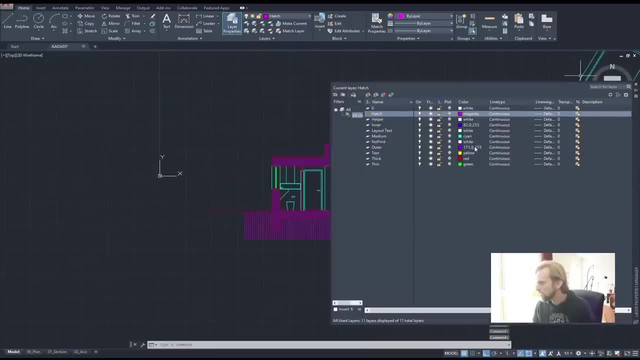 all of the other lines, so i'll just all of the other lines, so i'll just delete them, delete them, delete them, right. so honestly, then i can see that right. so honestly, then i can see that right. so honestly, then i can see that it's only the outer layer, that i'm, i'm. 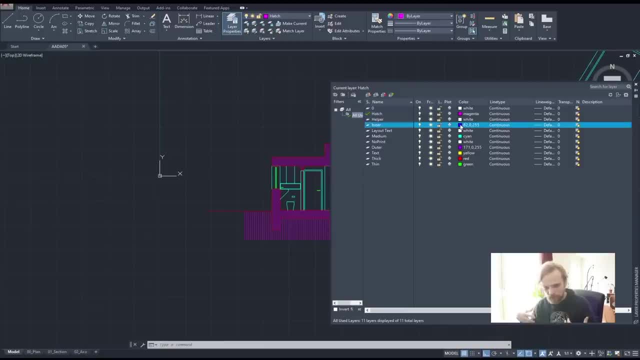 it's only the outer layer that i'm, i'm, it's only the outer layer that i'm. i'm still using the inner layer, still using the inner layer, still using the inner layer, which had all of the lines inside of, which had all of the lines inside of. 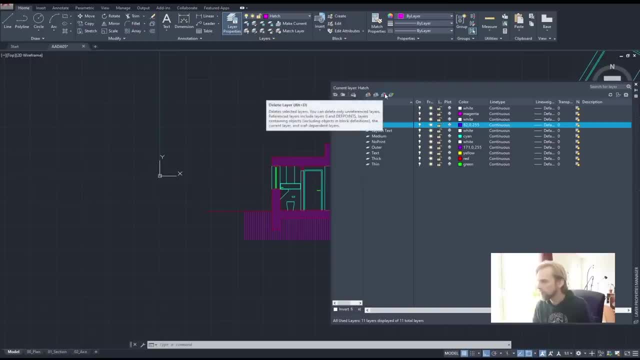 which had all of the lines inside of the person, the person, the person, i. i am not using that anymore, so i'll i. i am not using that anymore, so i'll i. i am not using that anymore, so i'll just delete it. just delete it. just delete it. delete the layer altogether selected. 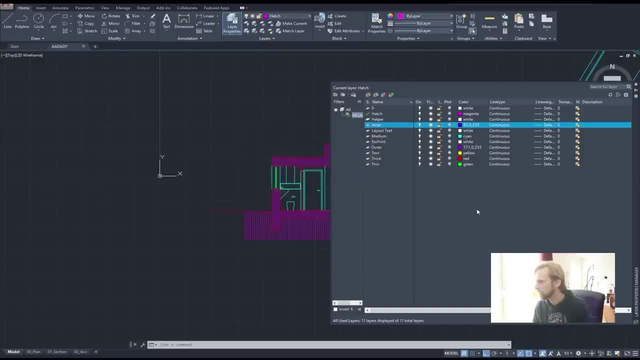 delete the layer altogether selected. delete the layer altogether: selected. layer was not deleted. layer was not deleted. layer was not deleted. i will not be deleting it. i will keep it. i will not be deleting it. i will keep it. i will not be deleting it. i will keep it forever. 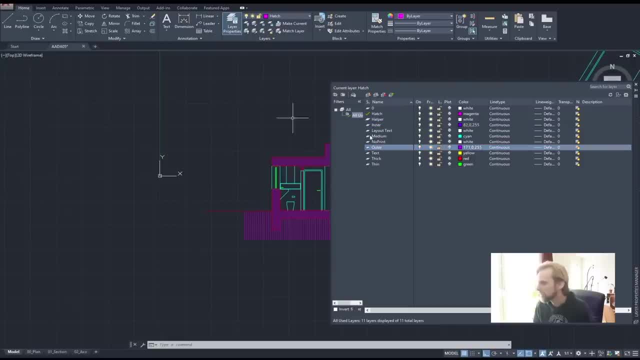 forever, forever. just don't worry about it anyway for the. just don't worry about it anyway for the. just don't worry about it anyway for the outer layer. outer layer, outer layer. uh, i don't care the color in which it's. uh, i don't care the color in which it's. 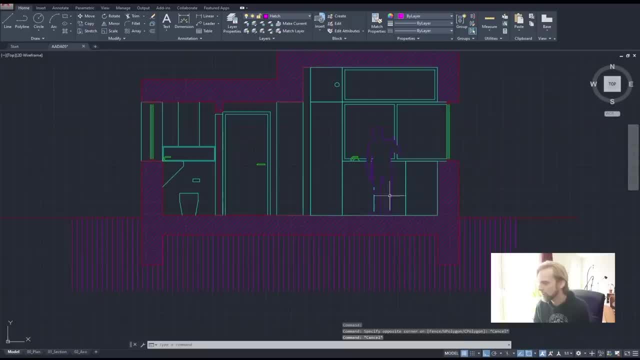 uh, i don't care the color in which it's shown here, but i do care the color in shown here, but i do care the color in shown here, but i do care the color in which it's shown in the layout, which it's shown in the layout. 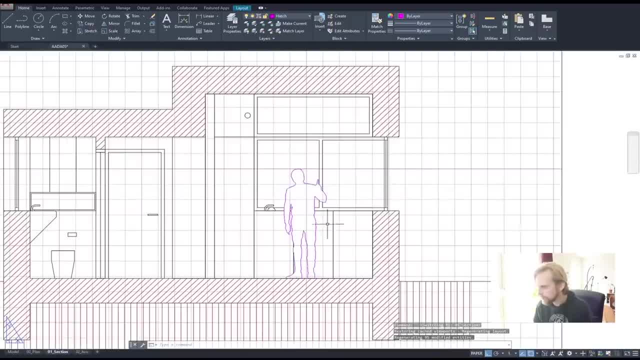 which it's shown in the layout, especially in the section layout right, especially in the section layout right, especially in the section layout right here, here, here, because right now it's purple right, because right now it's purple right, because right now it's purple right. so i'll go, i'll double click inside of. 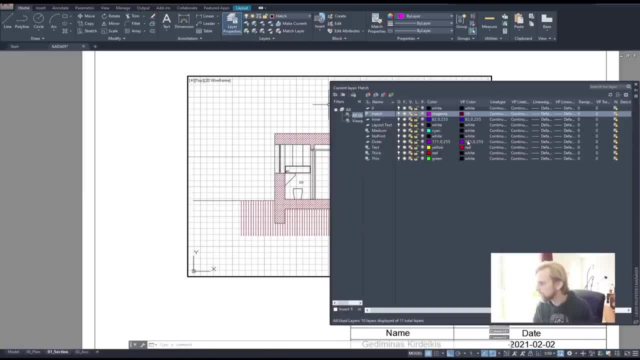 so i'll go, i'll double click inside of. so i'll go, i'll double click inside of that layout, click layer properties and that layout, click layer properties and that layout: click layer properties and change the color to index color. choose index color here and index color. choose index color here and. 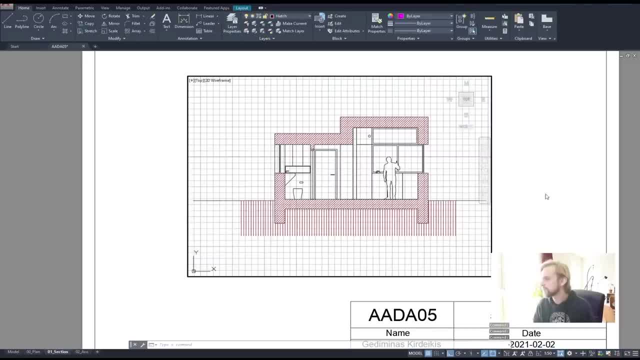 index color. choose index color here, and then to white, then to white, then to white. it close, that's it, double click out. it close, that's it, double click out. it close, that's it, double click out. we're good to go, we're good to go, we're good to go. so that's, that's the. 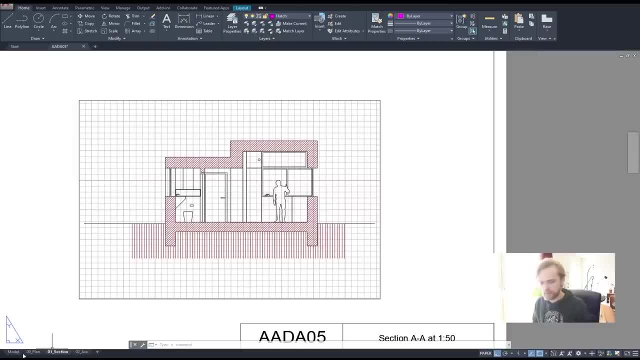 so that's that's the. so that's that's the. the person, the person, the person, um. let me do this again, uh, with the um. let me do this again, uh, with the um. let me do this again, uh, with the trees, trees, trees. so i will just go to my drawingcom. 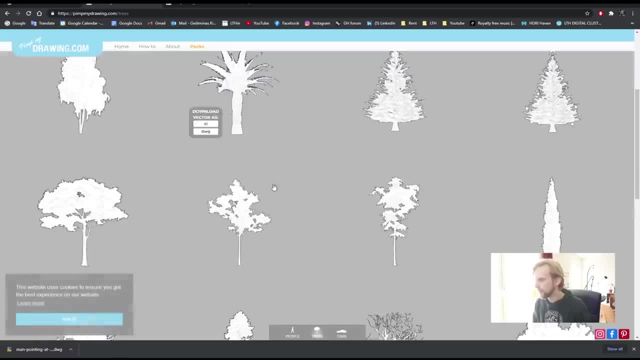 so i will just go to my drawingcom. so i will just go to my drawingcom. uh, here in the bottom i'll choose trees. uh, here in the bottom, i'll choose trees. uh, here in the bottom, i'll choose trees. i'll find a nice little. let's see this. 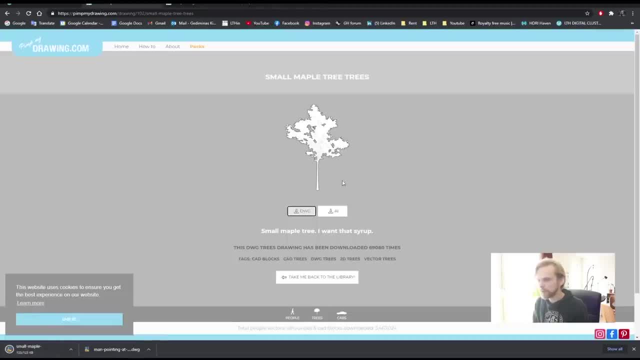 i'll find a nice little. let's see this. i'll find a nice little. let's see this guy right here. uh, download it as dwg guy right here. uh, download it as dwg guy right here. uh, download it as dwg. that's a small maple tree, that's perfect. 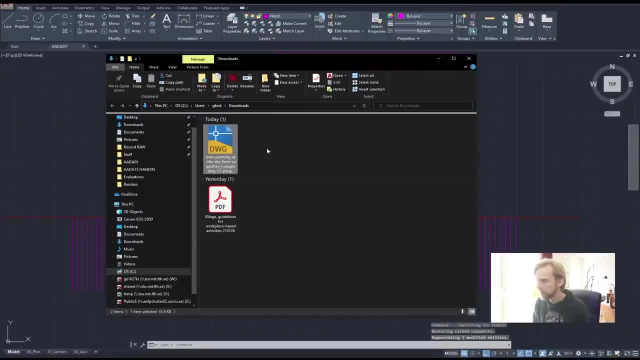 that's a small maple tree. that's perfect. that's a small maple tree. that's perfect in autocad. i'll make sure that i'm in in autocad. i'll make sure that i'm in in autocad. i'll make sure that i'm in my model space. 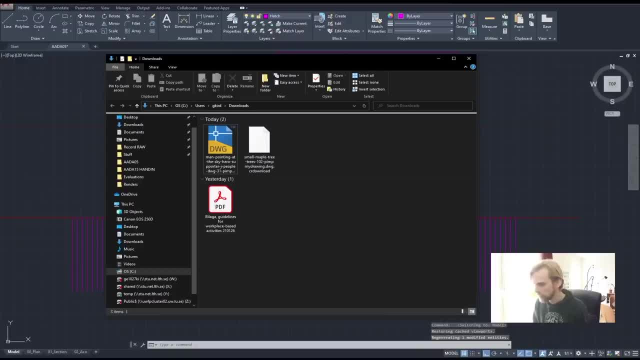 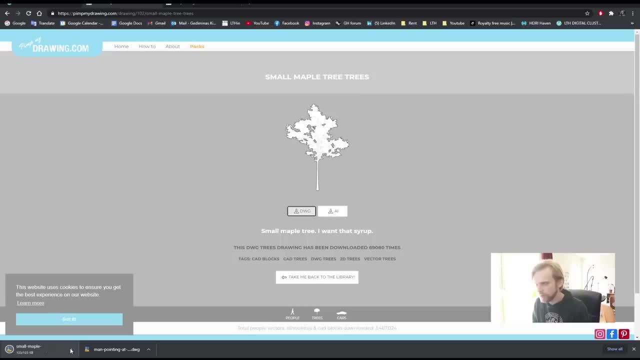 my model space, my model space. where is my maple tree five? it's still. where is my maple tree five? it's still. where is my maple tree five? it's still being downloaded, being downloaded, being downloaded. why is this so slow? why is this so slow? why is this so slow? 123 kilobytes. 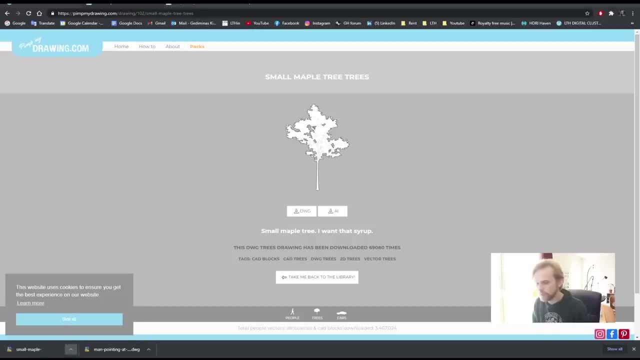 pause, pause, pause. oh okay, it's, it's downloaded actually, um. oh okay, it's, it's downloaded actually, um. oh okay, it's it's downloaded actually, um. so i'll just drag it in. so i'll just drag it in, so i'll just drag it in bam. 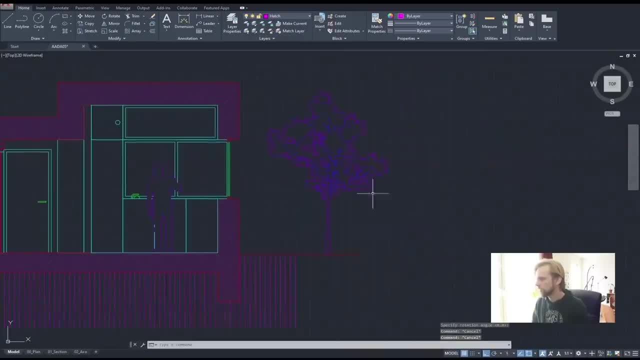 bam bam. i'll just place it like so: enter, enter. i'll just place it like so: enter, enter. i'll just place it like so: enter, enter, enter. so i have my small little maple. enter. so i have my small little maple. enter. so i have my small little maple tree. maybe i'll scale it up. 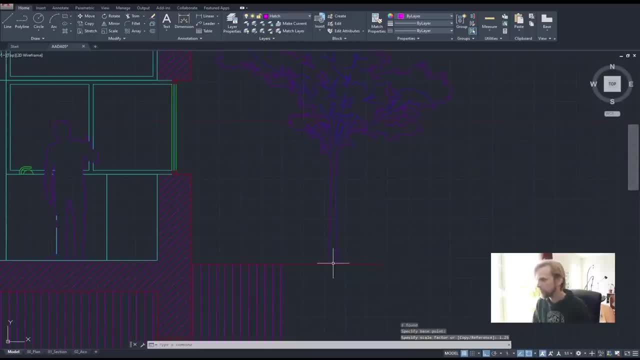 tree. maybe i'll scale it up. tree. maybe i'll scale it up um from this point: 1.25. um from this point: 1.25. um from this point: 1.25. just 125 percent. so that is a little bit. just 125 percent, so that is a little bit. 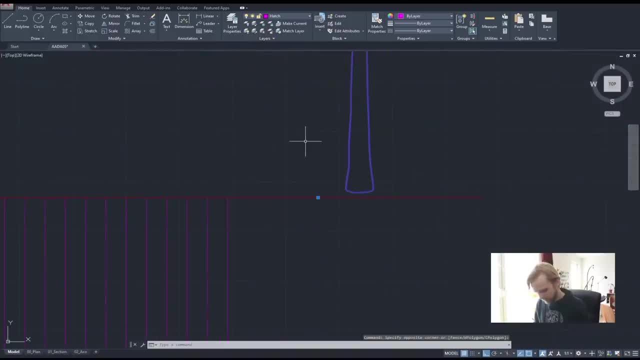 just 125 percent. so that is a little bit larger than the, larger than the, larger than the, than the building, and i will move it than the building and i will move it than the building and i will move it down, down, down. so i think that's that, that that looks. 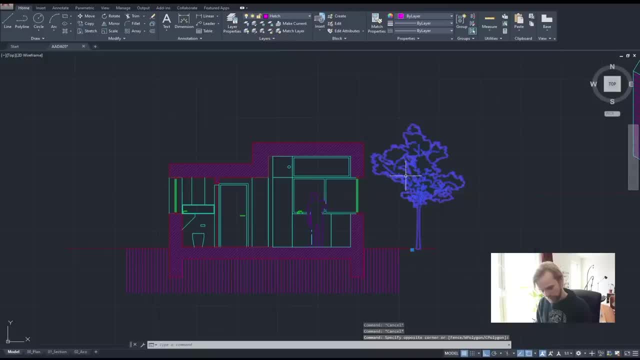 so i think that's that, that that looks. so i think that's that that that looks fine, fine, fine, um, perhaps i want it on the other side. um, perhaps i want it on the other side. um, perhaps i want it on the other side as well. so i'll just make a copy of it. 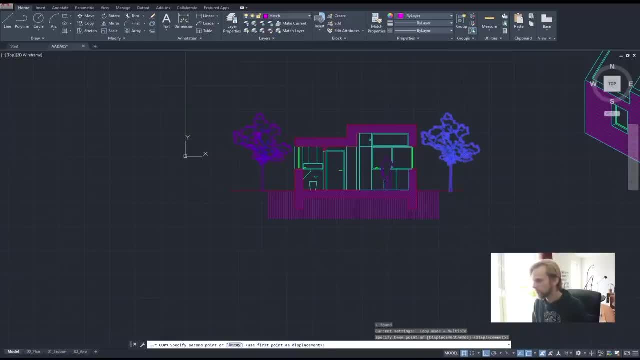 as well. so i'll just make a copy of it as well. so i'll just make a copy of it. i'll keep it as a blog, by the way in in. i'll keep it as a blog, by the way in in. i'll keep it as a blog by the way in in this case, because i don't really 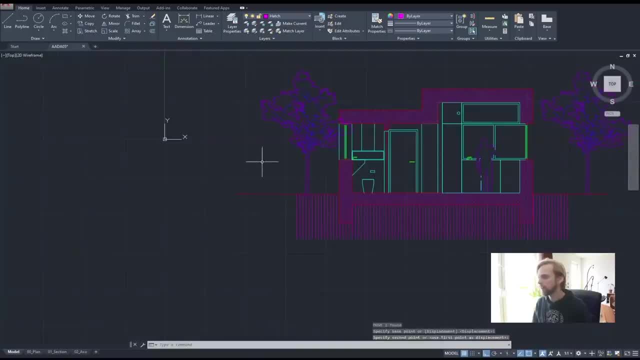 this case, because i don't really this case, because i don't really well in in case where the maple tree, well in in case where the maple tree, well in in case where the maple tree kind of goes, kind of goes, kind of goes behind the building, i would need to. 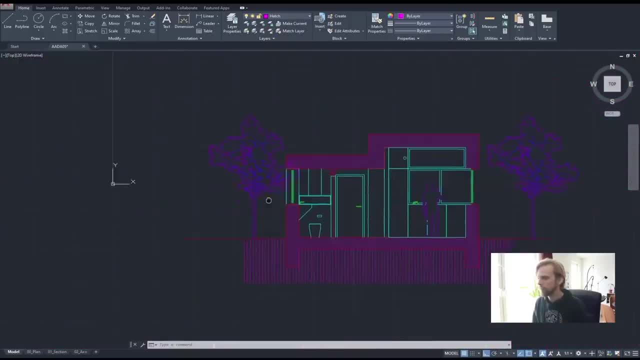 behind the building. i would need to behind the building, i would need to explode it and trim it away, explode it and trim it away, explode it and trim it away. but in other cases i don't, maybe i will. but in other cases i don't, maybe i will. 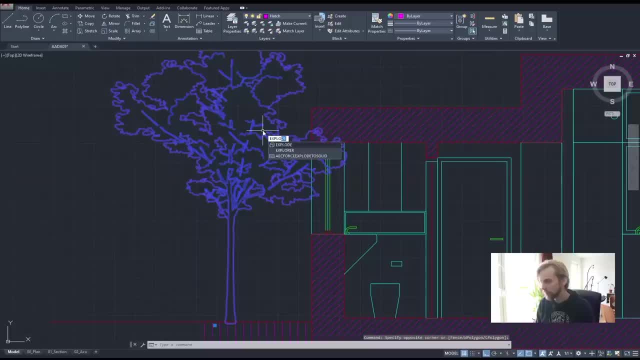 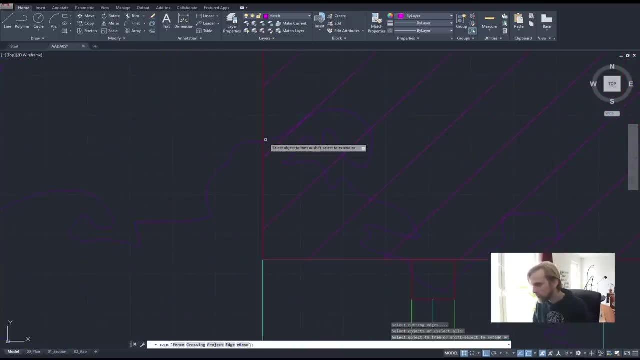 but in other cases i don't maybe i will. just to show you, just to show you, just to show you: explode, explode, explode. so i explode the block, so i explode the block, so i explode the block. trim enter, enter and i just trim away. trim enter, enter and i just trim away. 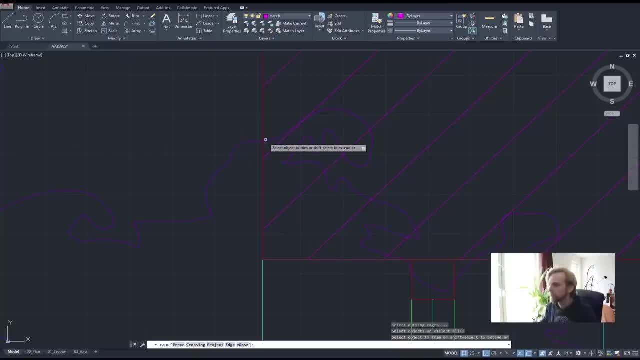 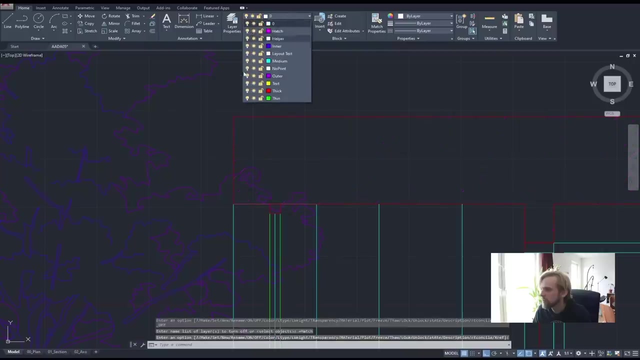 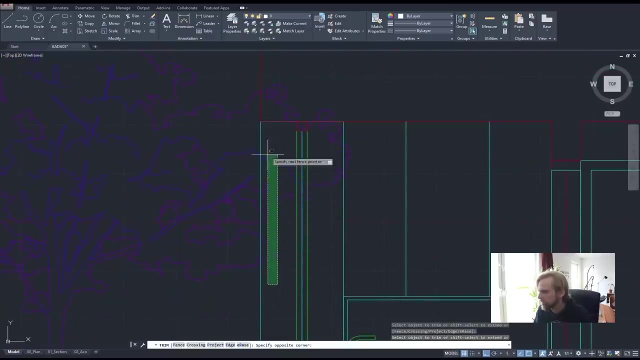 trim, enter, enter and i just trim away the oh, the oh, the oh. that's gonna be super laggy. my mouse is, that's gonna be super laggy. my mouse is that's gonna be super laggy. my mouse is frozen, frozen, frozen. too many lines. 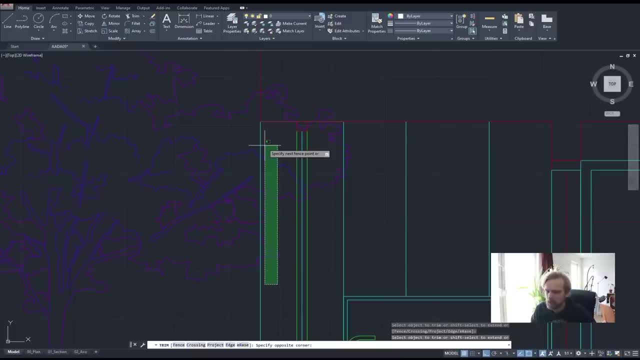 if it lags for you as well, this, this. if it lags for you as well, this, this. if it lags for you as well, this, this hard: just don't trim the trees hard. just don't trim the trees hard. just don't trim the trees right. just just don't don't have them. 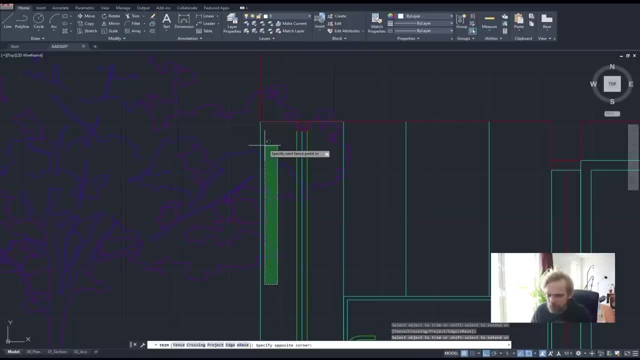 right, just just don't don't have them right, just just don't don't have them trimmed, trimmed, trimmed, um, um, um, i'll go make some coffee. while while i'll go make some coffee, while, while i'll go make some coffee, while while. this is, this is. 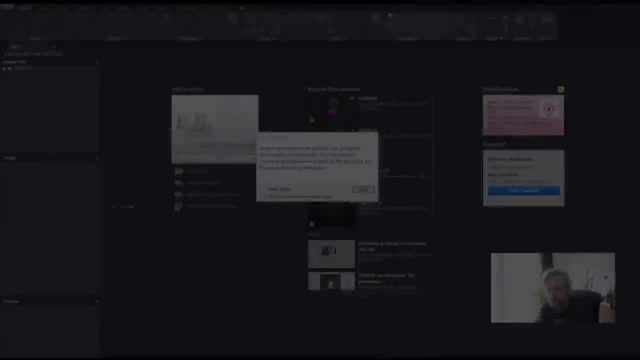 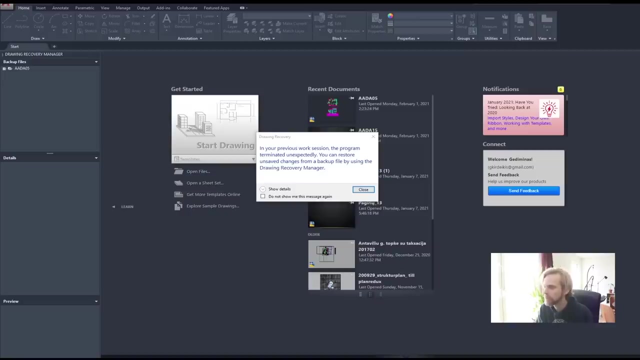 this is crashing and then we will continue: yep, so it completely crashed. yep, so it completely crashed. yep, so it completely crashed. which actually, which actually, which actually, i will use, i will use. i will use as an opportunity to show you how to, as an opportunity to show you how to. 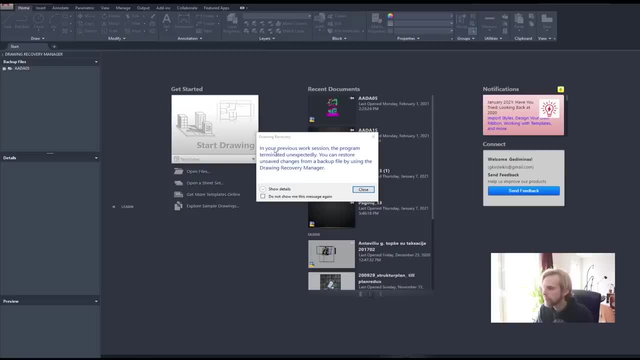 as an opportunity to show you how to. if you have a crash. what can you do if you have a crash? what can you do if you have a crash? what can you do about it? about it, about it, right so when you load autocad again, right so when you load autocad again. 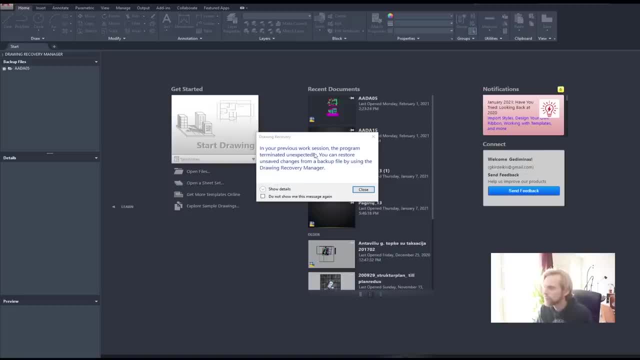 right. so when you load autocad again, it's going to say that in your previous, it's going to say that in your previous, it's going to say that in your previous work session, work session, work session- the program terminated unexpectedly- blah. the program terminated unexpectedly, blah. 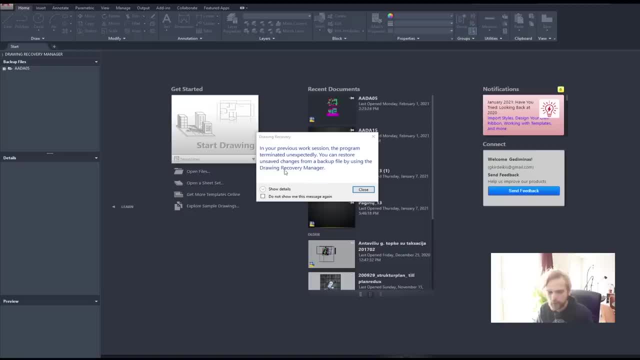 the program terminated unexpectedly, blah blah. and you can get a backup from your. and you can get a backup from your. and you can get a backup from your drawing recovery manager. drawing recovery manager. drawing recovery manager. cool, let's see how much it's saved. so cool, let's see how much it's saved. so. 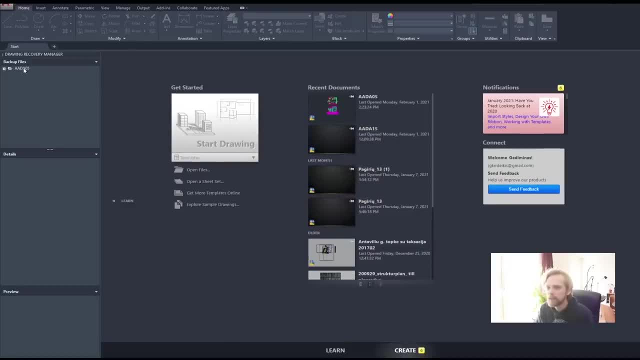 cool. let's see how much it's saved. so i'll just hit close. i'll just hit close. i'll just hit close, right here and i'll here on the left, right here and i'll here on the left, right here and i'll here on the left hand side of the screen. i can see my. 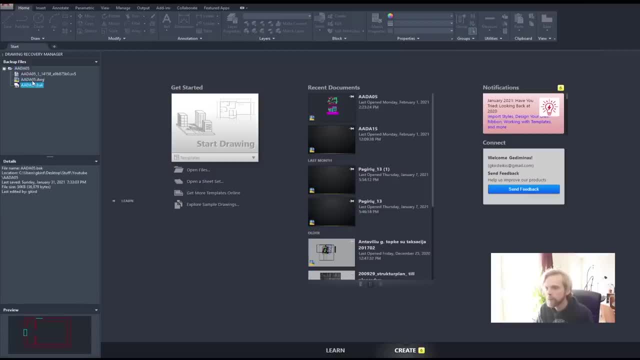 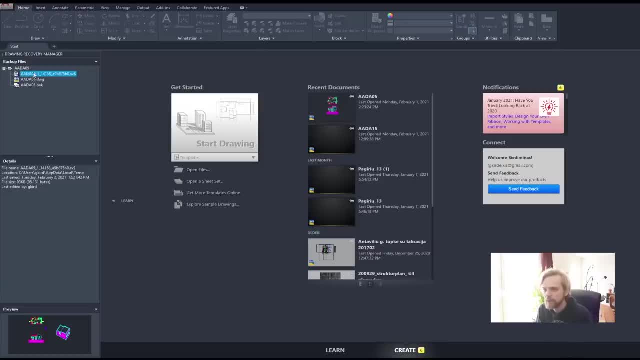 that is not good at all. let's see this one, let's see this one, let's see this one, let's see this guy right here. so as as. let's see this guy right here, so as as. let's see this guy right here, so as, as you're clicking through it, you can see. 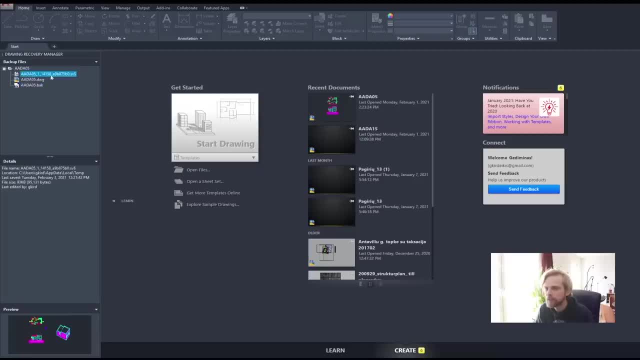 you're clicking through it, you can see, you're clicking through it, you can see, like these three versions and a8005, like these three versions and a8005, like these three versions and a8005, that the weird one, that the weird one, that the weird one, uh, kind of looks like there there is a guy. 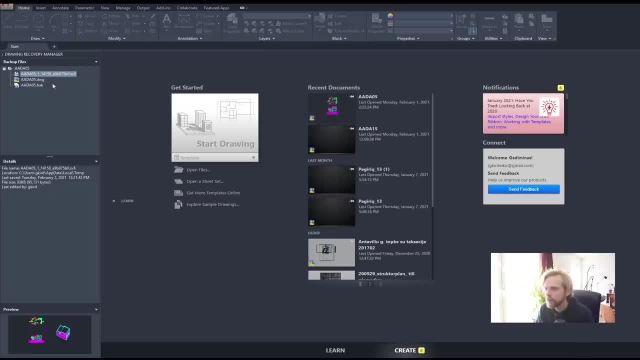 uh, kind of looks like there there is a guy. uh kind of looks like there there is a guy there, there, there. um, so at least that is, it has been saved. um, so, at least that is, it has been saved. um, so, at least that is, it has been saved. so i'm just going to double click on that. 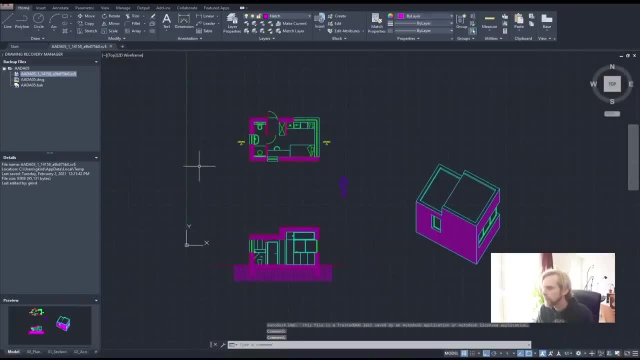 so i'm just going to double click on that. so i'm just going to double click on that and open it up, and that seems to be okay. um, at least it. and that seems to be okay. um, at least it. and that seems to be okay. um, at least it does have. 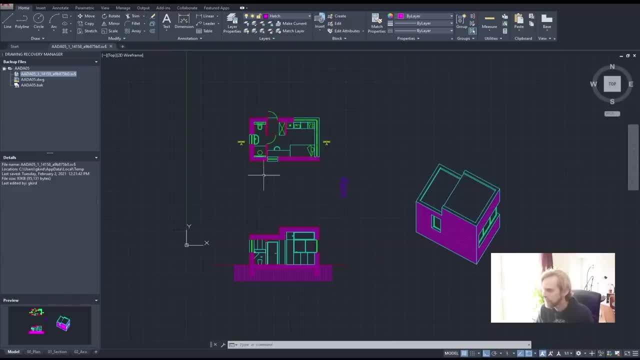 does have, does have the the stuff, uh like that, most of the the the stuff, uh like that, most of the the the stuff, uh like that, most of the stuff, that stuff, that stuff. that i have done so we're not missing too. i have done so, we're not missing too. 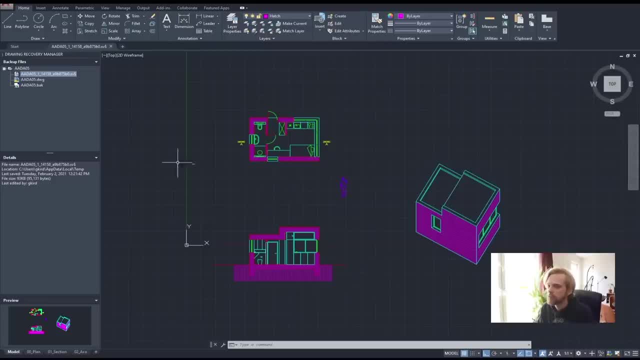 i have done so we're not missing too much, much, much. and let me change the camera exposure, uh, and let me change the camera exposure, uh, and let me change the camera exposure, uh, we're not missing too much. so we're not missing too much. so we're not missing too much. so i will just really quickly um. 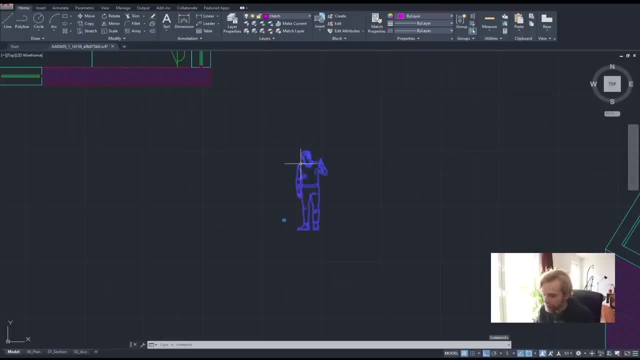 i will just really quickly, um, i will just really quickly, um, recreate what i have been doing and this recreate what i have been doing and this recreate what i have been doing, and this time around i will not be trimming the time around, i will not be trimming the. 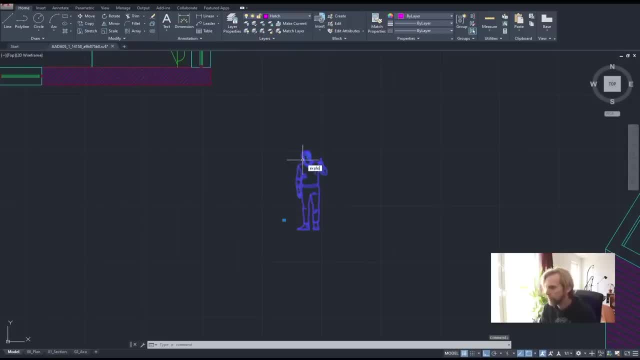 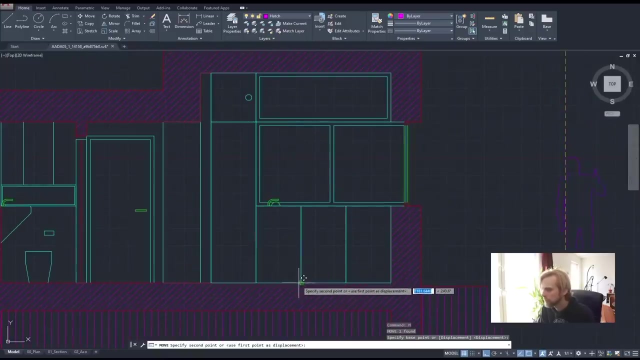 time around. i will not be trimming the trees, that's for sure. trees, that's for sure. trees, that's for sure. so let's float that. so that, get the outline move it. so that, get the outline move it. so that, get the outline move it. m it's from here to wherever it was. 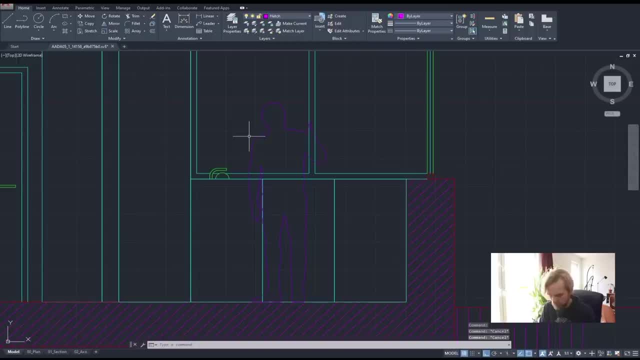 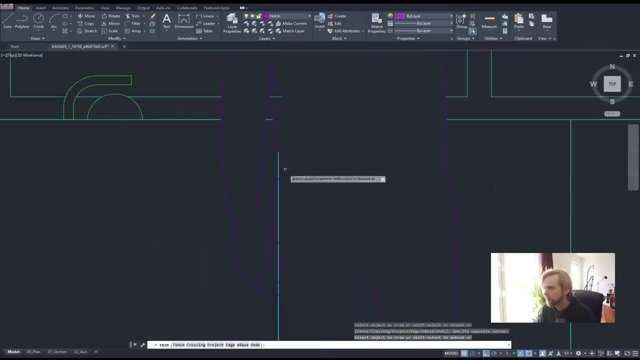 it's from here to wherever it was, it's from here to wherever it was. over here, fine, over here, fine, over here, fine, trim, enter, enter, wonder what's up with the trees. and then wonder what's up with the trees, and then wonder what's up with the trees, and then then crashing. it never used to crash. 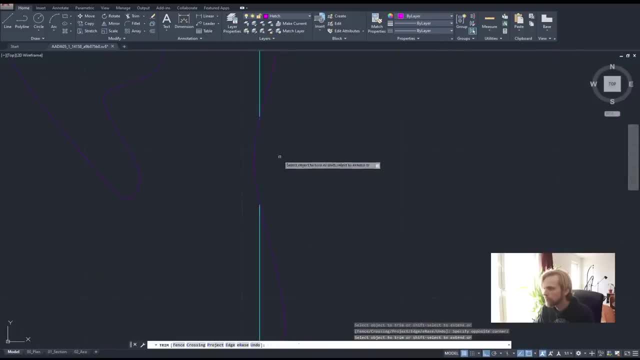 then crashing it never used to crash. then crashing it never used to crash before. maybe the new before, maybe the new before. maybe the new version really doesn't like the amount version, really doesn't like the amount version, really doesn't like the amount of points that the three polar lines. 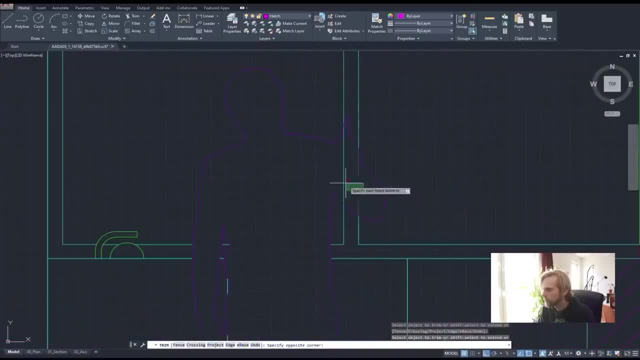 of points that the three polar lines, of points that the three polar lines have, have, have, uh, that's probably the the culprit. uh, that's probably the the culprit. uh, that's probably the the culprit behind it, behind it, behind it. uh, so just keep an eye out for that, uh. 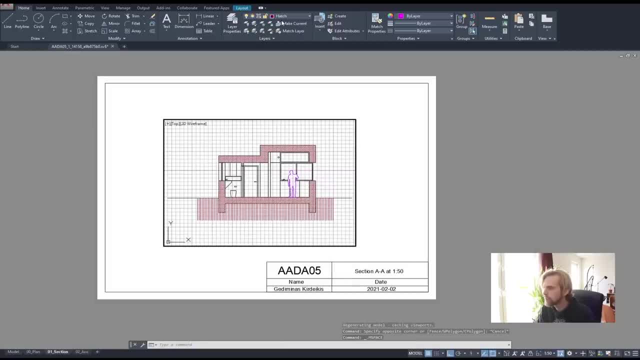 uh, so just keep an eye out for that. uh, uh, so just keep an eye out for that. uh, either way, this is fine. and now we just: either way, this is fine. and now we just: either way, this is fine. and now we just go to section and we change the. 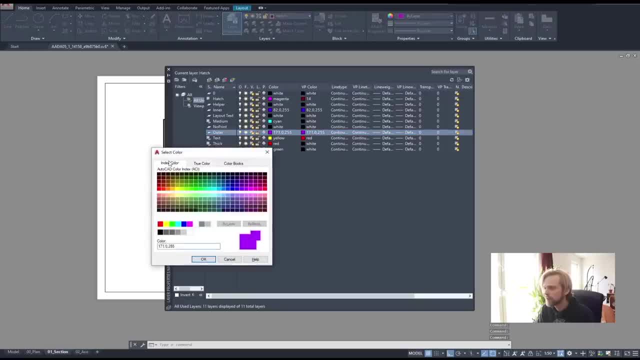 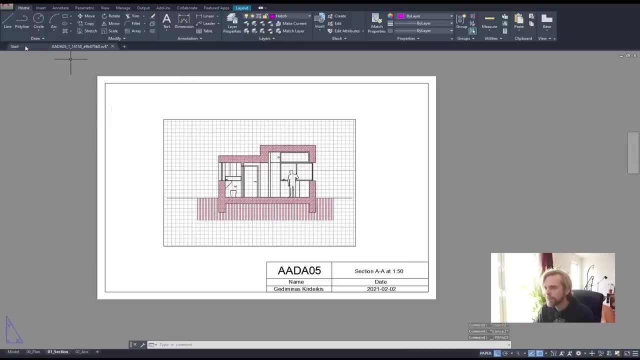 go to section and we change the go to section and we change the. the color of the outer line here. the color of the outer line here. the color of the outer line here to to, to white. there we go, um like that. there we go, um like that. 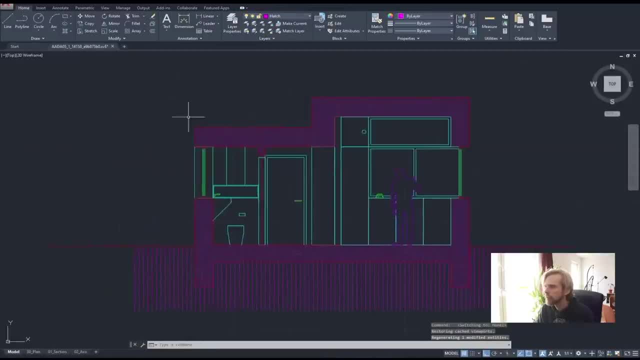 there we go, um like that: oops, oops, oops, go back to model. and uh, just to be sure i go back to model. and uh, just to be sure i go back to model. and uh, just to be sure i will save now. uh, keep saving. 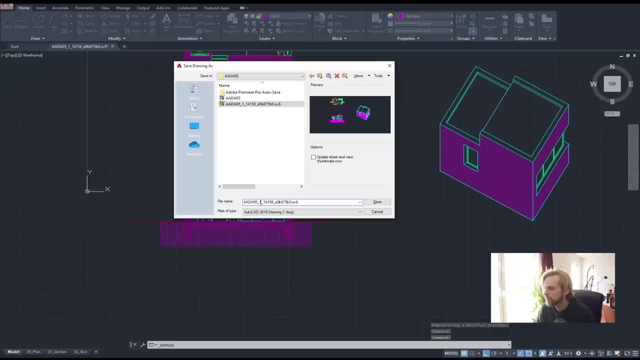 will save now, uh, keep saving. will save now, uh, keep saving. so i'll just save it um as 80 05. so i'll just save it um as 80 05, so i'll just save it um as 80 05, um, um, um new. 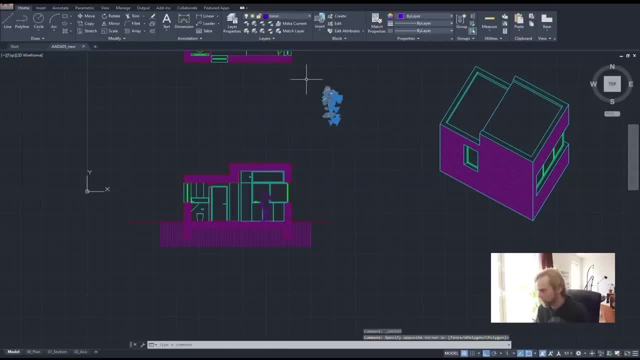 new, new, it's safe, it's safe, it's safe. there we go okay. so, oh yeah, and we don't there, we go okay. so oh yeah, and we don't there, we go okay. so oh yeah, and we don't need those, need those, need those. so the trees. 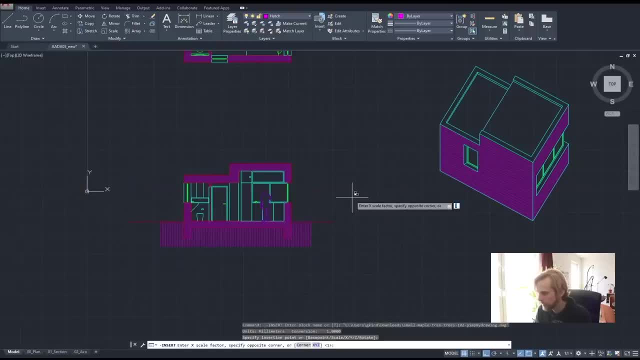 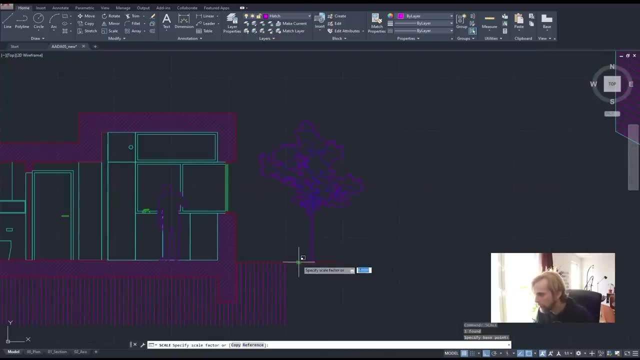 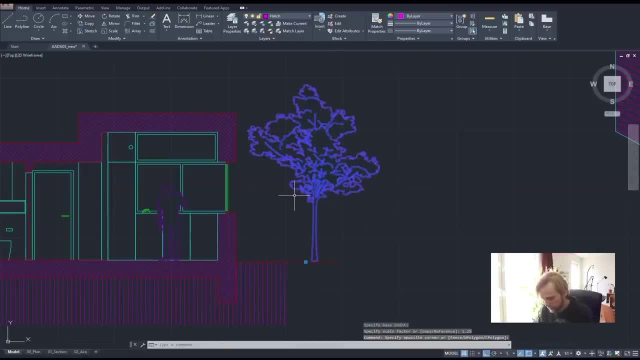 scale. scale from here 1.25, from here 1.25, from here 1.25, just a little bit bigger. just move it just a little bit bigger. just move it just a little bit bigger. just move it slightly down, so that it's kind of. 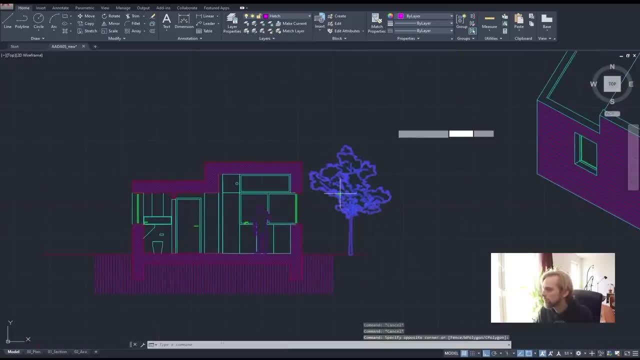 slightly down, so that it's kind of slightly down, so that it's kind of positioned, correctly copied to the other, positioned correctly copied to the other, positioned correctly copied to the other side, side side. my god, my god, my god, that's fine. um, it is what it is. so we 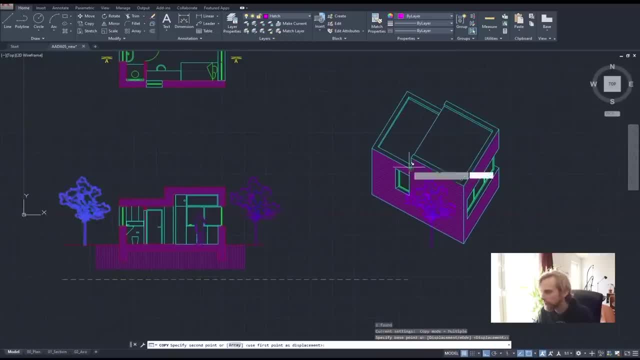 that's fine. um, it is what it is. so we, that's fine. um, it is what it is. so we have our trees here and i'll actually have our trees here, and i'll actually have our trees here, and i'll actually copy, copy, copy, um, um, 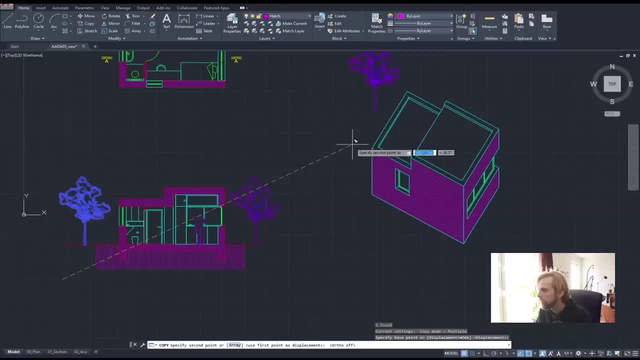 um, f8, f8, f8, just have a proper copy here. i'll say: just have a proper copy here. i'll say: just have a proper copy here. i'll say that one tree is located here, while the that one tree is located here, while the that one tree is located here, while the other one is kind of located somewhere. 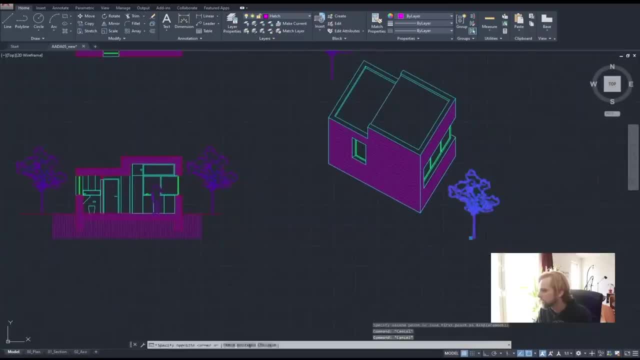 other one is kind of located somewhere. other one is kind of located somewhere here, here, here. maybe this one is, maybe this one is, maybe this one is actually here and it's actually actually here and it's actually actually here and it's actually a little bit bigger than the other one. 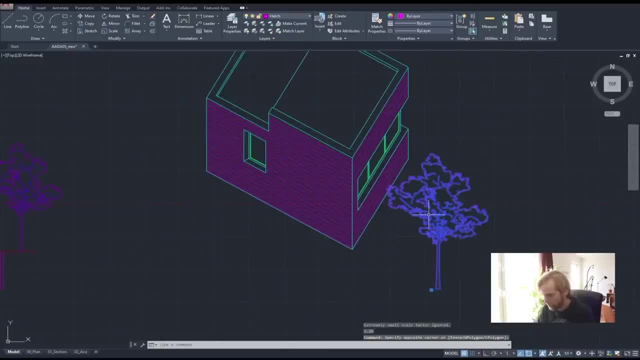 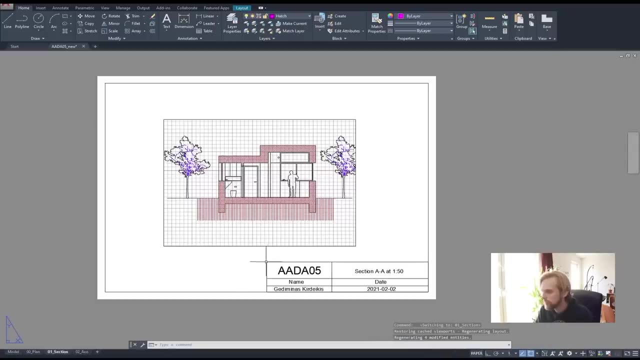 a little bit bigger than the other one, a little bit bigger than the other one. 1.25 again, 1.25 again, 1.25 again, like that. so let's look at it in this, like that. so let's look at it in this. 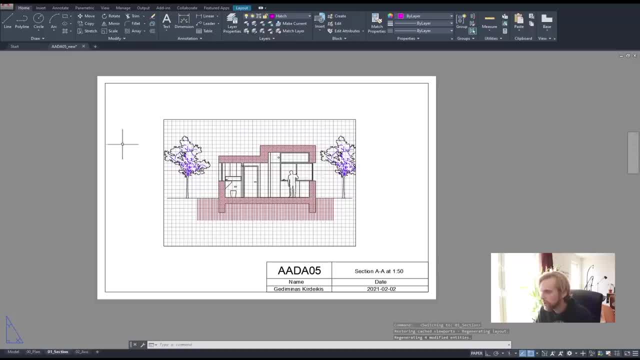 like that. so let's look at it in this section. so in this section i can see section. so in this section i can see section. so in this section i can see that the trees are being blocked off by that. the trees are being blocked off by that. the trees are being blocked off by the frame a little bit. so i'm going to. 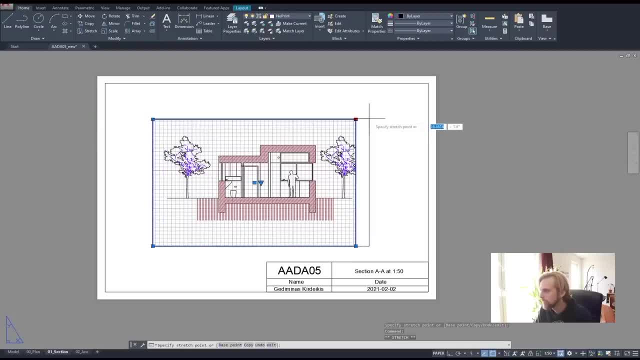 the frame a little bit. so i'm going to the frame a little bit, so i'm going to move the frame, move the frame, move the frame like that, like that, like that, and like that, and like that, and like that, just so that they are being shown. 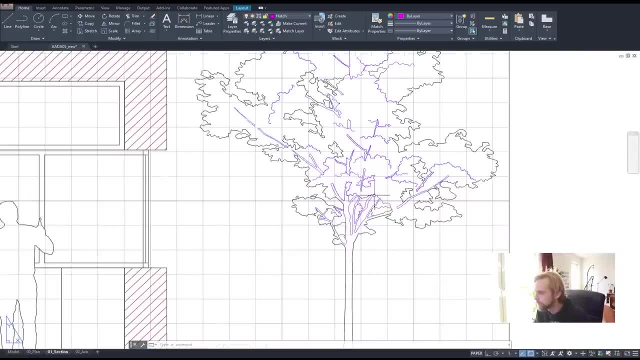 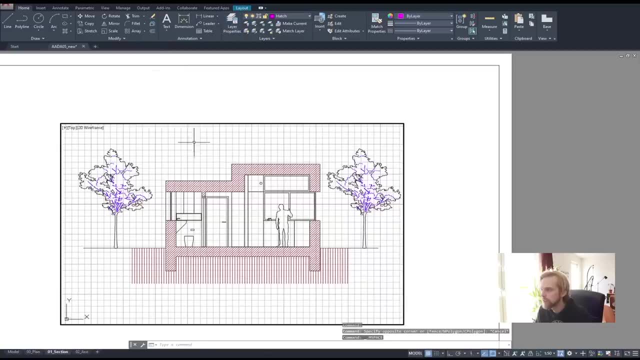 just so that they are being shown. just so that they are being shown. and also i will change the inner- uh, inner- areas of the trees to have a different color. so i'll go to oops. i first need to double click inside. i'll go to layer properties and here i will just change the. 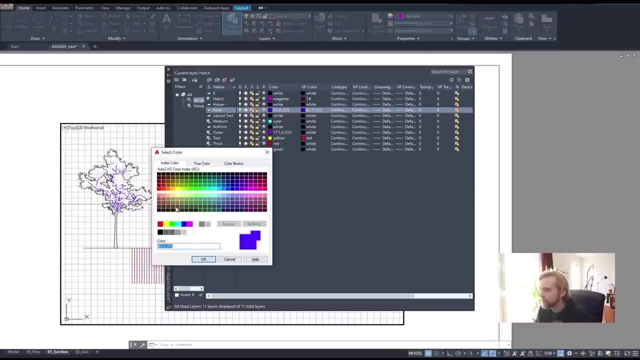 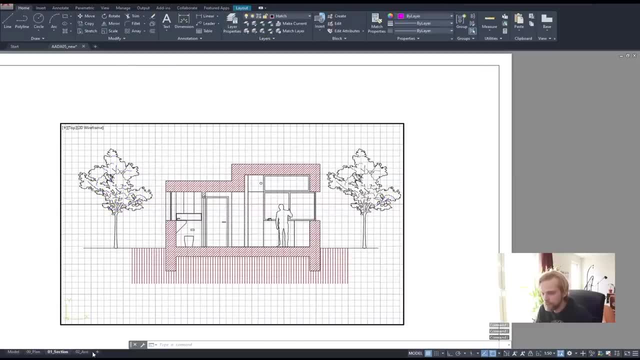 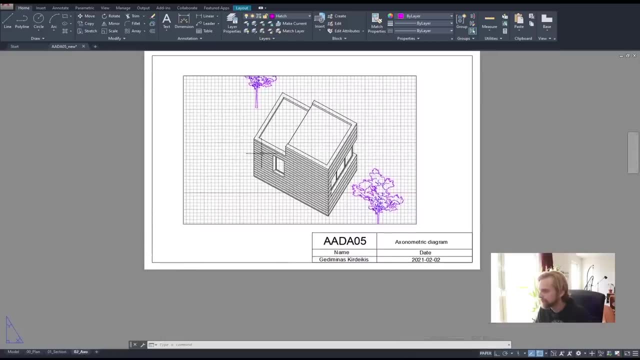 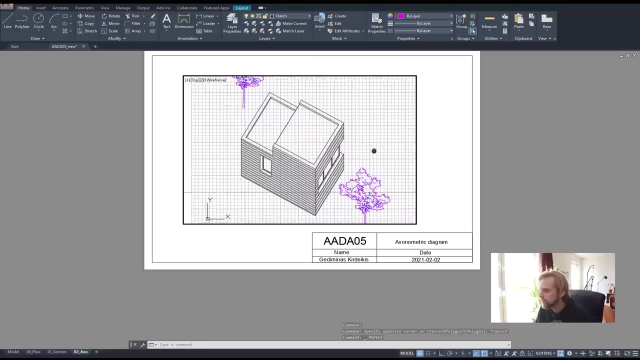 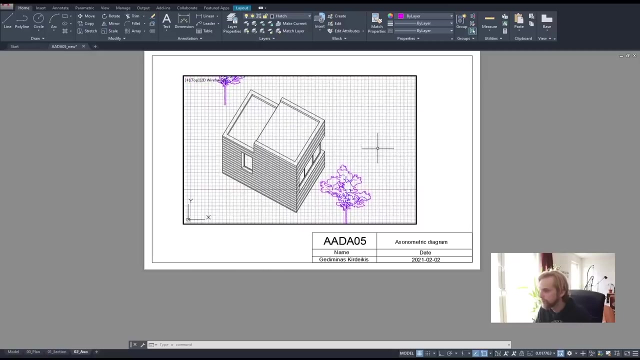 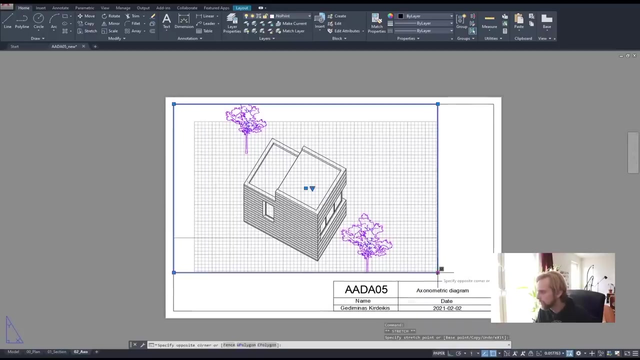 inner layer color to be medium gray, hit. ok, close, that's good. same thing for axo. oh, for axo we actually need. maybe we'll need to have a smaller axo. that's fine, i will just double click and scale out super vertical, though. click here and we make this bigger. let me just snap it to the, to the sides here, like that. 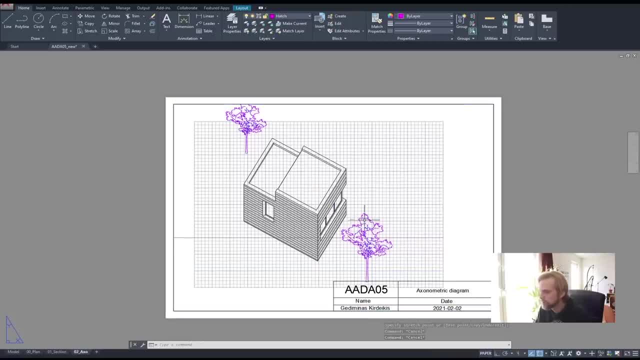 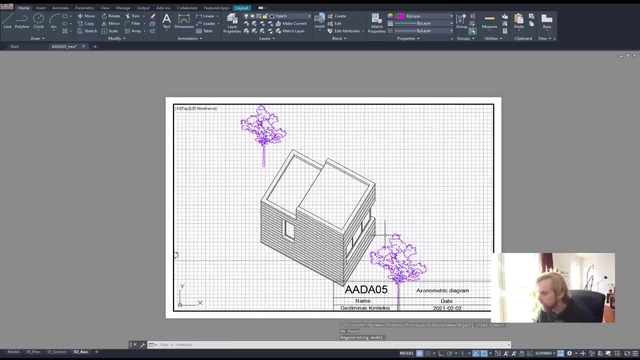 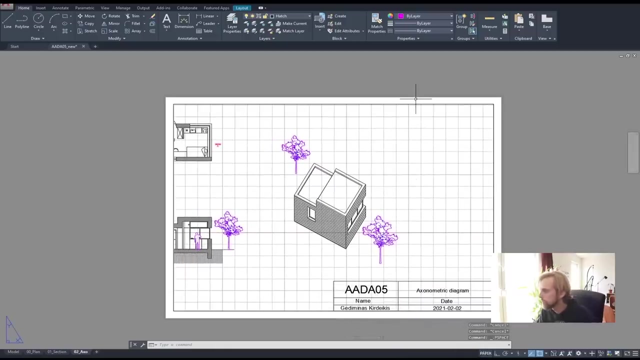 that is almost good enough, but i kind of want to move this tree up because i am dealing with the horizontal orientation of this. so i will go. or rather we can kind of select all of this z enter o enter zoom objects. we can't. maybe we can do it other way around if i just go to properties. 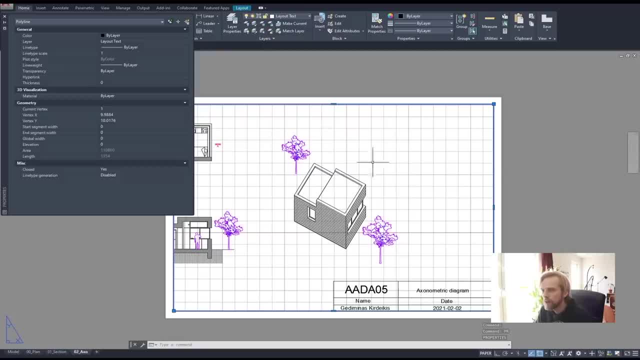 in the properties window. i'm going to go to properties, and here that's the, here the properties of the. what the hell? that's the pol line? oh, that's the frame, that's the frame. i don't want to select the frame, though, so how do we do this? we can select both of them and then from 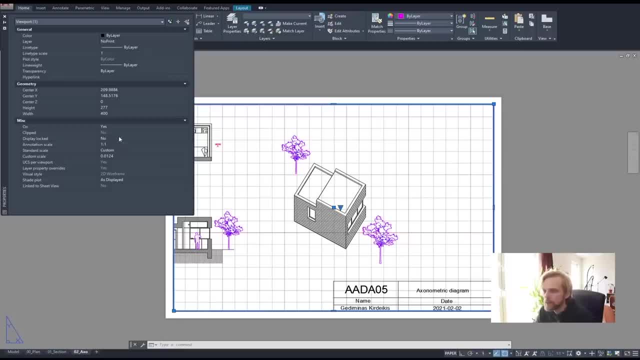 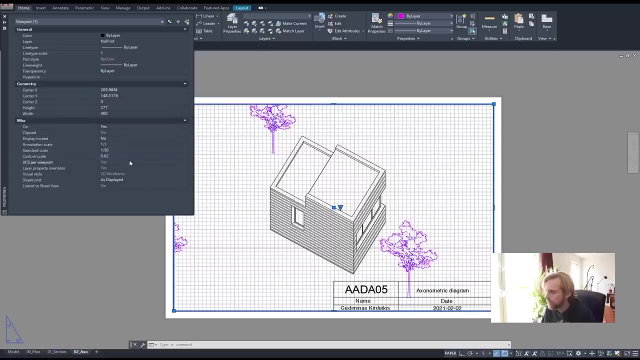 both of them. i will just choose viewport um, and here i will just change the, the scale. Let's use custom. and if I make this number larger, the scale should increase. So 0.02, looks like that. Let's do 0.017 or something like that. 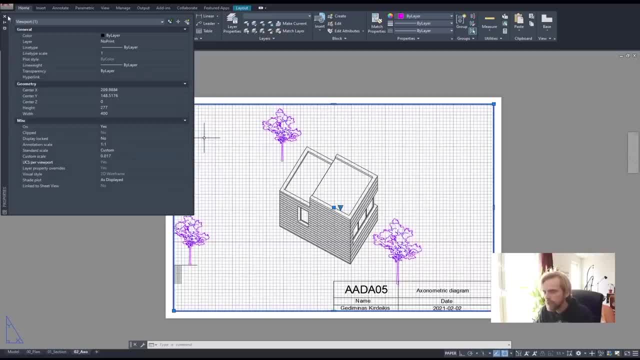 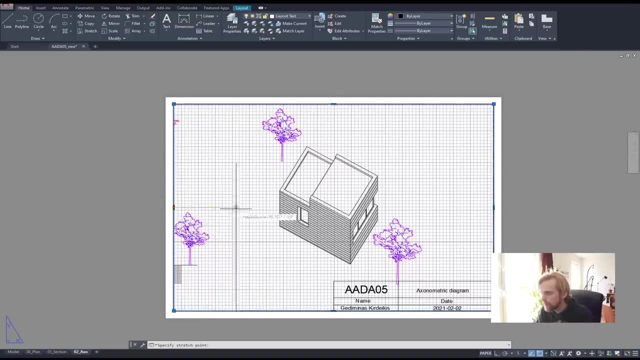 Whoops, 0.017.. There we go, that's fine. We can now clip around here like so. Well, that was the incorrect line. That is fine. Kind of still work with this. Move this in, like so. 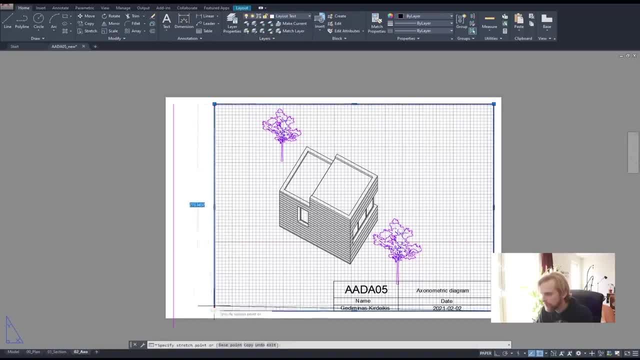 Grab the line. set Segment here, Snap it. No, we can't snap it. Grab that one then and snap it Now. it's fine. Okay, so it was just a little bit of cleaning up. There's nothing special about what I've done. 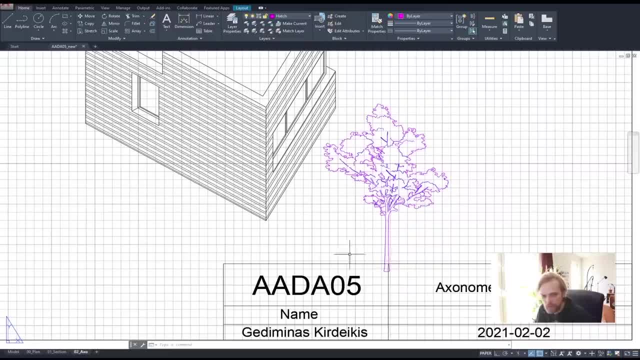 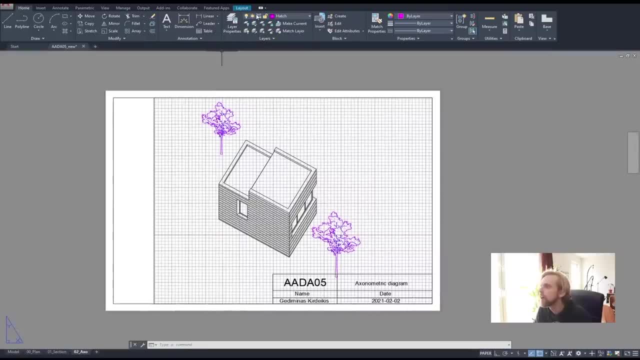 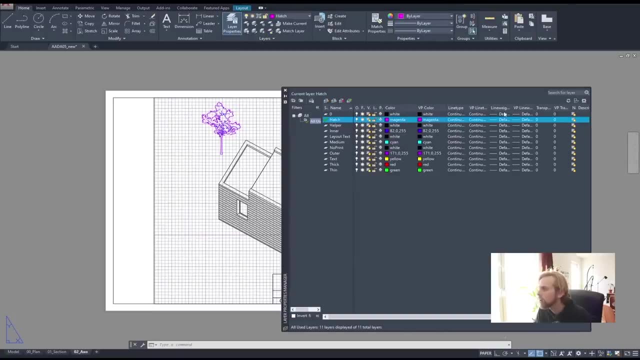 There is a little bit of a tree that's kind of sticking into the stamp, but that's fine. That's okay if it's doing that. Layer properties. Let me change the colors, Not for the hatch. Wait, Why is? 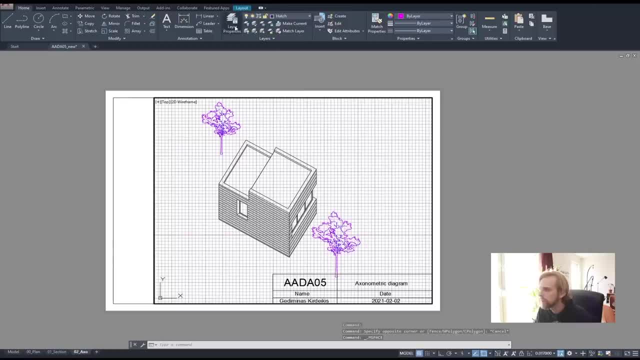 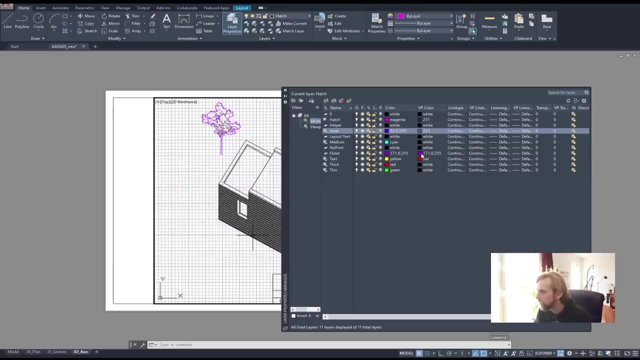 Oh right, right, right, right right. I need to double click inside and then change the layer properties to inner line being medium gray and the outer line being black, Or it says white but it's black. Okay, we're done. 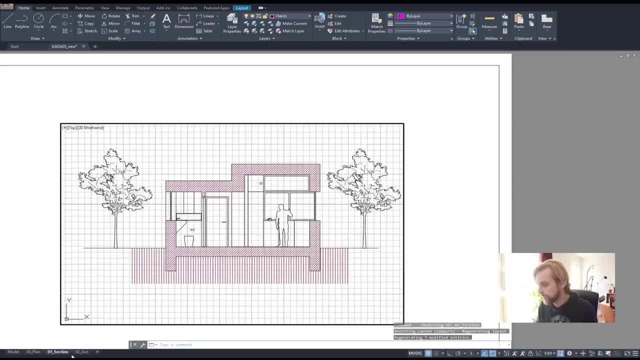 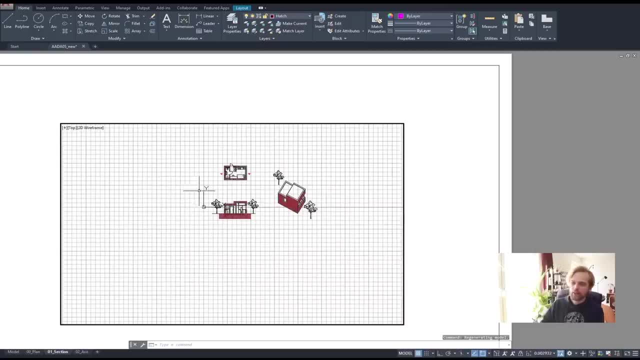 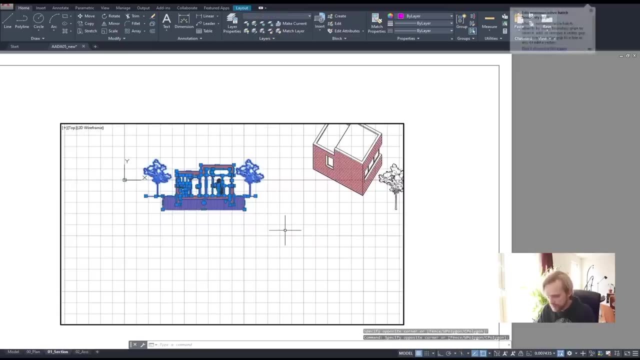 Good. So that's how you import stuff And apparently you can't trim. But that's good to know. Oh, I messed it up, So I accidentally zoomed out and now it's all messy. So I will need to kind of select all of this. 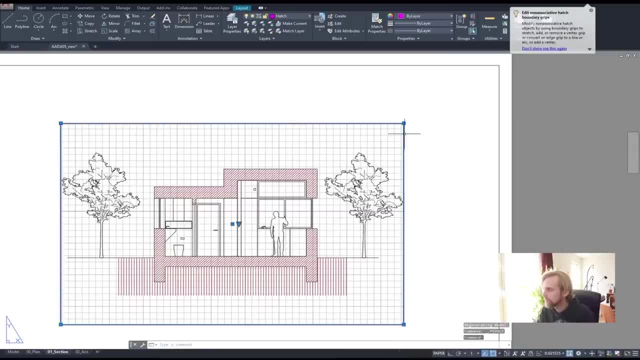 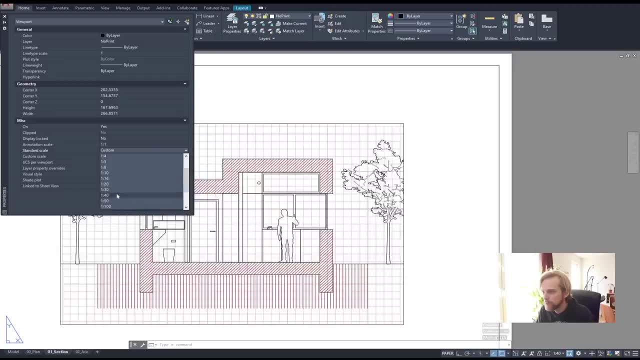 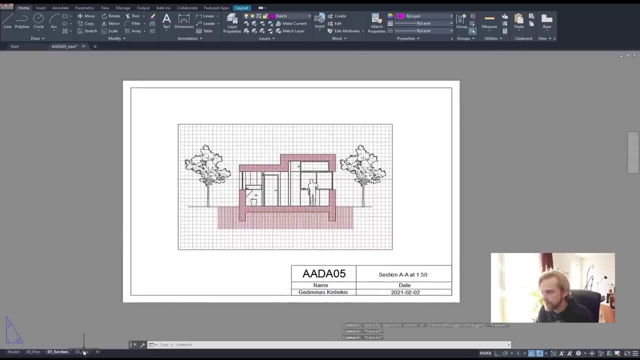 Zoom enter, oh, enter again. Double click out, Select the frame PR for properties And just make sure that the standard scale is set to 1 to 50.. There we go. So every time when you accidentally zoom out, you need to do this. 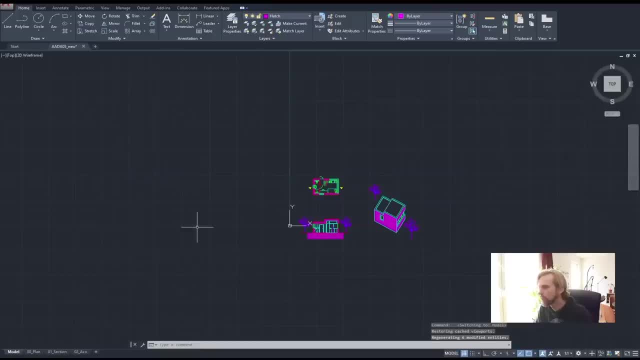 Axle is fine, Section is fine, Plan is fine. Okay, Model space: We have imported stuff. We have that, that, that Let's add grid lines, Let's add dashed lines And let's add measurements. Right, 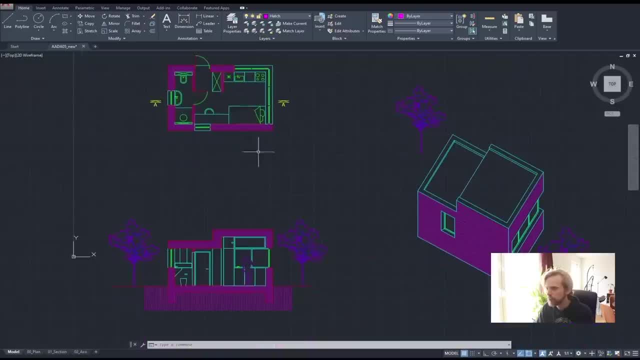 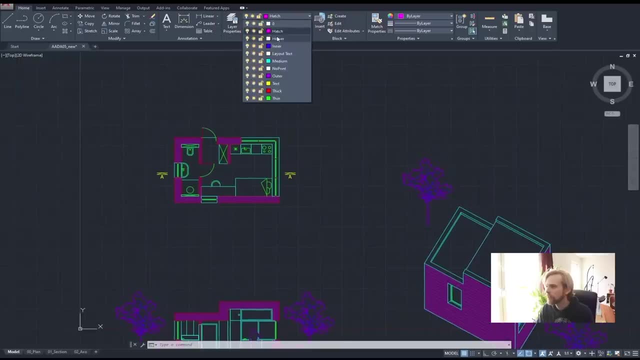 So the first thing that I'm going to do is I will add grid lines to both the plan and the section, And the way you do it is Well. first I'll just work with the helper line and I'll just draw them out. 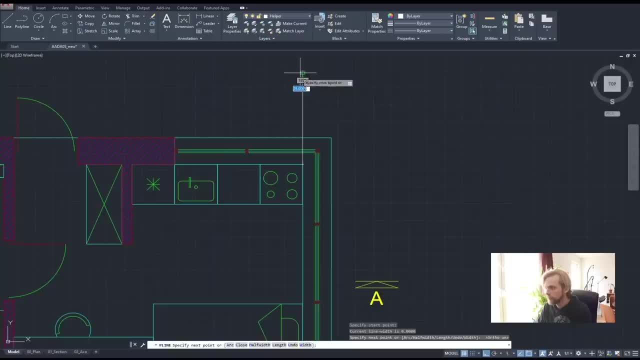 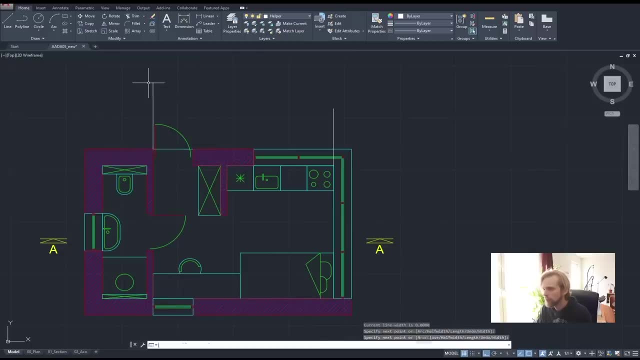 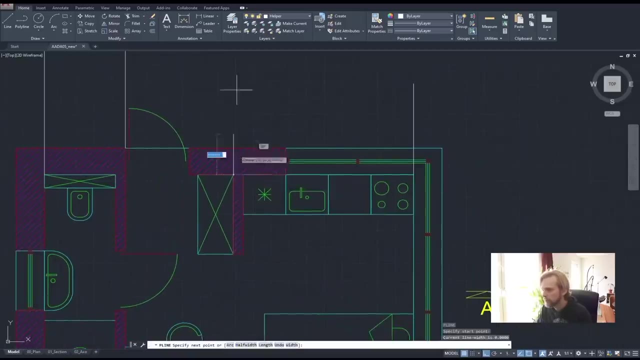 So the grid lines are usually anchored to the inner walls, inner side of the walls. So that's going to be one grid line, That is going to be another one, That is going to be the third one, Right here Probably. here is going to be the fourth one. 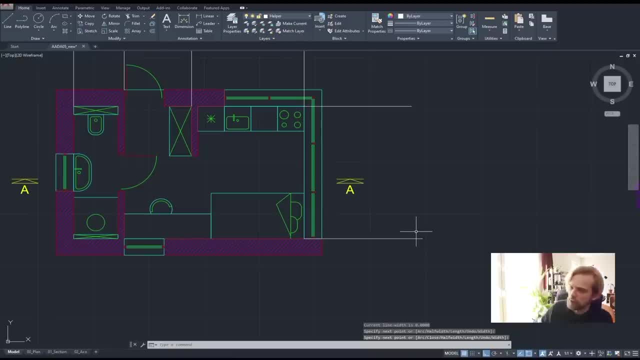 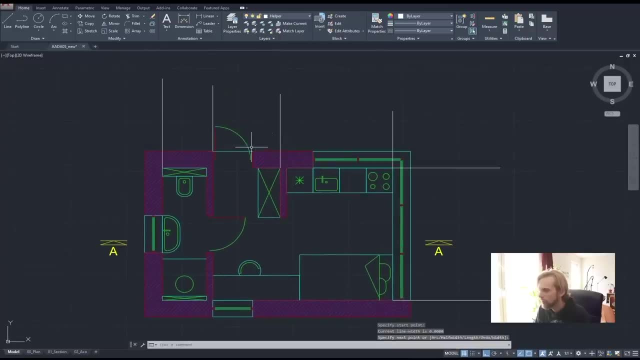 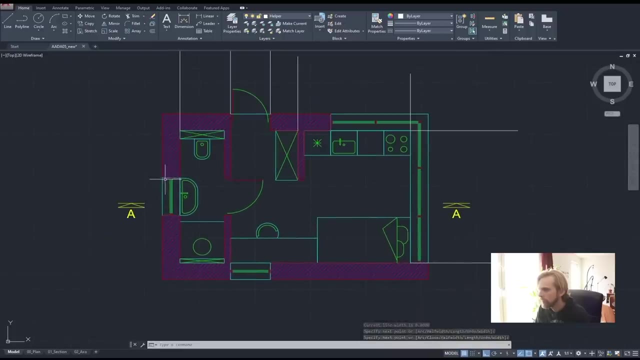 Fifth one, Sixth one: These are used for constructions. These are used for construction purposes and they are quite useful for that. Honestly, I'm thinking of adding a grid line here as well. I really want to add a grid line for this, but maybe that's not necessary. 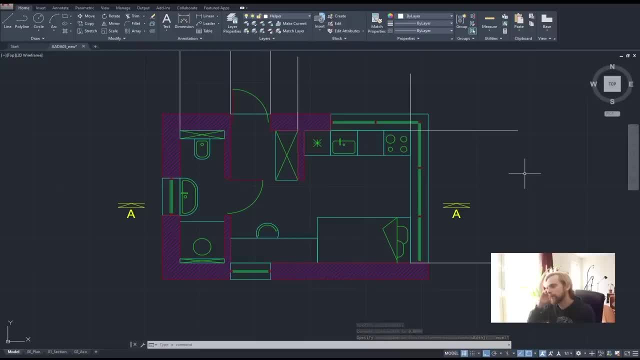 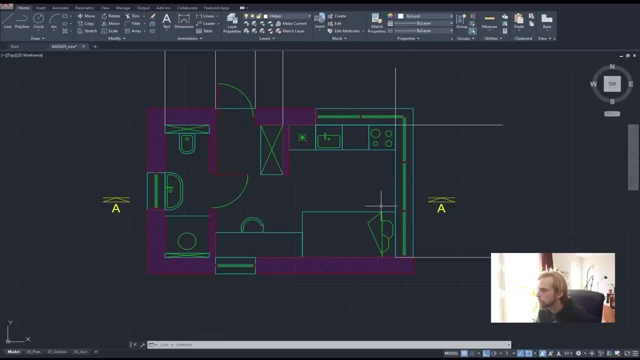 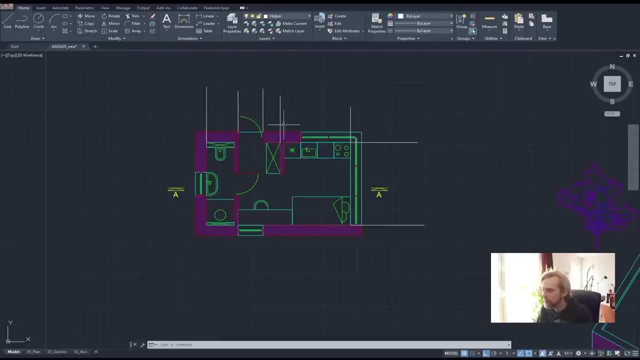 Maybe, Hmm, Sorry, I'm just thinking Real quick. I'm just thinking how much we should add. Let's stick to these grid lines for this particular example. Then I'm going to create a rectangle And my rectangle is going to be like so: 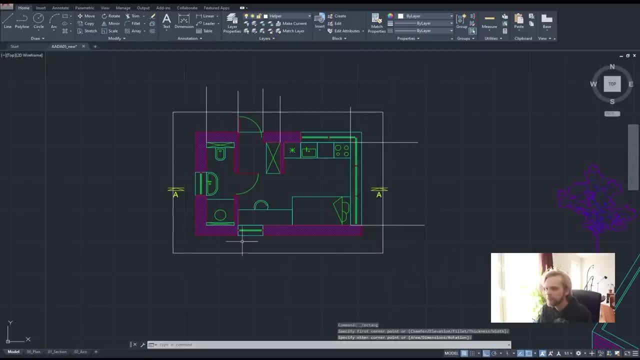 So I'm just kind of drawing around the building Right And I'm going to extend, So I'll select the rectangle, I'll extend these lines to that rectangle so that they penetrate through the building completely, like that. And also I will trim the lines that are extending away from the rectangle, like that. 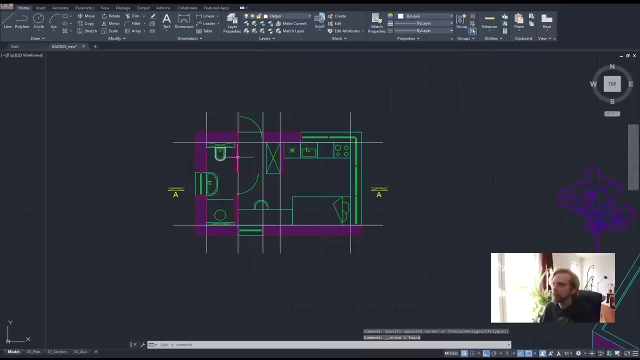 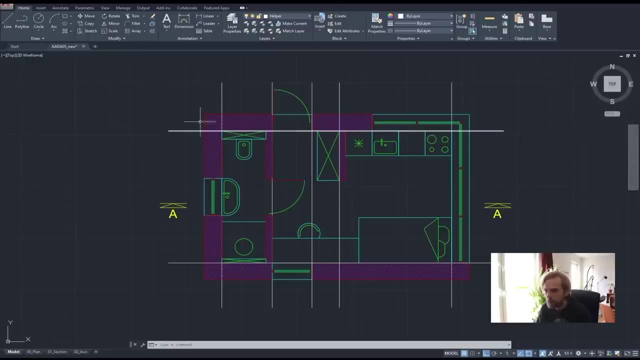 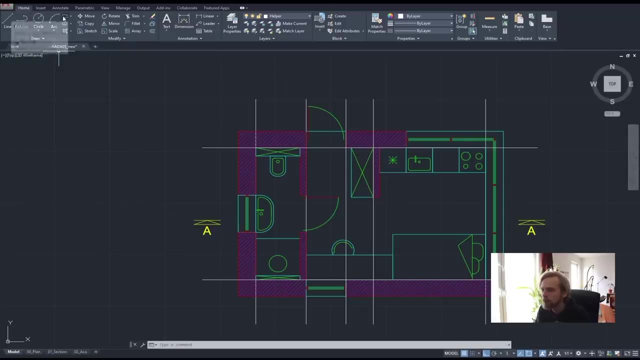 Once I've done that, I just can delete the rectangle altogether. So that's my grid lines, And they will have some sort of a markup at the end where I can kind of say what kind of grid lines I'm using. So I will just use a- let's just do a polyline. 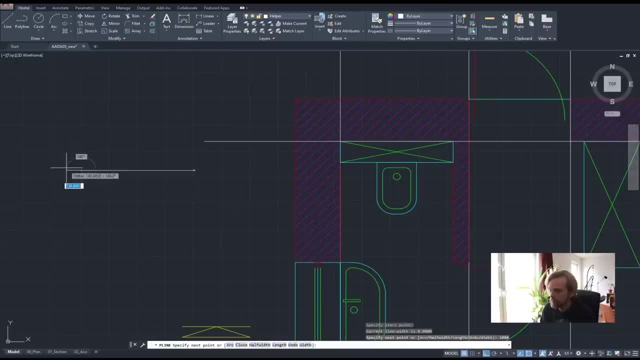 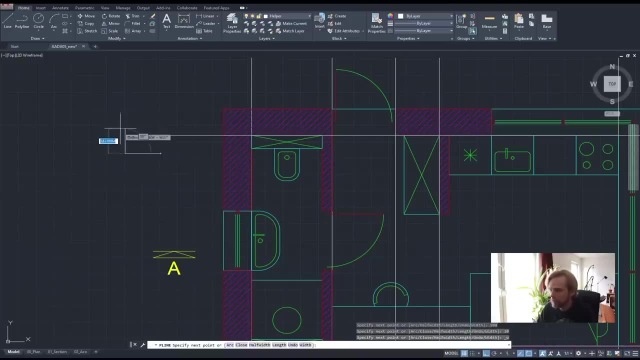 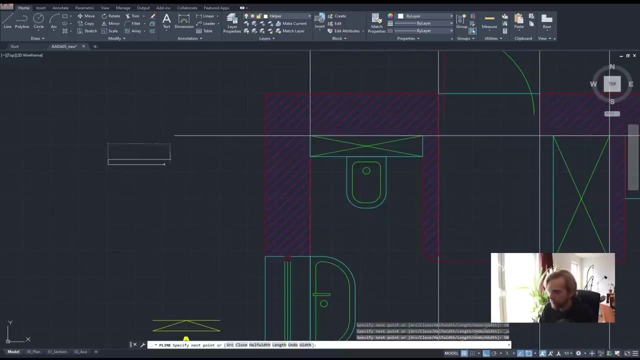 And let's just say the length is a meter. No, a meter is too much. 500 millimeters by 10 is too little. 50. Sure, 500 by 50. It's kind of a stylized ending for the grid line. 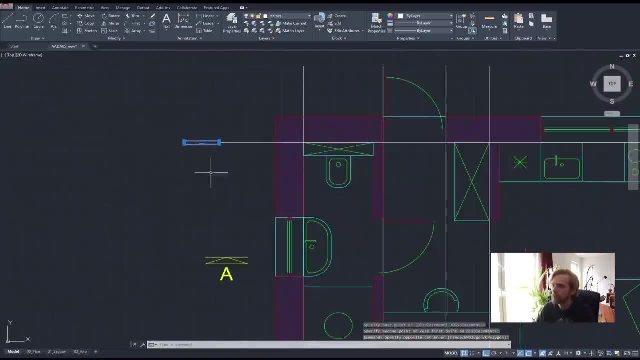 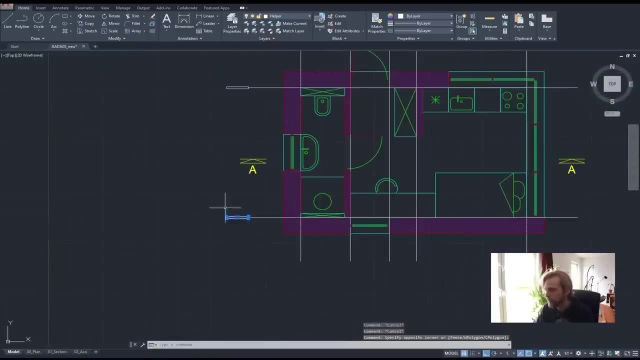 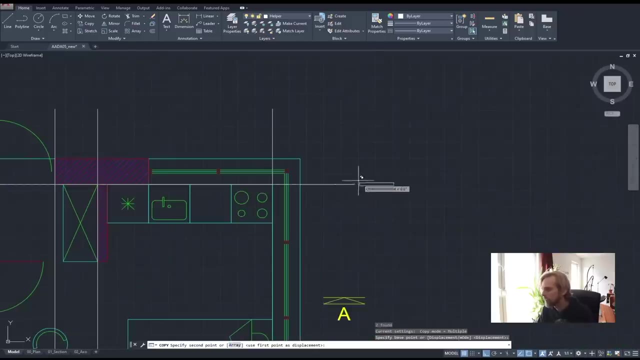 And from this midpoint I will just kind of move it to the first grid line here And I'll kind of copy it to all other positions, Like that: Take both of these, Copy them to the other side, Like so. And same thing for the verticals. 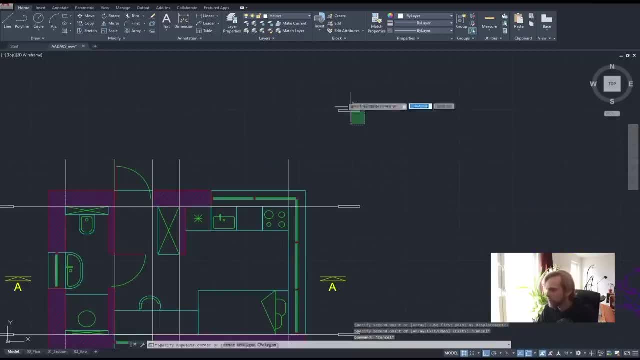 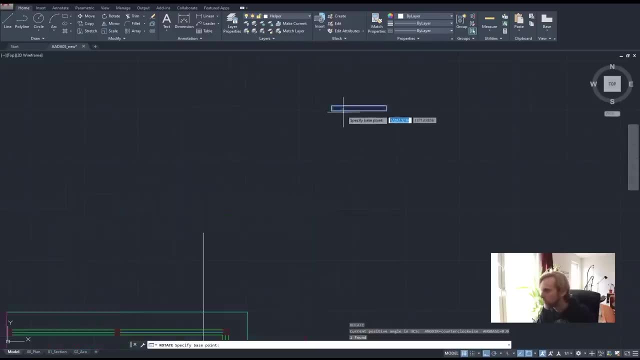 I'll just borrow this Like, so I will rotate it Or not Rotate Around this point. Vertical, There we go. Move to the first one, From midpoint to endpoint. here, Copy, Copy, Enter, And there we go. 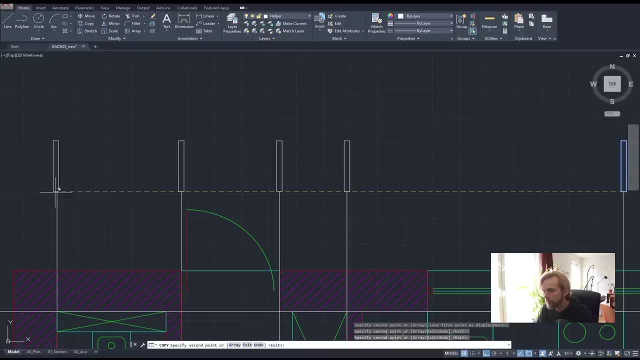 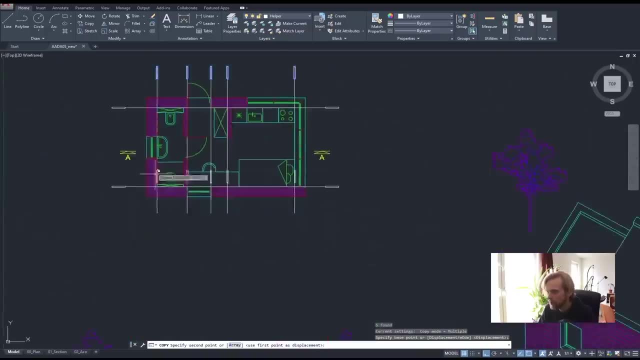 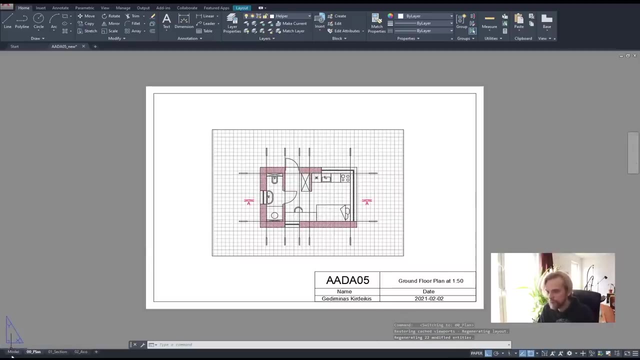 We just kind of go to town With them, Like that Copy From the top midpoint to the bottom endpoint of the grid lines: Let's make sure that everything fits in the plan. Everything does fit in the plan, That's great. 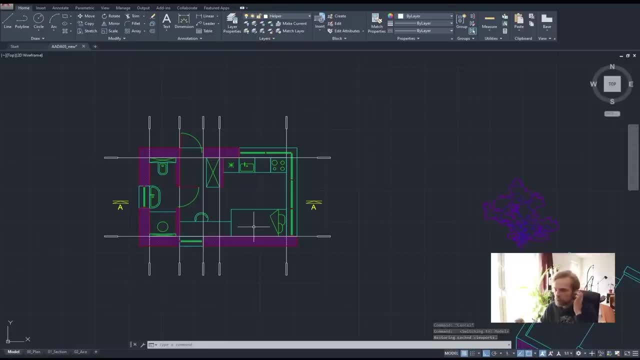 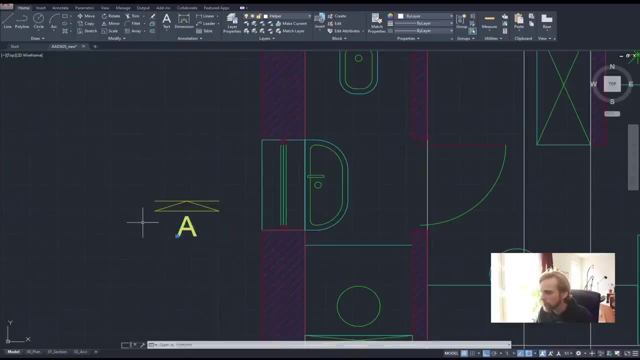 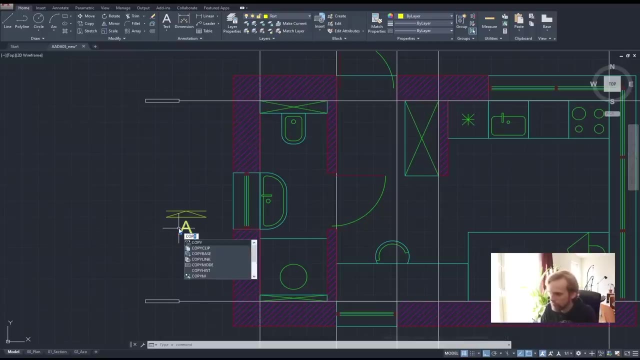 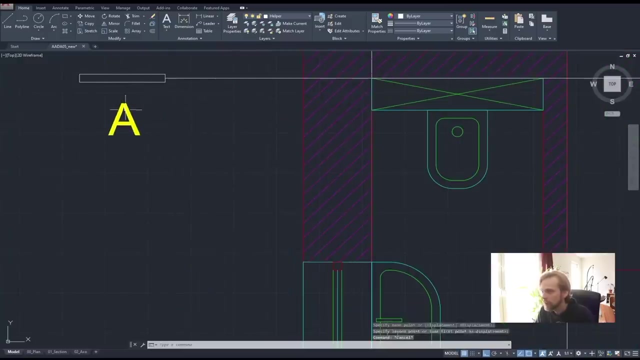 Let's go back here. So that's our grid lines. They do need markups, Basically naming for the grid lines, So I will borrow this text. I'll just copy it near the first horizontal grid line, Something like: so Let's go for below it. 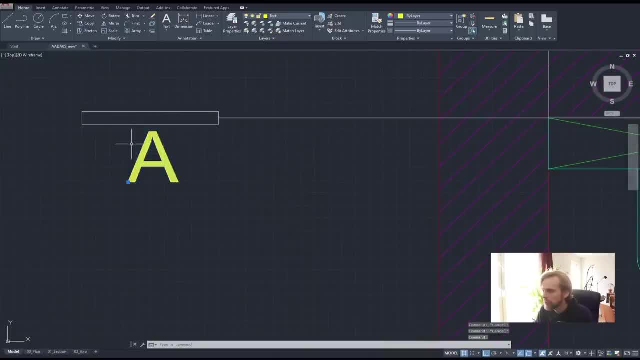 Right, And actually the text here can be smaller, So I'll just scale it. Scale it down by 0.5.. To a pretty small text. Let's just double check how it looks, So I'll just scale it. Scale it down by 0.5.. 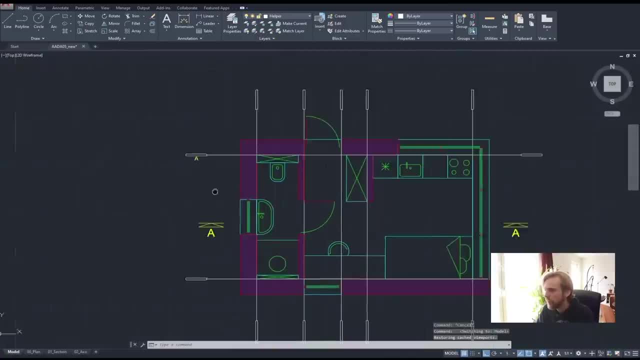 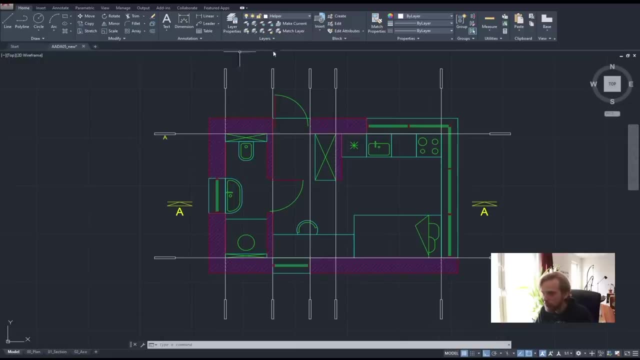 It looks like it's pretty small, But that's fine And it's basically going to be: horizontally I'm going to have grid line A and B And vertically I'm going to have 1,, 2,, 3,, 4, 5.. 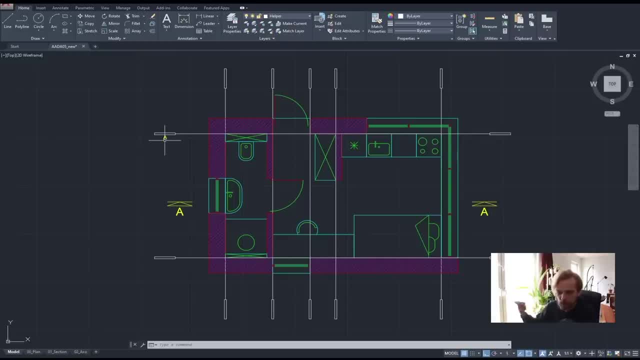 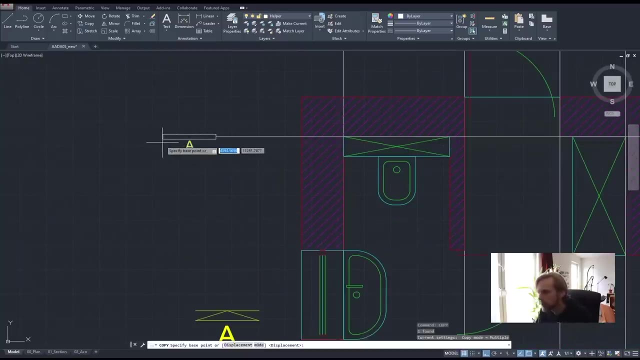 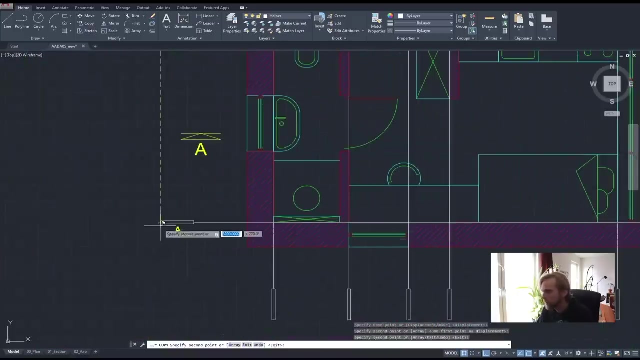 Right, So you always distinguish between directions by naming, And the naming is alphabetical in one direction And in the other one it's numbers. Usually use numbers for the direction which has more grid lines as well, So I'll just copy: A, A, A, A. 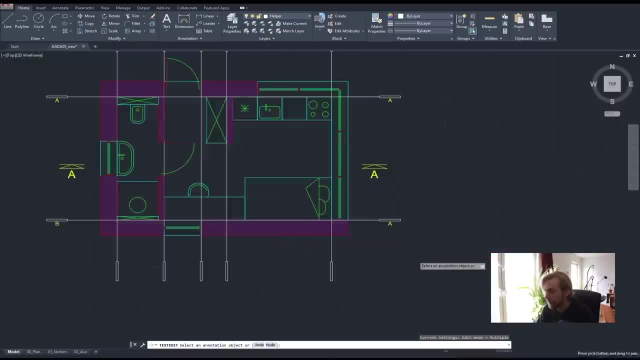 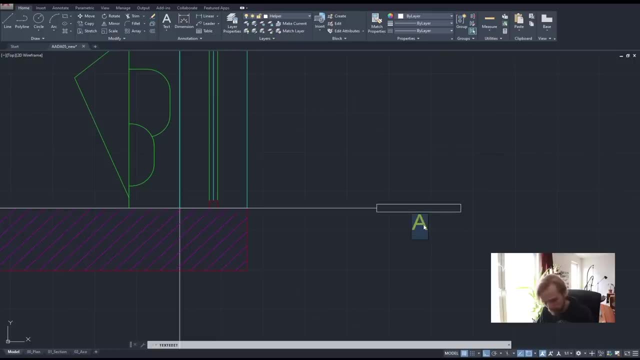 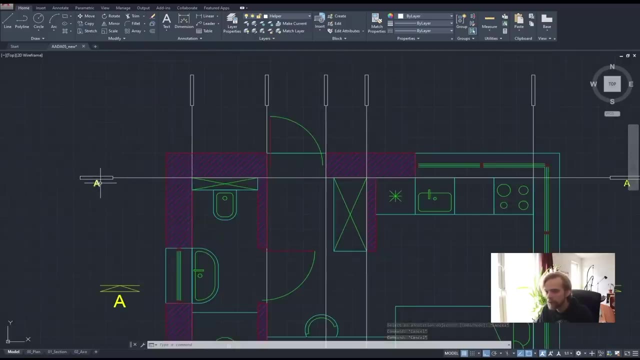 And this one I will just change to B. The XO doesn't need to have a grid line To have any grid lines Or any dimensions whatsoever. So A grid line, B grid line, That's great. Same thing for these guys right here. 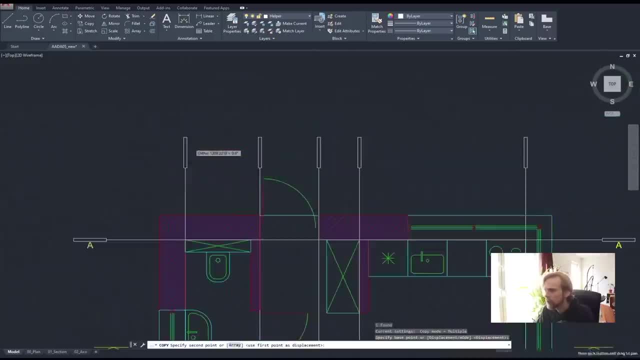 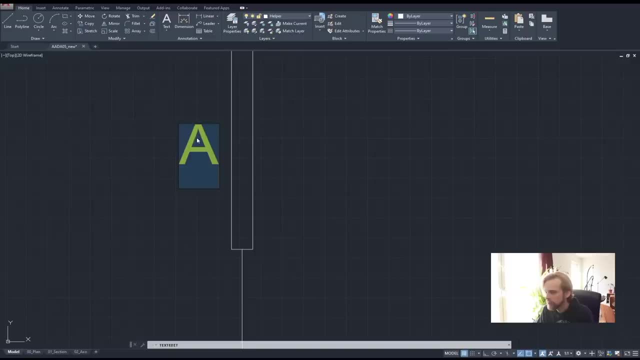 I'll just kind of Take this, Copy this Somewhere close by. It doesn't need to be perfectly precise, And I'll just rename this to 1.. I'll just kind of make a copy of it, So that's going to be 1.. 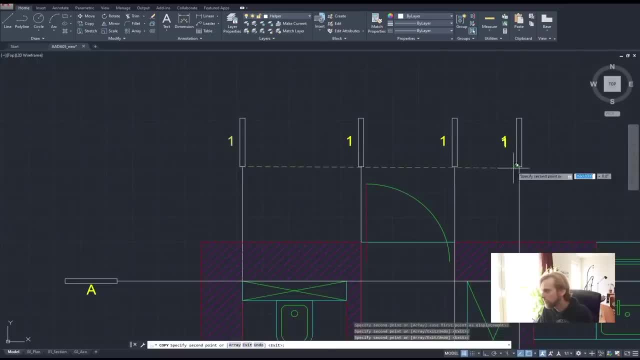 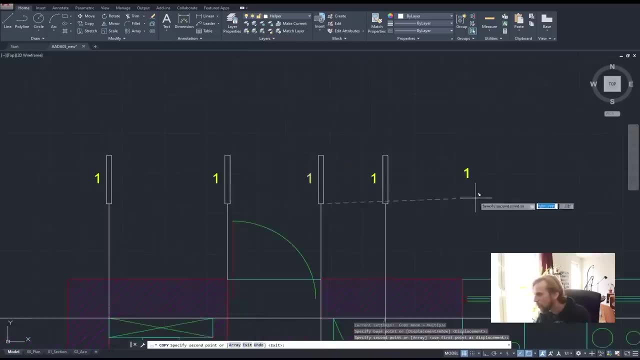 That's going to be 2., 3., 4.. Ah, messed up with the 4.. Copy 4 and 5.. Double click on the text. Rename it to 2.. Double click on the text. Rename it to 3.. 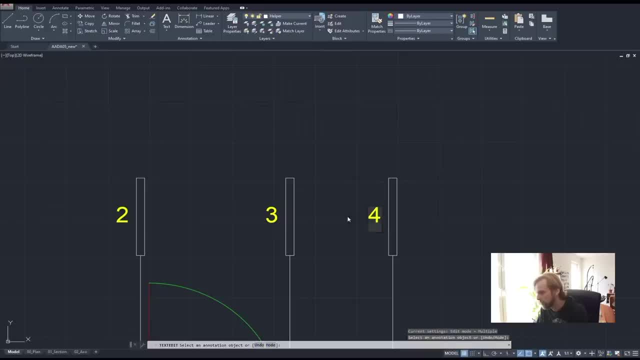 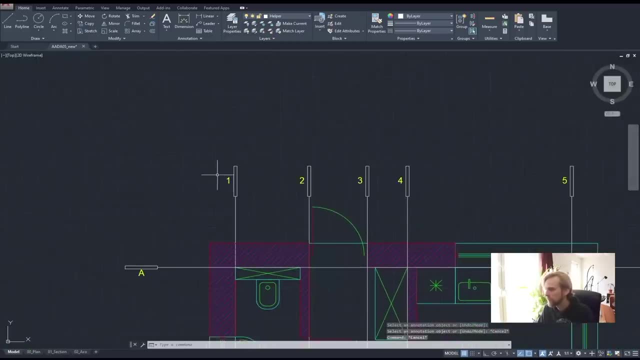 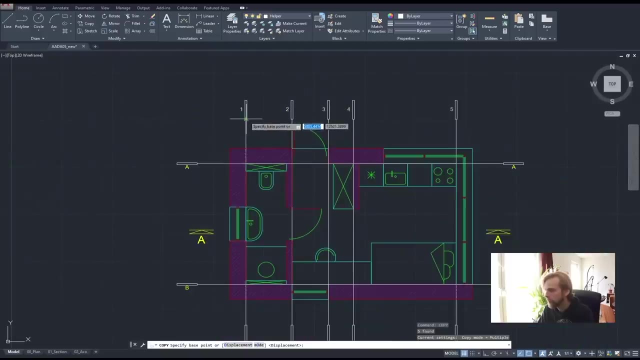 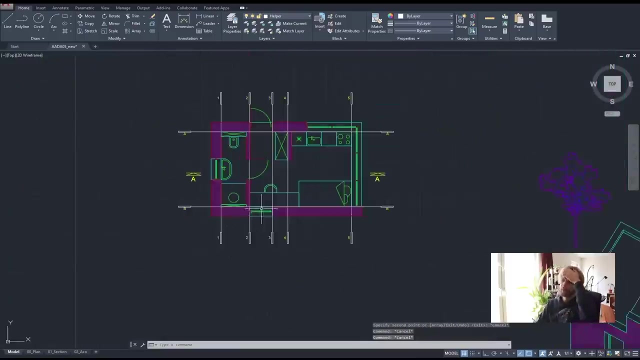 And the text 4.. And the text 5.. That's done. Now I just need to select these And copy them down. Copy, Copy From here to here. Okay, So we have our grid line markups done. 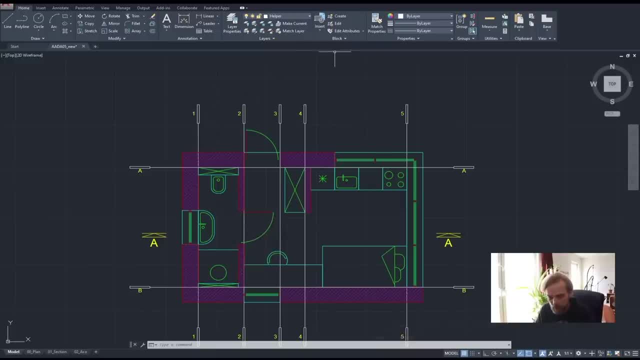 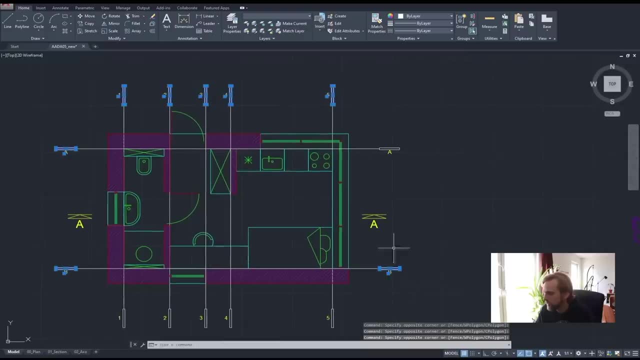 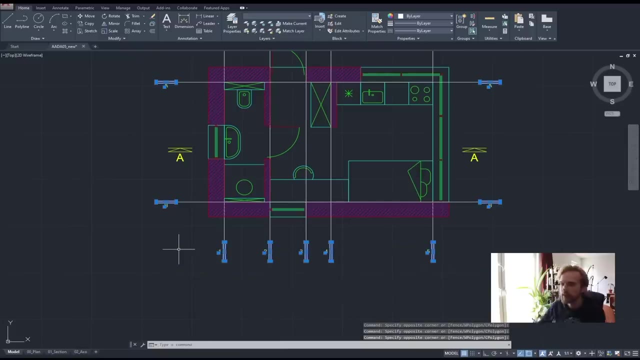 The grid lines themselves are still in the helper line layer, So I need to fix that. I will. Or axes: I guess we need to call them axes, Sorry. So we have grid lines and axes in this case, So I will select just the ends of them. 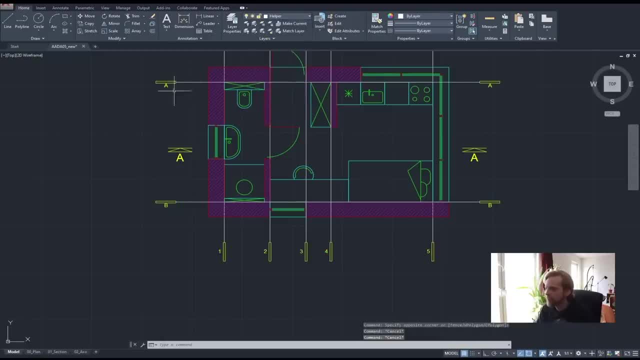 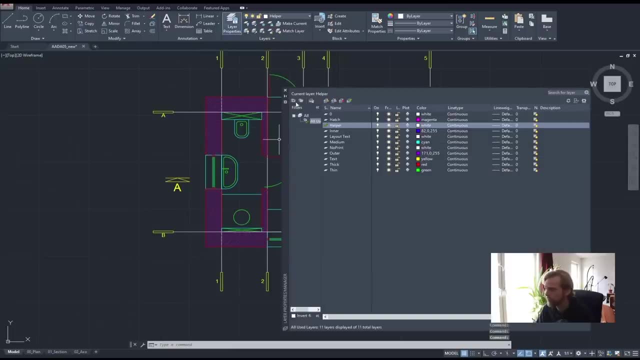 So I will select just the ends of them And I will change them to text layer So that the ends are going to be red And the axes themselves. I'm going to create a new layer for them. I'm going to create a new layer for them. 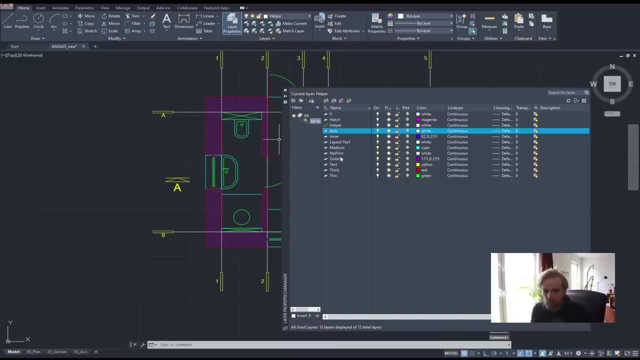 New layer And I'll call it axes Or axes, Doesn't matter, Axes. And I'll, here for now, just change the color of them to be also. And I'll, here for now, just change the color of them to be also. 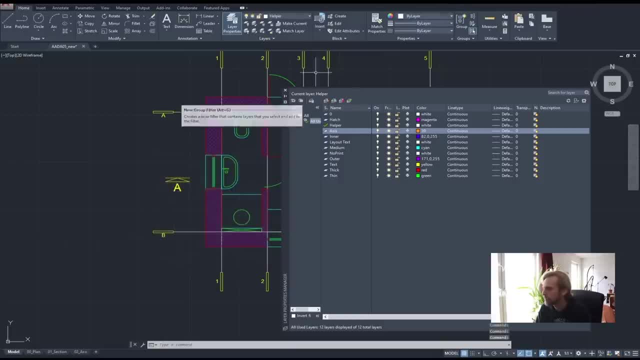 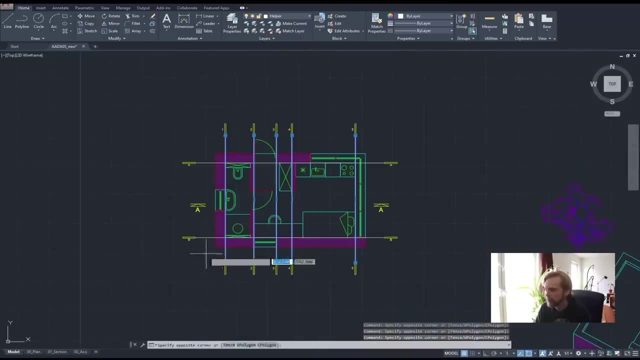 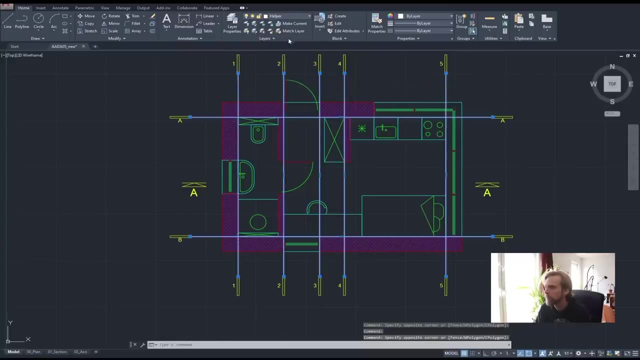 Maybe not yellow, Maybe let's do orange, Just to distinguish between them. So these are going to be done in orange. So these are going to be done in orange For now In the model space. I just select them. There we go. 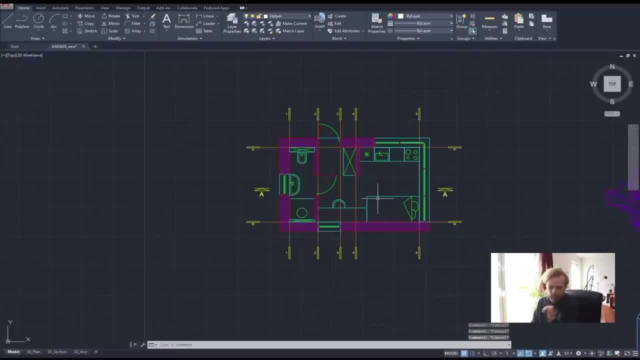 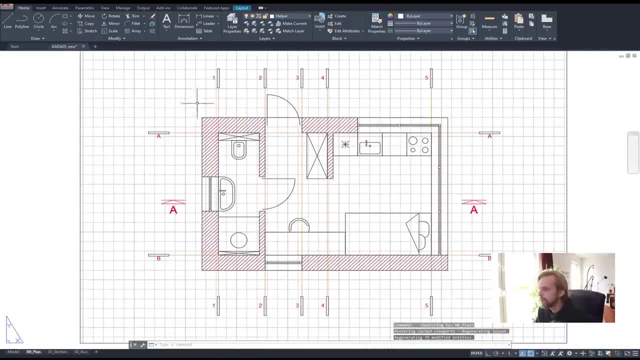 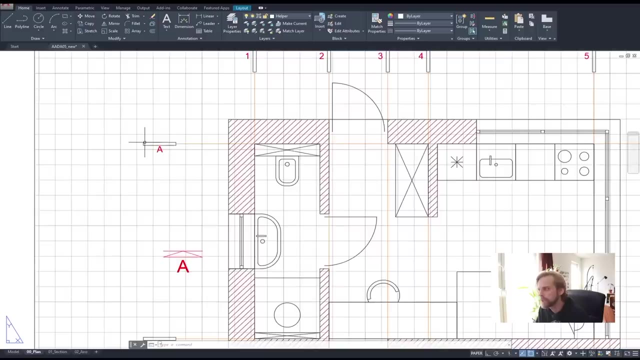 And we change this to axes layer. There we go. So that is done Almost, If I look at it in the plan Layout. Why is this? Why is this? That's strange. It should be red, right, It's in the model space, it's red. 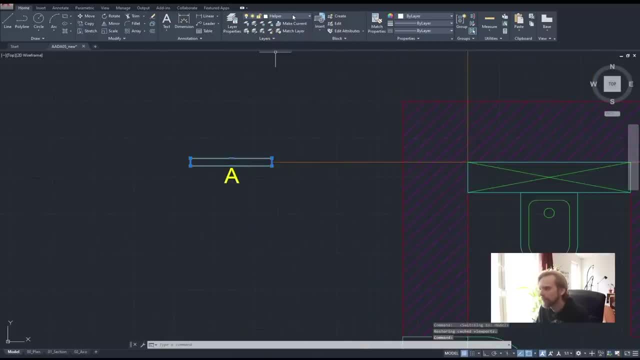 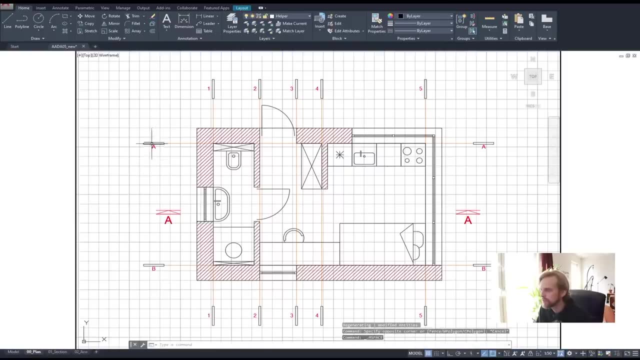 It's in the model space, it's red. It's in the model space, it's red. Sorry, The model space is in the green layer. Why is it here Still shown as black? Just give me a second. Just give me a second. 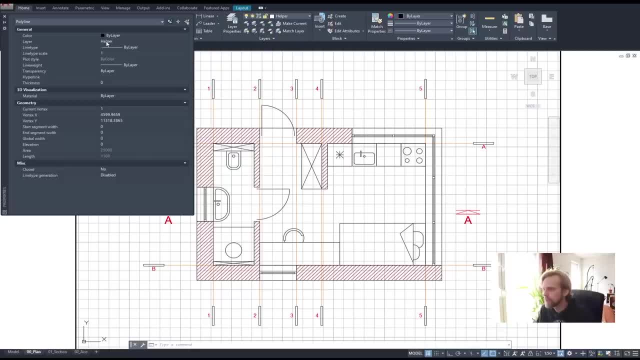 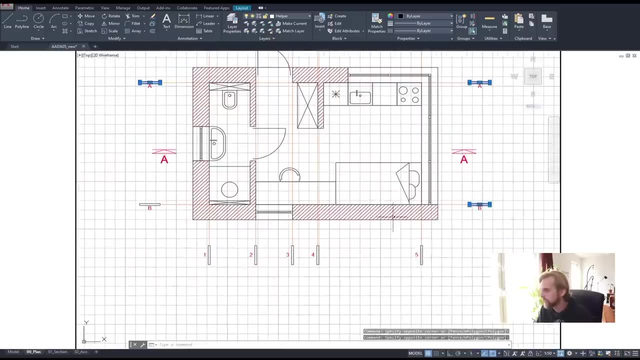 Layer helper So it doesn't update. What the hell? That is a bug. Again, That is super weird. Sure, we can change them here While we are in the model space, While we are in the model space In the layout. 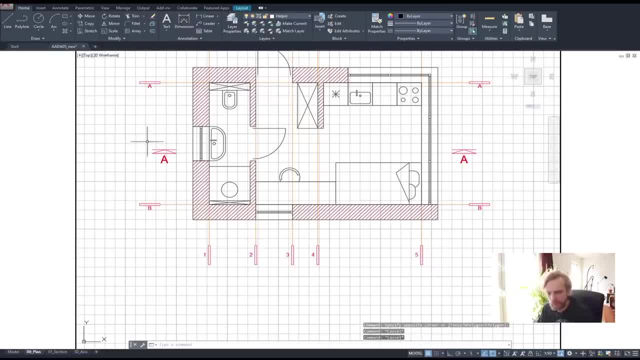 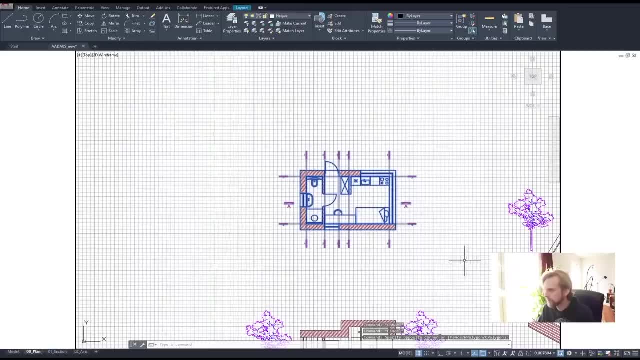 I can force them to be in the text layer. I can force them to be in the text layer. I don't know why that happens, And now I messed it up. I messed up the scale. That's fine. Zoom Enter. 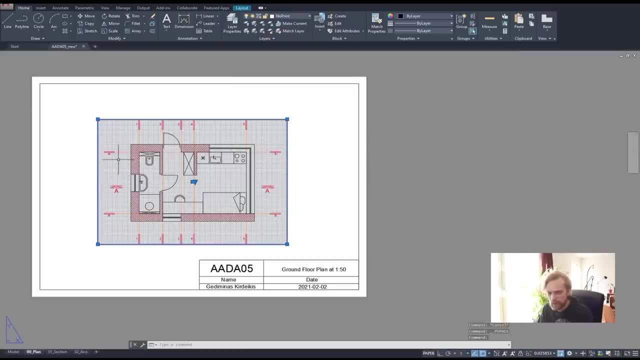 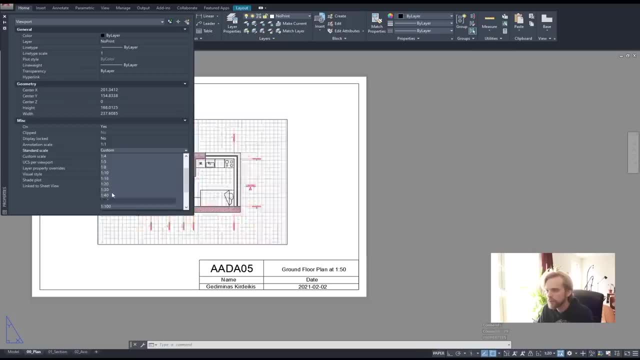 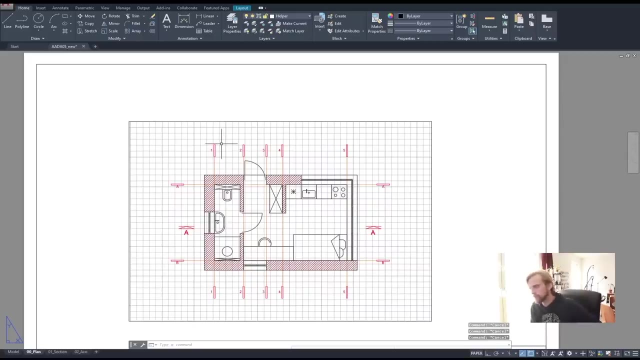 Z, Enter, O Enter. Zoom into it. Double click out, Select the frame properties And change the scale again to 1 to 50.. And change the scale again to 1 to 50. It's super strange that it isn't that reactive. 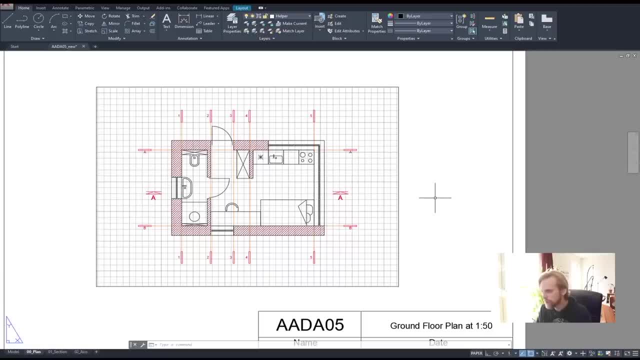 It didn't have these kind of bugs in previous versions. It didn't have these kind of bugs in previous versions. I assume you will not have these bugs if you are working with an older version. I assume you will not have these bugs if you are working with an older version. 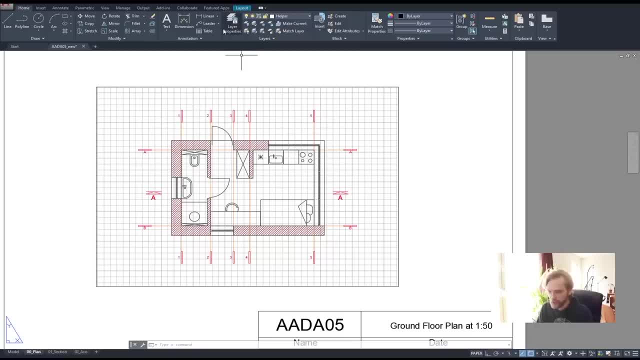 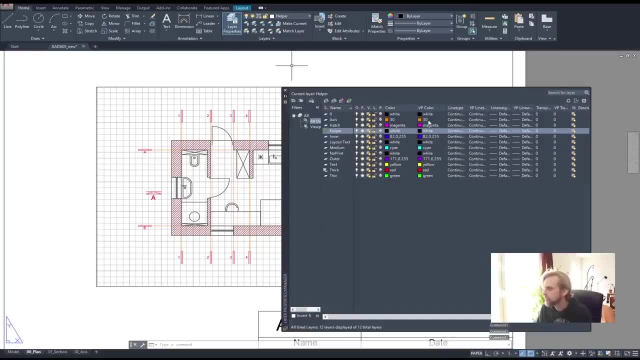 Anyway, The lines themselves. I want to change some properties of them, So I'll go to: Or the axis lines, I'll go to layer properties And here where I see axes, First of all I'll change the color of them. 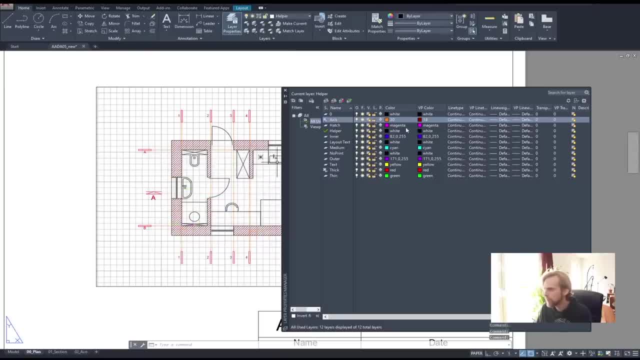 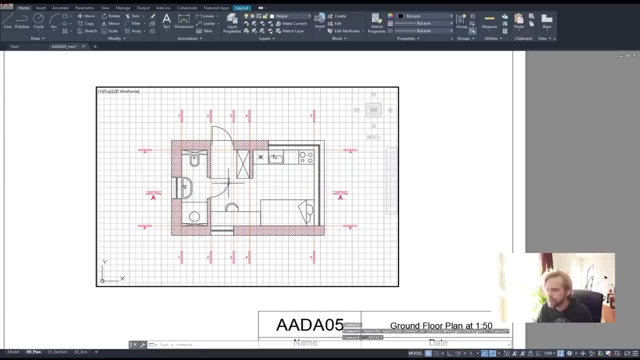 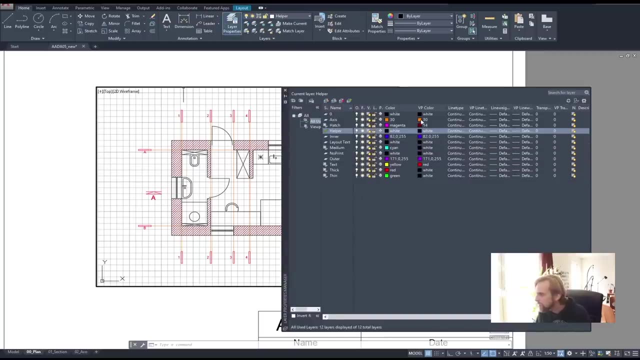 And I'll change the color to probably Dark red Color. Let's just hope that it kind of works. Oh, I need to be inside of the model space. I need to be inside of the model space Layer properties. Here we change the axis layer. 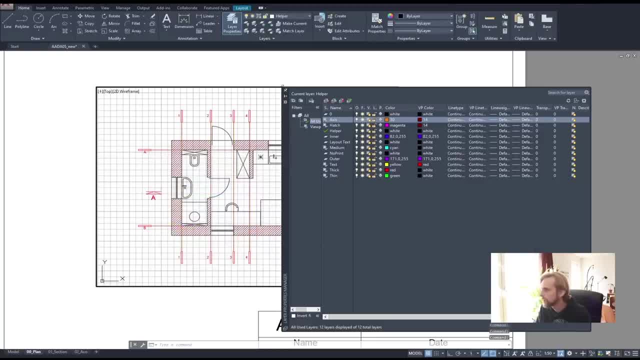 Color to dark red. Color to dark red. There we go. So that is done. But also, while I'm at it, I don't want this to be a solid line. I want this to be a dashed line, So I will mess around with the line type. 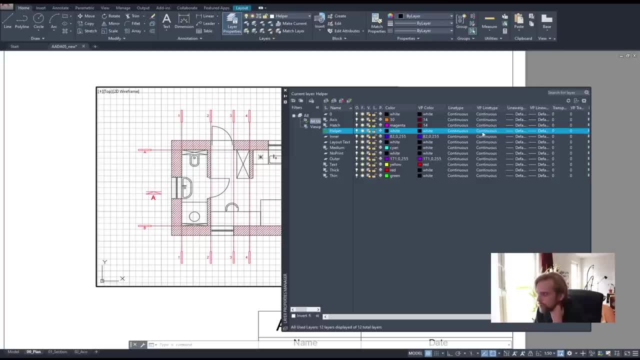 So I will mess around with the line type Right, The viewport Line type Right. So while I'm still here, Where I see VP line type, I'll click on this continuous Name. Wait, Am I in the helper? 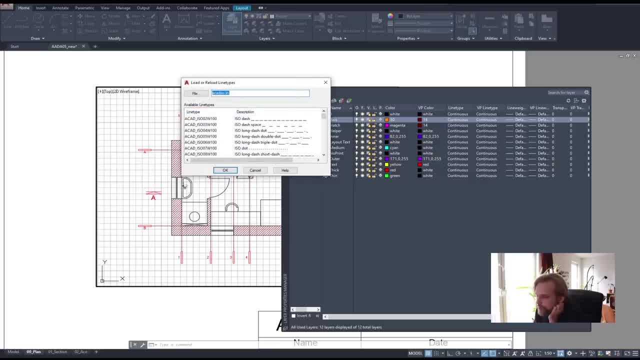 No, For the axis Continuous, And I'll load a line type that I want, And in this case, for these particular lines, I want it to be dashed Dash dot Right, So I'll just hit OK. So now it got imported. 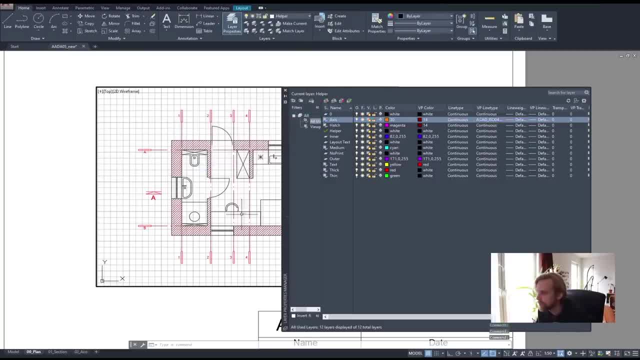 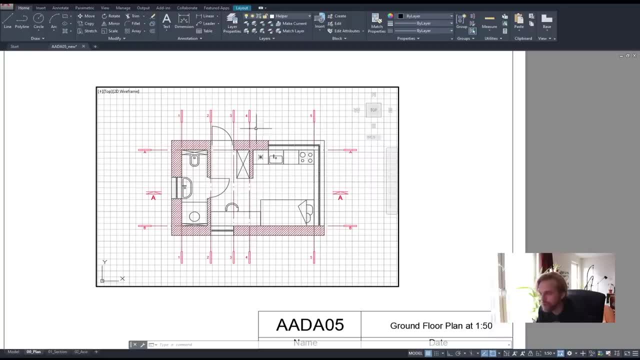 And we can use this line type, Right, And I'll just choose it And use OK, And now I can see that my line types Have been updated And now they are dash dotted. You can change the line type scale, But I wouldn't suggest doing it. 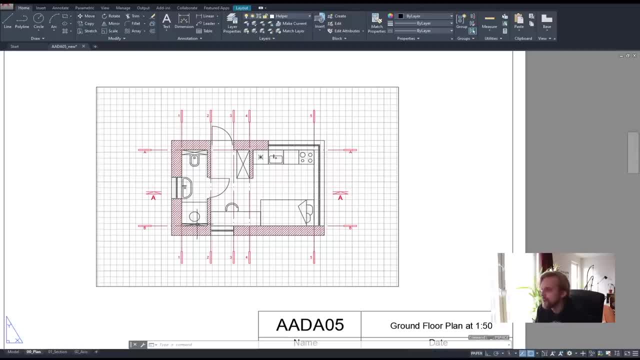 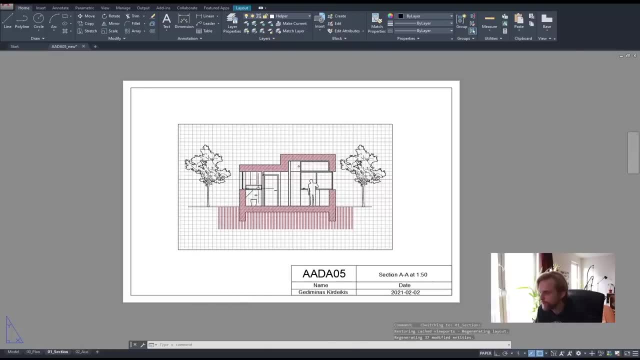 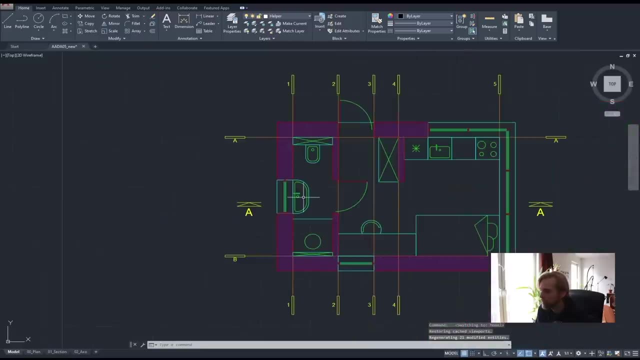 If it works OK. So we have this going. That's great. Let's jump into the section Right here, And we kind of need to add the grid lines To the section as well. So I'll go back to the model space. 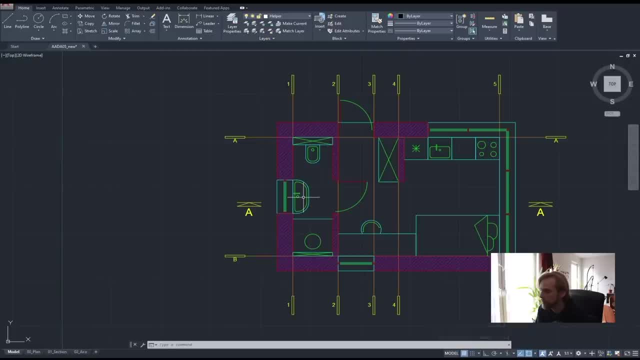 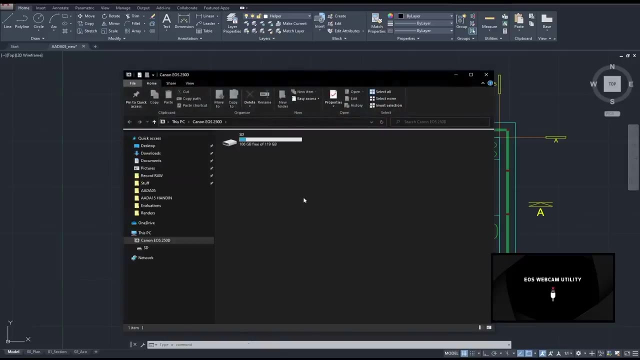 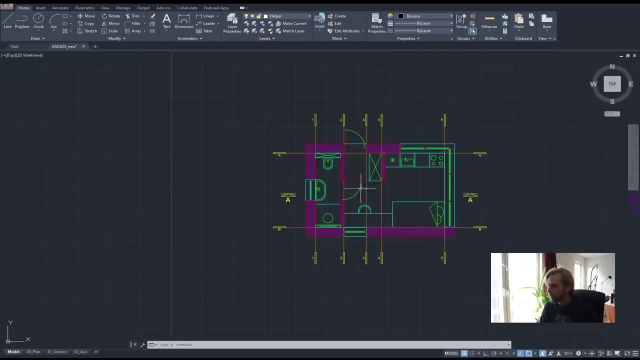 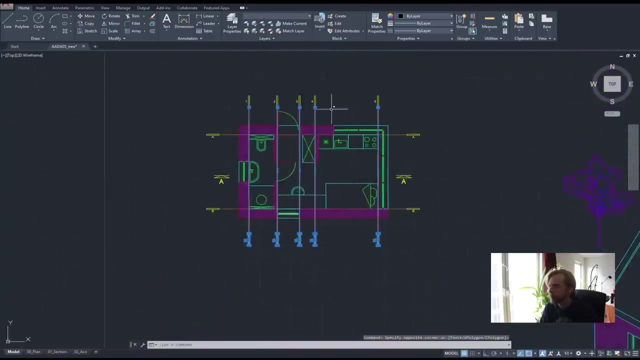 My battery ran out. This is a long tutorial. Just give me a second New battery, please. There we go, Should be good. Uh huh, So Section Right: The way you add grid lines to the section Once you have them in the plan. 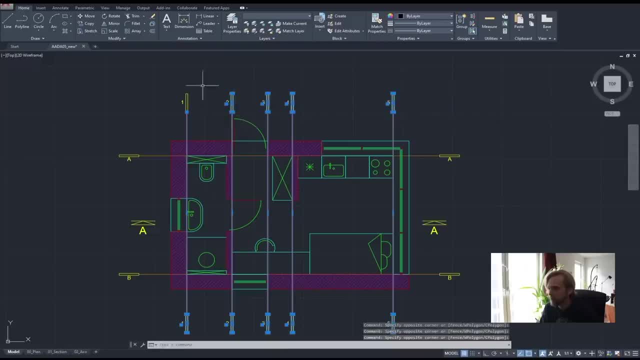 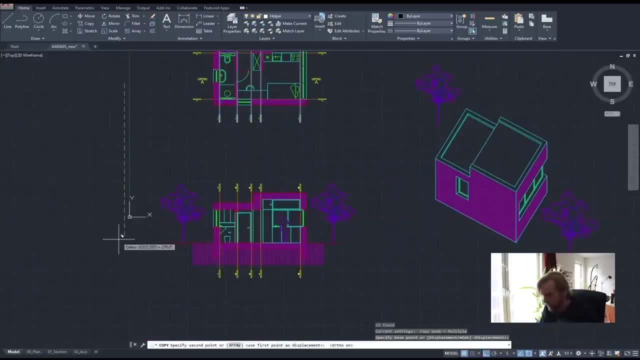 Is super simple. You just grab the ones that you already have made In the correct direction And you just copy them Down, Perfectly down, Like. so That's it, That's done. Because these perfectly align Right, You will not be seeing grid lines A and B. 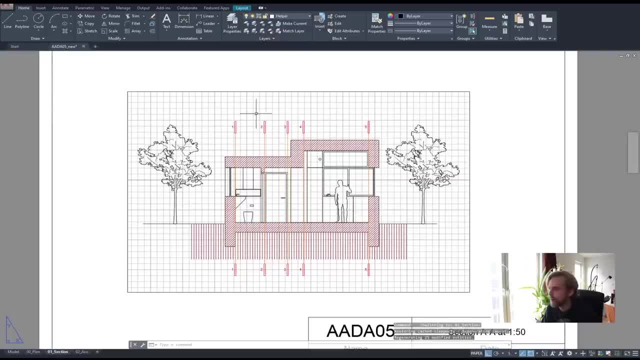 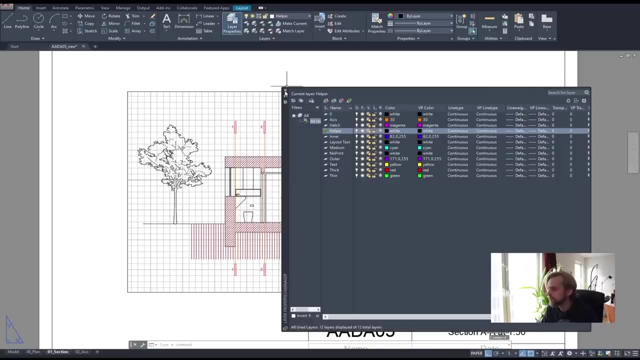 In the section Naturally. Then there's some change And here it actually updates, I don't know. So here we need to change The display as well Of these grid lines, So I'll go to layer properties, Double click. 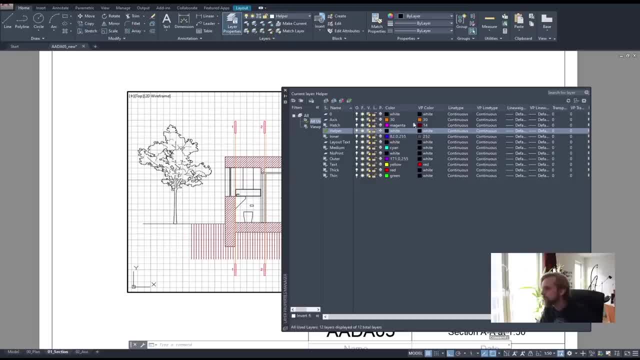 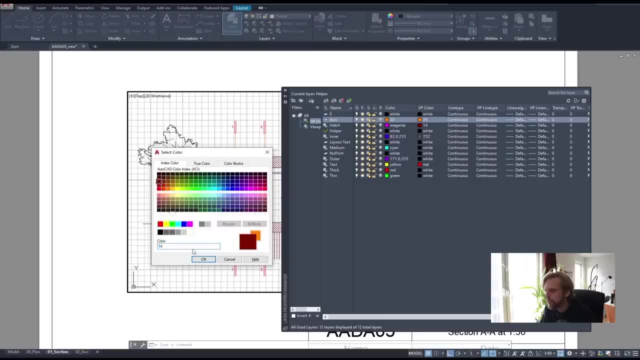 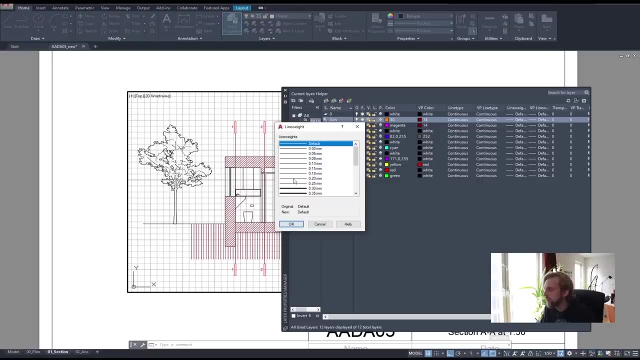 Layer properties Change from From the axis Color To be That dark red color that I wanted And the line weight Or line type: VP line type: I will change. Wait, There we go. VP line type: I will change to dashed. 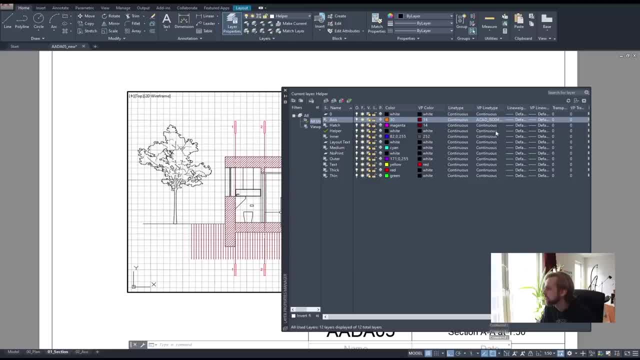 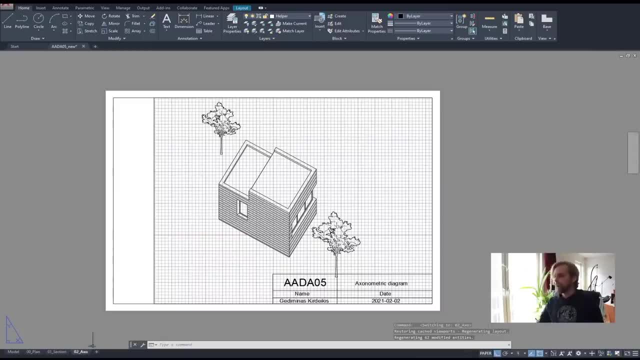 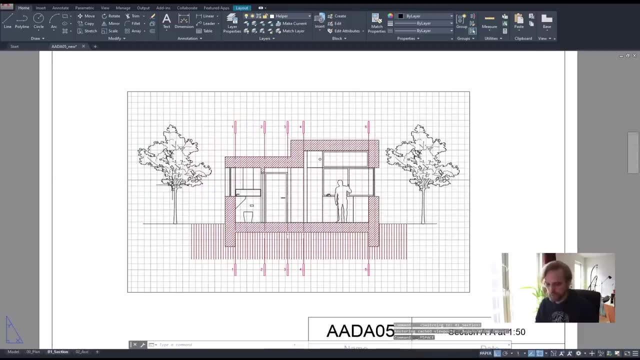 Okay, That is done. That is it Okay. Okay, So We don't need to do anything with this. This looks fine. This looks fine. Oh yeah, Double click out of it So that you don't accidentally zoom in. 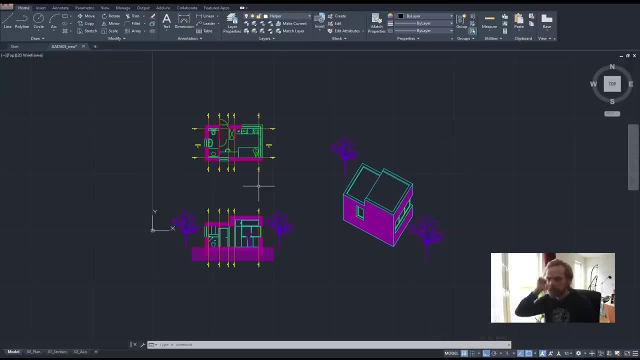 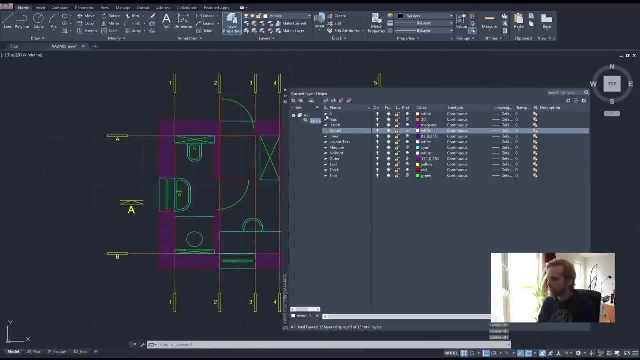 To the drawing Now. one last thing, Before we plot everything out, Is adding dimensions, And I'll start with the plan, As per usual, Dim. Just kinda Name it, dim For dimensions, And I will make it red In this case. 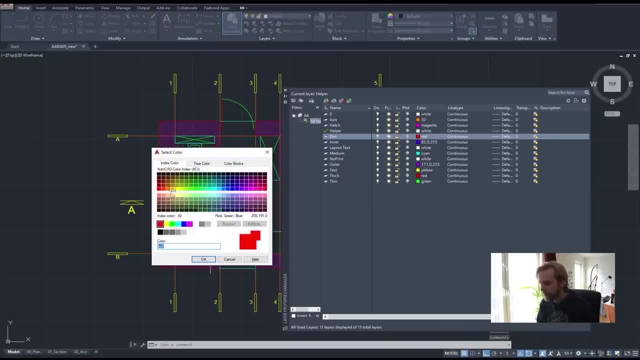 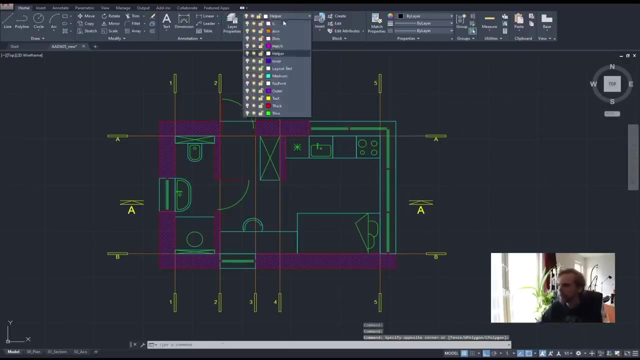 Or We are using red color, So let me make it Orange. We are using pink, We are running out of colors here. Let's just have white, then That's fine. That's fine, It should be done in white. 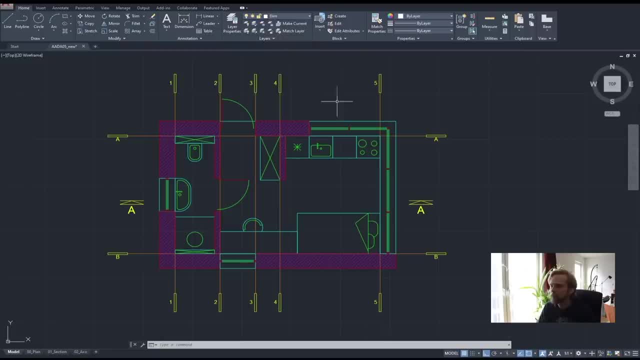 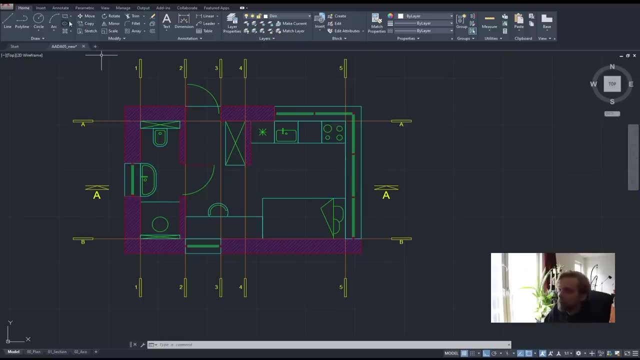 Color, Let's find it Dim. There we go. So dimensions. One last thing: If we go to the annotate tab Here, Here we have the settings for our text, For our dimensions And what not. So there is. 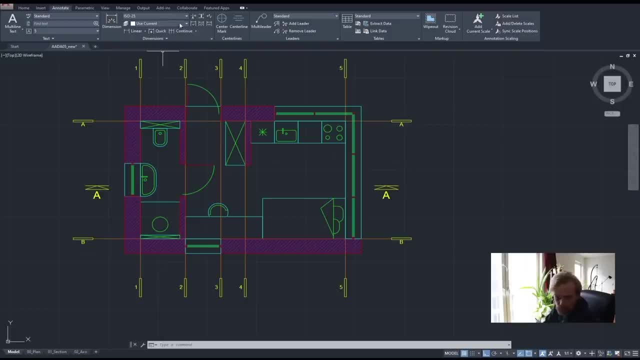 There are presets Already Right Annotate tab, Dimensions, sub tab Right here, And there are preset dimensions That we can see here, And these are not that great. We want to make our own, So what I'm going to click on? 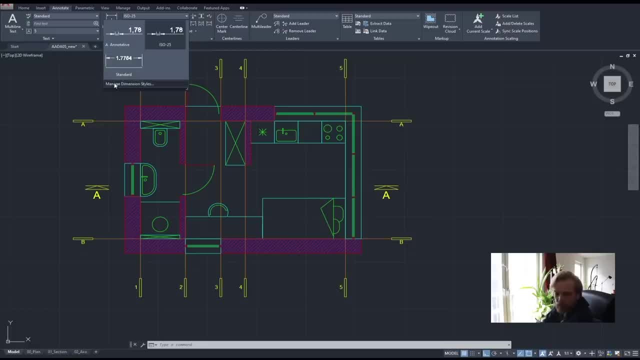 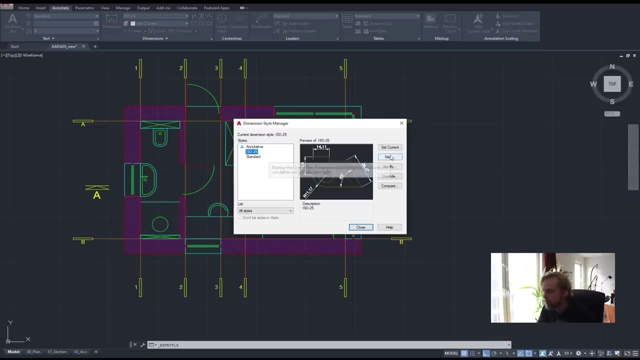 Is this: manage dimension styles. So again, You click on this drop down box And you choose manage dimension styles Right here, Which will give you this table Dimension Right, And I'm going to do exactly that. New, I'll call it. 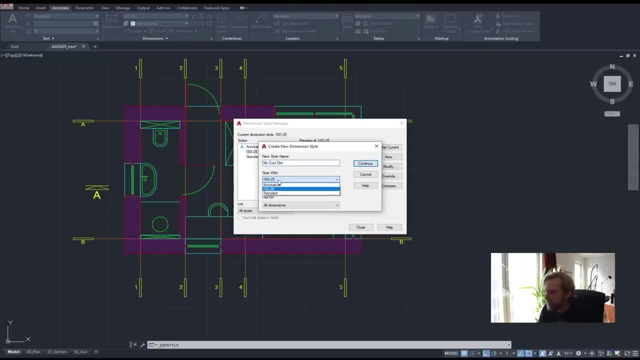 My cool dim, My cool dimension, And I'll start with Whatever, Either standard or ISO. You do not start with annotative, though That is something else. Do not tick mark annotative. The way annotative works is As you're zooming out. 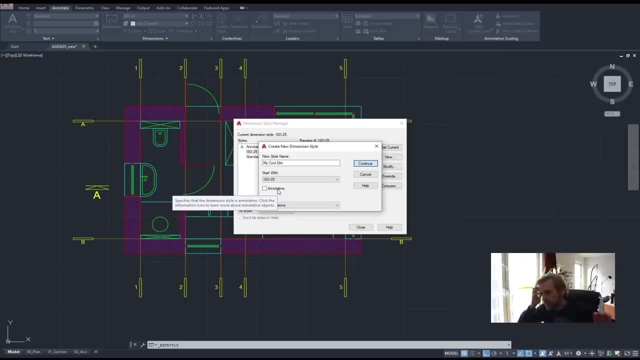 It will increase in size, So they are kind of locked in size In terms of millimeters. You don't really want that In this particular project. In larger projects You do use annotative, But that's going to be later. 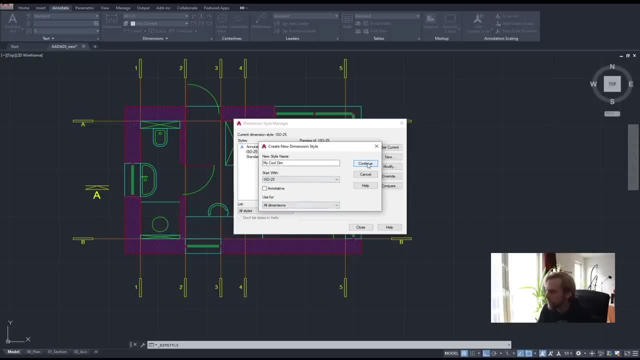 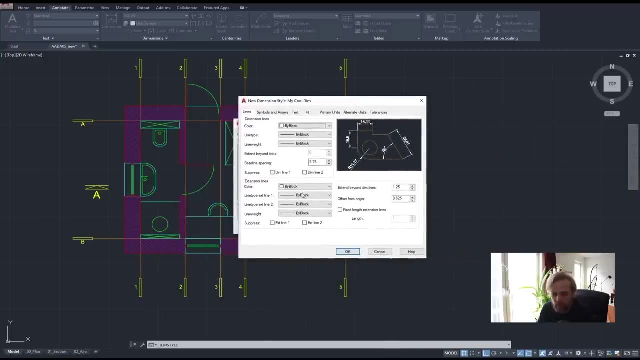 That's going to be much later. Use for all dimensions: Yes, So do this. Hit continue. And this is where you kind of set up All of your dimensions. Color is going to be By layer, That's important, So all of your dimensions. 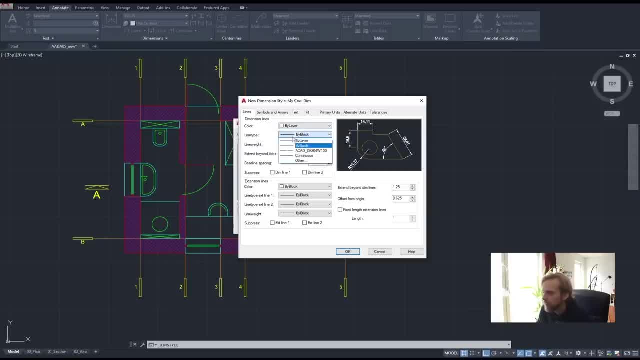 Are going to be colored by the layer In which they are in. Then line type is going to be by layer And line weight is going to be by layer. So we are controlling the dimensions Through layer, Not through block. Then you have baseline spacing. 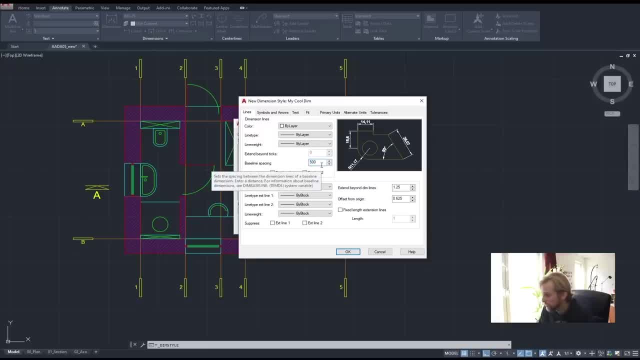 If I change this to 500, for instance, Nothing happens. Whatever, Then we ignore it. Is it a bug? again, We'll see if it's a bug or not. You do have suppression though. So suppression is If you kind of change these things. 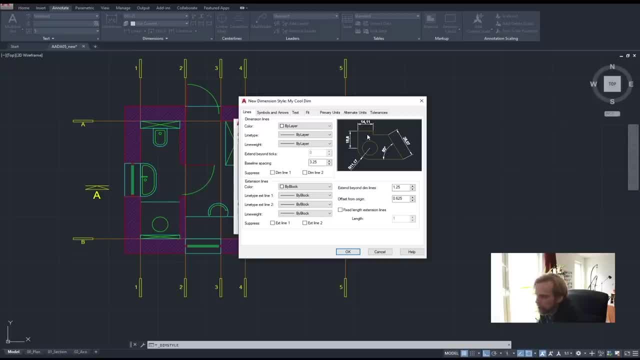 You can see what Changes here. So if we suppress them lines, Both of them, You don't see the arrows anymore, Right? So we don't want that to happen. As you can see, Extend beyond them lines. This is, by the way, in millimeters. 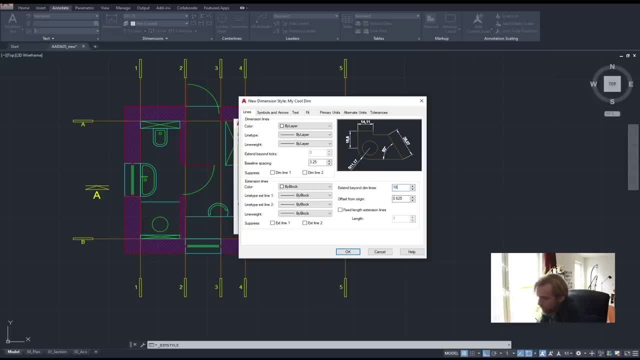 So this is very, very small. If I change this to 10. You can see that These lines get extended Much further. So here I'm just going to say- And this is where we are going to Kind of start messing it up- 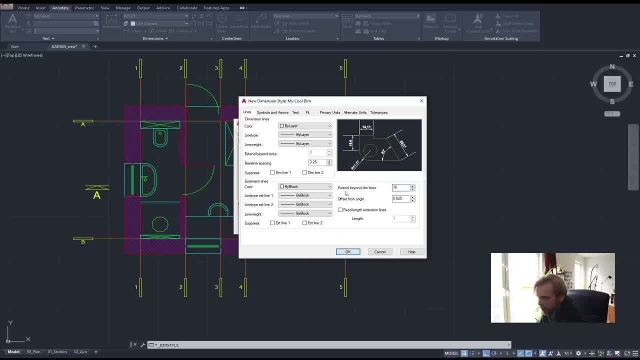 For now, let's keep it at 10.. We will come back to this. We will indeed come back to this Everywhere where you see, by block, You change to by layer. This is just the way you do it: By layer Right. 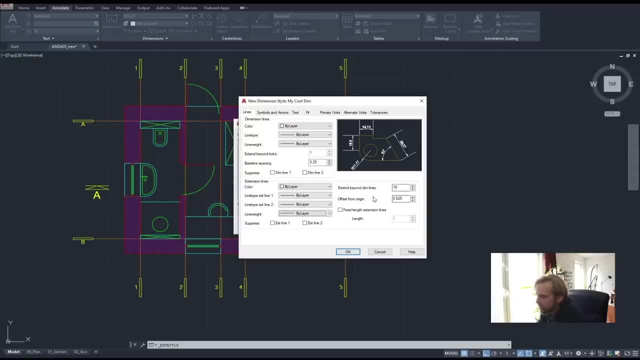 We will come back to the extension In just a second, Also to the offset, But for now I want to change the symbols. So in architecture we don't use arrows, We use dashes Or ticks, Architectural ticks. So the arrow heads are architectural ticks. 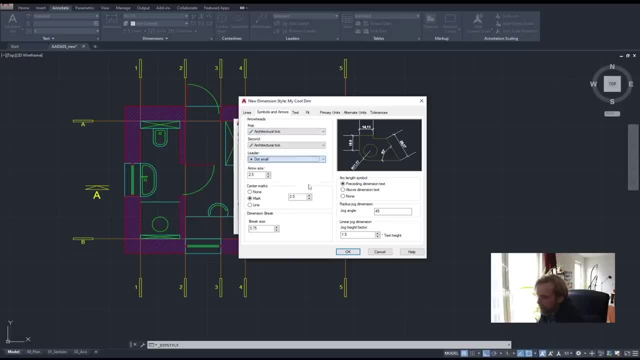 The leader is architectural tick Or the leader can be a dot as well. That's fine. We can use a dot For the arrow size. This is 2.5 mm in size. That is way too small, Because this is like 400 mm thickness. 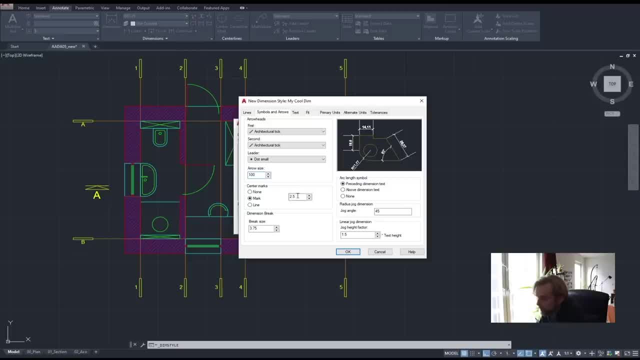 So we want the tick mark to be Around 100 mm, And now you can see How it messes up the view. That's fine, We will fix it. Center marks: We will not be working with center marks, That's fine. 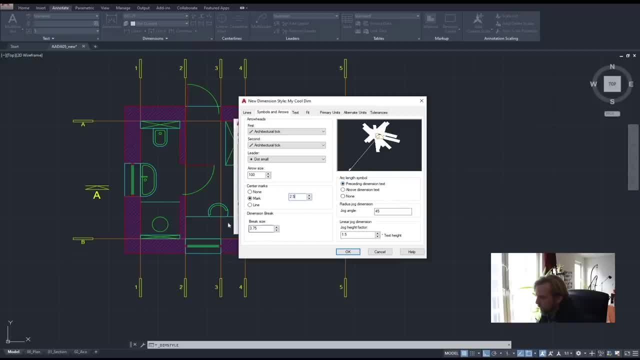 Arc length symbol. We don't care about anything Else here. Yeah, So it's just these four things here. Then for the text, We will change the text height, So the text height right now is again. Oh, by the way, 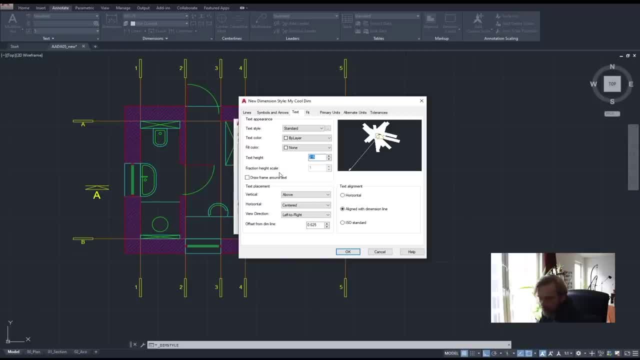 Text color by layer. Text height: We will change this to higher Text, of course, And we will use Something around. I want to say 75 mm, I will just do 75. And now you can see That we are back in business. 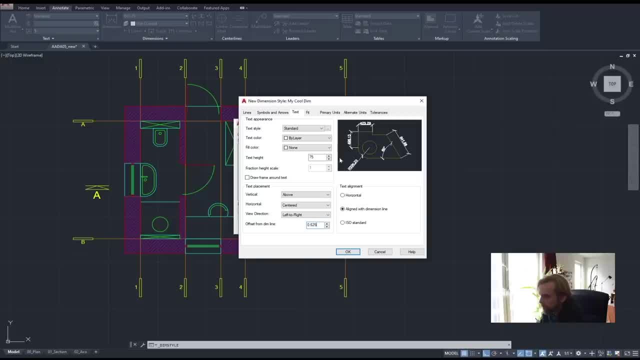 So it's kind of Back to what it was Before. Text placement. I do want to offset it, So it needs to be above And centered To the dimension line, But I do want it to be offset Above it a little bit more. 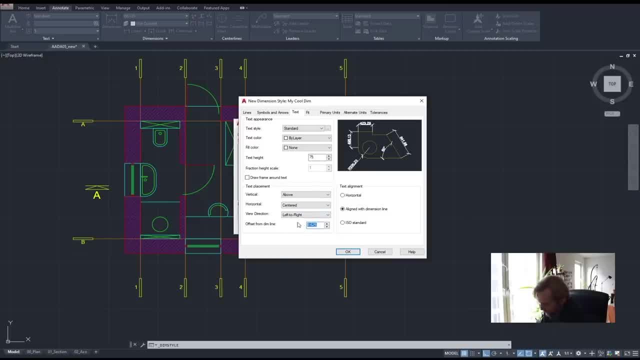 So I will just give it like If the text size is 75.. And offset it by 25.. So it's kind of It has a gap here. Text alignment aligned with dimension line: Perfect, That's fine. Nothing else here. 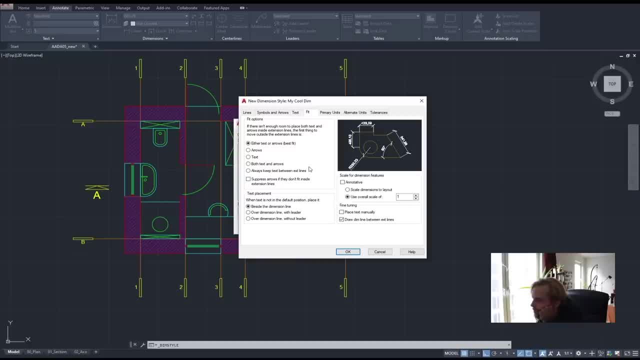 Fit For the fit. The only thing that I change Is text placement. If it doesn't fit In the dimensions, It needs to be over the dimension line With a leader. If Text doesn't fit here, Then it's going to draw this line here. 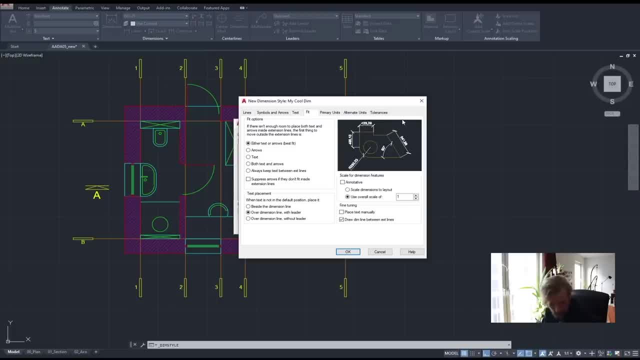 Like an angled line And it will show a text Somewhere else. Then Here you can see That it's not full numbers, It's with a comma And we are dealing with millimeters, So we don't do this. 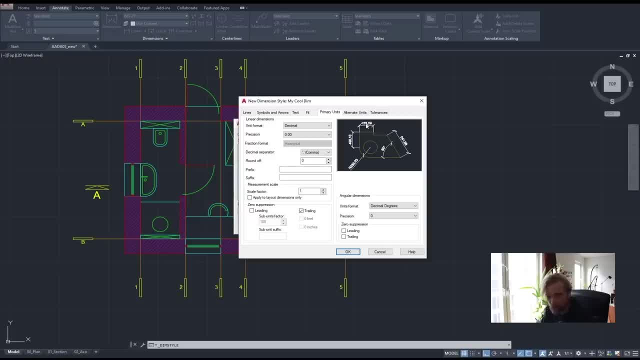 We need to Show only full numbers. So In primary units, Where it says precision, I will change the precision to 0. So it only gives us full numbers. So we have that done. Tolerances, we don't care about. 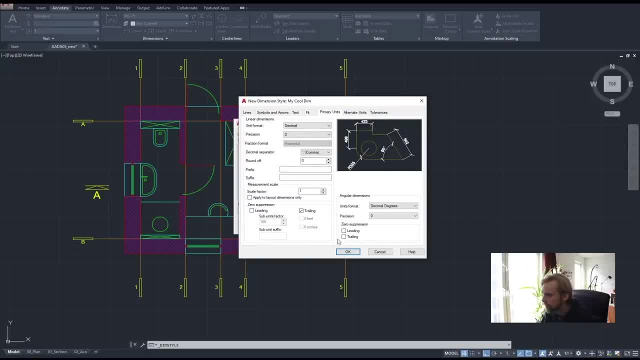 Alternative units we don't care about. Do we care about anything else here? No, No, we don't. Back to lines, tab Under extend them lines. I had it as 10.. So 10 now is super small. I will have it as 100.. 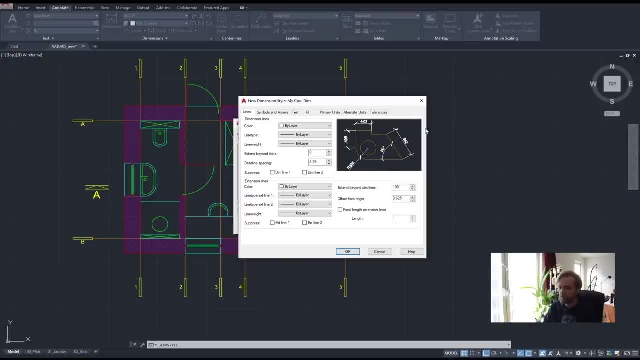 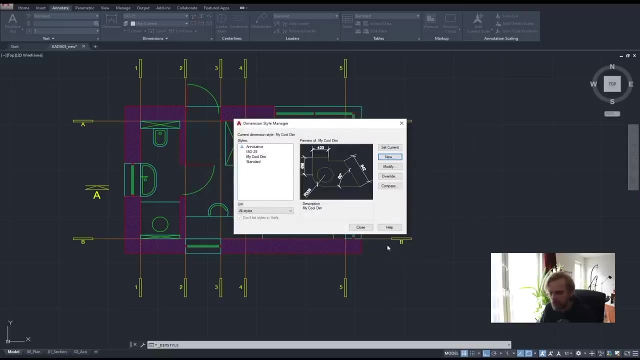 So it takes, extend The dimension lines. extend by 100.. Alright, I think that's it. I think that is it. That's all we need to do. Let me double check. Yeah, everything seems fine. My cool dimension is now my. 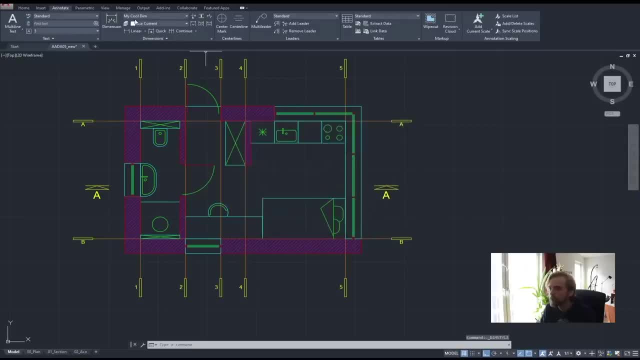 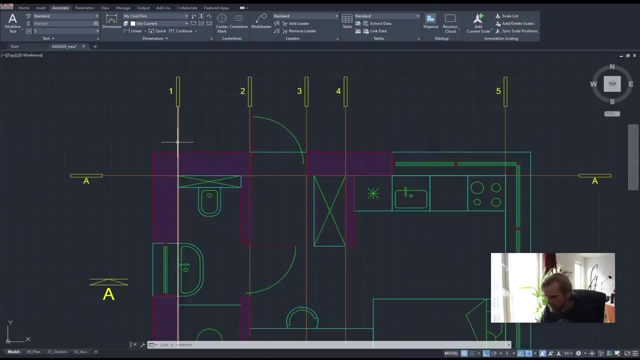 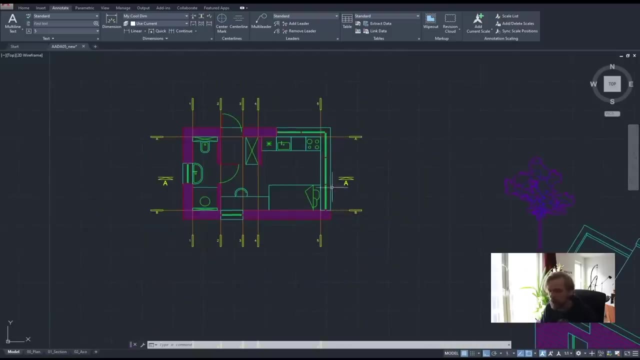 New created dimension style. I will click close. I will make sure that it's my Active dimensional style here And now I can start adding dimensions. So In the top And on the side Here I want to add dimensions. 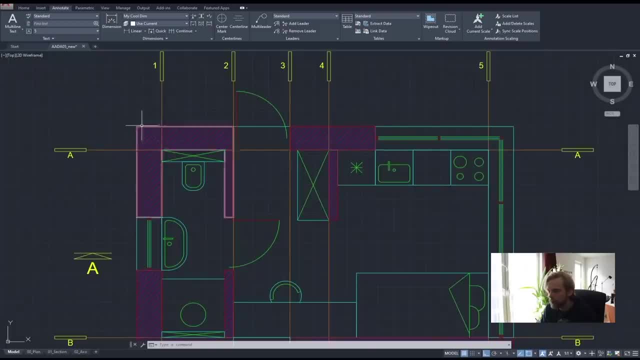 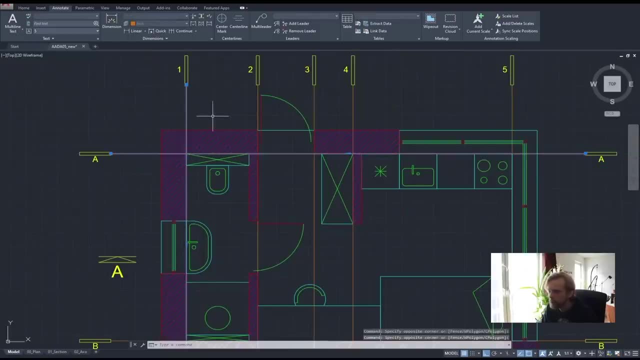 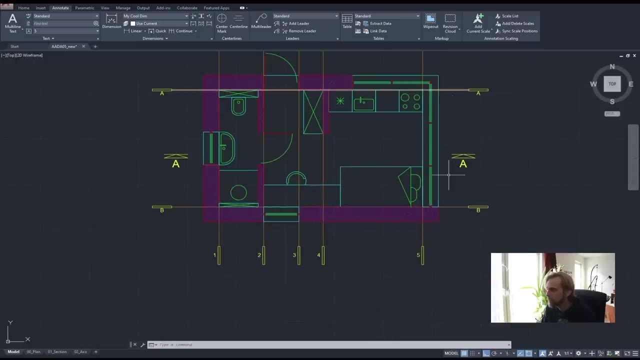 And also I kind of want to anchor the dimensions To somewhere. Maybe the corner here Or maybe this intersection between 1 and A Is going to be my anchoring point. That's fine, So these guys Will have dimensions. 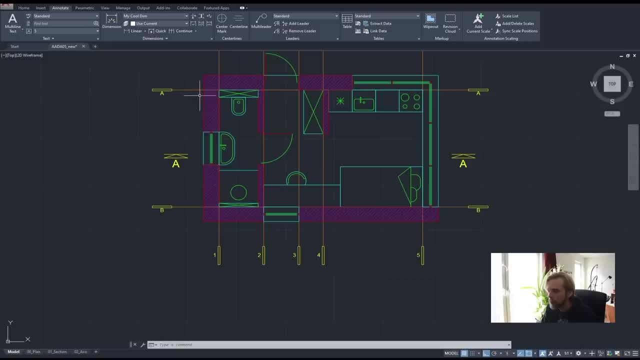 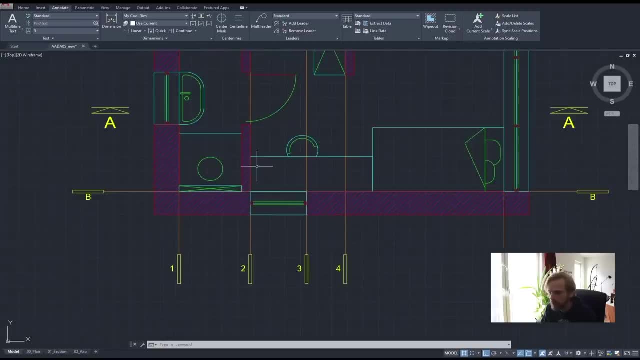 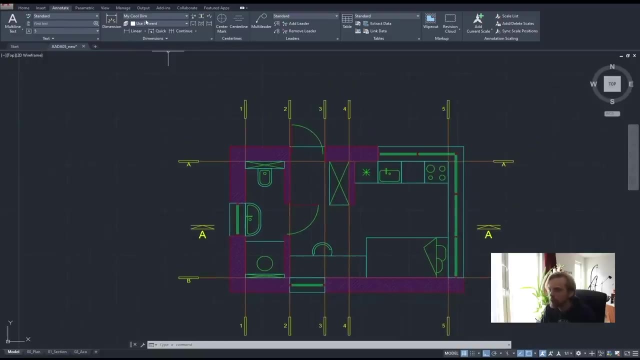 Anchored to the Axes, So on this side I can just add some additional dimensions Here and there That I want to showcase. Maybe I won't, Maybe just for the windows, Let's do it. So my cool dim is my active dimension. 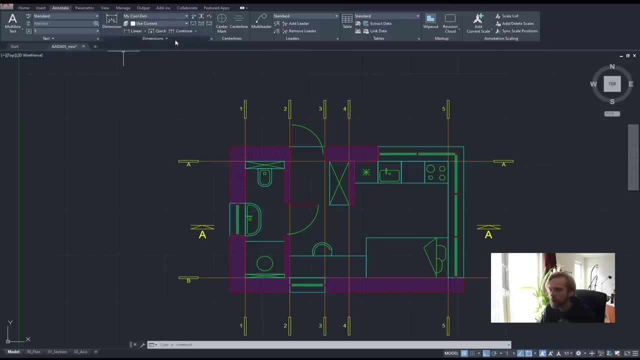 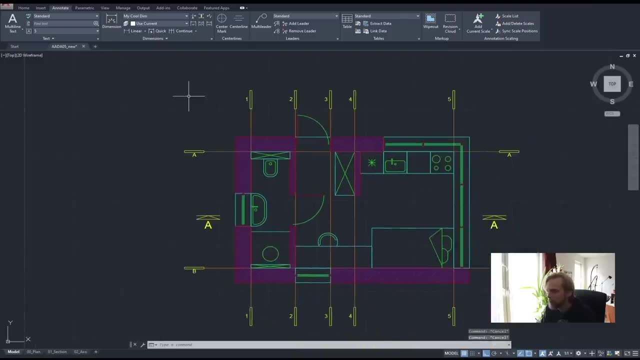 And here I have Two options for the dimension styles. Well, there is actually more options here, Because if you want an aligned dimension, You can have that as well. I will show you all of them, Or at least three of them. So, linear dimension. 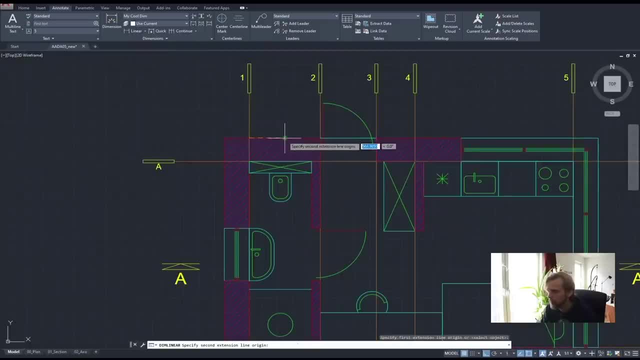 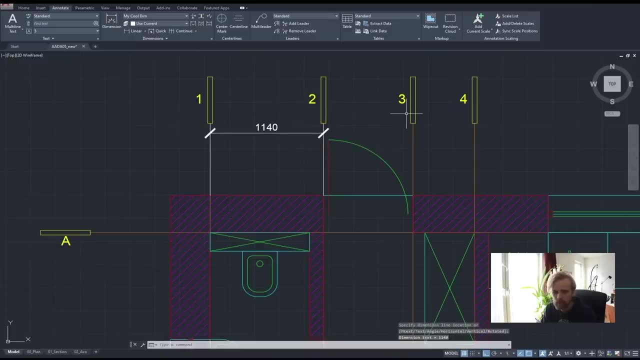 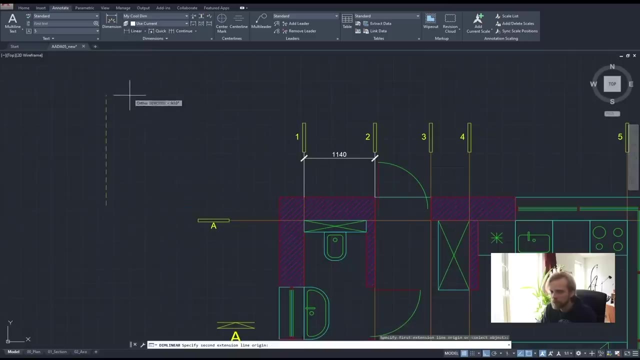 Is basically, If I click on it, And I click on first point, Click on the second point, Drag it out. You know That is a linear, Linear dimension. So the thing about linear dimension Is that it can only go. 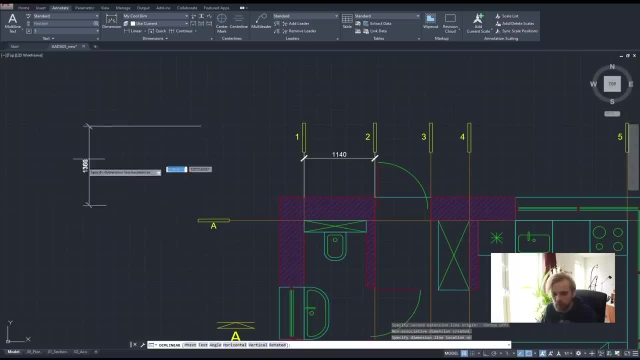 Either horizontally Or vertically Right. It can't go at an angle. I need to use What is called an aligned dimension. Where is it? Where is it? Where is it? Ah, there it is. So We click on the small icon. 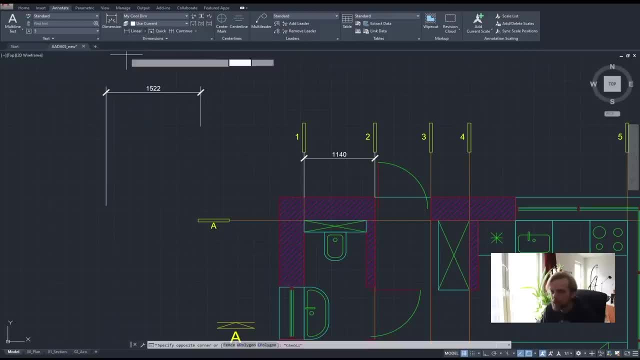 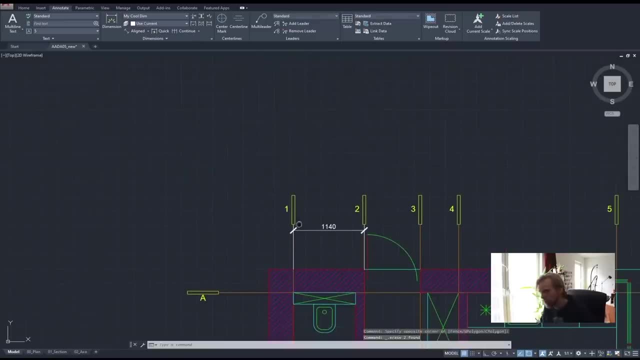 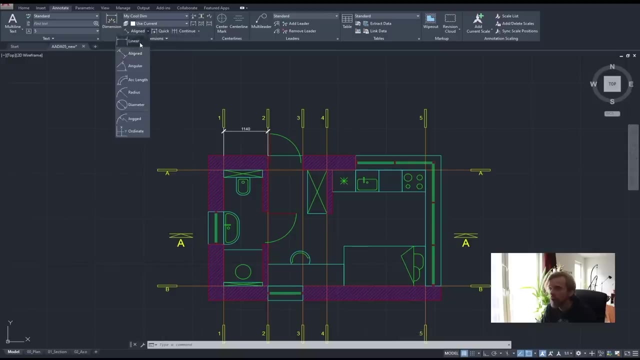 Right next to linear dimension. Expand it And we can see aligned dimension here. If I select aligned And I click click, Then it creates this angled dimension, Right. So if you don't have any aligned dimensions, Just know that you can have those. 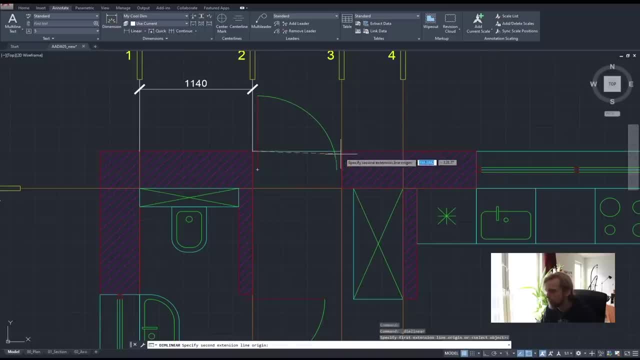 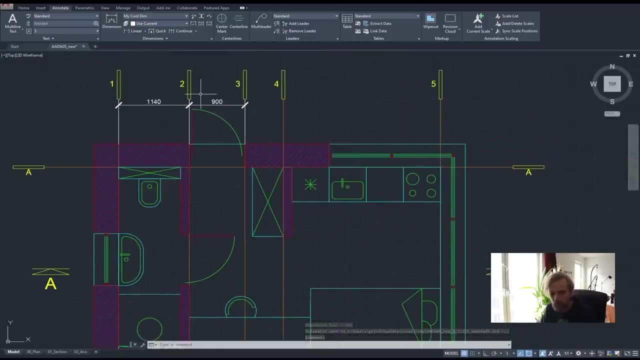 I will just be using linear Linear From here to here. If you want to have, If you don't want to kind of Keep repeating the dimension command, You can use Continue This Pool right here, Which basically just will continue on. 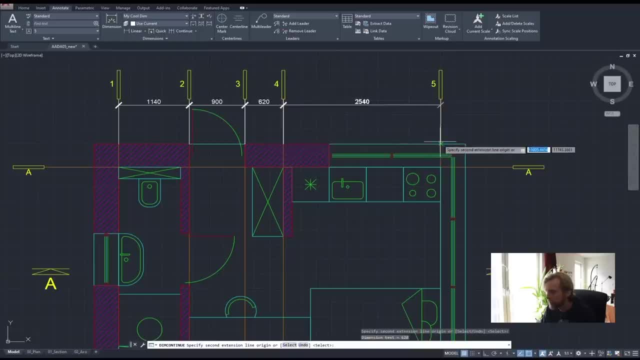 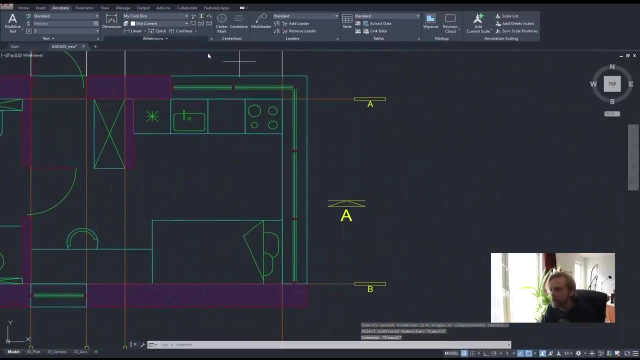 From the last dimension that you've done And you can just kind of Then only click once, And once you're done You just hit enter And it's going to add the dimensions Right. So then I'm usually the way I do it. 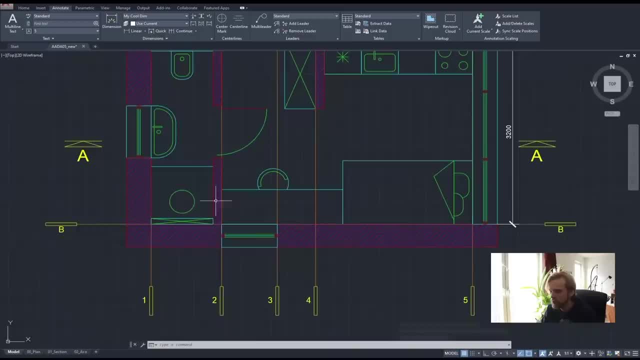 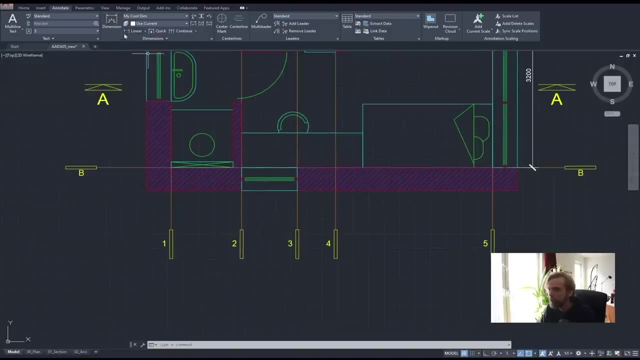 Is I create a single linear dimension And then, if I want to continue from it, I just click on continue And then do it that way. Now for the For some additional anchoring. I will do, I will do a linear dimension. 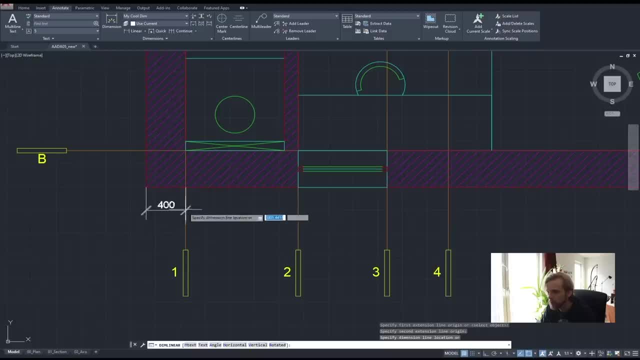 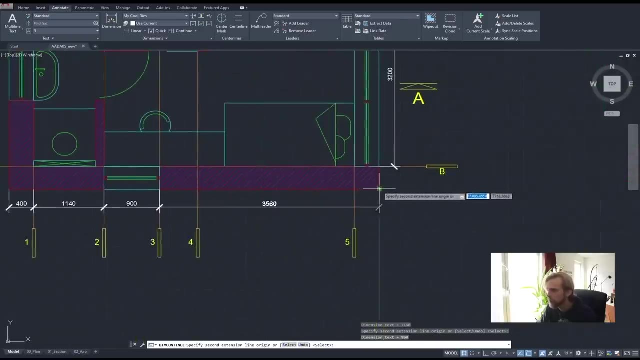 Between the corner Of the building To the axis one, That is going to be four hundred millimeters. Then I'll continue it Until the start of the Of the window, Then until here, And then I'll kind of continue it. 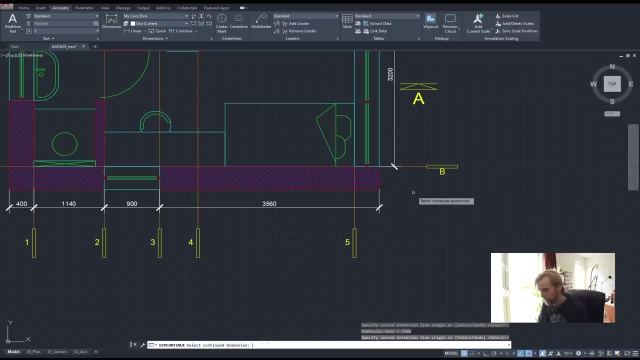 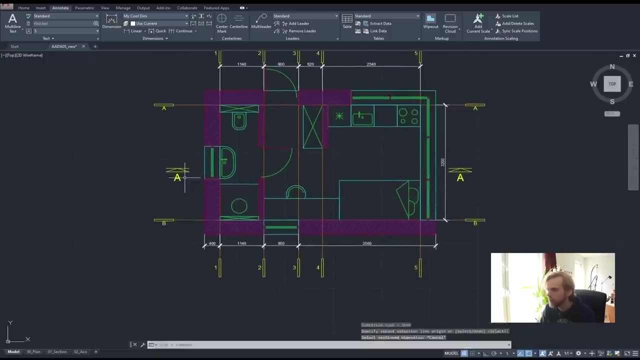 All the way through To the end of the building, Like so. So now I have registered these two Corner points here And also the position of the window According to those two corner points. Linear dimension from here to here, Or sorry. 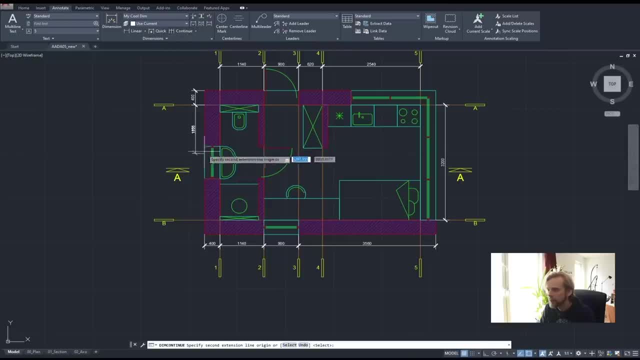 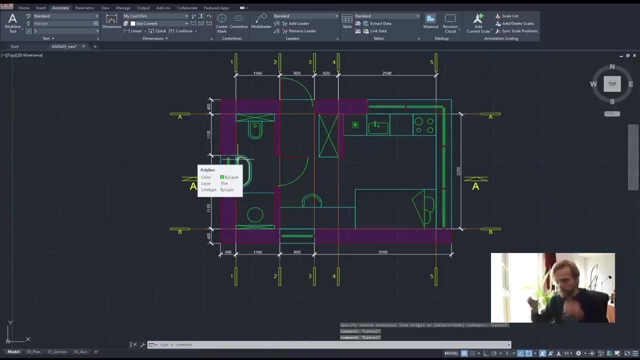 My bad. First of all from here to here, Then continue it until here, Here, And actually just until here. We don't need to anchor it to here, Or do we? Well, maybe we can, Why not? So that's done. 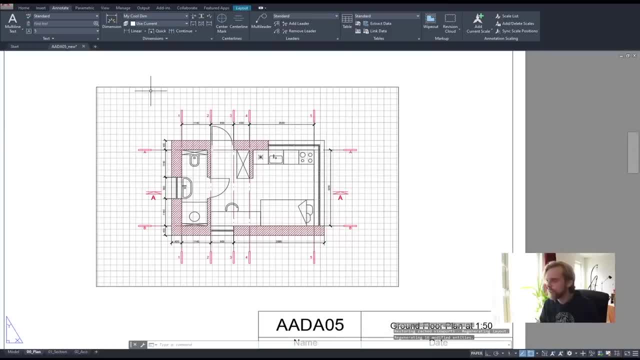 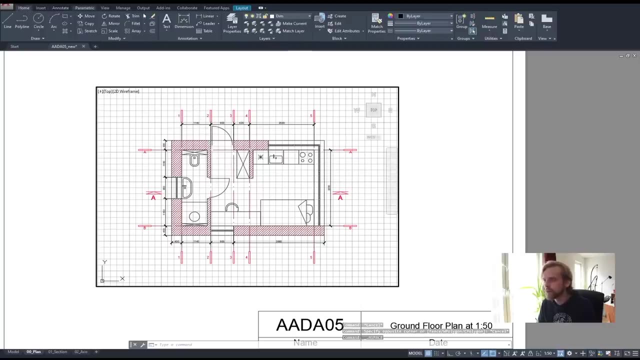 That is done. If we look at it in the plan view, That is how it looks, like It's not showing. Oh yeah, That's fine. It doesn't need to show up As red for now, But I will double click inside. 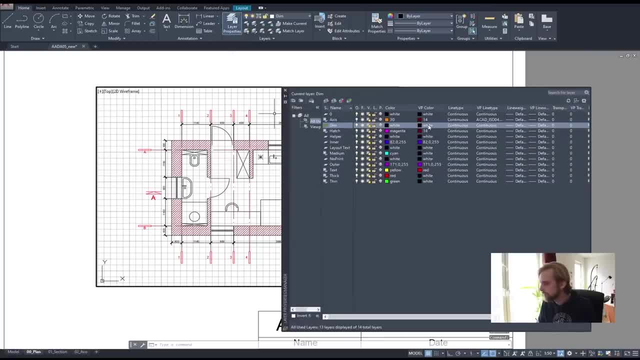 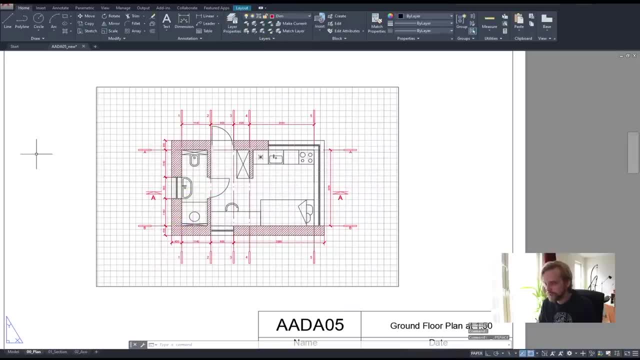 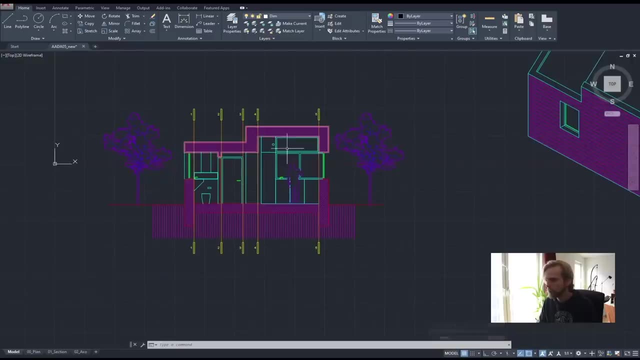 I will go to the layer properties tab And for dimensions, I will change their color to red, Like that Cool, Okay, so that's done. That is done Now for the section. So for the section: I do have dimensions here. 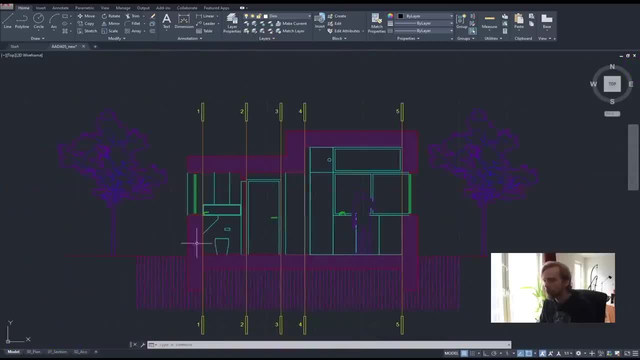 But since this is such a small project, I will not be adding them. But what you do have Is you have elevations. You mark out different altitudes For different things, So we won't have a lot of elevations here. 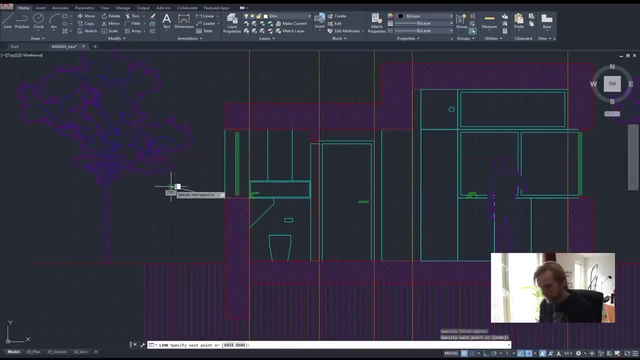 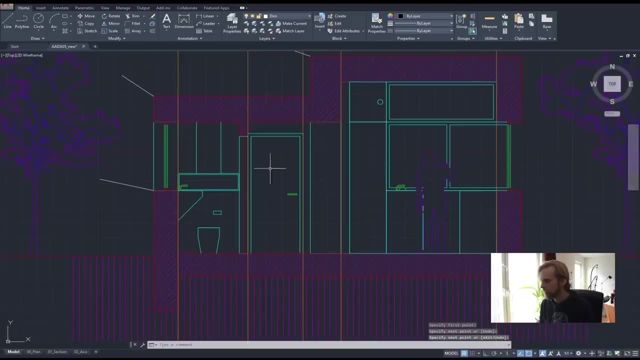 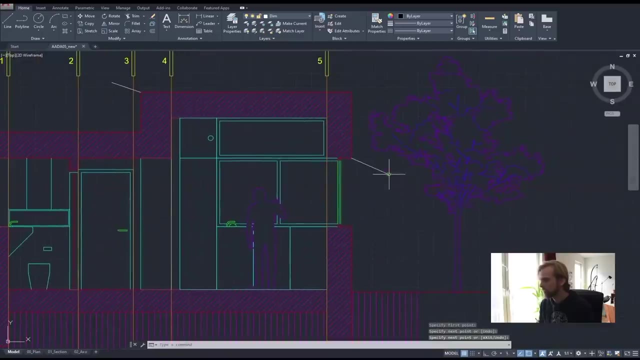 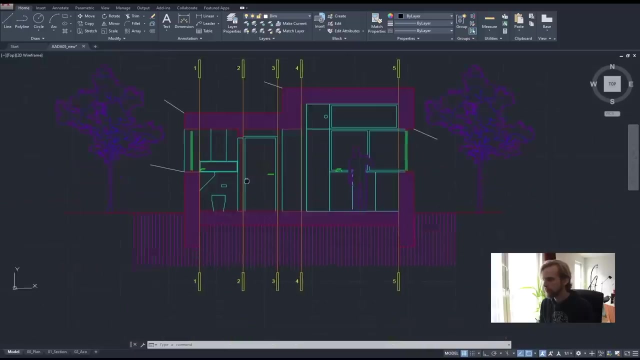 We will have one here. I will just kind of draw lines Here. There is going to be an elevation here And I want an elevation here, But that doesn't really matter. And an elevation here, Well, yeah, Elevation showing what's zero. 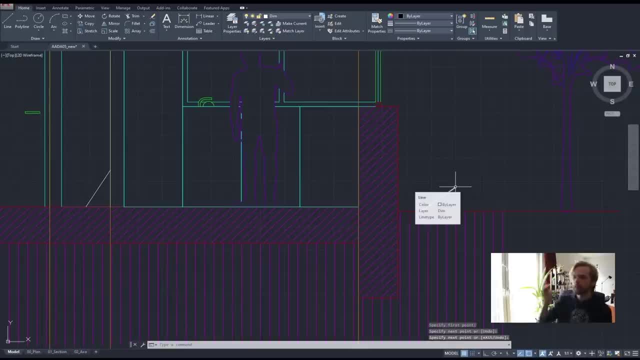 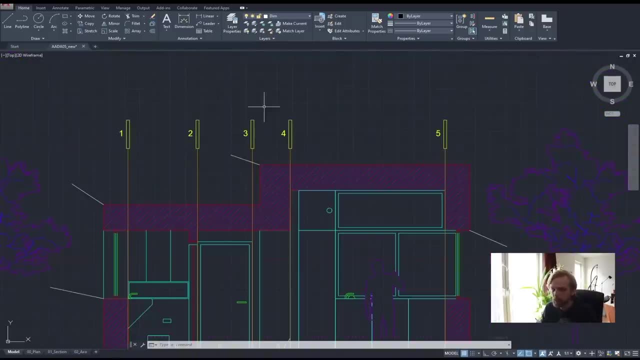 What do we consider to be zero, Right? So These are the elevations that I want to mark out, And for that I first need a markup of the elevations. So there are different styles of markups, The one that I like using. 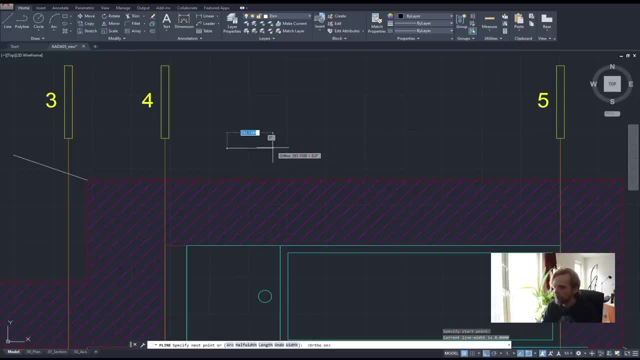 Is this. So we start drawing from the horizontal line And I will just do like 500 mm. That's too large. Let's do 250 mm, Like so. So we just have like this horizontal line, That's 250 mm. 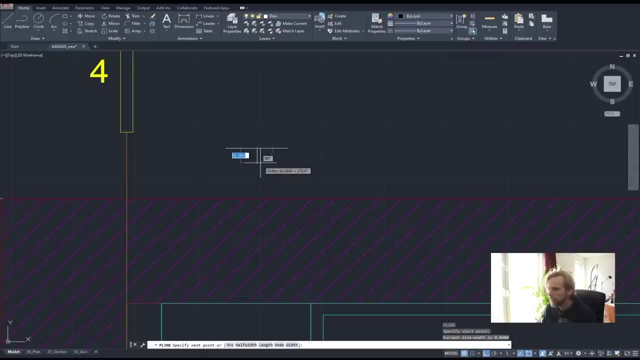 Then I am going to draw down By, Let's say, 50 mm, Like that. This is going to be my helper line. That's enough for me to kind of. This amount of lines Is enough for me to draw out my markup. 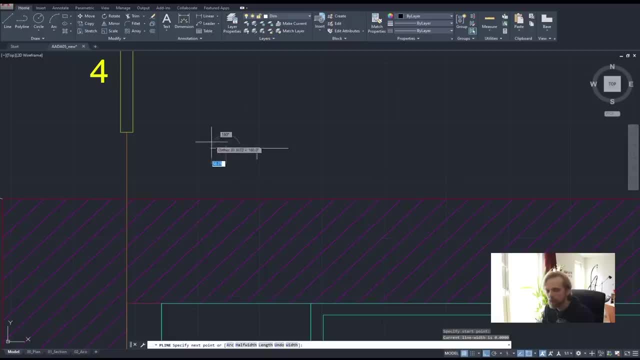 So let me do it real fast: Fall line tool: From this left hand side point To the end, To the bottom, Then we move across Up Like that And we extend it like so. So this is: You can treat this fall line. 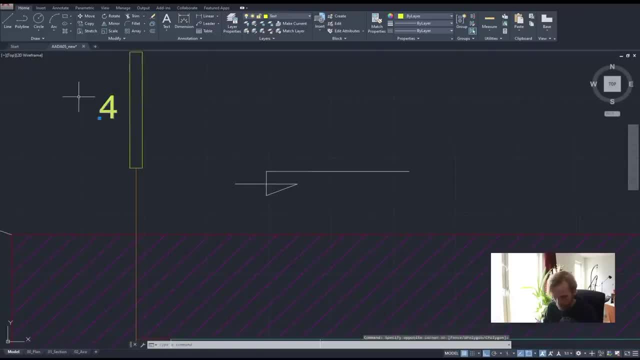 Basically as an arrow Right, And then I am just going to borrow a number Here, Since I already have it Move Like that, And I am just going to kind of Change the layer of the number To dimensions. Double click on it. 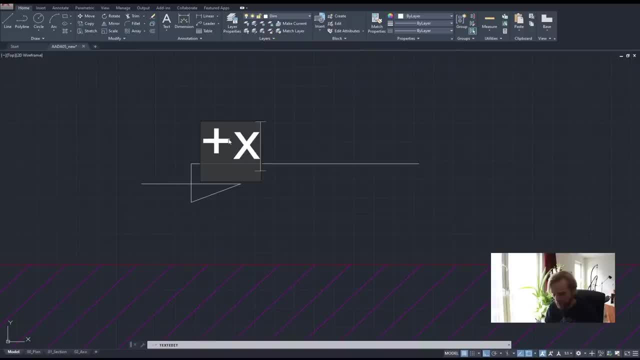 And change it to plus X, point XXXXX, Or three X's Right. So this is how Altitudes are written. While dimensions are written in millimeters, Altitudes are always written in meters, With three digits after the comma. 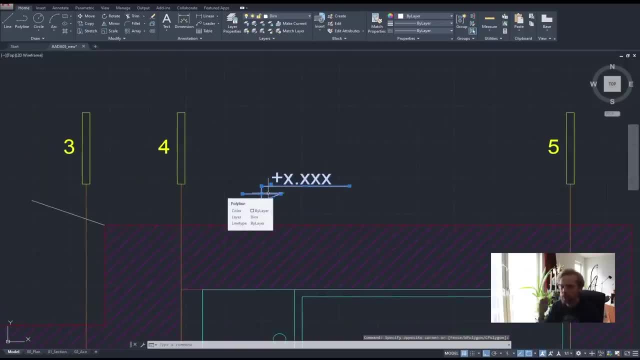 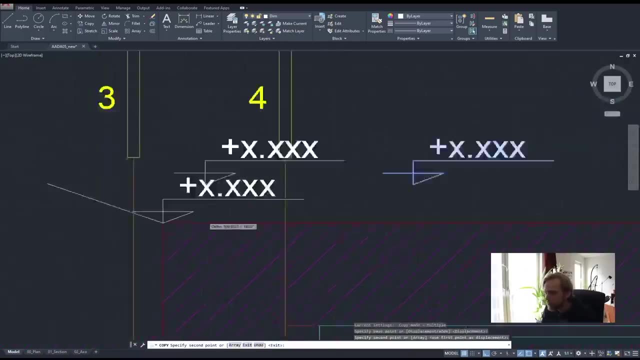 This is how you distinguish between What's an altitude And what's an elevation, Or what's a dimension, rather. So let me copy this From this point. I will want to show this point here. I will want to show this point here. 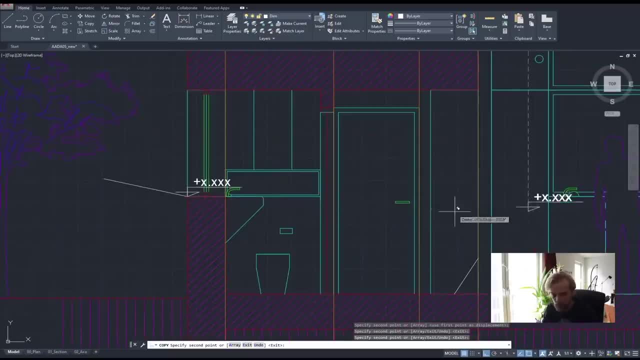 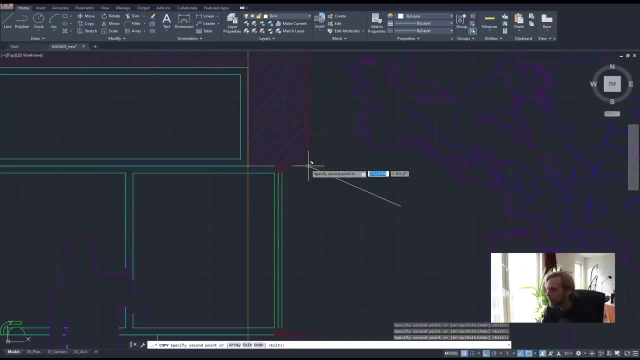 I will want to show this point here And you can see the graphical System. I will want to show this point here, Point on the ground, And this point right here, Right, So let's get rid of the helper lines now. 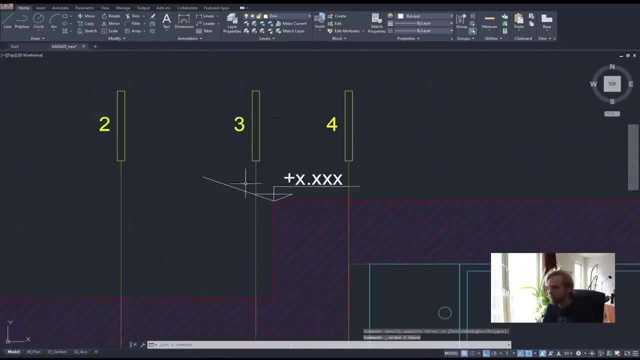 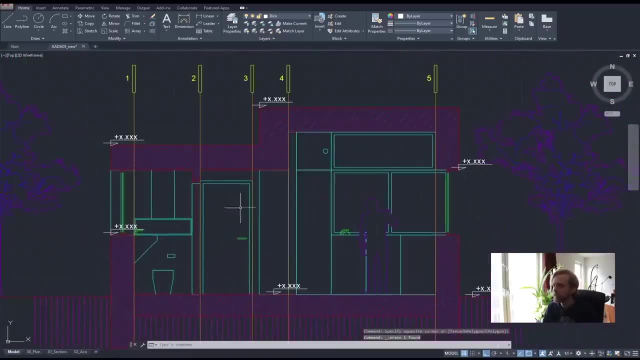 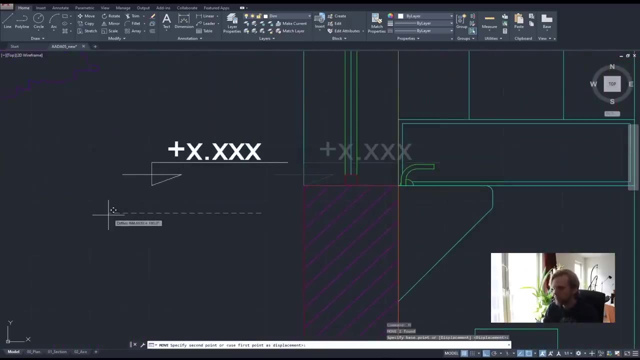 That, that, that- No need for that, That, That And that. And now let's start Kind of cleaning everything up. So this guy right here Intersects with the building. I will just move it to the side And I will create one more line segment. 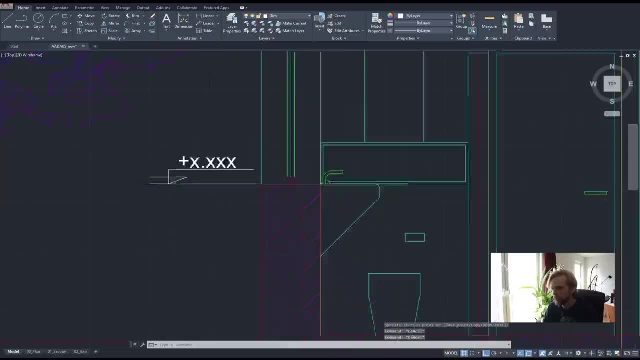 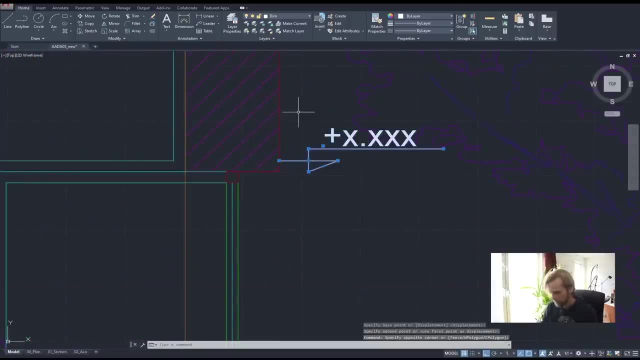 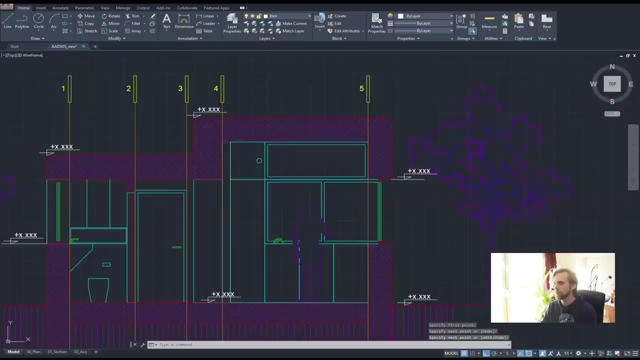 That kind of Does its thing like so, And for this one The same thing, But in this case It doesn't need to extend too much. A little bit more, Like that Line segment, Drag it out like: so, Everything else is okay. 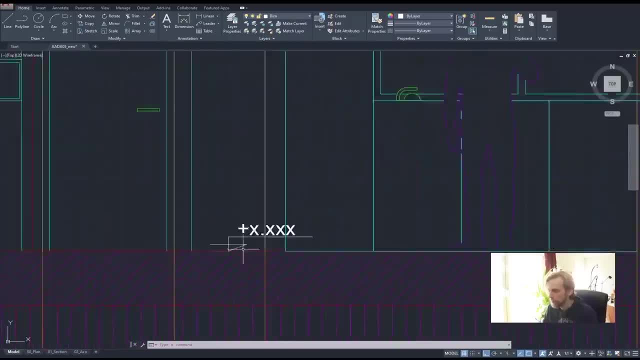 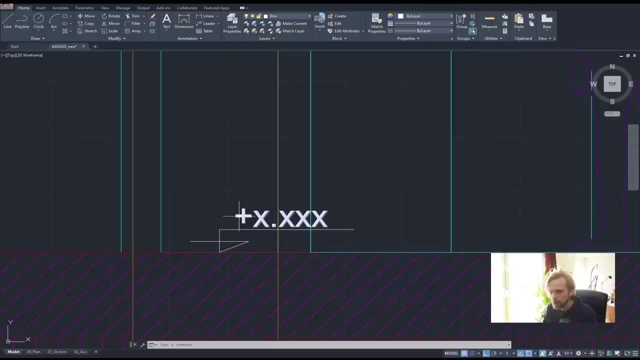 Everything else is not in the way. So now, So Always, the floor plate, Like the top of the floor, Is 0.000.. So it's neither plus nor minus. It's actually plus, minus, Right? So I will. 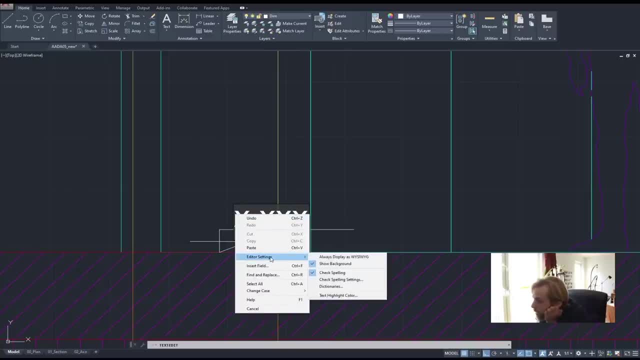 How do you? I forgot How to insert a special character. Oh no, Well, if you don't, Ah, If you can't use a special character, You can always do this: Plus minus. That works as well. 0.000.. 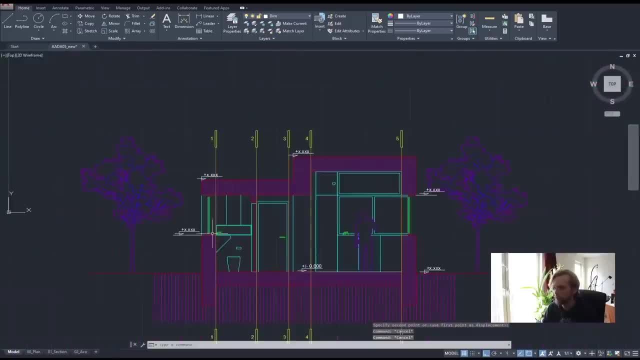 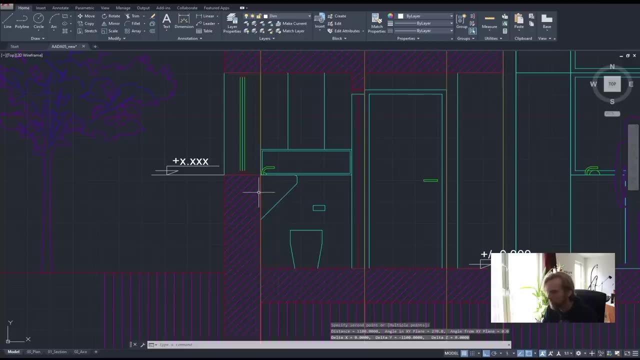 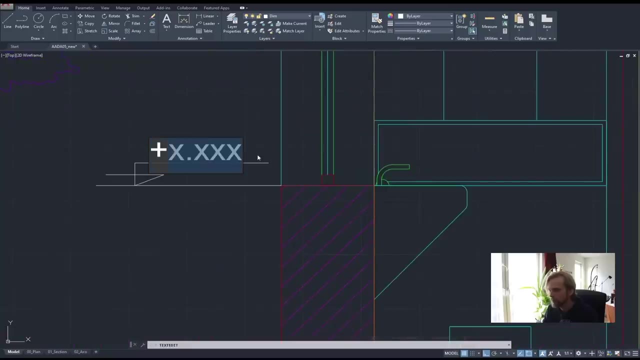 Right, That is our starting elevation And that is our floor plate. Then I know that this is, Let me just- Actually I don't Let me- measure the distance. This is 1.1 meters above the floor plate Right. 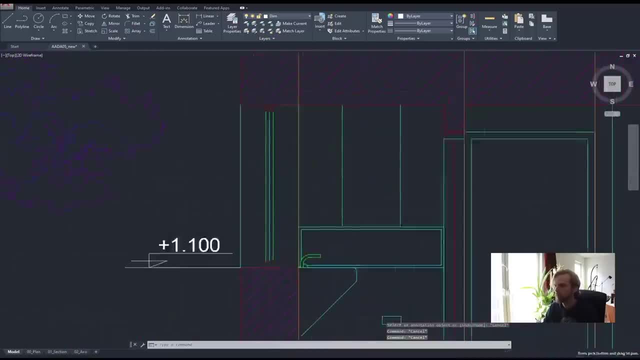 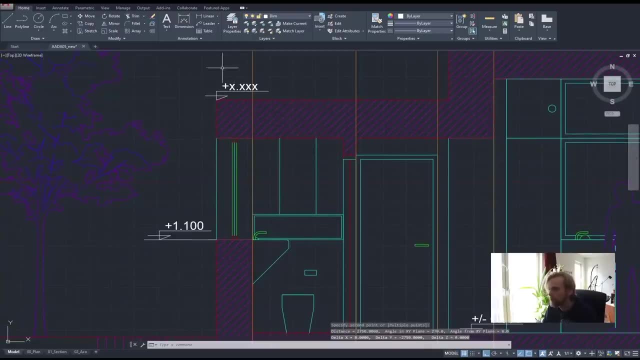 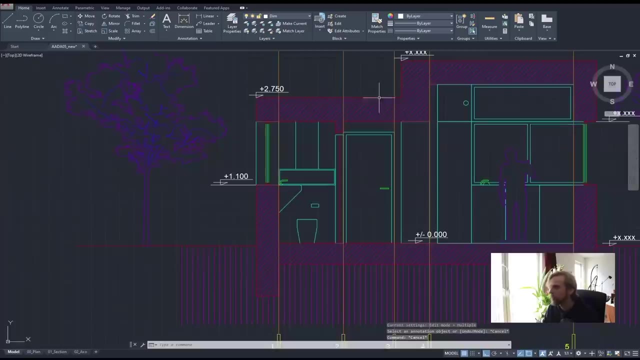 1.100.. Right, That's the altitude, And this one is going to be, Again measure distance From here to here: 2750.. So it's going to be plus 2.750.. Then here we will have. 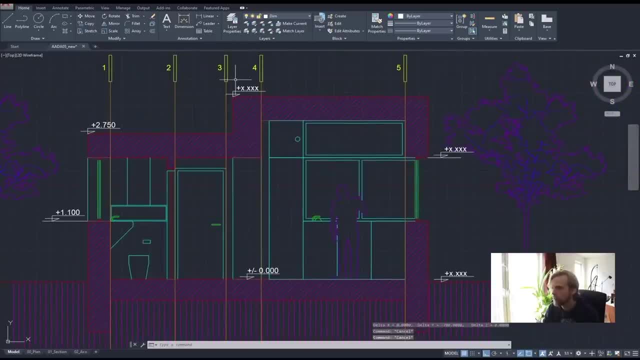 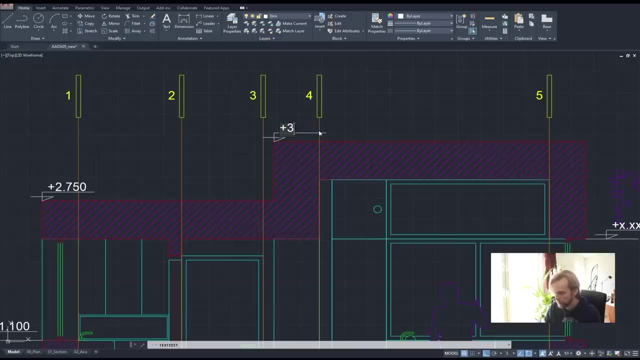 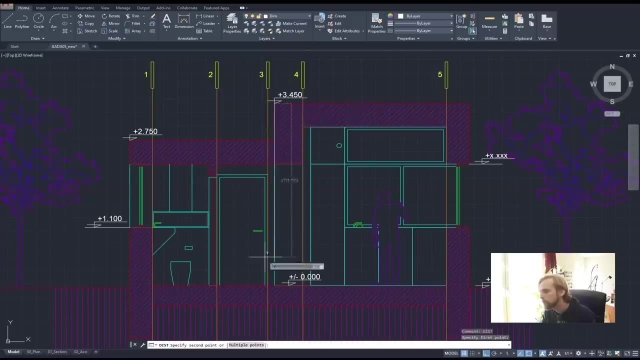 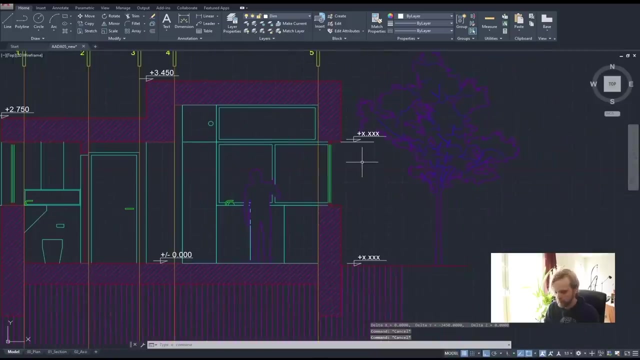 Probably- I'll just measure this- 700.. So 3450.. 3450. Wow, Feels weird. Wait, Is it really 3450?? Yes, it is Okay. And then this height Right here. Distance from. 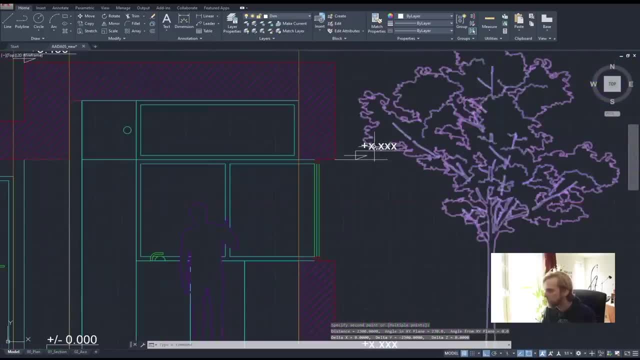 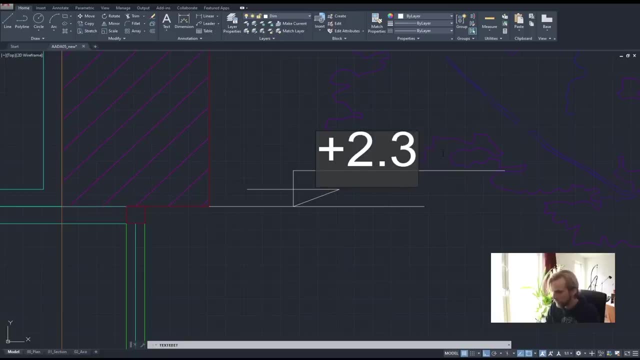 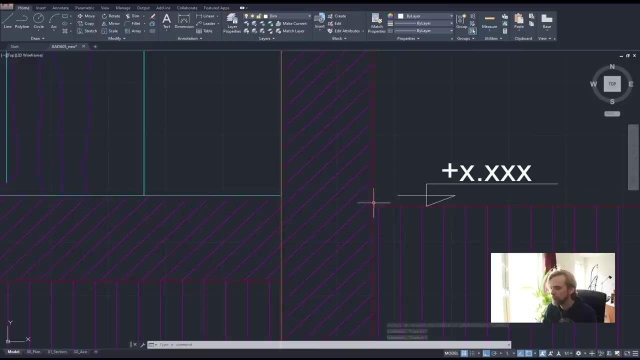 Let's see this line To here: 2300.. Plus 0.300. And the last one: here It's going to be. I remember I just moved it by 5 centimeters down, So it's going to be negative. 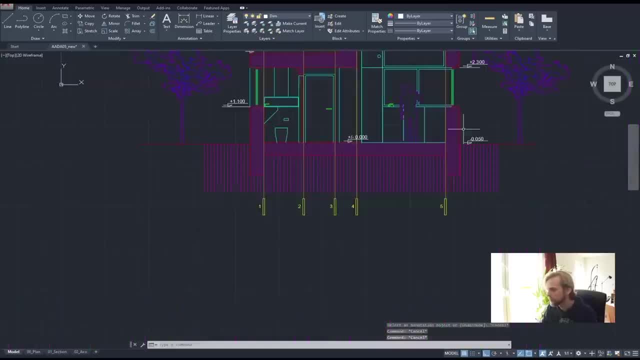 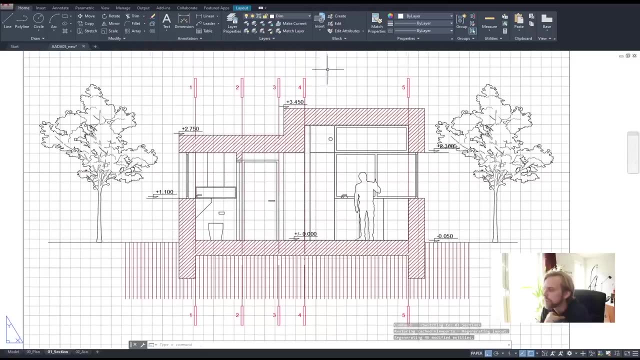 Right Minus 0.050.. That's it. That's all of the elevations. Let's look at them in this section. That's how they look like in this section, And I want to change their colors In this section as well. 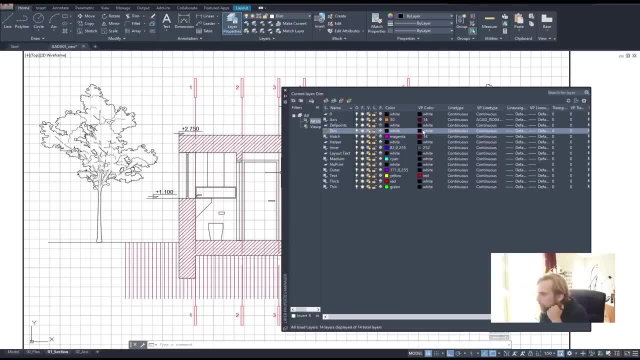 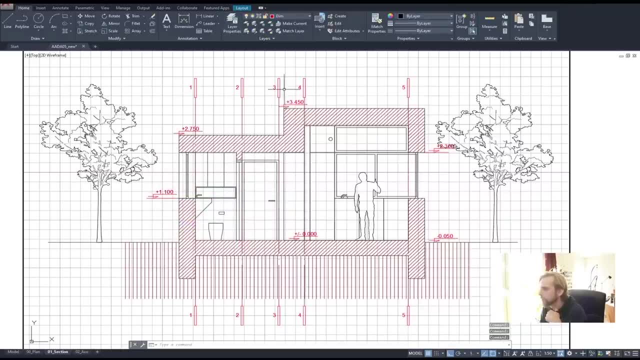 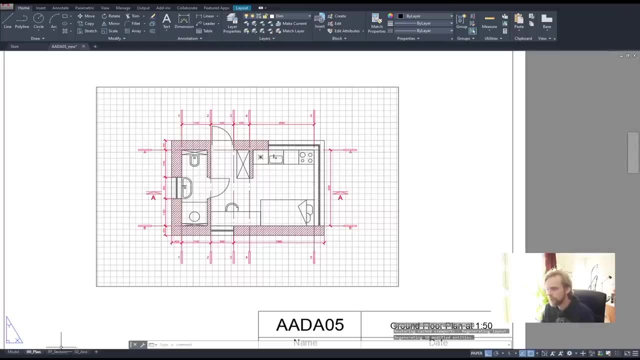 Properties, Double click. Don't forget to double click. Go to layer properties Dimension And here just change it to Whatever color we're using. We are using red color For these markups. Double click out. We're good to go. 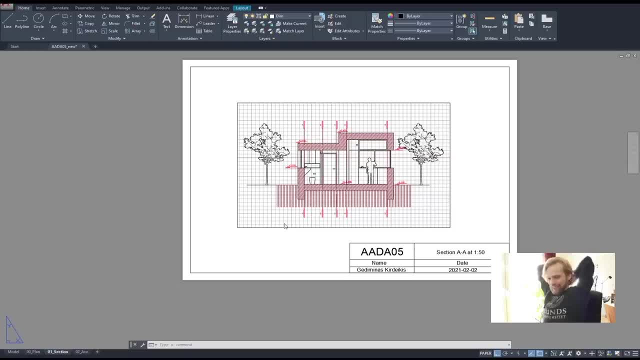 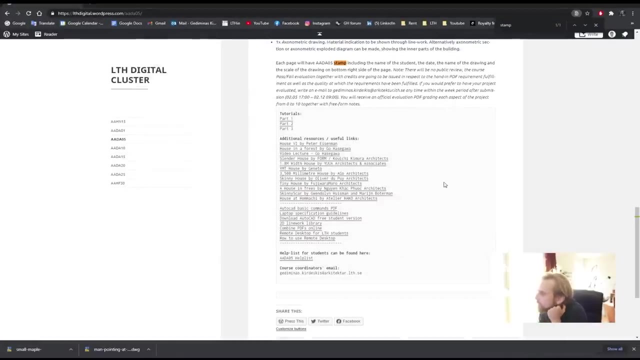 Okay, So we have our plan, We have our section, And what we need to do Is to actually plot this out Right To create a PDF, Or actually Let me. I'm now scared that I'm rushing And I will forget something important. 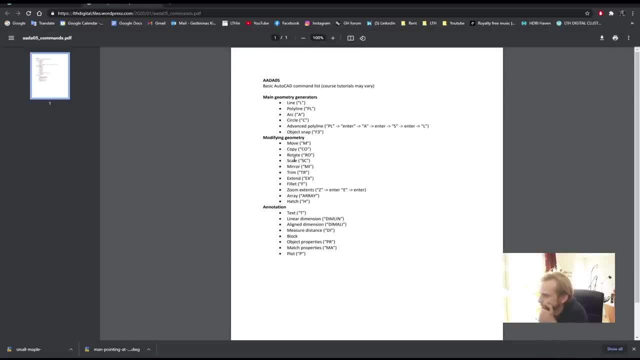 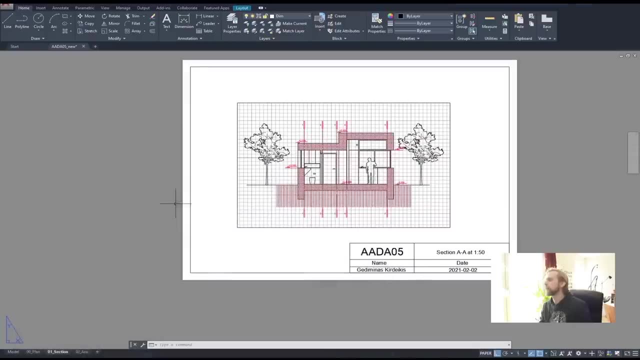 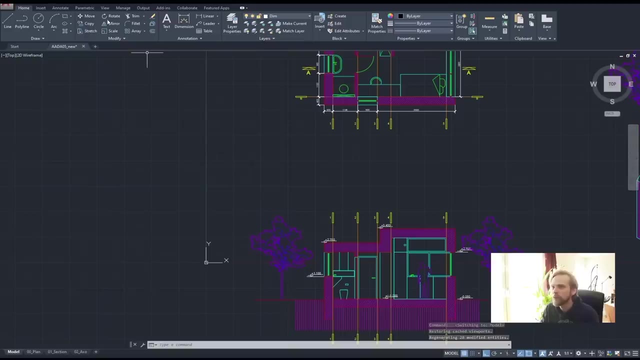 So let me just Double check Match properties, Okay. So One last trick. I guess, If you have, let's say, A line Here, Right, Come on A line Right, And it's in dimensions layer. 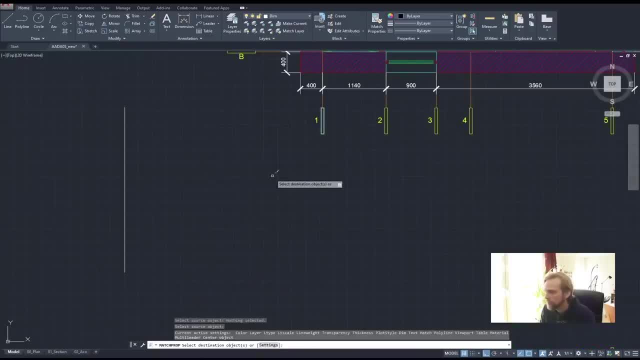 And you want to change its layer. You can match, Match properties, MA The object to which You want to match the properties to Like that And it's going to Move it in the same layer As the source And change all of the properties. 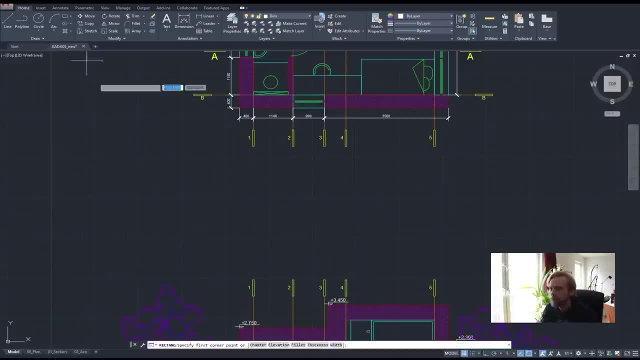 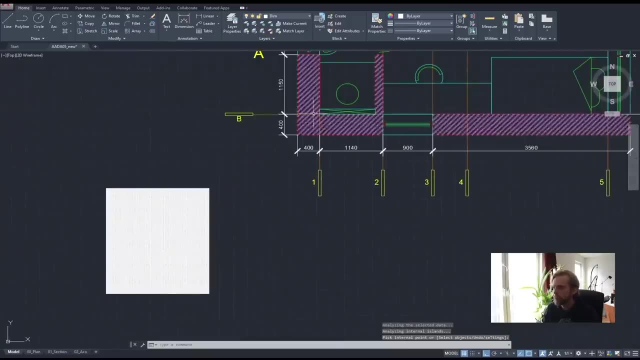 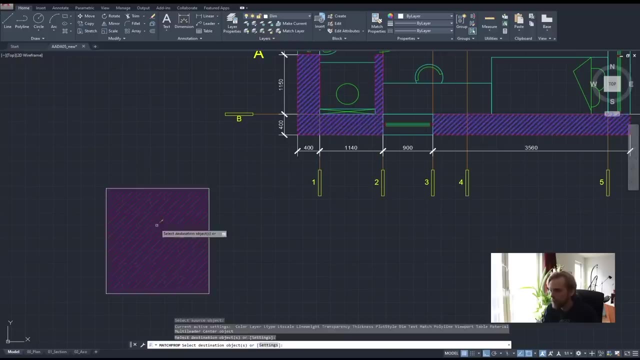 To be the same of the source. Usually it's used for hatches. If I have, If I have a hatch, You know something like this And I want to make it Exactly the same as this. I can match properties Enter from this hatch. 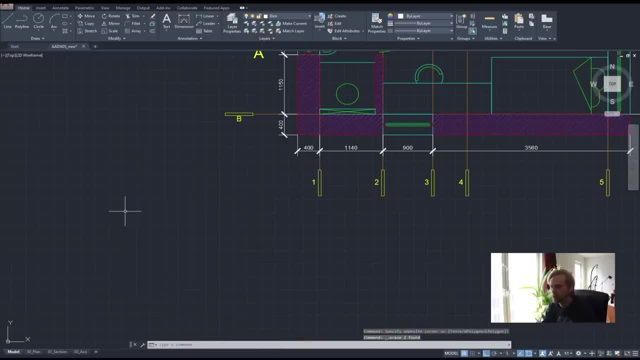 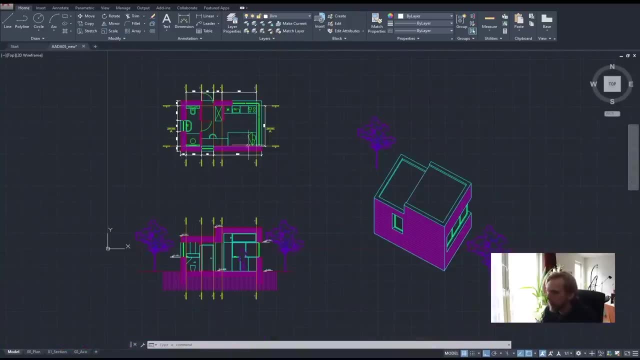 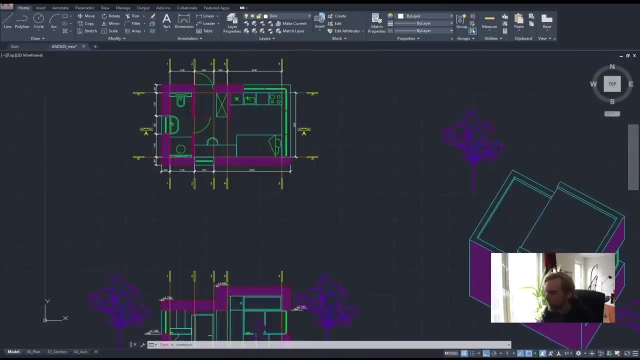 To this hatch Right, So it just kind of matches These two hatches together. Quite useful, Quite a useful little tool. No, We are not still plotting it out. I haven't told you about the. I haven't done one last thing. 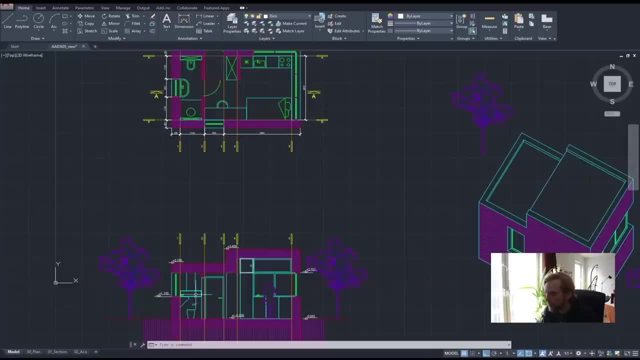 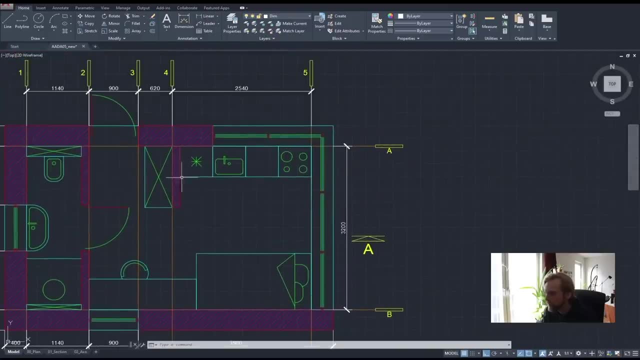 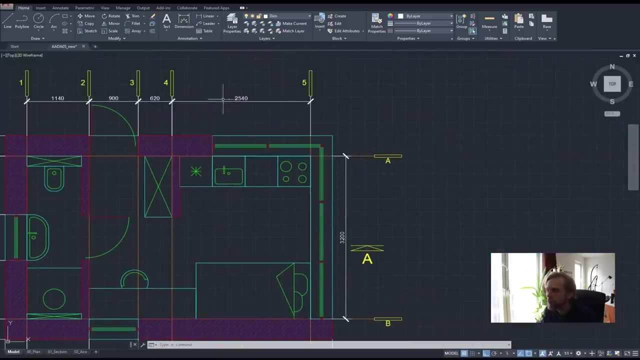 Which is adding dashed lines Here. we won't have any dashed lines, Will we? No, Almost nothing is above, But here, Here we will have a dashed line, Because there is like a cupboard above And that cupboard is going to be. 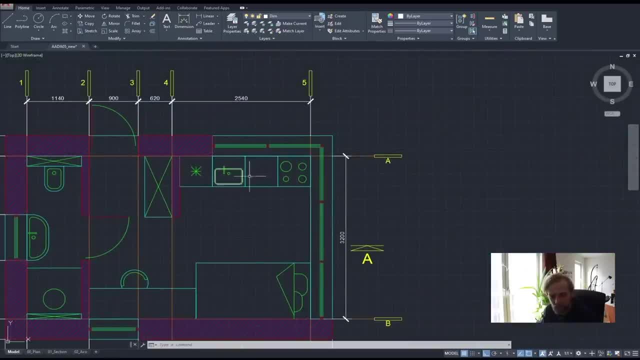 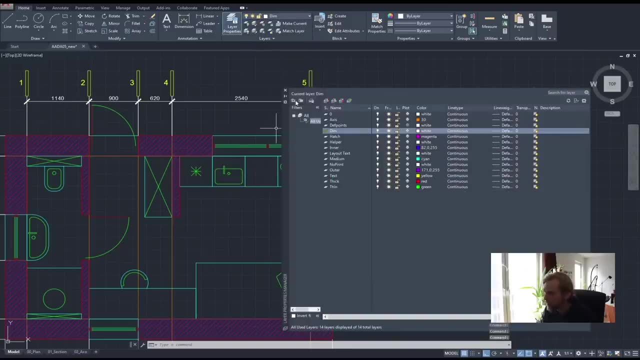 A little bit thinner Than the, Than the block Here. So I'm going to Create a new layer And I'll change to dashed. So this layer Will have all of the dashed lines And I'll change the dashed lines color. 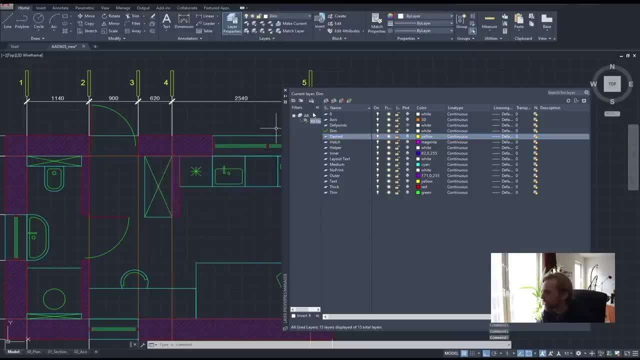 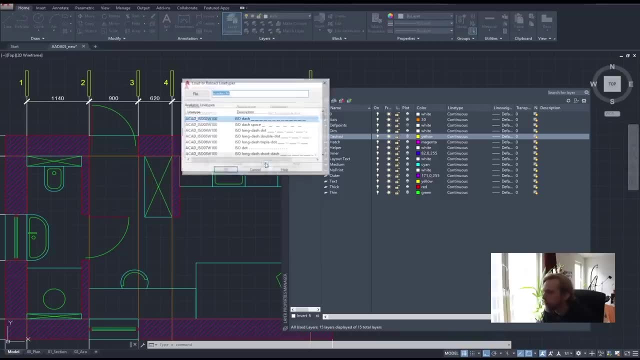 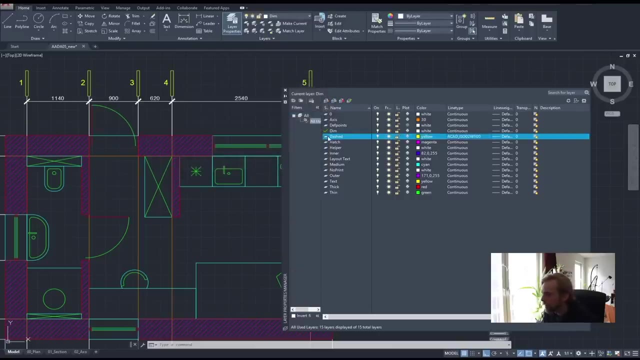 To also yellow. Let's go for yellow. That's fine, And in the line type I will change. Actually, I will change it here in the line type. I will change it to Load it And I'll change it to just. 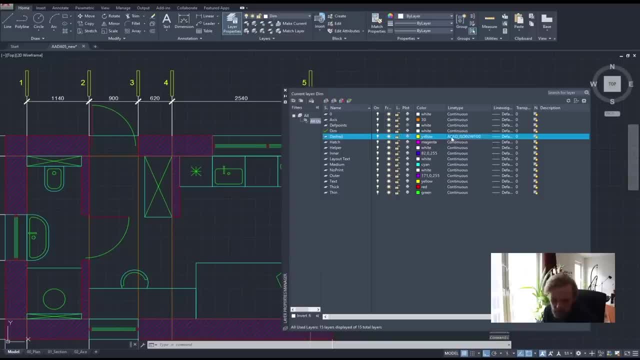 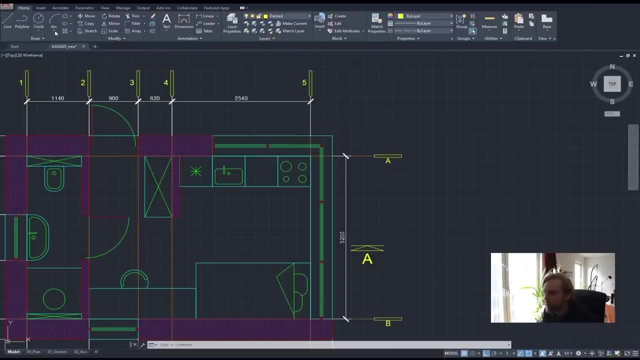 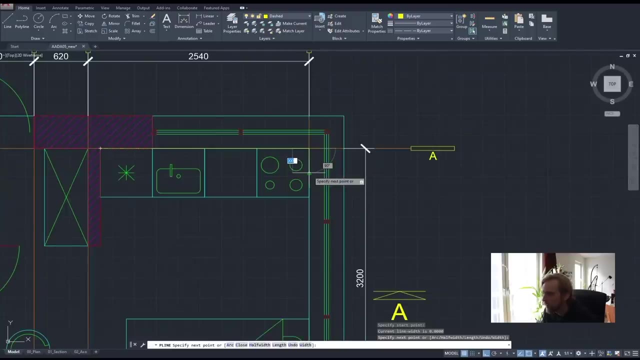 Iso dash, Okay, Choose it. Okay. And now we have a dashed layer That's yellow And I'll change it to All line here. That's going to go all the way to Here, And we'll- Actually we can kind of do this. 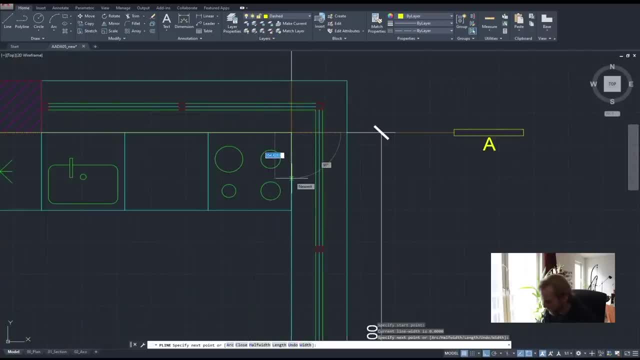 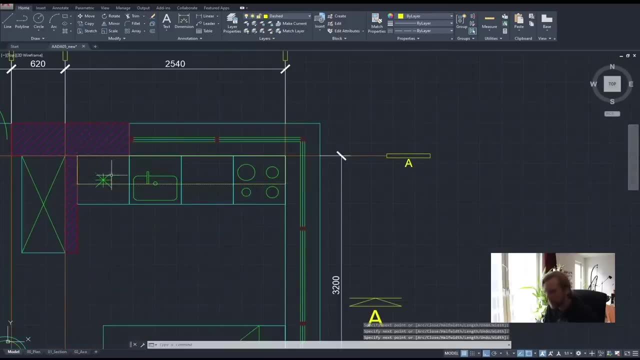 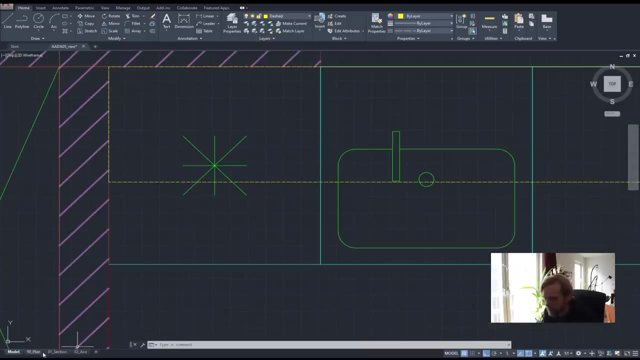 That would look pretty cool. Now Let's stick to it. 350, let's say Like that That. So this is basically a cupboard above And you can see it's dashed, But the dash is very, very thin. It's actually so thin. 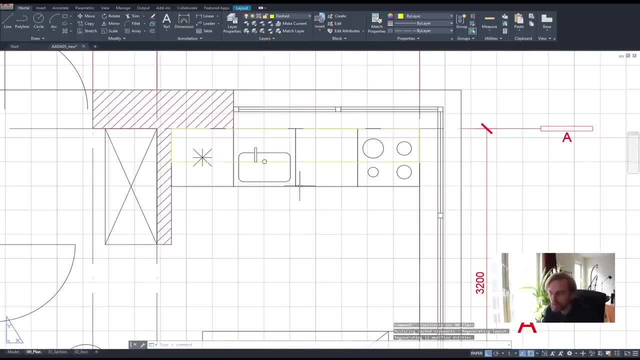 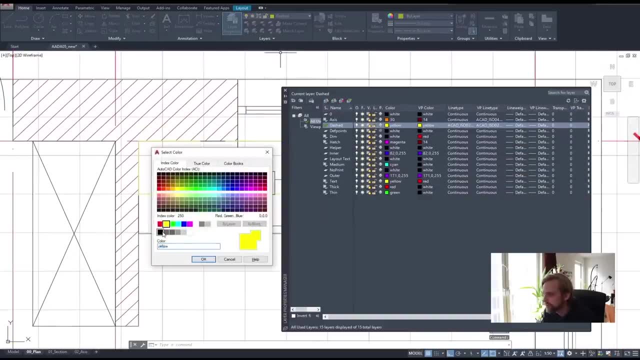 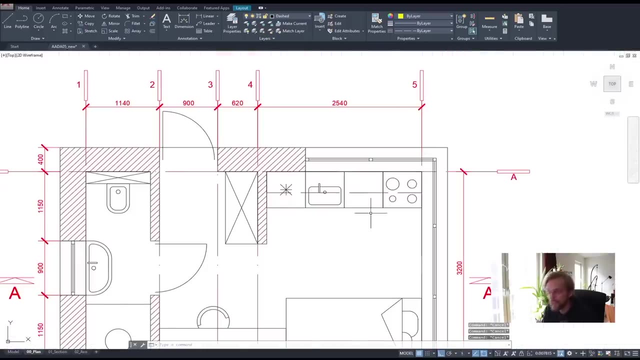 In the plan here And it's not Right. That's because, Well, you don't really see it do. It's super yellow, So let me change the color of it to black. There we go, So it is dashed here. 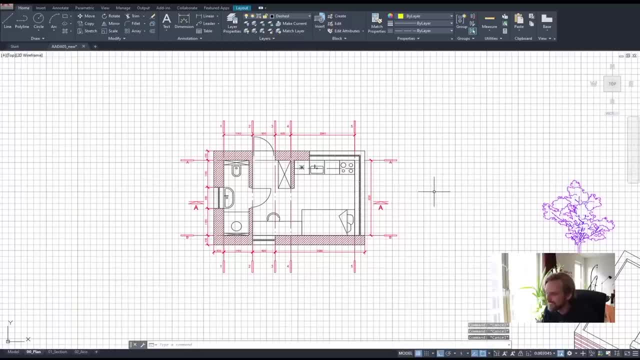 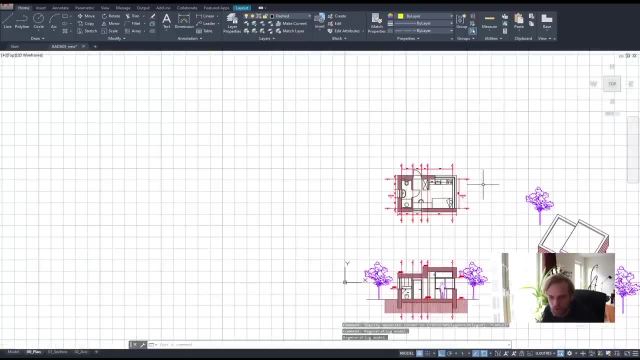 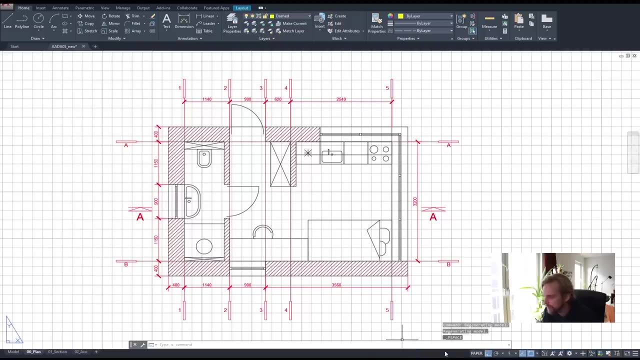 Right, Oh, I messed it up. By the way, If you can't zoom out Of the model space As you're in the viewport, You can always click here. Where it says model, You can click on it And then you are going to be in the paper space. 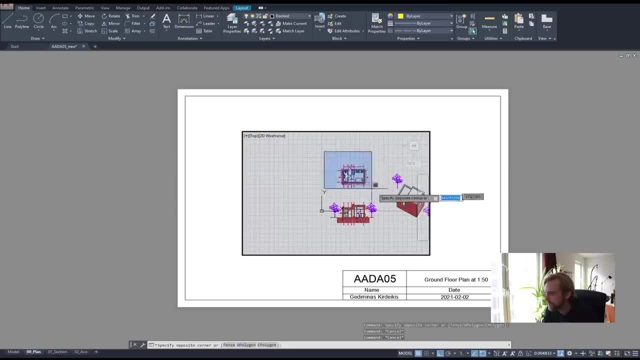 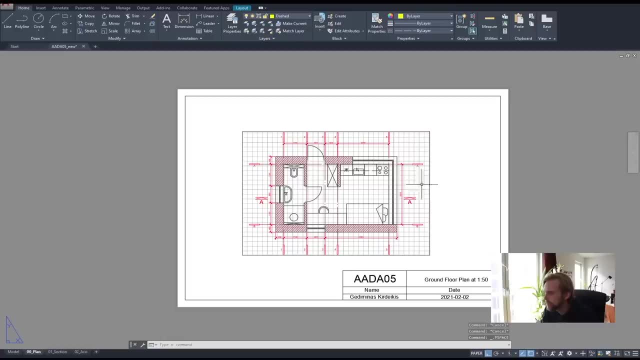 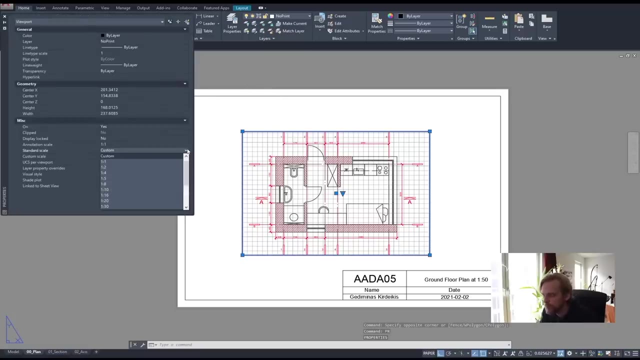 Right, So you don't necessarily need to click out. So let me fix this again. Come on, Z enter, O enter, Double click out. Select this Properties. Keep messing it up. 1,, 2,, 50. That. 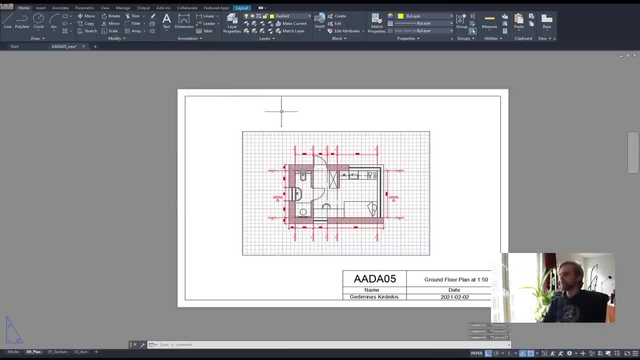 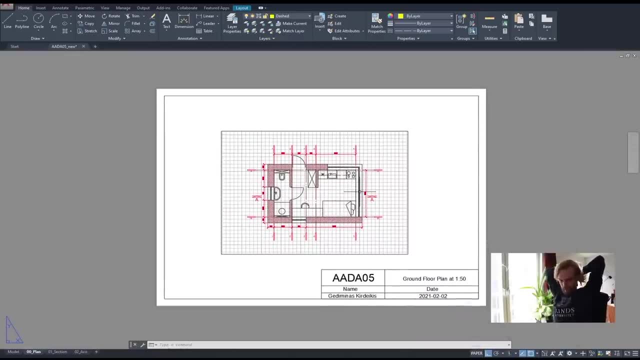 That's done, Okay, So now that's a dashed line, right there, Whew. Last thing: Thicknesses. Right, Everything right now is the same thickness. We don't want that. We want the thicknesses to be different, And I will use global values. 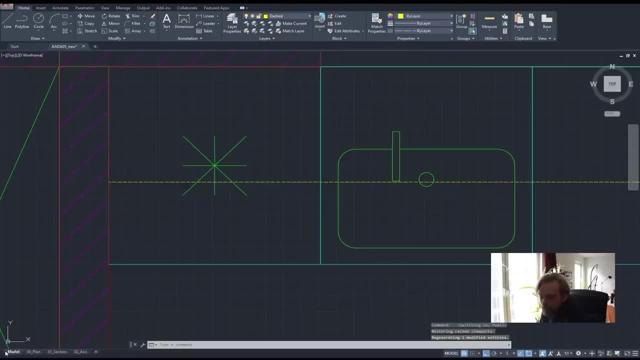 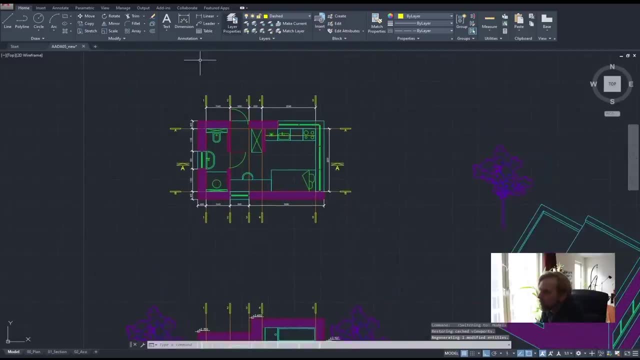 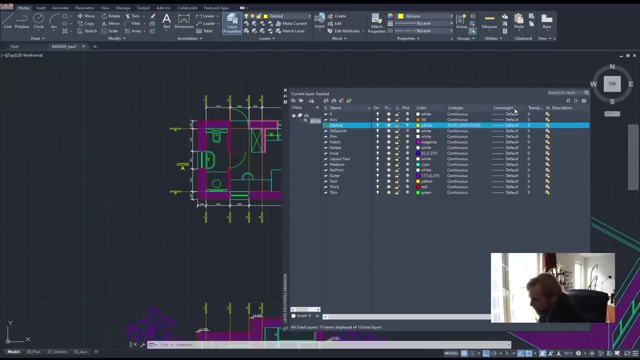 Rather than local values For thicknesses In the model space, Rather than individually Or separately in every layout. So I'll go to the layer properties Tab here. And thicknesses are controlled through Line widths, So The thinnest line that you can have. Which still Prints out by most of the Plotters Is 0.09 mm. Anything Thinner than that. Some older printers Will have problems with it, And by older I mean Printers that are used a lot. 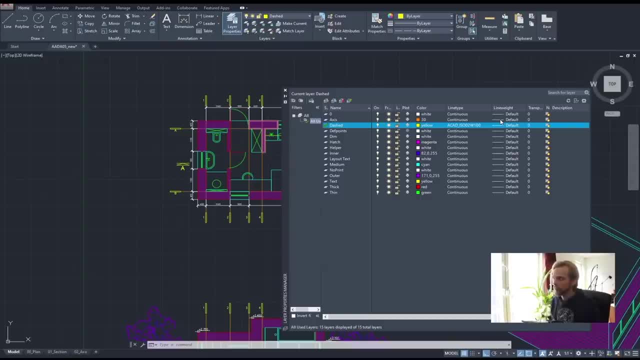 So in the school, for instance, Anything lower than 0.09.. Will not print out that well. When I say 0.09. I mean 0.09 mm. So those will not print out that well. So instead We are going to. 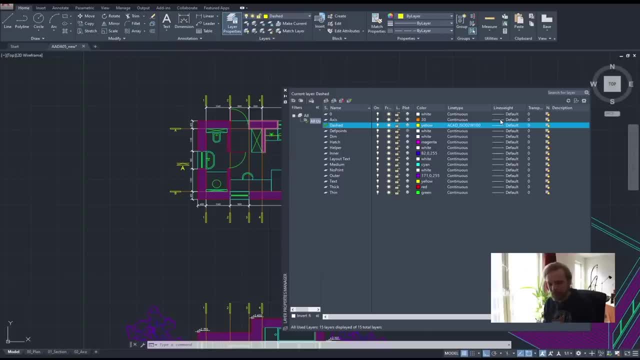 Lock our smallest Thickness of the line To 0.09.. And then everything Besides that Will keep increasing In thickness. In regards to that, There is something else That I wanted to mention. Alright, If you are printing with white lines, 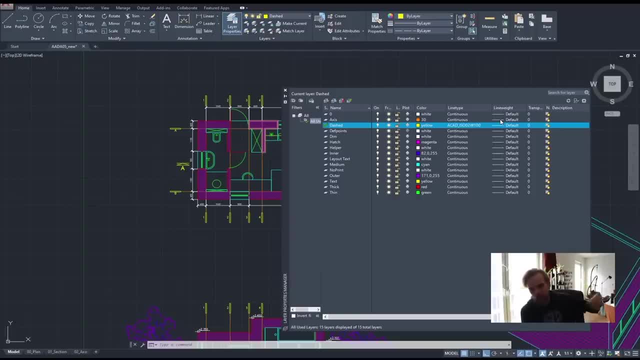 Above Black background, So white on black. The thickness of the lines Needs to be a little bit thicker Because there is A little bit of color bleed, Of the black color. So If your lines are too thin They will get eaten up. 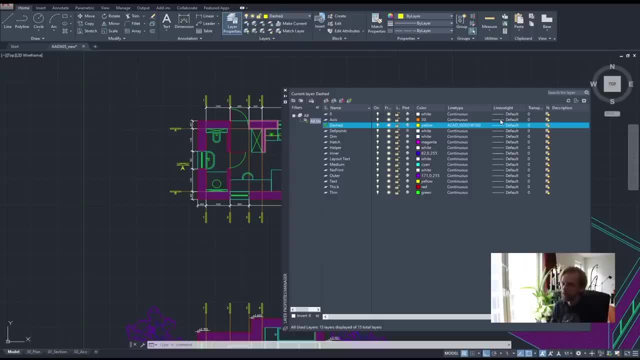 So if you are printing with white on black, I would suggest Smallest line thickness To be 0.12 mm Rather than 0.09.. So here With the line weights, Let's go to town with them, So axes. 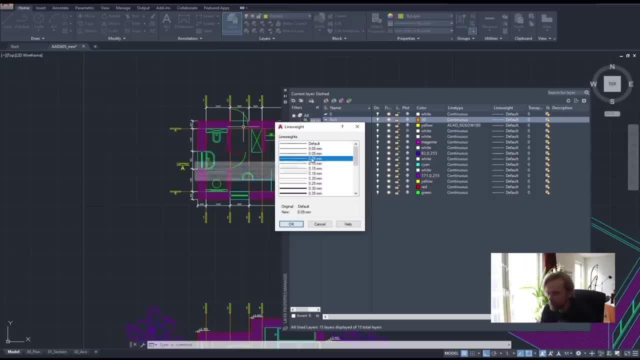 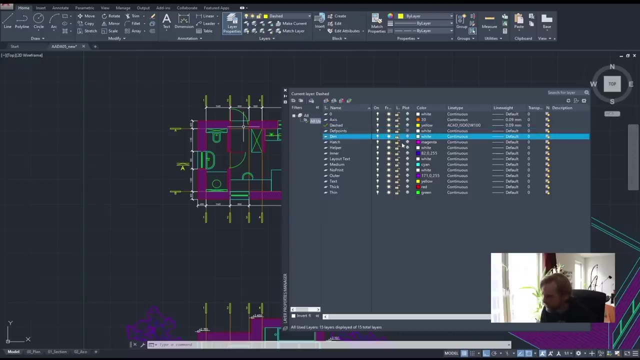 Axes are usually very thin, So I will use 0.09.. On them, Dashed line Is also a thin one. I will use 0.09.. Definition points: I have no idea what those are. We ignore them. 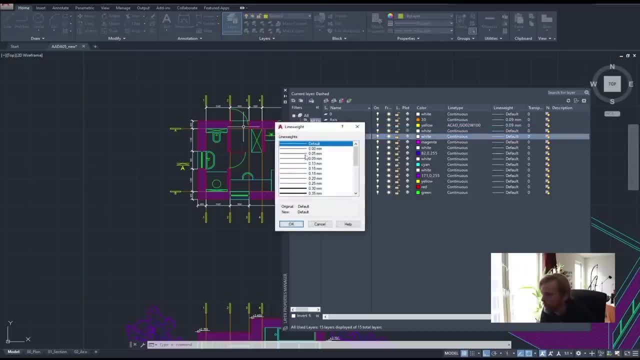 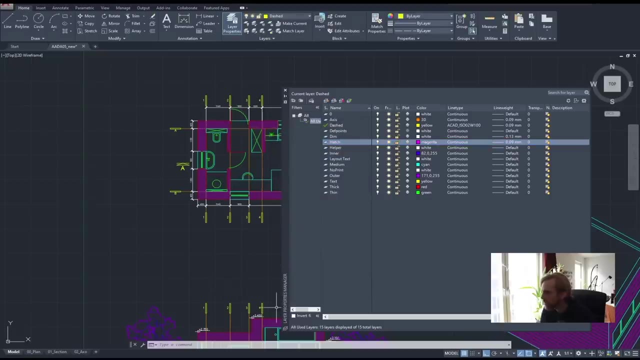 Dimension. Dimension lines are usually a little bit thicker, So I will use 0.13.. Hatch Depends on your style, But I prefer using very thin lines: 0.09.. Helper- We are not using helper layer. We are not printing with the helper layer. 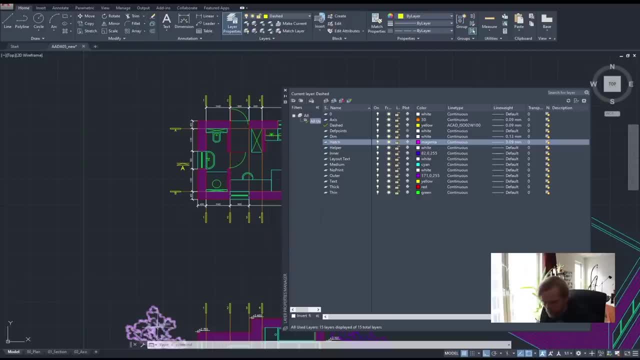 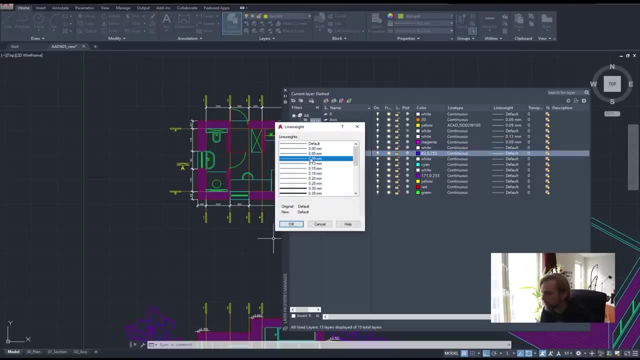 So we don't care. Inner, That's inner lines for the trees. Those can be super thin, 0.09.. Then we have layout text That can be A little bit thicker: 0.15.. Medium Line thickness needs to be. 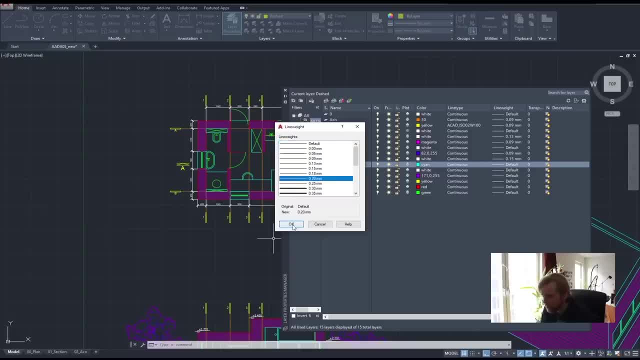 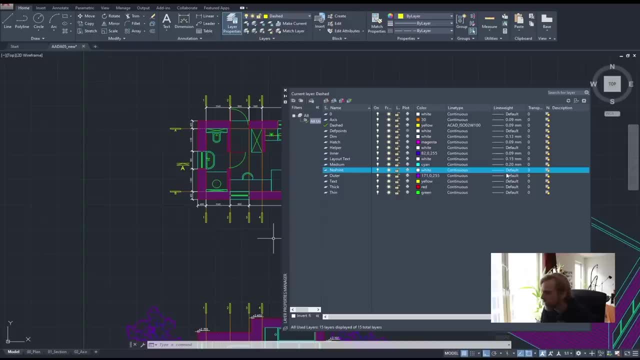 Thicker than all of these, So I will choose 0.2.. No print: That's important. Remember we created the no print layer That one shouldn't be printed, So we control it through the line weights We scroll down. 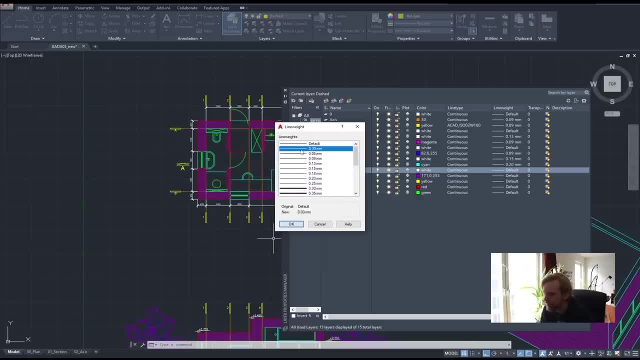 We don't scroll down, We scroll up And we see 0.00.. Basically, lines that don't have any thickness, So no print Will have 0.00.. Outer line For these things Will probably be medium, Same as medium. 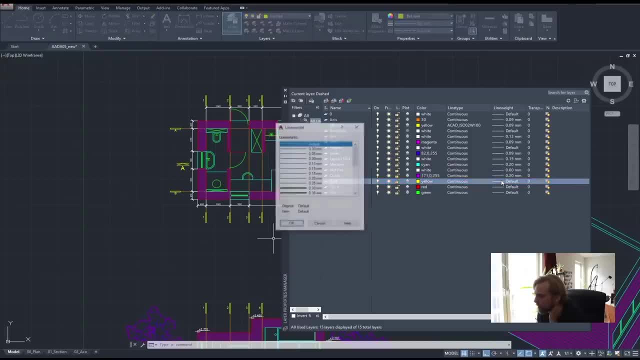 So I will use 0.2.. Text Text can be Somewhere in between Something close to dimensions. So dimensions are 0.13.. So let's use 0.13.. For the text Thick lines, I will go for 0.4.. 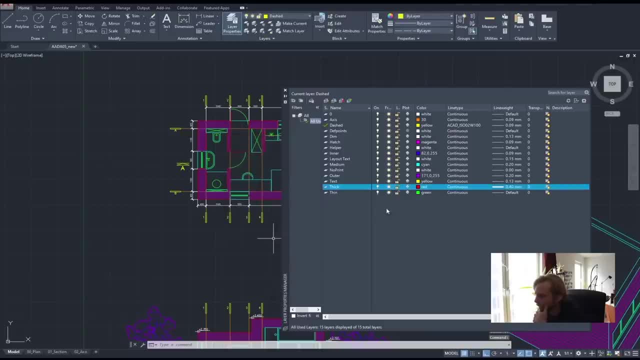 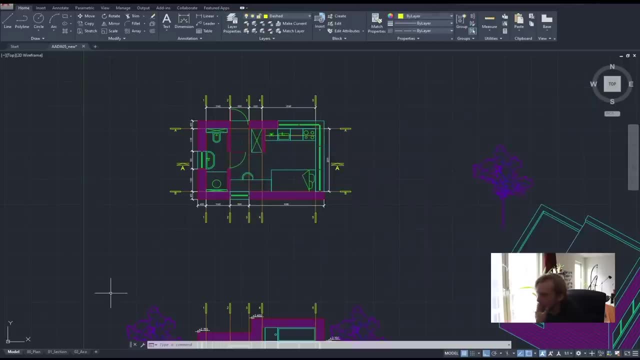 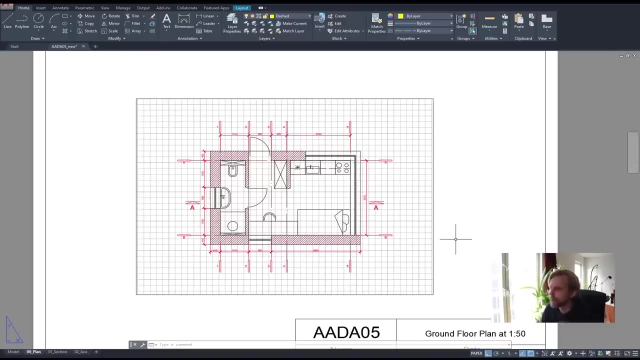 So double the thickness Of the outer lines, And thin lines are, of course, 0.09.. Yeah, Let's see. Let's take a look. You can't really see it here. We need to start plotting it out For you to actually. 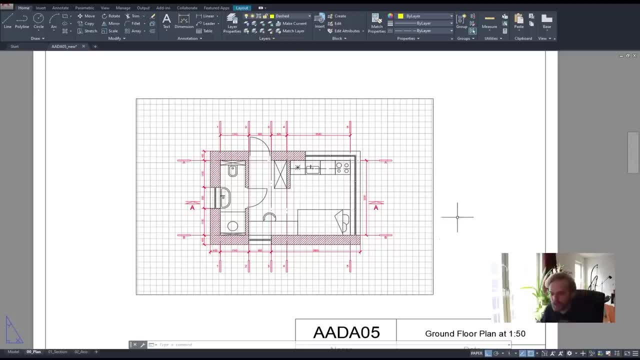 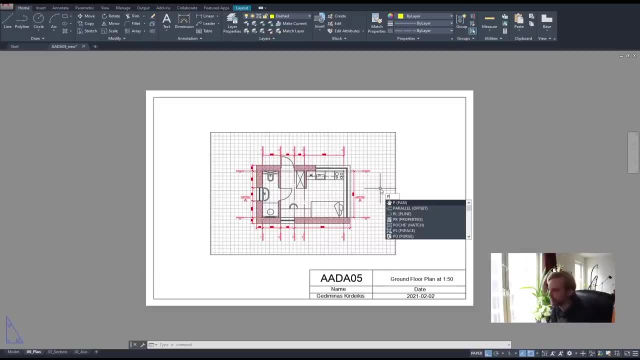 For you to actually see it. So let's plot everything out. Shortcut for Plotting stuff out Or exporting PDFs Is P. No, I lied, It's not P, Just write plot, I guess. Plot Enter. 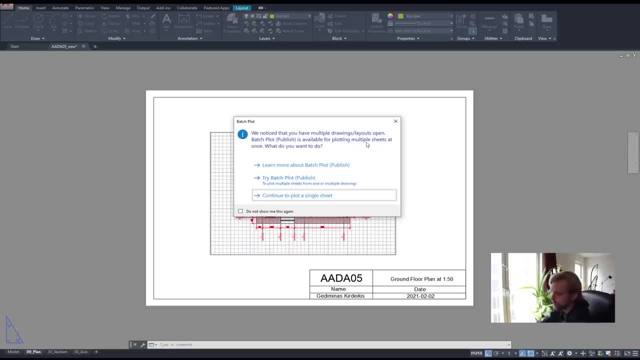 It will ask you for this. We noticed that you have multiple drawings. It's available for plotting multiple sheets At once. What you want to do Is to plot them At once, Or you can plot them out one by one For this particular purpose. 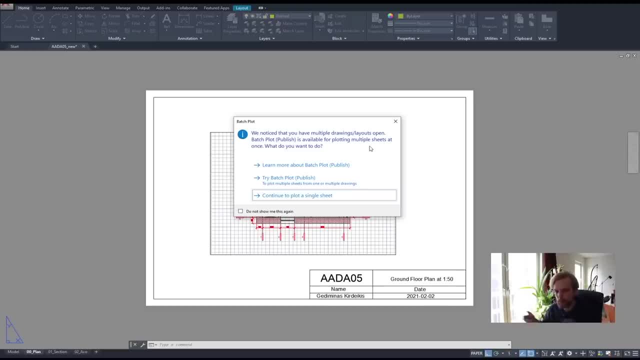 I will be plotting them out one by one Just so that I can show you How you can combine them with the Online tools Into one PDF. So I will say: continue to plot a single sheet, But you can use Try batch plot. 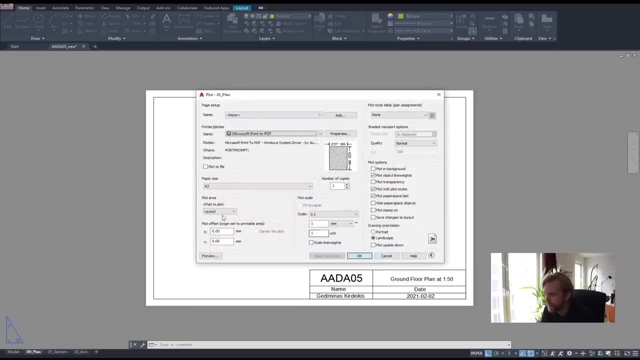 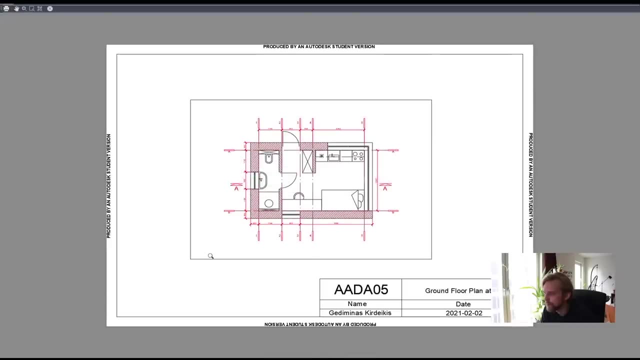 You can use that as well. So I'll continue This plot settings again, And I can actually click on Preview here To see How it's going to look like. Produced by Autodesk student version. Great, So That's education version. 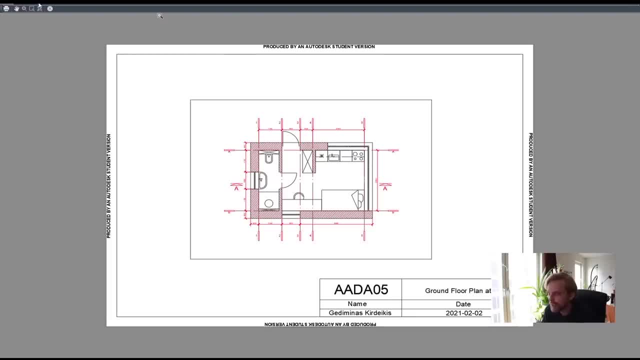 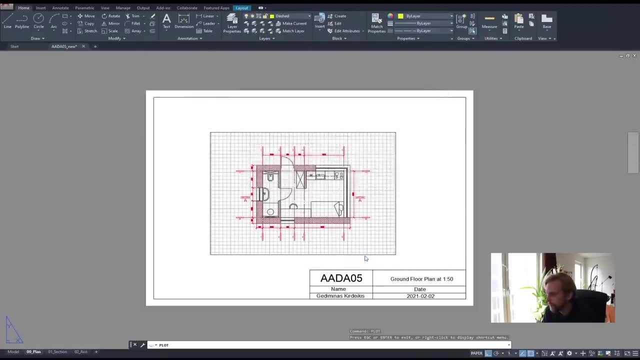 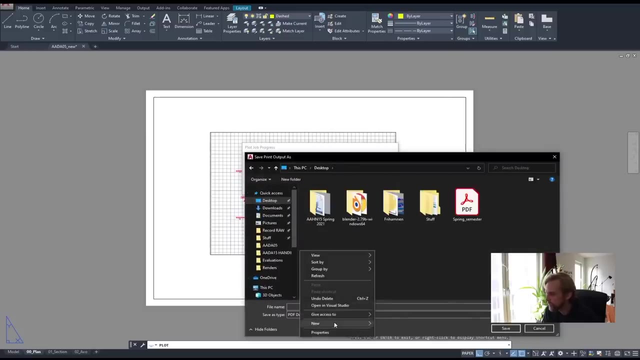 Right there. So we are going to be plotting out this Right. I just Click the close button. Okay, And I'll just plot it to My desktop. Let me just create a new folder here. I'll just call it. 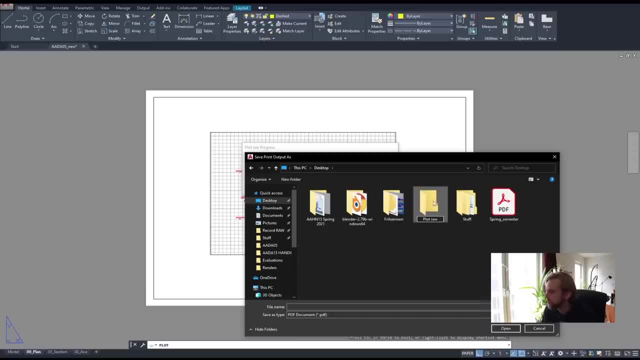 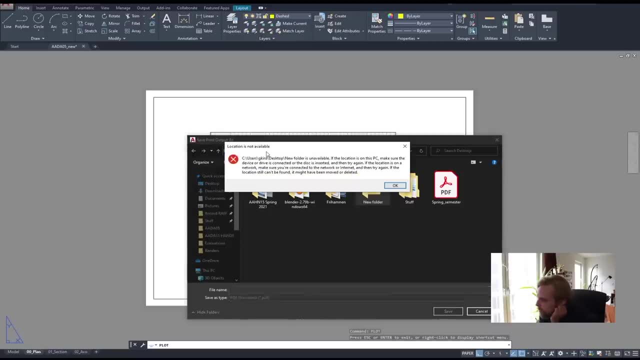 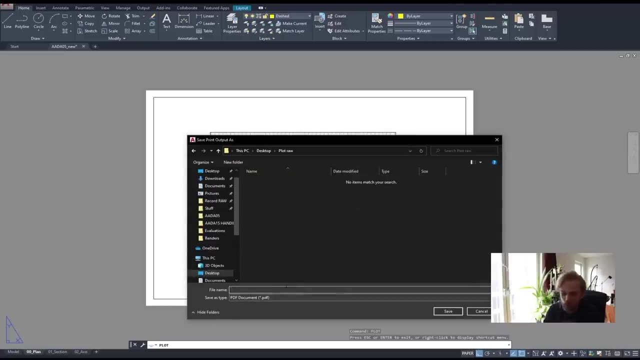 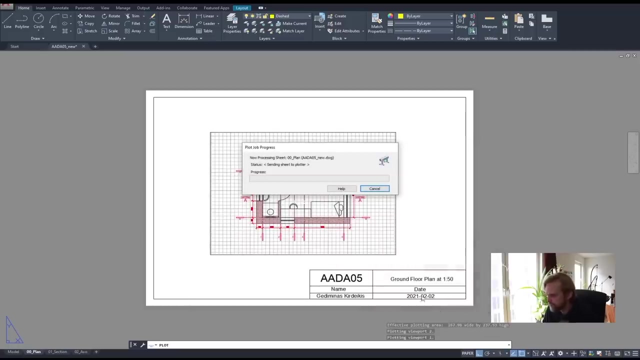 Plot raw, Plot raw. Why are you crashing Again? Location is not available. It is, It's right here. Sure, I'll call it. We are plotting out the plan, So I'll just call it Plan And it's done. 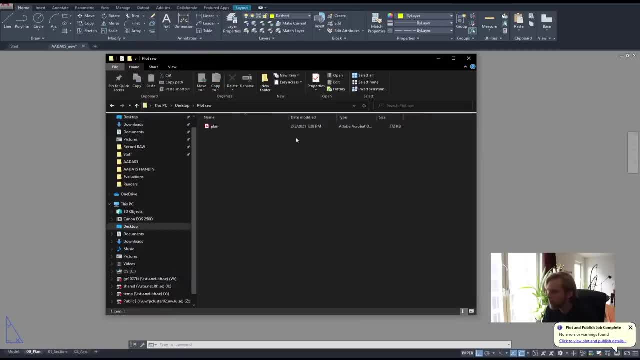 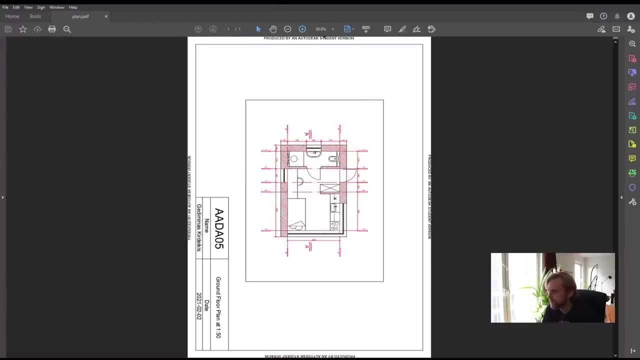 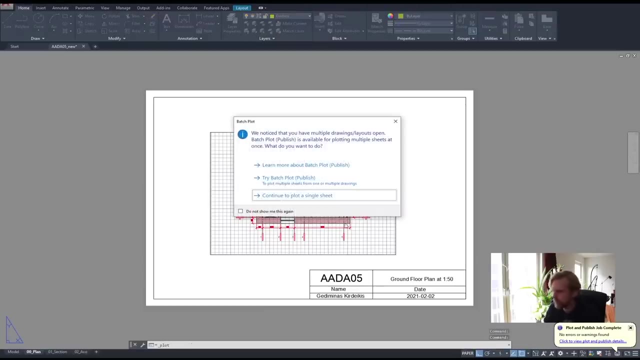 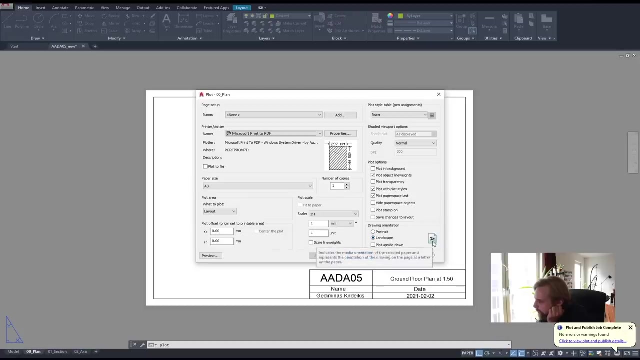 And I can kind of take a look at it Right here. Desktop Plot raw Plan. Double click that. For some reason rotated, That's whatever. Why is it rotated? Let's see Slasky format. That's fine. 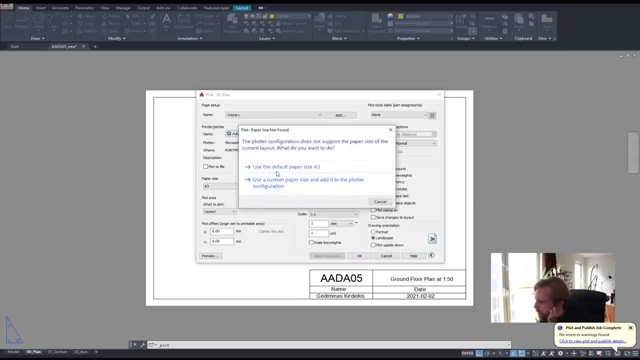 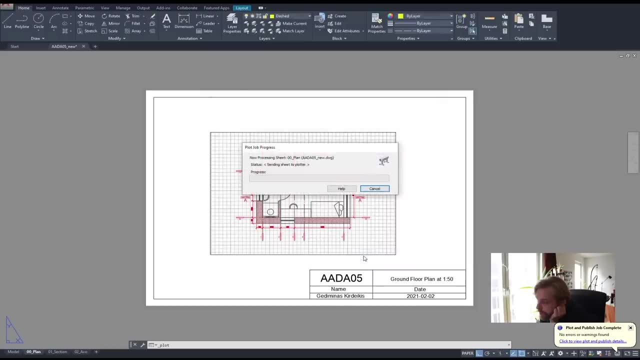 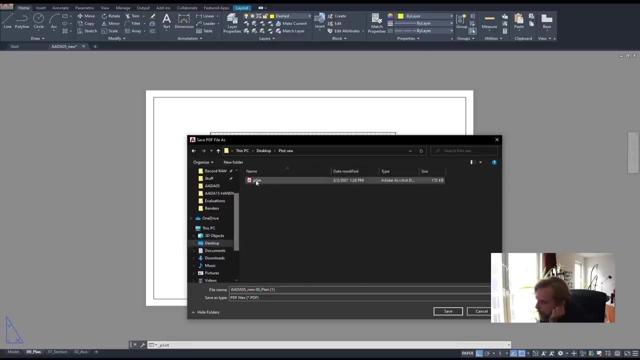 What if I use a different Plotting technique- Adobe PDF- And I plot it this way? I'm just kind of checking What works more stable at this point, So I'll overwrite it, And I need to close this To be able to overwrite it. 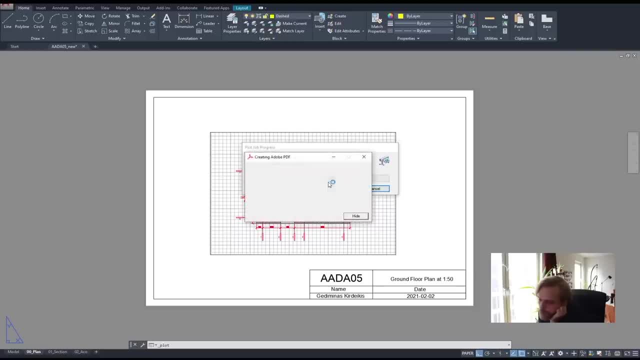 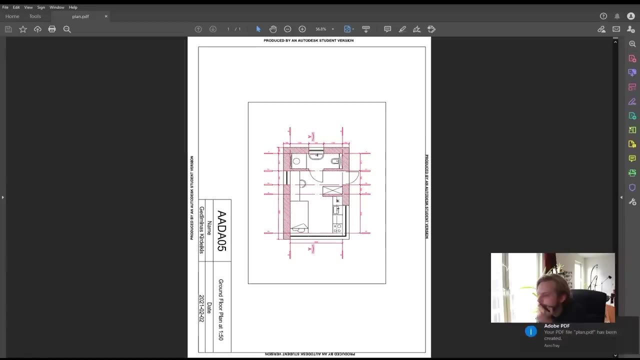 Let's see if Adobe PDF Will do us good. Definitely slower, Definitely slower. Come on, You can do it. It's not a big project. Oh my god man. Oh, there we go. It's also rotated, Okay, so that's weird. 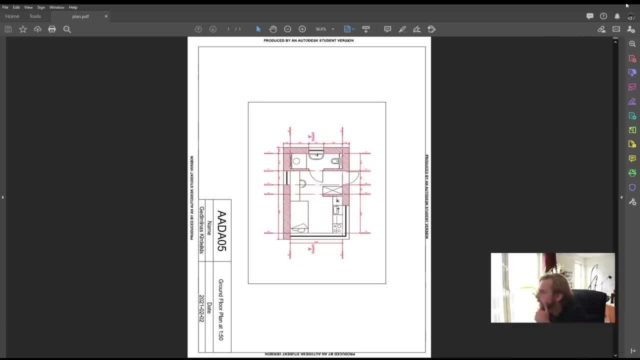 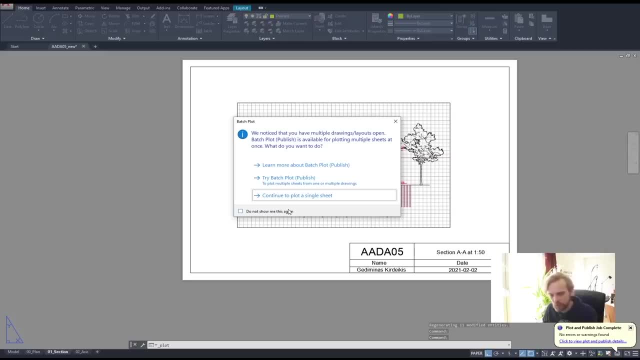 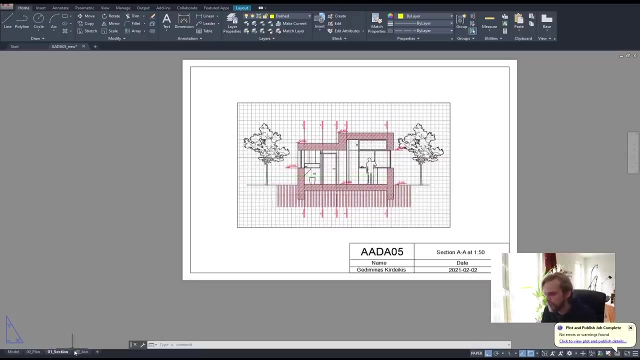 But that's fine, We can have it rotated, That's okay. So we have that. Then let's do the section. By the way, shortcuts Even faster shortcut is control P Continue Plot, That's section Save. And then for EXO. 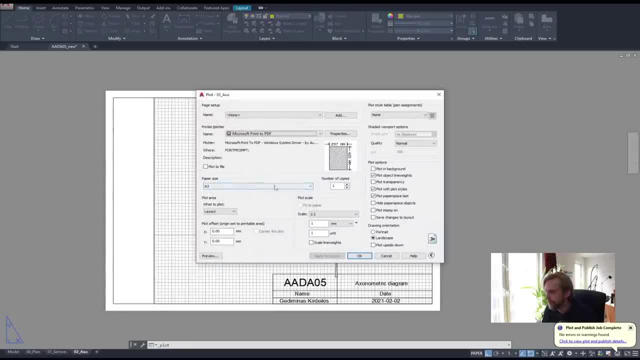 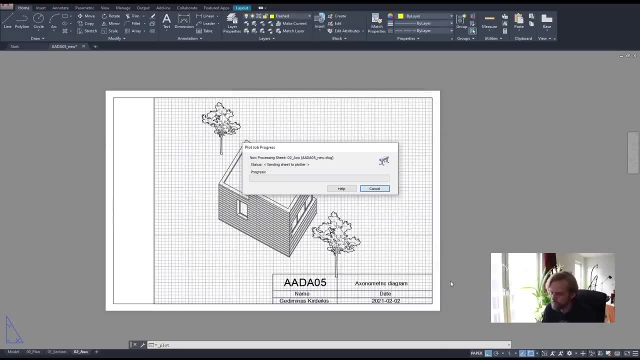 Control P, Plot A3.. EXO Save And of course you will have. You will have more. You will have the title page as well, But not. I'm curious to see What you'll come up with. I will not be showing you the title page. 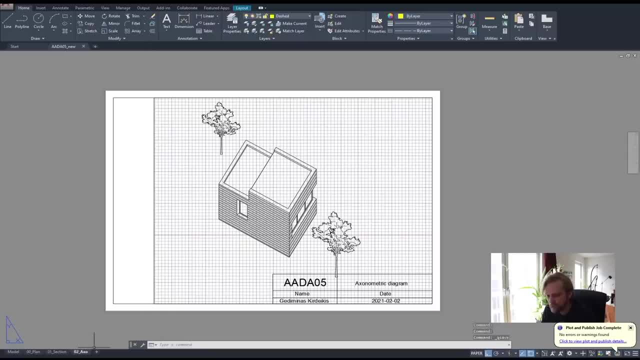 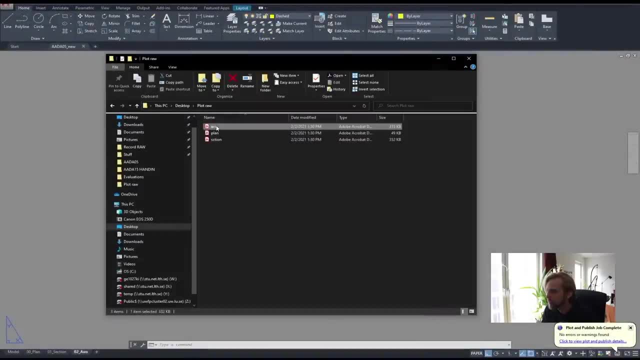 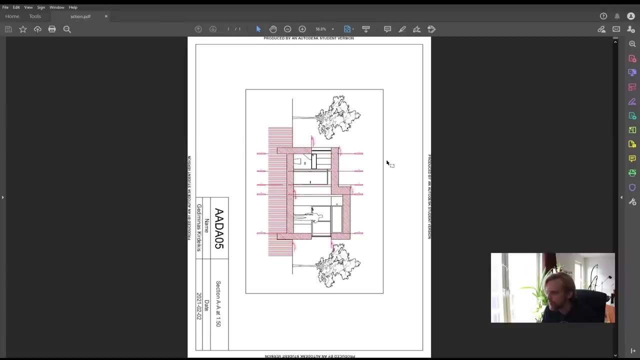 Let me just save this file, Just in case It crashes again. So we have these three, We have the plan Right here, We have the EXO Right here And we have the section Which I mispronounced Right here. 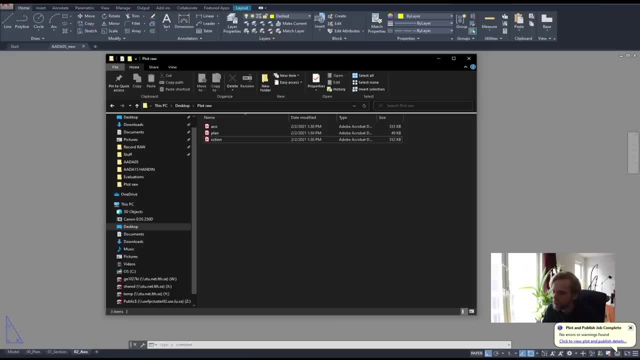 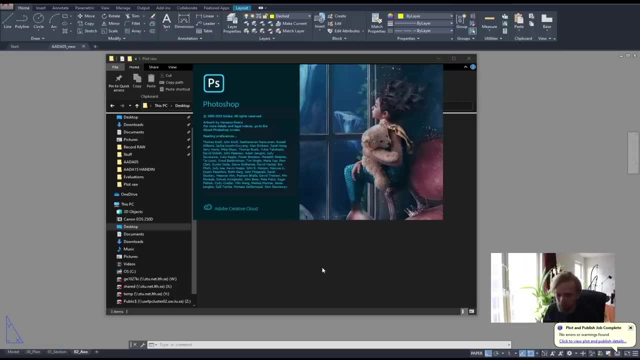 Everything seems to be in order, Even though it's a little bit messy. Then what you can do- honestly, I shouldn't probably be showing you this, But what you can do- is You can open them up in Photoshop, Just quickly, Really quickly. 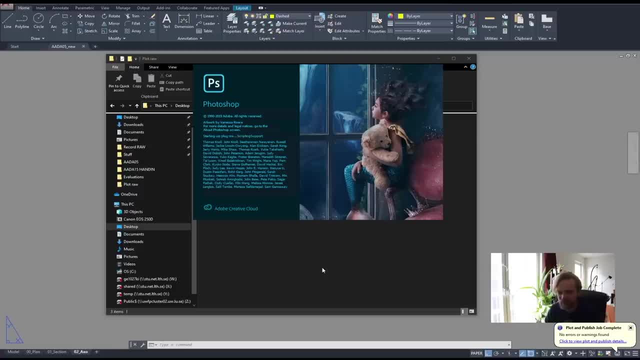 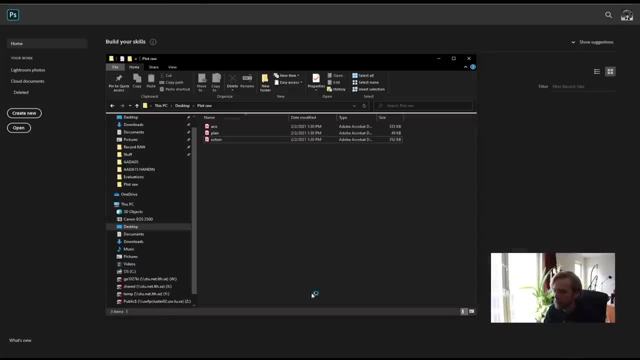 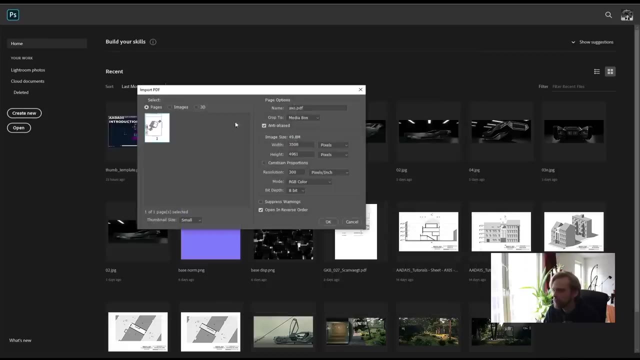 I'll show you How to kind of connect this to the previous Previous course That we had. So let's open up Photoshop. I'll just take All three of these, Drag and drop them in As copies And I will. 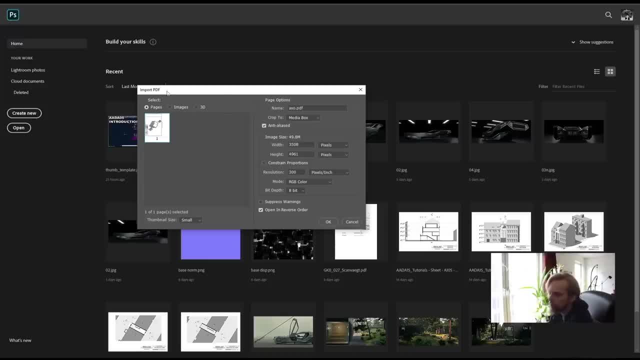 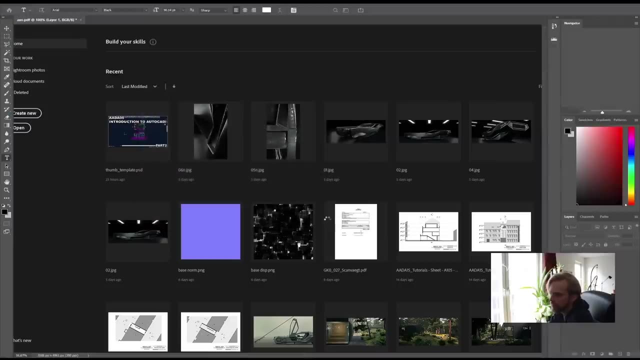 As I have Dropped them in. It's going to ask me How do I want to import this Very important to have media box Set as cropping Rather than bounding box? That's very important. Everything else is whatever Hit OK. 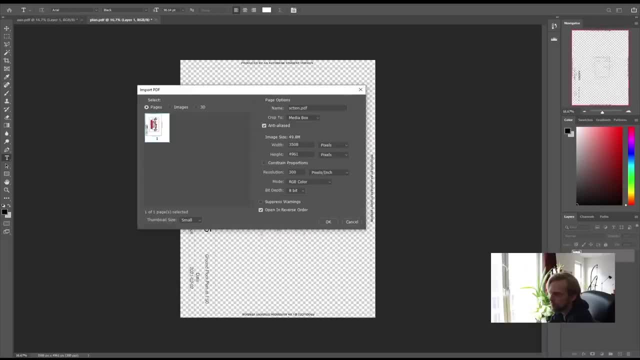 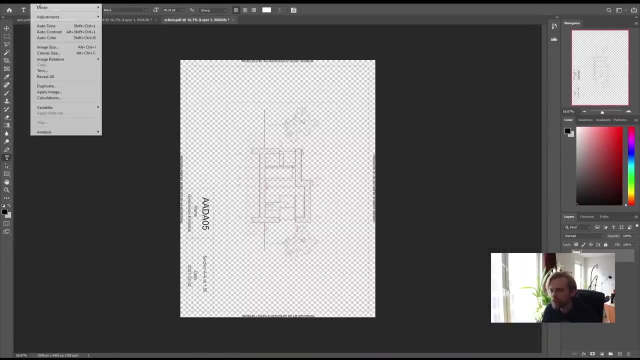 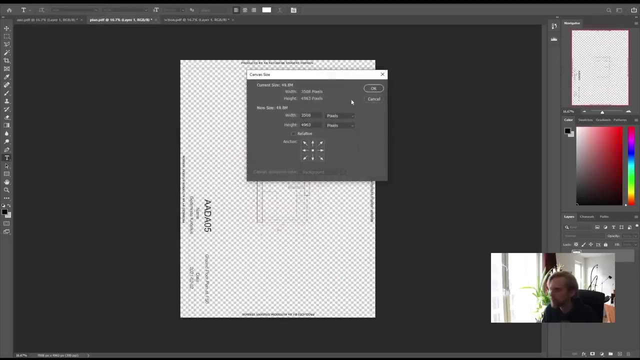 Then here media box OK, And here media box OK. So we have now them opened up in Photoshop. I can go to image Image rotation. Counterclockwise Image: Oops, That's kind of a size, That's bad. 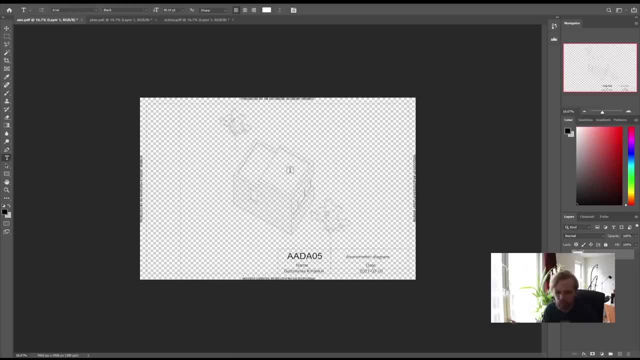 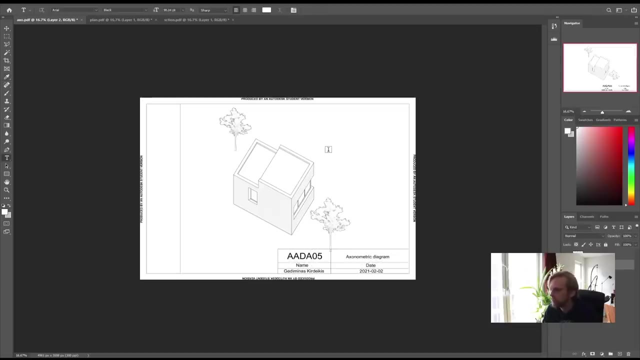 Image. Image rotation Counterclockwise, So I have them rotated back to normal orientation And I also can add: Like: create a new layer, Drag it below the existing layer. Grab the white color. Create a 5 to fill. 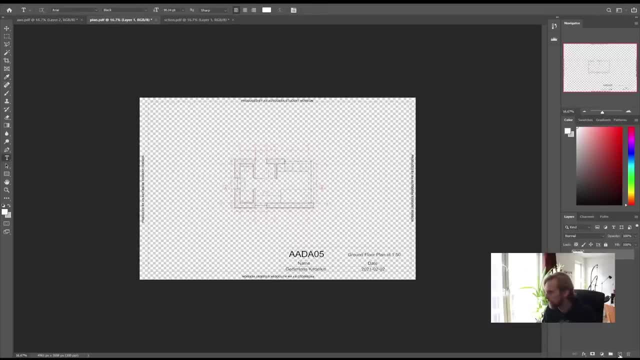 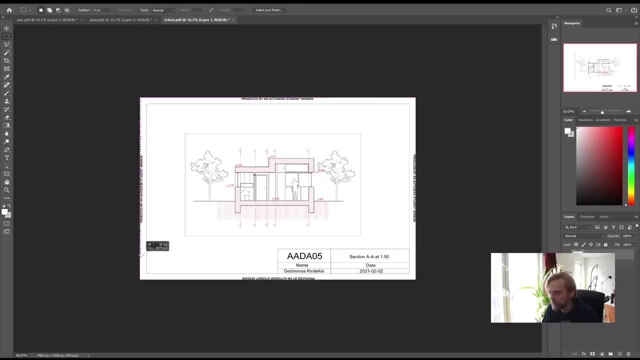 And basically just create White background. that way I'm going to do the same thing For all of them, Like that, Like that, And also I can, While I'm at it, I can come in here And I can kind of select the. 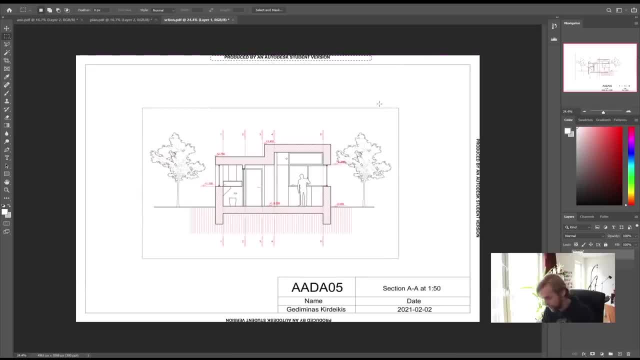 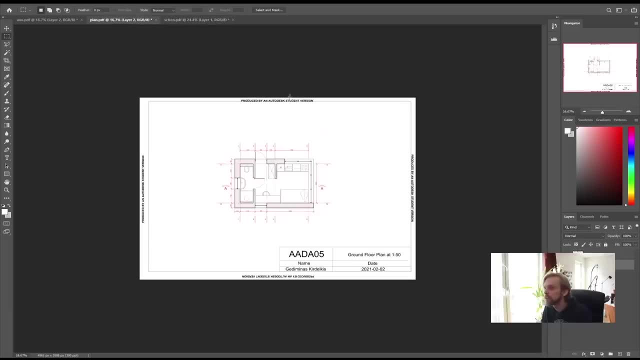 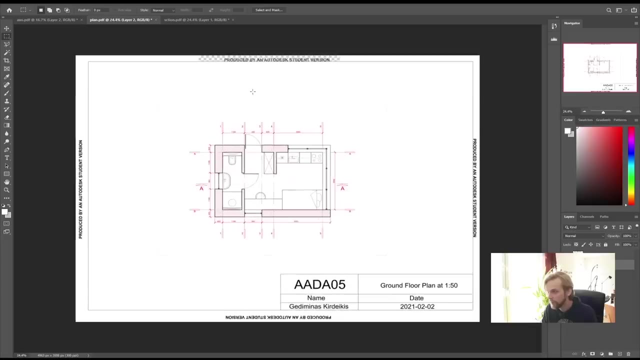 Autodesk student version. Then you just: No, no, no, no, This was done with a professional version, Alright. No, no, no, It's a normal professional version. Oops, Control D Or control Z. There we go. This one will need a little bit. 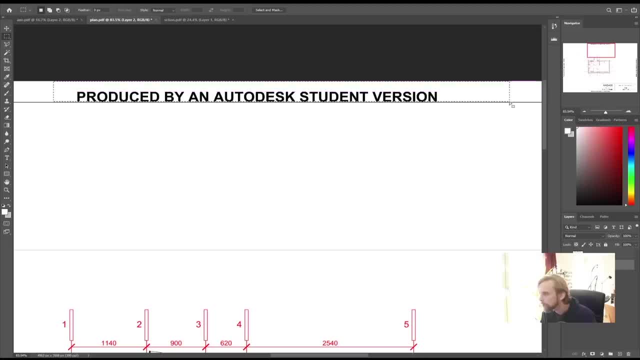 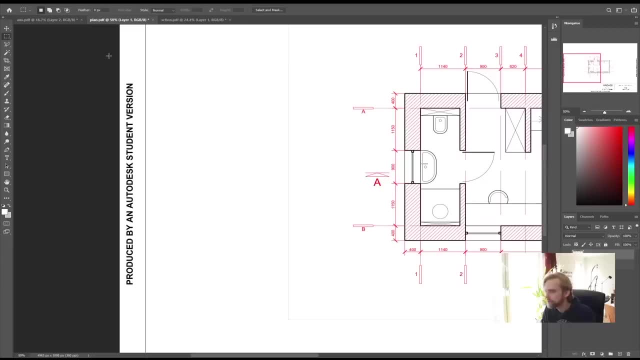 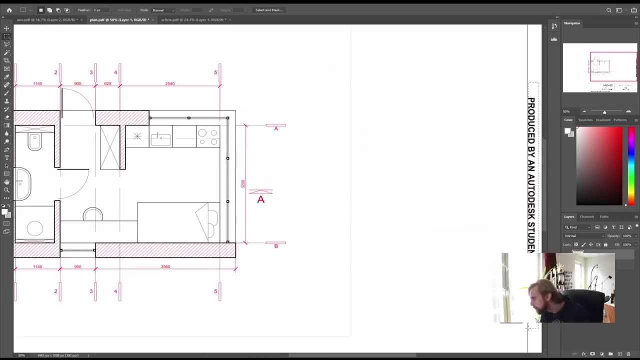 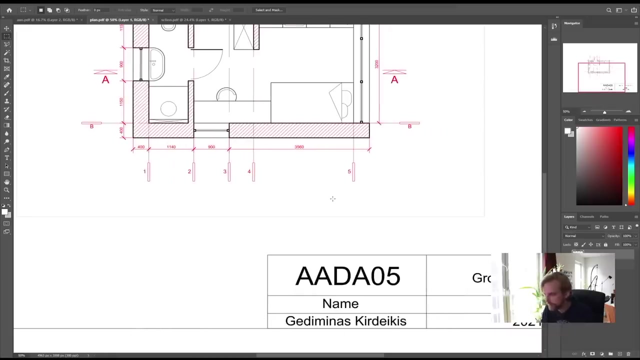 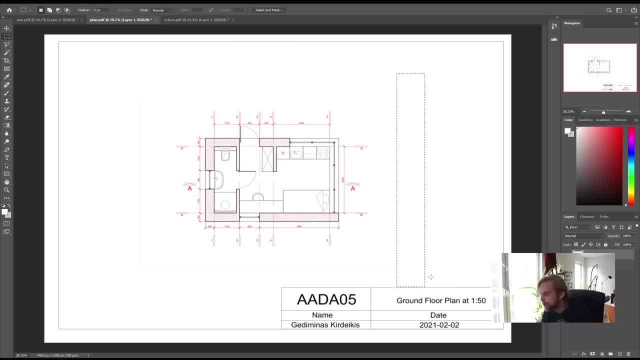 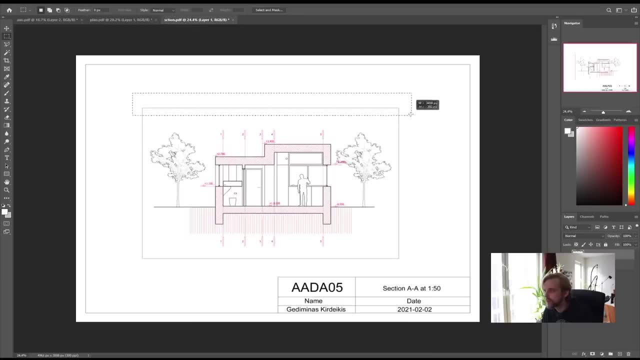 While I'm here, I can kind of- You can still see a little bit of the border. No, no, no, We delete the border. There we go. So I messed up a little bit there. Apparently, The regular plotting technique Still keeps. 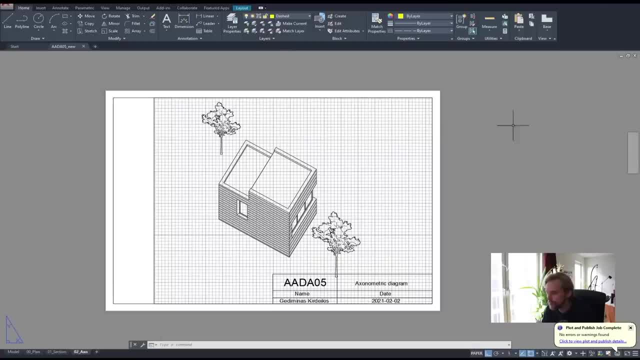 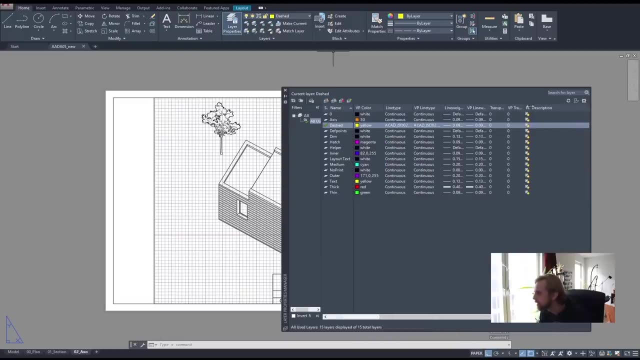 Like a tiny bit of the border. That's fine. There's also an option for you to Go in here. Where is it? Go in here? Select this object And I believe There needs to be. There needs to be like. 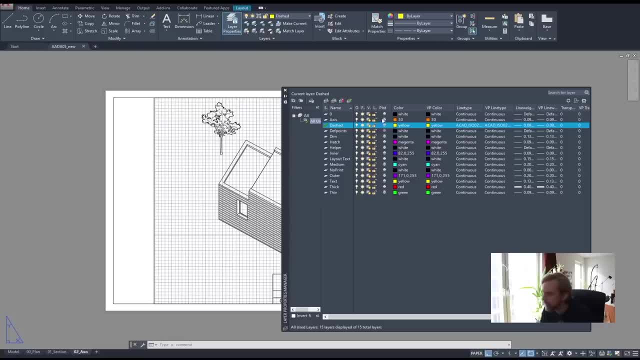 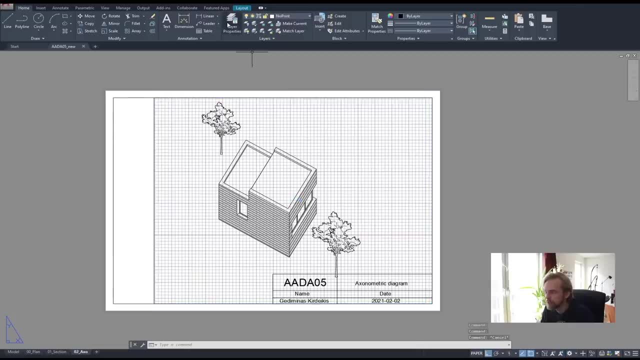 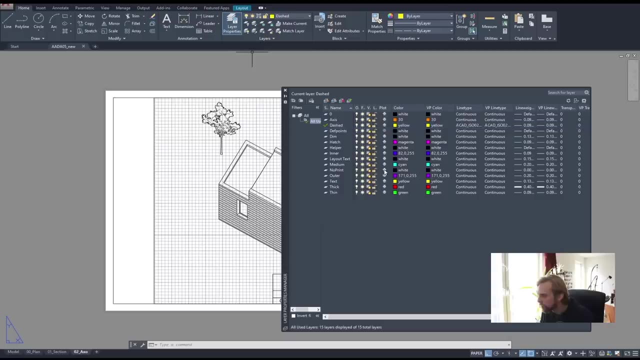 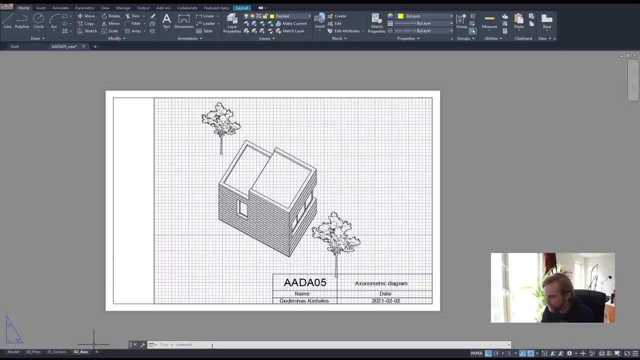 No print option here. Yeah, there we go. So there's also, like This whole segment here Where we can change The border, The no print layer, To be Actually No print Like. so That's something To know. 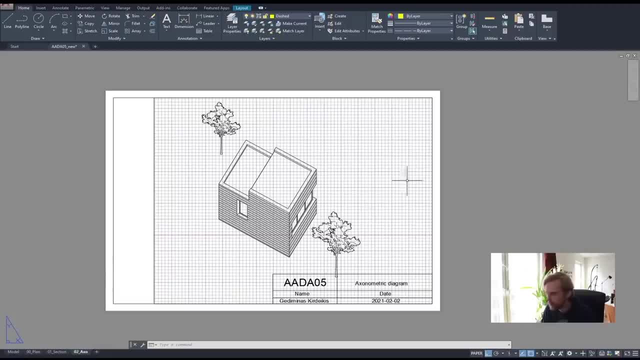 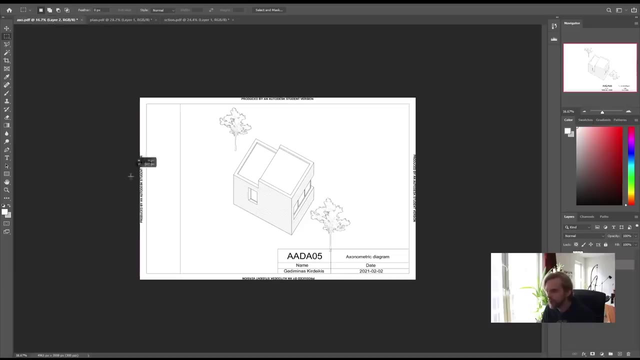 So it's either changing it to 0.000. Millimeters in thickness Or not printing it out altogether. Apparently, 0.000 doesn't always work, Which is news to me. It used to work. I feel old, Oh yeah. 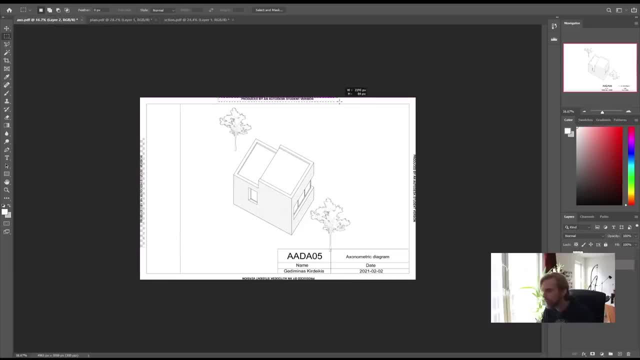 Axle. We need to clean up the axle, Delete that, Delete that I am deleting The wrong things, Or rather The wrong layer. There we go, There we go, There we go. And now Precision, Precision. 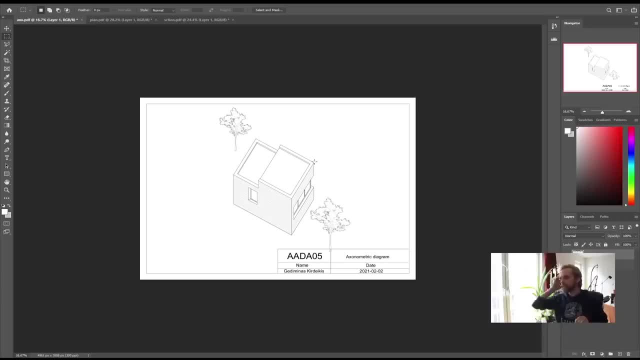 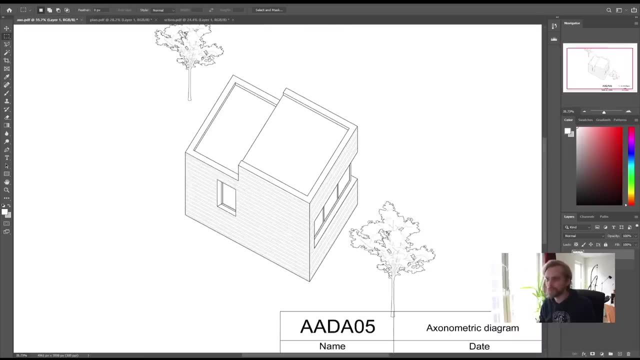 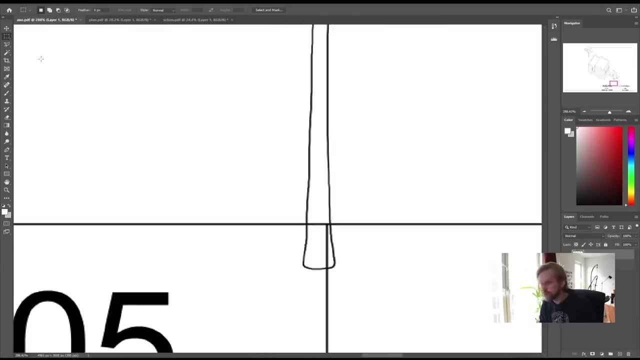 There we go. Good enough, Good enough. What else can we do with this? I don't really want to do anything more with this. You could, While you're in Photoshop, You could kind of add Color, texture Or what not, to it. 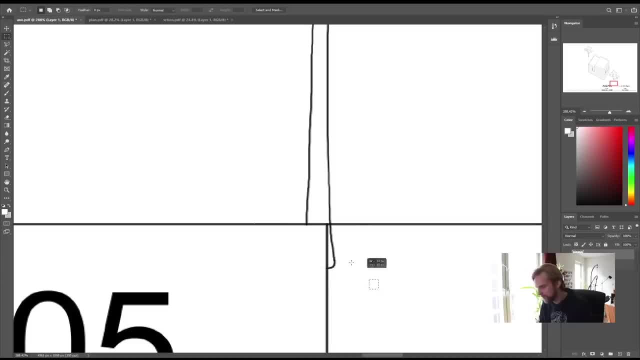 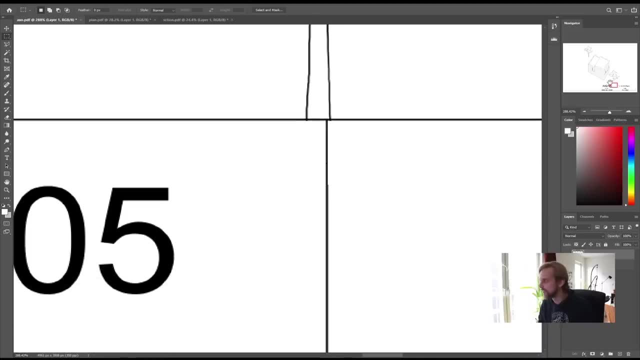 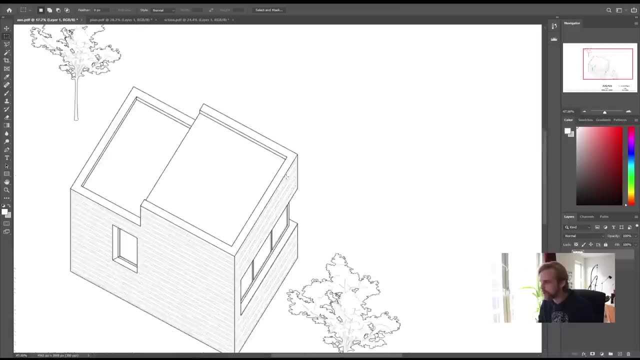 But I don't really want to do it. What I want to do is Clean this bad boy up. So this is actually. This shows very well The difference between Vector graphics And raster graphics. See how the lines are not infinite. 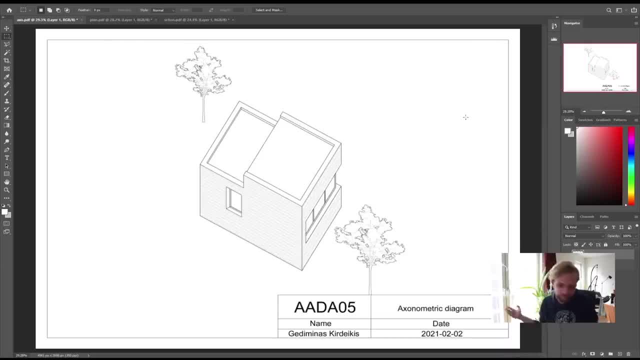 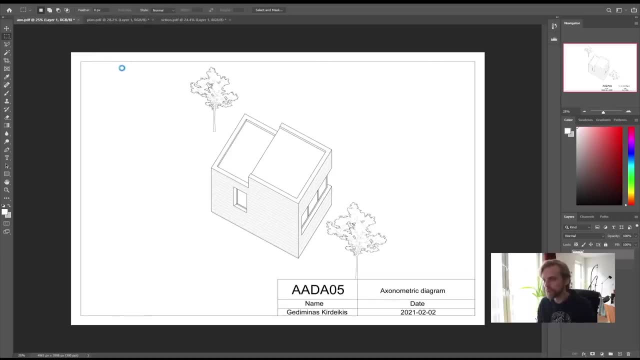 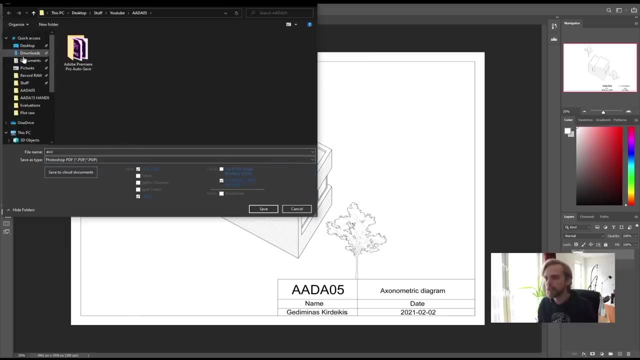 In resolution anymore With them in Photoshop Right, And Photoshop works with pixels, So these three are now cleaned up. I'll just save them. Just control S to save. Choose Photoshop PDF. I'll go to my desktop Plot raw. 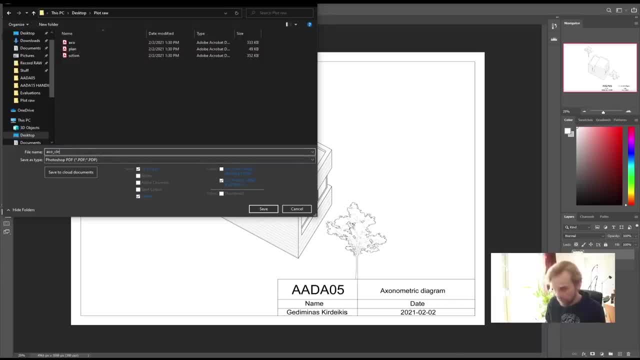 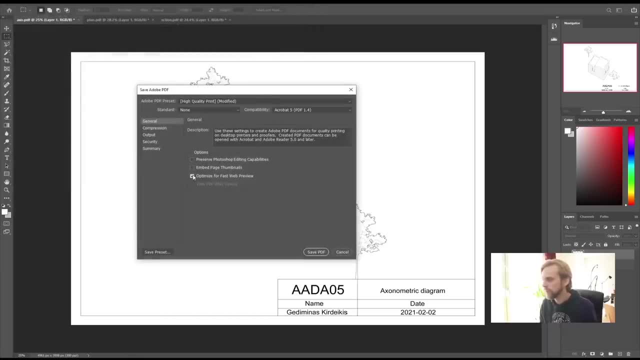 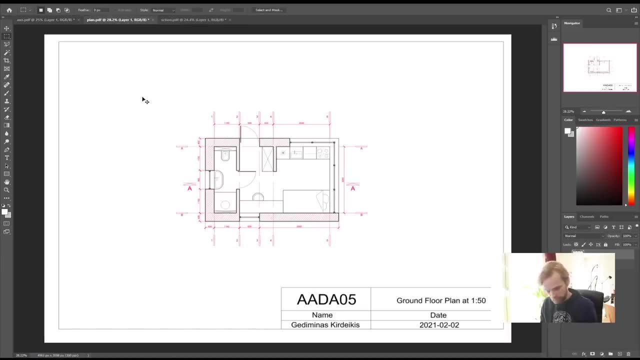 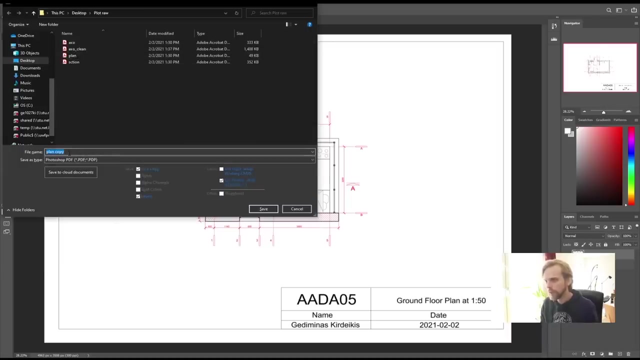 And I'll just kind of override them, Or let's just do Exo clean Like that. I will not be saving the layers. Hit OK, Everything else here is fine. Hit, save And same thing here. PDF Plan. 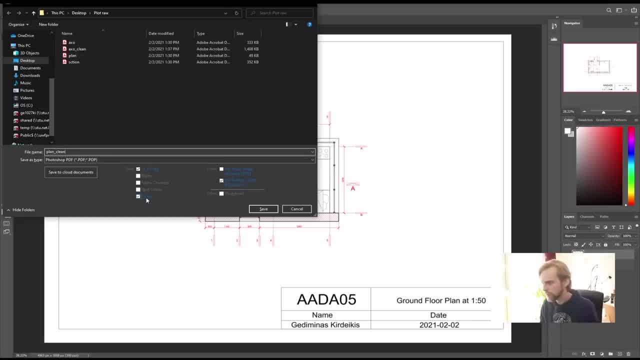 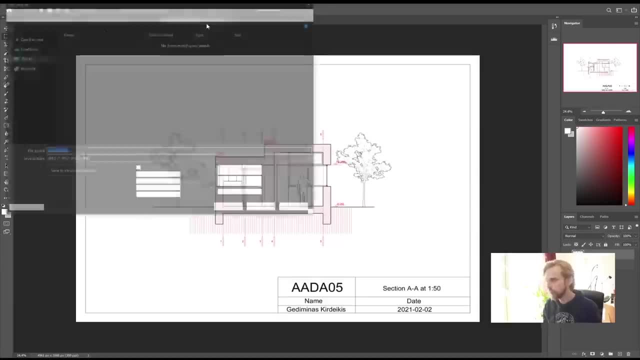 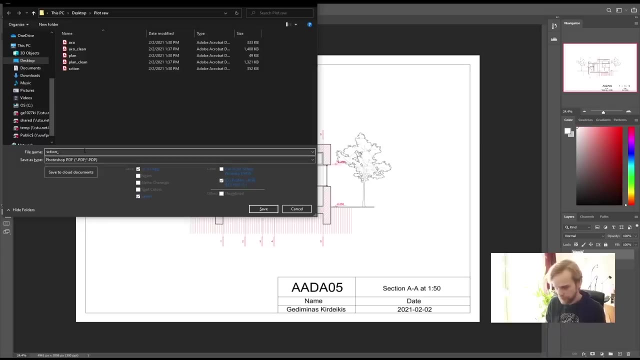 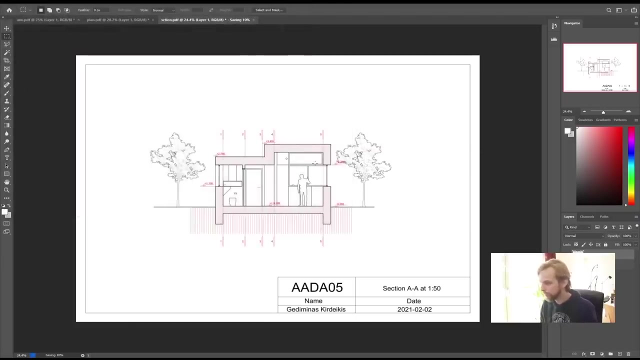 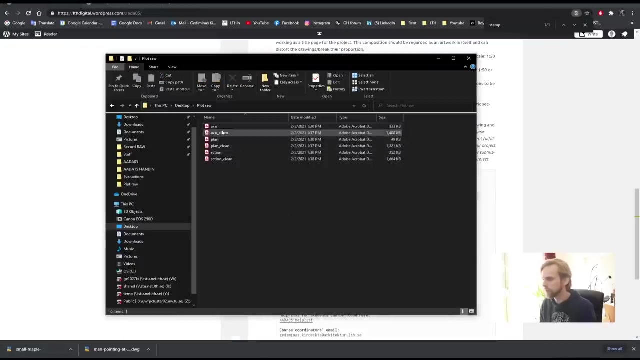 Clean- No layers, Save Section PDF Section: Clean: No layers, Save. OK, We are almost there. Last thing Is combining them. So you can either combine them with Adobe PDF By just kind of selecting. 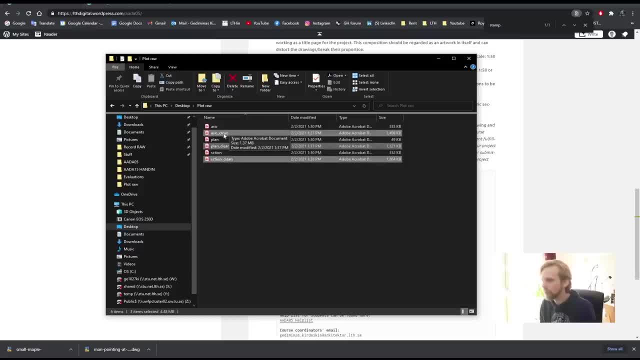 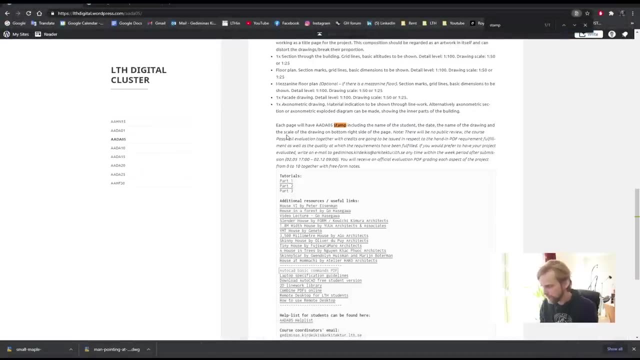 All three of them, Or Acrobat reader Selecting all three of them, Right clicking on them, And then you Combine files in Acrobat. So if you don't have that option, Right. If you don't have that option, Then you. 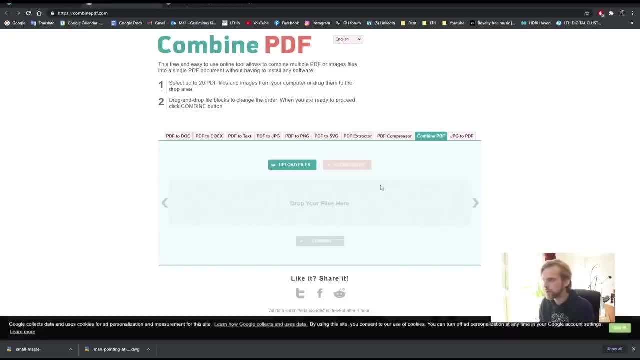 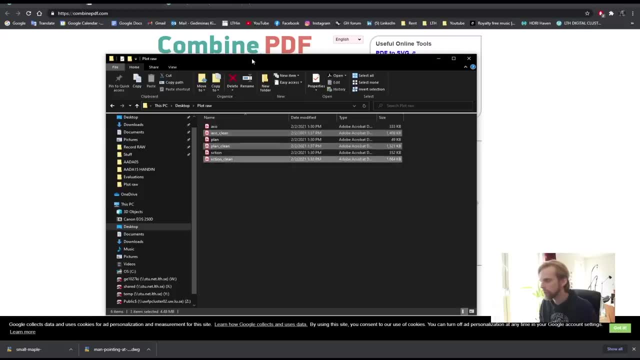 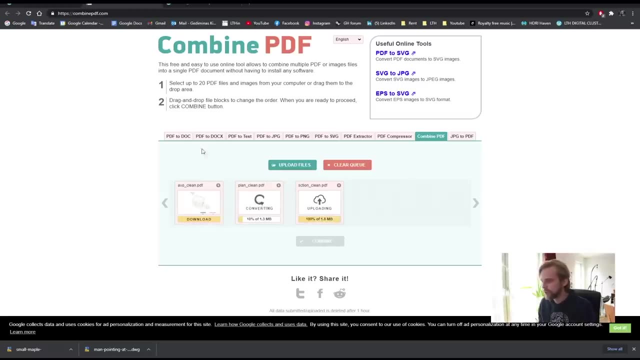 Then you need to use the website Combine PDFs online, Which is also super neat. Drop your files here, Exoplan Section. There we go, Drag and drop them in. It's uploading. Uploading. It's done, And now I can kind of arrange them. 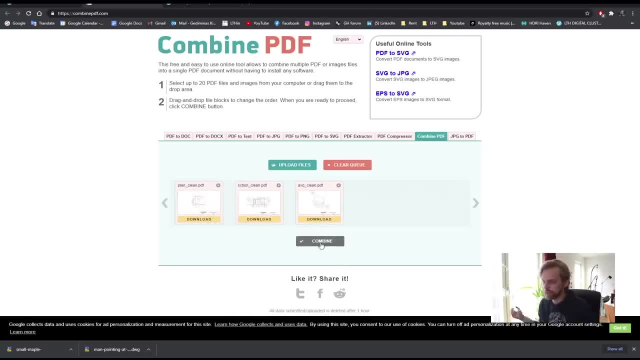 So first I want the plan, Then I want the section, Then I want the exo, And then I just click on combine And now it's downloaded Here. Join folder. My computer is just Not up to par today. Come on. 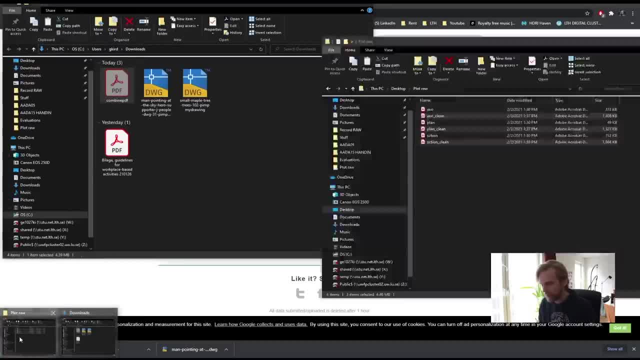 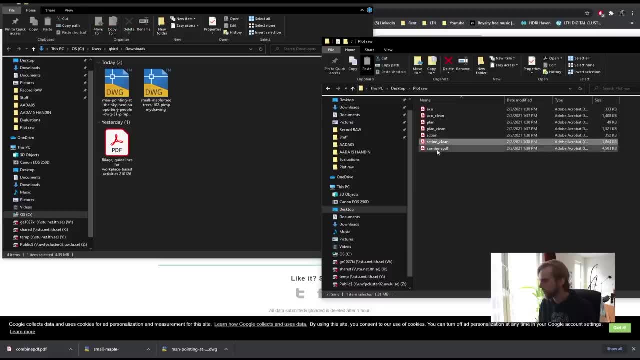 You can do it. It's just opening a folder. I have that And I will just add it To To the plot row for the folder Sure, And I'll say AADA05.. Kiridekis Gediminas. 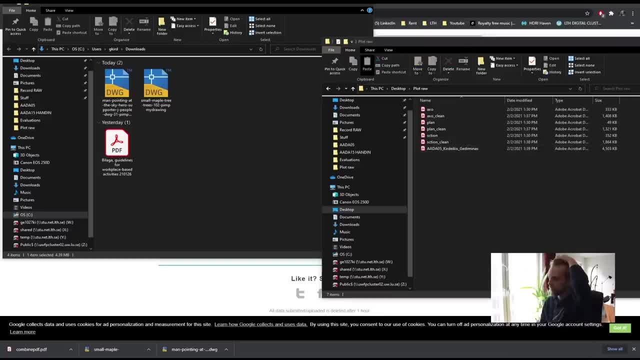 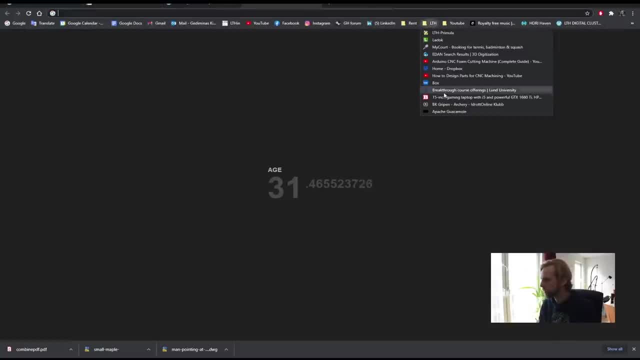 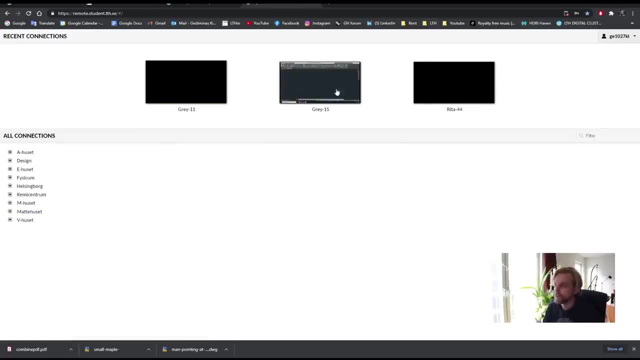 Right, Then I will. I can either email it to myself And use the. Use the. Use the- How is it called? Remote student desktop To login to one of the computers And open up the email from the, The computer in the school. 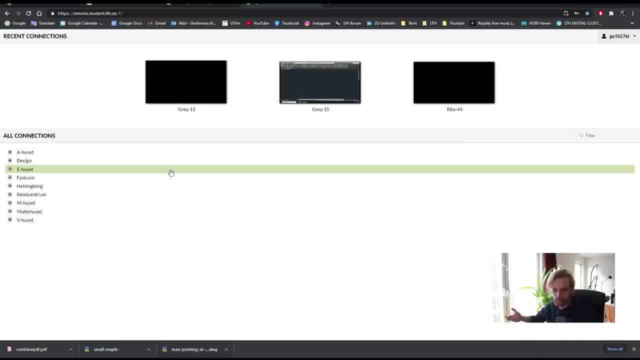 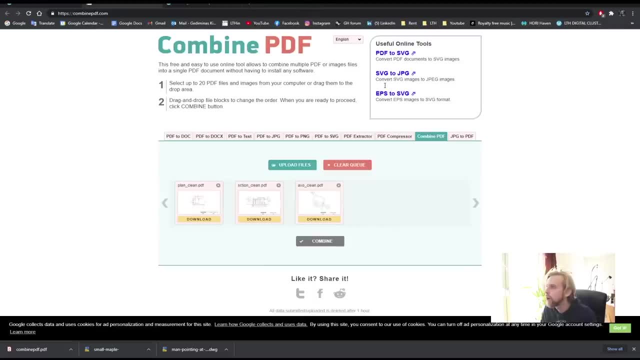 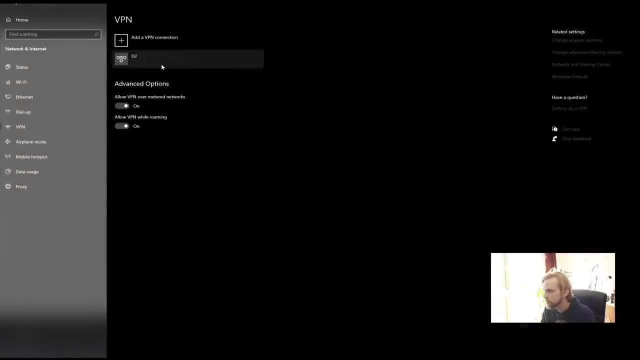 And upload it to the, To the server from there, Which is a viable solution And super easy to do, Or I can just simply. If you are a little bit more Technology Focused, I guess You can just connect To the computer.